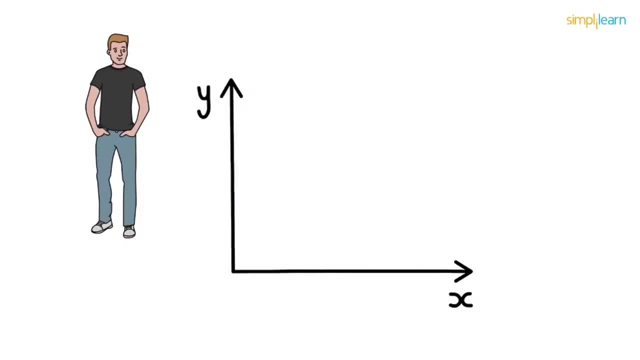 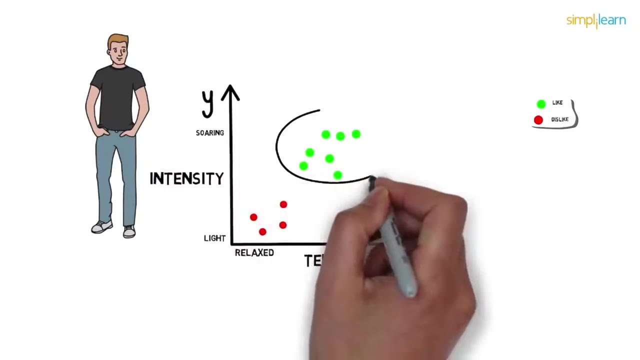 voice For simplicity, let's just use tempo and intensity. So here, tempo is on the x-axis, ranging from relaxed to fast, whereas intensity is on the y-axis, ranging from light to soaring. We see that Paul likes the song with fast. 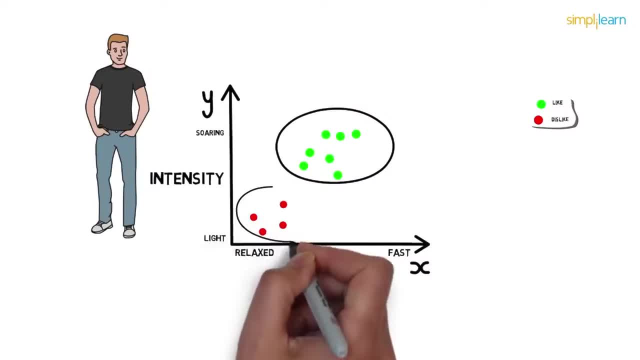 tempo and soaring intensity, while he dislikes the song with relaxed tempo and light intensity. So now we know Paul's choices. Let's say Paul listens to a new song. Let's name it as song A. Song A has fast tempo and a soaring intensity. 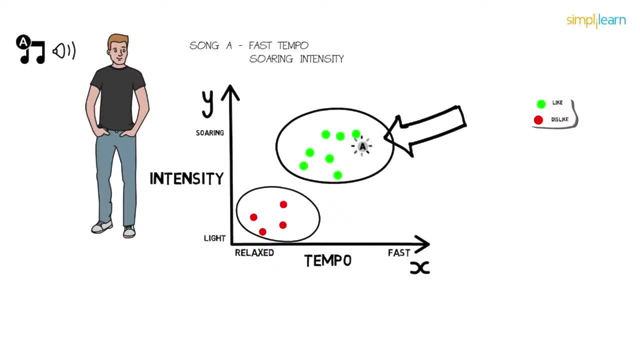 So it lies somewhere here. Looking at the data, can you guess whether Paul will like the song or not? Correct, So Paul likes this song. By looking at Paul's past choices, we were able to classify the unknown song very easily, Right? 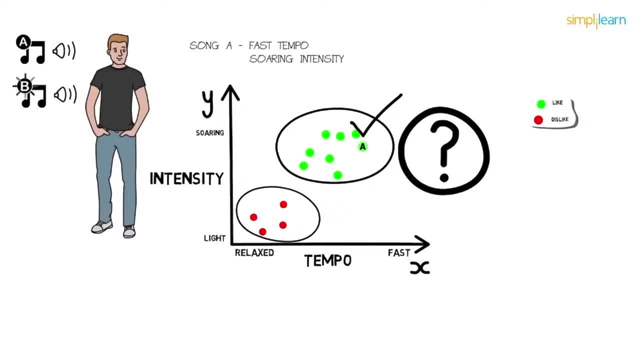 Let's say now Paul listens to a new song, Let's label it as song B. So song B lies somewhere here, with medium tempo and medium intensity, Neither relaxed nor fast, neither light nor soaring. Now can you guess whether Paul likes it or not? Not able to guess whether Paul will like, 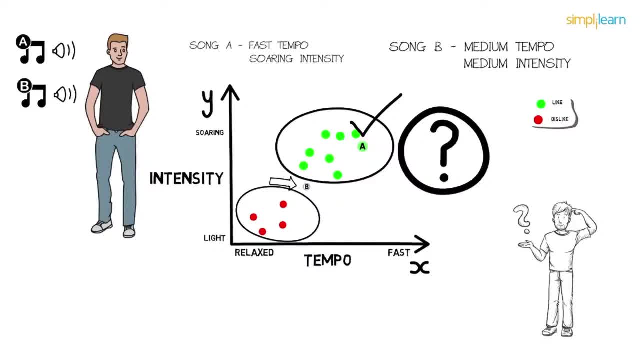 it or dislike it? Are the choices unclear? Correct, We could easily classify song A, But when the choice became complicated, as in the case of song B, yes, and that's where machine learning comes in. Let's see how. In the same example for song B, if we draw a circle around song B, we see that there. 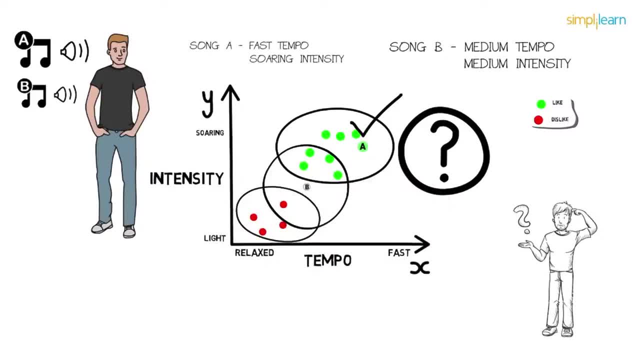 are 4 votes for like, whereas 1 vote for dislike. If we go for the majority votes, we can say that Paul will definitely like the song. That's all. This was a basic machine learning algorithm. also It's called k-nearest neighbors, So this is just a small example. in one of the 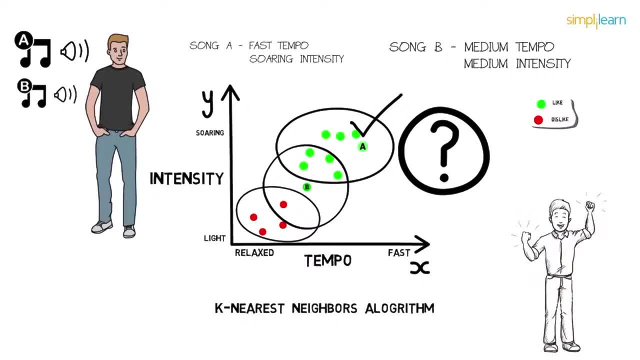 many machine learning algorithms Quite easy, right, Believe me it is. But what happens when the choices become complicated, as in the case of song B? That's when machine learning comes in. It learns the data, builds the prediction model, and when the new data 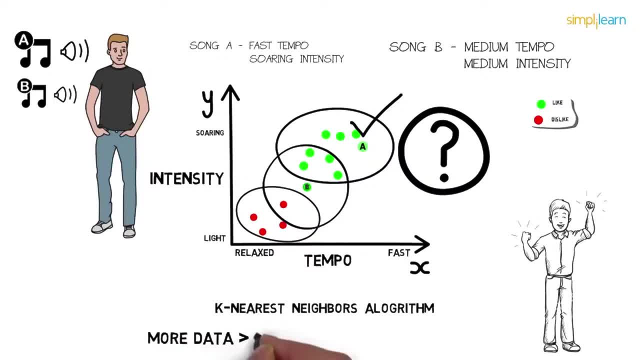 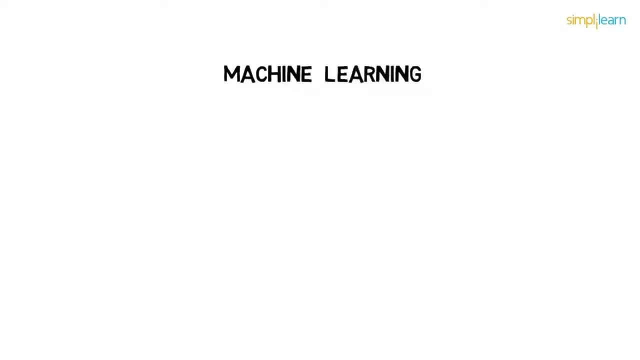 point comes in, it can easily predict for it. More the data, better the model, higher will be the accuracy. There are many ways in which the machine learns. It could be either supervised learning, unsupervised learning or reinforcement learning. Let's first quickly understand supervised learning. 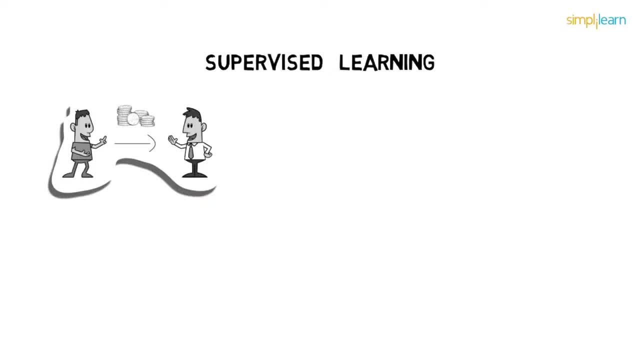 Suppose your friend gives you 1 million coins of 3 different currencies, say 1 rupee, 1 euro and 1 dirham. Each coin has different weights. For example, a coin of 1 rupee weighs 3 grams, 1 euro weighs 7 grams and 1 dirham weighs 4 grams. Your model will predict the. 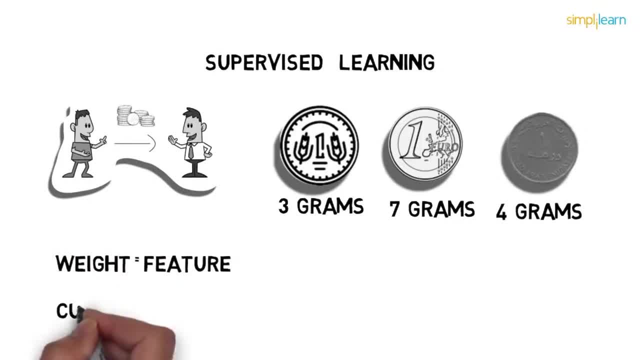 currency of the coin. Here your weight becomes the feature of coins, while currency becomes their label. When you feed this data to the machine learning model, it learns which feature is associated with which label. For example, it will learn that if a coin is of 3 grams. 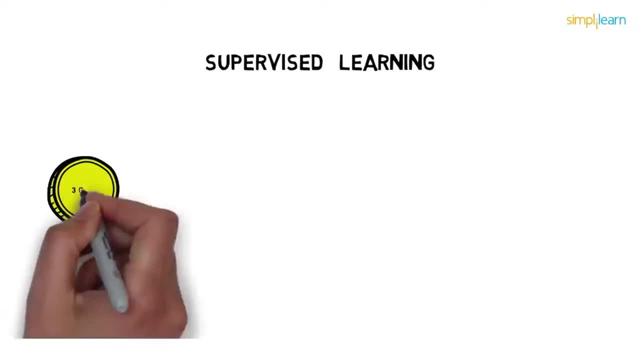 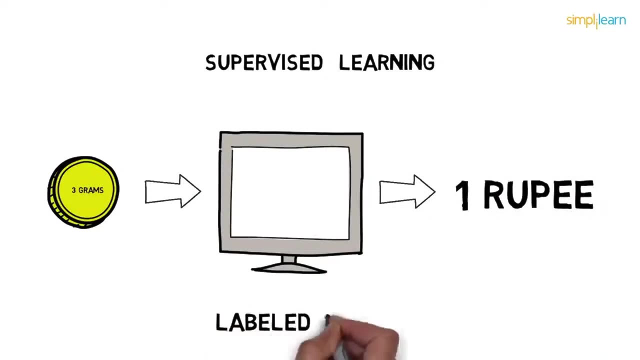 it will be a 1 rupee coin. Let's give a new coin to the machine. On the basis of the weight of the new coin, your model will predict the currency. Hence supervised learning uses labeled data to train the model. Here the machine knew the features. 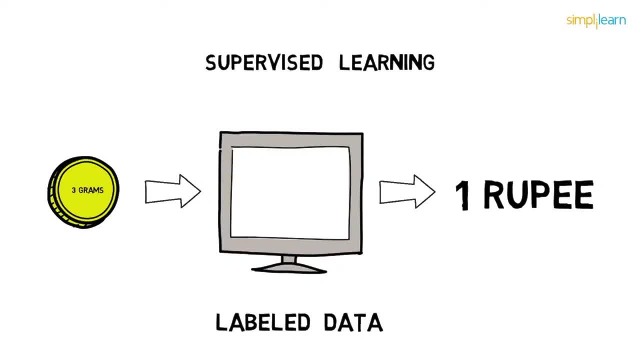 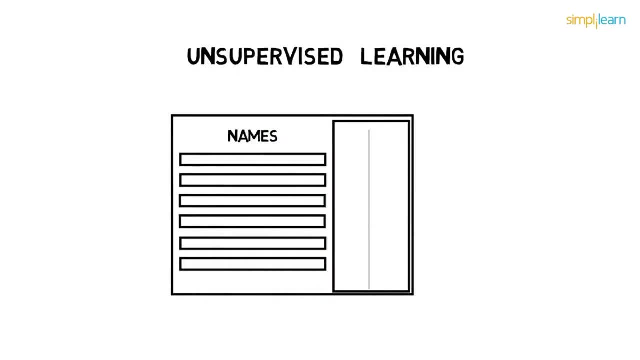 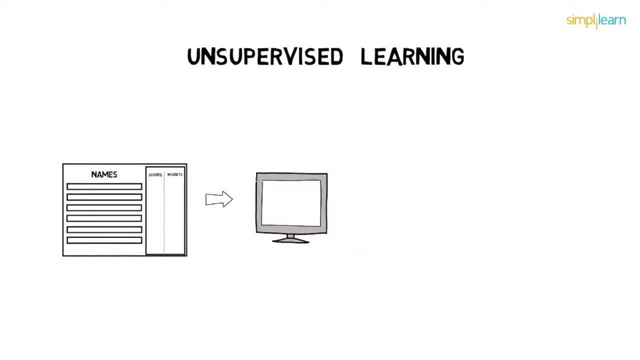 of the object and also the labels associated with those features. On this note, let's move to unsupervised learning and see the difference. Suppose you have the cricket data set of various players, with their respective scores and wickets taken. When we feed this data set to the machine, the machine identifies the pattern of player. 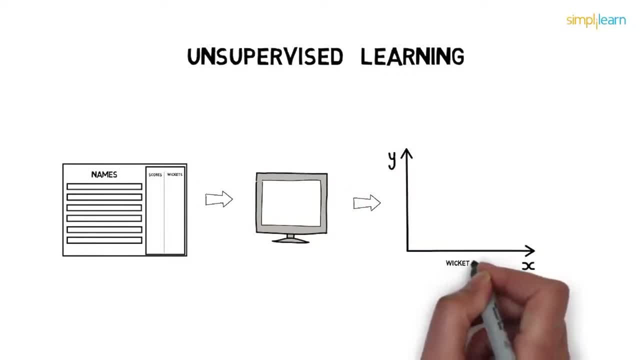 performance. So it plots this data with the respective wickets on the x-axis while runs on the y-axis. By looking at the data, you will clearly see that there are two clusters. The one cluster are the players who scored high runs and took less wickets, while the other cluster is of the players who scored less runs. 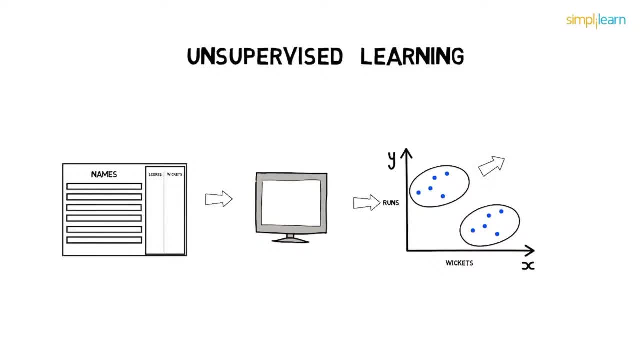 but took many wickets. so here we interpret these two clusters as batsmen and bowlers. the important point to note here is that there were no labels of batsmen and bowlers. hence the learning with unlabeled data is unsupervised learning. so we saw supervised learning where the data was labeled. 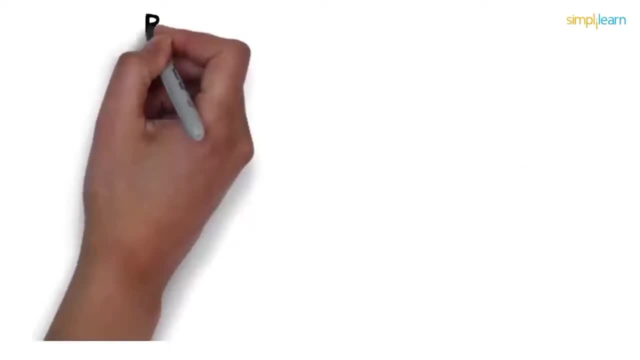 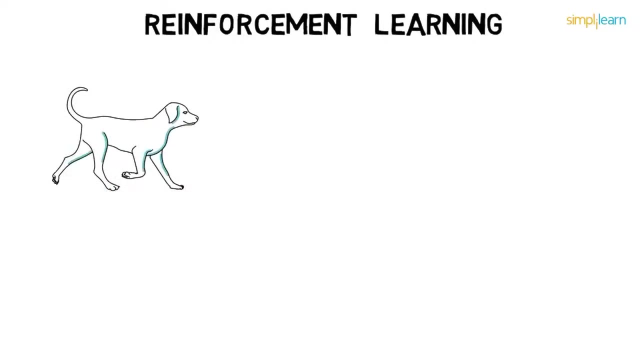 and the unsupervised learning, where the data was unlabeled. and then there is reinforcement learning, which is a reward-based learning, or we can say that it works on the principle of feedback. here, let's say, you provide the system with an image of a dog and ask it to identify it. the system 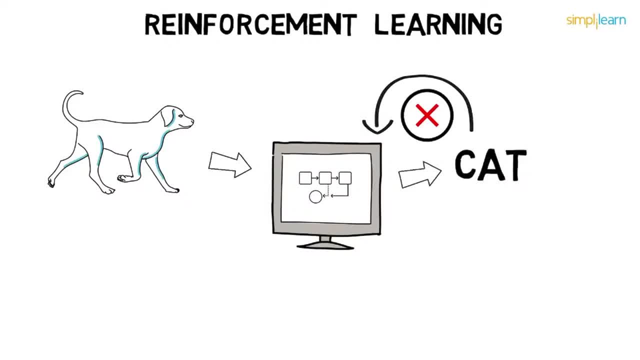 identifies it as a cat. so you give a negative feedback to the machine, saying that it's a dog's image. the machine will learn from the feedback and finally, if it comes across any other image of a dog, it will be able to classify it correctly. that is reinforcement learning to generalize. 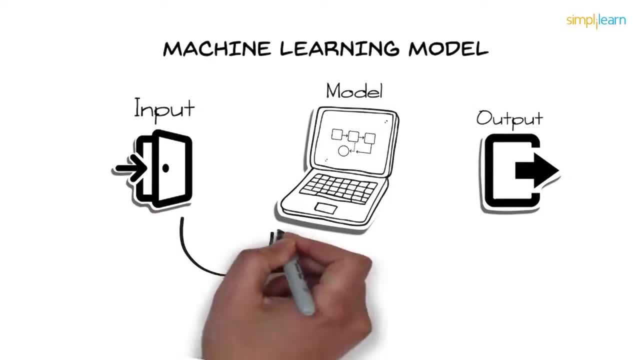 machine learning model. let's see a flowchart. input is given to a machine learning model, which then gives us a flowchart and then gives us a flowchart which gives us a flowchart. which gives us a gives the output according to the algorithm applied. if it's right, we take. 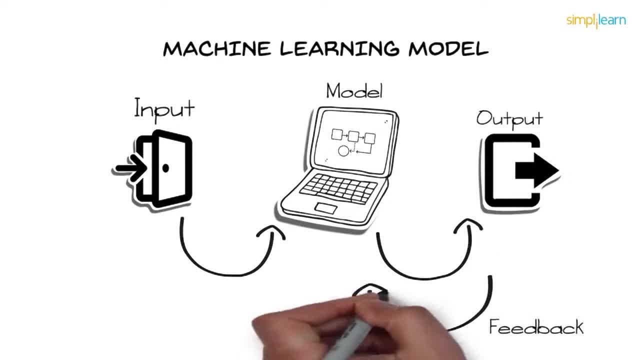 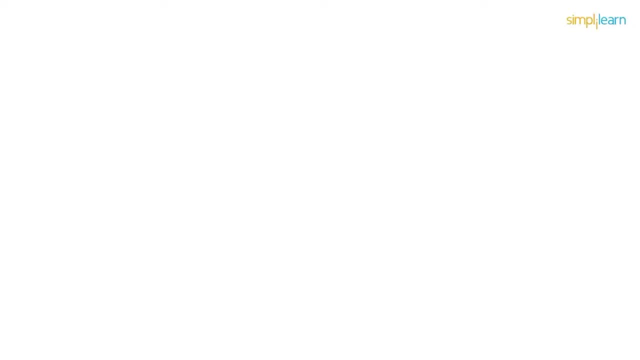 the output as a final result. else we provide feedback to the training model and ask it to predict until it learns. I hope you've understood supervised and unsupervised learning. so let's have a quick quiz. you have to determine whether the given scenarios uses supervised or unsupervised learning, simple right. 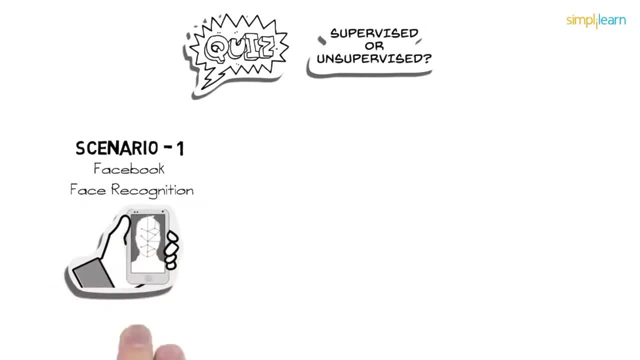 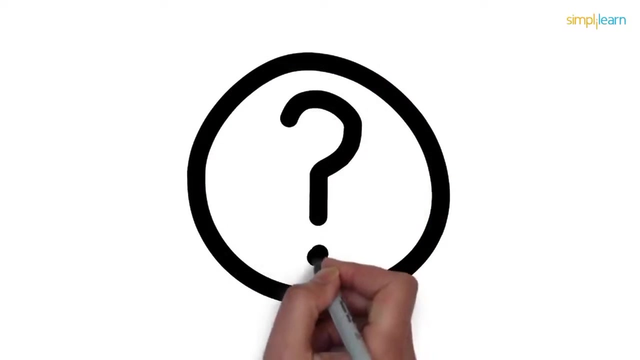 scenario one: Facebook recognizes your friend in a picture from an album of tagged photographs. scenario to: Netflix recommends new movies based on someone's past movie choices. scenario 3: analyzing bank data for suspicious transactions and flagging fraud transactions. think wisely and comment below your answers. moving on, don't you sometimes wonder how is machine learning possible in today's 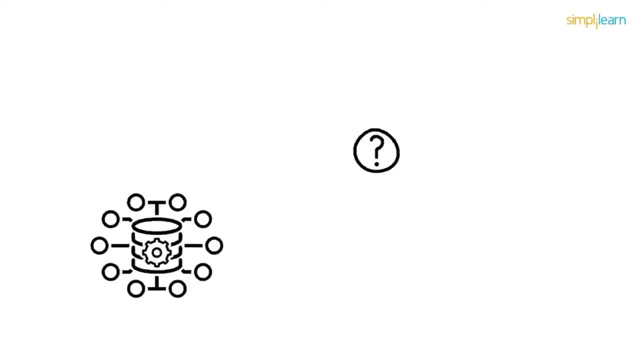 era. well, that's because today we have humongous data available. everybody's online, either making a transaction or just surfing the internet, or just using the internet to make a transaction or just surfing the internet or just surfing the internet or just surfing the internet online, either making a transaction or just surfing the internet or just surfing. 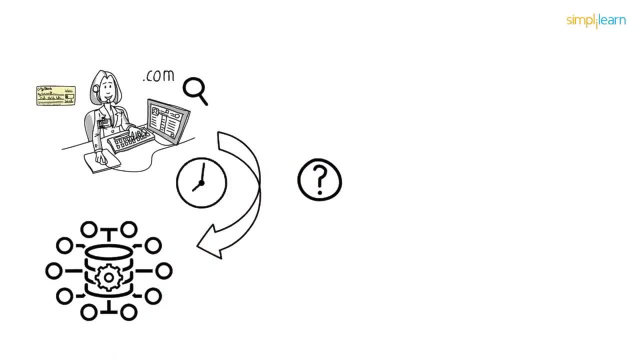 the internet or just surfing the internet, and that's generating a huge the internet. and that's generating a huge the internet and that's generating a huge amount of data every minute. and that amount of data every minute, and that amount of data every minute, and that data, my friend, is the key to analysis. 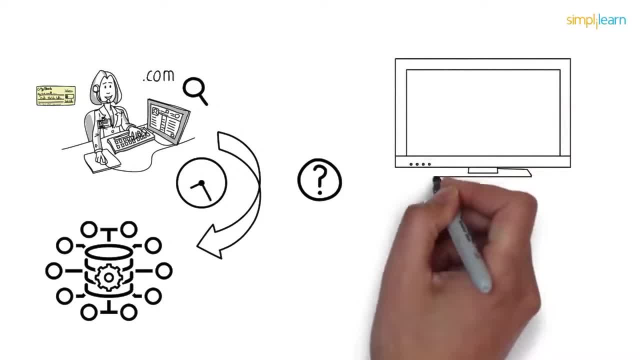 data, my friend, is the key to analysis. data, my friend, is the key to analysis also. the memory handling capabilities of also the memory handling capabilities of also the memory handling capabilities of computers have largely increased, which computers have largely increased, which computers have largely increased which helps them to process such a huge amount. 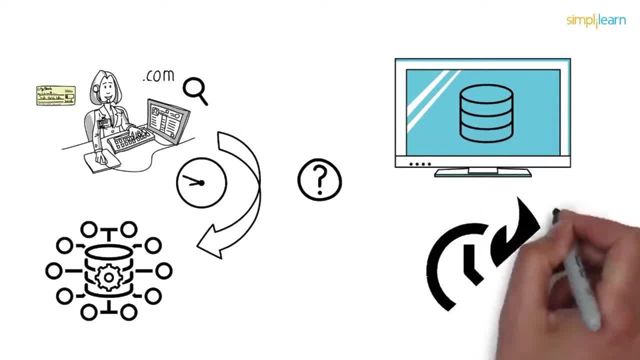 helps them to process such a huge amount. helps them to process such a huge amount of data at hand without any delay. and yes, of data at hand without any delay. and yes, of data at hand without any delay. and yes, computers now have great computational. computers now have great computational. 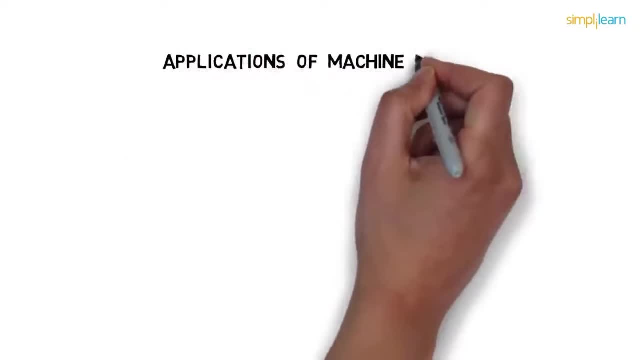 computers now have great computational powers, so there are a lot of powers. so there are a lot of powers, so there are a lot of applications of machine learning out applications of machine learning, out applications of machine learning out there, to name a few. machine learning is there. to name a few: machine learning is. 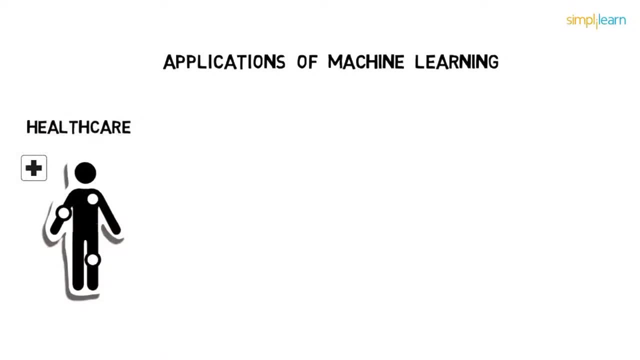 there. to name a few, machine learning is used in healthcare, where diagnostics are used in healthcare, where diagnostics are used in healthcare, where diagnostics are predicted for doctors. review the predicted for doctors. review the predicted for doctors. review the sentiment analysis that the tech giants sentiment analysis that the tech giants. 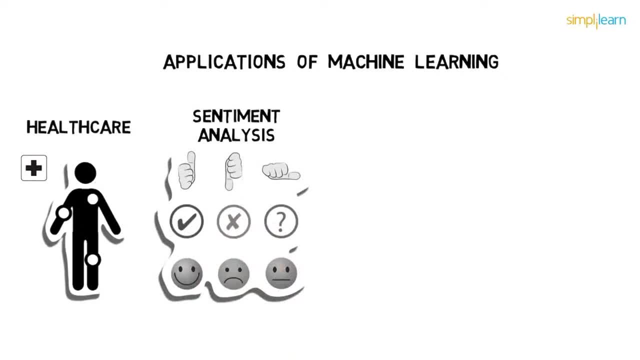 sentiment analysis that the tech giants are doing on social media is another. are doing on social media is another. are doing on social media is another. interesting application of machine. interesting application of machine. interesting application of machine learning: fraud detection in the finance. learning, fraud detection in the finance. 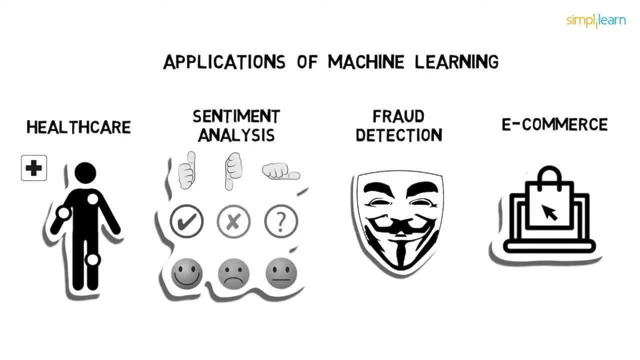 learning, fraud detection in the finance sector, and also to predict customer sector, and also to predict customer sector, and also to predict customer churn in the e-commerce sector. while churn in the e-commerce sector, while churn in the e-commerce sector. while booking a gap you must have encountered. 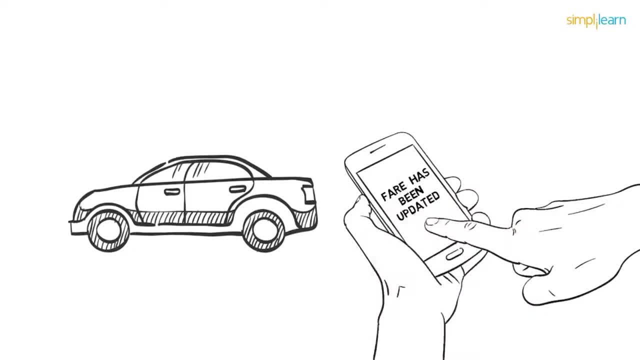 booking a gap. you must have encountered booking a gap. you must have encountered surge pricing, often where it says the surge pricing. often where it says the surge pricing. often where it says the fair of your trip has been updated. fair of your trip has been updated. fair of your trip has been updated, continue booking. yes, please, I'm getting. 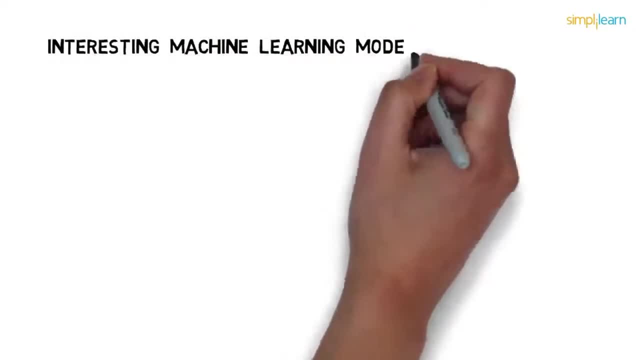 continue booking. yes, please, I'm getting continue booking. yes, please, I'm getting late for office. well, that's an late for office. well, that's an late for office. well, that's an interesting machine learning model, which interesting machine learning model, which interesting machine learning model which is used by global taxi giant uber, and. 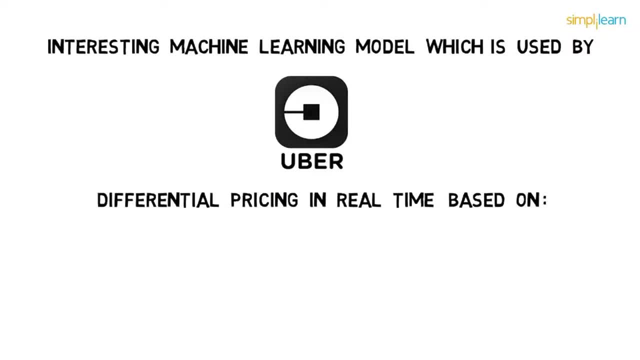 is used by global taxi giant uber, and is used by global taxi giant uber and others where they have differential others, where they have differential others, where they have differential pricing in real-time based on demand. the pricing in real-time based on demand. the pricing in real-time based on demand. the number of cars available. bad weather. 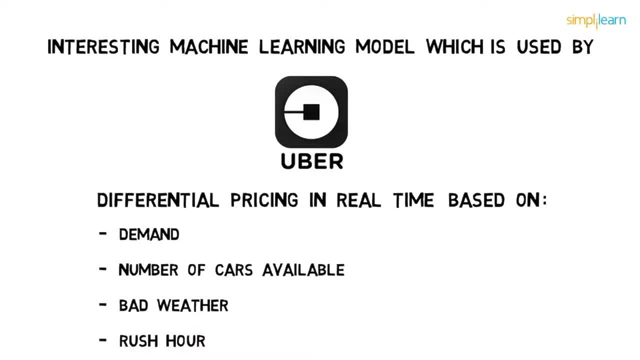 number of cars available, bad weather. number of cars available, bad weather, rush hour, etc. so they use the surge rush hour etc. so they use the surge rush hour, etc. so they use the surge pricing model to ensure that those who pricing model, to ensure that those who pricing model, to ensure that those who need a cab can get one. also it uses 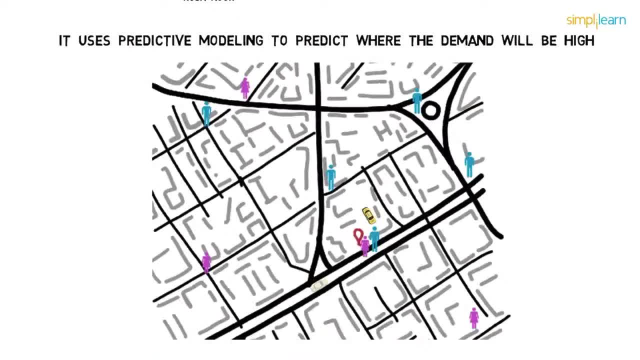 need a cab, can get one also. it uses need a cab, can get one also. it uses predictive modeling to predict where the predictive modeling to predict where the predictive modeling to predict where the demand will be high with a goal that demand will be high, with a goal that. 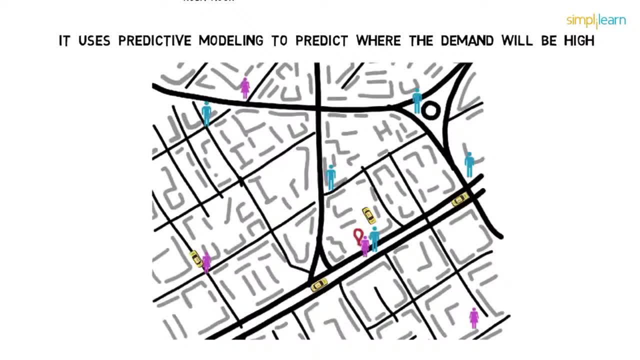 demand will be high, with a goal that drivers can take care of the demand and drivers can take care of the demand and drivers can take care of the demand and surge pricing can be minimized. great, hey, surge pricing can be minimized. great, hey, surge pricing can be minimized, great, hey, Siri, can you remind me to book a cab at? 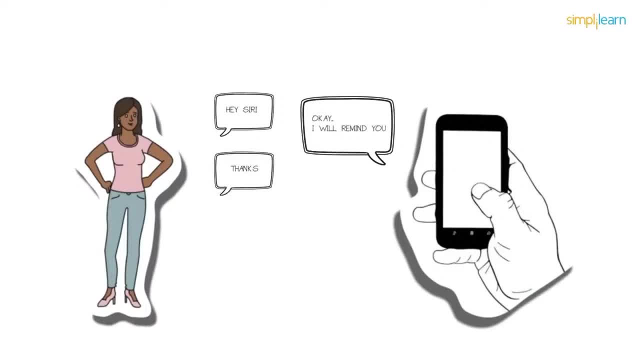 Siri. can you remind me to book a cab at Siri? can you remind me to book a cab at 6 pm today? okay, I'll remind you thanks. 6 pm today. okay, I'll remind you thanks. 6 pm today. okay, I'll remind you thanks, no problem. comment below some. 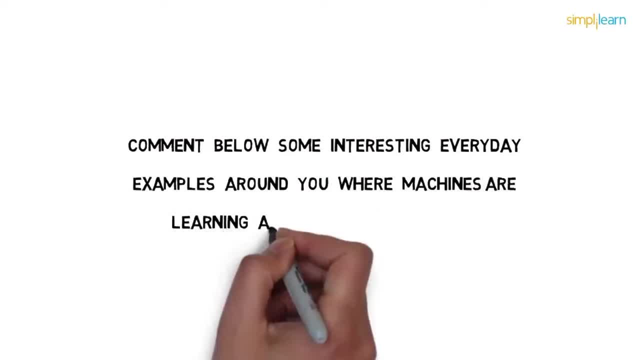 no problem comment below some. no problem comment below some interesting everyday examples around you. interesting everyday examples around you, interesting everyday examples around you where machines are learning and doing, where machines are learning and doing, where machines are learning and doing amazing jobs. hi guys, this is a picture. 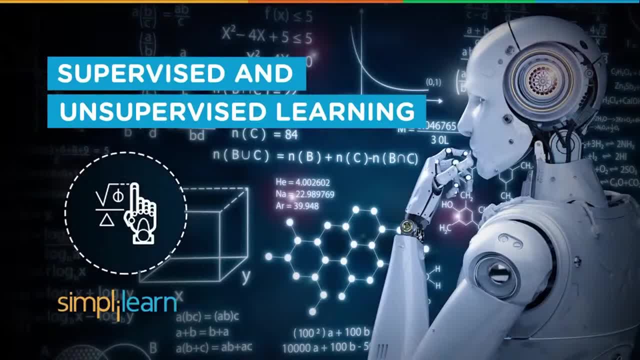 amazing jobs, hi guys. this is a picture. amazing jobs, hi guys. this is a picture from simply learn, and we are going to from simply learn, and we are going to from simply learn, and we are going to talk about the two types of machine. talk about the two types of machine. 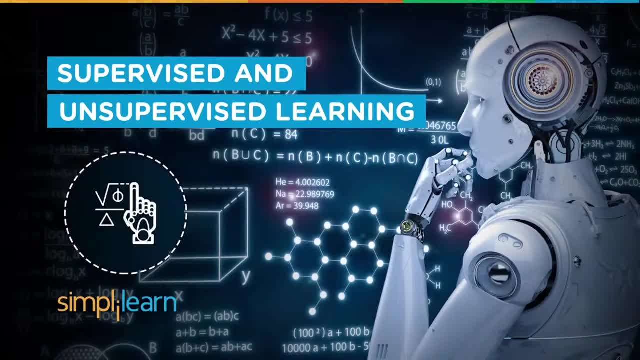 talk about the two types of machine learning: supervised and unsupervised learning supervised and unsupervised learning supervised and unsupervised, learning their types and applications, but learning their types and applications. but learning their types and applications, but before we talk about them, let's. before we talk about them, let's. 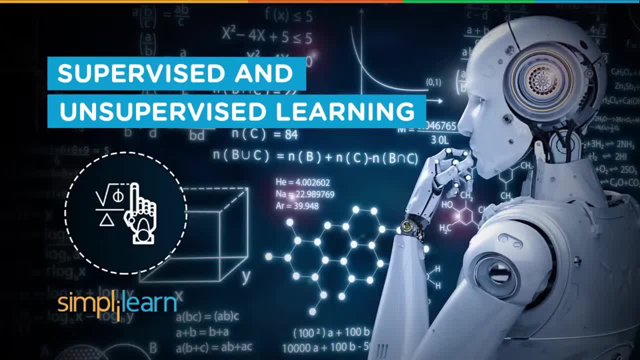 before we talk about them. let's quickly understand what is machine learning. quickly understand what is machine learning. quickly understand what is machine learning these days. applications use these days. applications use these days, applications use artificial intelligence in machine learning to artificial intelligence in machine learning, to artificial intelligence in machine learning to optimize speech recognition. I 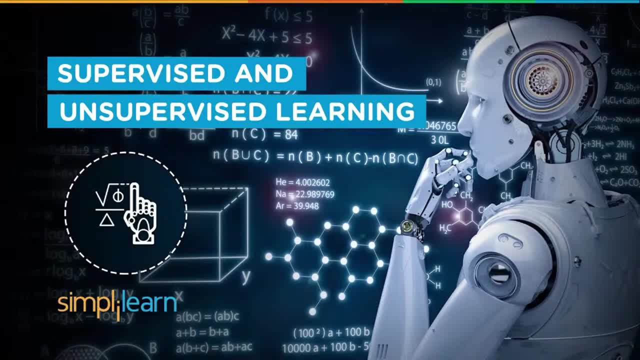 optimize speech recognition. I optimize speech recognition. I usually are silly things I want to know. usually are silly things I want to know. usually are silly things I want to know, like hey Siri, how far is the nearest? like hey Siri, how far is the nearest? like hey Siri, how far is the nearest subway? so whenever we ask something to 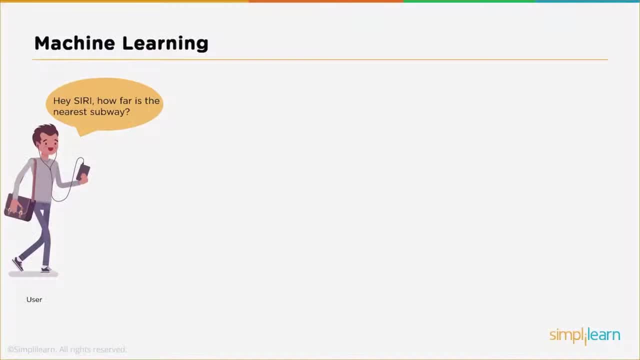 subway. so whenever we ask something to subway, so whenever we ask something to Siri, a powerful speech recognition kicks Siri. a powerful speech recognition kicks Siri. a powerful speech recognition kicks off and converts the audio into its off, and converts the audio into its off and converts the audio into its corresponding textual form, which is then. 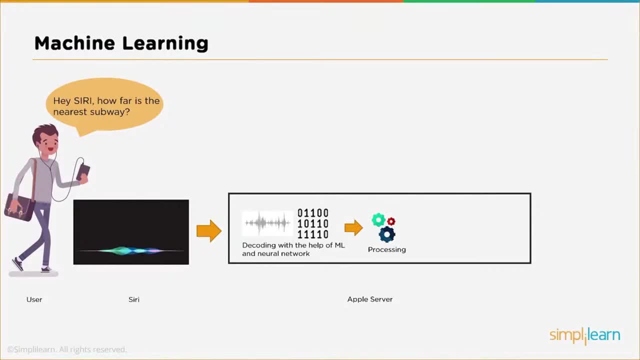 corresponding textual form, which is then corresponding textual form, which is then sent to the Apple servers for further, sent to the Apple servers for further, sent to the Apple servers for further processing. then neural language processing, then neural language processing, then neural language processing algorithms are run to. processing algorithms are run to. 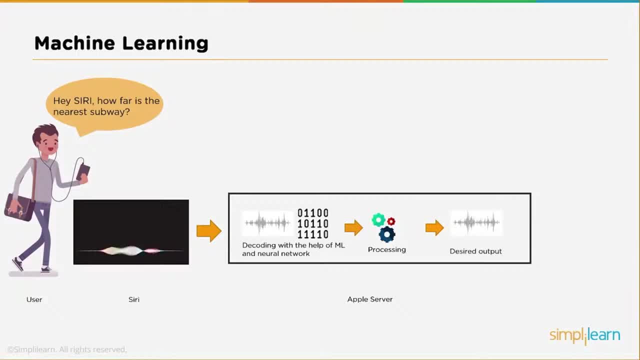 processing algorithms are run to understand the users intent, and then understand the users intent, and then understand the users intent, and then, finally, Siri tells you the answer. well, finally, Siri tells you the answer. well, finally, Siri tells you the answer. well, this is what machine learning is all. 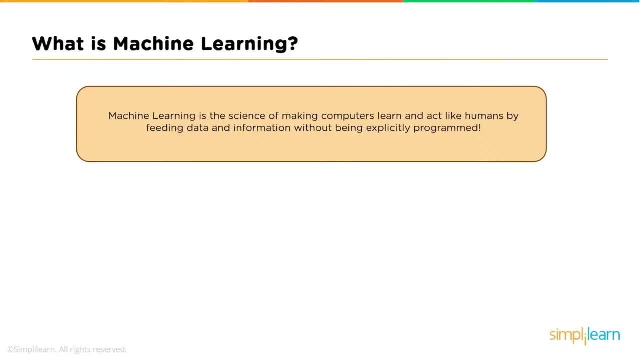 this is what machine learning is all. this is what machine learning is all about: making the machines learn and act. about making the machines learn and act. about making the machines learn and act like humans by feeding them with data like humans, by feeding them with data like humans, by feeding them with data and information without being explicitly 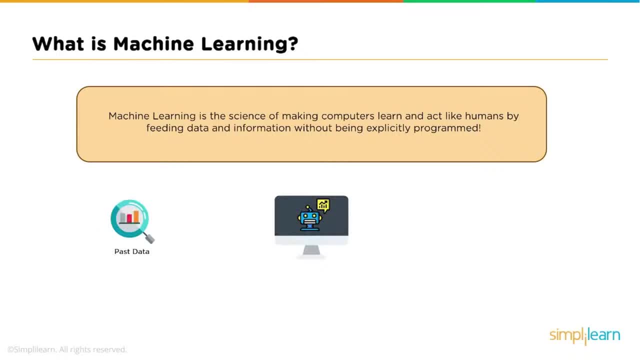 and information without being explicitly and information without being explicitly programmed, as we saw in the previous programmed, as we saw in the previous programmed, as we saw in the previous example, when the data comes in machines, example, when the data comes in machines- example, when the data comes in machines- immediately starts analyzing the data. 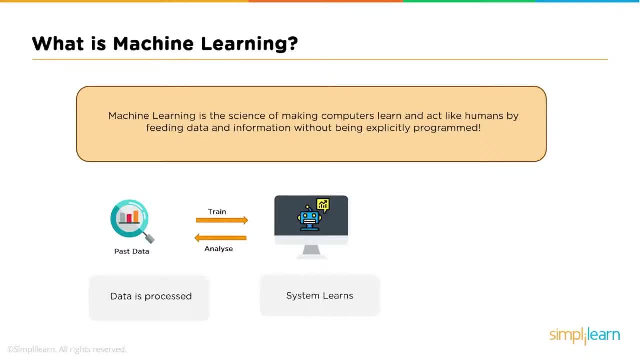 immediately starts analyzing the data, immediately starts analyzing the data and eventually gets trained on it. and and eventually gets trained on it, and and eventually gets trained on it and learns it now when a new data point. learns it now when a new data point. learns it now when a new data point comes in: machine accurately makes. 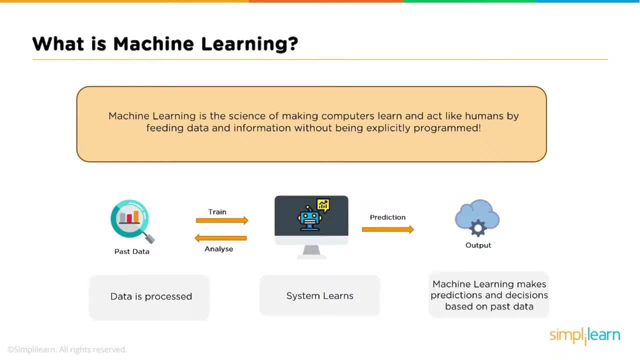 comes in machine accurately makes- comes in machine accurately makes prediction and decisions based on the prediction and decisions based on the prediction and decisions based on the past data. now that you know what is past data, now that you know what is past data, now that you know what is machine learning, let's talk about 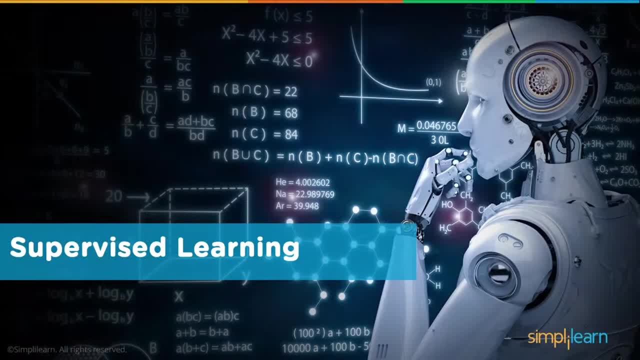 machine learning. let's talk about machine learning. let's talk about supervised and unsupervised learning. supervised and unsupervised learning. supervised and unsupervised learning. supervised learning, as the name suggests. supervised learning, as the name suggests. supervised learning, as the name suggests, works under supervision. that is it's. 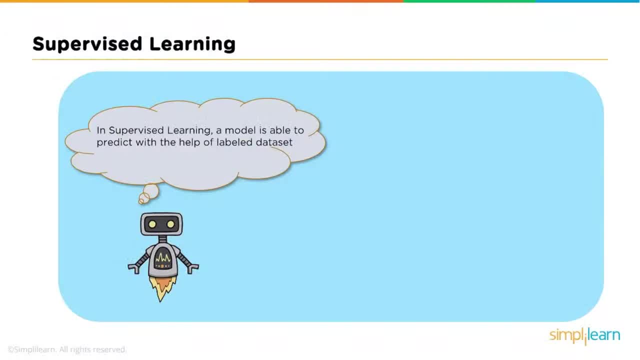 works under supervision. that is it's works under supervision. that is it's learning in which machine is trained. learning in which machine is trained. learning in which machine is trained with data which is fell labeled, and then with data which is fell labeled, and then with data which is fell labeled, and then predicts with the help of the label data. 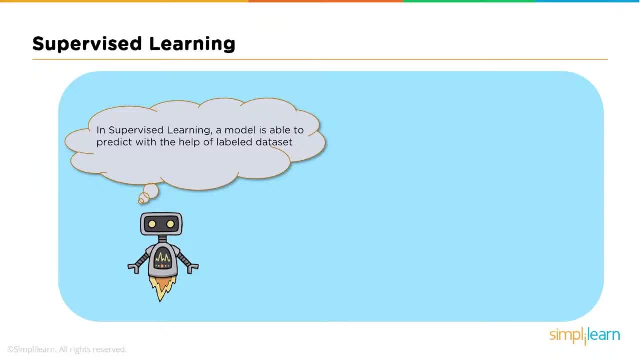 predicts with the help of the label data, predicts with the help of the label data set. but what is a label data set data set? but what is a label data set data set? but what is a label data set data for which you already know the target, for which you already know the target? 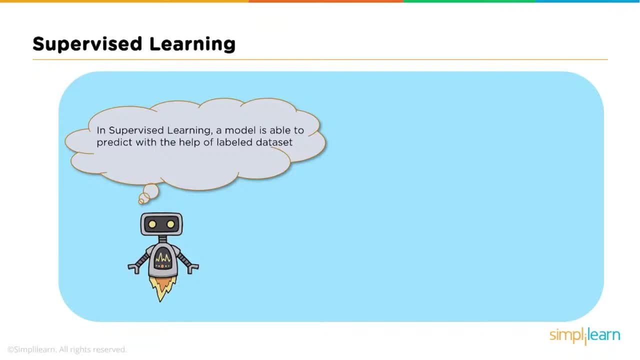 for which you already know the target answer is called a label data. like I answer is called a label data. like I answer is called a label data. like I. show you an image and tell you that it's. show you an image and tell you that it's. 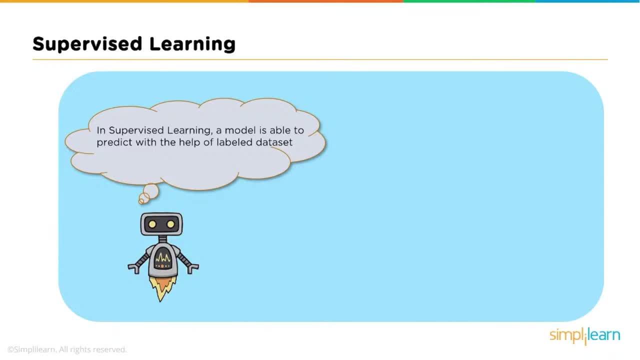 show you an image and tell you that it's a dog, then it's a label data, while if I a dog, then it's a label data, while if I a dog, then it's a label data, while if I show you an image without telling you, show you an image without telling you. 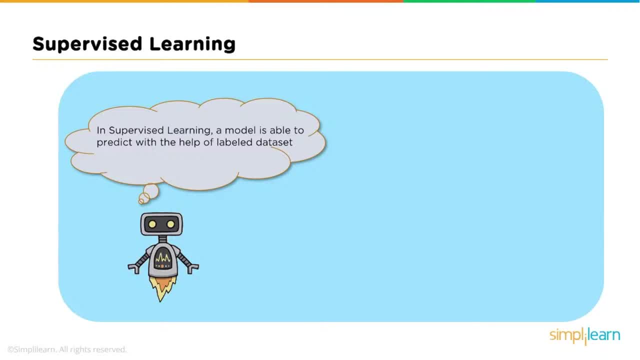 show you an image without telling you what exactly it is? then it's an unlabeled. what exactly it is? then it's an unlabeled what exactly it is? then it's an unlabeled data. now let's see we have images. which data? now let's see we have images which. 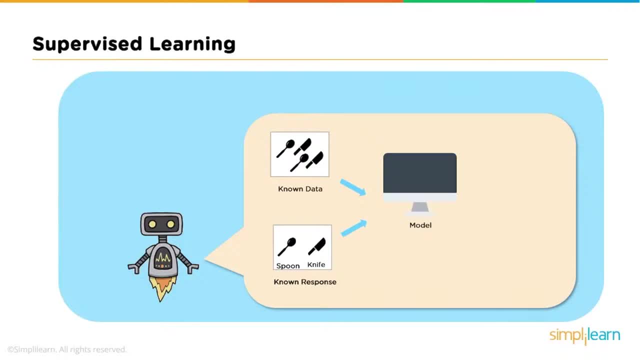 data. now let's see. we have images which are labeled as spoon or knife. we then are labeled as spoon or knife. we then are labeled as spoon or knife. we then feed it to the machine which analyzes, feed it to the machine which analyzes, feed it to the machine which analyzes and learns the association of these. 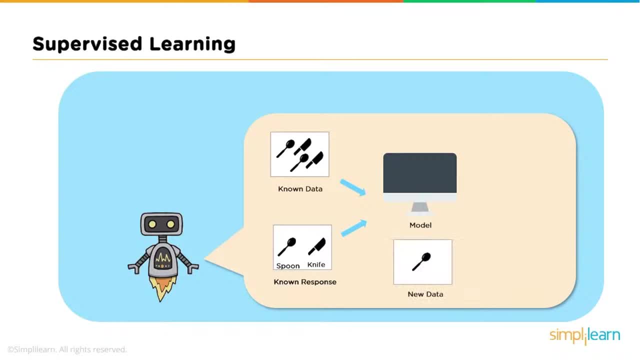 and learns the association of these and learns the association of these images with its labels based on its images, with its labels based on its images, with its labels based on its features, such as shape size, sharpness, features such as shape size, sharpness, features such as shape size, sharpness, etc. now there are new images fed to the 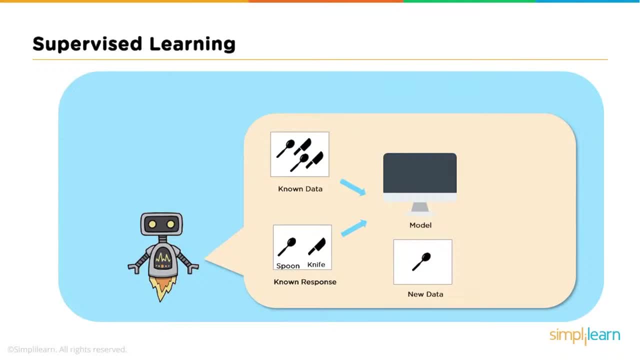 etc. now there are new images fed to the, etc. now there are new images fed to the machine without any label, with the help machine, without any label, with the help machine, without any label, with the help of the past data the machine is able to, of the past data the machine is able to. 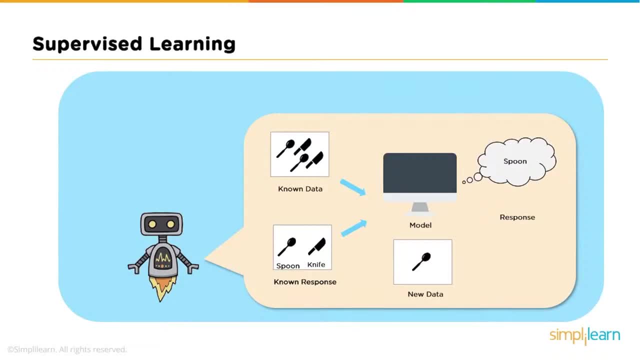 of the past data, the machine is able to predict accurately and tell that it's a predict accurately, and tell that it's a predict accurately and tell that it's a spoon. hence, in supervised machine spoon, hence in supervised machine spoon, hence in supervised machine learning, the algorithm teaches the model. 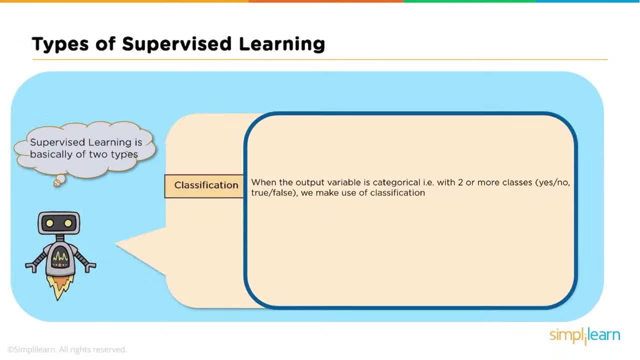 learning. the algorithm teaches the model learning. the algorithm teaches the model to learn from the labeled example. that, to learn from the labeled example. that. to learn from the labeled example that we provide, so supervised learning can be. we provide, so supervised learning can be. we provide, so supervised learning can be further divided into classification and 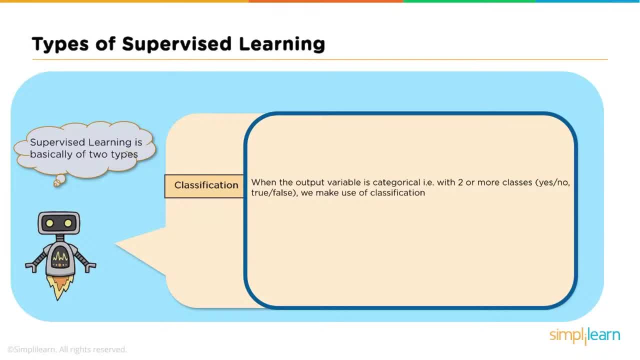 further divided into classification and further divided into classification and regression. it is a classification problem. regression it is a classification problem. regression it is a classification problem. variable is a real or continuous value. variable is a real or continuous value. variable is a real or continuous value. for example, salary based on work. 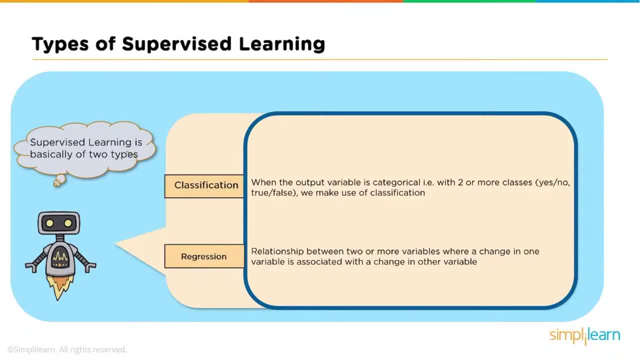 for example, salary based on work. for example, salary based on work experience, weight based on height. so it experience weight based on height. so it experience weight based on height. so it creates a predictive model showing trends, creates a predictive model showing trends, creates a predictive model showing trends and data. so now, if I say, will I get a? 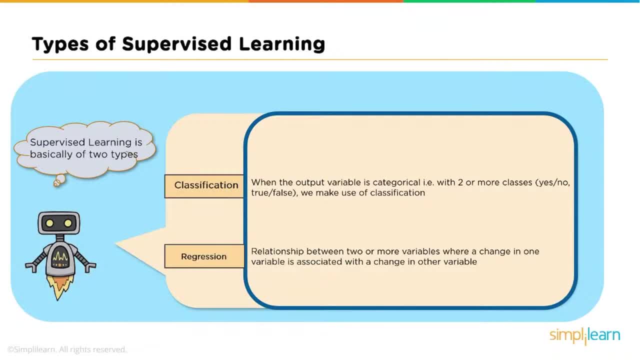 and data. so now, if I say, will I get a and data. so now if I say will I get a salary raise or not, that's classification salary raise or not, that's classification, salary raise or not, that's classification. but if I say how much salary raise, will I? 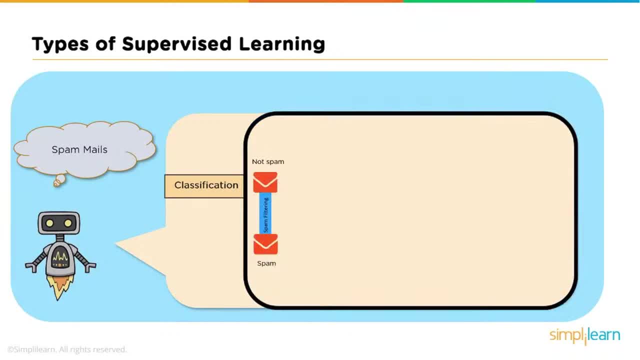 but if I say how much salary raise, will I? but if I say how much salary raise, will I get that is regression now. let's get. that is regression now. let's get. that is regression now. let's look at what it looks like this is done. look at what it looks like this is done. 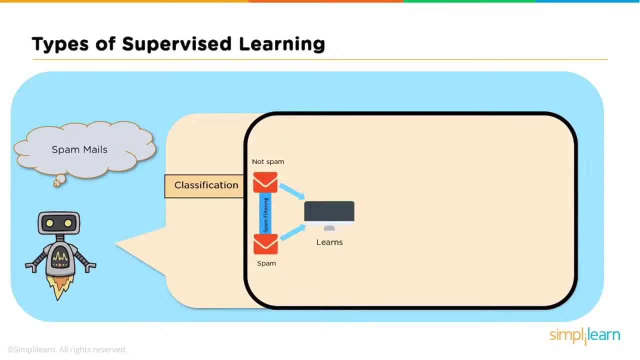 look at what it looks like. this is done based on a lot of spam filters, like based on a lot of spam filters, like based on a lot of spam filters like firstly reviewing the content of the. firstly reviewing the content of the. firstly reviewing the content of the email, then review the email header, and. 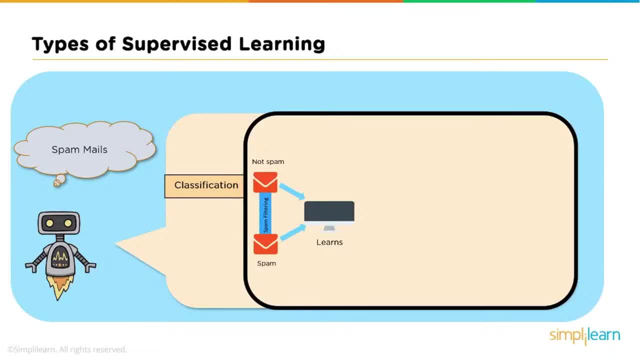 email, then review the email header and email. then review the email header and search if it contains any falsified search. if it contains any falsified search. if it contains any falsified information. this is done based on some information. this is done based on some information. this is done based on some keywords like free lottery price claim. 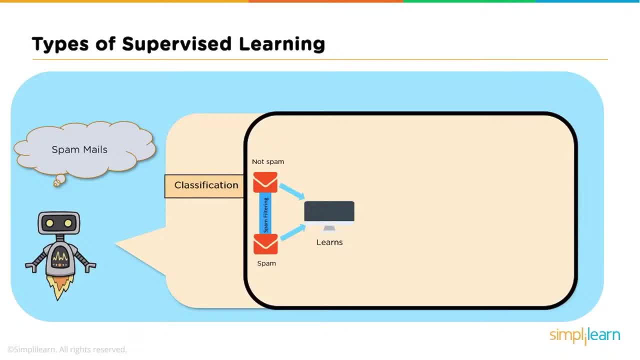 keywords like free lottery price claim. keywords like free lottery price claim, etc. then general blacklist filters to: etc. then general blacklist filters to etc. then general blacklist filters to stop emails that come from already. stop emails that come from already. stop emails that come from already blacklisted known spammers and etc. so 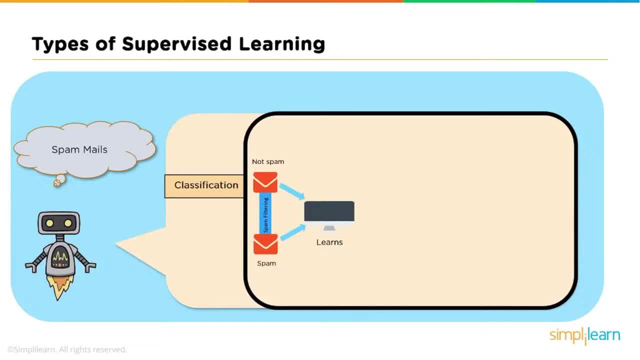 blacklisted, known spammers and etc. so blacklisted, known spammers and etc. so all these filters scores the email which all these filters scores, the email which all these filters scores, the email which is known as spam score. the lower the is known as spam score, the lower the. 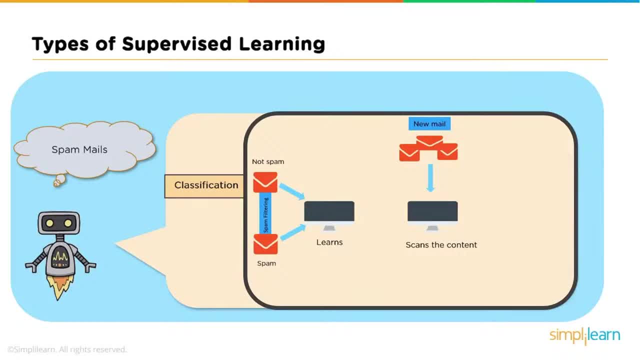 is known as spam score. the lower the total spam score of the email. it is more total spam score of the email. it is more total spam score of the email. it is more likely that the email will land in. likely that the email will land in. likely that the email will land in subscribers in boxes. so, based on the 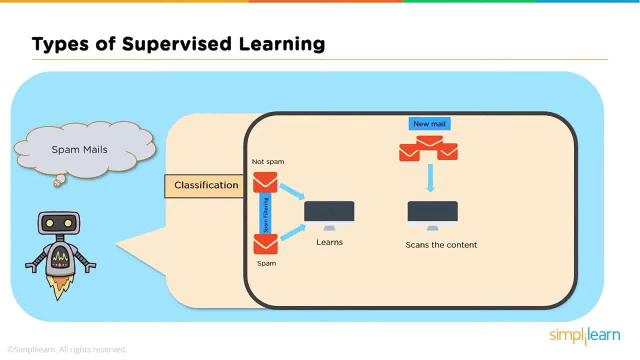 subscribers in boxes. so based on the subscribers in boxes. so based on the content labels and spam score of the new content labels and spam score of the new content labels and spam score of the new incoming mail. the algorithm decides incoming mail. the algorithm decides incoming mail. the algorithm decides whether it should land in inbox or the. 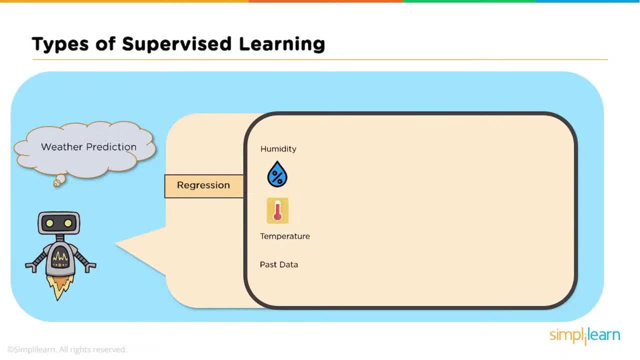 whether it should land in inbox or the, whether it should land in inbox or the spam folder. now let's quickly understand spam folder. now. let's quickly understand spam folder. now. let's quickly understand regression. so let's say we have two regression. so let's say we have two. 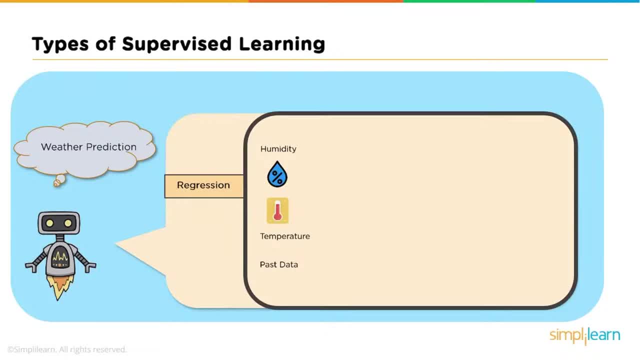 regression. so let's say we have two variables, that is, temperature and variables. that is temperature and variables, that is temperature and humidity. where temperature is the humidity, where temperature is the humidity, where temperature is the independent variable and humidity is the independent variable and humidity is the independent variable and humidity is the dependent variable, such that, as the 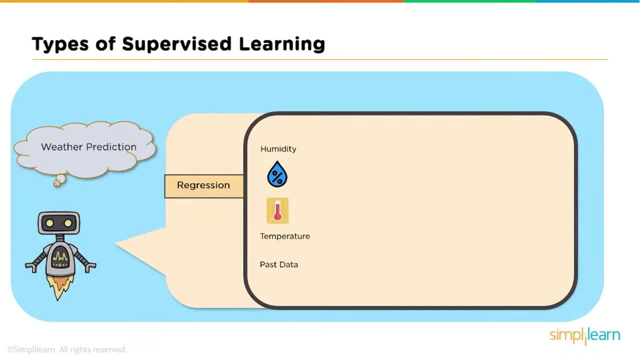 dependent variable, such that, as the dependent variable, such that, as the temperature increases, humidity decreases, temperature increases, humidity decreases, temperature increases, humidity decreases. hence they're correlated when we feed, hence they're correlated when we feed. hence they're correlated. when we feed this data to a regression model, it will 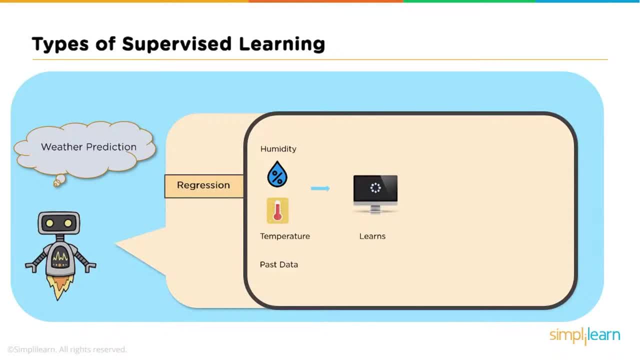 this data to a regression model. it will this data to a regression model. it will understand the relationship between. understand the relationship between understand the relationship between these two variables and how one variable, these two variables and how one variable, these two variables and how one variable depends on the other. after the machine. 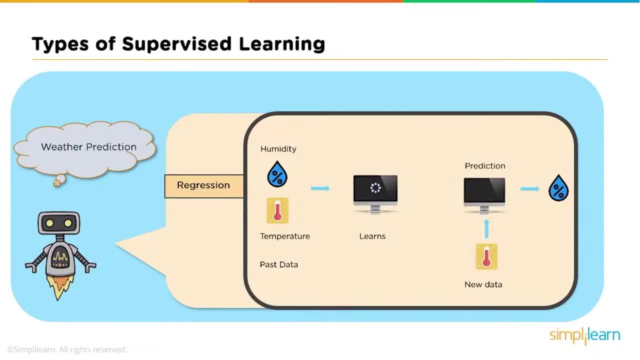 depends on the other. after the machine depends on the other. after the machine is trained, it can easily predict the is trained. it can easily predict the is trained. it can easily predict the humidity based on the given temperature. humidity based on the given temperature. humidity based on the given temperature. well, that was about regression. now let's. 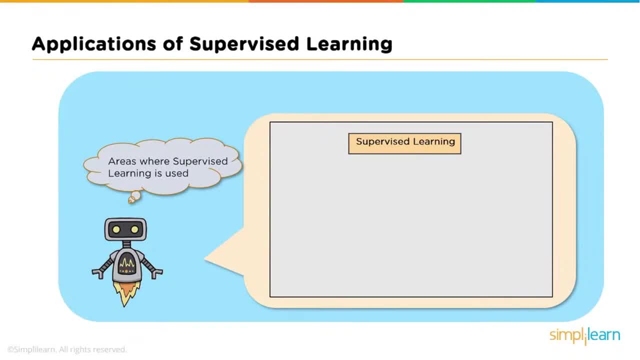 well, that was about regression now. let's- well, that was about regression now let's see some real-life applications. where see some real-life applications? where see some real-life applications where supervised learning is used? so supervised learning is used, so supervised learning is used. so supervised learning is used in risk assessment. to. 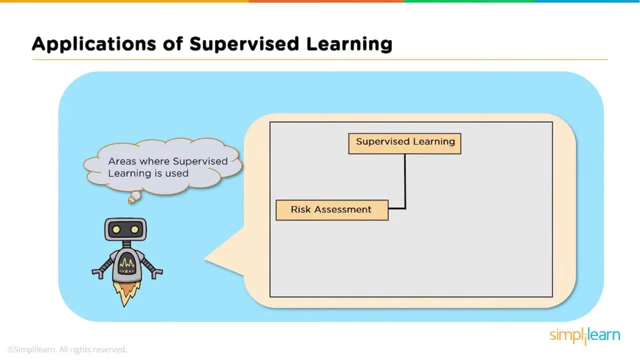 supervised learning is used to assess risk in financial services or an assess risk in financial services or an assess risk in financial services or an insurance domain to minimize the risk insurance domain. to minimize the risk insurance domain. to minimize the risk. portfolio of the companies image. portfolio of the companies image. 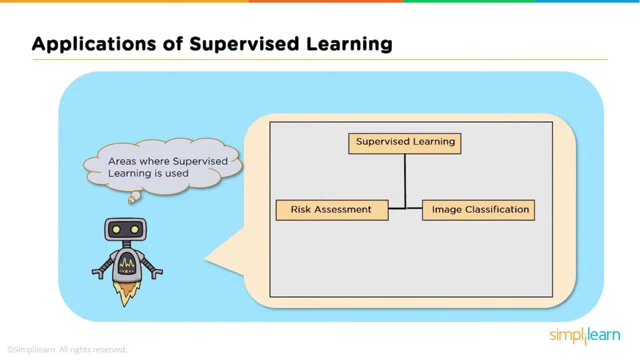 portfolio of the companies. image classification: Facebook recognizes your classification. Facebook recognizes your classification. Facebook recognizes your friend in a picture from an album of friend, in a picture from an album of friend, in a picture from an album of tagged photos. so image classification is tagged photos. so image classification is. 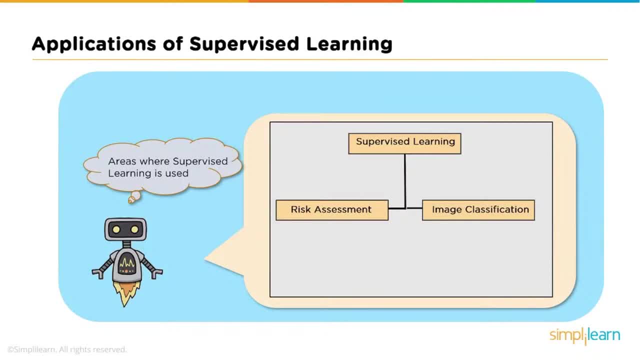 tagged photos. so image classification is one of the key use cases, of one of the key use cases, of one of the key use cases of demonstrating supervised machine, demonstrating supervised machine, demonstrating supervised machine learning algorithms- obviously a lot learning algorithms, obviously a lot learning algorithms. obviously a lot more goes into all these, like 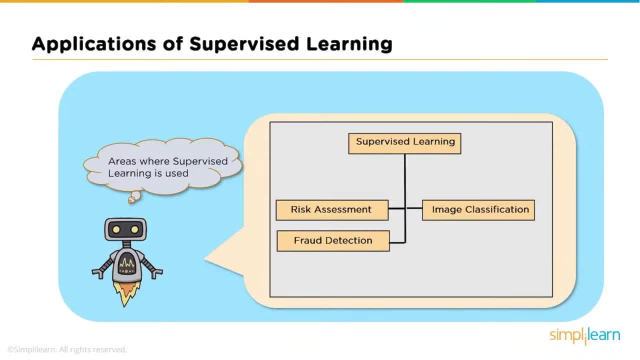 more goes into all these. like more goes into all these, like convolutional neural networks, etc. fraud, convolutional neural networks, etc. fraud, convolutional neural networks etc. fraud detection, whether the transactions made detection, whether the transactions made detection, whether the transactions made by the user are authentic or not. and 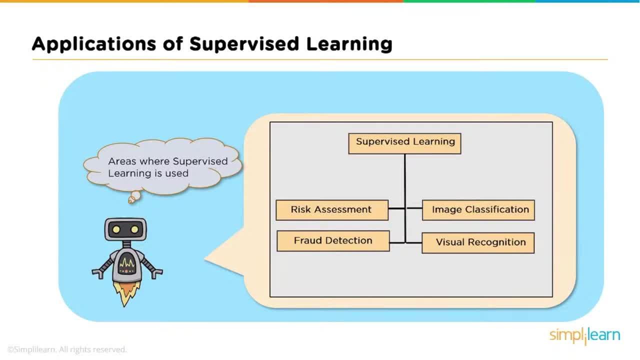 by the user are authentic or not, and by the user are authentic or not. and visual recognition: the ability of a visual recognition, the ability of a visual recognition, the ability of a machine learning model to identify machine learning model, to identify machine learning model to identify objects, places, people and actions. and 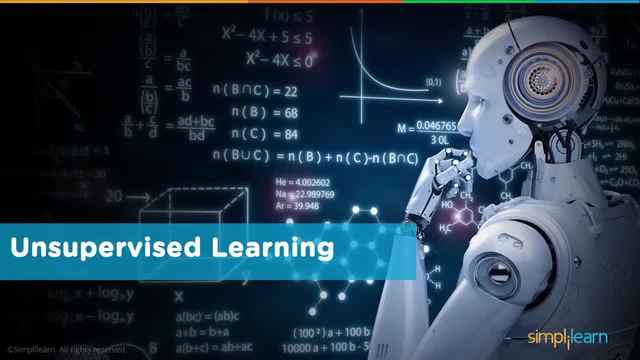 objects, places, people and actions and objects, places, people and actions and images. now, let's quickly talk about images now. let's quickly talk about images. now let's quickly talk about unsupervised learning in unsupervised, unsupervised learning in unsupervised unsupervised learning. in unsupervised learning, there is no supervision, that is. 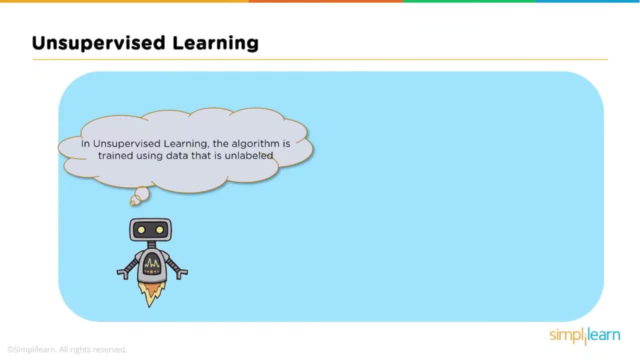 learning. there is no supervision that is learning. there is no supervision, that is. no training will be given to the machine. no training will be given to the machine. no training will be given to the machine allowing it to act on the data which is, allowing it to act on the data which is. 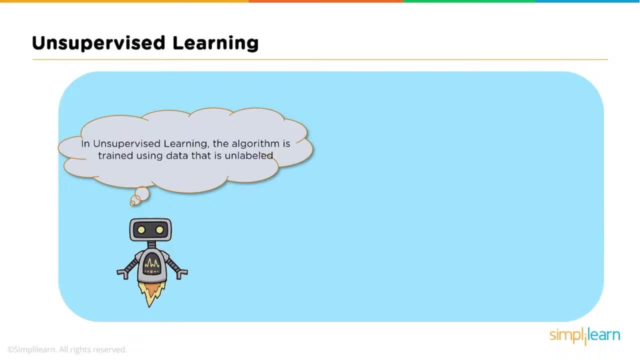 allowing it to act on the data which is not labeled. hence machine tries to not labeled. hence machine tries to not labeled. hence machine tries to identify patterns and give the response: identify patterns and give the response. identify patterns and give the response. let's take a similar example as before. 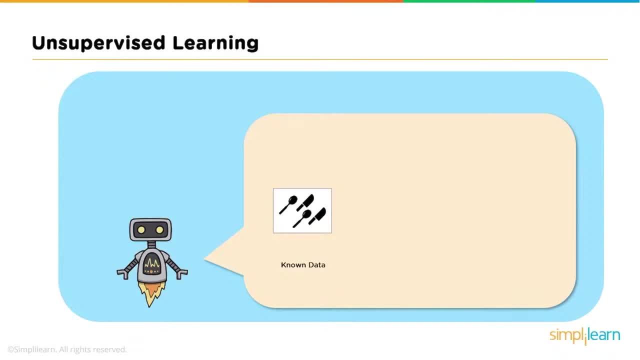 let's take a similar example as before. let's take a similar example as before, but this time we do not tell the machine. but this time we do not tell the machine. but this time we do not tell the machine, whether it's a spoon or a knife. the. 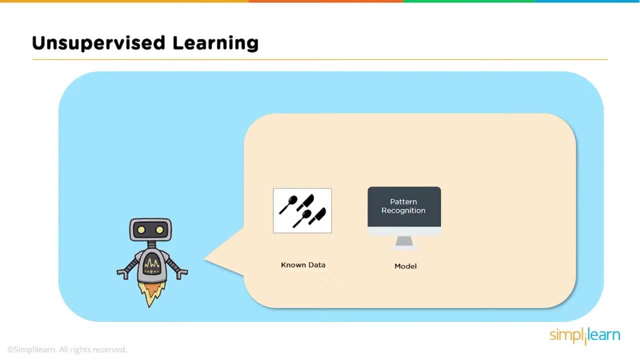 whether it's a spoon or a knife, the whether it's a spoon or a knife, the machine identifies patterns from. the machine identifies patterns from. the machine identifies patterns from the given set and groups them based on their given set. and groups them based on their given set and groups them based on their patterns, similarities, etc. again, 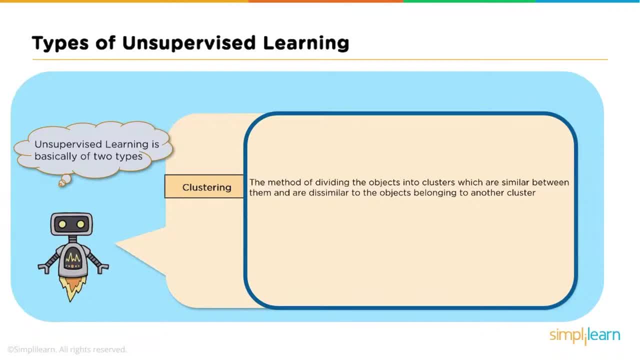 patterns, similarities, etc. again patterns, similarities, etc. again unsupervised learning can be further unsupervised learning can be further unsupervised learning can be further grouped into clustering and association. grouped into clustering and association. grouped into clustering and association. clustering is basically where the machine, clustering is basically where the machine. 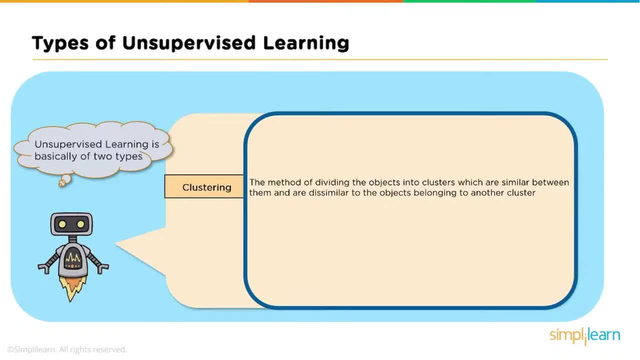 clustering is basically where the machine forms groups based on the behavior of the forms groups, based on the behavior of the forms groups, based on the behavior of the data. secondly, association: it is a rule data. secondly, association: it is a rule data. secondly, association: it is a rule based machine learning to discover. 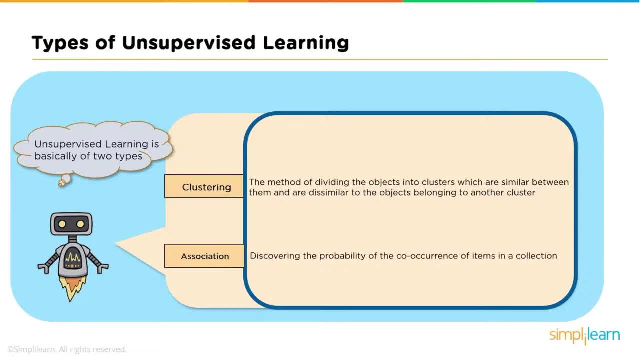 based machine learning to discover. based machine learning to discover interesting relation between variables, in interesting relation between variables, in interesting relation between variables in large data sets, for example. which large data sets, for example. which large data sets, for example, which customer made similar product purchases. customer made similar product purchases. 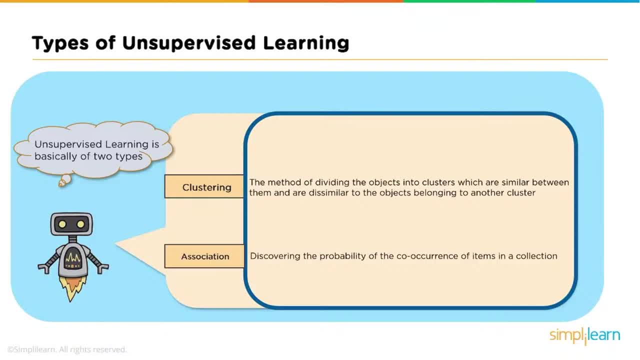 customer made similar product purchases is clustering, whereas association is is clustering, whereas association is is clustering, whereas association is which products were purchased together, which products were purchased together, which products were purchased together. now, let's understand clustering with the. now, let's understand clustering with the. now let's understand clustering with the help of an example. 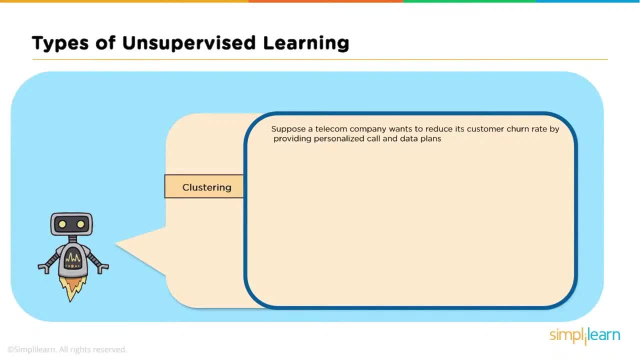 help of an example. help of an example to reduce their churn rate: a telecom to reduce their churn rate. a telecom to reduce their churn rate. a telecom company studies the behavior of the company studies. the behavior of the company studies the behavior of the customers- customers, customers based on average call duration and. 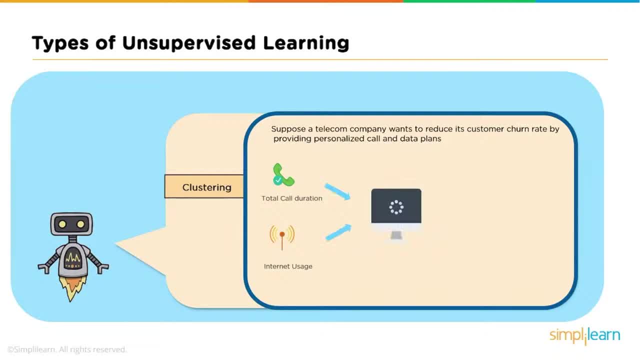 based on average call duration. and based on average call duration and internet usage. and observes that, while internet usage and observes that, while internet usage, and observes that, while some customers call duration is quite, some customers call duration is quite some customers call duration is quite high. others have heavy internet usage. the 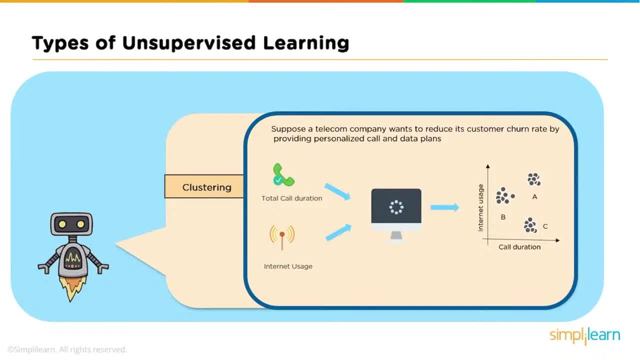 high. others have heavy internet usage. the high. others have heavy internet usage. the customers are grouped based on their customers are grouped based on their customers, are grouped based on their observed behavior and a strategy is observed behavior and a strategy is observed behavior and a strategy is adopted to minimize churn rate and 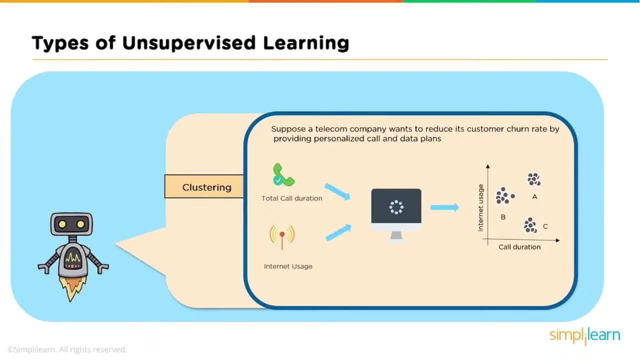 adopted to minimize churn rate and adopted to minimize churn rate and maximize profit by suitable promotions. maximize profit by suitable promotions. maximize profit by suitable promotions and campaigns and campaigns and campaigns, as you can see in the chart on the right. as you can see in the chart on the right. 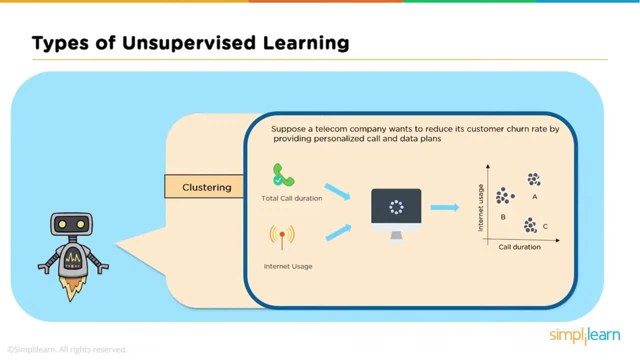 as you can see in the chart on the right hand side customers in group a uses more hand side customers in group a uses more hand side customers in group a uses more data and also have high quadration group data. and also have high quadration group data and also have high quadration group b customers are heavy internet users. 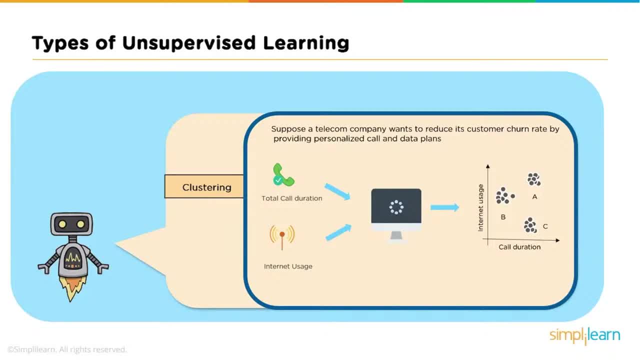 b customers are heavy internet users. b customers are heavy internet users, while group c customers have high, while group c customers have high, while group c customers have high quadration. so group b will be given more quadration, so group b will be given more quadration. so group b will be given more data benefit plans, while group c will be 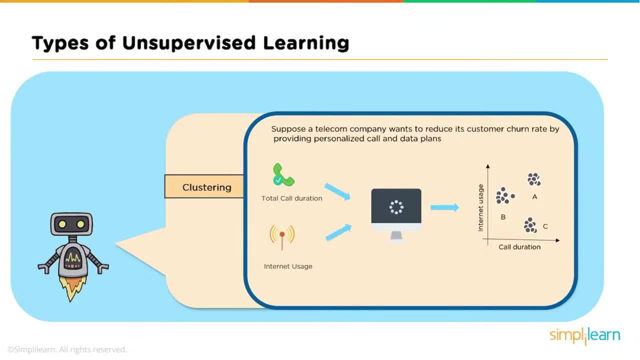 data benefit plans, while group c will be data benefit plans, while group c will be given cheaper call rates to buy their given cheaper call rates to buy their given cheaper call rates to buy their loyalty. so this was the example of loyalty. so this was the example of 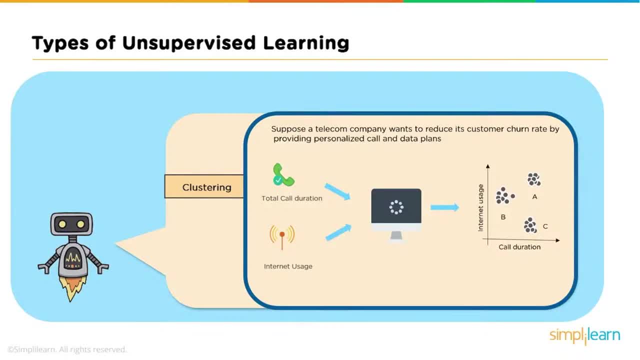 loyalty. so this was the example of clustering. now let's understand clustering. now let's understand clustering. now let's understand association with another example. let's association with another example. let's say customer 1 goes to a supermarket. say customer 1 goes to a supermarket. say customer 1 goes to a supermarket and buys these products, say bread, milk. 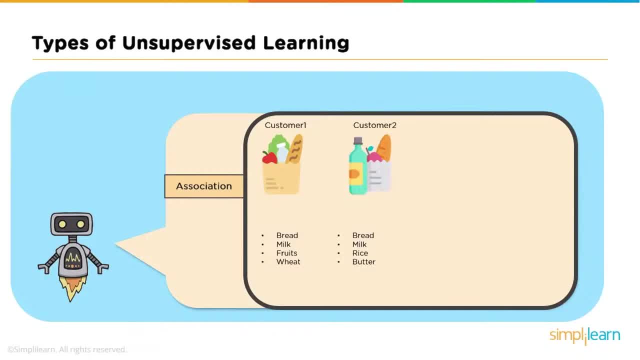 and buys these products. say bread, milk and buys these products. say bread, milk, fruits wheat, then customer 2 goes and fruits wheat. then customer 2 goes and fruits wheat. then customer 2 goes and buys bread, milk, rice and butter now. buys bread, milk, rice and butter now. 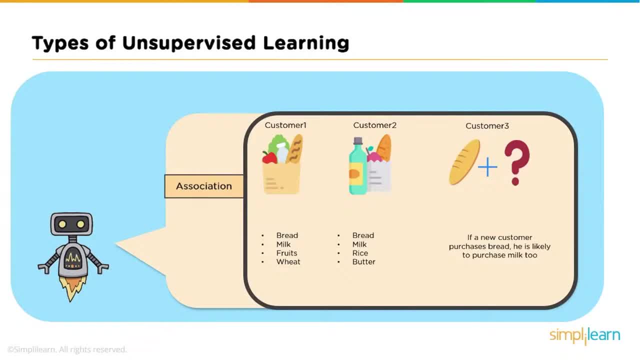 buys bread, milk, rice and butter. now, when customer 3 goes and buys bread, it when customer 3 goes and buys bread, it when customer 3 goes and buys bread, it is highly likely that he will also buy, is highly likely that he will also buy. is highly likely that he will also buy milk. hence, relationship is established. 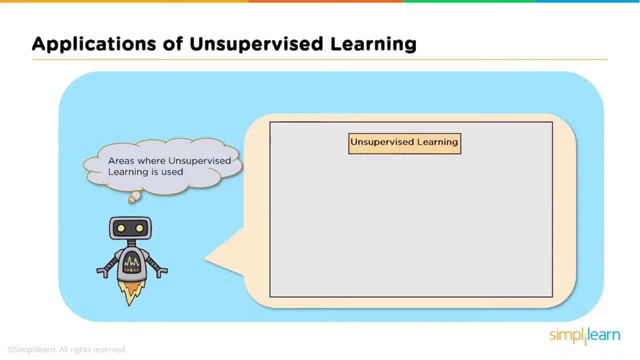 milk, hence, relationship is established. milk, hence, relationship is established based on customer behavior and based on customer behavior and based on customer behavior, and recommendations are made now. let's look at recommendations are made now. let's look at recommendations are made now. let's look at some real-life applications of. 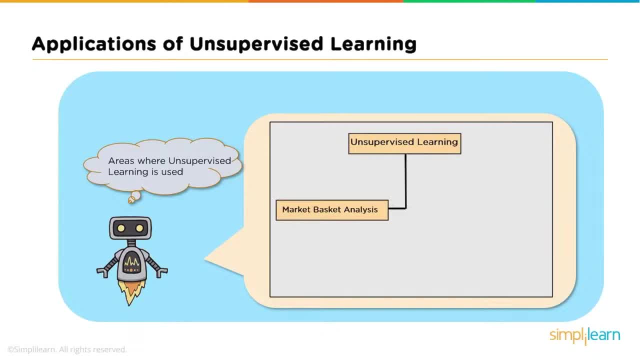 some real-life applications of some real-life applications of unsupervised learning market basket. unsupervised learning market basket. unsupervised learning market basket analysis is a machine learning model. analysis is a machine learning model. analysis is a machine learning model based on the algorithm that if you buy a, 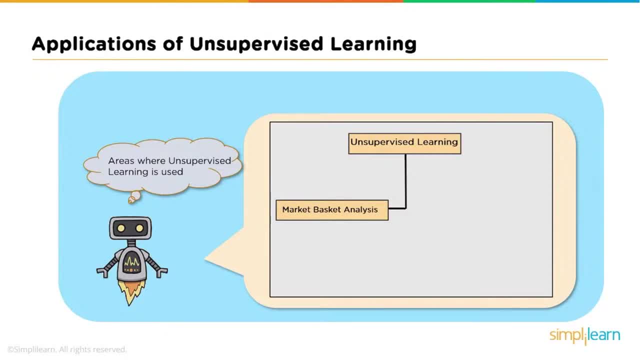 based on the algorithm that, if you buy a. based on the algorithm that if you buy a certain group of items, you are less or certain group of items you are less or certain group of items you are less or more likely to buy another group of, more likely to buy another group of. 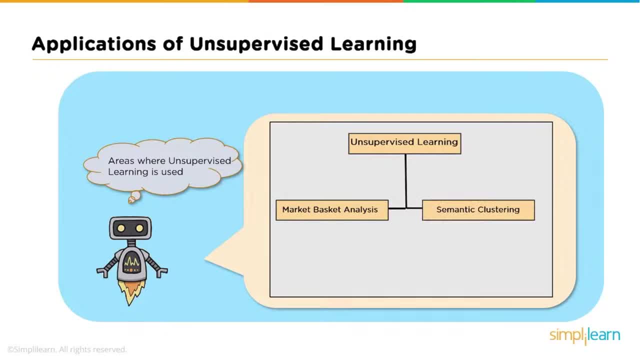 more likely to buy another group of items. semantic clustering semantically. items semantic clustering semantically. items semantic clustering semantically. similar words share similar context. similar words share similar context. similar words share similar context. people post their queries on websites in. people post their queries on websites in. 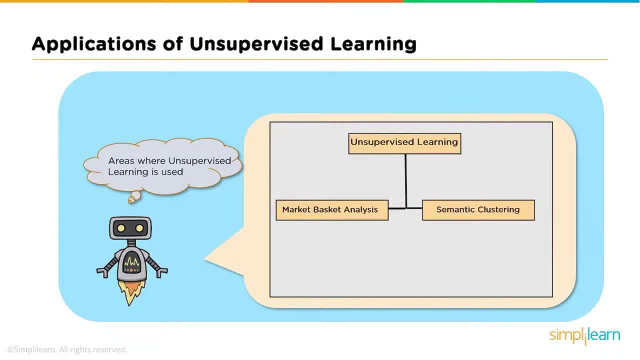 people post their queries on websites in their own ways. semantic clustering their own ways. semantic clustering their own ways. semantic clustering groups: all responses in a cluster with groups. all responses in a cluster with groups. all responses in a cluster with same meaning to ensure that the customer. same meaning, to ensure that the customer. 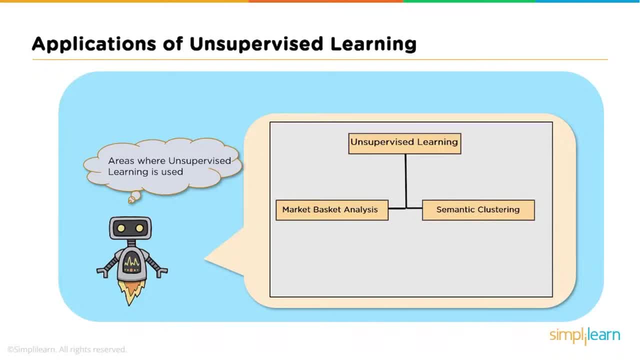 same meaning: to ensure that the customer finds the information they want quickly. finds the information they want quickly, finds the information they want quickly and easily. it plays an important role in, and easily. it plays an important role in, and easily. it plays an important role in information retrieval. good browsing. 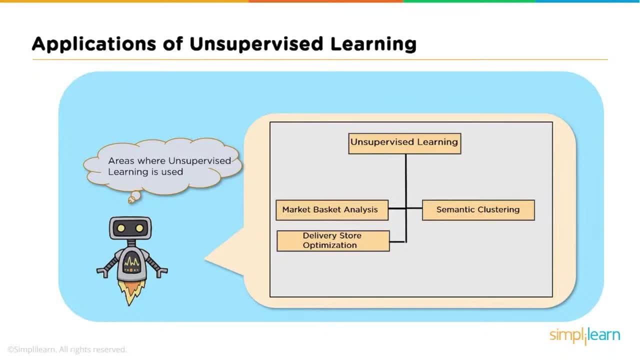 information retrieval. good browsing information retrieval. good browsing experience and comprehension delivery experience and comprehension delivery experience and comprehension delivery. store optimization. machine learning store optimization. machine learning store optimization. machine learning models are used to predict the demand. models are used to predict the demand. models are used to predict the demand and keep up with the supply. also to open. 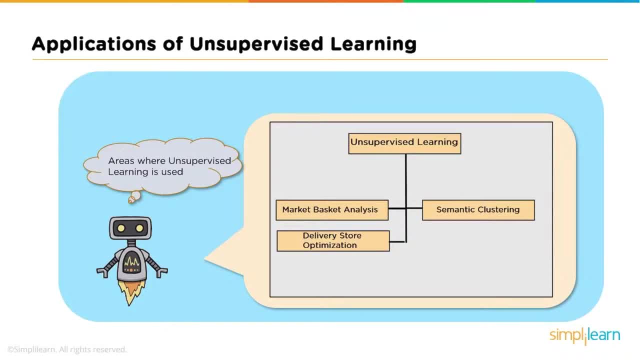 and keep up with the supply also. to open and keep up with the supply also to open stores where demand is more and stores where demand is more and stores where demand is more. and optimizing routes for more efficient. optimizing routes for more efficient, optimizing routes for more efficient deliveries according to past data and 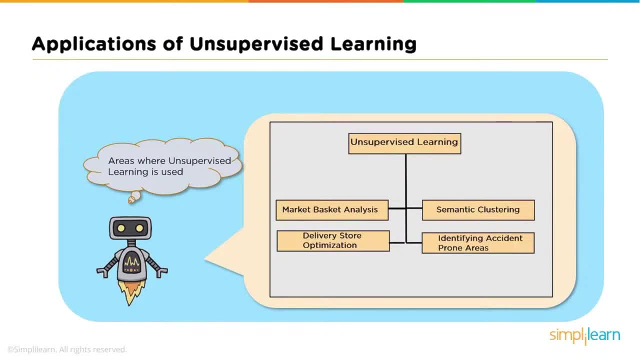 deliveries according to past data and deliveries according to past data and behavior. we can also use unsupervised behavior. we can also use unsupervised behavior. we can also use unsupervised machine learning models to identify machine learning models. to identify machine learning models to identify accident prone areas based on the 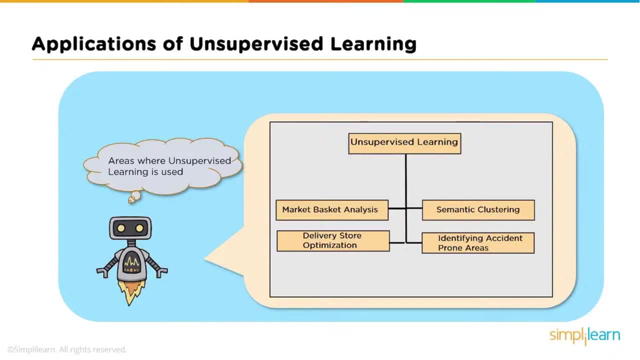 accident prone areas based on the accident prone areas based on the intensity of those accidents and the intensity of those accidents and the intensity of those accidents. and the area in order to introduce safety area in order to introduce safety area, in order to introduce safety measures. by now, i hope you have. 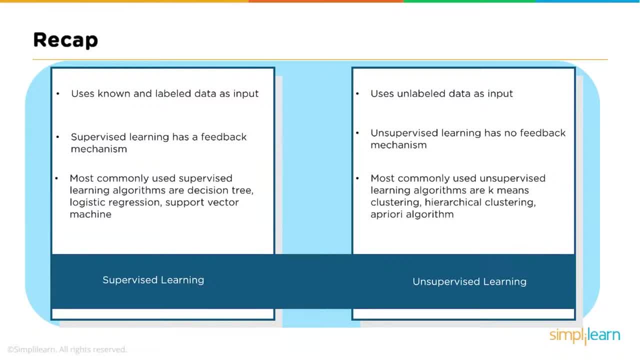 measures by now. i hope you have measures by now. i hope you have understood, supervised and unsupervised. understood, supervised and unsupervised. understood, supervised and unsupervised. learning for a quick recap. let's see a learning for a quick recap. let's see a learning for a quick recap. let's see a few differences between the two. the most. 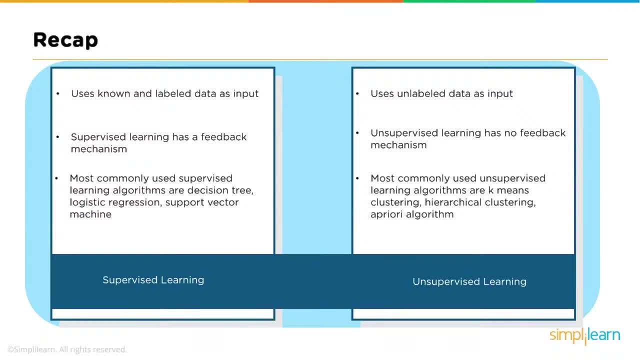 few differences between the two, the most few differences between the two. the most fundamental difference is that fundamental difference is that fundamental difference is that supervised learning uses known and label. supervised learning uses known and label. supervised learning uses known and label data and unsupervised learning uses. 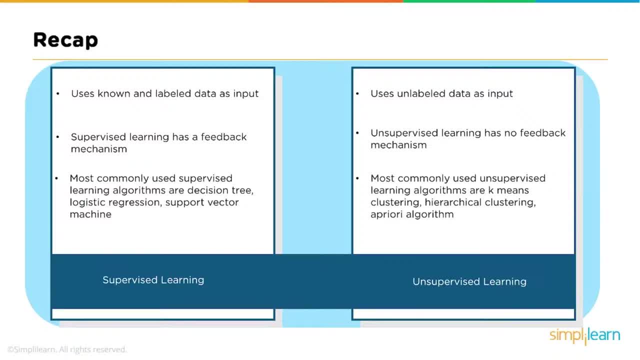 data and unsupervised learning uses data and unsupervised learning uses unlabeled data as their input. secondly, unlabeled data as their input. secondly, unlabeled data as their input. secondly, supervised learning follows a feedback. supervised learning follows a feedback, supervised learning follows a feedback mechanism, while unsupervised learning 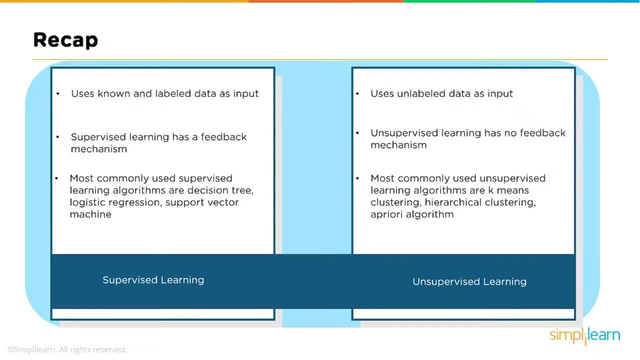 mechanism, while unsupervised learning mechanism, while unsupervised learning does not also the most commonly used, does not also the most commonly used, does not also the most commonly used? algorithms in supervised learning are algorithms in supervised learning. are algorithms in supervised learning are decision tree, decision tree. 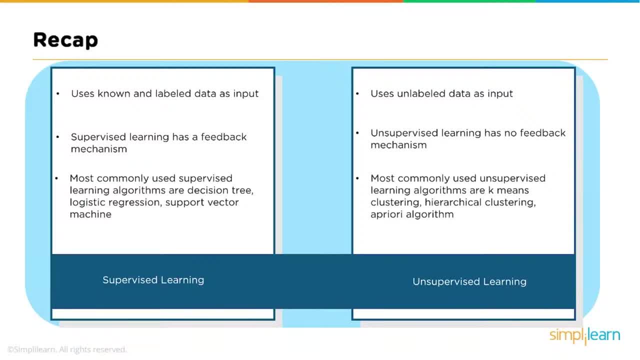 decision tree: logistic regression support vector. logistic regression support vector. logistic regression support vector machine etc. and in unsupervised machine etc. and in unsupervised machine etc. and in unsupervised learning. there k means clustering, learning, there k means clustering learning. there k means clustering, hierarchical clustering a priori. 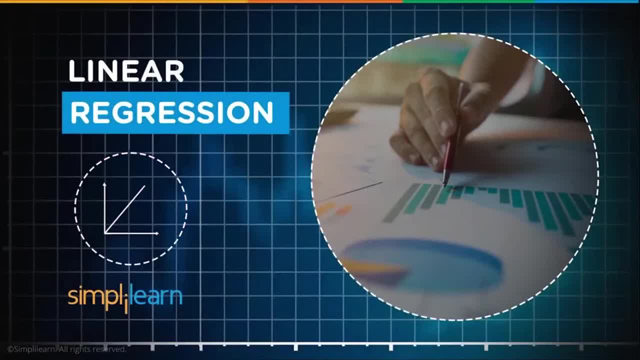 hierarchical clustering a priori. hierarchical clustering a priori. algorithm and many more. welcome to algorithm. and many more welcome to algorithm and many more welcome to linear regression. my name is richard linear regression. my name is richard linear regression. my name is richard kirschner. i'm with simply learn let's. 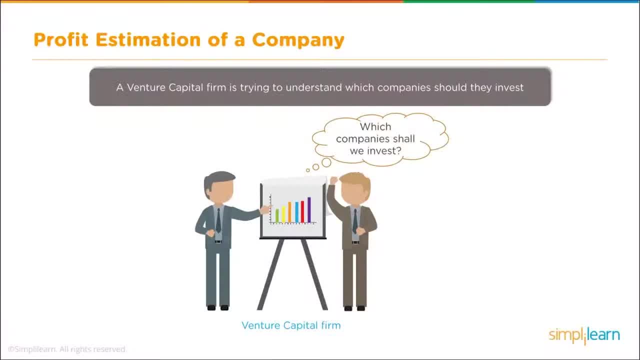 kirschner, i'm with, simply learn. let's, kirschner, i'm with, simply learn. let's take a look at a venture capitalist. take a look at a venture capitalist, take a look at a venture capitalist firm and try to understand which firm and try to understand which. 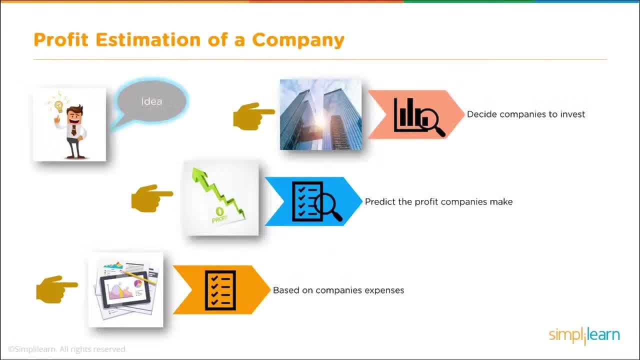 firm and try to understand which companies they should invest in. so companies they should invest in, so companies they should invest in. so we'll take the idea that we need to. we'll take the idea that we need to. we'll take the idea that we need to decide the companies to invest in. we 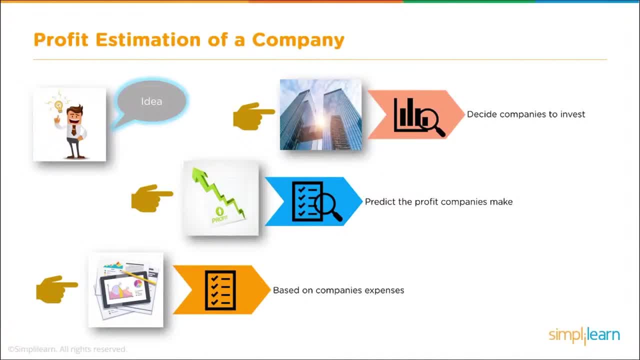 decide the companies to invest in. we decide the companies to invest in. we need to predict the profit. the company need to predict the profit. the company need to predict the profit the company makes, and we're going to do it based on makes and we're going to do it based on. 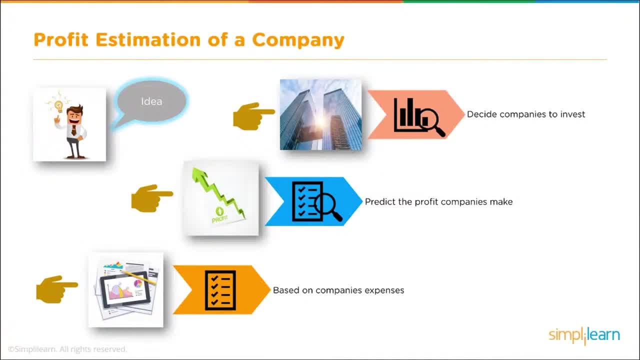 makes, and we're going to do it based on the company's expenses and even just a the company's expenses, and even just a the company's expenses, and even just a specific expense. in this case, we have specific expense. in this case, we have specific expense. in this case, we have our company, we have the different. 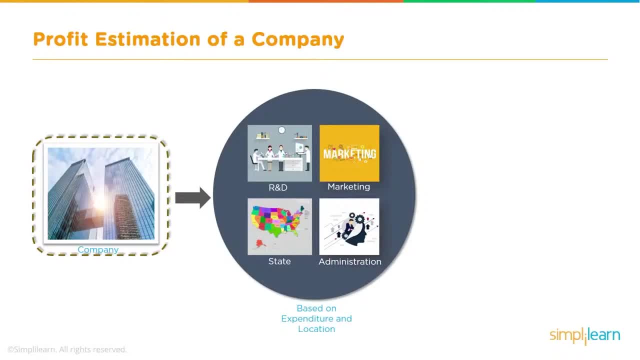 our company. we have the different our company. we have the different expenses. we have our r? d, which is your expenses. we have our r? d, which is your expenses. we have our r? d, which is your research and development. we have our research and development. we have our. 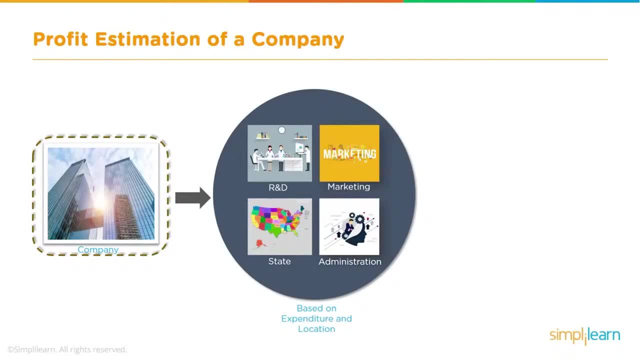 research and development. we have our marketing, marketing, marketing. we might have the location we might have. we might have the location we might have. we might have the location we might have. what kind of administration is going? what kind of administration is going, what kind of administration is going through based on all this different? 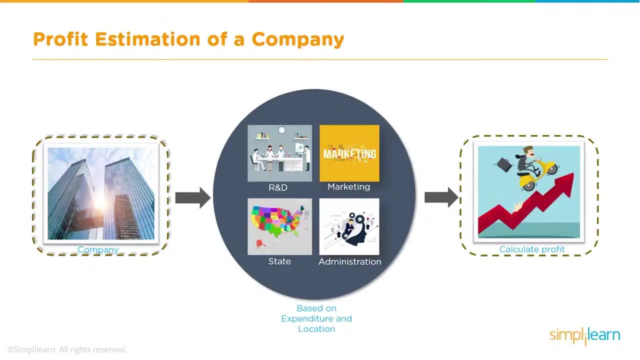 through. based on all this different through, based on all this different information, we would like to calculate information. we would like to calculate information. we would like to calculate the profit. now, in actuality, there's is usually about 23 to 27 different markers that they look at if they're a heavy duty investor. 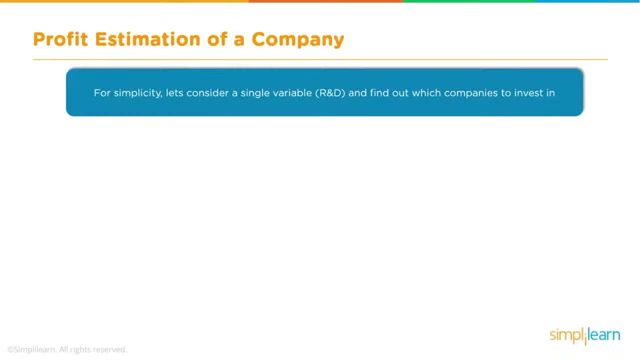 We're only gonna take a look at one basic one. We're gonna come in and, for simplicity, let's consider a single variable, R and D, and find out which companies to invest in based on that. So we take our R and D, we're plotting the profit based on the R and D expenditure. 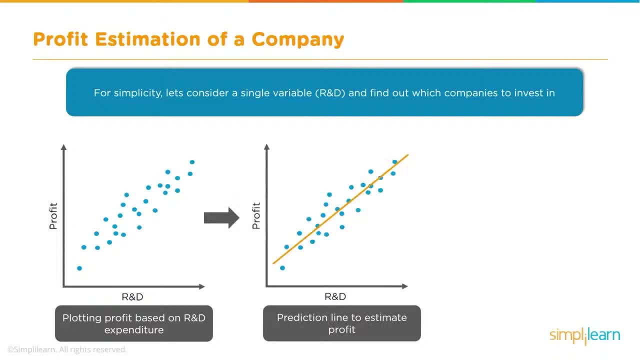 how much money they put into the research and development. And then we look at the profit that goes with that. We can predict a line to estimate the profit. So we draw a line right through the data. When you look at that you can see how much they invest in the R and D. 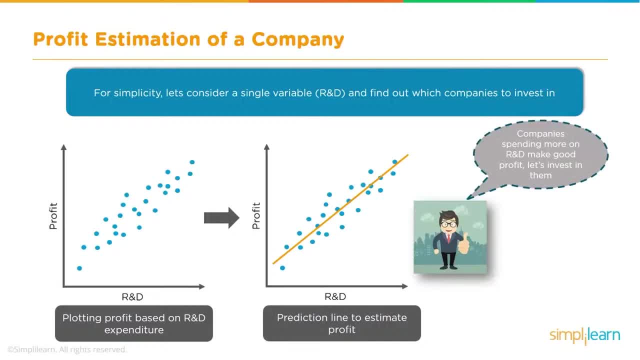 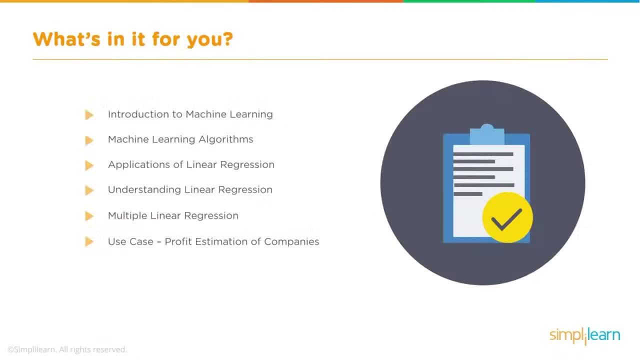 is a good marker as to how much profit they're gonna have. We can also note that companies spending more on R and D make good profit, So let's invest in the ones that spend a higher rate in their R and D. What's in it for you? 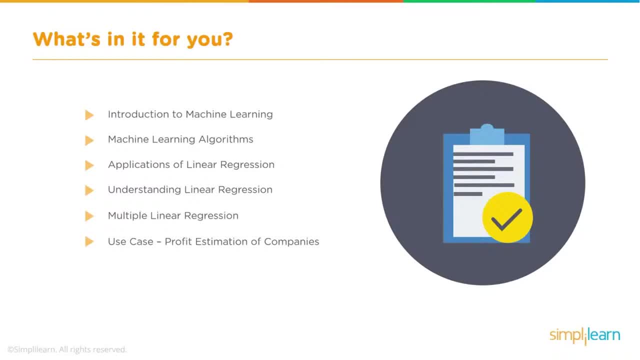 First we'll have an introduction to machine learning, followed by machine learning algorithms. These will be specific to linear regression and where it fits into the larger model. Then we'll take a look at applications of linear regression: understanding linear regression and multiple linear. 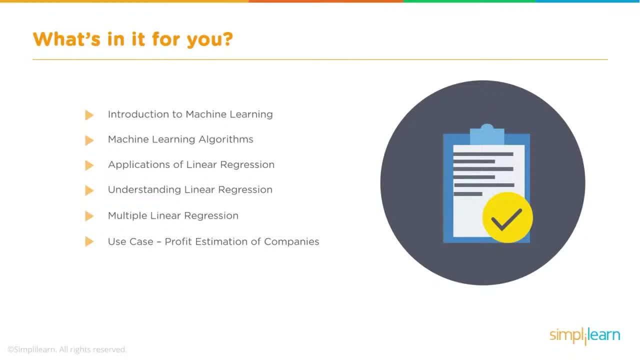 finally, we'll roll up our sleeves and do a little programming in use case profit estimation of companies. Let's go ahead and jump in. Let's start with our introduction to machine learning, along with some machine learning algorithms and, where that fits in, with linear regression. 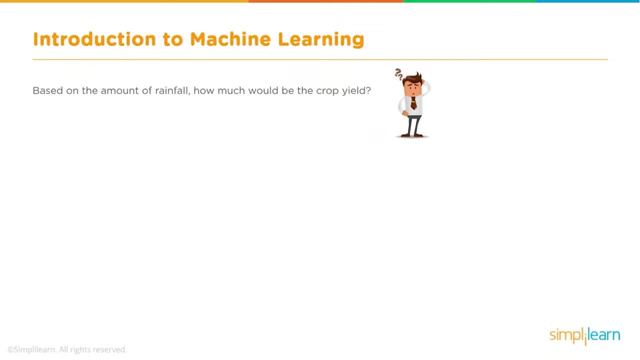 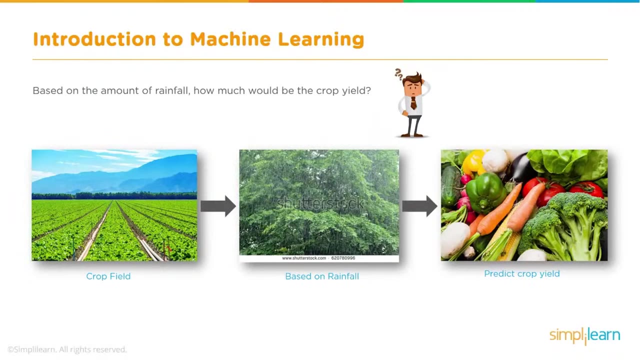 Let's look at another example of machine learning. Based on the amount of rainfall, how much would be the crop yield? So here we have our crops, we have our rainfall and we wanna know how much we're gonna get from our crops this year. 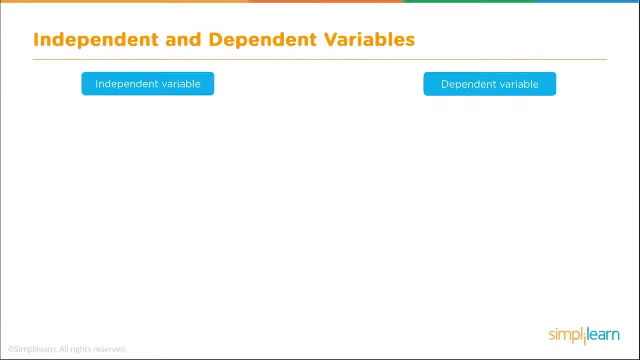 So we're gonna introduce two variables: Independent and dependent. The independent variable is a variable whose value does not change by the effect of other variables and is used to manipulate the dependent variable. It is often denoted as X. In our example, rainfall is the independent variable. 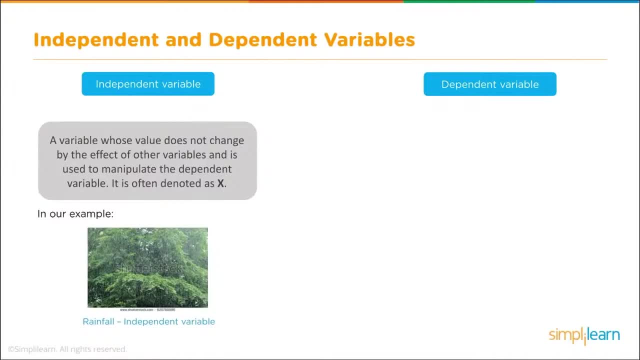 This is a wonderful example, because you can easily see that we can't control the rain, but the rain does control the crop. So we talk about the independent variable controlling the dependent variable. Let's define dependent variable as a variable whose value change when there is any manipulation of the variable. 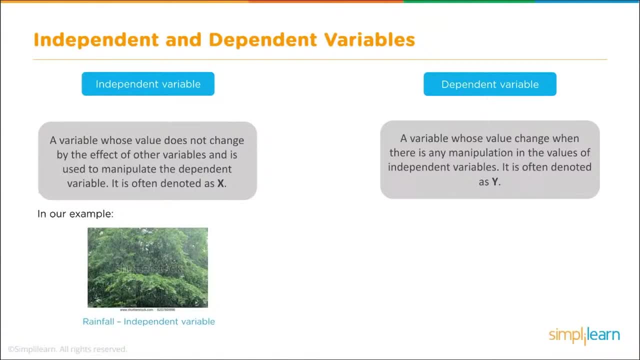 So what we're gonna do is we're gonna calculate the values of the independent variables. It is often denoted as Y And you can see here our crop yield is dependent variable and it is dependent on the amount of rainfall received. Now that we've taken a look at a real-life example, 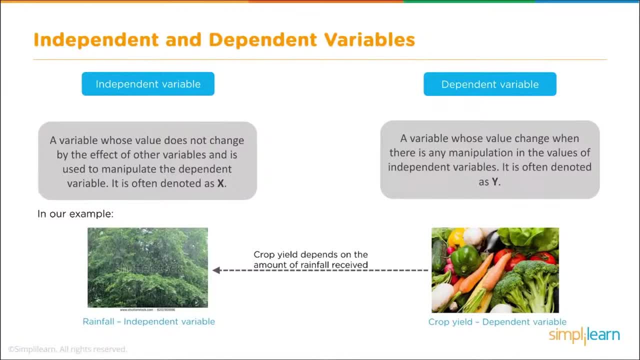 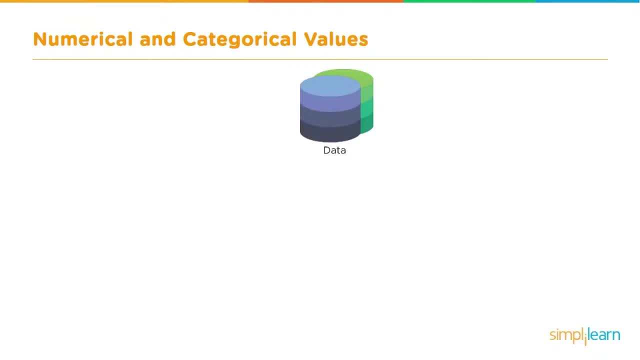 let's go a little bit into the theory and some definitions on machine learning and see how that fits together with linear regression, Numerical and categorical values. Let's take our data coming in. This is kind of random data from any kind of project. 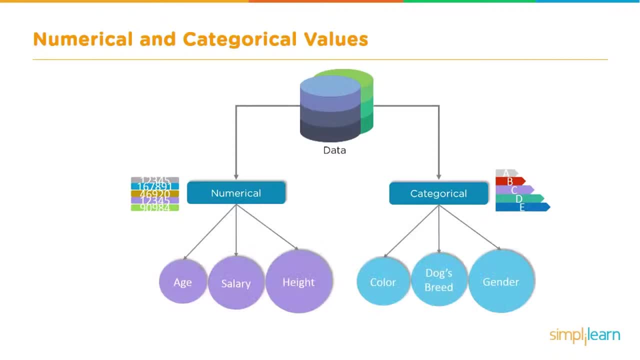 We wanna divide it up into numerical and categorical values, and categorical. So numerical is numbers, age, salary, height, Where categorical would be a description, the color a dog's breed, gender. Categorical is limited to very specific items, where numerical is a range of information. Now that you've seen the difference between, 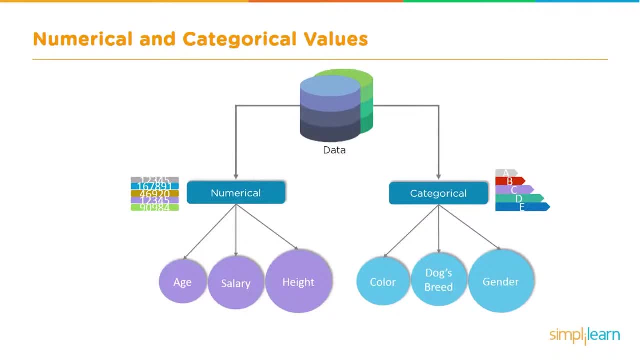 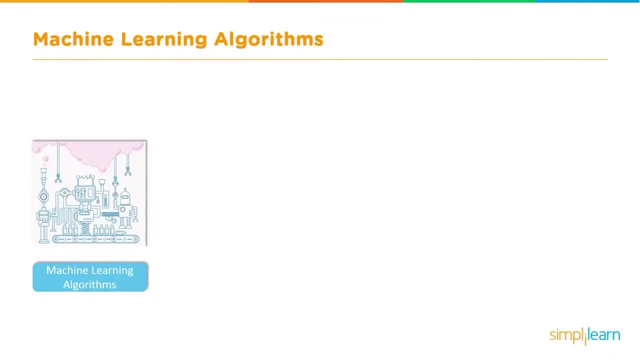 numerical and categorical data. let's take a look at some different machine learning definitions. When we look at our different machine learning algorithms, we can divide them into three areas: Supervised, unsupervised, reinforcement. We're only going to look at 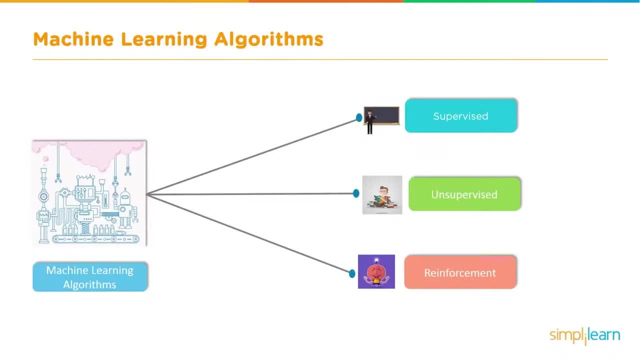 supervised. today, Unsupervised means we don't have the answers and we're just grouping things. Reinforcement is where we give positive and negative feedback to our algorithm to program it, and it doesn't have the information until after the fact. But today we're just looking. 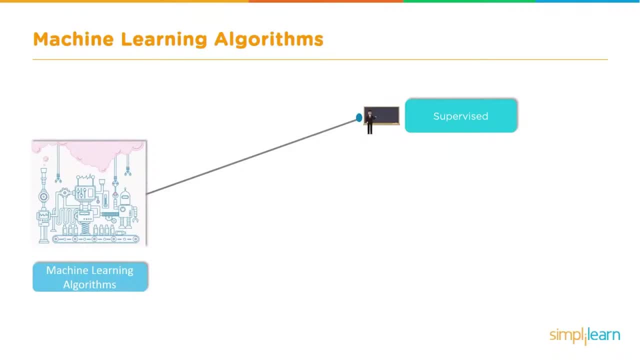 at supervised, because that's where linear regression fits in. In supervised data. we have our data already there and our answers for a group, And then we use that to program our model and come up with an answer. The two most common uses for that is through the 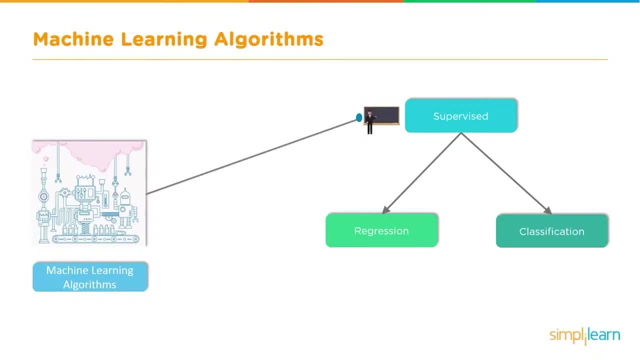 regression and classification. Now we're doing linear regression, so we're just going to focus on the regression side. And in the regression we have simple linear regression, we have multiple linear regression and we have polynomial linear regression. Now, on these three simple 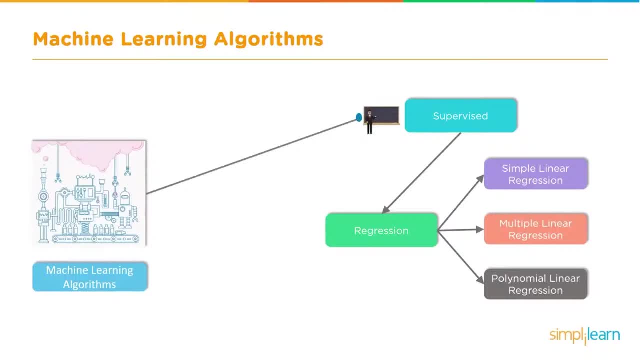 linear regression is the examples we've looked at so far, where we have a lot of data And we draw a straight line through it. Multiple linear regression means we have multiple variables. Remember where we had the rainfall and the crops, We might add additional. 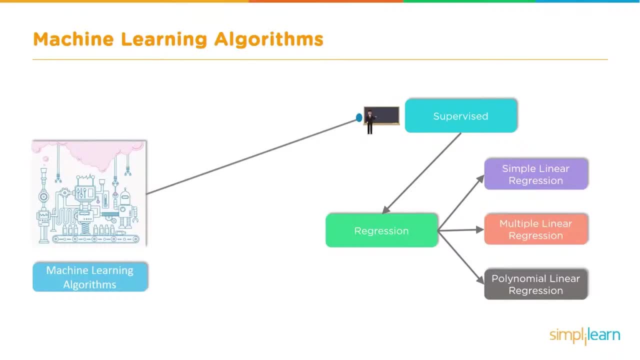 variables in there, like how much food do we give our crops, When do we harvest them. Those would be additional information add into our model And that's why it'd be multiple linear regression. And finally we have polynomial linear regression, That is, instead of drawing a line, we can draw a. 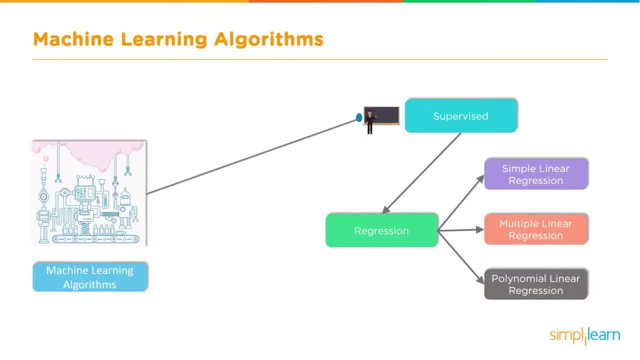 curved line through it. Now that you see where regression model fits into the machine learning and we're specifically looking at linear regression, let's go ahead and take a look at applications for linear regression. Let's look at a few applications of linear regression: Economic. 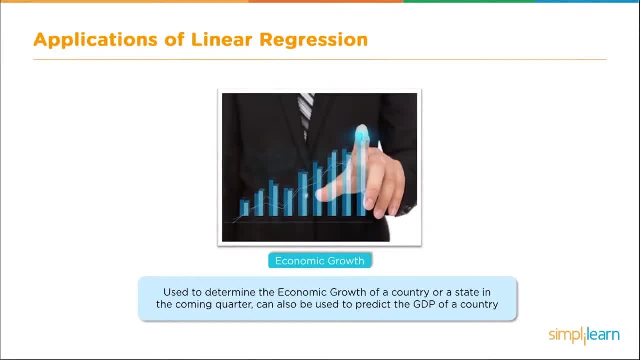 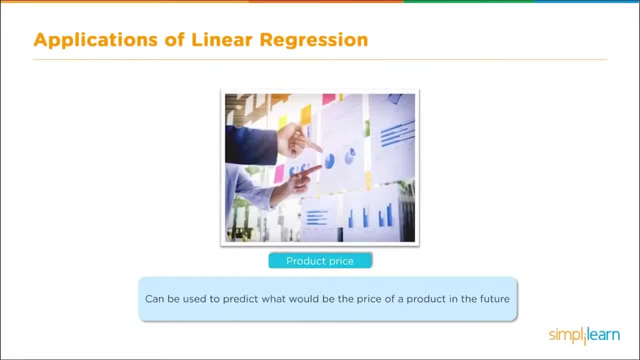 growth used to determine the economic growth of a country or a state in the coming quarter. can also be used to predict the GDP of a country. Product price can be used to predict what would be the price of a product in the future. You can guess whether it's going to go up. 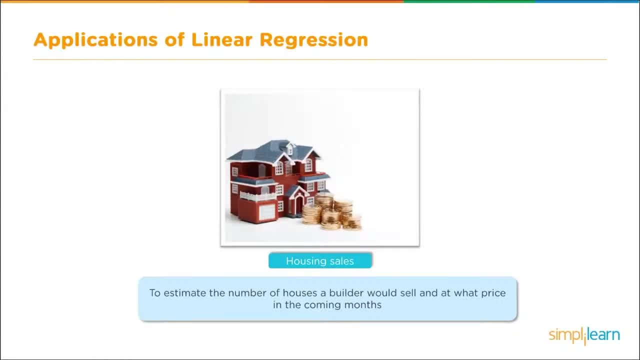 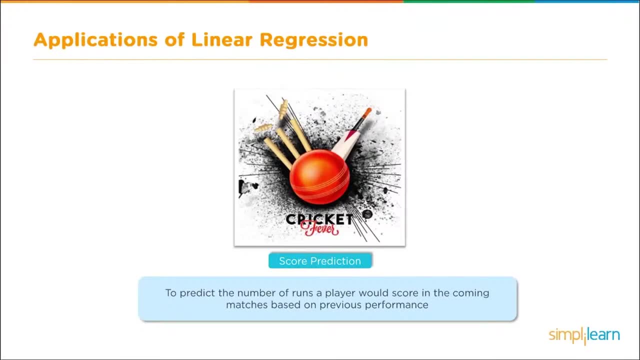 or down, or should I buy it today? Housing sales: to estimate the number of houses a builder would sell, and what price, in the coming months. Score predictions- cricket fever: to predict the number of runs a player would score in the coming matches based on the previous. 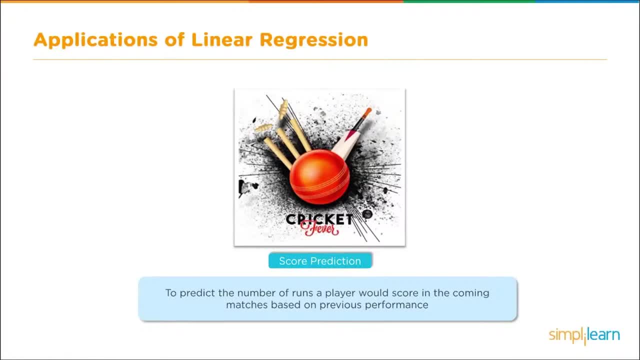 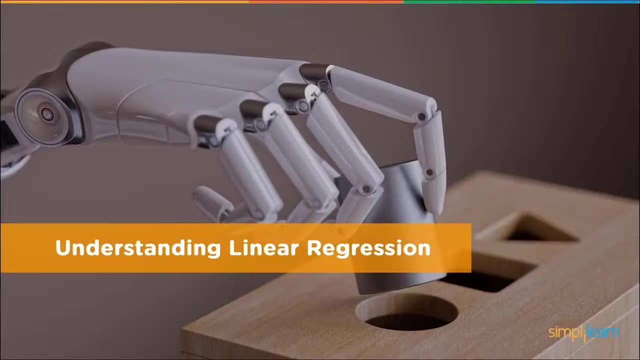 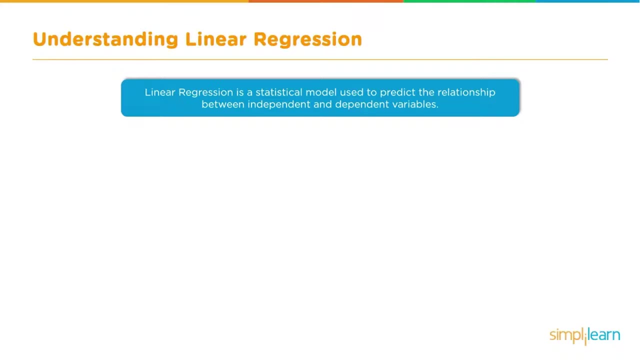 performance. I'm sure you can figure out other applications you could use linear regression for. So let's jump in and let's understand linear regression and dig into the theory Understanding linear regression. Linear regression is the statistical model used to predict the relationship between independent and dependent variables. 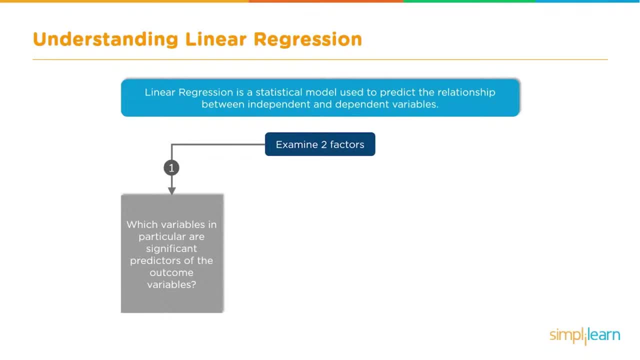 By examining two factors. The first important one is which variables in particular are significant predictors of the outcome variable, And the second one that we need to look at closely is how significant is the regression line to make predictions with the highest possible accuracy. If it's inaccurate, we can't use it, So it's very important we find out the 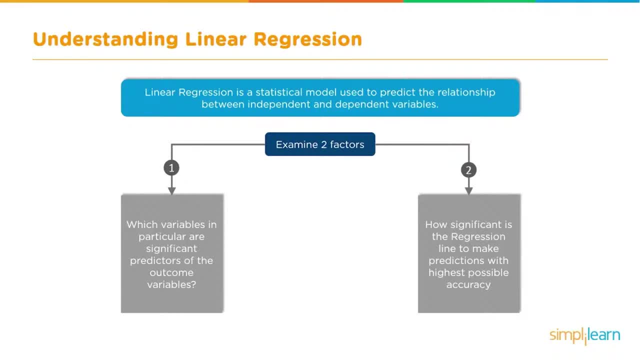 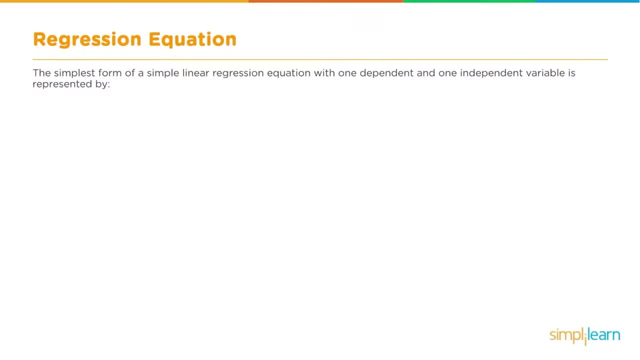 most accurate line we can get. Since linear regression is based on drawing a line through data, we're going to jump back and take a look at some Euclidean geometry. The simplest form of a simple linear regression equation with one dependent and one independent variable is represented by y equals m times x plus c. And if you look at our model here, 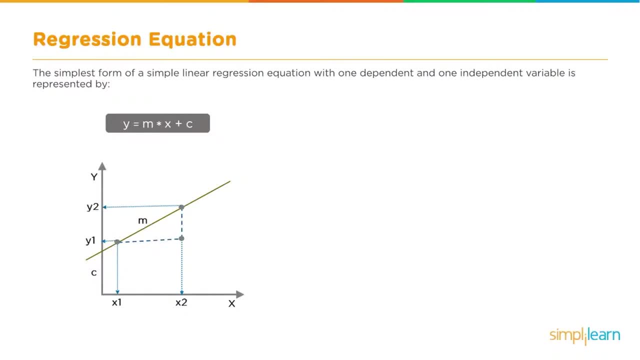 we plotted two points on here: x1 and y1,, x2 and y2.. y being the dependent variable- Remember that from before- And x being the independent variable. So y depends on whatever x is. m, in this case, is the slope. 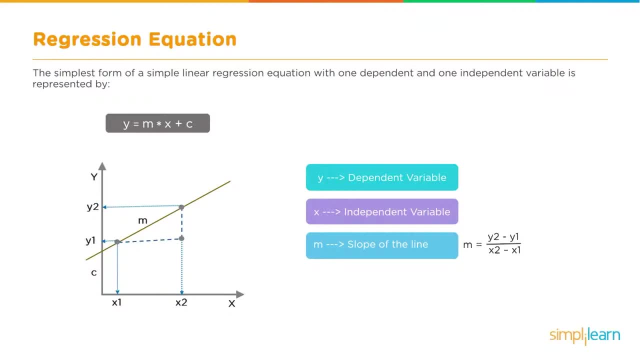 m is the slope of the line, where m equals the difference in the y2 minus y1 and x2 minus x1.. And finally we have c, which is the coefficient of the line, or where it happens to cross the zero axes. Let's go back and look at an example we used earlier of linear regression. We're going 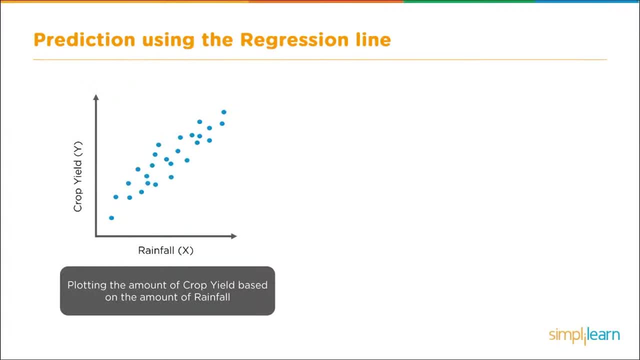 to go back to plotting the amount of crop yield based on the amount of rainfall. And here we have our rainfall- Remember, we cannot change rainfall- And we have our crop yield Which is dependent on the rainfall. We have our independent and our dependent variables. 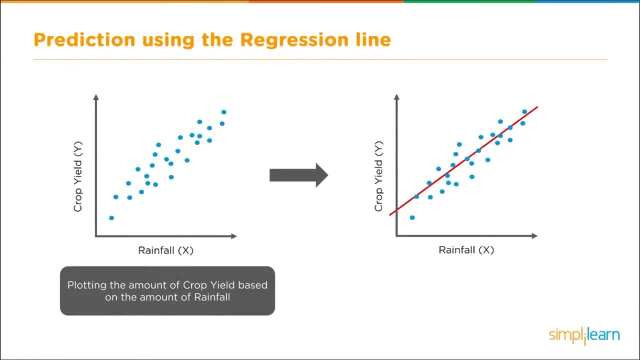 We're going to take this and draw a line through it as best we can through the middle of the data, And then we look at that and we put the red point on the y-axis as the amount of crop yield you can expect for the amount of rainfall represented by the green dot. 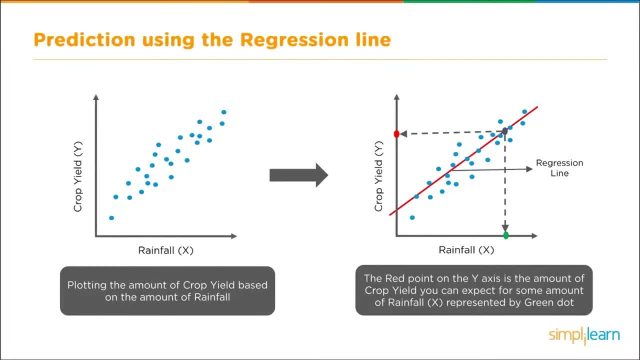 So if we have an idea what the rainfall is for this year and what's going on, then we can guess how good our crops are going to be. And we've created a nice line right through the middle to give us a nice mathematical formula. 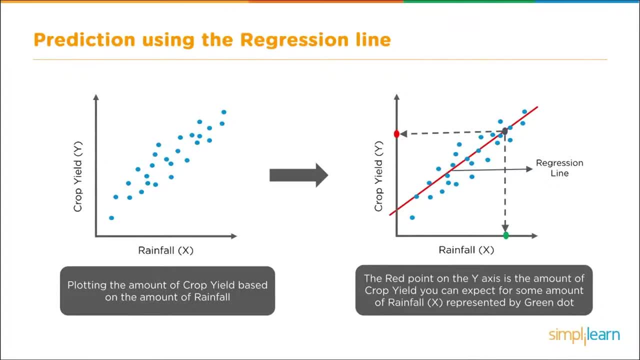 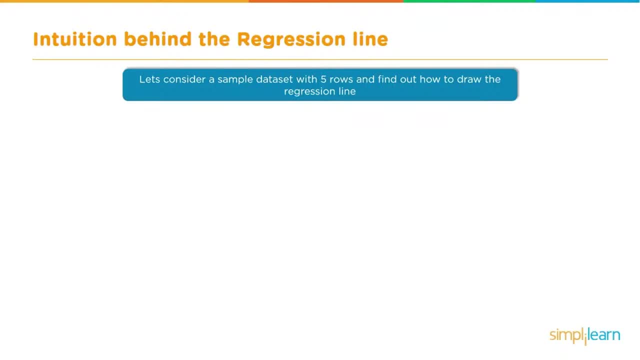 Let's take a look and see what the math looks like behind this. Let's look at the intuition behind the regression line. Now, before we dive into the math and the formulas that go behind this and what's going on behind the scenes, I want you to 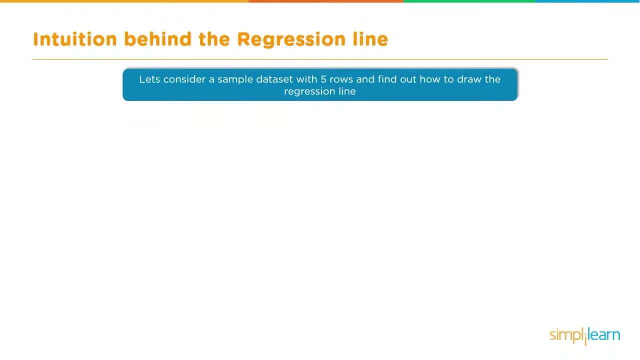 note that when we get into the case study and we actually apply some Python script, that this math that you're gonna see here is already done automatically for you. You don't have to have it memorized. It is, however, good to have an idea what's going on. so if people reference the different terms, you'll 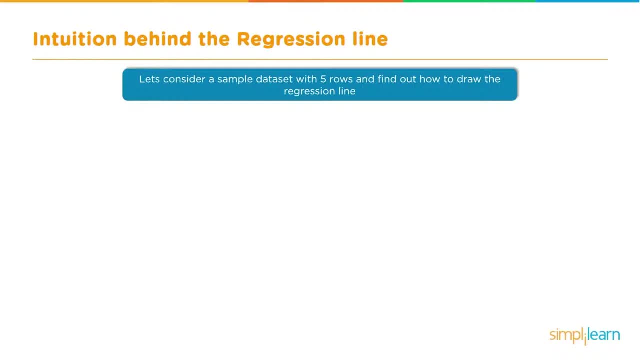 know what they're talking about. Let's consider a sample data set with five rows and find out how to draw the regression line. We're only going to do five rows because if we did like the rainfall with hundreds of points of data, that would be very hard to see what's going on with the mathematics. So we'll 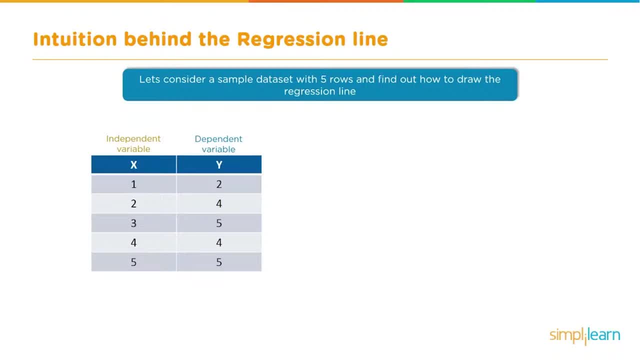 go ahead and create our own two sets of data and we have our independent variable x and our dependent variable y, and when x was 1, we got y equals 2, when x was 2, y was 4, and so on and so on. If we go ahead and plot this data on a, 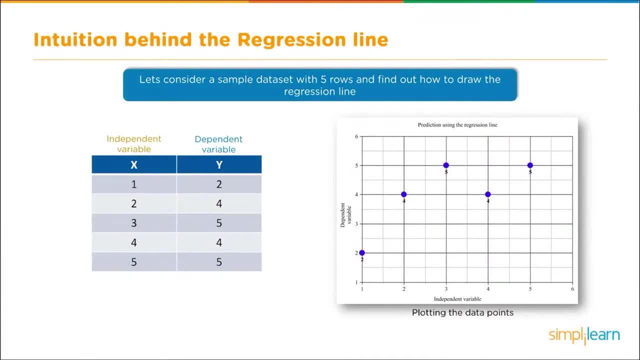 graph we can see how it forms a nice line through the middle. You can see where it's kind of grouped, going upwards to the right. The next thing we want to know is what the means is of each of the data coming in: the x and the y. The means: 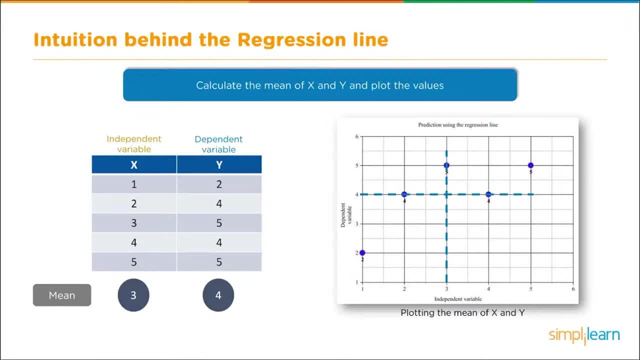 doesn't mean anything other than the average. so we add up all the numbers and divide by the total. so 1 plus 2 plus 3 plus 4 plus 5 over 5 equals 3, and the same for y, we get 4.. If we go ahead and plot the means on the, 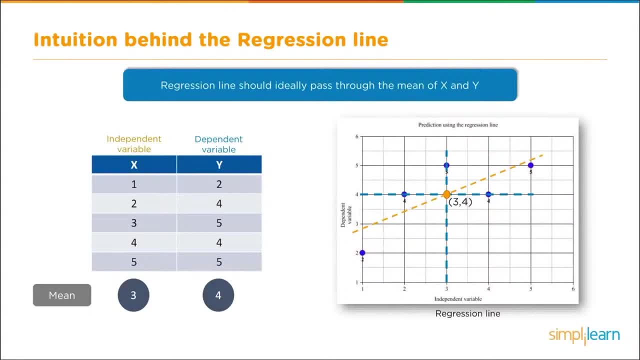 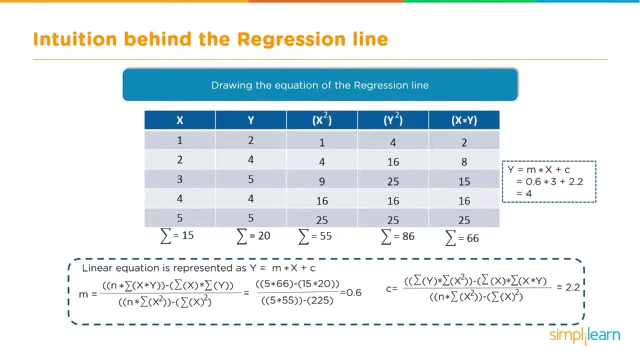 graph, we'll see we get 3 comma 4, which draws a nice line down the middle, A good estimate. Here we're going to dig deeper into the math behind the regression line. Now remember before I said you don't have to have all these formulas. 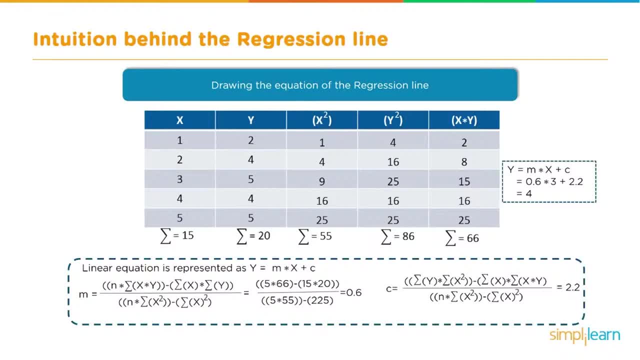 memorized or fully understand them, even though we're going to go into a little more detail of how it works. and if you're not a math whiz and you don't know if you've never seen the Sigma character before, which looks like a little bit like an e that's opened up. that just means summation, That's all. 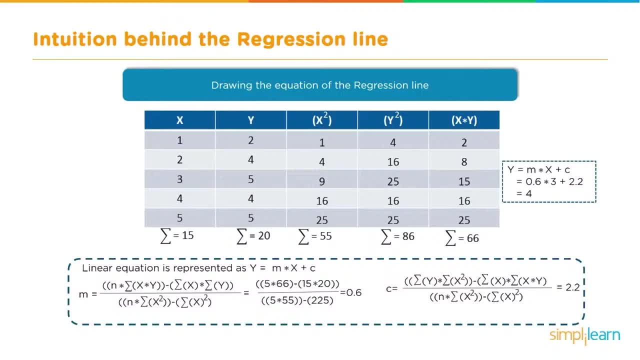 that is So. when you see the Sigma character, it just means we're adding everything in that row, And for computers this is great because as a programmer you can easily iterate through each of the xy points and create all the information you need. So in the top half you can see where we've broken that down. 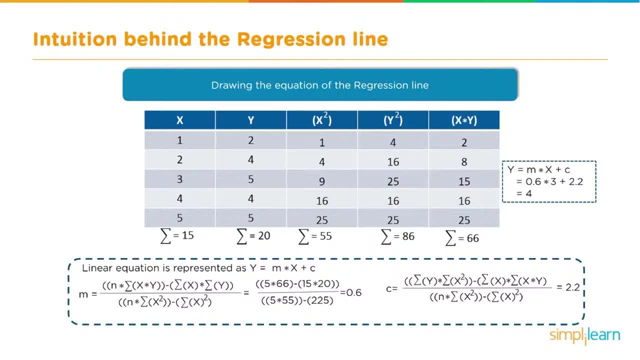 into pieces and as it goes through the first two points, it computes the squared value of x, the squared value of y and x times y, and then it takes all of x and adds them up, All of y, adds them up, All of x squared adds them up, and so on and so on, And you 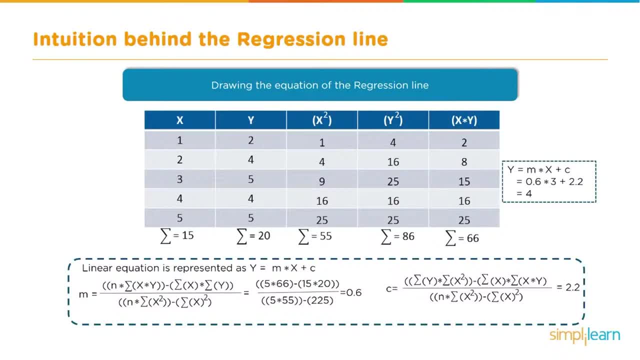 can see, we have the sum of equal to 15. the sum is equal to 20 all the way up to x times y, where the sum equals 66. This all comes from our formula for calculating a straight line where y equals the slope times x plus the. 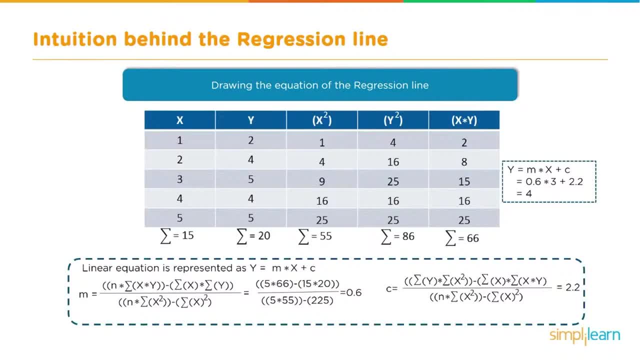 coefficient c. So we go down below and we're going to compute more like the averages of these and we'll explain exactly what that is in just a minute and where that information comes from is called the squared value. So we're going to do that in detail in a few minutes. All you need to do is look at. 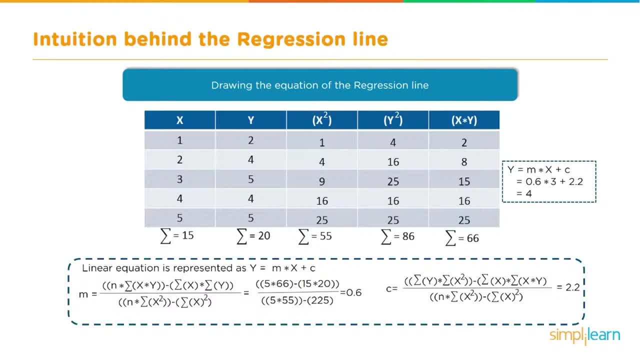 the formula and see how we've gone about computing it line by line instead of trying to have a huge set of numbers pushed into it. And down here you'll see where the slope m equals and the top part. if you read through the brackets, you have the number of data points times the sum of x times y, which we computed. 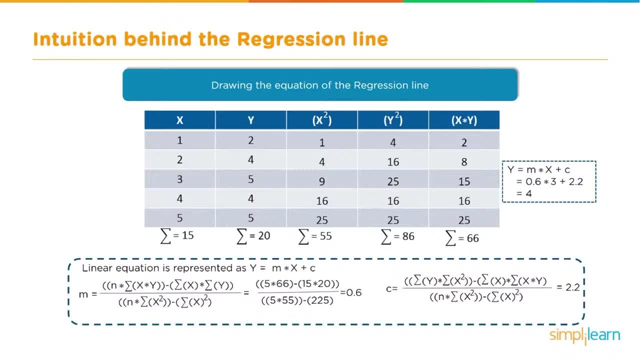 one line at a time there, and that's just the 66. And take all that and you subtract it from the sum of x times the sum of y, and those have both been computed. so you have 15 times 20, and on the bottom we: 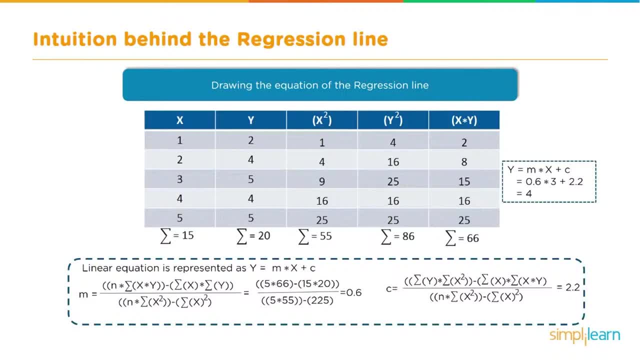 have the number of lines times the sum of x squared, easily computed as 86 for the sum minus. I'll take all that and subtract the sum of x squared and we end up as we come across with our formula. you can plug in all those numbers which. 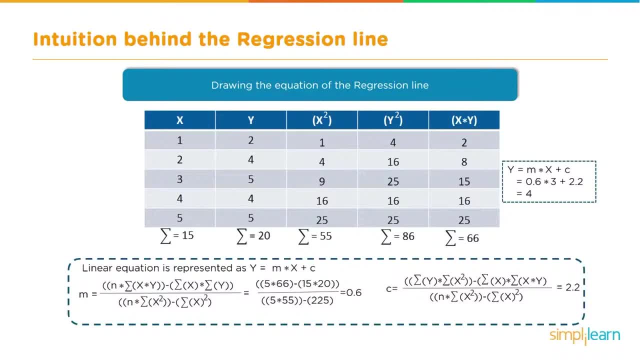 is very easy to do on the computer. you don't have to do the math on a piece of paper or calculator And you'll get a slope of 0.6 and you'll get your c coefficient. if you continue to follow through that formula, you'll see it comes out as equal to 2.2.. Continuing. 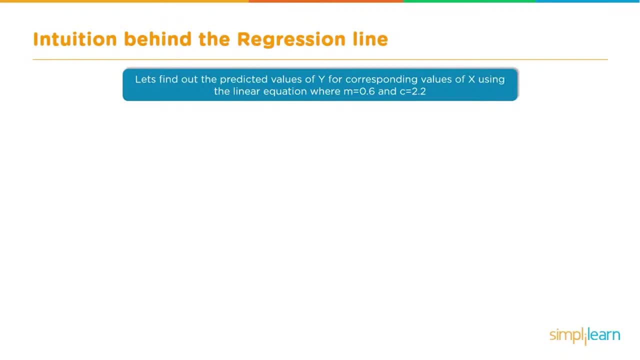 deeper into what's going behind the scenes. let's find out the predicted values of y for corresponding values of x using the linear equation where m equals 0.6 and c equals 2.2.. We're going to take these values and we're going to 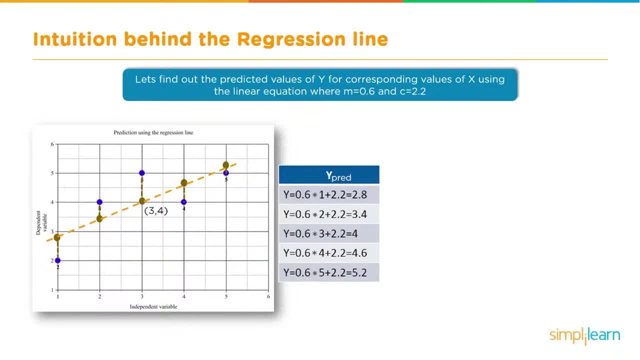 go ahead and plot them. we're going to predict them. so y equals 0.6 times where x equals 1 plus 2.2 equals 2.8.. So on and so on, and here the blue points represent the actual y values and the. 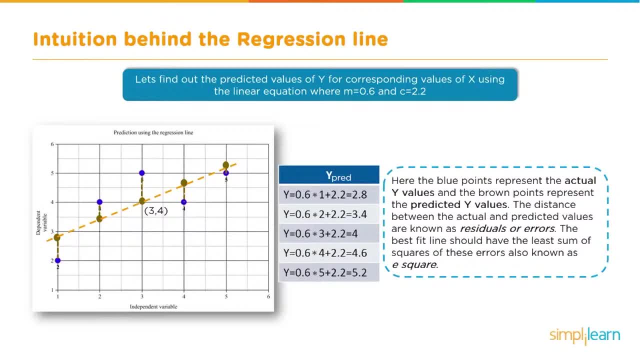 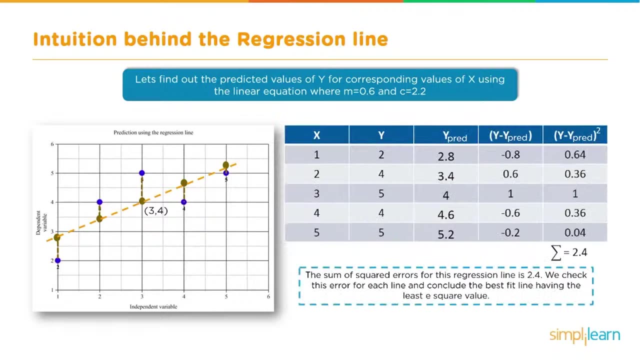 brown points represent the predicted y values based on the model we created. The distance between the actual predicted values is known as residuals or errors. The best fit line should have the least sum of squares of these errors, also known as e-square. If we put these into a nice chart, we can see x and you can see y. 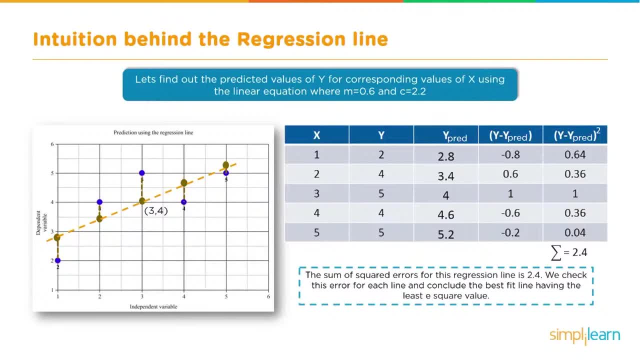 what we actual values were. You can see y predicted. You can easily see where we take y minus y predicted and we get an answer. What is the difference between those two? And if we square that y minus y prediction squared, we can then sum those squared values. That's where we get the 0.64 plus. 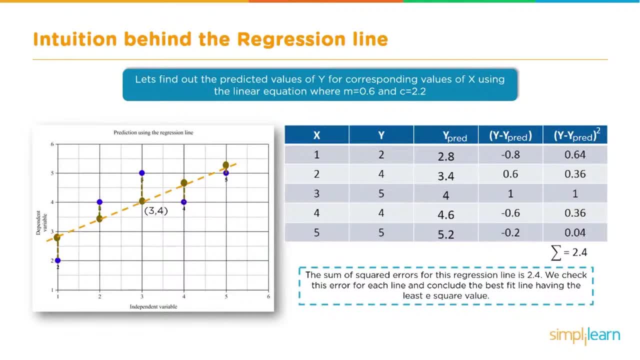 the 0.36 plus 1 all the way down until we have a summation equals 2.4.. So the sum of squared errors for this regression line is 2.4.. We check this error for each line and conclude the best fit line having the least e-square value In a. 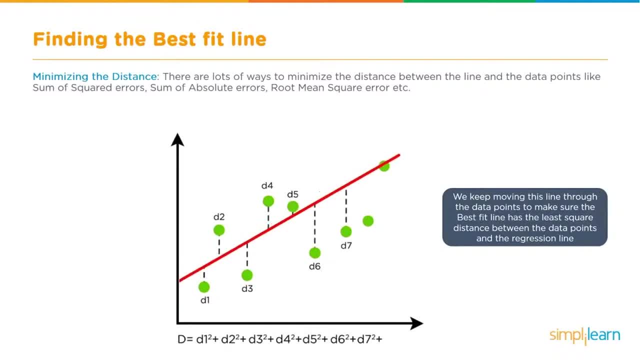 nice model representation. we can see here where we keep moving this line through the data points to make sure the best fit line has the least squared distance between the data points and the regression line. Now we only looked at the most commonly used formula for minimizing the distance. There are lots of ways to minimize the 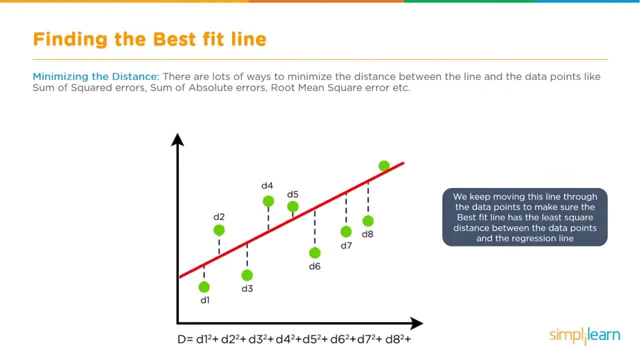 distance between the line and the data points, like sum of squared errors, sum of absolute errors, root mean, square error, etc. What you want to take away from this is, whatever formula being used, you can easily, using computer programming and iterating through the data, calculate the different parts of it. That way, these complicated formulas, you 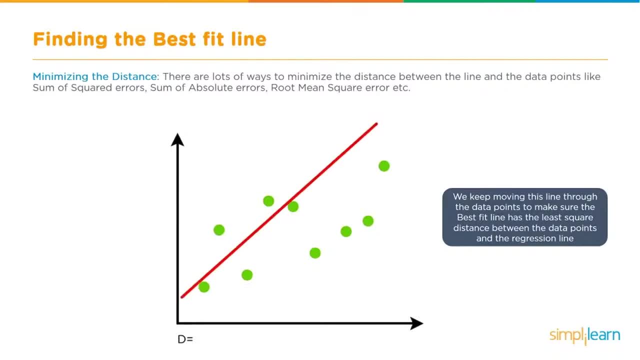 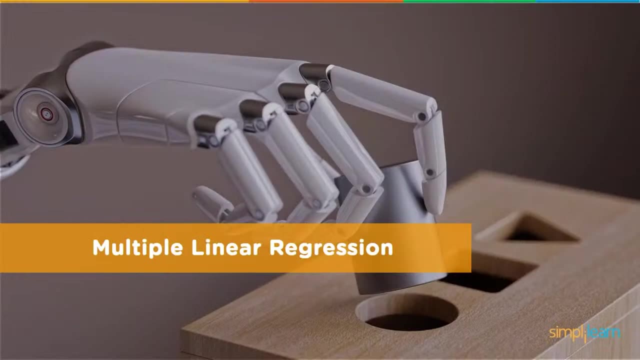 see with the different summations and absolute values are easily computed one piece at a time. Up until this point, we've only been looking at two values: x and y. well, in the real world is very rare that you only have two values when you're figuring out a solution. So let's move onto the next topic: Multiple linear regression. Let's take a brief. 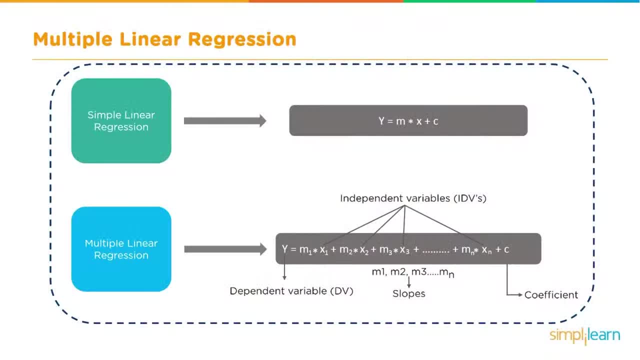 look at what happens when you have multiple inputs. So in multiple linear regression we have. well, we'll start with the simple linear regression where we had y equals m plus x plus c and we're trying to find the value of y. Now, with multiple linear regression, we have multiple variables. 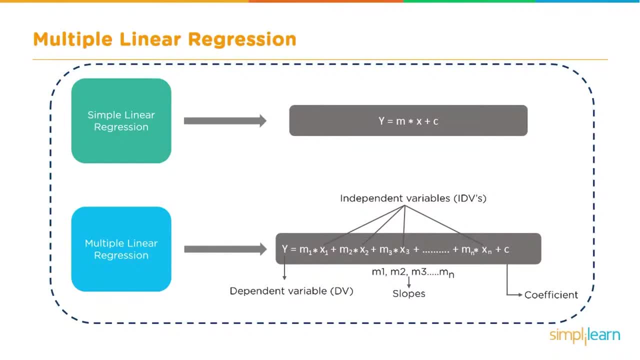 coming in. So instead of having just x, we have x1,, x2,, x3, and instead of having just one slope, each variable has its own slope attached to it. As you can see, here we have m1,, m2, m3 and we still. 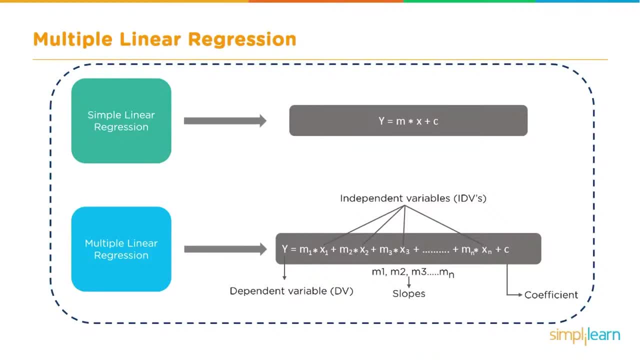 just have the single coefficient. So when you're dealing with multiple linear regression, you basically take your single linear regression and you spread it out, So you have y equals m1 times x1, plus m2 times x2, so on all the way to m to the nth, x to the nth, and then you add your coefficient. 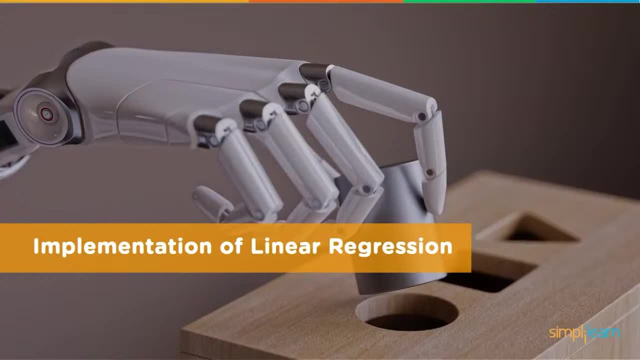 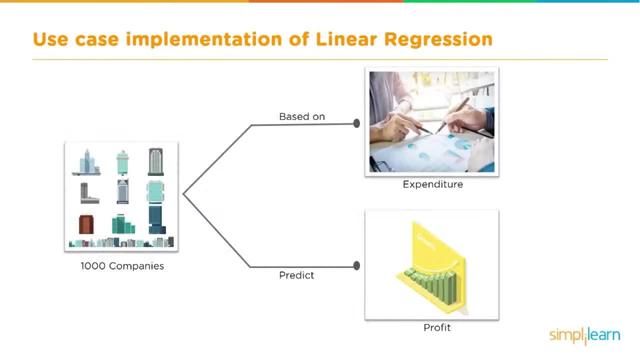 on there. Implementation of linear regression. Now we get into my favorite part. Let's understand how multiple linear regression works by implementing it in Python. If you remember, before we were looking at a company and, just based on its R&D, trying to figure out its profit. We're going to. 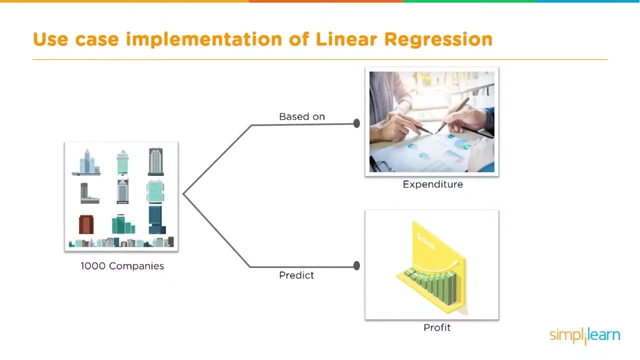 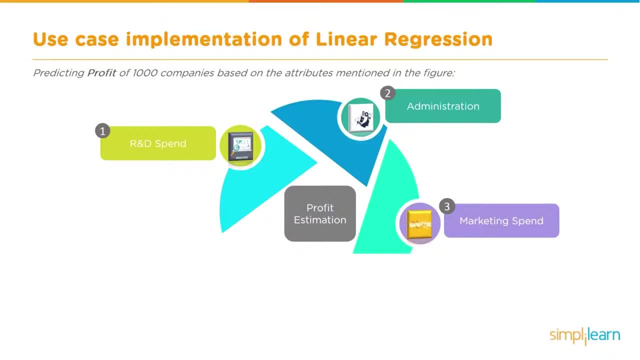 start looking at the expenditure of the company. We're going to go back to that. We're going to predict its profit. but instead of predicting it just on the R&D, we're going to look at other factors like administration costs, marketing costs and so on, and from there we're going to see if we 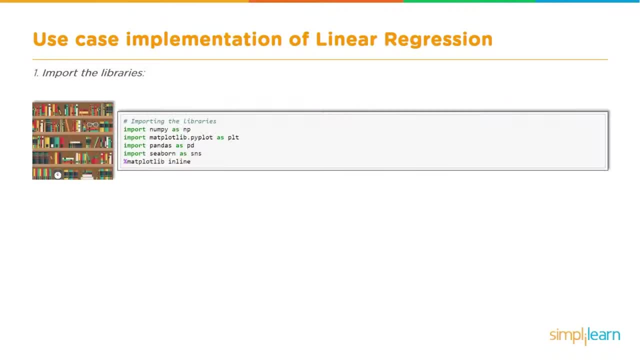 can figure out what the profit of that company is going to be. To start our coding, we're going to begin by importing some basic libraries and we're going to be looking through the data before we do any kind of linear regression. We're going to take a look at the data to see what 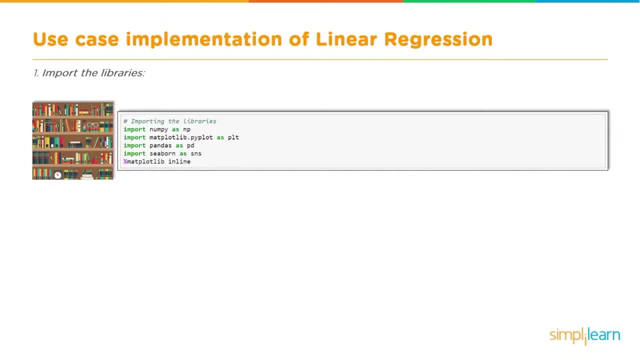 we're playing with. Then we'll go ahead and format the data to the format we need to be able to run it in the linear regression model and then from there we'll go ahead and solve it and just see how valid our solution is. So let's start with importing the basic libraries. Now I'm going to 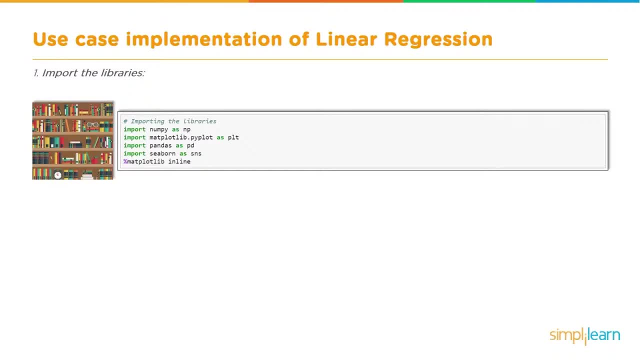 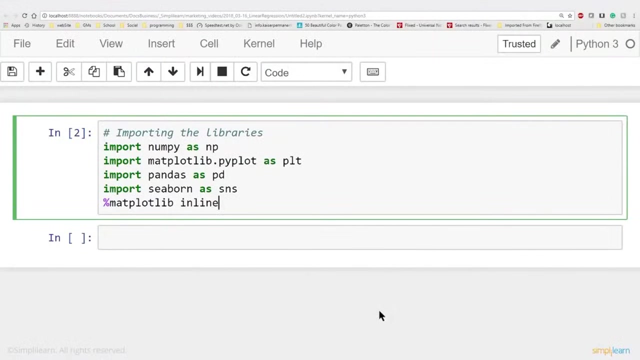 be doing this in Anaconda Jupyter Notebook, a very popular IDE. I enjoy it because it's such a visual to look at and it's so easy to use. Just any IDE for Python will work just fine for this, so break out your favorite Python IDE. So here we are in our Jupyter Notebook. Let me go ahead and paste our 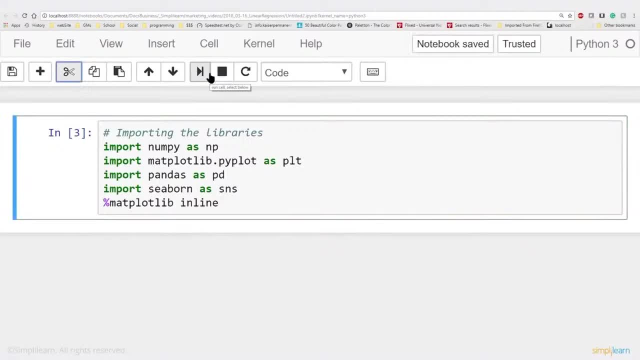 first piece of code in there and let's walk through what libraries we're importing. First we're going to import numpy as np and then I want you to skip one line and look at import pandas as pd. These are very common tools that you need with most of your linear regression. The numpy, which stands for: 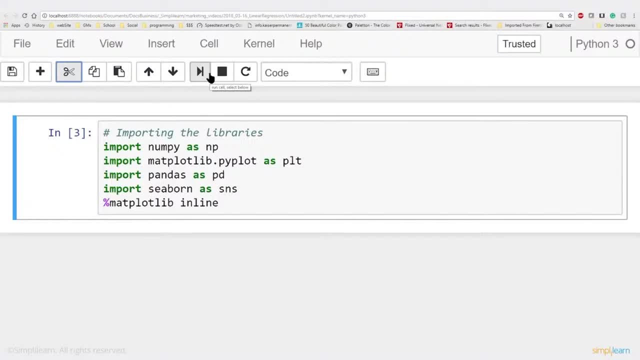 pd, and you have to almost have that for your sklearn toolbox. You always import that right off the beginning, Pandas. although you don't have to have it for your sklearn libraries, it does such a wonderful job of importing data, setting it up into a data frame so we can manipulate it rather. 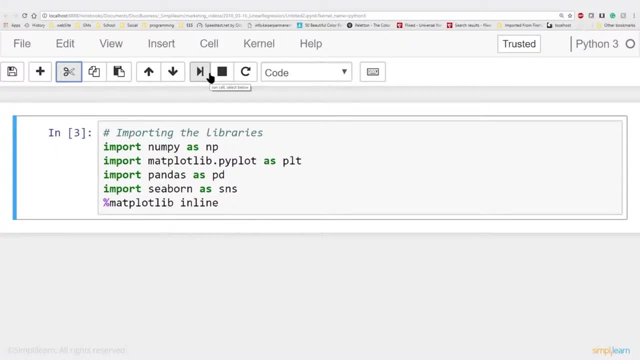 easily and it has a lot of tools also in addition to that. So we usually like to use the pandas when we can, and I'll show you what that looks like. The other three lines are for us to get a visual of this data and take a look at it. So we're going to import matplotlibrarypyplot as plt and then 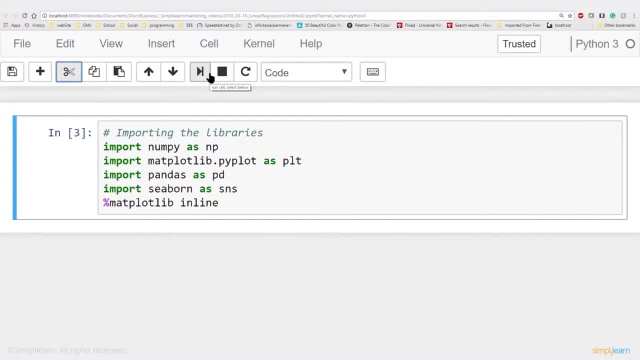 seaborn as sns. Seaborn works with the matplot library, so you have to always import matplot library and then seaborn sits on top of it And we'll take a look at what that looks like. You could use any of your own plotting libraries you want. There's all kinds of ways to look at the. 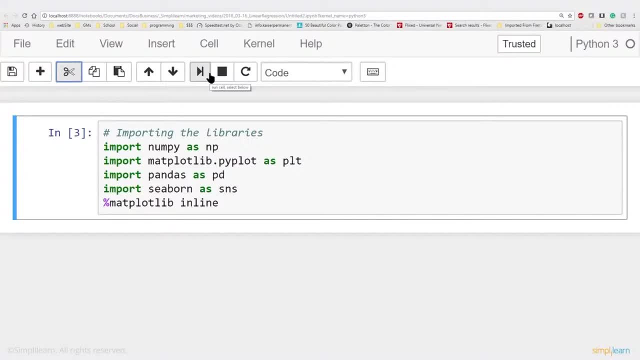 data. These are just very common ones and the seaborn is so easy to use that it just looks beautiful. It's a nice representation that you can actually take and show somebody. And the final line is the amberson matplotlibrary inline. That is only because I'm doing an inline IDE. My 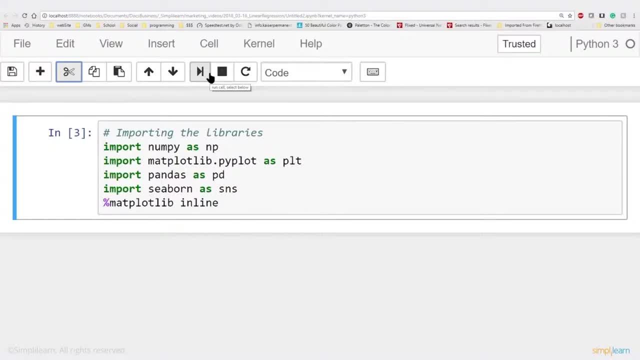 interface in the Anaconda Jupyter Notebook requires I put that in there or you're not going to see the graph when it comes up. Let's go ahead and run this. It's not going to be that interesting because we're just setting up variables. In fact, it's not going to do anything that we can see, but it is. 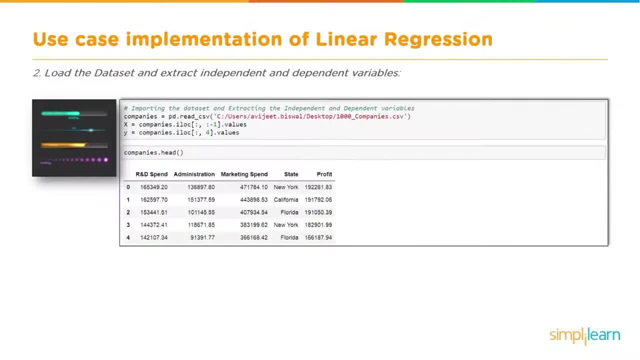 importing these different libraries and setup. The next step is load the data set and extract independent and dependent variables. Now here in the slide you'll see companies equals pdreadcsv, and it has a long line there with the file at the end 1000companiescsv. You're going to have to change this to fit whatever setup you. 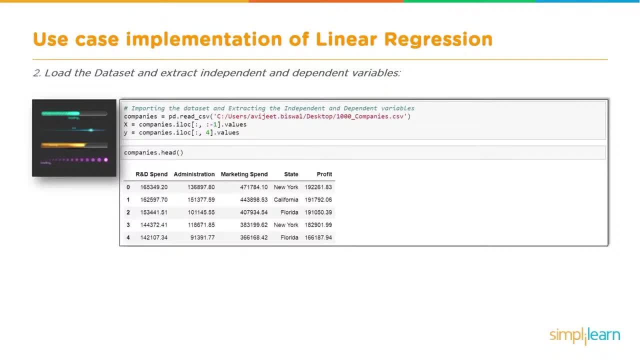 have And the file itself you can request. Just go down to the commentary below this video and put a note in there and Simply Learn will try to get in contact with you and supply you with that file so you can try this coding yourself. So we're going to add this code in here and we're going to see 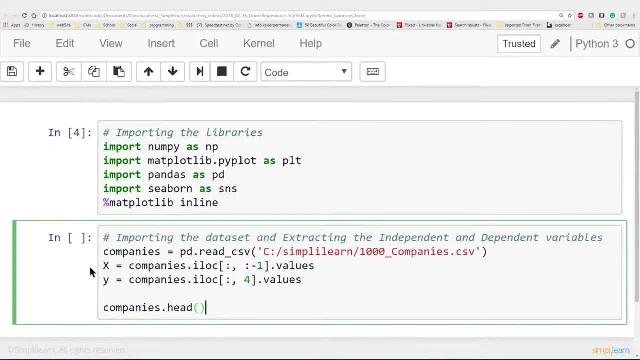 that I have companies equals pdreadcsv And I've changed this path to match my computer C colon slash, simply learn: slash 1000 underscore companies dot csv And then below there we're going to set the x equals to companies under the i location And because this is companies is a pd data set, I can use this nice. 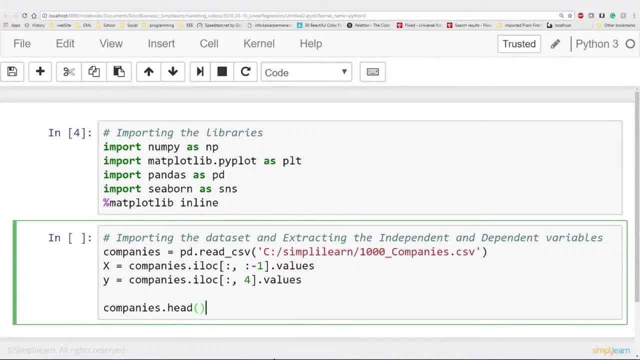 notation that says: take every row. that's what the colon, the first colon, is comma, except for the last column. That's what the second part is, where we have a colon minus one And we want the values set into there. So this is no longer a data set, a pandas data set, But we can easily extract the data from our pandas data set with this notation. 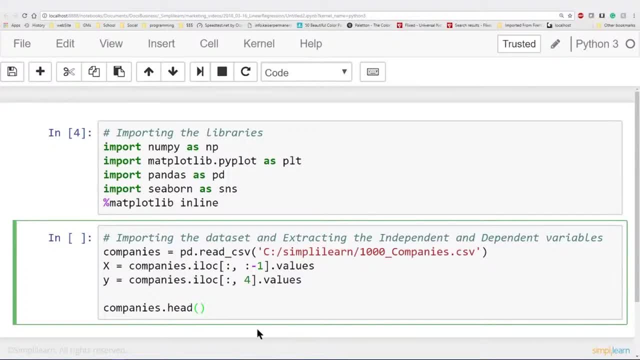 And then y we're going to set equal to the last row. Well, the question is going to be: what are we actually looking at? So let's go ahead and take a look at that, And we're going to look at the companies dot head, which lists the first five rows of data. 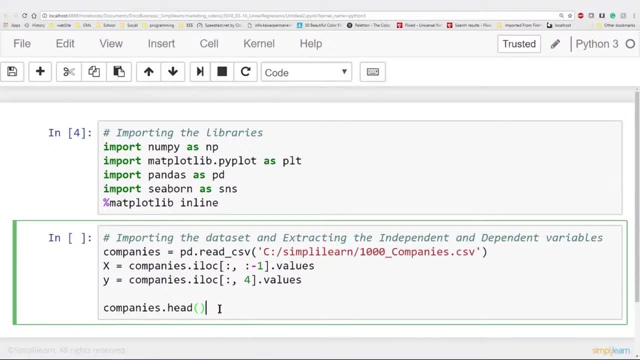 And I'll open up the file in just a second so you can see where that's coming from. But let's look at the data in here. as far as the way the pandas sees it, When I hit run, you'll see it breaks it out into a nice setup. 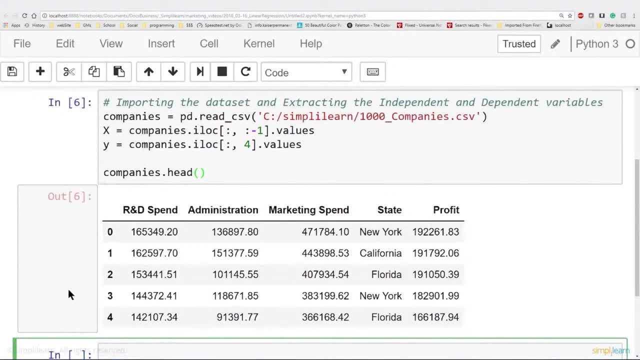 This is what pandas- one of the things pandas is really good about- is it looks just like an Excel spreadsheet. You have your rows And remember, when we're programming, we always start with zero, We don't start with one. So it shows the first five rows- Zero: one, two, three, four- And then it shows your different columns. 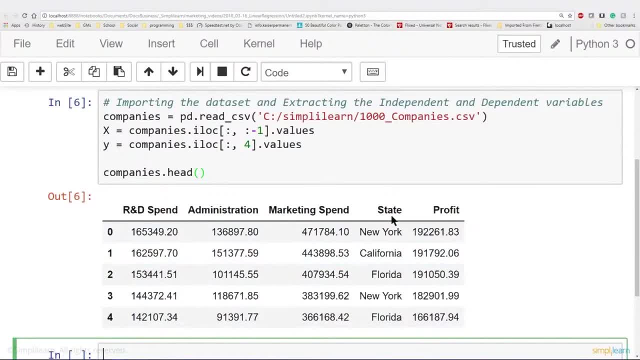 R&D spend, administration, marketing spend, state profit. It even notes that the top are column names. It was never told that, but pandas is able to recognize a lot of things that they're not the same as the data rows. Why don't we go ahead and open this file up in a CSV so you can actually see the raw data? 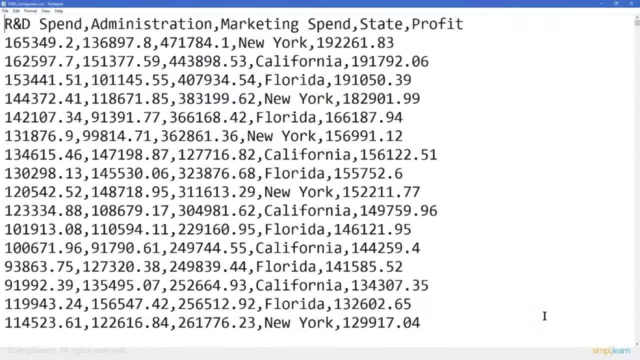 So here I've opened it up as a text editor And you can see at the top we have R&D spend, administration, marketing, spend, state, profit, carries, return. I don't know about you, but I'd go crazy trying to read files like this. That's why we use the pandas. 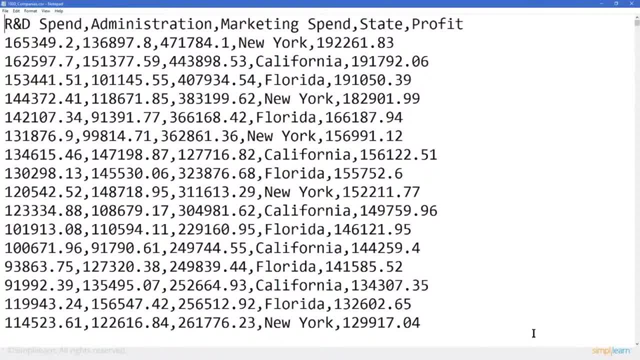 You could also open this up in an Excel and it would separate it, since it is a comma separated variable file. But we don't want to look at this one. We want to look at something we can read rather easily. So let's flip back and take a look at that. 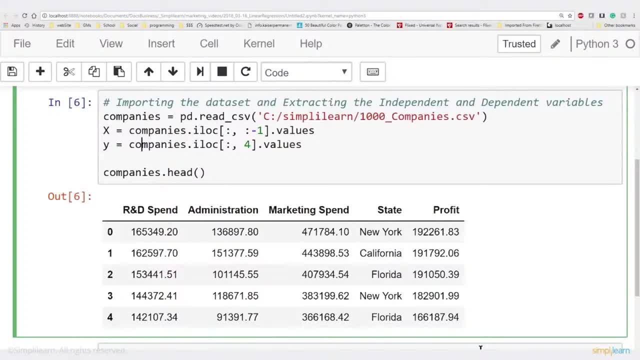 Top part, the first five rows. Now, as nice as this format is where you can see the data, to me it doesn't mean a whole lot. Maybe you're an expert in business and investments and you understand what. $165,349.20 compared to the administration cost of $136,897.80. so on, so on. 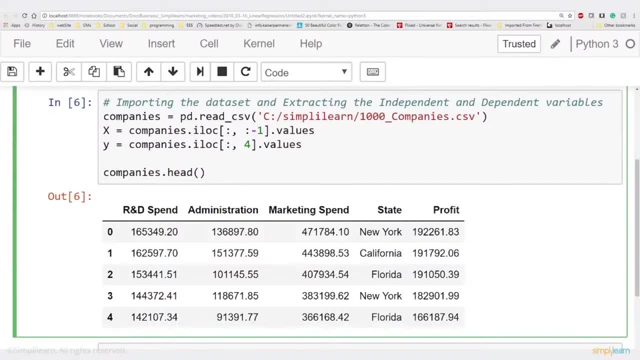 It helps to create the profit of $192,261.83.. That makes no sense to me whatsoever, No pun intended. So let's flip back here and take a look at our next set of code, where we're going to graph it, so we can get a better understanding of our data and what it means. 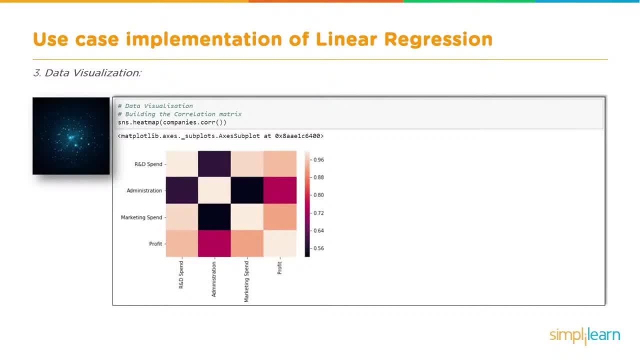 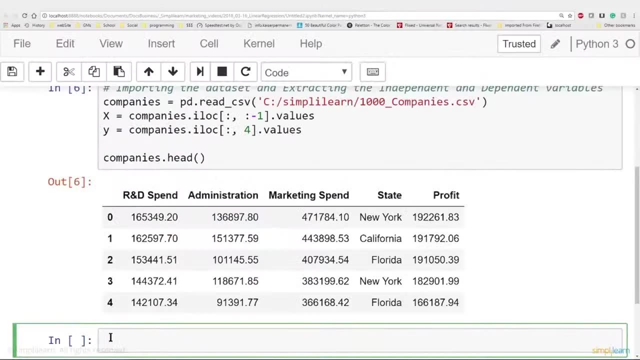 So at this point we're going to use a single line of code to get a lot of information so we can see where we're going with this. Let's go ahead and paste that into our notebook and see what we got going. And so we have the visualization. and again we're using SNS, which is pandas. 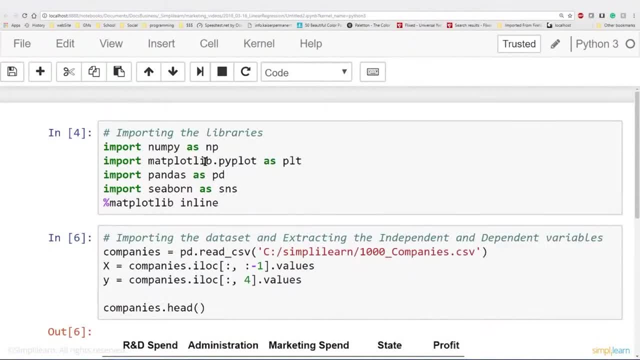 As you can see, we imported the matplotlibrarypyplot as PLT, Which then we're going to use as a reference, And we imported the seaborn as SNS, And then that final line of code helps us show this in our inline coding. Without this it wouldn't display and you could display it to a file and other means. 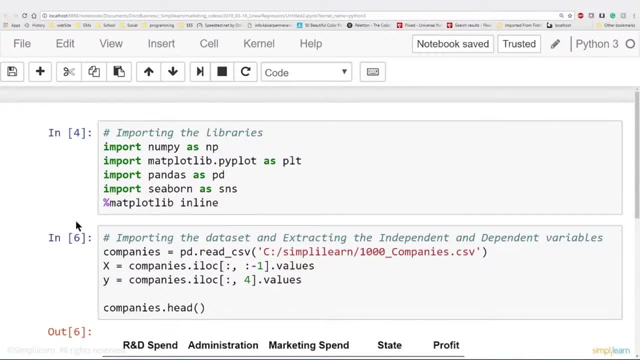 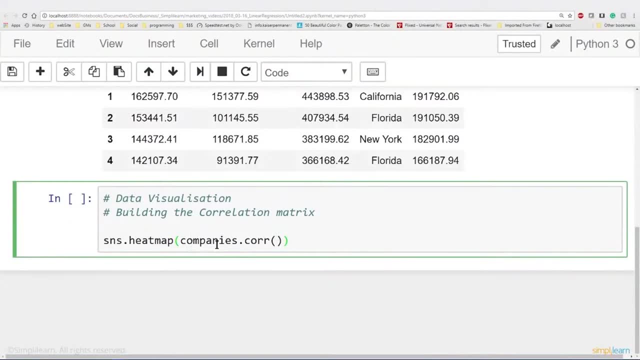 And that's the matplotlibrary inline with the amber sign at the beginning. So here we come down to the single line of code. Seaborn is great because it actually recognizes the panda data frame, So I can just take the companiescore for coordinates. 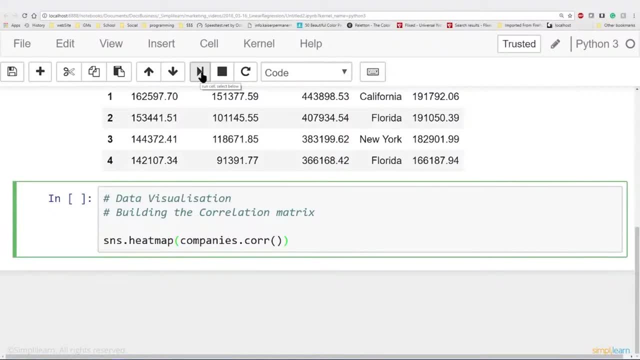 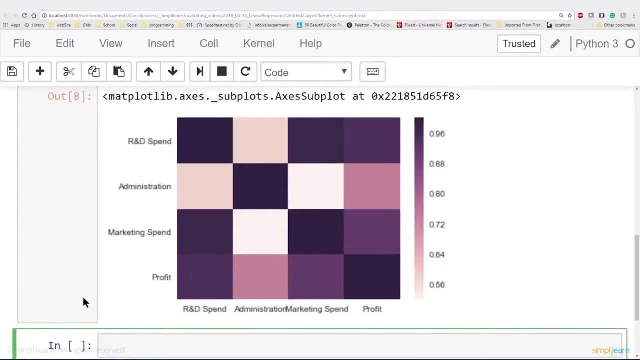 And I can put that right into the seaborn. And when we run this we get this beautiful plot. And let's just take a look at what this plot means. If you look at this plot on mine, the colors are probably a little bit more purplish and blue than the original one. 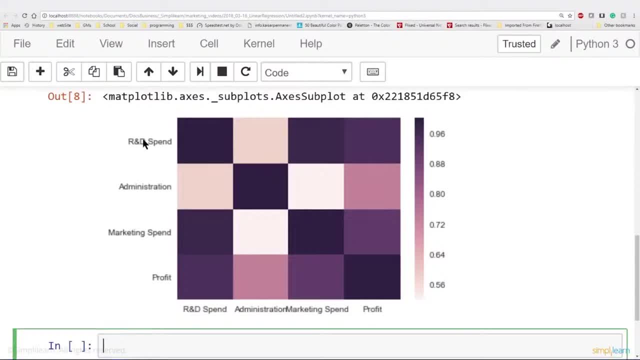 We have the columns and the rows, We have R and D spending, We have administration, We have marketing spending and profit. And if you cross index any two of these- since we're interested in profit- If you cross index profit with profit, it's going to show up. if you look at the scale on the right way up in the dark. 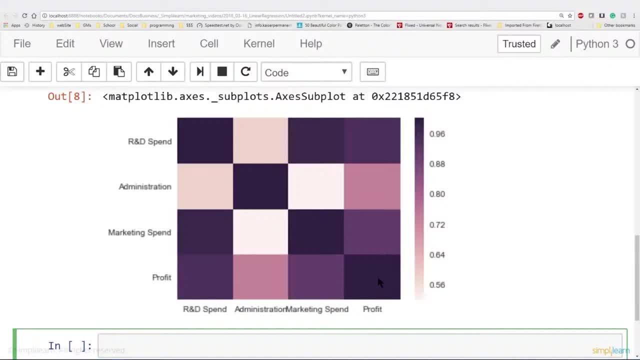 Why? Because those are the same data. They have an exact correspondence. So R and D spending is going to be the same as R and D spending and the same thing with administration costs. So right down the middle you get this dark row, or dark diagonal row that shows that this is the highest corresponding data. 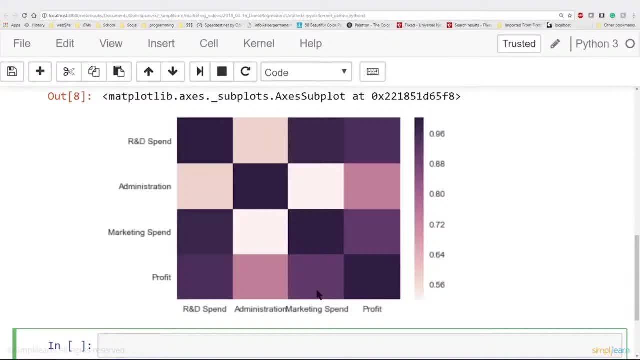 That's exactly the same And as it becomes lighter there's less connections between the data. So we can see: with profit, obviously profit is the same as profit. And next it has a very high correlation with R and D spending, which we looked at earlier. 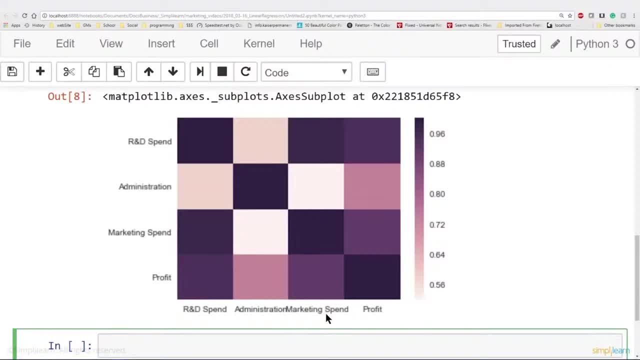 And it has a slightly less connection to marketing spending and even less to how much money we put into the administration. So now that we have a nice look at the data, let's go ahead and dig in and create some actual useful linear regression models So that we can predict values and have a better profit. 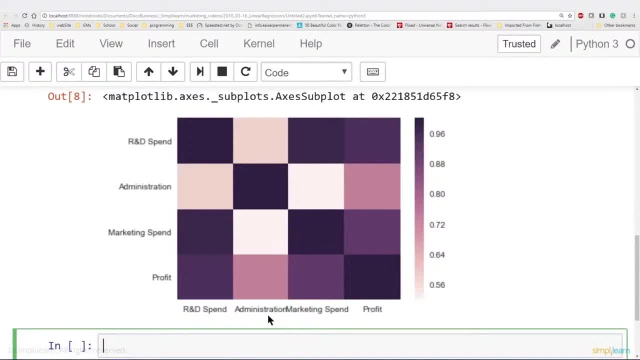 Now that we've taken a look at the visualization of this data, we're going to move on to the next step. Instead of just having a pretty picture, We need to generate some hard data, some hard values. So let's see what that looks like. 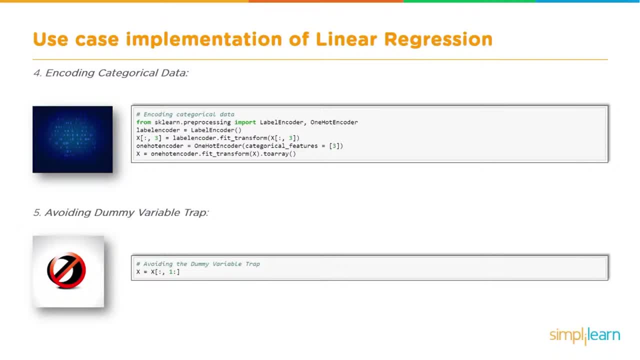 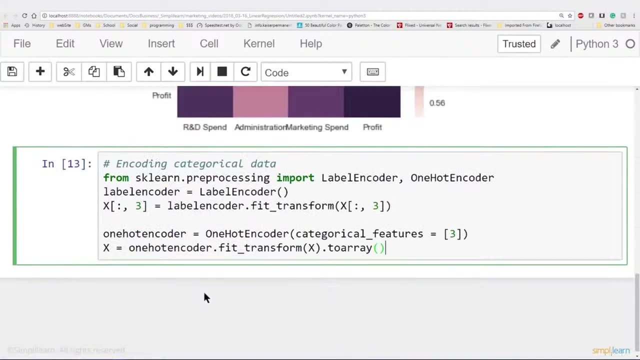 We're going to set up our linear regression model in two steps. The first one is we need to prepare some of our data so it fits correctly, And let's go ahead and paste this code into our Jupyter notebook, And what we're bringing in is we're going to bring in the sklearn preprocessing. 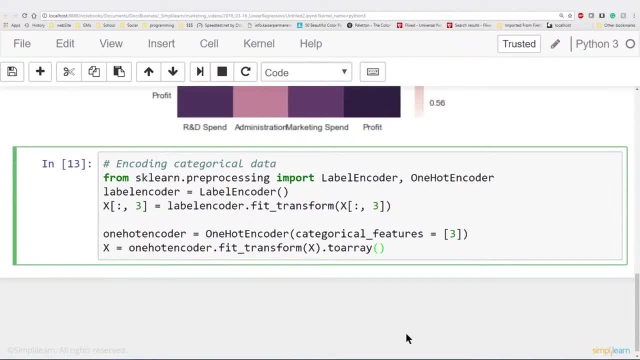 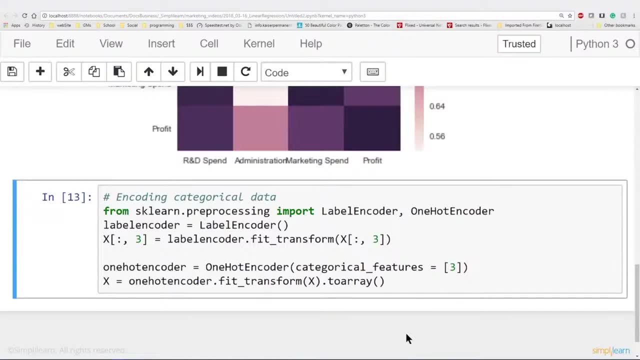 Where we're going to import the label encoder and the one hot encoder. To use the label encoder, we're going to create a variable called label encoder And set it equal to capital L Label, capital E encoder. This creates a class that we can reuse for transferring the labels back and forth. 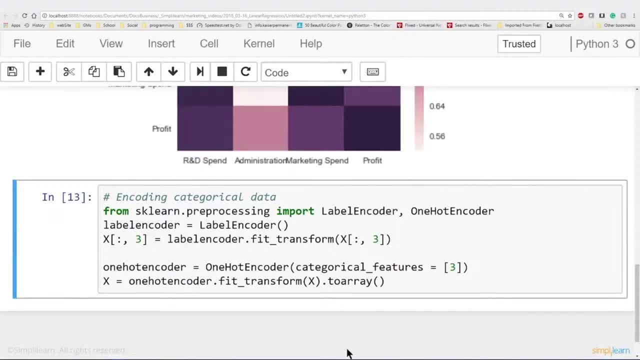 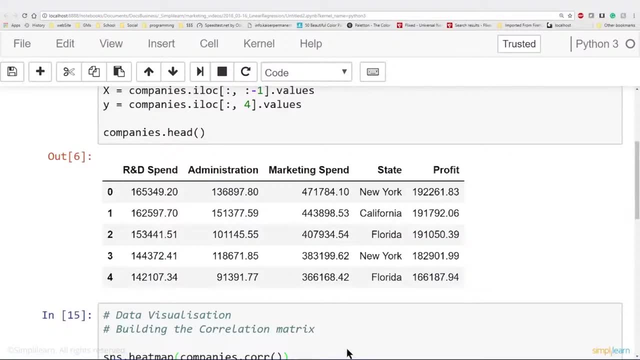 Now about now, you should ask: what labels are we talking about? Let's go take a look at the data we processed before and see what I'm talking about here. If you remember when we did the companies dot head and we printed the top five rows of data, 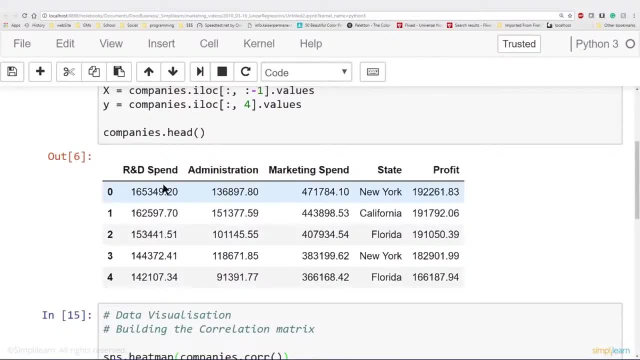 We have our columns going across. We have column 0, which is R&D spending, Column 1, which is administration, Column 2, which is marketing spending, And column 3 is state And you'll see under state we have New York, California, Florida. 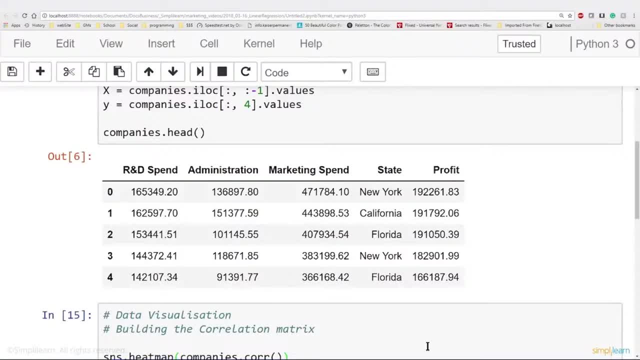 Now to do a linear regression model. it doesn't know how to process New York. It knows how to process a number. So the first thing we're going to do is we're going to change that- New York, California and Florida- And we're going to change those to numbers. 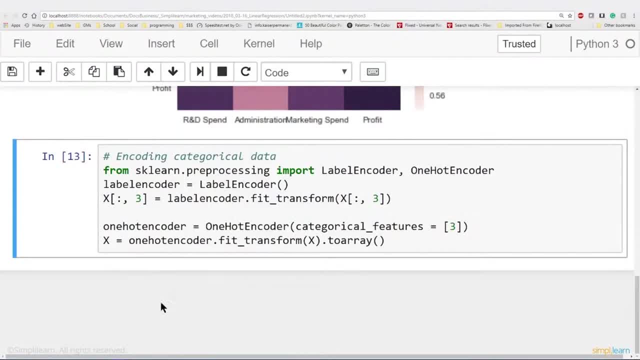 That's what this line of code does here X equals, and then it has the colon comma 3 in brackets. The first part. the colon comma, means that we're going to look at all the different rows, So we're going to keep them all together. 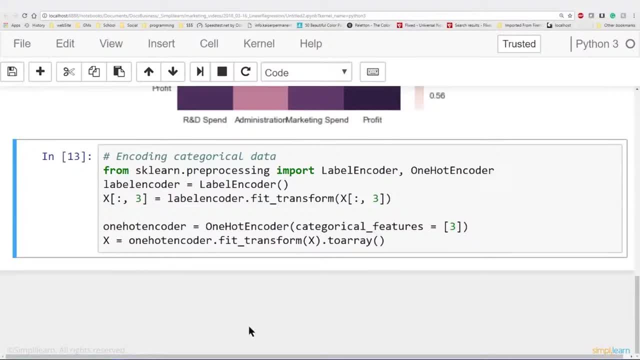 But the only row we're going to edit Is the third row And in there we're going to take the label coder And we're going to fit and transform the X, also the third row. So we're going to take that third row and we're going to set it equal to a transformation. 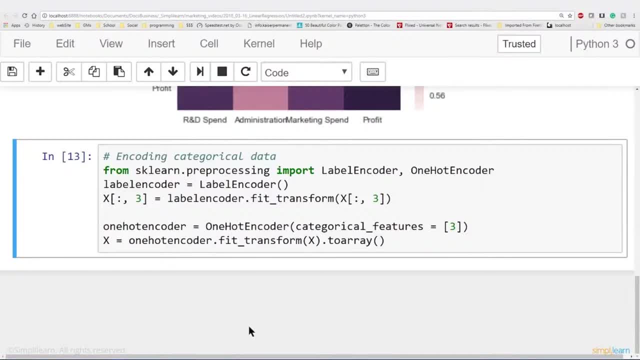 And that transformation basically tells it that instead of having a New York, it has a 0 or a 1 or a 2.. And then, finally, we need to do a one hot encoder Which equals one hot encoder. categorical features equals 3.. And then we take the X and we go ahead and do that equal to one hot encoder. 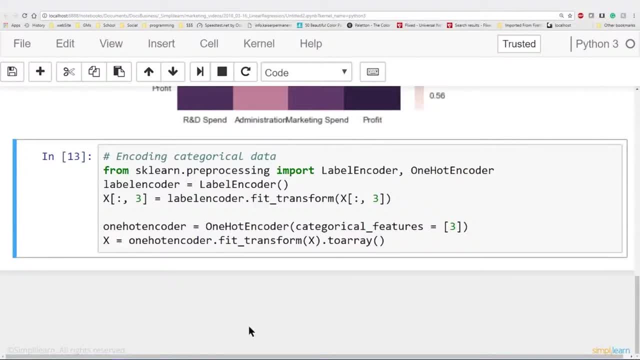 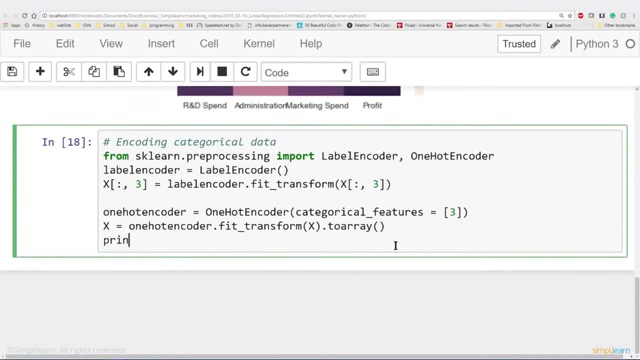 Fit. transform X to array. This final transformation preps our data for us, So it's completely set the way we need it. It's just a row of numbers. Even though it's not in here, Let's go ahead and print X. 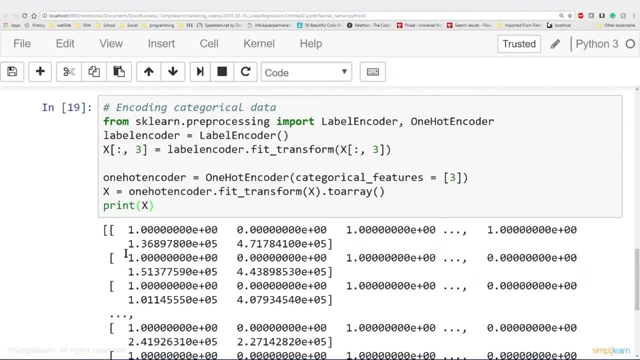 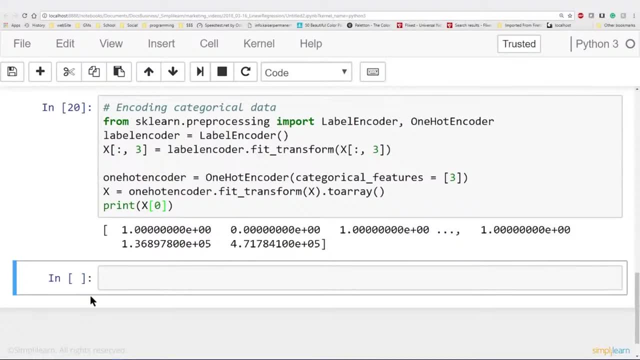 And just take a look at what this data is doing, You'll see you have an array of arrays And then each array is a row of numbers. And if I go ahead and just do row 0. You'll see I have a nice organized row of numbers that the computer now understands. 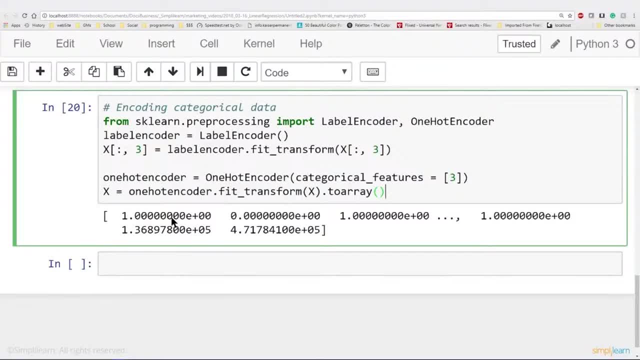 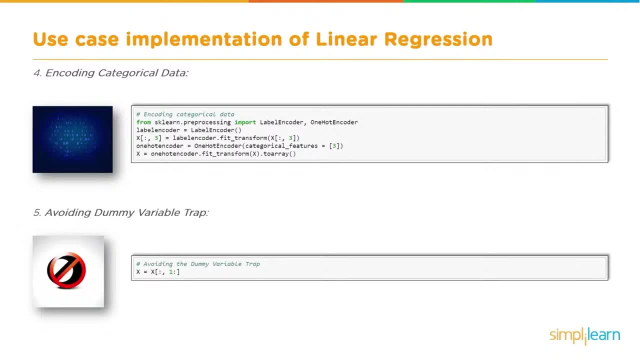 We'll go ahead and take this out there, because it doesn't mean a whole lot to us. It's just a row of numbers. Next, on setting up our data, We have avoiding dummy variable trap. This is very important. Why? Because the computer has automatically transformed our header into the setup. 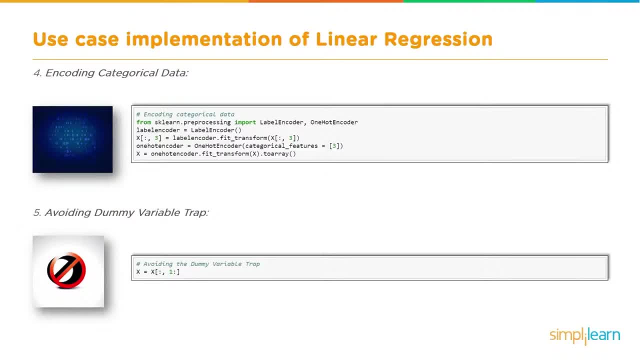 And it's automatically transformed all these different variables. So when we did the encoder, The encoder created two columns And what we need to do is just have the one, Because it has both the variable and the name. That's what this piece of code does here. 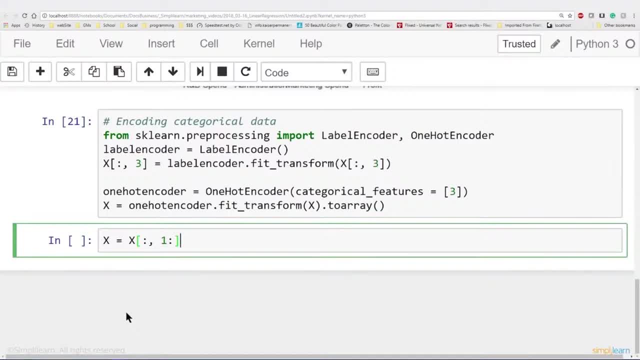 Let's go ahead and paste this in here And we have x equals x, colon, comma, one colon. All this is doing is removing that one extra column we put in there when we did our one hot encoder and our label encoding. Let's go ahead and run that. 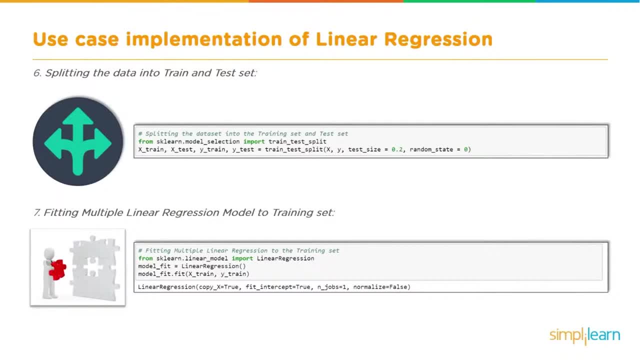 And now we get to create our linear regression model And let's see what that looks like here, And we're going to do that in two steps. The first step is going to be in splitting the data Now, whenever we create a predictive model of data, 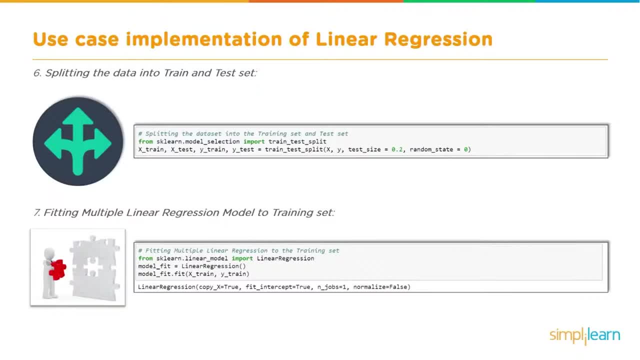 We always want to split it up. so we have a training set And we have a testing set. That's very important. Otherwise we'd be very unethical without testing it to see how good our fit is, And then we'll go ahead and create our multiple linear regression model. 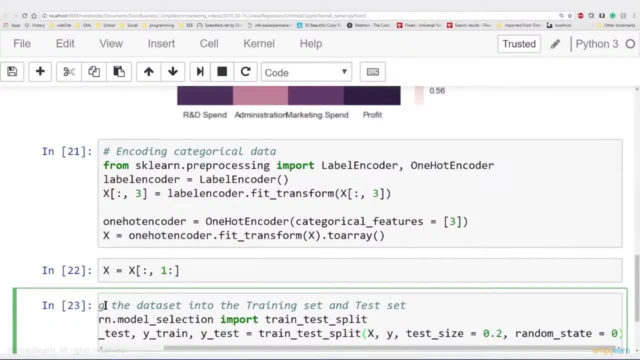 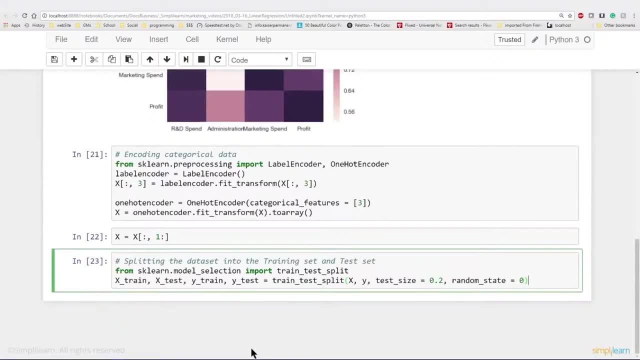 And train it and set it up. Let's go ahead and paste this next piece of code in here And I'll go ahead and shrink it down a size or two So it all fits on one line. So from the sklearn module selection. 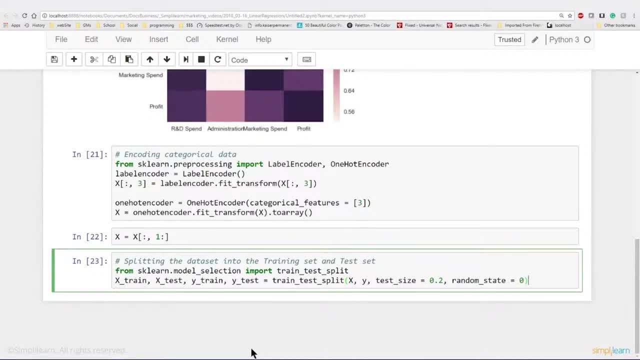 We're going to import train test split And you'll see that we've created four completely different variables. We have capital X train. Capital X test. Smaller case Y train. Smaller case Y test. That is the standard way that they usually reference these. 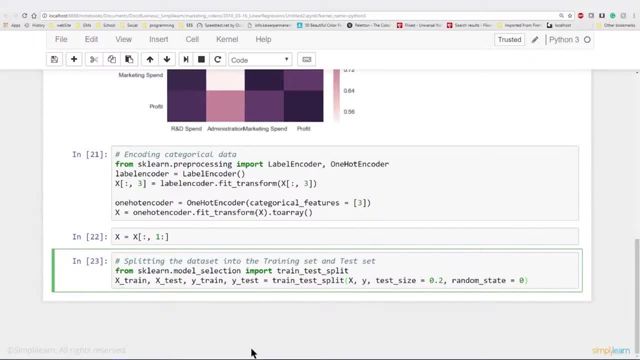 When we're doing different models, You usually see that at capital X You see the train and the test and the lower case Y. What this is is: X is our data going in, That's our R&D spin, our administration, our marketing. 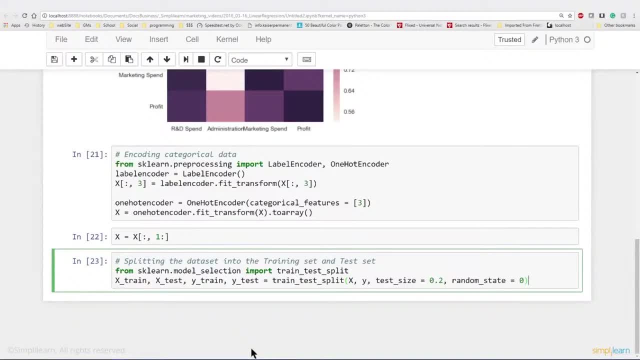 And then Y, which we're training, is the answer. That's the profit, Because we want to know the profit of an unknown entity. That's what we're going to shoot for in this tutorial. The next part: train test split. 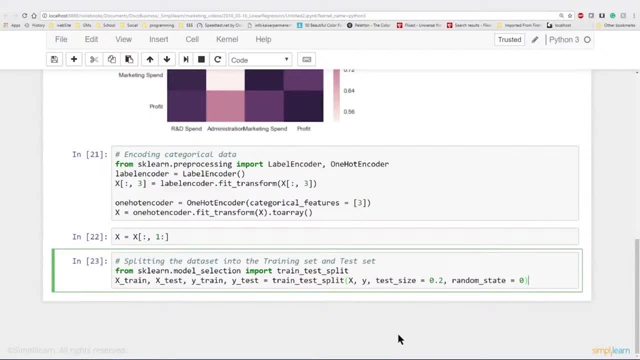 We take X and we take Y. We've already created those. X has the columns with the data in it And Y has a column with profit in it, And then we're going to set the test size equals .2.. That basically means 20%. 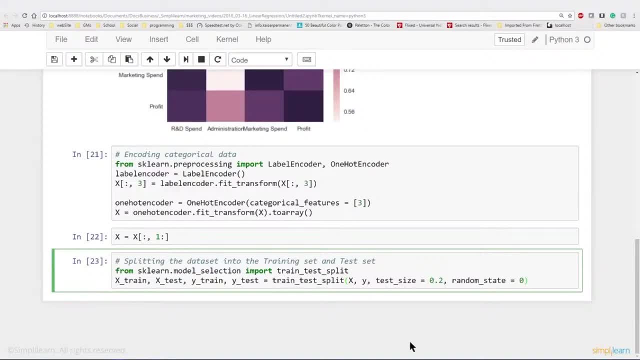 So 20% of the rows are going to be tested. We're going to put them off to the side. So, since we're using a thousand lines of data, That means that 200 of those lines We're going to hold off to the side to test for later. 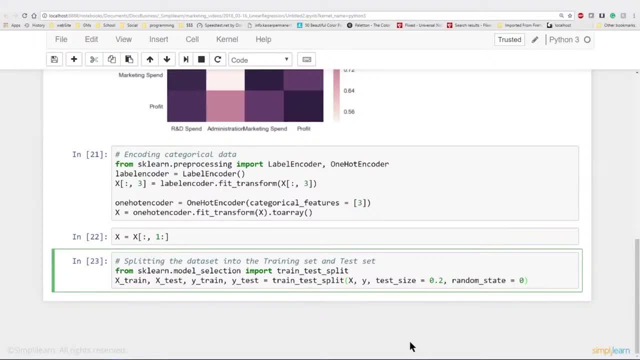 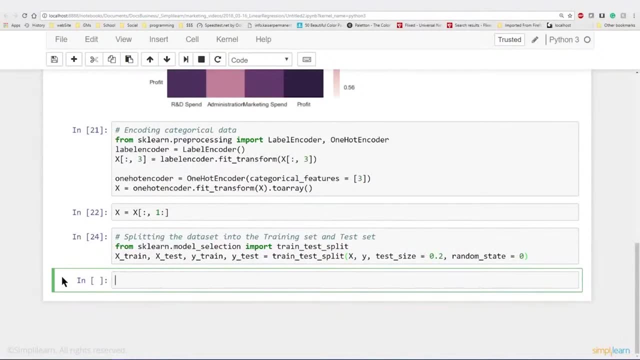 And then the random state equals zero. We're going to randomize which ones it picks to hold off to the side. We'll go ahead and run this. It's not overly exciting because it's setting up our variables. But the next step is. 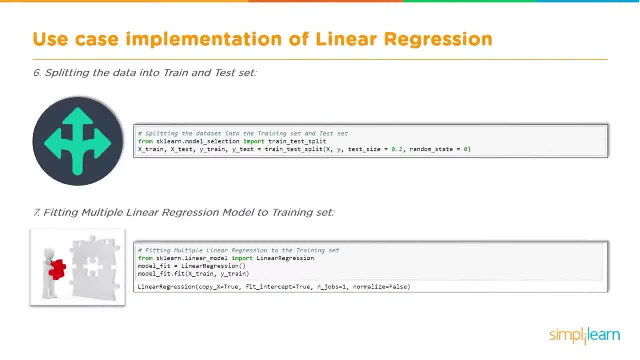 The next step: we actually create our linear regression model. Now that we got to the linear regression model, We get that next piece of the puzzle. Let's go ahead and put that code in there and walk through it. So here we go. 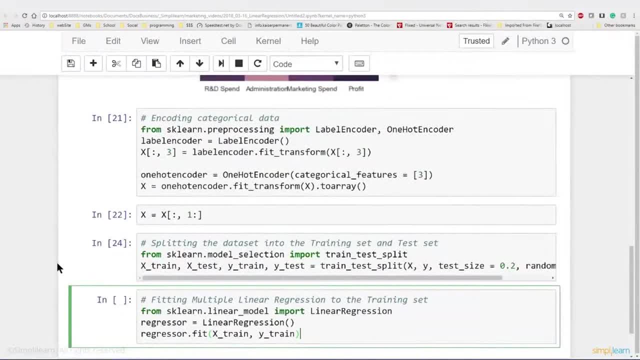 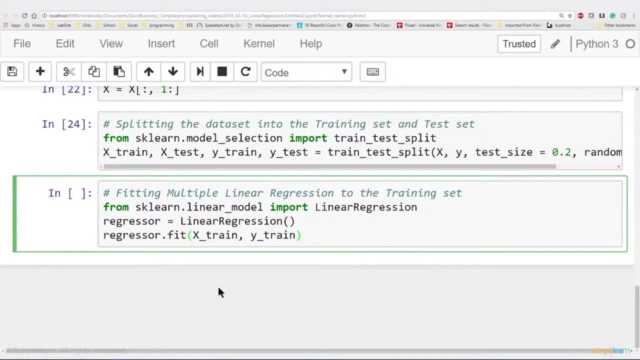 We're going to paste it in there And let's go ahead. and since this is a shorter line of code, Let's zoom up there so we can get a good look. And we have from the sklearnlinear underscore model, We're going to import linear regression. 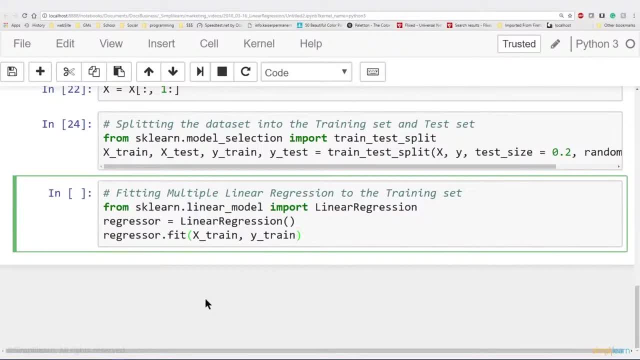 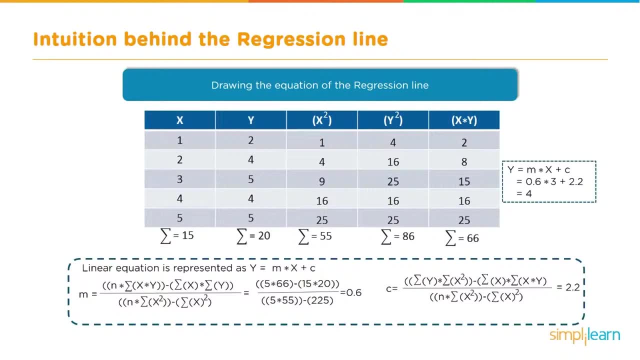 Now, I don't know if you recall from earlier When we were doing all the math. Let's go ahead and flip back there and take a look at that. Do you remember this Where we had this long formula on the bottom And we were doing all this sumization? 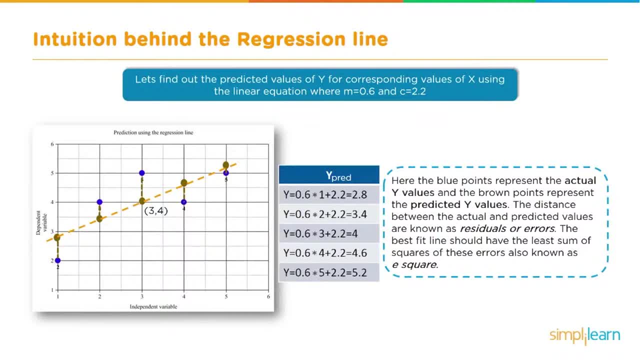 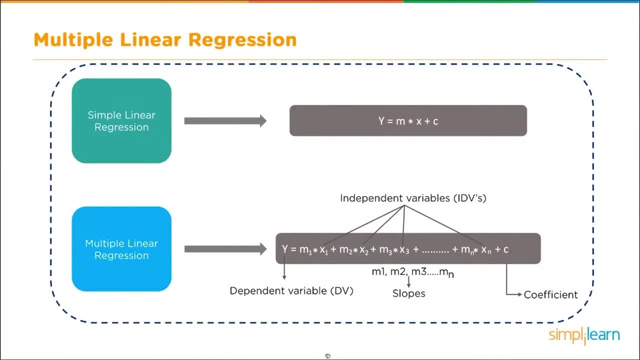 And then we also looked at setting it up with the different lines, And then we also looked all the way down to multiple linear regression, Where we're adding all those formulas together. All of that is wrapped up in this one section. So what's going on here? 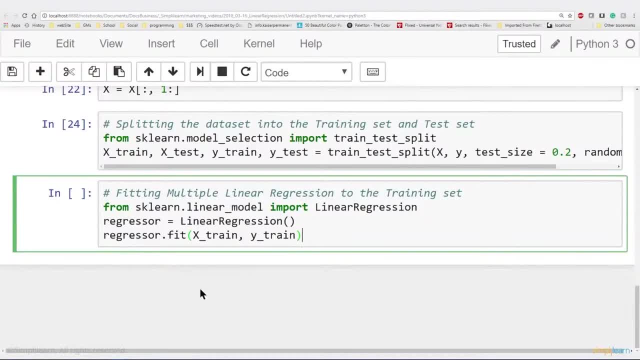 I'm going to create a variable called regressor, And the regressor equals the linear regression. That's the linear regression model That has all that math built in, So we don't have to have it all memorized or have to compute it individually. 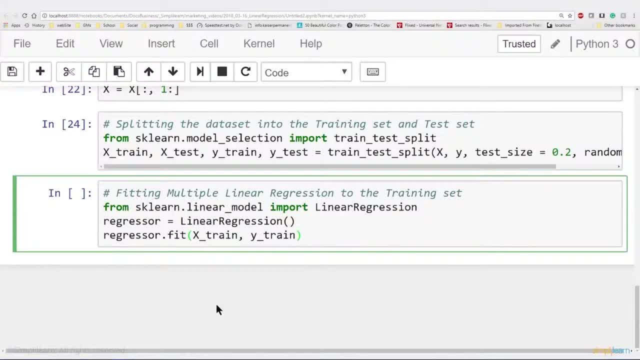 And then we do the regressorfit. In this case, we do X train and Y train, Because we're using the training data, X being the data in and Y being profit, What we're looking at- And this does all that math for us. 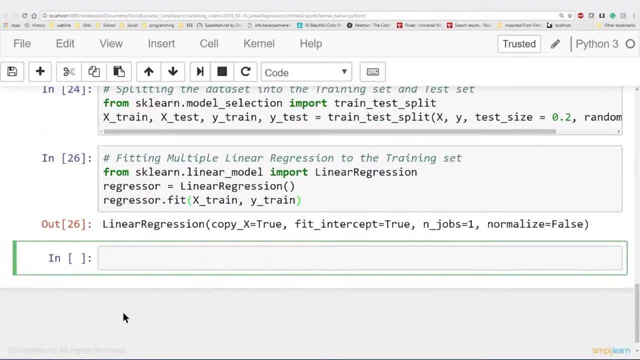 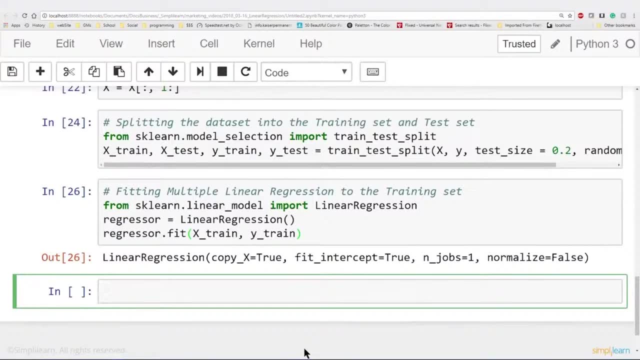 So within one click and one line We've created the whole linear regression model And we fit the data to the linear regression model And you can see that when I run the regressor It gives an output Linear regression. It says copy X equals true. 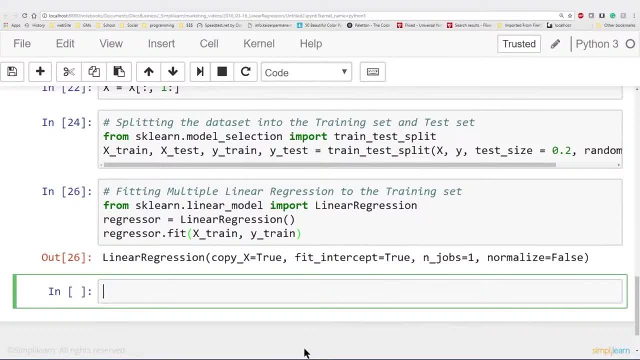 Fit intercept equals true. In jobs equals one. Normalize equals false. It's just giving you some general information On what's going on with that regressor model. Now that we've created our linear regression model, Let's go ahead and use it. 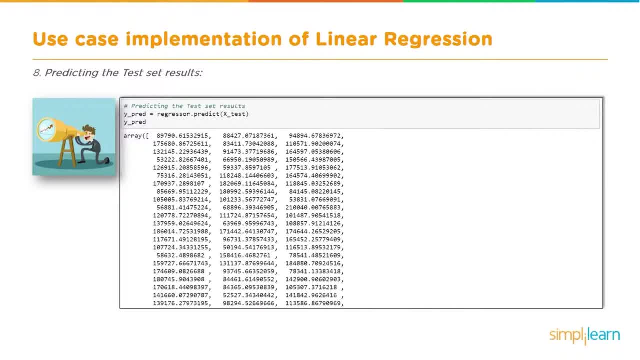 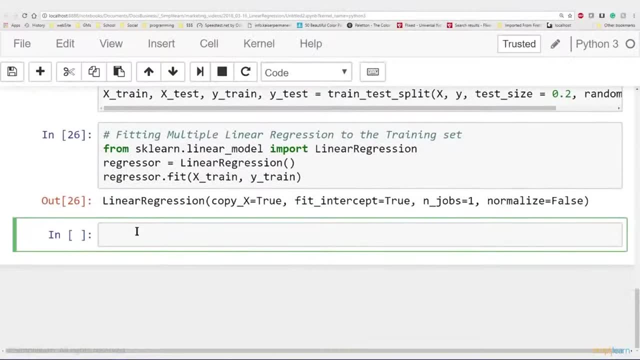 And, if you remember, We kept a bunch of data aside. So we're going to do a Y predict variable And we're going to put in the X test And let's see what that looks like. Scroll down, Scroll up a little bit. 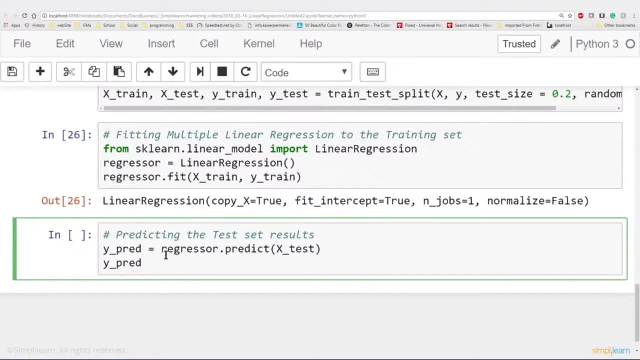 Paste that in here. Predicting the test set results. So here we have Y predict Equals regressor dot predict X test going in And this gives us Y predict. Now, because I'm in Jupyter inline, I can just put the variable up there. 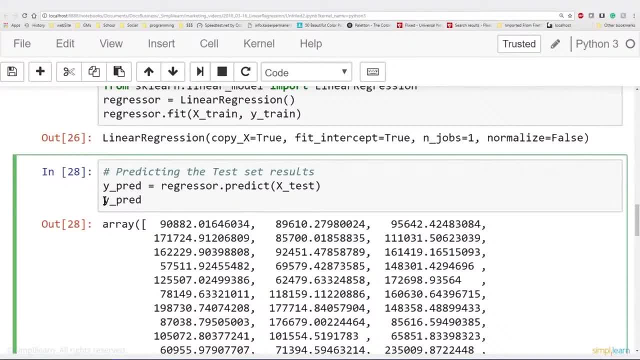 And when I hit the run button It'll print that array out. I could have just as easily done Print Y, predict. So if you're in a different IDE- That's not an inline setup Like the Jupyter notebook- You can do it this way. 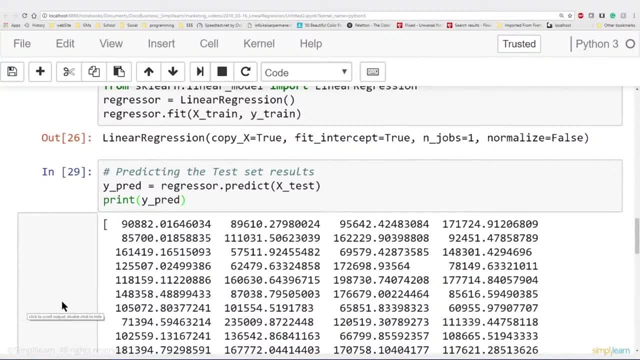 Print Y predict And you'll see that For the 200 different test variables We kept off to the side, It's going to produce 200 answers. This is what it says. the profit are For those 200 predictions. But let's don't stop there. 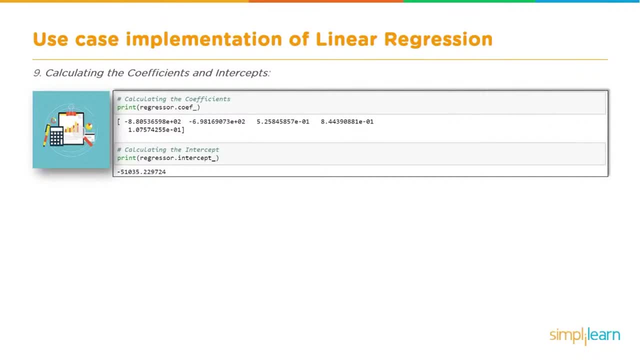 Let's keep going And take a couple look- We're going to take just a short detail here- And calculating the coefficients And the intercepts. This gives us a quick flash At what's going on behind the line. We're going to take a short detour here. 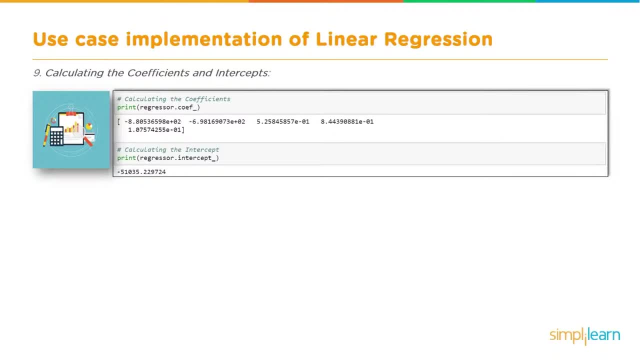 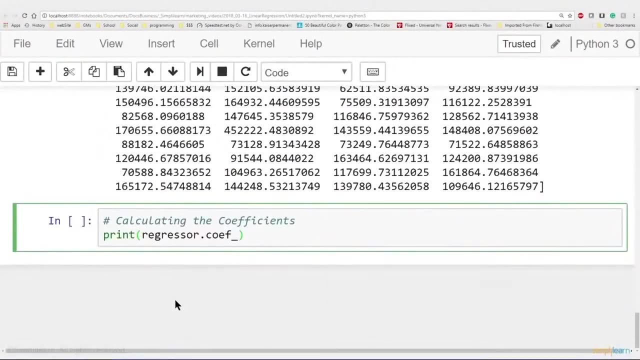 And we're going to be calculating The coefficient and intercepts So you can see what those look like. What's really nice About our regressor we created Is it already has a coefficients for us And we can simply just print. 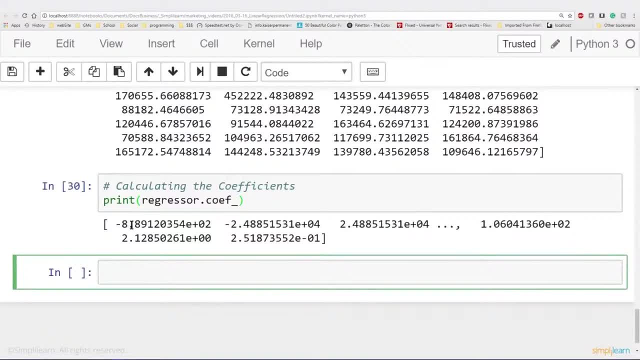 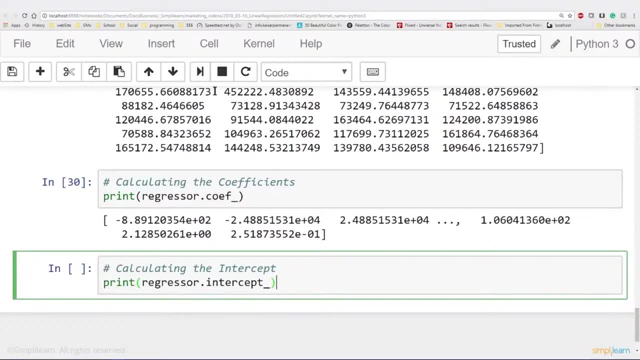 Regressor dot coefficient underscore. When I run this You'll see our coefficients here And if we can do the regressor coefficient, We can also do the regressor intercept. And let's run that And take a look at that. 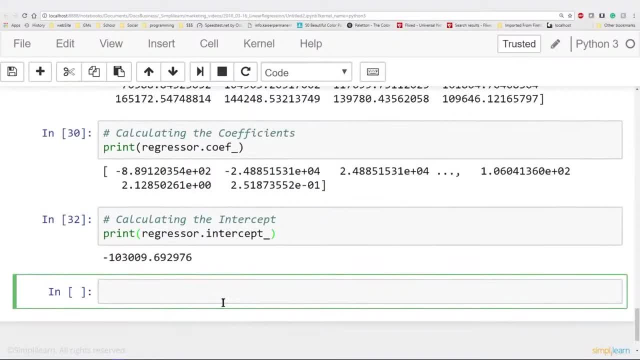 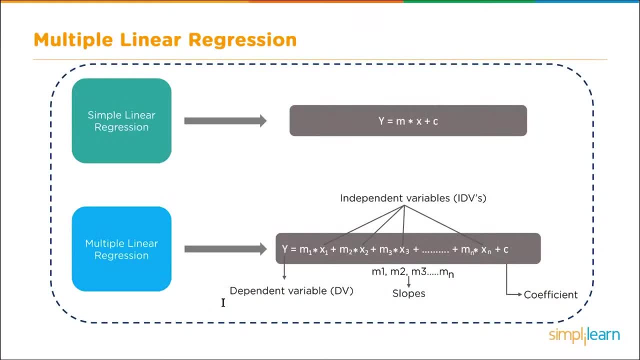 This all came from the multiple regression model And we'll flip over So you can remember where this is going into And where it's coming from. You can see the formula down here, Where Y equals M1 times X1.. Plus M2 times X2.. 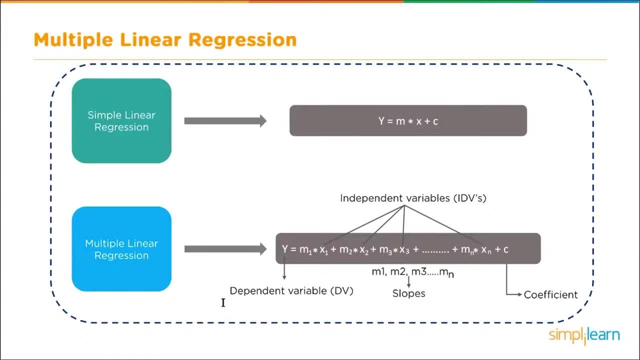 And so on and so on, Plus C the coefficient, So these variables fit right into this formula. Y equals slope 1 times column 1 variable, Plus slope 2 times column 2 variable. All the way to the M, into the N. 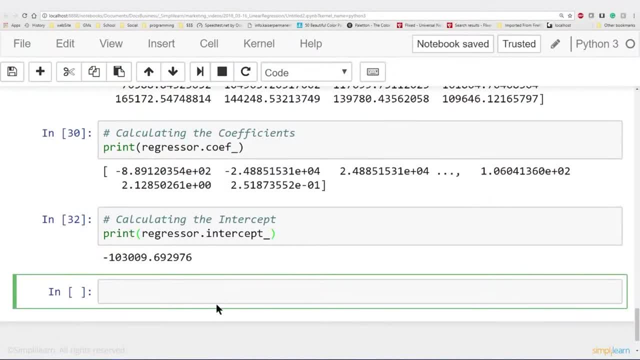 And X to the N plus C the coefficient, Or in this case You have minus 8.89 to the power of 2.. Etc, Etc Times, the first column And the second column And the third column, And then our intercept. 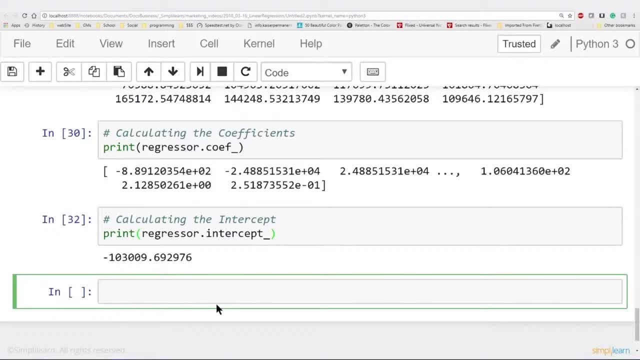 Is the minus 1030.. 0.009.. Boy, it gets kind of complicated when you look at it. This is why we don't do this by hand anymore. This is why we have the computer To make these calculations easy to understand. 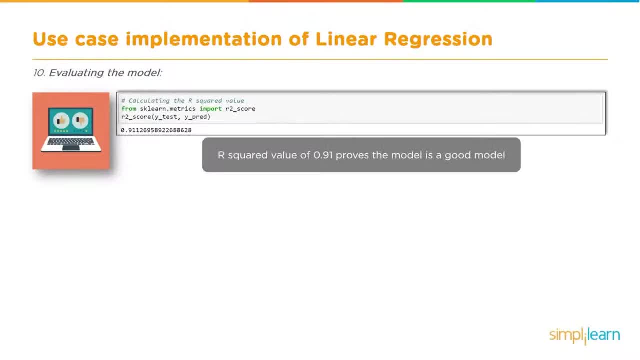 And calculate. Now, I told you that was a short detour And we're coming towards the end of our script. As you remember, from the beginning I said, if we're going to divide this information, We have to make sure it's a valid model. 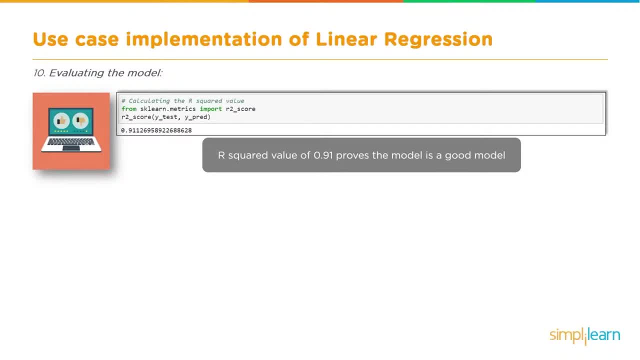 That this model works And understand how good it works. So calculating the R squared value: That's what we're going to use To predict how good our prediction is. And let's take a look at what that looks like in code. And so we're going to use this. 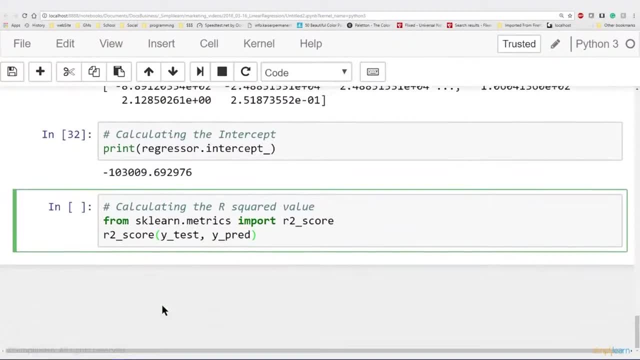 From sklearnmetrics. We're going to import R2 score. That's the R squared value. We're looking at the error. So in the R2 score We take our Y test Versus our Y predict Y test is the actual values we're testing. 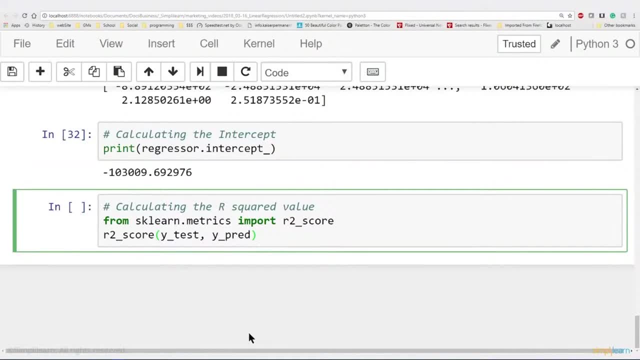 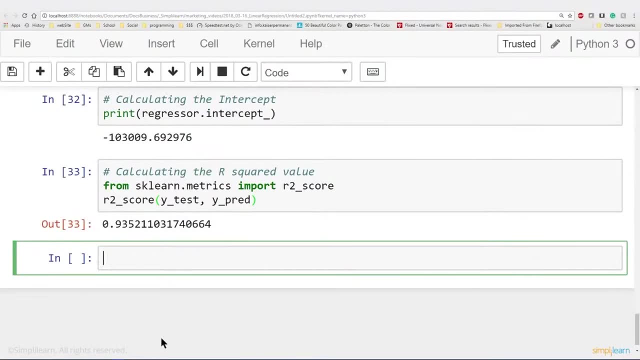 That was the one that was given to us. That we know are true. The Y predict of those 200 values Is what we think it was true And when we go ahead and run this We get a .9352.. That's the R2 score. 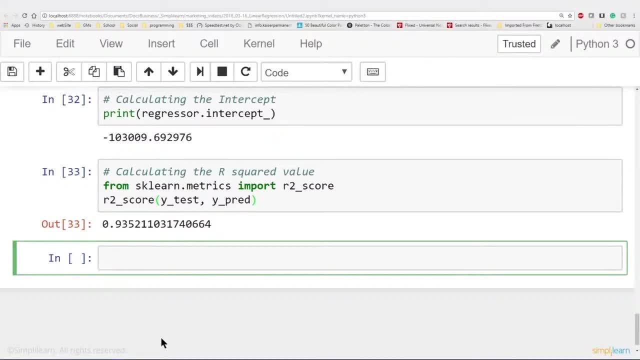 Now it's not exactly a straight percentage, So it's not saying it's 93% correct, But you do want that in the upper 90s. Oh and higher Shows that this is a very valid prediction Based on the R2 score. 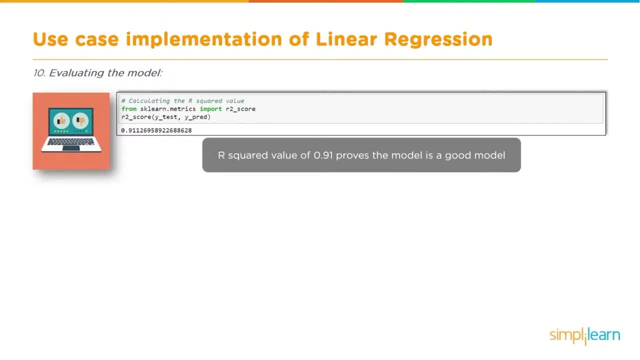 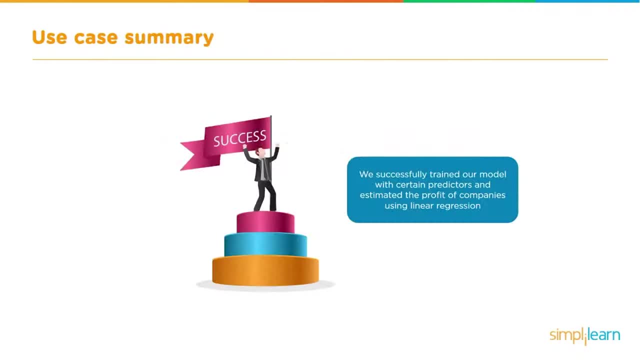 And if R squared value of .91.. Or 92, as we got on our model? Remember it does have a random generation involved. This proves the model is a good model, Which means success. Yay, We successfully trained our model With certain predictors. 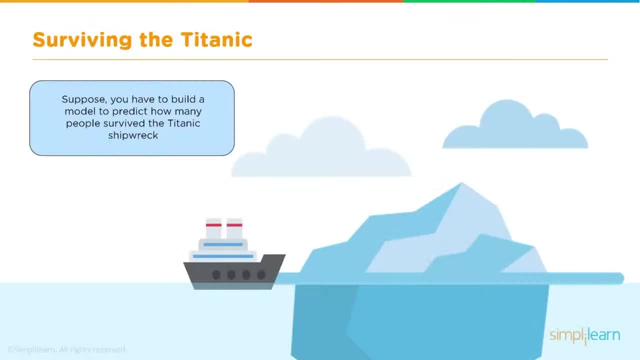 And estimated the profit of the companies Using linear regression. What is logistic regression? Let's say we have to build a predictive model Or a machine learning model To predict whether the passengers Of the Titanic ship Have survived or not. So how do we do that? 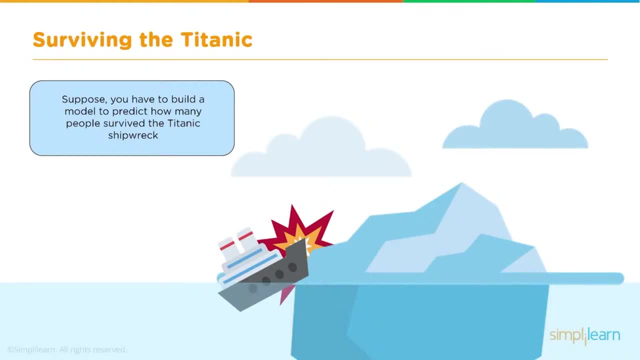 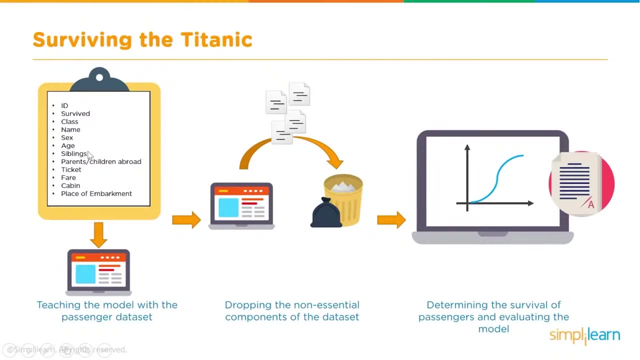 So we use logistic regression To build a model for this. How do we use logistic regression? So we have the information about the passengers, Their ID, Whether they survived or not, Their class and name, and so on and so forth, And we use this information. 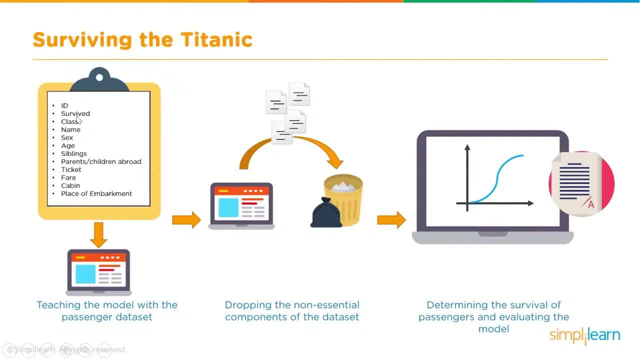 Where we already know Whether the person has survived or not. That is the labeled information, And we help the system to train Based on this information, Based on this labeled data- This is known as labeled data- And during the process of building the model, 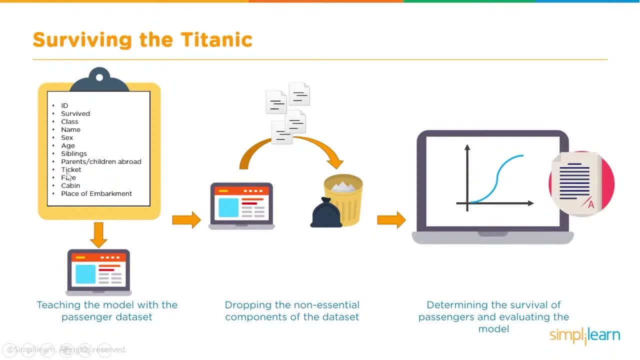 We probably will remove Some of the non-essential parameters Or attributes. here We only take those attributes That are required To make these predictions, And once we train the model, We run new data through it Whereby the model will predict. 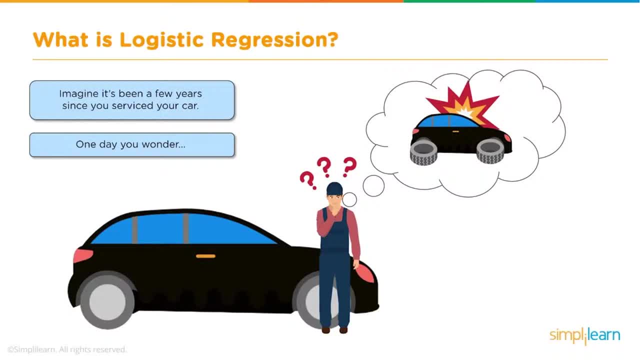 Whether the passenger has survived or not. Alright, What is logistic regression? As I mentioned earlier, Logistic regression is an algorithm For performing binary classification. So let's take an example And see how this works. Let's say your car has not been serviced. 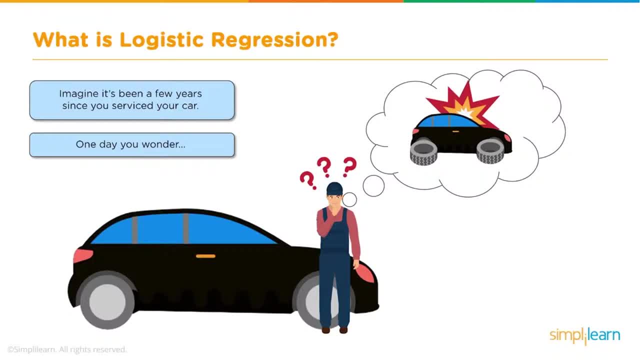 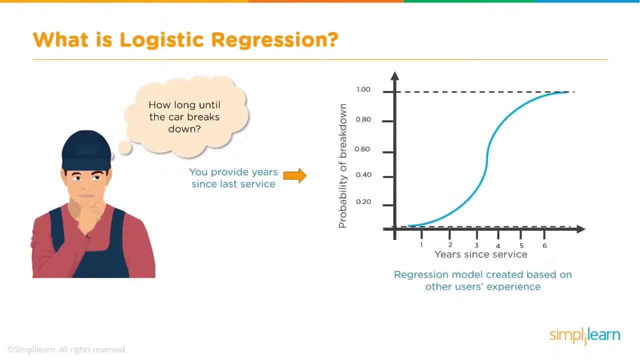 For quite a few years. This is like a classification problem: Find out whether your car will break down Or not. So how are we going to perform this classification? So here is how it looks If we plot the information Along the X and Y axis. 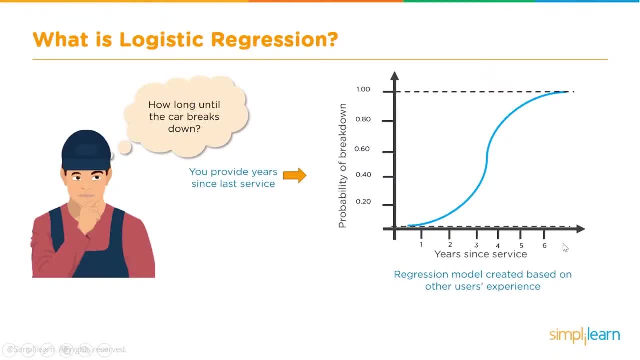 X is the number of years Since the last service was performed And Y is the probability Of your car breaking down. And let's say, this information was This data, rather, Was collected from several car users, It's not just your car. 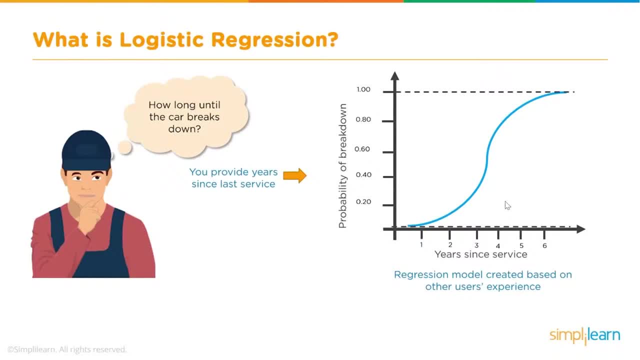 But several car users. So that is our labeled data. So the data has been collected And for the number of years And when the car broke down And what was the probability, And that has been plotted Along X and Y axis. 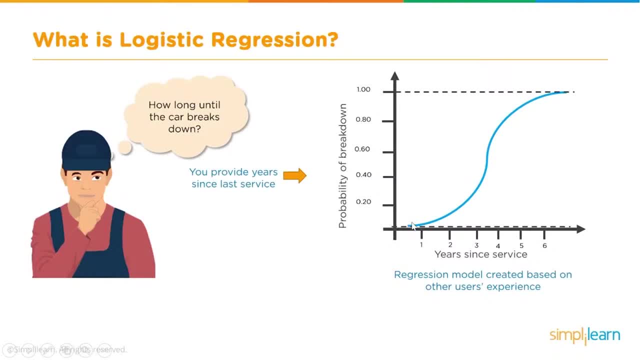 So this provides an idea. From this graph, We can find out whether Your car will break down or not. We'll see how. So first of all, The probability can go from 0 to 1.. Where Probability can be between 0 and 1.. 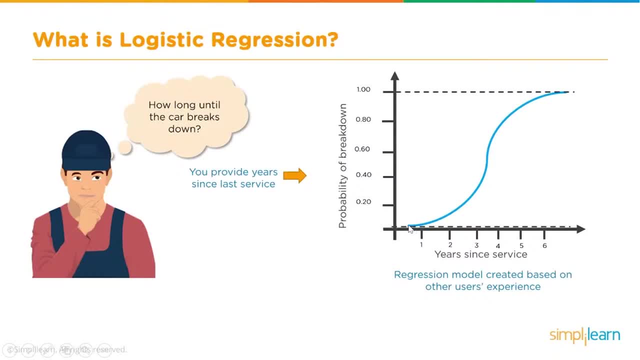 And, as we can imagine, It is intuitive as well. As the number of years are On the lower side, Maybe 1 year, 2 years or 3 years Till after the service, The chances of your car breaking down Are very limited. 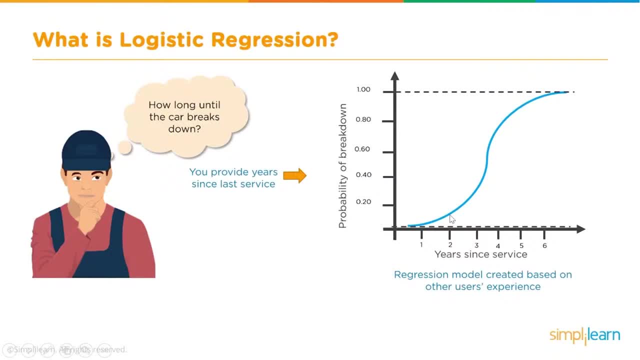 So, for example, Chances of your car breaking down, The probability of your car breaking down Within 2 years of your last service, Are 0.1, probability 0.3, and so on. But as the number of years increases, 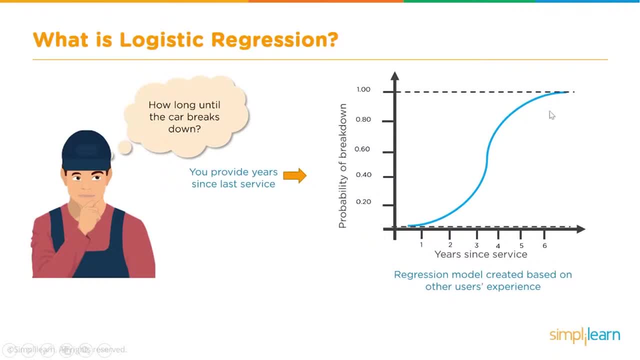 Let's say, if it was 6 or 7 years, There is almost a certainty That your car is going to break down. That is what this graph shows. So this is an example of an application Of the classification algorithm, And we will see. 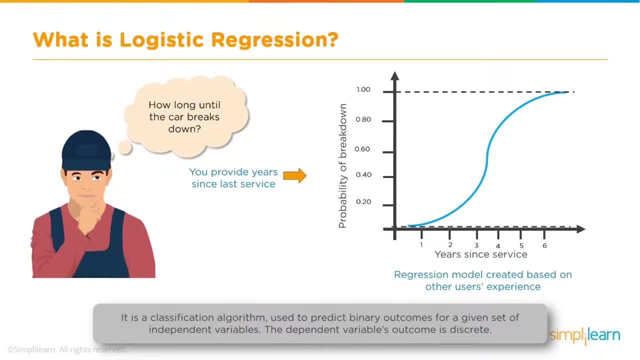 In little details How exactly logistic regression is applied here. One more thing needs to be added here Is that the dependent variables outcome Is discrete. So if we are talking about Whether the car is going to break down Or not, So that is a discrete value. 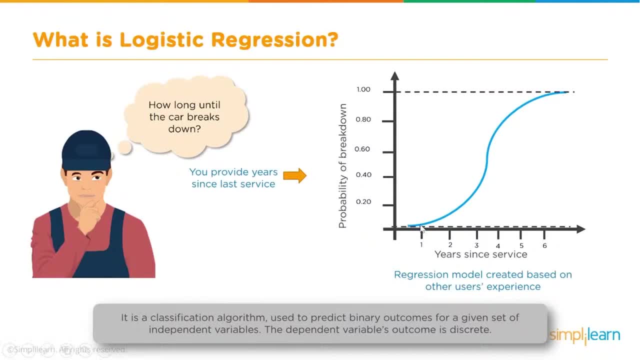 The Y that we are talking about, The dependent variable that we are talking about. What we are looking at is Whether the car is going to break down Or not, Yes or no. That is what we are talking about. So here the outcome is discrete. 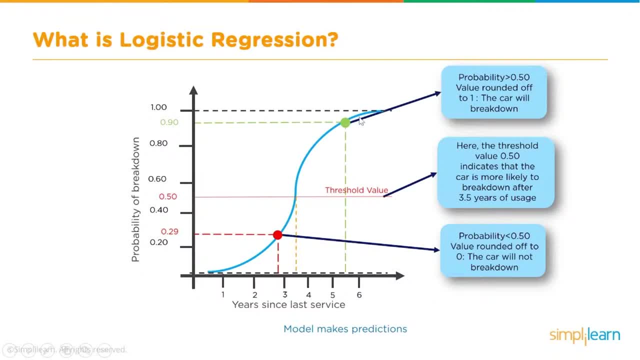 And not a continuous value. So this is how the logistic regression curve looks. Let me explain a little bit. To determine the class, The outcome, rather. So, for a logistic regression curve, A threshold has to be set, Saying that, Because this is a probability calculation, 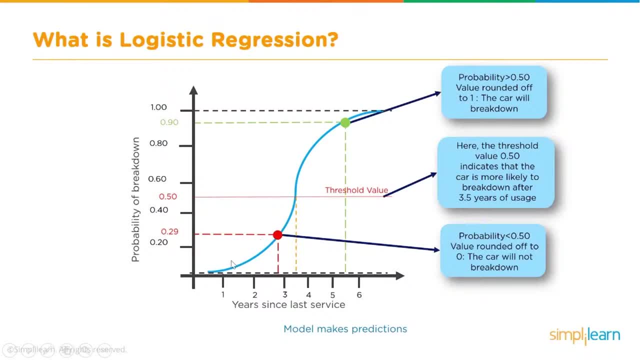 Remember, this is a probability calculation And the probability itself Will not be 0 or 1.. But based on the probability We need to decide what the outcome should be. So there has to be a threshold, Like, for example, 0.5 can be the threshold. 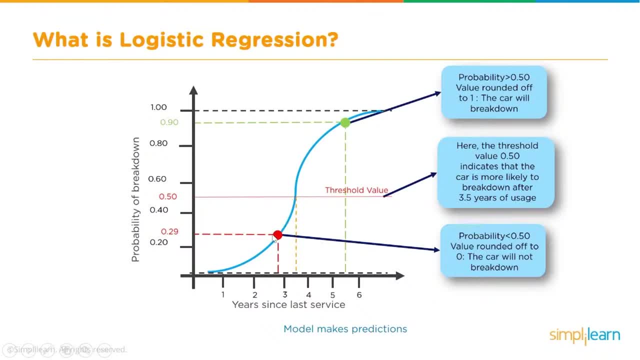 Let us say, in this case, The value of the probability below 0.5. Is considered to be 0. And any value above 0.5. Is considered to be 1.. So an output of, Let us say, 0.8.. 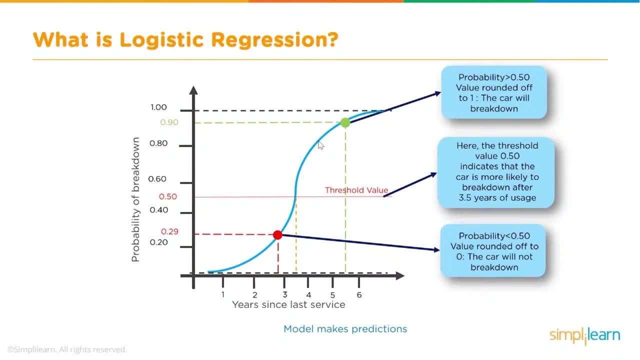 Will mean that the car will break down. So that is considered as an output of 1.. And let us say, An output of 0.29. Is considered as 0. Which means that the car will not break down. So that is the way logistic regression works. 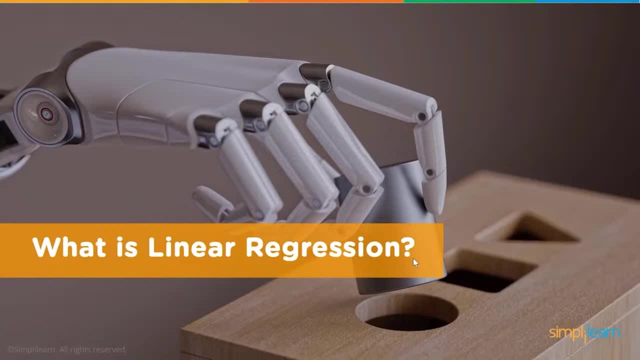 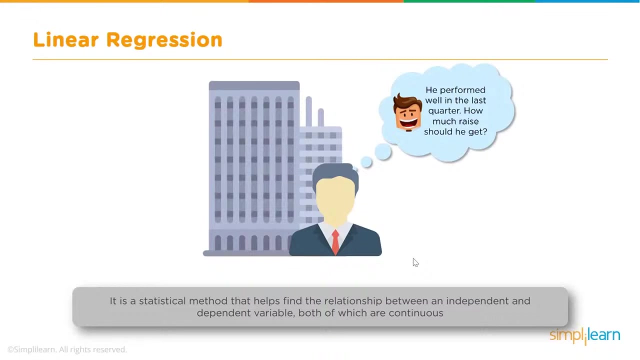 Now let us do a quick comparison Between logistic regression And linear regression, Because they both have The term regression in them, So it can cause confusion, So let us try to remove that confusion. So what is linear regression? Linear regression is a process. 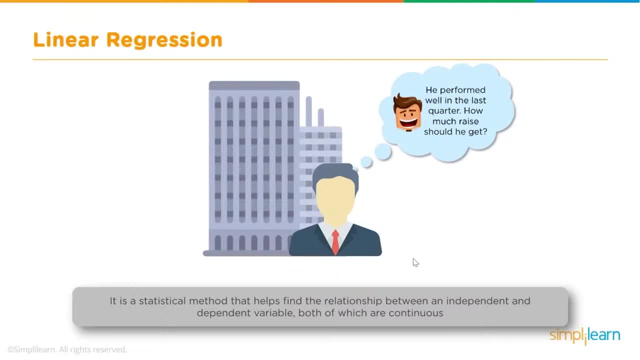 Is once again an algorithm For supervised learning. However, here you are going to find A continuous value. You are going to determine a continuous value. It could be the price of a real estate property. It could be your hike- How much hike you are going to get. 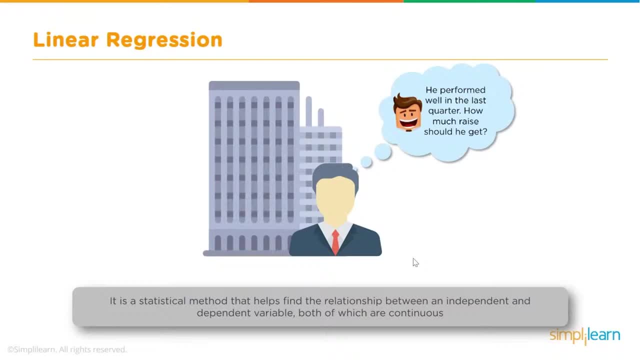 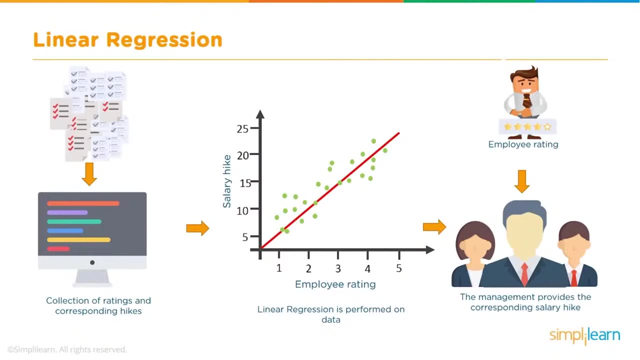 These are all continuous values. These are not discrete Compared to a yes or no kind of response That we are looking for in logistic regression. So this is one example of a linear regression. Let us say The HR team of a company. 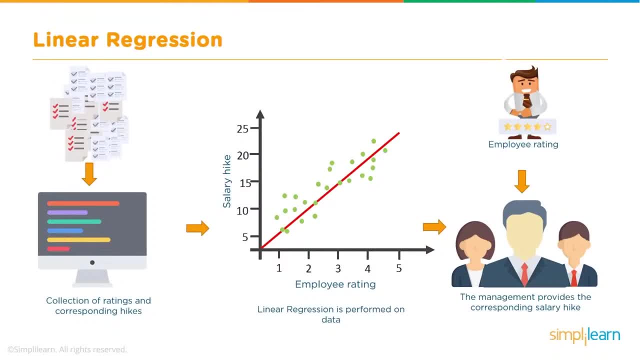 Tries to find out what should be the salary hike Of an employee, So they collect all the details of their existing employees, Their ratings and their salary hikes, What has been given, And that is the labeled information That is available, And the system learns from this. 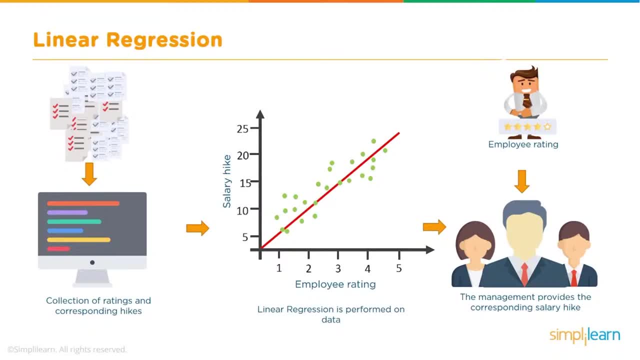 Strain And it learns from this labeled information So that when a new employee's information is fed, Based on the rating, It will determine what should be the hike. So this is a linear regression problem And a linear regression example. Now salary is a continuous value. 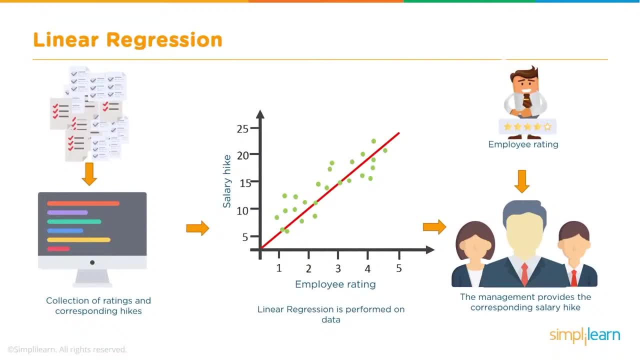 You can get 5000.. 5500. 5600.. It is not discrete Like a cat or a dog, Or an apple or a banana. These are discrete, Continuous values. So this where you are trying to find Continuous values. 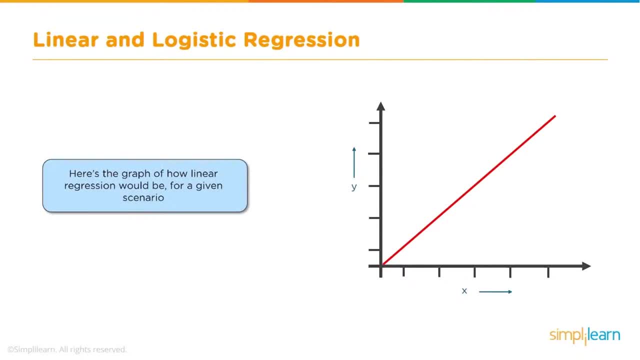 Is where we use linear regression. So let us say, Just to extend on this scenario, We now want to find out Whether this employee is going to get a promotion Or not, So we want to find out. That is a discrete problem. 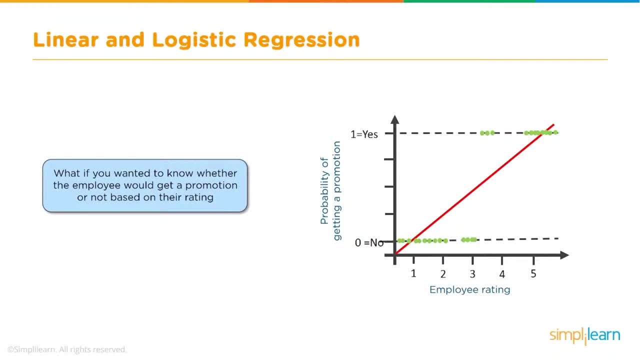 A yes or no kind of a problem. In this case. We actually cannot use linear regression, Even though we may have labeled data So based on the employee rating. These are the ratings. And then some people got the promotion And this is the ratings. 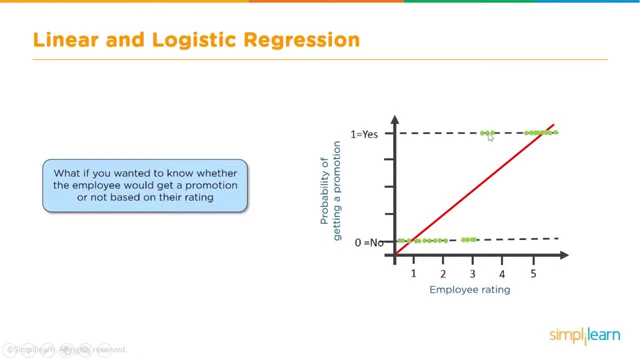 For which people did not get promotion. That is a no And this is the rating for which people got promotion. We just plotted the data About whether a person has got An employee has got promotion Or not, So there is nothing in between. 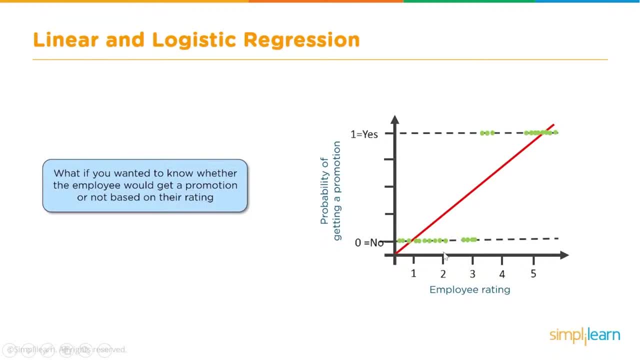 And what is the employees rating? And ratings can be continuous. That is not an issue In this case, Whether employee got promotion Yes or no. So if we try to plot that And we try to find a straight line, This is how it would look. 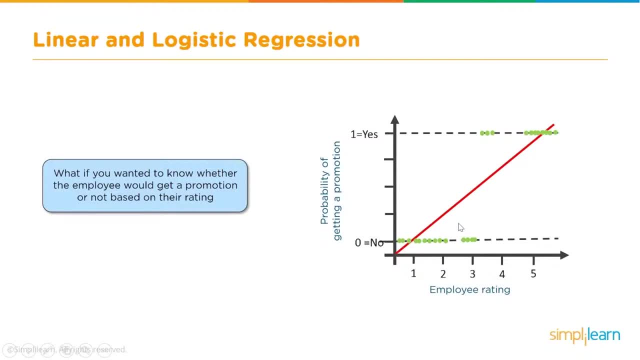 And, as you can see, It does not look very right Because looks like there will be lot of errors. This root mean square error, If you remember, for linear regression Would be very, very high And also the values cannot go beyond 0.. 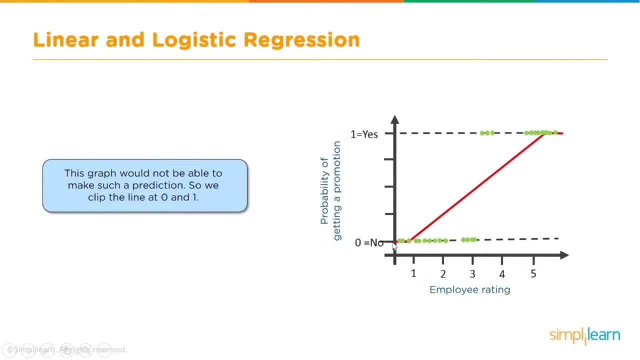 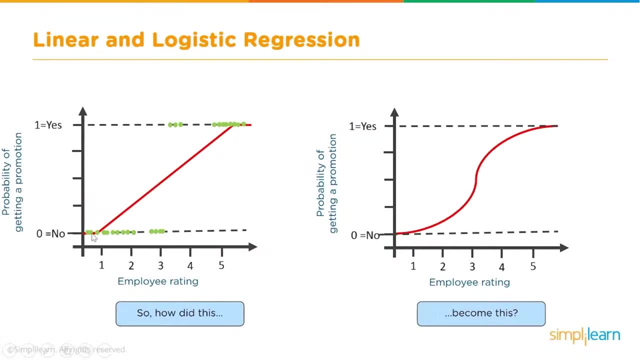 Or beyond 1.. So it is clipped at 0 and 1.. But still this straight line Does not look right. Therefore, instead of using A linear equation, We need to come up with something different, And therefore the logistic regression. 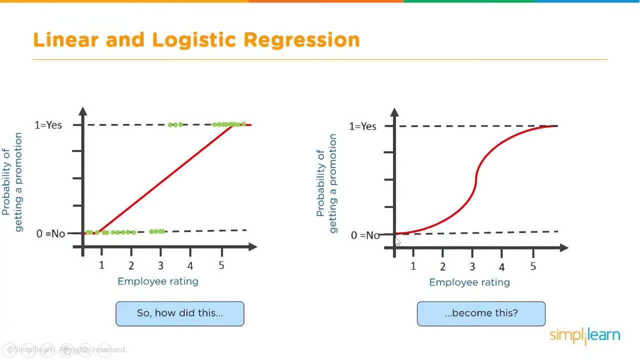 Model looks Somewhat like this. So we calculate the probability, And if we plot that probability- Not in the form of a straight line, But we need to use some other equation- We will see very soon what that equation is Then. it is a gradual process. 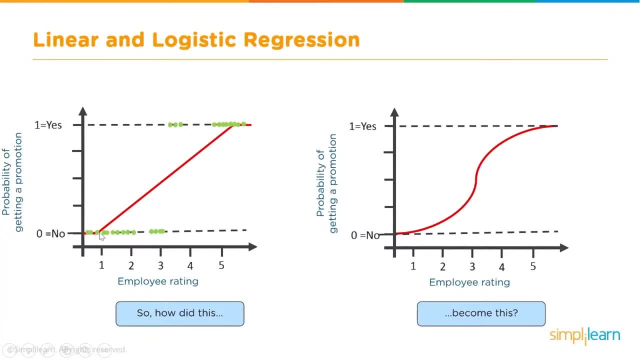 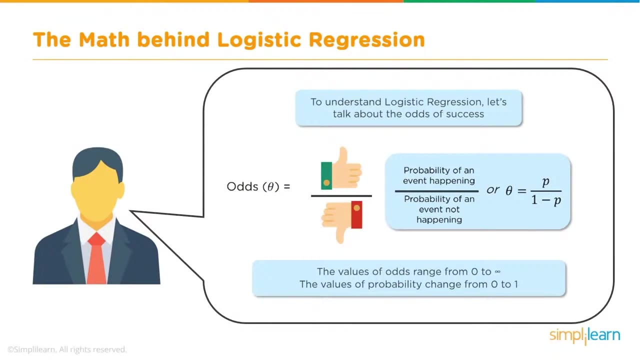 So you see here, People with some of these ratings Are not getting any promotions And then slowly, at certain rating, They get promotions. So it is a gradual process And this is how the math Behind logistic regression looks. So we are trying to find the odds. 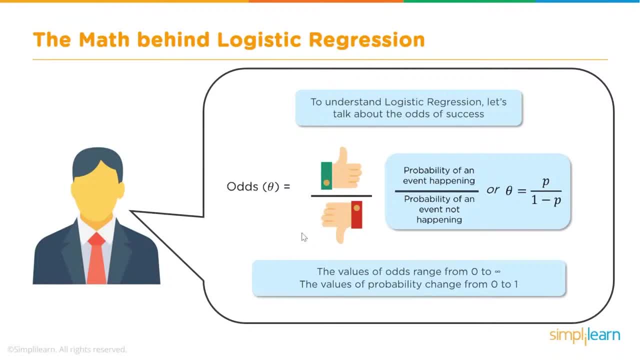 For a particular event happening. And this is the formula For finding the odds. So the probability of an event happening Divided by the probability Of the event not happening. So p if it is the probability Of the event happening. Probability of the person getting a promotion. 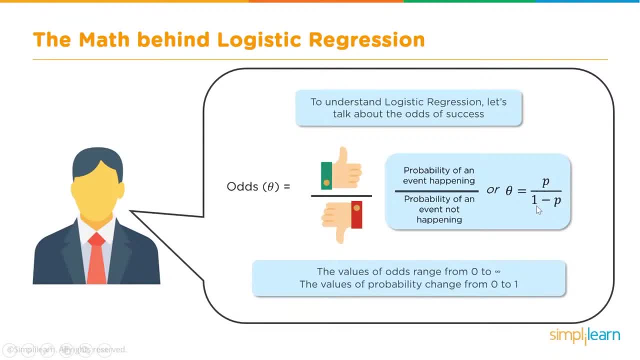 And divided by the probability Of the person not getting a promotion, That is 1 minus p. So this is how you measure the odds. Now, the values of the odds Range from 0 to infinity, So when this probability Is 0.. 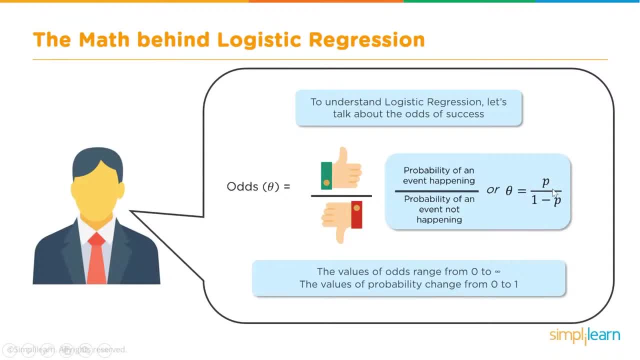 Then the value of the odds Is equal to 0. And when the probability becomes 1. Then the value of the odds Is 1 by 0. That will be infinity, But the probability itself remains Between 0 and 1.. 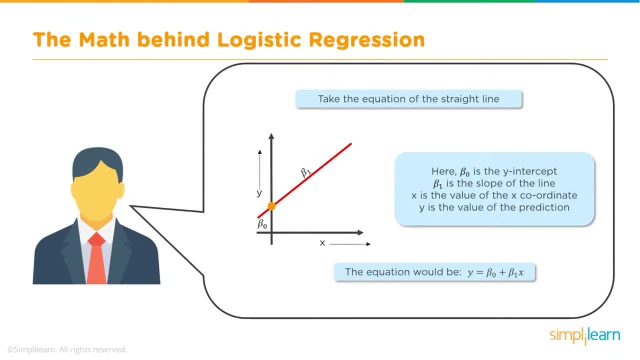 Now this is how an equation of a straight line looks. So y is equal to beta 0. Plus beta 1, x, Where beta 0 is the y intercept And beta 1 is the slope of the line, If we take the odds equation. 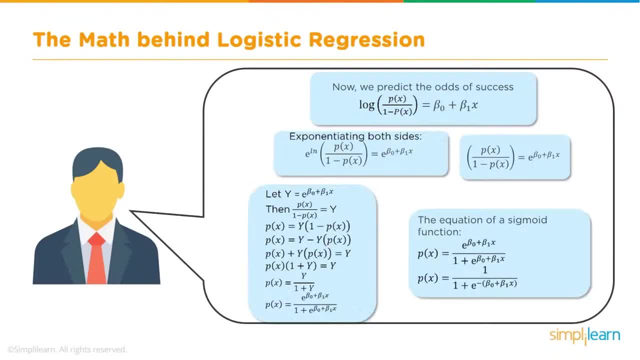 And take a log of both sides. Then this would look somewhat like this- And the term logistic Is actually derived from the fact That we are doing this: The log of p x By 1 minus p x. This is an extension of the calculation of odds. 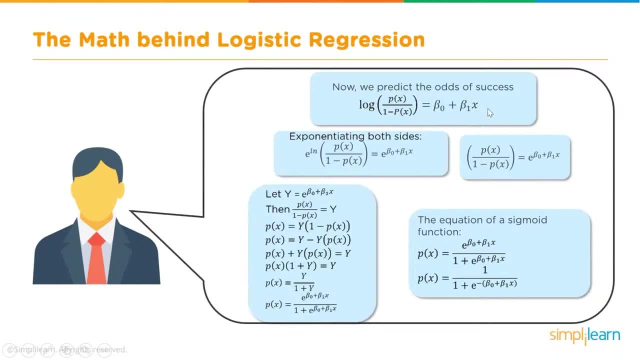 That we have seen And that is equal to beta 0 plus beta 1 x, Which is the equation of the straight line. And now, from here, If you want to find out the value of p x, You will see, we can take. 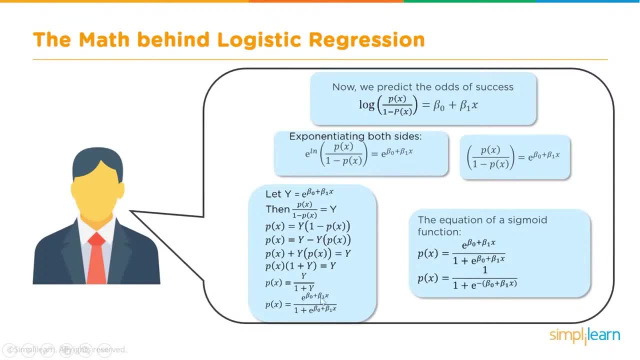 The exponential on both sides And then if we solve that equation, We will get the equation Of p? x like this: p x is equal to 1 by 1 plus e, to the power of beta 0 plus beta 1 x. 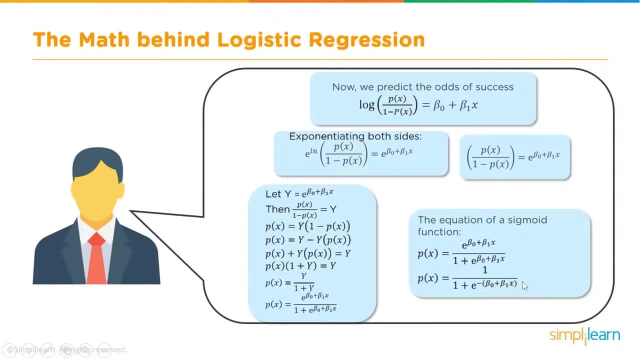 And recall. This is nothing but the equation of the line Which is equal to y. y is equal to beta 0 plus beta 1 x. So this is the equation Also known as the sigmoid function. This is the equation of the logistic regression. 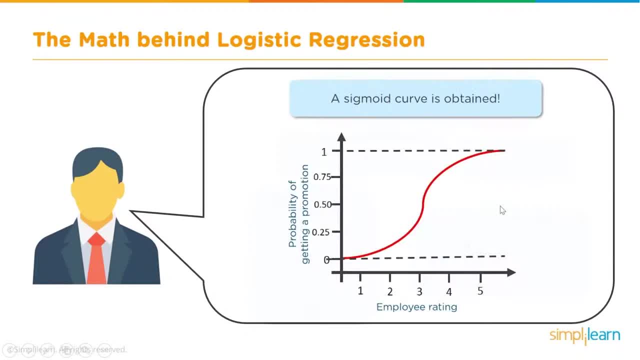 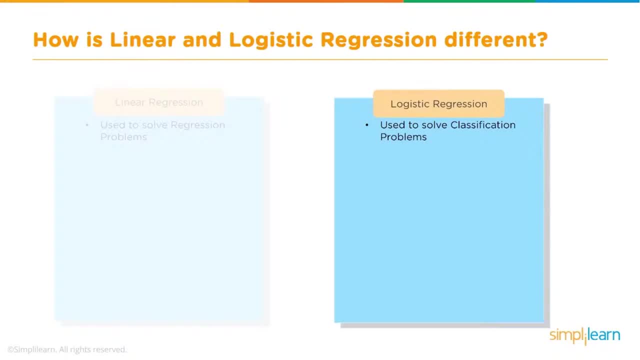 Alright. And if this is plotted, This is how the sigmoid curve is obtained. So let's compare Linear and logistic regression, How they are different from each other. Let's go back. Linear regression is solved Or used to solve regression problems. 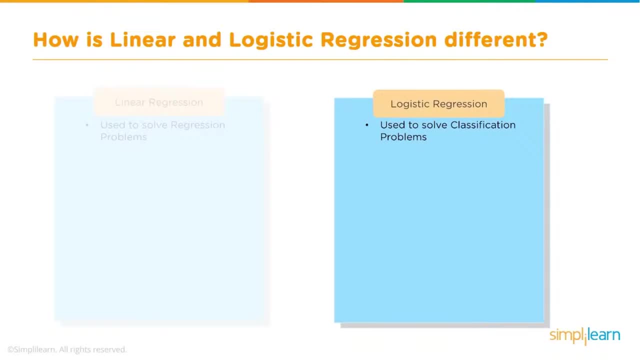 And logistic regression Is used to solve classification problems, So both are called regression. But linear regression Is used for solving regression problems Where we predict continuous values, Whereas logistic regression Is used for solving Classification problems Where we have to predict discrete values. 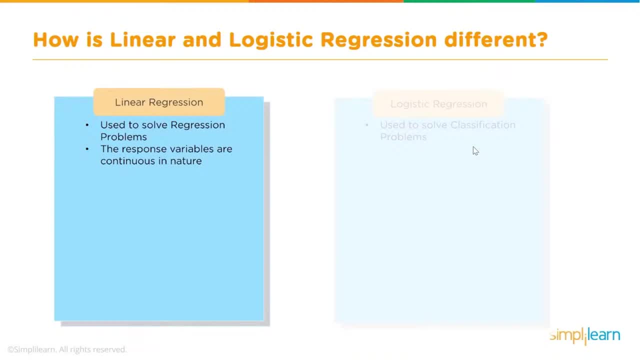 The response variables In case of linear regression Are continuous in nature, Or categorical or discrete in nature, And linear regression Helps to estimate the dependent variable When there is a change in the independent variable, Whereas here, In case of logistic regression, 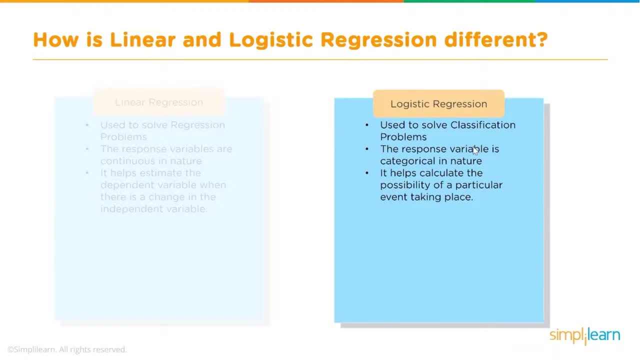 It helps to calculate the probability Or the possibility Of a particular event happening, And linear regression, as the name suggests, Is a straight line. That's why it's called linear regression, Whereas logistic regression Is a sigmoid function And the curve is 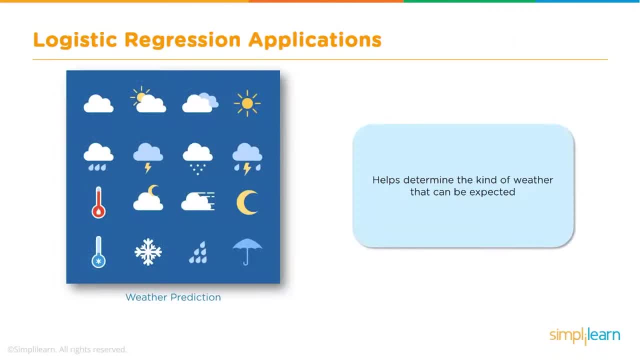 An S. It's an S shaped curve. This is another example of application of logistic regression In weather prediction: Whether it's going to rain or not rain. Now keep in mind Both are used in weather prediction. If we want to find the discrete values, 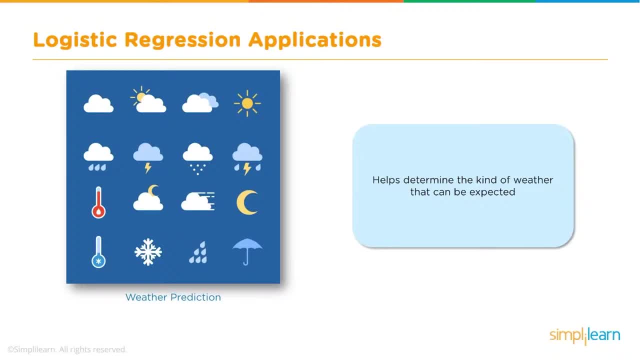 Like whether it's going to rain or not rain. That is a classification problem. We use logistic regression, But if we want to determine What is going to be the temperature tomorrow, Then we use linear regression. So just keep in mind These are some examples of logistic regression. 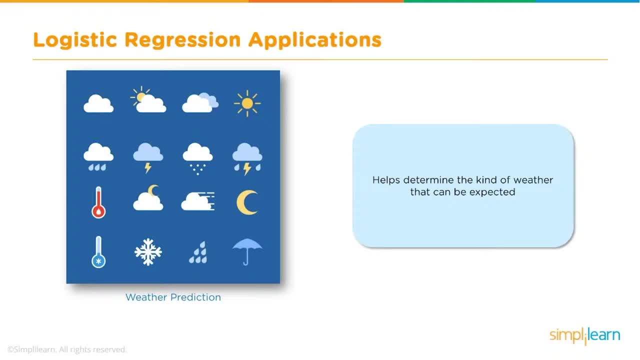 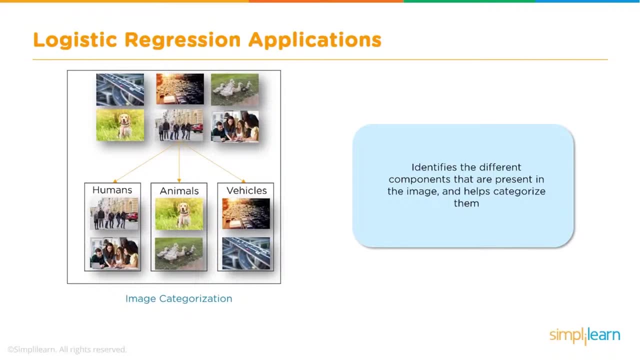 So we want to find out Whether it's going to be rain or not, Whether it's going to be sunny or not, Whether it's going to snow or not. These are all logistic regression examples. A few more examples: Classification of objects. 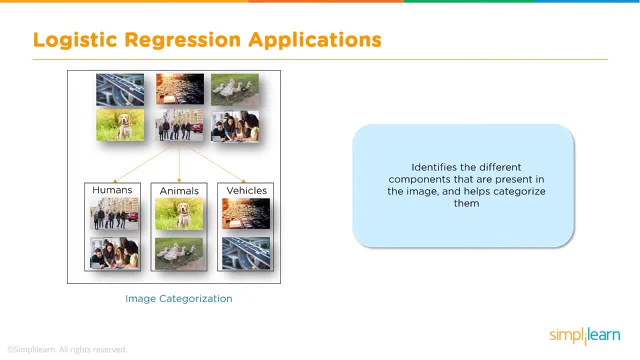 This is again another example of logistic regression. Now here, of course, One distinction is that These are multi-class classification, So logistic regression Is not used in its original form, But it is used In a slightly different form. So we say: 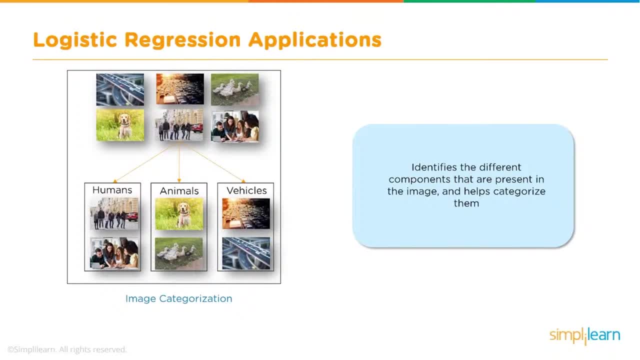 Whether it is a dog or not a dog. I hope you understand. So instead of saying Is it a dog or a cat or an elephant, We convert this into saying Because we need to keep it to binary classification. So we say: 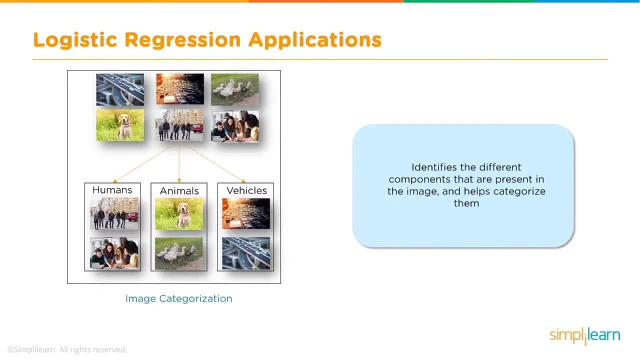 Is it a dog or not a dog? Is it a cat or not a cat? So that's the way logistic regression can be used For classifying objects. Otherwise, there are other techniques Which can be used. Logistic regression is used to find: 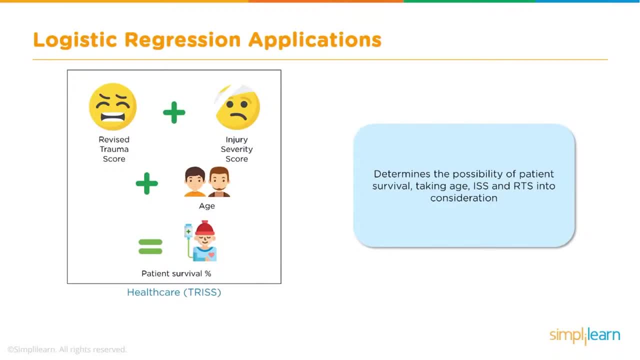 The survival rate of a patient. So they take multiple parameters Like trauma score, Age and so on and so forth, And they try to predict The rate of survival. Alright, now finally, let's take an example And see how we can apply. 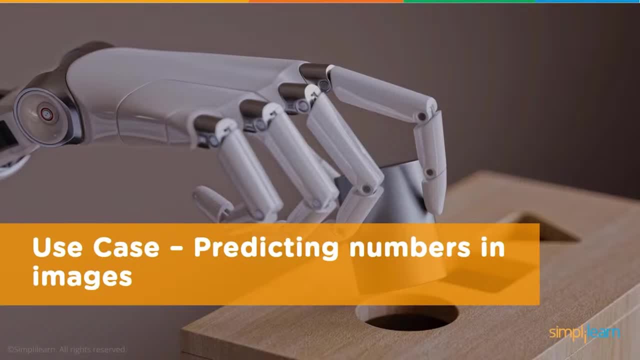 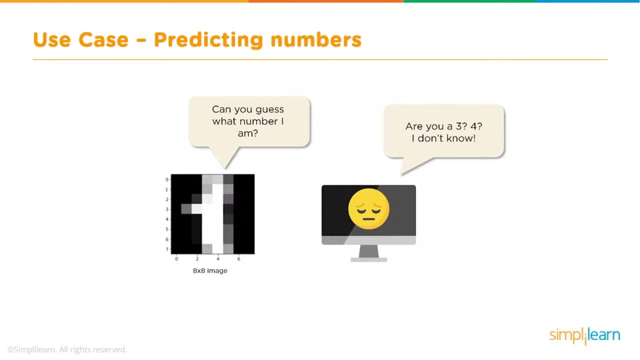 Logistic regression To predict the number that is shown in the image. So this is actually A live demo. I will take you into jupiter notebook And show the code, And before that Let me take you through a couple of slides. 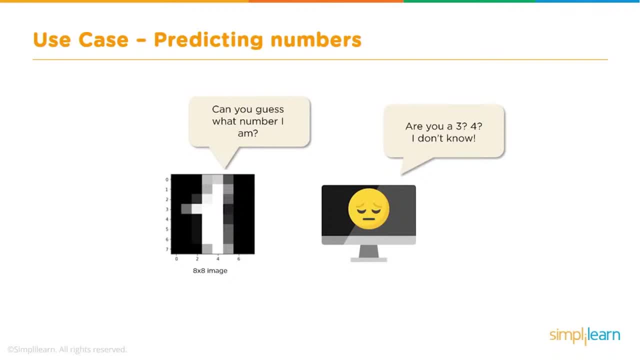 To explain what we are trying to do. So let's say you have an 8x8 image And the image has a number 1234.. And you need to train your model To predict what this number is. So how do we do this? 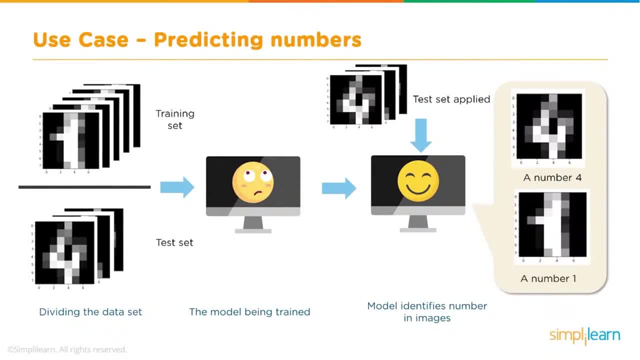 So the first thing is obviously, In any machine learning process, You train your model. So in this case, we are using logistic regression, So and then we provide a training set To train the model, And then we integrate our model list With the test data. 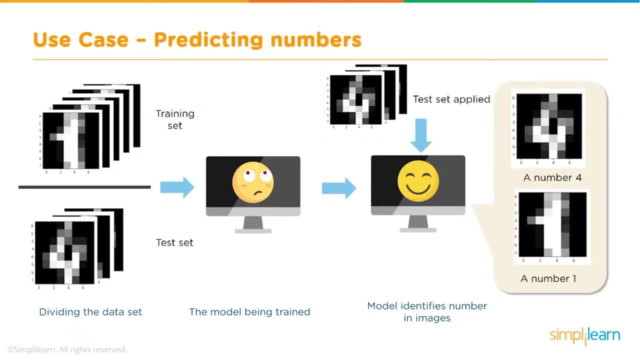 Which means that, like any machine learning process, We split our initial data into two parts: Training set and test set. With the training set, we train our model And then, with the test set, we test the model Till we get good accuracy, And then we use it for inference. 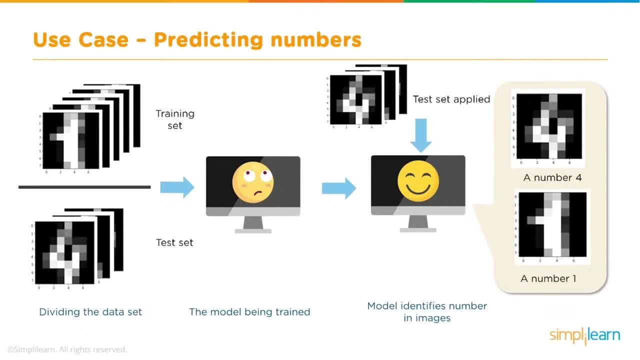 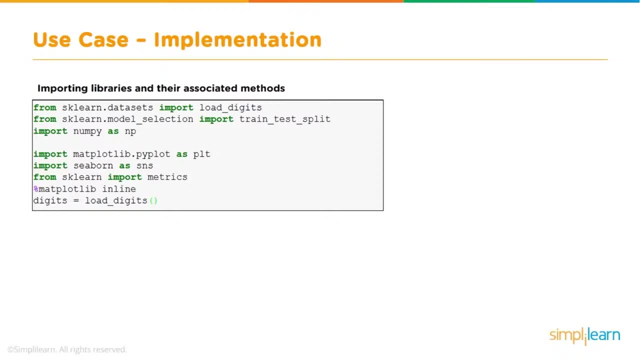 Right. So that is typical methodology Of training, testing And then deploying of machine learning models. So let's take a look at the code And see What we are doing. So I will not go line by line, But just take you through some of the blocks. 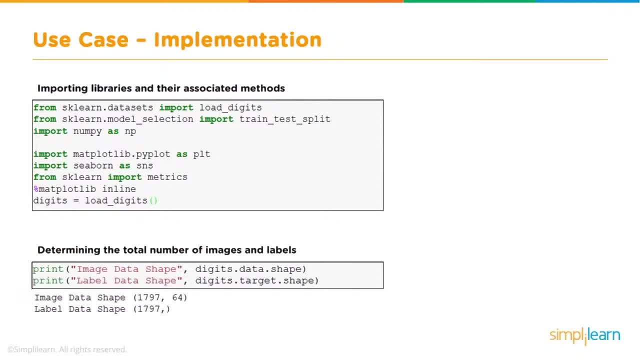 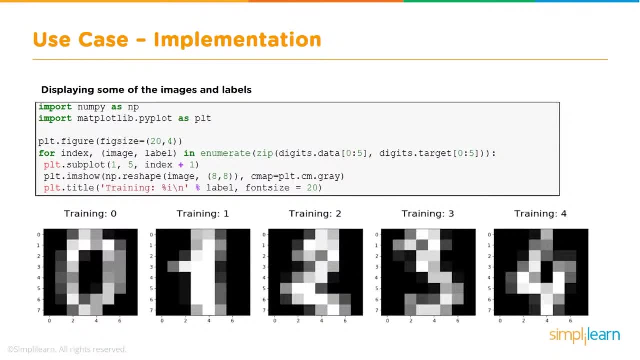 So first thing we do Is import all the libraries And then we basically take a look at the images And see what is the total number of images We can display using matplotlib. Some of the images Or a sample of these images: 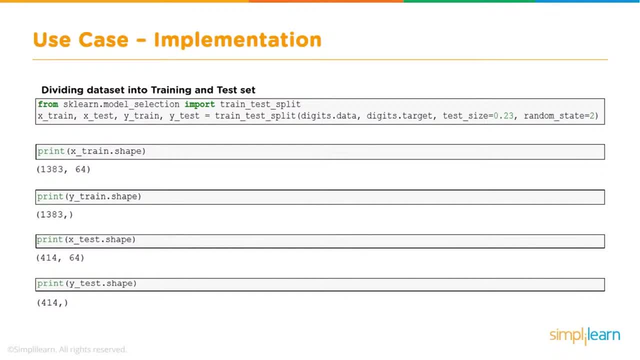 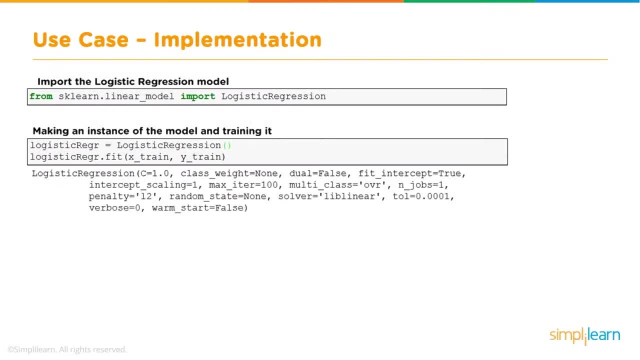 And then we split the data into training and test, As I mentioned earlier, And we can do some exploratory analysis, And then We build our model, We train our model with the training set And then we test it with our test set. 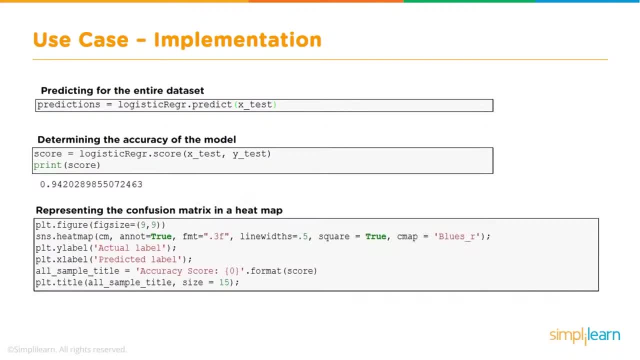 And find out how accurate our model is, Using the confusion matrix, The heat map, And use heat map for visualizing this, And I will show you in the code What exactly is the confusion matrix And how it can be used For finding the accuracy. 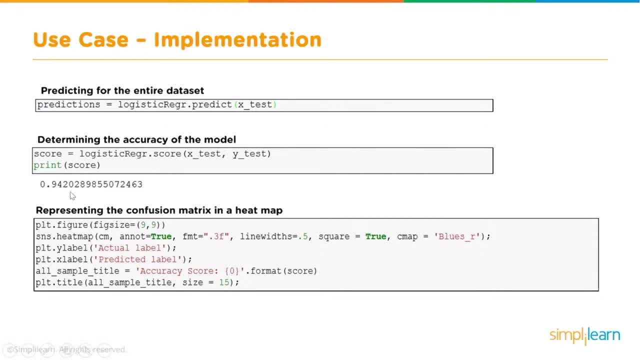 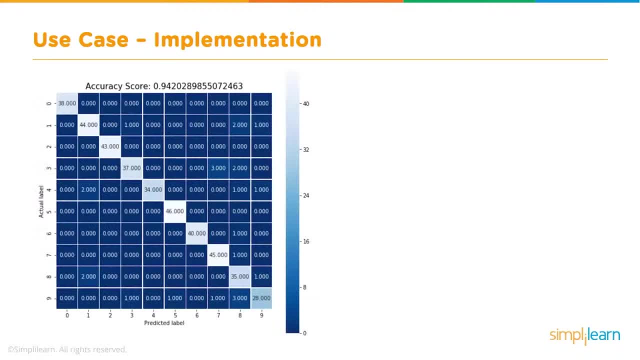 In our example, We get an accuracy of about 0.94., Which is pretty good, Or 94%, which is pretty good. Alright, So this is an example of a confusion matrix And this is used for Identifying the accuracy. 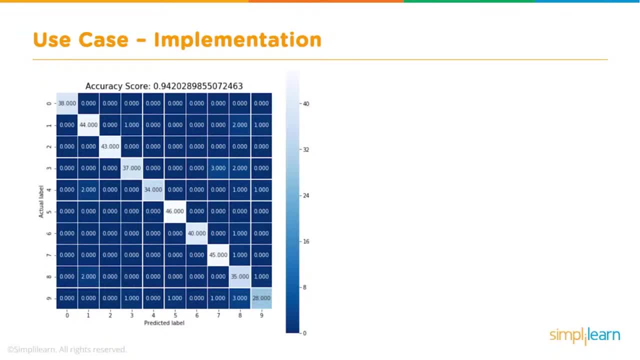 Of a classification model Like a logistic regression model. So the most important part In a confusion matrix Is that, first of all, As you can see, this is a matrix And the size of the matrix Depends on how many outputs We are expecting. 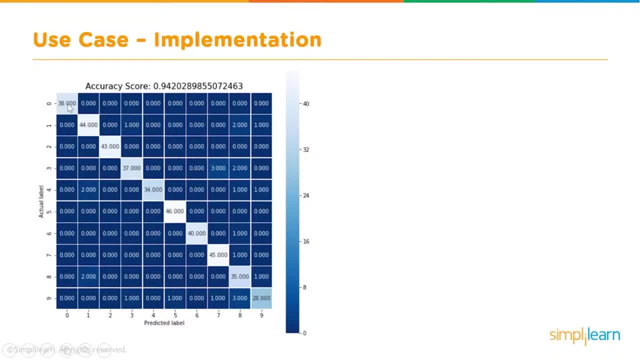 So the most important part here Is that the model will be Most accurate The maximum numbers In its diagonal, Like in this case. That's why it has almost 93-94%, Because the diagonal should have The maximum numbers. 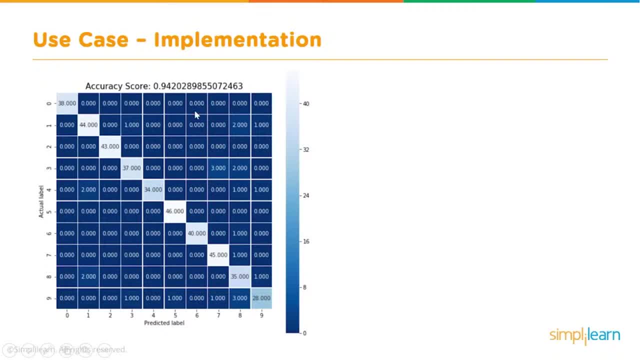 And the others other than diagonal. The cells other than the diagonal Should have very few numbers. So here that's what is happening. So there is a 2 here, There is a 1 here, But most of them are along the diagonal. 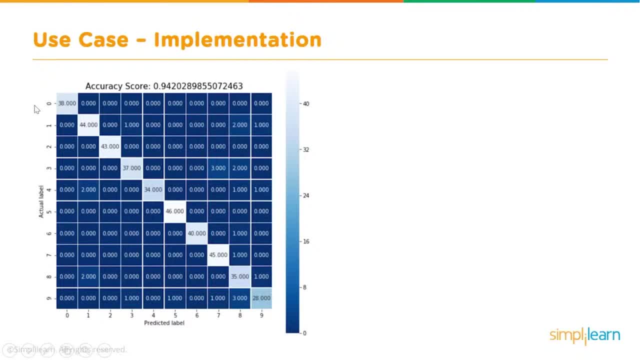 What does this mean? The number that has been Fed is 0. And the number that has been detected Is also 0. So the predicted value and the actual value Are the same. So along the diagonals, that is true. 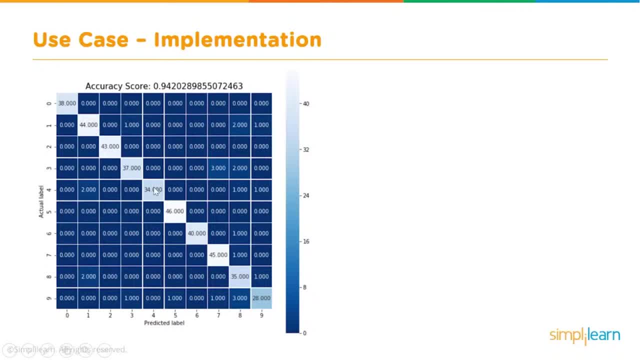 Which means that let's take this diagonal. If the maximum number is here, That means that, Like here, in this case, it is 34.. Which means that 34 of the images That have been fed, Or rather, actually there are 2 misclassifications in there. 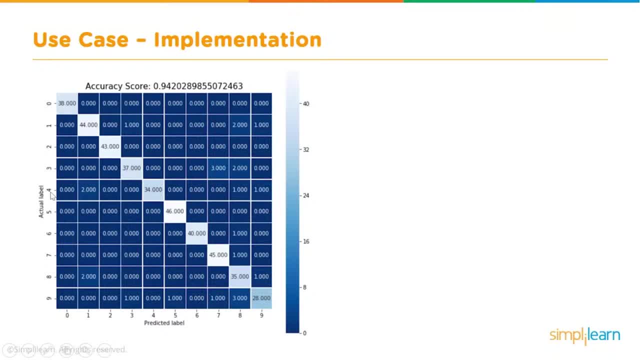 So 36 images Have been fed Which have number 4. And out of which 34 have been predicted Correctly as number 4. And one has been predicted as number 8. And another one has been predicted as Number 9.. 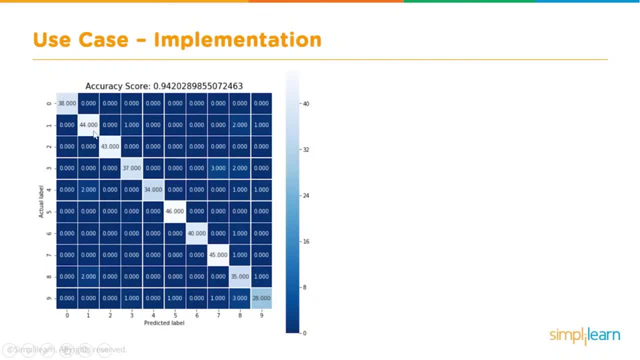 So these are 2 misclassifications. So that is the meaning of saying that The maximum number should be in the diagonal. So, if you have all of them, So for an ideal model Which has, let's say, 100% accuracy. 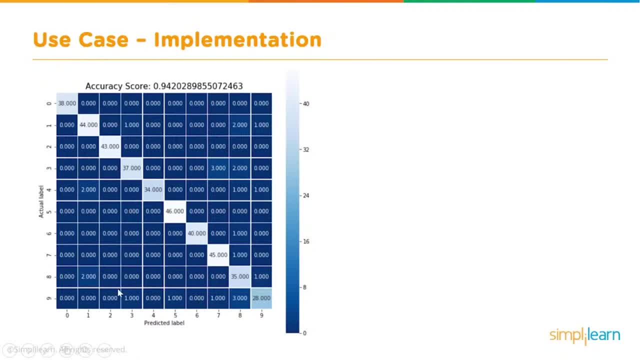 Everything will be only in the diagonal. There will be no numbers In all other cells. So that is like a 100% accurate model. Okay, So that is just of how to use this matrix, How to use this confusion matrix. I know the name. 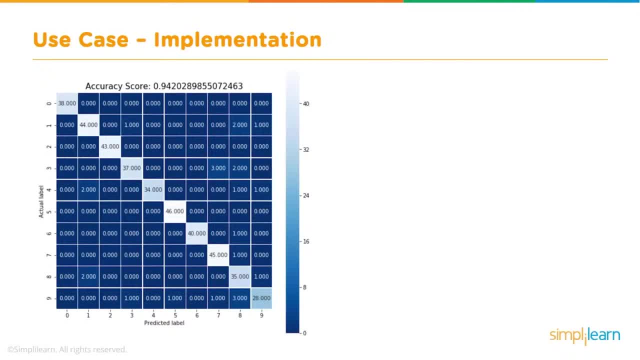 Is a little funny sounding Confusion matrix, But actually it is not very confusing, It is very straight forward. So you are just plotting what has been predicted And what is the labeled information, Or what is the actual data That is also known as the ground truth sometimes. 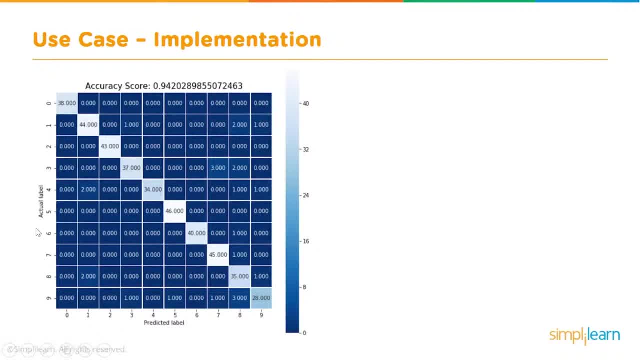 Okay, these are some fancy terms that are used: The predicted label And the actual label. Okay, so we are showing a little bit more information here. So 38 have been predicted, And here you will see that All of them have been predicted correctly. 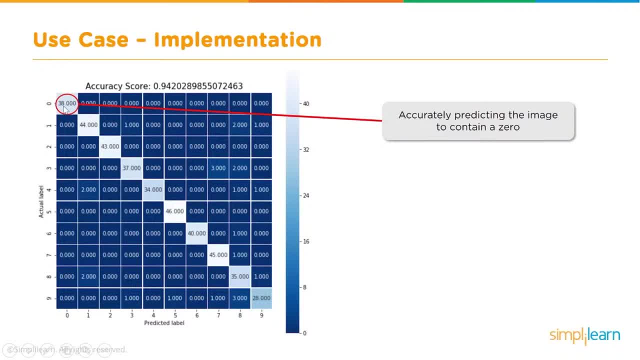 There have been 38 zeros And the predicted value And the actual value is exactly the same, Whereas in this case It has. There are, I think, 37 plus 5.. 42 have been fed The images. 42 images are of digit 3.. 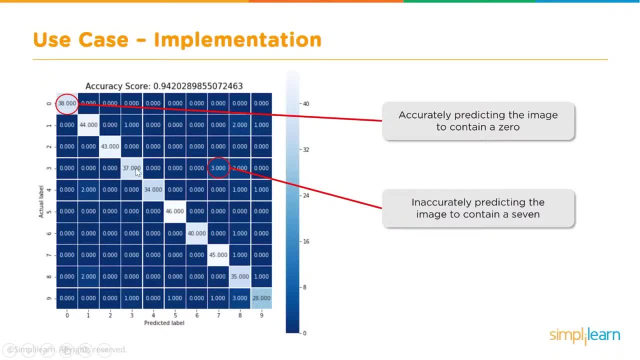 And the accuracy is Only 37 of them have been accurately predicted. 3 of them Have been predicted as number 7. And 2 of them have been predicted as number 8.. And so on and so forth. Okay, alright. 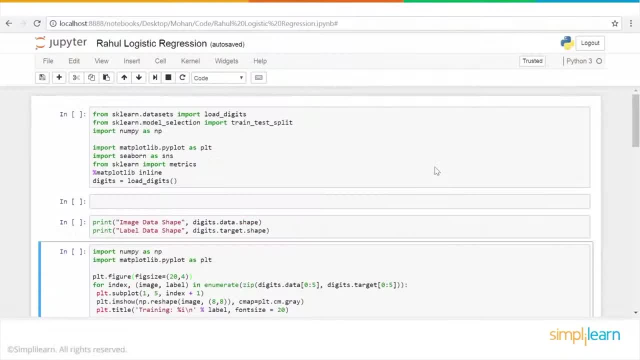 So with that, let's go into Jupyter Notebook And see how the code looks. So this is the code In Jupyter Notebook For logistic regression. In this particular demo, What we are going to do is Train our model With digits. 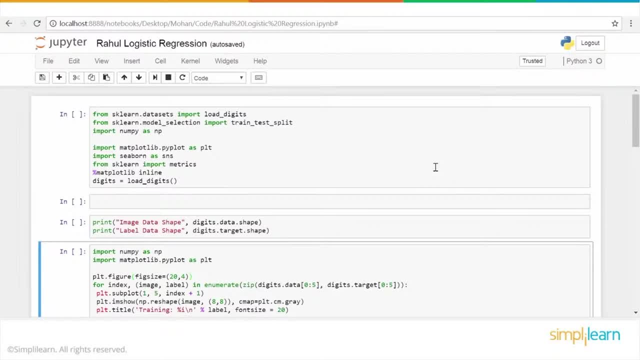 Which are the images Which have digits from, Let's say, 0 to 5 or 0 to 9.. And then we will See how well it is trained And whether it is able to predict these numbers Correctly or not. 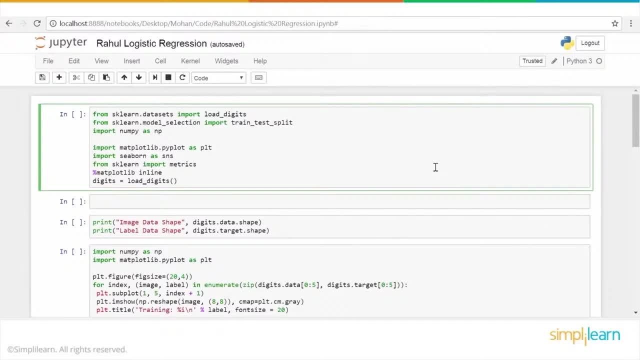 So let's get started. So the first part is as usual. We are importing some libraries That are required, And then the last line In this block Is to load the digits And run this code. Then here we will Visualize the shape of these digits. 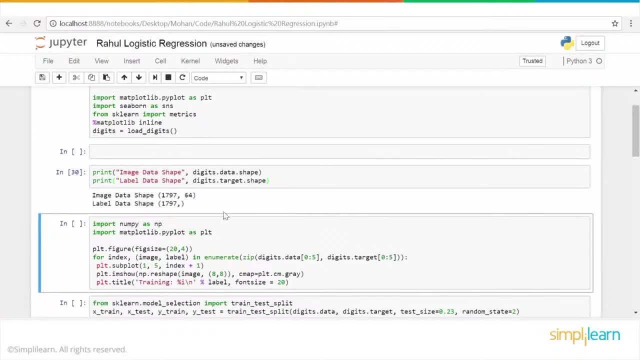 So we can see here, If we take a look, This is how the shape is: 1797 by 64.. These are like 8 by 8 images. So that's what is reflected in this shape. Now from here onwards, 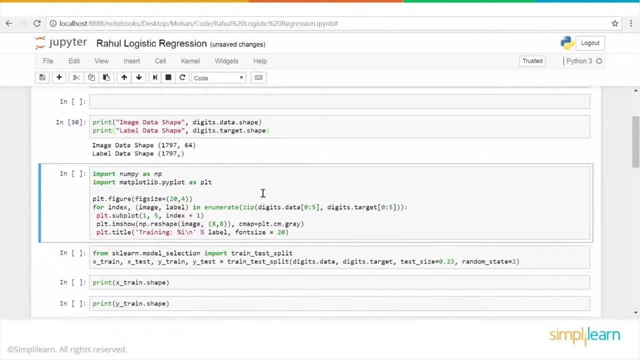 We are basically once again importing Some of the libraries that are required, Like numpy and matplot, And we will take a look at Some of the sample images That we have loaded. So this one, for example, Creates a figure And then we go ahead. 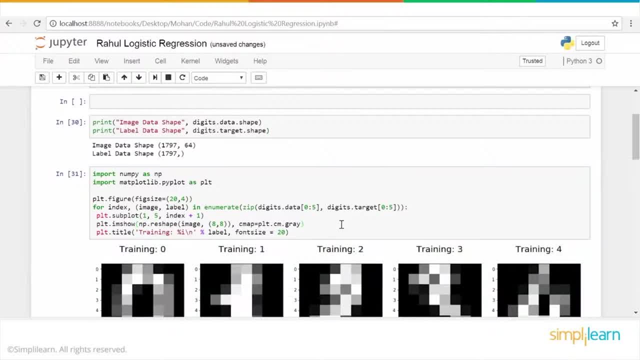 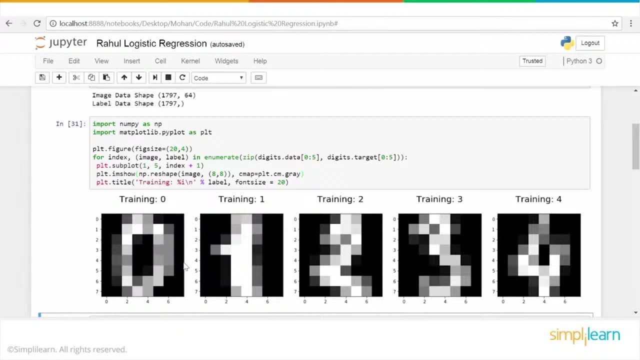 And take a few sample images To see how they look. So let me run this code So that it becomes easy to understand. So these are about 5 images, Sample images that we are looking at: 0,, 1,, 2,, 3,, 4.. 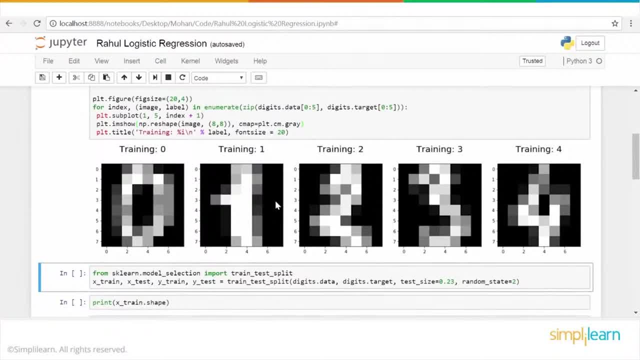 So this is how the images, This is how the data is, And based on this, We will run our logistic regression model And then we will test it And see how well it is able to recognize. So the way it works is. 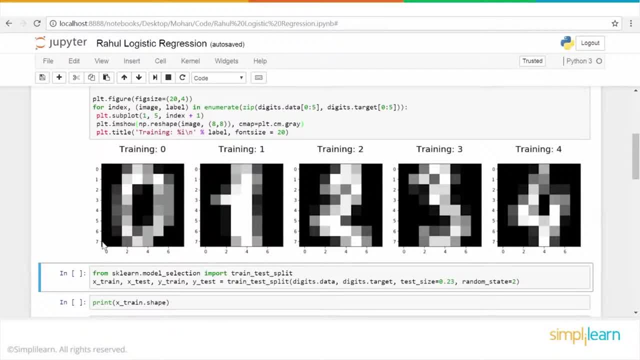 The pixel information. So, as you can see here, This is an 8 by 8 pixel Kind of a image And each pixel, Whether it is activated or not activated, That is the information Available for each pixel Now, based on the pattern. 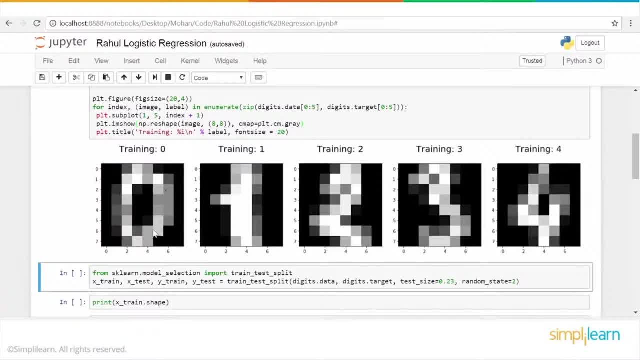 Of this activation and non activation Of the various pixels. It will be identified As a 0, for example, Similarly, as you can see. So overall, each of these numbers Actually has a different pattern Of the pixel activation, And that is pretty much. 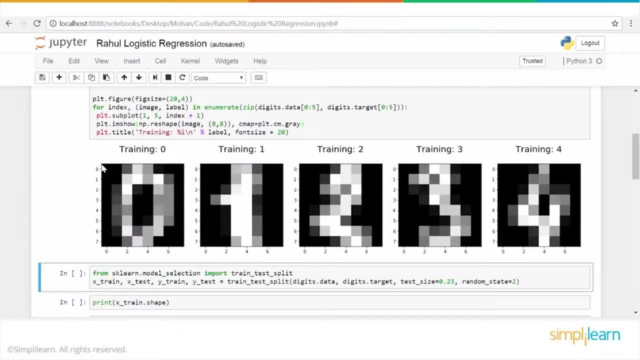 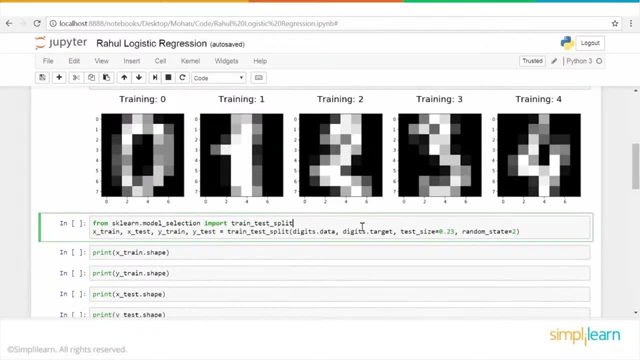 That our model needs to learn. For which number? What is the pattern of the activation of the pixels? Right, So that is what we are going to train our model. Okay, So the first thing we need to do Is to split our data. 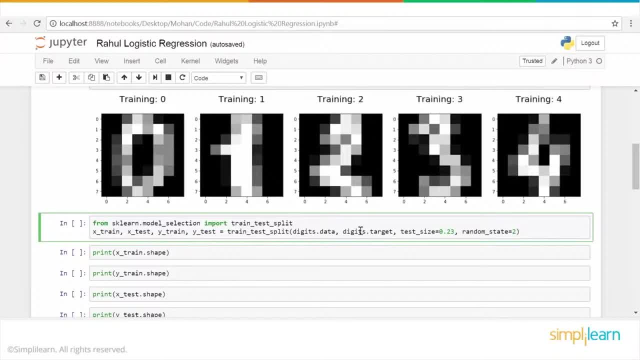 Into test data set Right. So whenever we perform any training, We split the data into training and test So that the training data set is used To train the system. So we pass this probably multiple times And then we test it with the test data set. 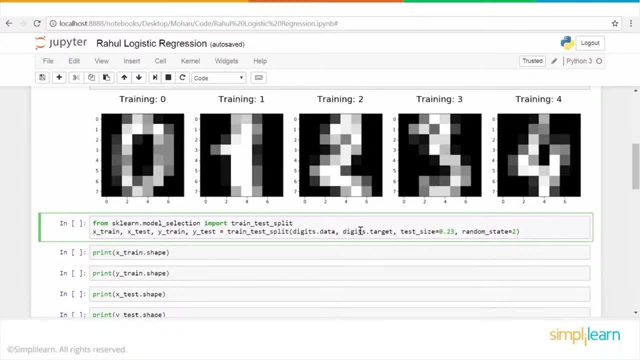 And the split is Usually in the form of. There are various ways in which you can split this data. It is up to the individual preferences. In our case, here We are splitting in the form of 23 and 77. So when we say test size, 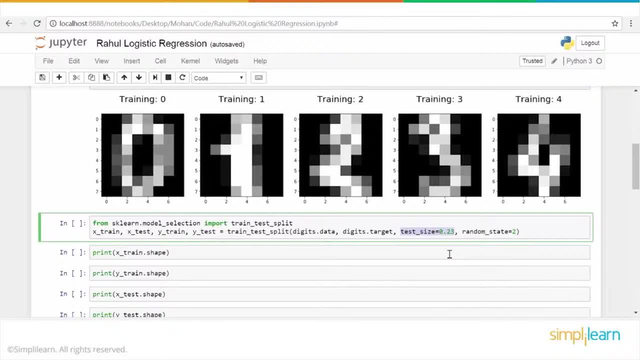 As 0.23.. That means 23 percent Of that entire data Is used for testing And the remaining 77 percent Is used for training. So there is a readily available function Which is called Train test split. So we don't have to write any special code. 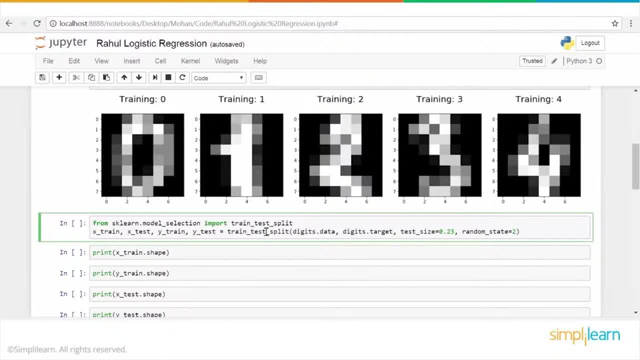 For the splitting. It will automatically split the data Based on the proportion that we give here, Which is test size. So the test size- Automatically, training size- will be determined And we pass the data that we want to split And the results will be stored in. 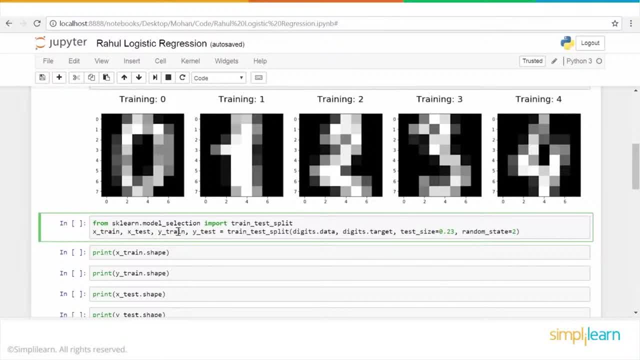 X underscore train And Y underscore train For the training data set. And what is X underscore train? These are the features, Which is like the independent variable And Y underscore train Is the label. So in this case, What happens is: 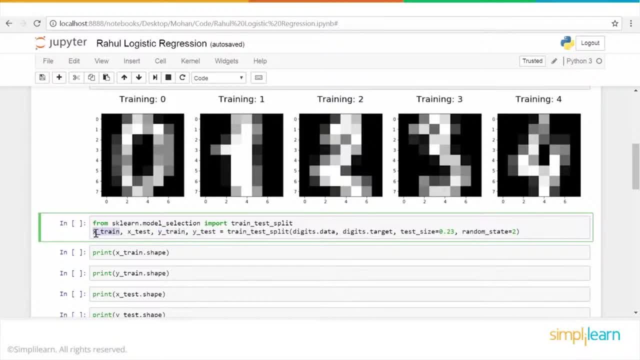 We have the input value, Which is in X underscore train, And since this is labeled data, For each of them, Each of the observations, We already have the label information Saying whether this digit is a zero Or a one Or a two. 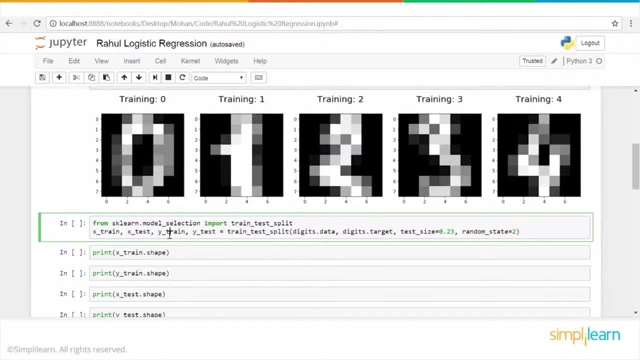 So this is what will be used for comparison To find out whether the system is able to Recognize it correctly Or there is an error. For each observation, it will compare with this. So this is the label. So the same way. 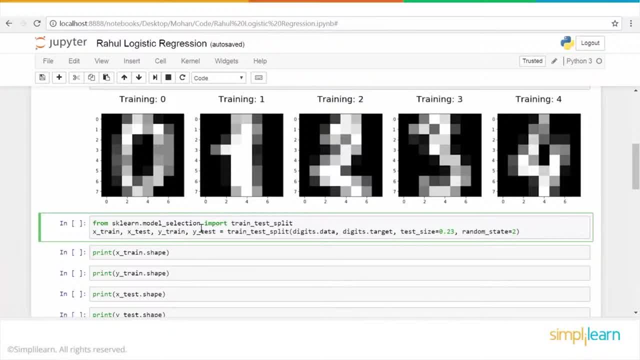 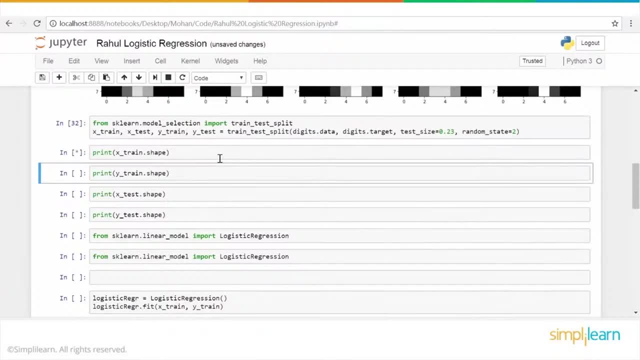 For the training data set. X underscore test. Y underscore test Is for the test data set. So let me go ahead and execute this code as well, And then we can go and check quickly. What is the? How many entries are there? 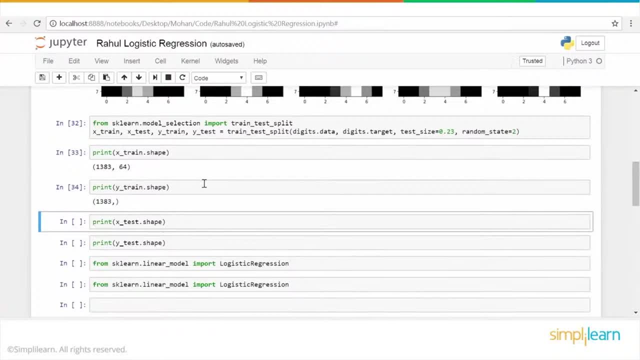 And in each of these, So X underscore train, The shape is 1383 by 64.. And Y underscore train has 1383.. Because there is nothing like The second part is not required here. And then X underscore train is 414.. 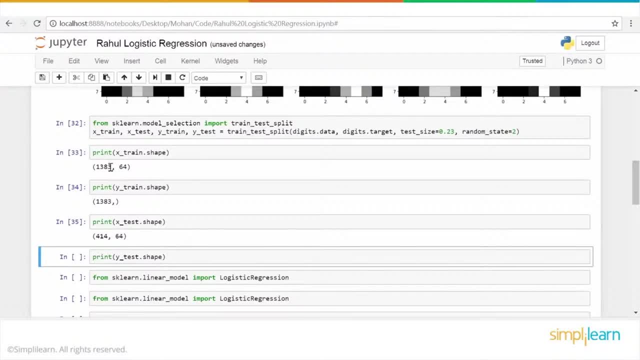 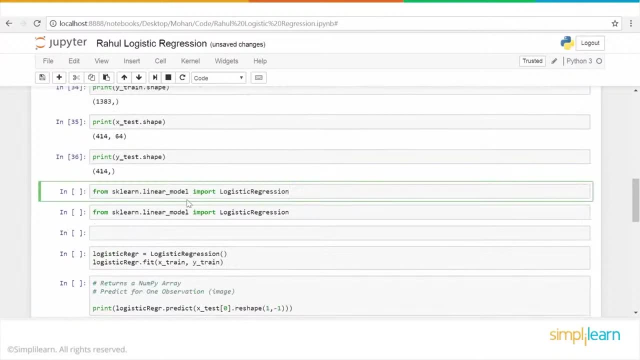 So actually there are 414 observations In test And 1383 observations in train. So that's basically What these four lines of code are saying. Okay, Then we import the Logistic regression library And which is a part of scikit learn. 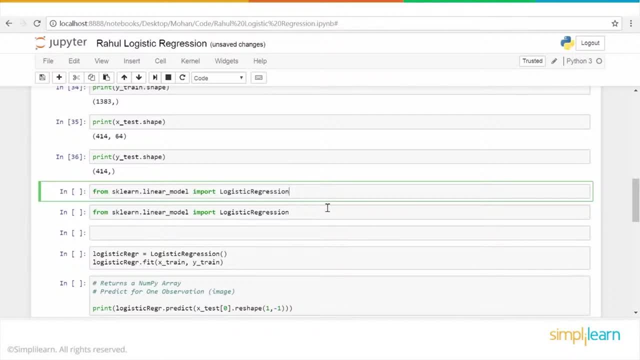 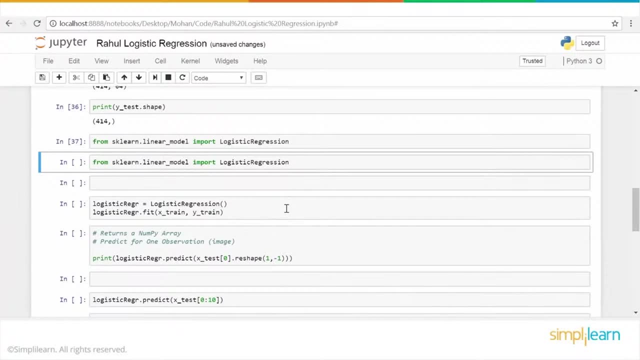 So we don't have to implement The logistic regression process itself. We just call these the function, And let me go ahead and execute that So that We have the logistic regression Library imported. Now we create an instance of logistic regression. 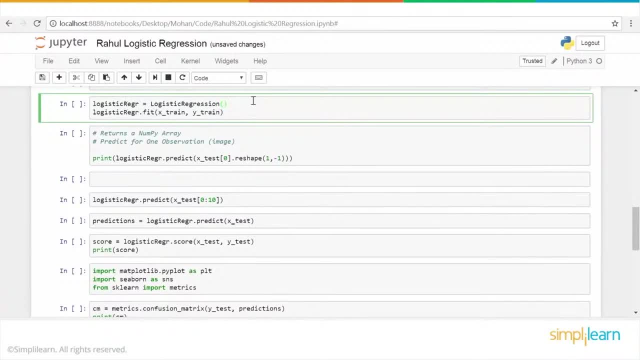 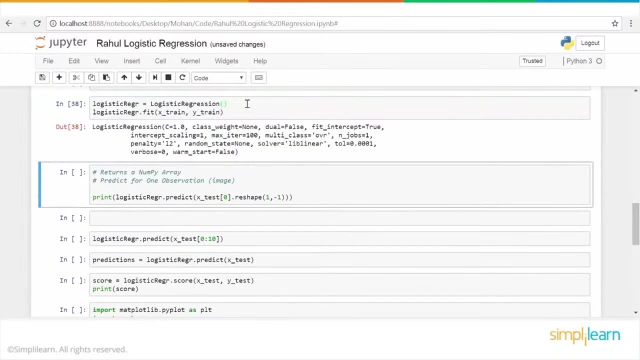 Right, So logistic R E G R Is an instance of logistic regression And then we use that For training our model. So let me first execute this code. So these two lines, So the first line- Basically creates an instance of logistic regression model. 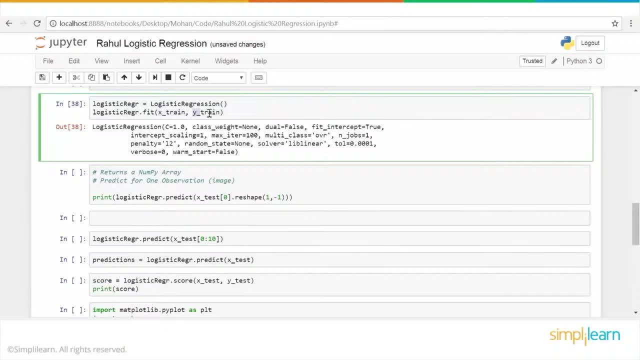 And then the second line Is where we are passing Our data To the predictors, And this is our target. We are passing this data set To train our model. So once we do this, In this case the data is not large. 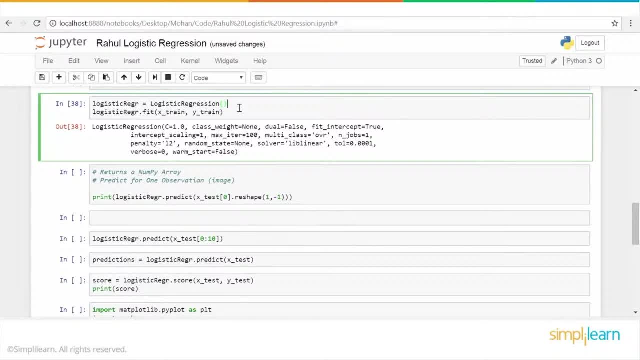 But by and large The training is what takes usually a lot of time. So we spend in machine learning Activities, in machine learning projects We spend a lot of time For the training part of it. So here the data set is relatively small. 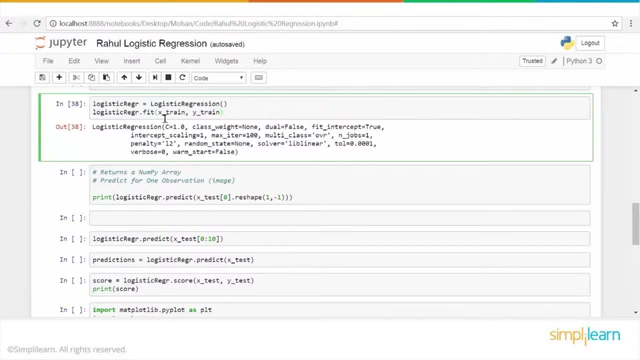 So it was pretty quick. So now our model has been trained Using the training data set And we want to see How accurate this is. So what we will do is We will test it out in probably phases, So let me first try out. 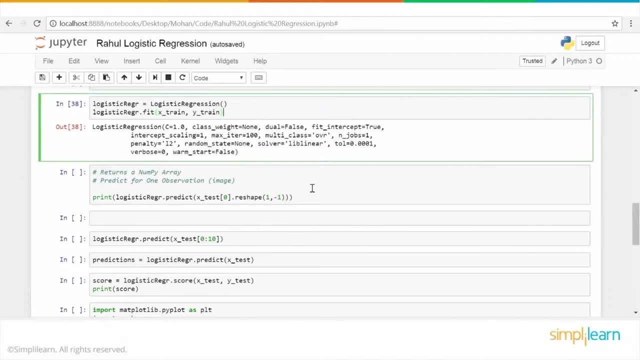 How well this is working for One image. I will just try it out with one image, The first entry in my test data set, And see whether it is Correctly predicting or not, And in order to test it, So for training purpose. 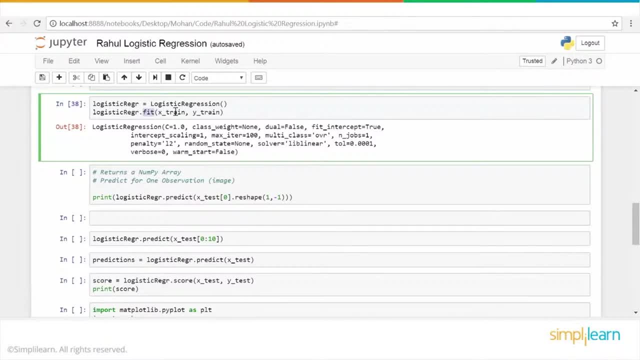 We will use a fit method. There is a method called fit, Which is for training the model And once the training is done, If you want to test for a particular value, New input- You use the predict method. So let's run the predict method. 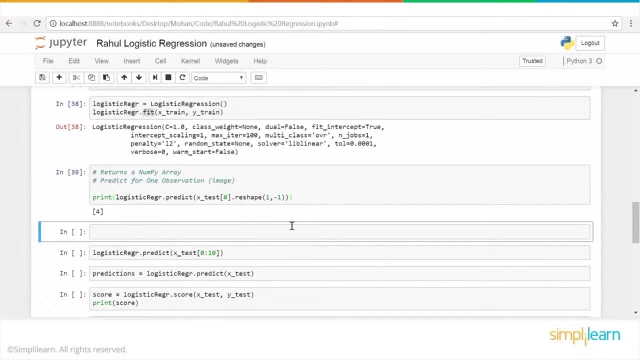 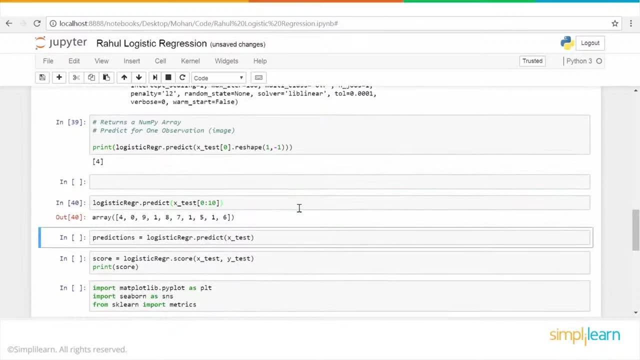 And we pass this particular image And we see that The shape is, Or the prediction is, 4.. So let's try a few more. Let me see for the next 10.. Seems to be fine, Let me just go ahead. 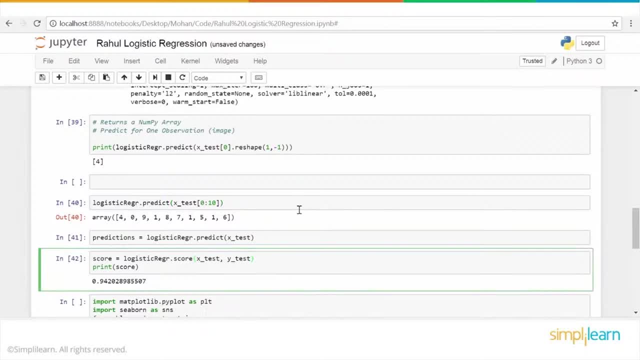 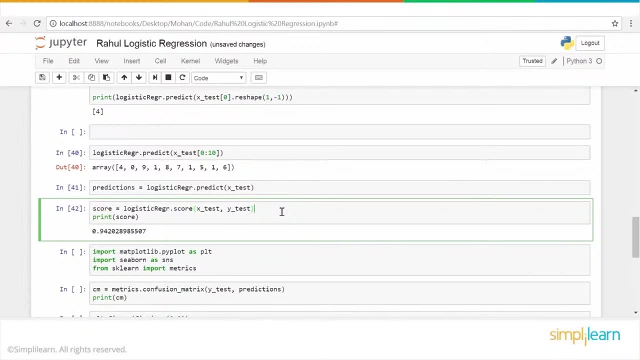 And test the entire data set. That's basically what we will do. So now we want to find out How accurately this has performed. So we use the score method To find what is the percentage Of accuracy, And we see here that it has. 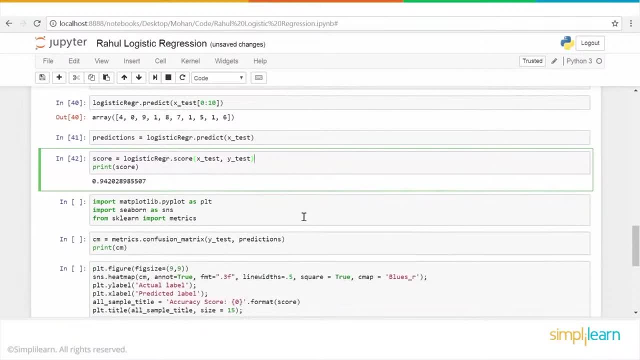 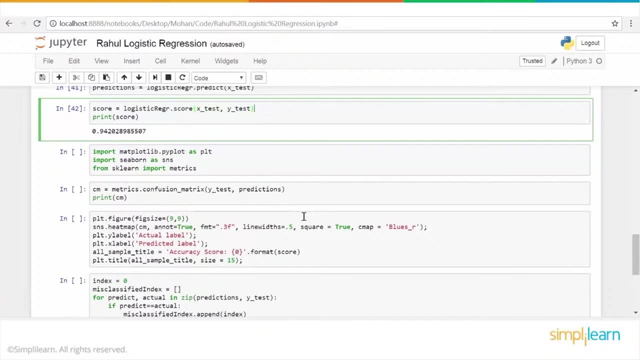 Performed up to 94% accurate. So that's on this part. Now, what we can also do is We can also see this accuracy Using what is known as Confusion matrix, And try that as well, So that we can also visualize. 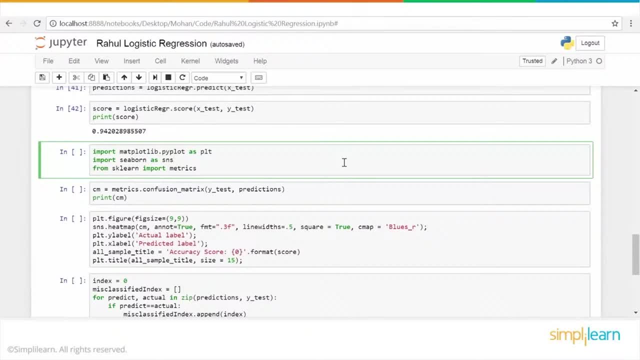 How well this model Has done. So let me execute this piece of code, Which will basically import Some of the libraries that are required, And we basically create A confusion matrix, An instance of confusion matrix, By running confusion matrix And passing these values. 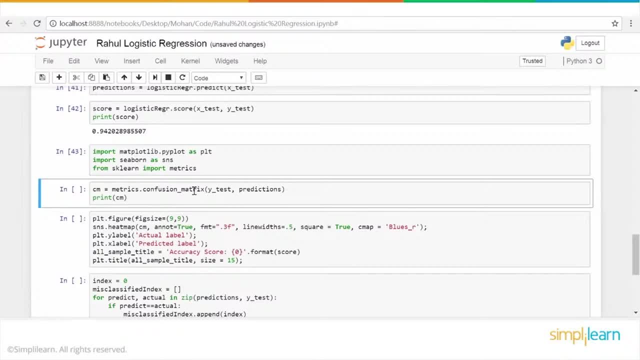 So we have So this confusion- underscore Matrix method And we have Three parameters: One is the y underscore test And the other is the prediction. So what is the y underscore test? These are the labeled values, Which we already know. 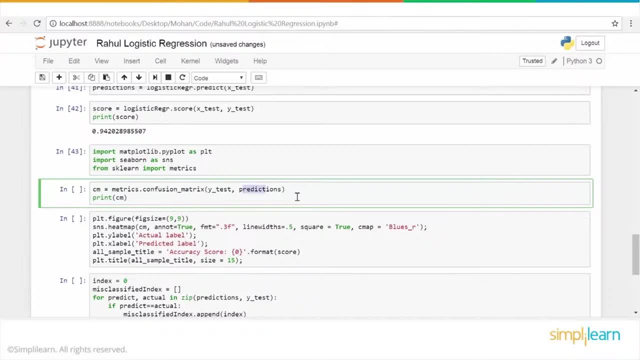 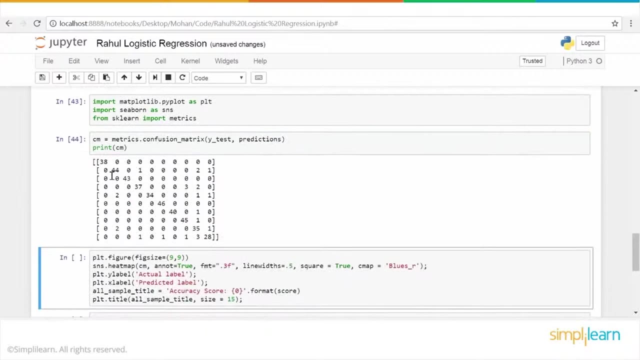 For the test data set And predictions are what The system has predicted For the test data set. Okay, So this is known to us And this is what the system has. The model has generated The confusion matrix looks As the name suggests. 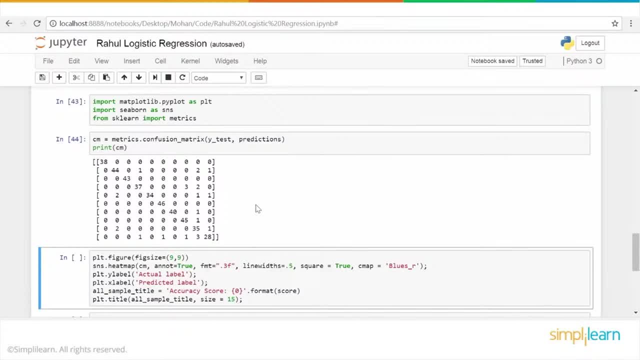 It is a matrix And the key point out here Is that the accuracy of the model Is determined by how many numbers Are there in the diagonal. The more the numbers in the diagonal, The better the accuracy is Okay. And first of all, 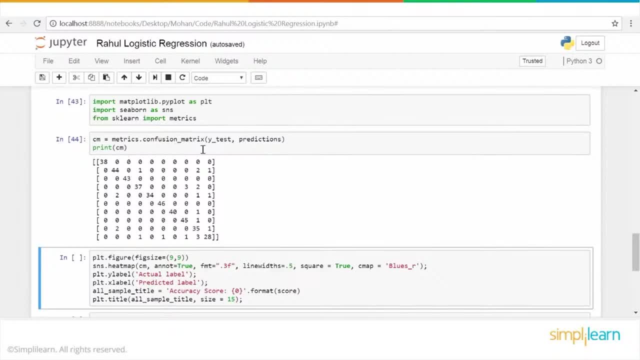 The total sum of all the numbers In this whole matrix Is equal to the number of observations In the test data set. That will be equal to the number of Observations in the test data set And then out of that The maximum number of them. 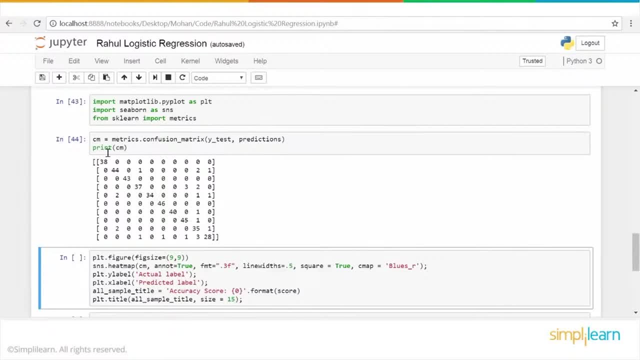 Should be in the diagonal. That means the accuracy is pretty good. If the numbers in the diagonal are less- And in all other places There are a lot of numbers, Which means the accuracy is very low- The diagonal indicates a correct prediction. 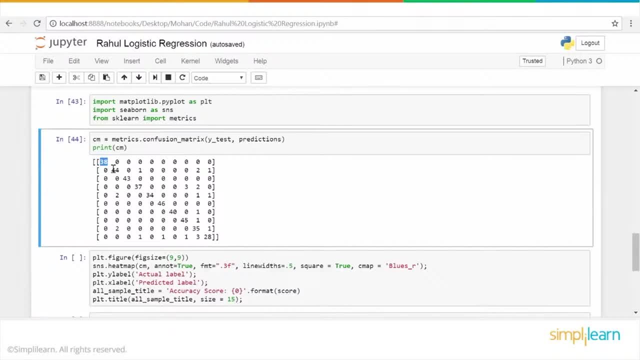 This means that the actual value Is same as the predicted value. Here again, Actual value is same as the predicted value. You see a number here. That means the actual value is something And the predicted value is something else, Right? Similarly here. 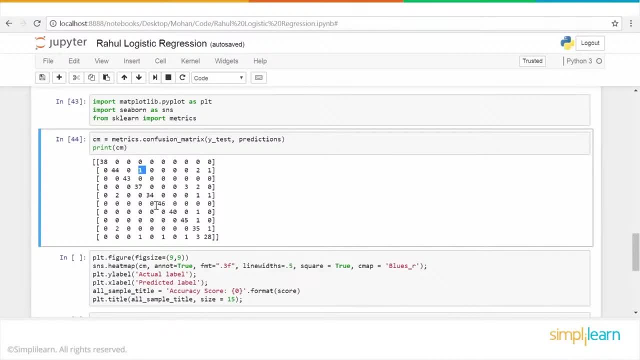 The actual value is something And the predicted value is something else. So that is basically How we read the confusion matrix. Now how do we find the accuracy? You can actually add up the Total values in the diagonal, So it's like 38 plus 44 plus 43.. 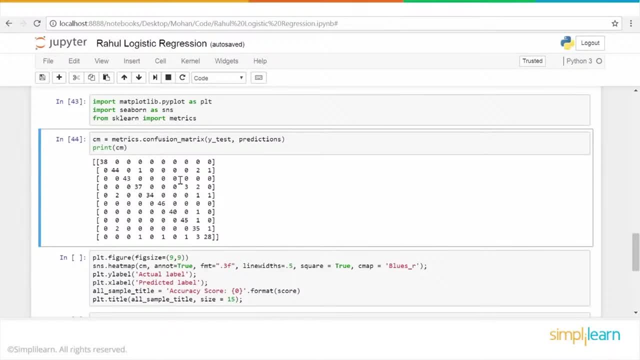 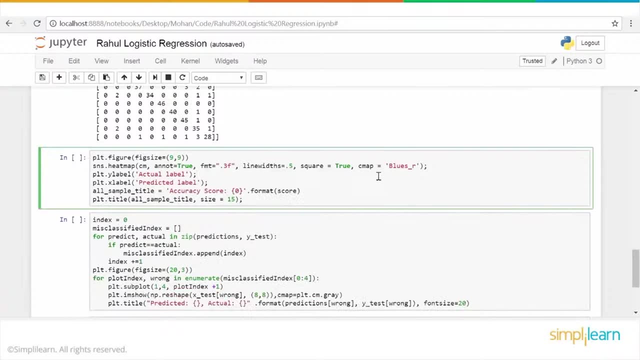 And so on, And divide that And you can see That we get the, The percentage accuracy, Using the confusion matrix. Now let us visualize this confusion matrix In a slightly more sophisticated way, Using a heat map. So we will create a heat map. 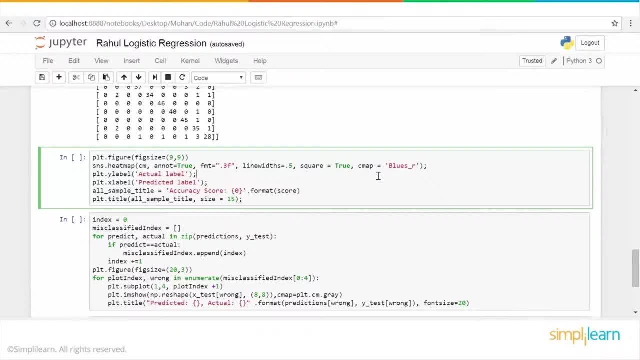 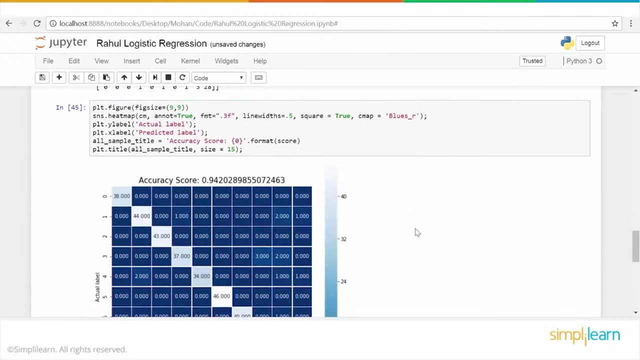 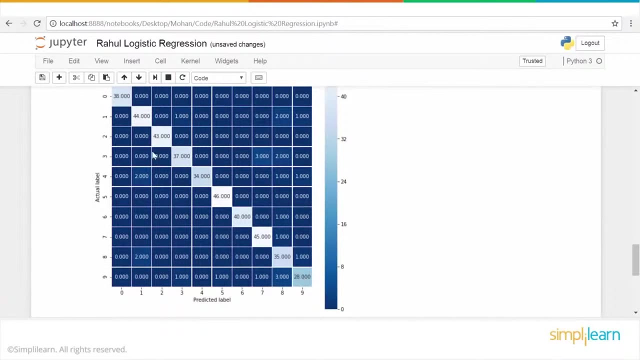 With some, We'll add some colors as well. It's like a more visually, Visually more appealing. So that's the whole idea. So if we Let me run this piece of code: Diagonals: again, All the values are here. 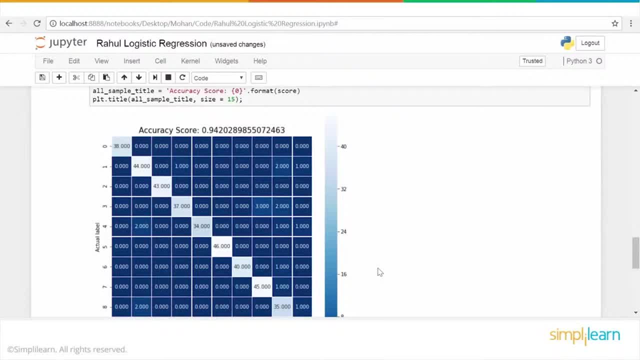 Most of the values, Which means reasonably. This seems to be reasonably accurate. And, yeah, Basically the accuracy score is 94%. This is calculated, as I mentioned, By adding all these numbers Divided by the total test values Or the total number of observations. 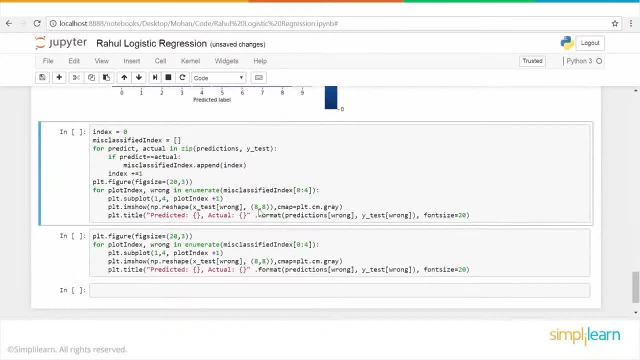 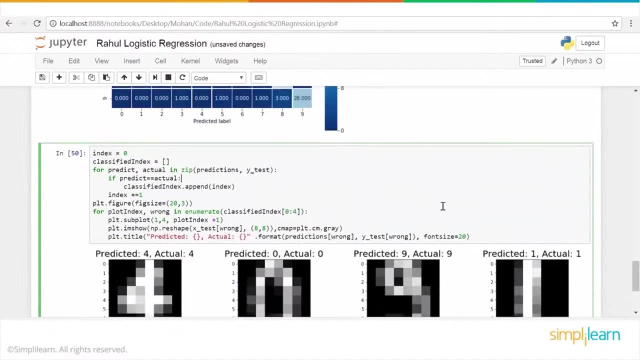 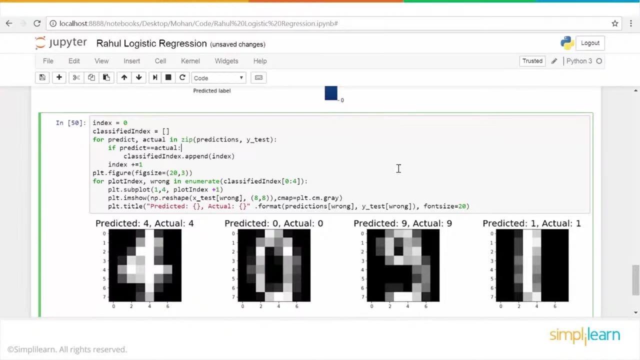 In test data set. Okay, So this is the confusion matrix. So now that we have seen The confusion matrix, Let's take a quick sample And see how well The system has classified, And we will take a few examples Of the data. 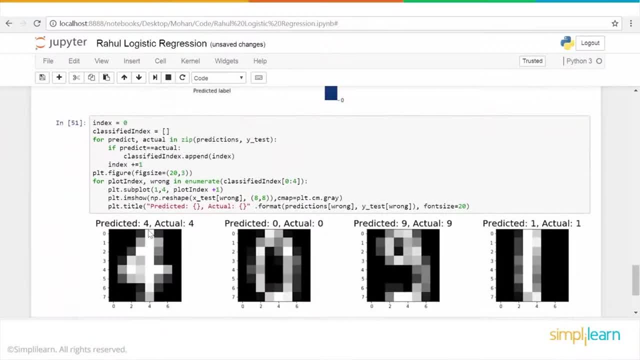 So if we see here, We picked up randomly a few of them. So this is number four, Which is the actual value And also the predicted value. Both are four. This is an image of zero, So the predicted value is also zero. 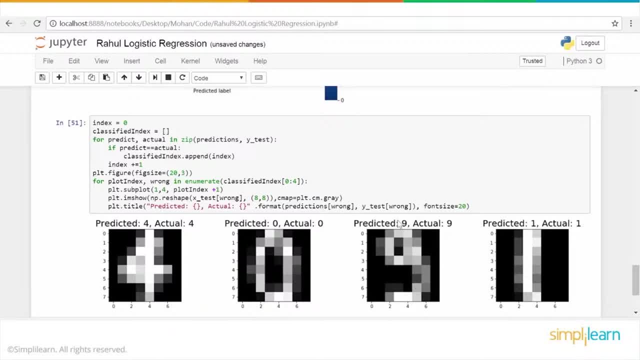 This is the image of nine, So this has also been predicted correctly: Nine And the actual value is nine. And this is the image of one And again, this has been predicted correctly, As like the actual value. So this was a quick demo. 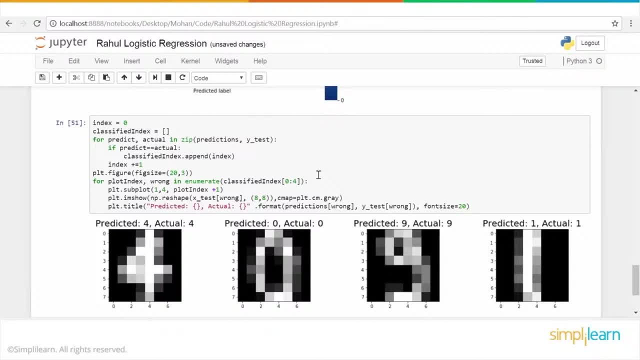 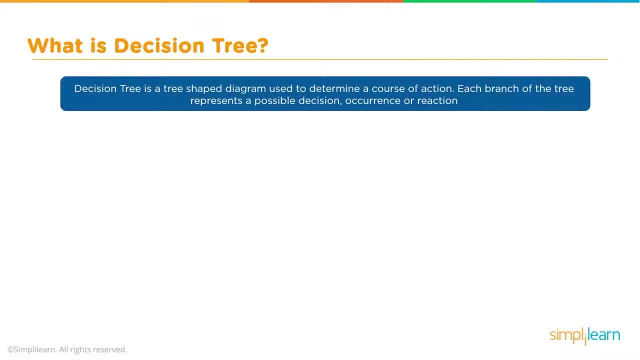 Of logistic regression: How to use logistic regression To identify images. What is a decision tree? Let's go through a very simple example Before we dig in deep. Decision tree is a tree shaped diagram Of action. Each branch of the tree represents a possible decision. 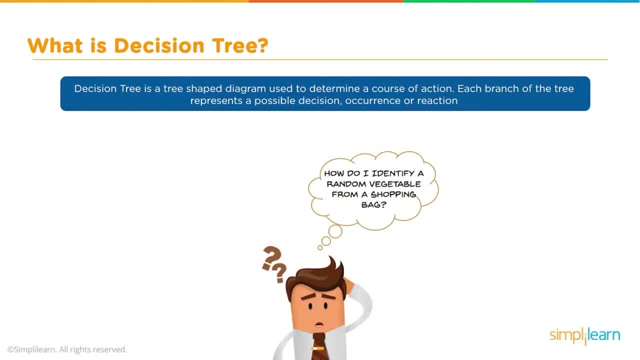 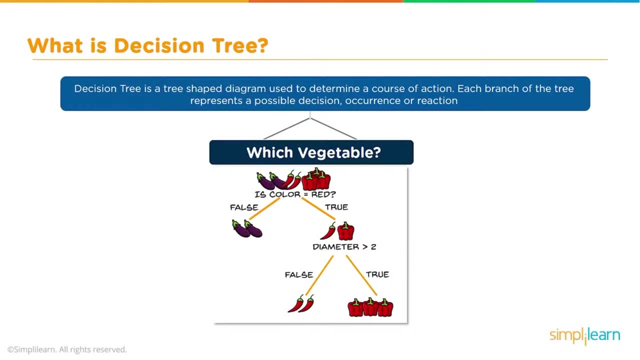 Or occurrence Or reaction. Let's start with a simple question: How to identify a random vegetable from a shopping bag? So we have this group of vegetables in here And we can start off by asking a simple question: Is it red? And if it's not, 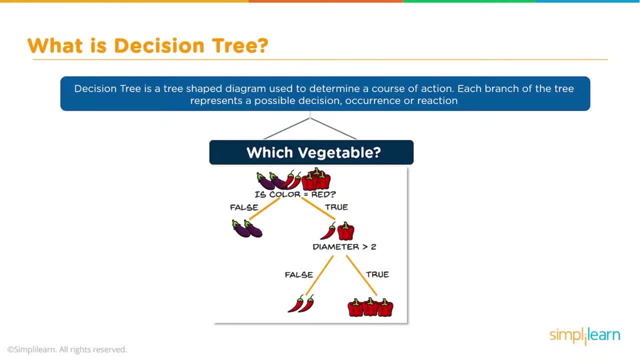 Then it's going to be the purple fruit to the left, Probably an eggplant. If it's true, It's going to be one of the red fruits. Is the diameter greater than two? It's a capsicum family, So it's a capsicum. 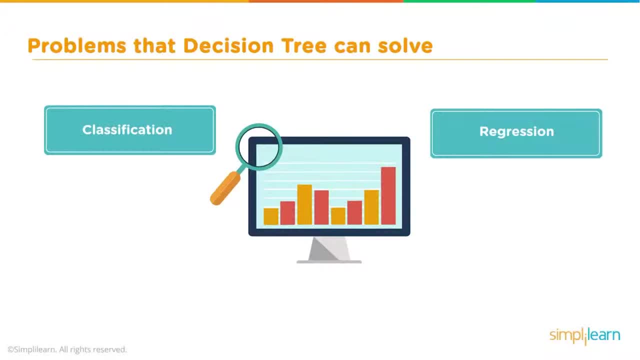 Problems that decision tree can solve. So let's look at the two different categories The decision tree can be used on. It can be used on the classification, The true, false, yes, no. And it can be used on regression, Where we figure out what the next value is. 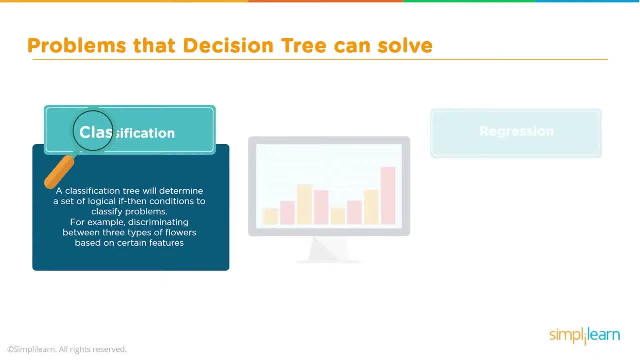 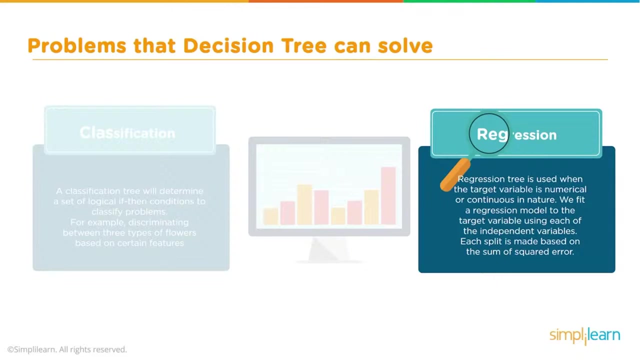 In a series of numbers Or a group of data. In classification, The classification tree will determine a set of logical, If then conditions to classify problems. For example, If we want to solve a problem based on certain features In regression, A regression tree is used when the target variable 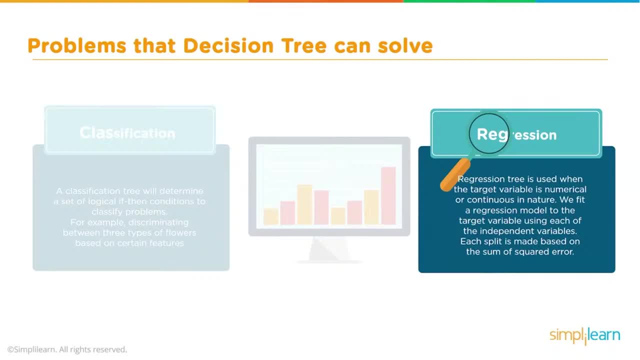 Is numerical or continuous in nature, We fit the regression model to the target variable Using each of the independent variables. Each split is made based on the sum Of squared error. Before we dig deeper Into the mechanics of the decision tree, Let's take a look at the advantages. 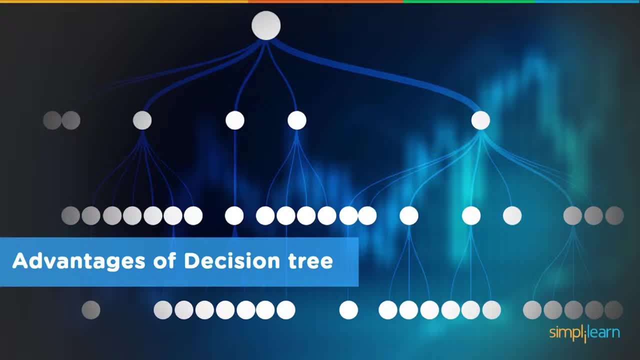 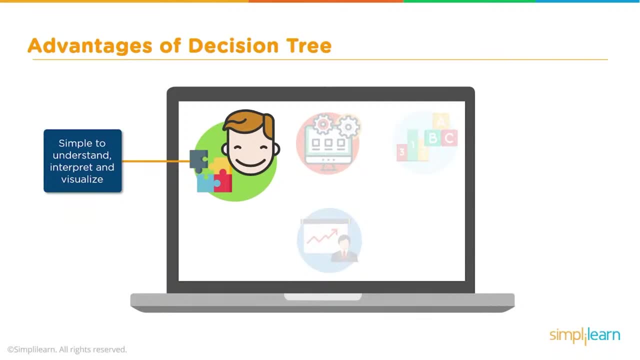 Of using a decision tree And we'll also take a glimpse at the disadvantages. The first thing you'll notice Is that it's simple to understand, Interpret and visualize. It really shines here Because you can see exactly what's going on in a decision tree. 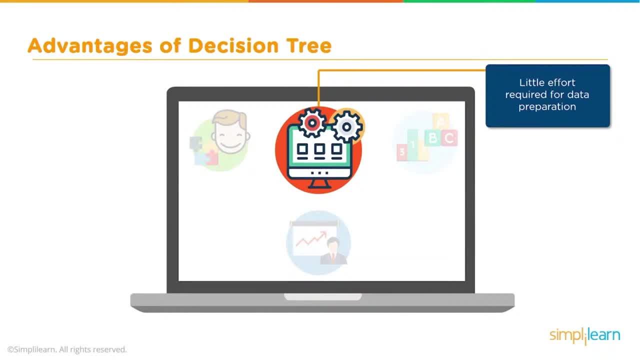 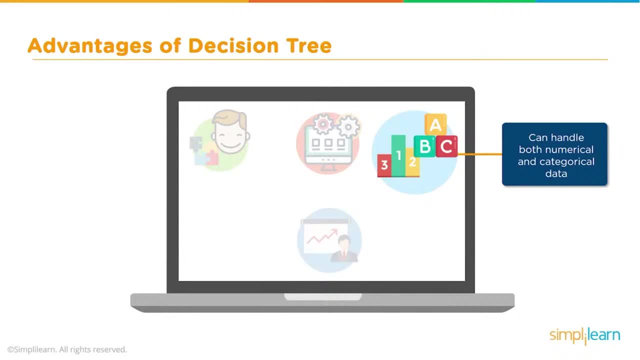 Little effort is required for data preparation, So you don't have to do special scaling. There's a lot of things you don't have to worry about When using a decision tree. It can handle both numerical and categorical data, As we discovered earlier. 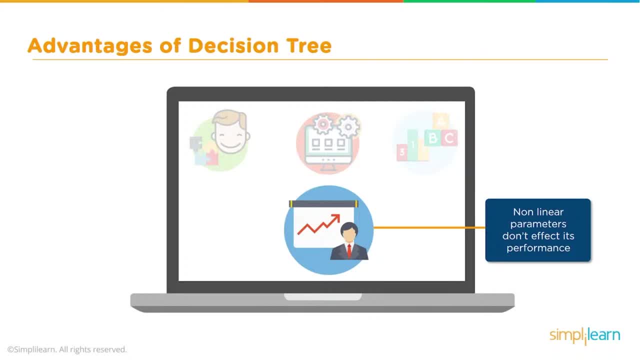 And non-linear parameters Don't affect its performance. So even if the data doesn't fit An easy curved graph, You can still use it to create an effective decision Or predict If we're going to look at the advantages Of a decision tree. 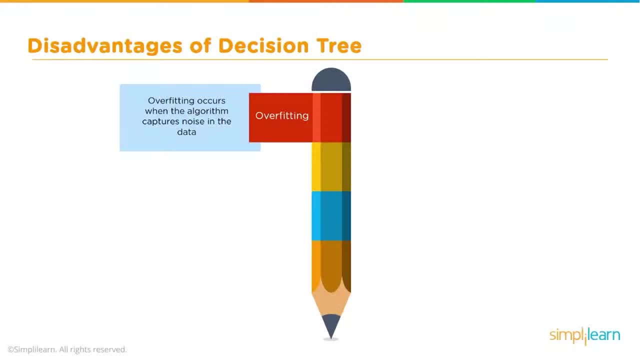 We also need to understand the disadvantages Of a decision tree. The first disadvantage is overfitting. Overfitting occurs when the algorithm Captures noise in the data. That means you're solving for one specific instance Instead of a general solution. 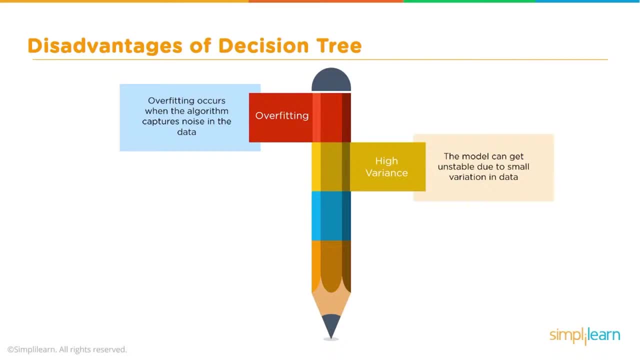 For all the data. High variance. The model can get unstable due to small variation in data. Low bias tree: A highly complicated decision tree Tends to have a low bias, So we need to work with new data Decision tree. important terms. 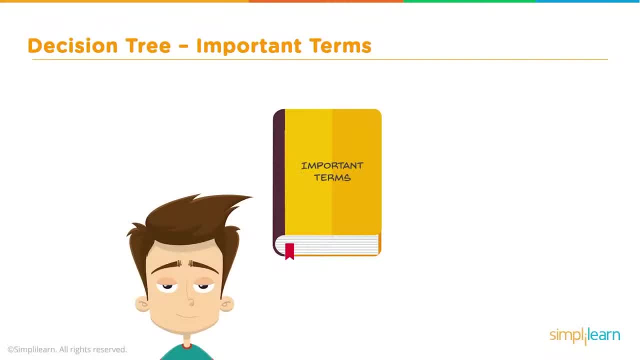 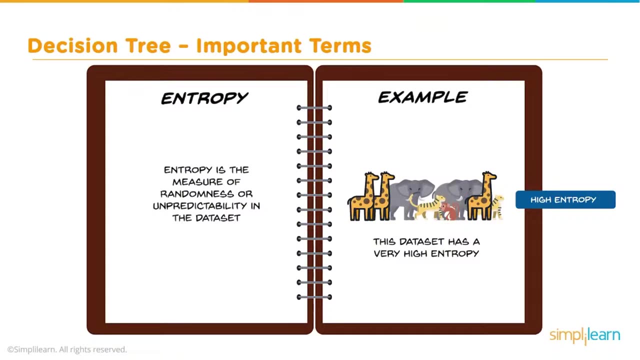 Before we dive in further, We need to look at some basic terms. We need to have some definitions To go with our decision tree And the different parts we're going to be using. We'll start with entropy. Entropy is a measure of randomness. 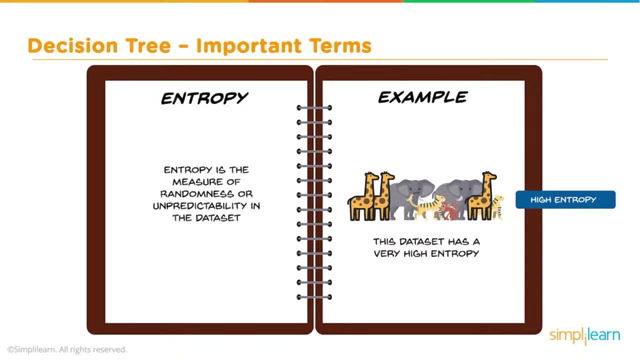 Or unpredictability in the data set. For example, We have a group of animals. In this picture There's four different kinds of animals And this data set is considered to have a high entropy Based on looking at just the four animals. 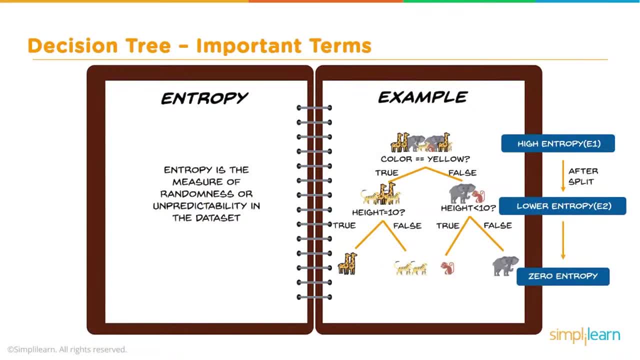 As a big clump of entities. So as we start splitting it into subgroups, We come up with our second definition, Which is information gain. Information gain: It is a measure of decrease in entropy After the data set is split. So in this case, 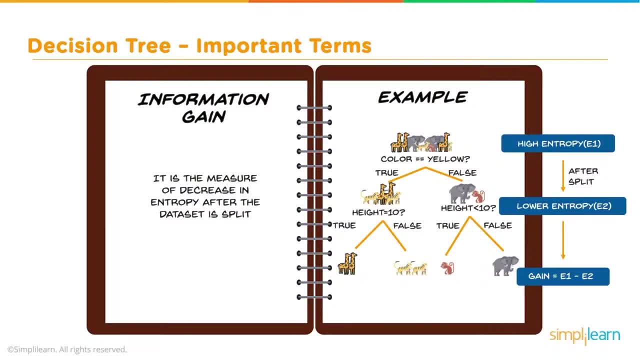 Based on the color yellow, We've split one group of animals on one side As true, and those who aren't yellow as false. As we continue down the yellow side, We split based on the height, As true or false equals 10.. 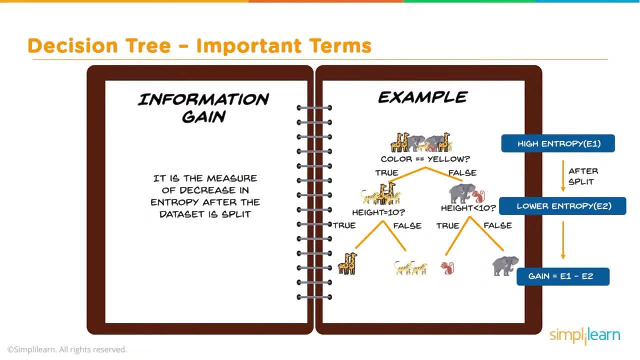 And on the other side, Height is less than 10.. True or false? And, as you see, as we split it, The entropy continues to be less and less and less, And so our information gain is simply the entropy, E1 from the top. 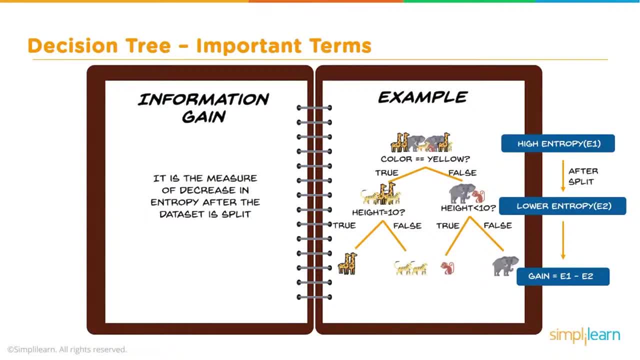 And how it's changed to E2 in the bottom, And we'll look at the deeper math, Although you really don't need to know a huge amount of math When you actually do the programming in Python, Because it will do it for you. 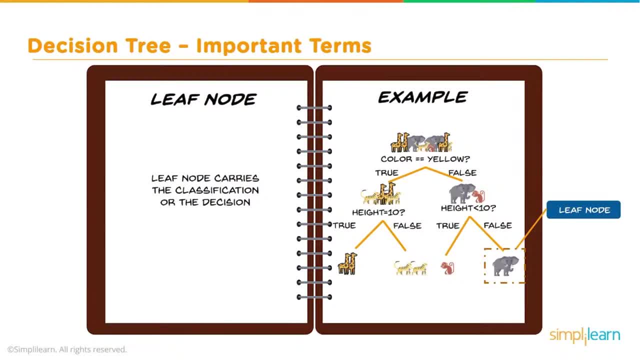 But we'll look on the actual math And how they compute entropy. This node carries the classification or the decision, So it's the final end at the bottom. The decision node Has two or more branches. This is where we're breaking the group up into different parts. 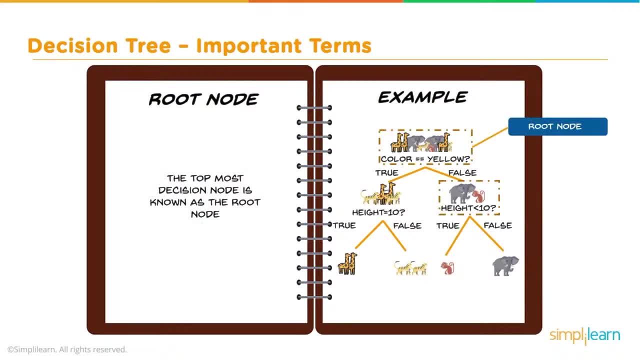 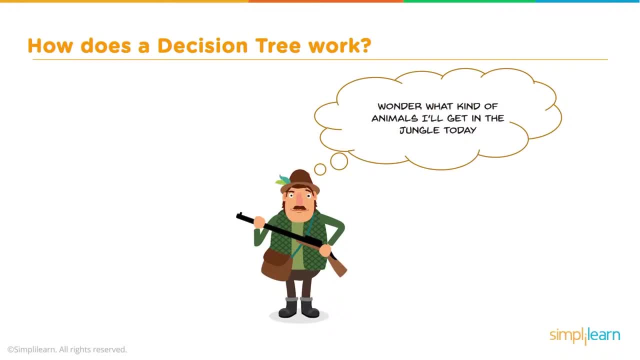 And finally you have the root node. The top most decision node Is known as the root node. How does a decision tree work? Wonder what kind of animals I'll get the jungle today. Maybe you're the hunter with the gun, Or if you're more into photography, 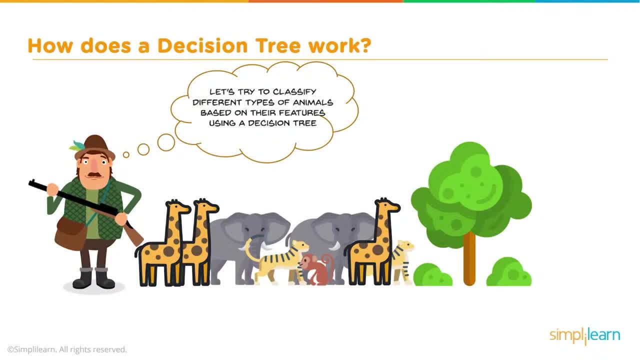 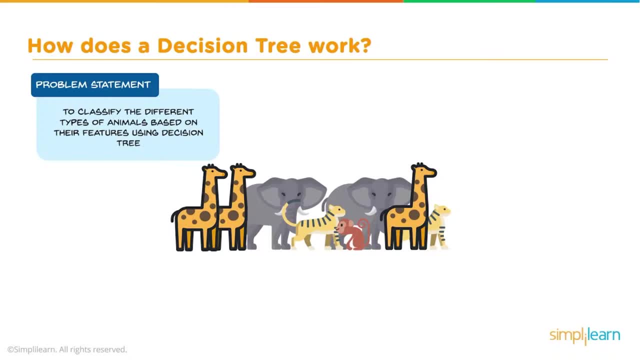 You're a photographer with a camera, So let's look at this group of animals. These are different types of animals Based on their features using a decision tree. So the problem statement is To classify the different types of animals Based on their features using a decision tree. 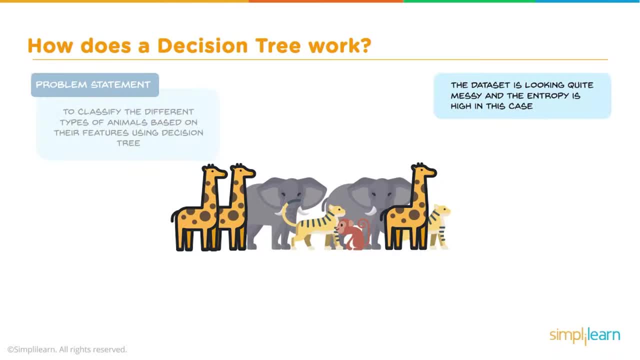 The data set is looking quite messy And the entropy is high in this case. So let's look at a training set Or a training data set, And we're looking at color, We're looking at height, And then we have our different animals. 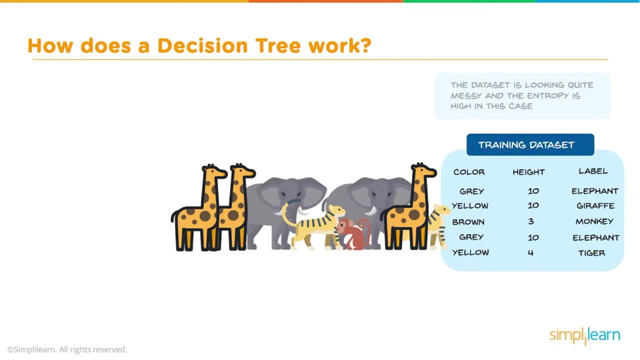 We have our elephants, our giraffes, our monkeys and our tigers, And they're of different colors and shapes. Let's see what that looks like. We have to frame the conditions That split the data in such a way That the information gain is the highest. 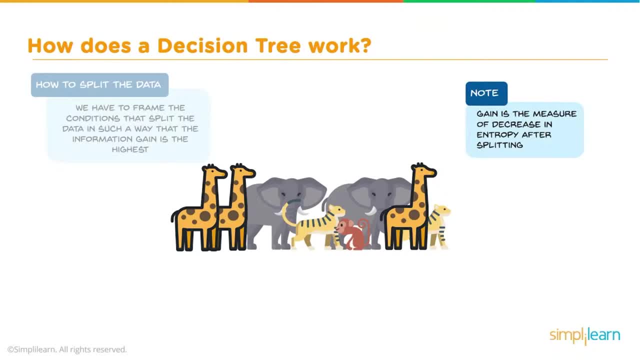 Note: Gain is the measure of decrease in entropy After splitting. So the formula for entropy is the sum. That's what this symbol looks like. It looks kind of like a funky E Of K, Where I equals 1 to K. 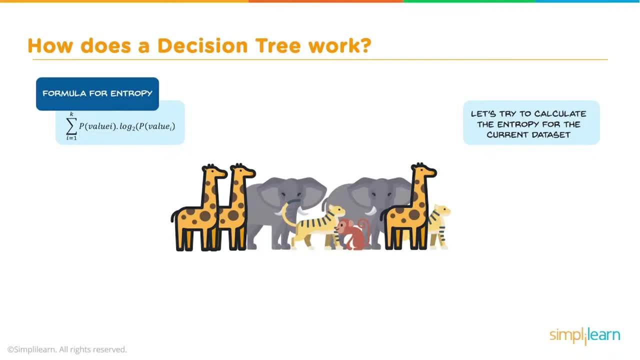 K would represent the number of animals, The different animals in there, Where value or P Value of I, Value of I is the log base 2 of the same, The percentage of that animal. Let's try to calculate the entropy for the current data set. 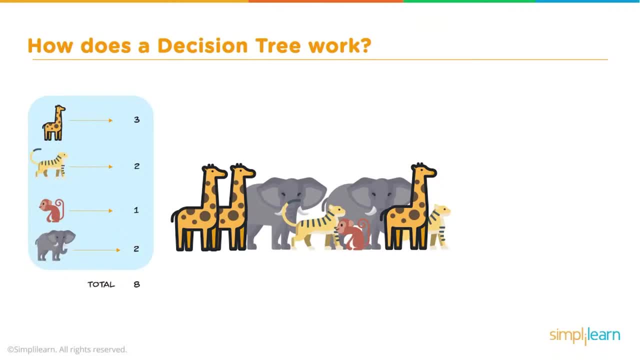 And take a look at what that looks like And don't be afraid of the math. You don't really have to memorize this math, Just be aware that it's there And this is what's going on in the background. And so we have 3 giraffes. 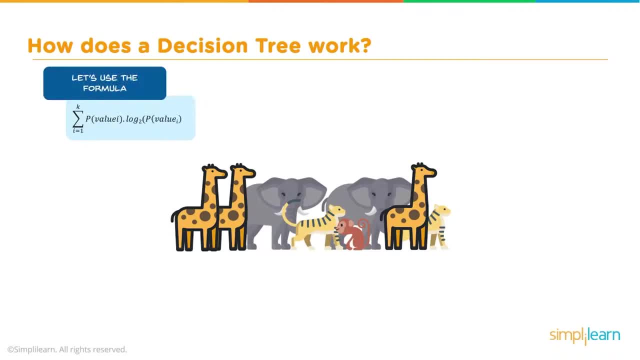 2 tigers, 1 monkey, 2 elephants- A total of 8 animals gathered And if we plug that into the formula, 2 elephants over a total of 8.. Times the log: Usually they use base 2 on the log. 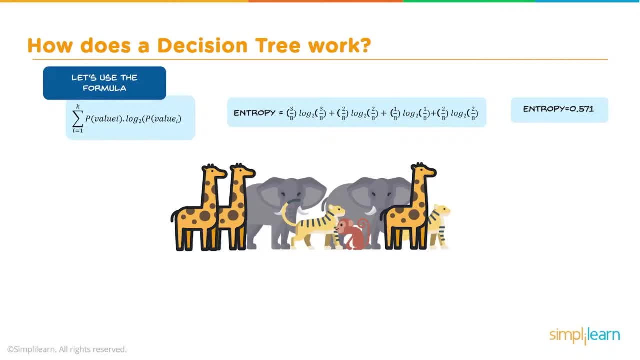 So log base 2 of 3 over 8.. Plus, In this case let's say it's the elephants, 2 over 8. 2 elephants over a total of 8. Times log base 2. 2 over 8.. 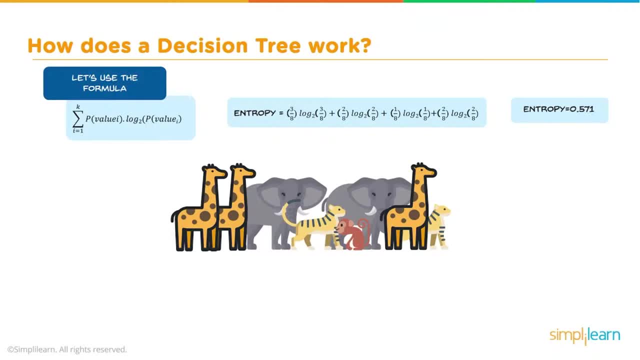 Plus 1 monkey over a total of 8. Log base 2. 1 over 8. And plus 2 over 8 of the tigers. Log base 2 over 8. Plus 1 over 8.. The program will actually calculate the entropy of the data set. 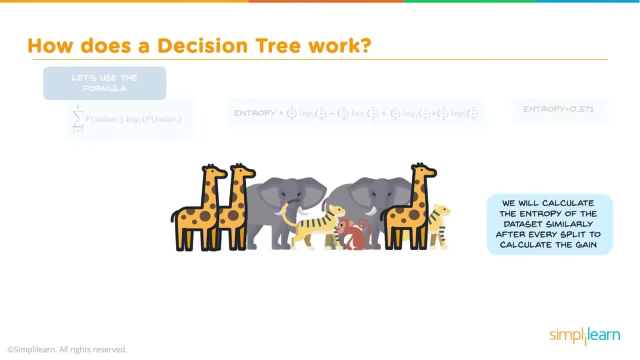 similarly after every split, to calculate the gain. Now we're not going to go through each set, one at a time, to see what those numbers are. We just want you to be aware that this is a formula or the mathematics behind it. Gain can be calculated by finding the difference. 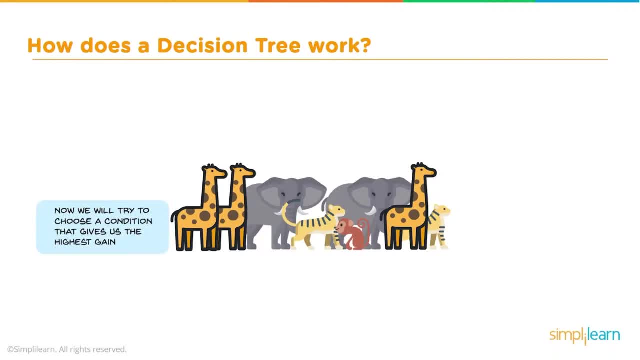 of the subsequent entropy values after a split. Now we will try to choose a condition that gives us the highest gain. We will do that by splitting the data using each condition and checking that the gain we get out of them, The highest gain, will be used to make the first split. 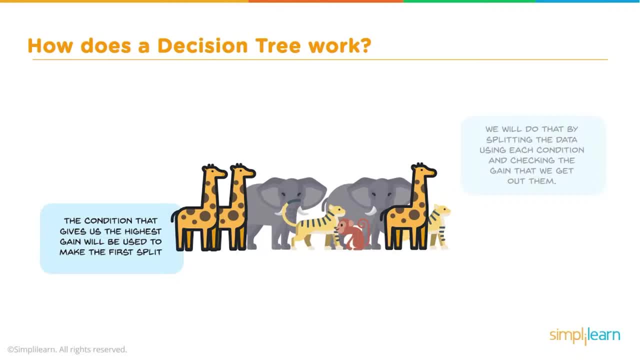 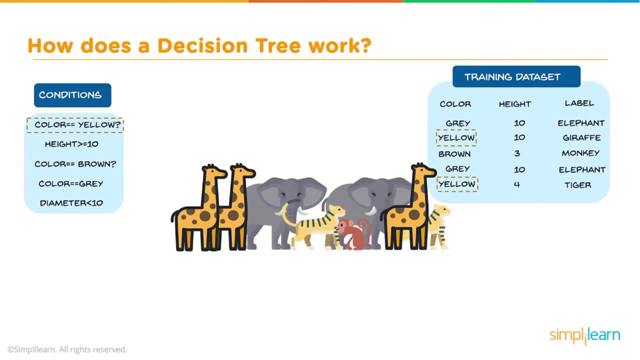 Can you guess what that first split will be? just by looking at this image, As a human, it's probably pretty easy to split it. Let's see if you're right. If you guessed the color yellow, you're correct. Let's say the condition that gives us the maximum gain. 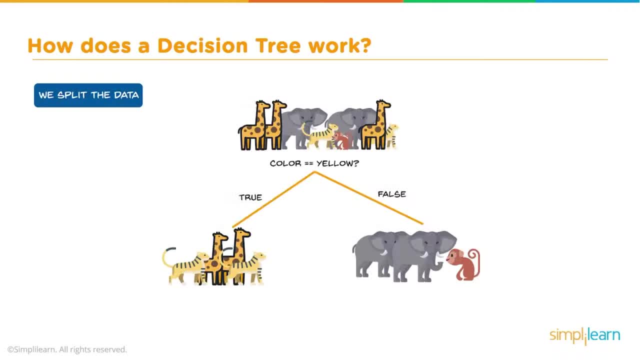 is yellow. So we will split the data based on the color yellow. If it's true, that group of animals goes to the left. If it's false, it goes to the right. The entropy after the splitting has decreased considerably. However, we still need some splitting. 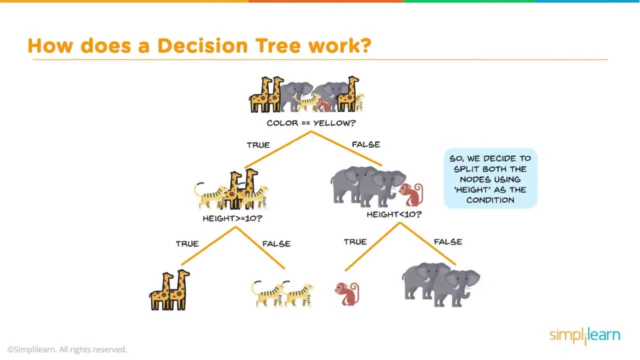 at both the branches to attain an entropy value equal to zero. So we decide to split both the nodes, using height as the condition. Since every branch now contains single label type, we can say that entropy, in this case, has reached the least value. And here you see, we have the giraffes, the tigers. 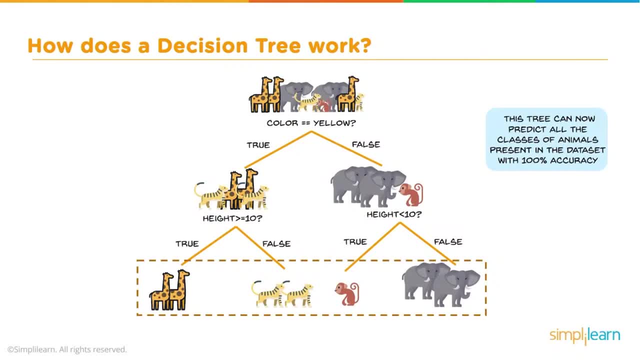 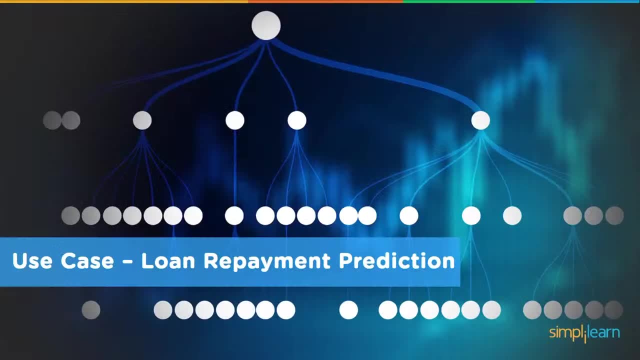 the monkey and the elephants, all separated into their own groups. This tree can now predict all the classes of animals present in the data set with 100% accuracy. That was easy Use Case. Let's get into my favorite part and open up some Python. 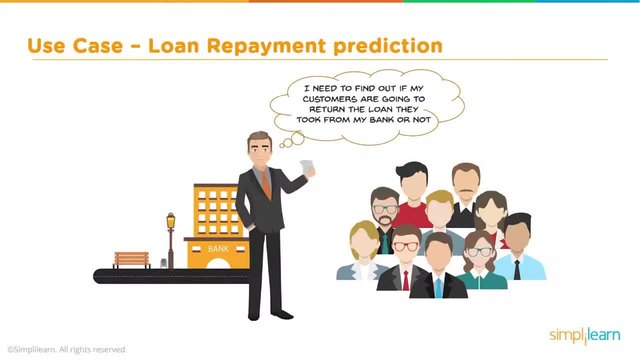 and see what the programming code and the scripting looks like. In here we're going to want to do a prediction, And we start with this individual here who's requesting to find out how good his customers are going to be, whether they're going to repay their loan or not. 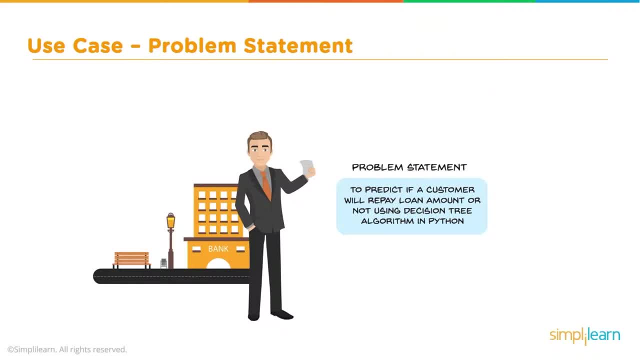 for his bank, And from that we want to generate a problem statement to predict if a customer will repay a loan amount or not. And then we're going to be using the decision tree algorithm in Python. Let's see what that looks like and let's dive into the code. 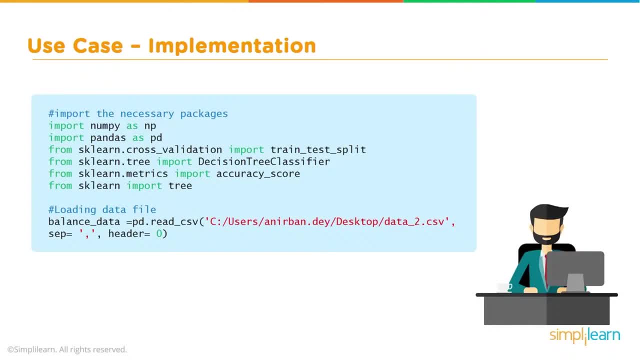 For the first steps of implementation. we're going to start by importing the necessary packages that we need from Python and we're going to load up our data and take a look at what the data looks like. So the first thing I need is: I need something to edit my Python. 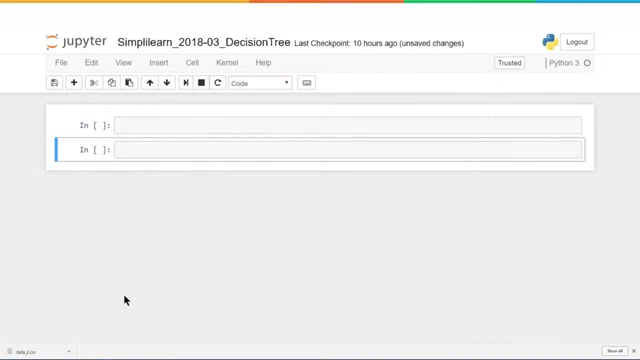 and run it in. So let's flip on over, And here I'm using the Anaconda Jupyter notebook. Now you can use any Python IDE you like to run it in, but I find the Jupyter notebook's really nice for doing things on the fly. 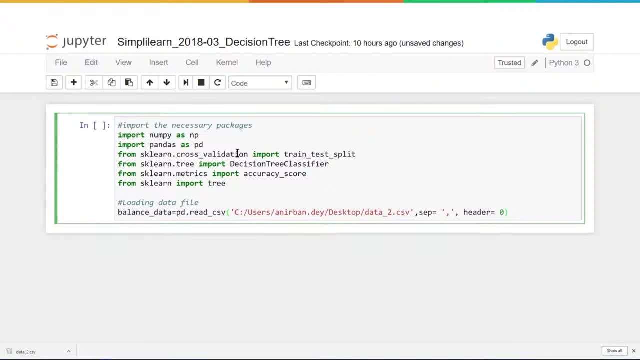 And let's go ahead and just paste that code in the beginning and before we start let's see what we're bringing in And then we're going to do a couple things in here. We have to make a couple changes as we go through this first part of the import. 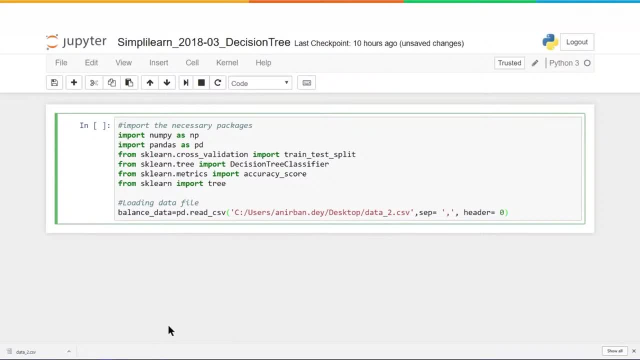 The first thing we bring in is numpy as np. That's very standard When we're dealing with mathematics, especially with very complicated machine learning tools. you almost always see the numpy come in for your numbers. It's called number Python. It has your mathematics in there. 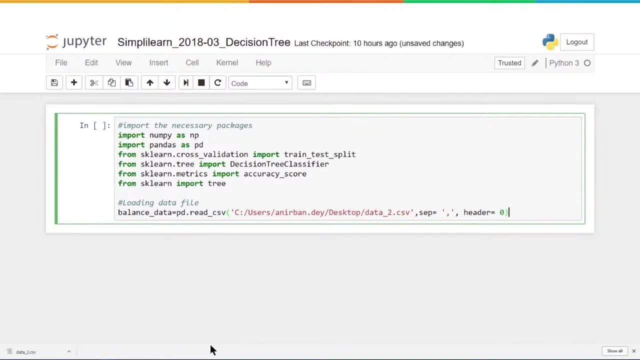 In this case we actually could take it out, but generally you'll need it for most of your different things you work with. And then we're going to use pandas as pd. The pandas is a data frame setup And you can liken this to: 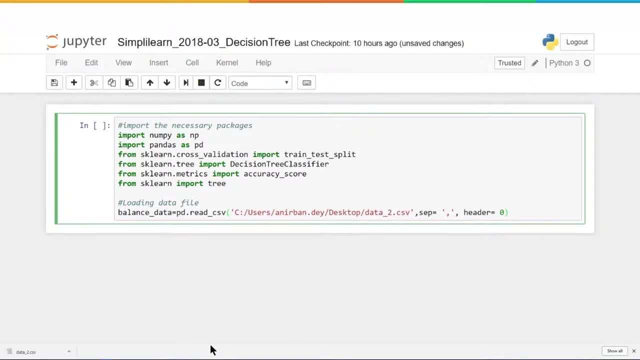 taking your basic data and storing it in a way that looks like an Excel spreadsheet. So as we come back to this, when you see np or pd, those are very standard uses. you'll know that that's the pandas And I'll show you a little bit more when we explore the data in just a minute. 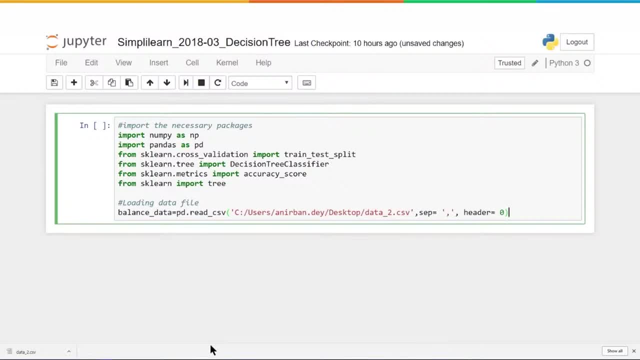 Then we're going to need to split the data. So I'm going to bring in our train, test and split. And this is coming from the sklearn package: cross-validation. In just a minute we're going to change that, So let's go over that too. 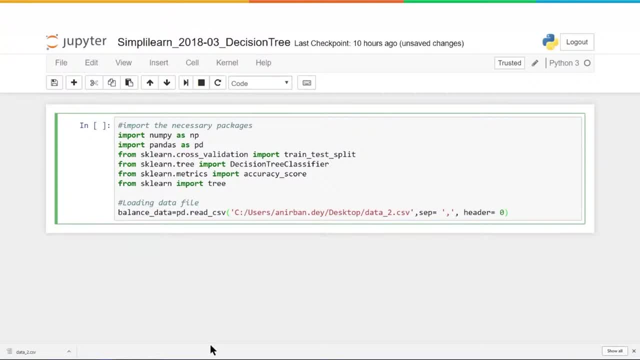 And then there's also the sktree import decision tree classifier. That's the actual tool we're using. Remember, I told you, don't be afraid of the mathematics, It's going to be done for you. Well, the decision tree classifier has all that mathematics in there for you. 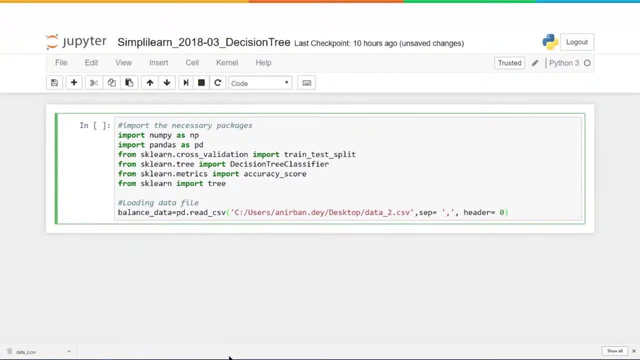 So you don't have to figure it back out again. And then we have sklearnmetrics for accuracy score. We need to score our setup. That's the whole reason. we're splitting it between the training and testing data. And finally, we still need the sklearn import tree. 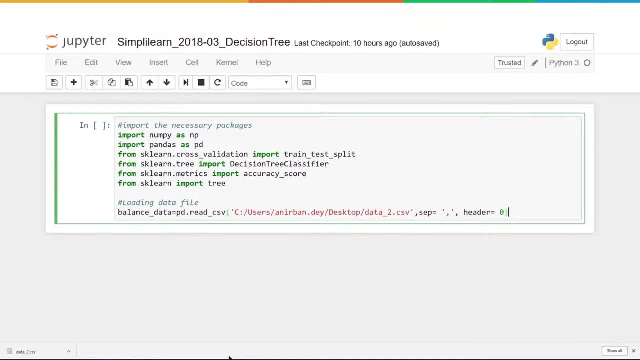 And that's just the basic tree function for the decision tree classifier. And finally, we're going to load our data down here And I'm going to run this and we're going to get two things on here. One, we're going to get an error. 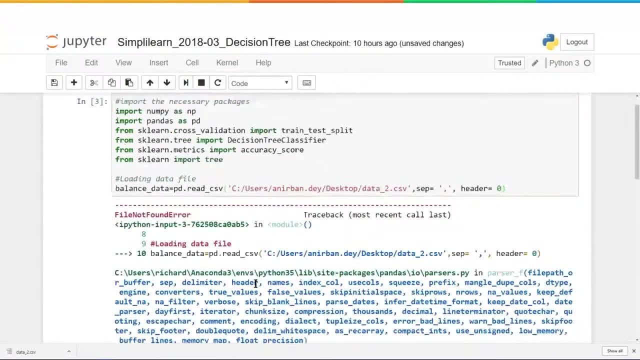 And two, we're going to get a warning. Let's see what that looks like. So the first thing we had is: we have an error. Why is this error here? Well, it's looking at this and says: I need to read a file. 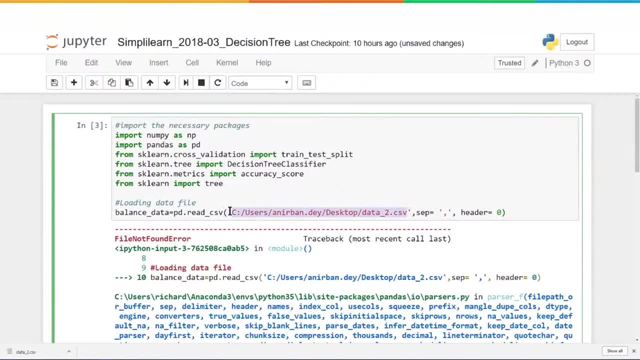 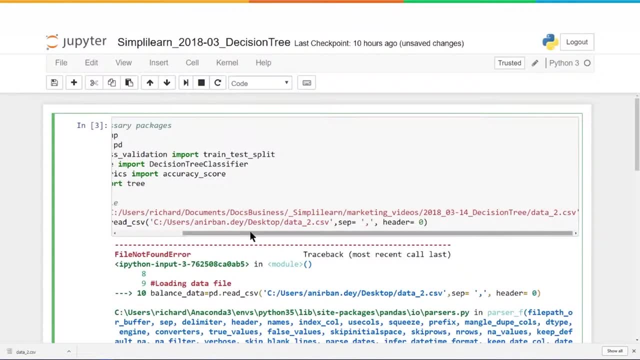 And when this was written, the person who wrote it, this is their path where they stored the file. So let's go ahead and fix that, And I'm going to put in here the full path. I'm just going to call it full file name. 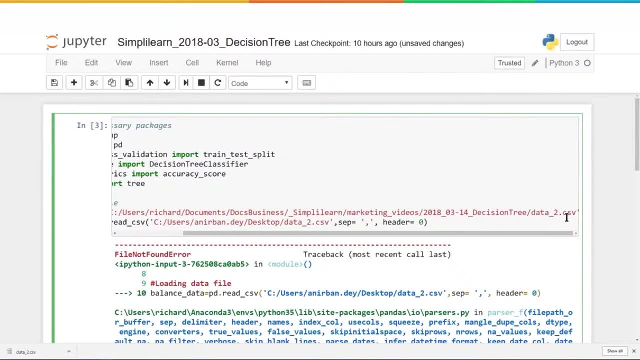 And you'll see. it's on my C drive and there's this very lengthy setup on here where I stored the data2.csv file. Don't worry too much about the full path, because on your computer it will be different: The data.2.csv file. 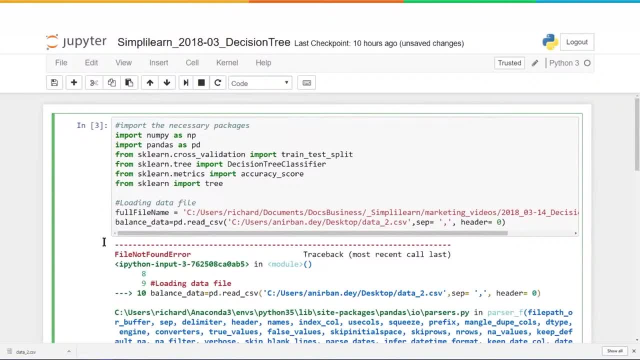 was generated by sklearn. If you want a copy of that, you can comment down below and request it here in the YouTube, And then, if I'm going to give it a name- full file name- I'm going to go ahead and change it here. 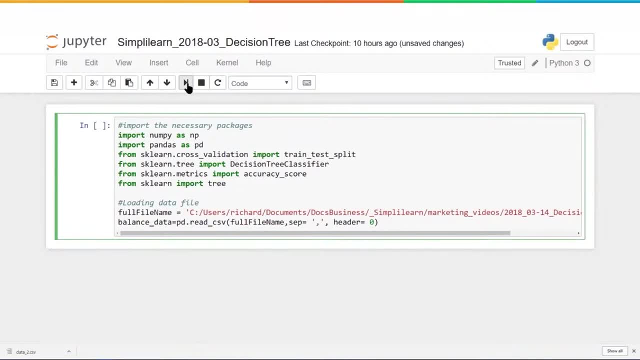 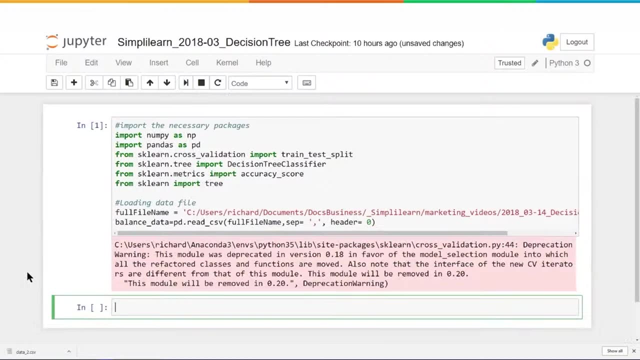 to full file name. So let's go ahead and run it now and see what happens. And we get a warning. When you're coding, understanding these different warnings and these different errors that come up is probably the hardest lesson to learn. So let's just go ahead and take a look at this. 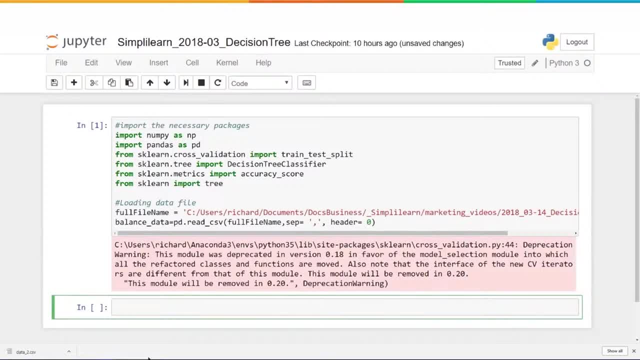 and use this as an opportunity to understand what's going on here. If you read the warning, it says the cross-validation is depreciated. So it's a warning on it's being removed And it's going to be moved in favor of the model selection. 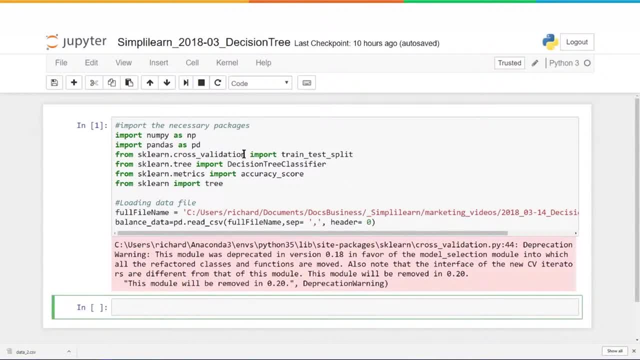 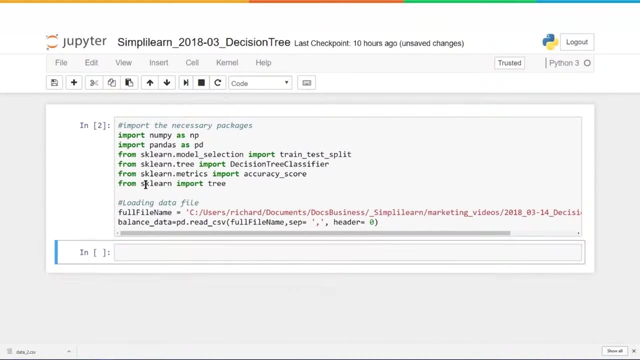 So if we go up here, we have sklearncross-validation, and if you research this and go to the sklearn site, you'll find out that you can actually just swap it right in there with model selection. And so when I come in here and I run it again, 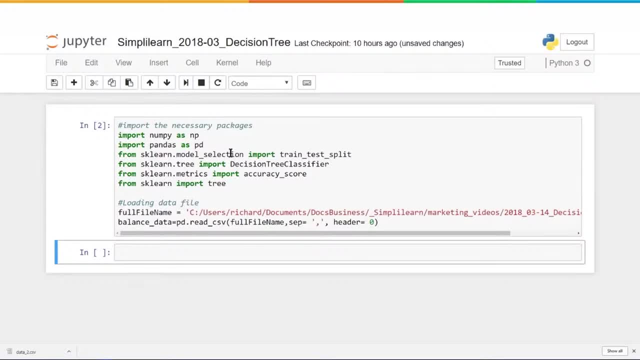 that removes a warning. What they've done is they've had two different developers develop it in two different branches, And then they decided to keep one of those and eventually get rid of the other one. That's all that is, And very easy and quick to fix. 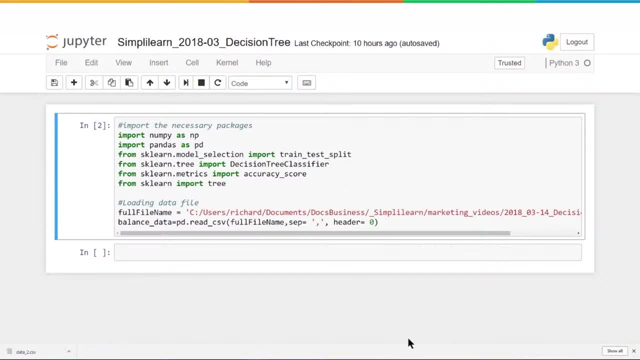 Before we go any further, I went ahead and opened up the data from this file. Remember the data file we just loaded on here, The data underscore two dot csv. Let's talk a little bit more about that and see what that looks like both as a text file. 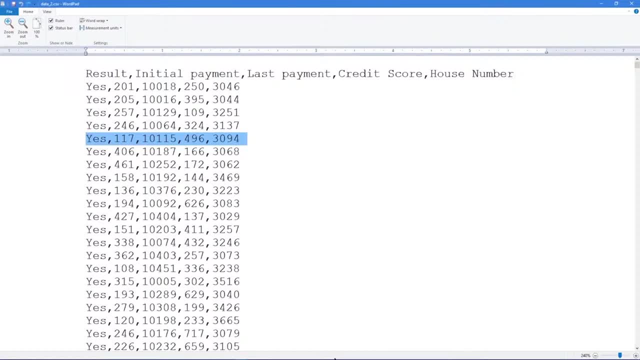 and in a spreadsheet. This is what it looks like as a basic text file. You can see at the top they've created a header and it's got one, two, three, four, five columns and each column has data in it. And let me flip this over. 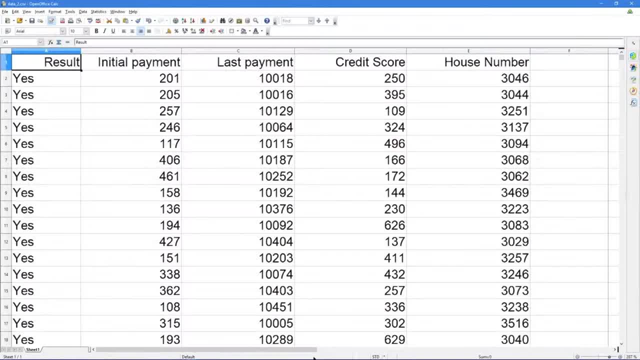 because we're also going to look at this in an actual spreadsheet. so you can see what that looks like. And here I've opened it up in the OpenOffice calc, which is pretty much the same as Excel, and zoomed in and you can see we've got our columns and our rows of data. 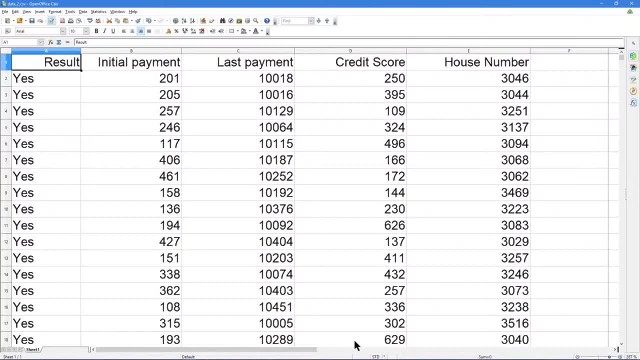 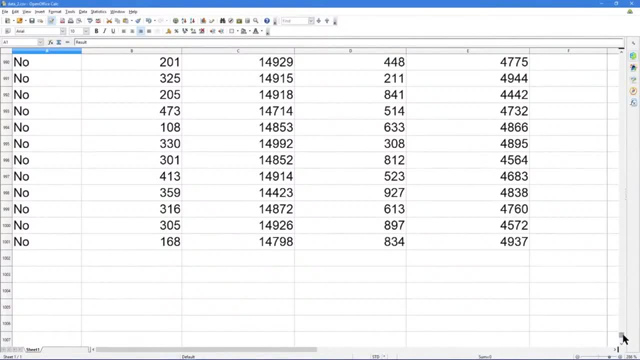 A little easier to read in here. Initial payment, last payment: credit score, house number. If we scroll way down, we'll see that this occupies a thousand and one lines of code or lines of data, with the first one being a column and then one thousand lines of data. 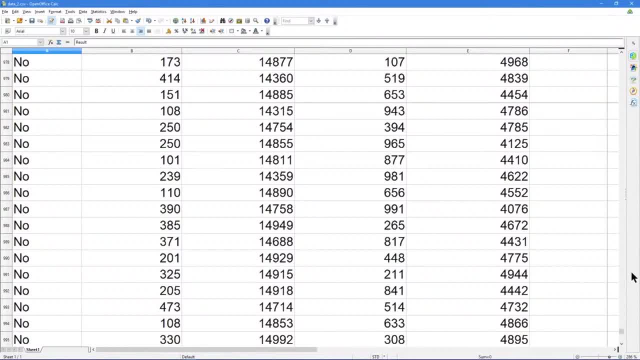 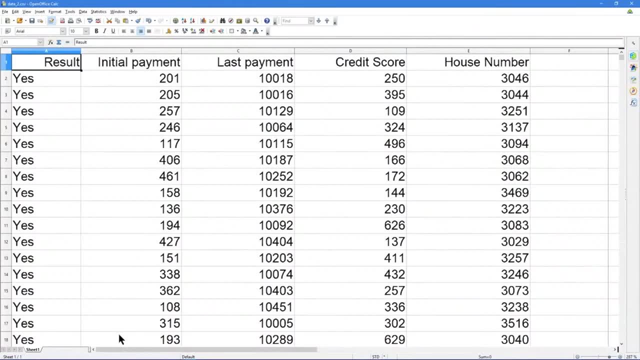 Now, as a programmer, if you're looking at a small amount of data, I usually start by pulling it up in different sources so I can see what I'm working with. With larger data, you won't have that option. It'll just be too large. so you need to either bring in a small amount. 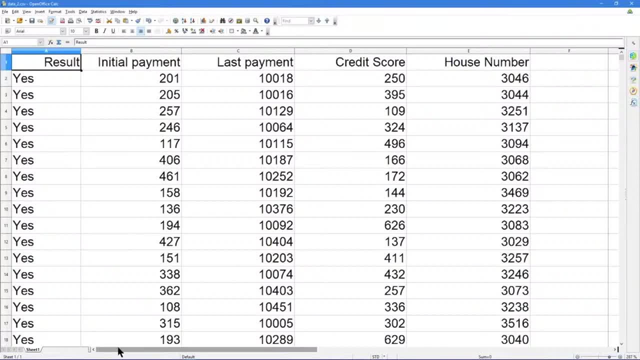 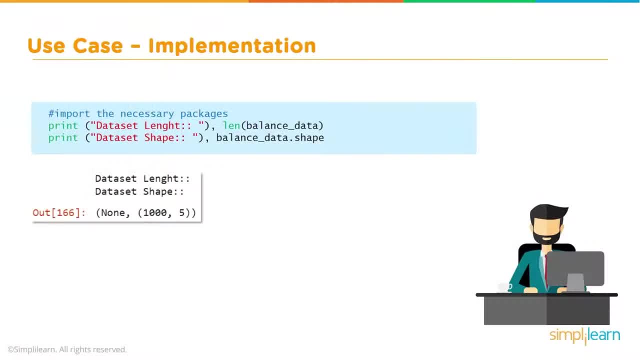 that you can look at it like we're doing right now, or we can start looking at it through the Python code. So let's go ahead and move on and take the next couple steps to explore the data using Python. Let's go ahead and see what it looks like. 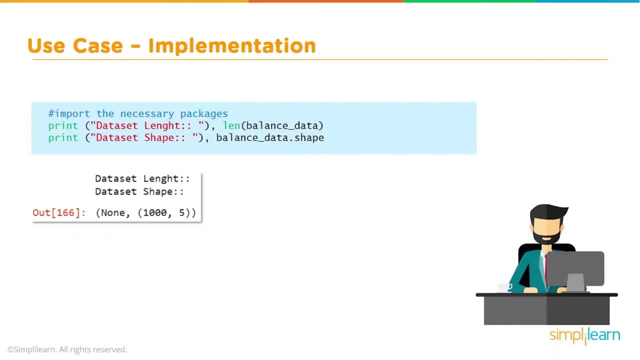 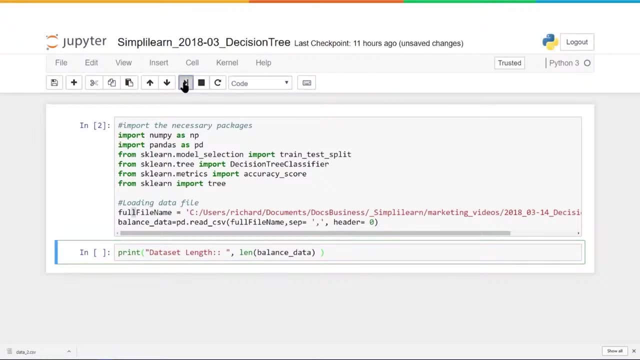 in Python to print the length and the shape of the data. So let's start by printing the length of the database. We can use a simple lin function from Python, And when I run this, you'll see that it's a thousand long. And that's what we expected. 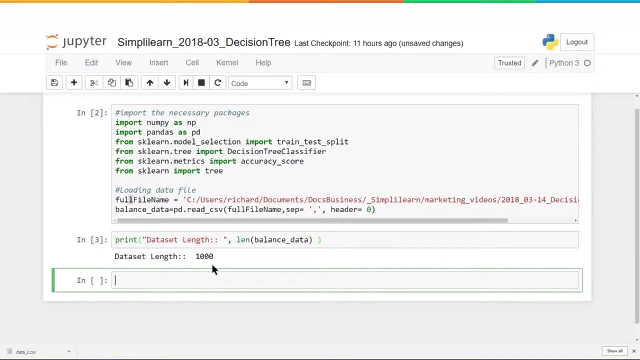 There's a thousand lines of data in there. if you subtract the column head- This is one of the nice things when we did the balance data from the Panda. Read CSV, you'll see that the header is row zero, so it automatically removes a row and then shows the data separate. 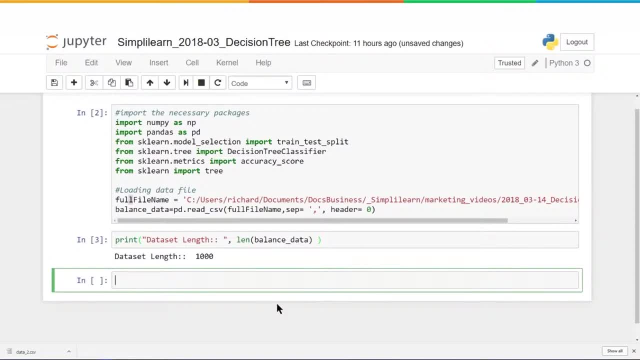 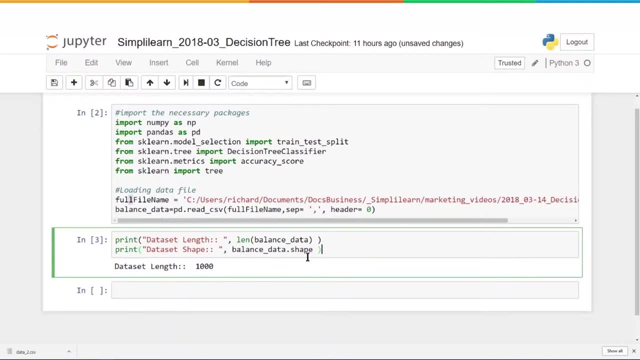 It does a good job sorting that data out for us, And then we can use a different function and let's take a look at that. And again, we're going to utilize the tools in Panda And, since the balance underscore data was loaded as a Panda data frame, 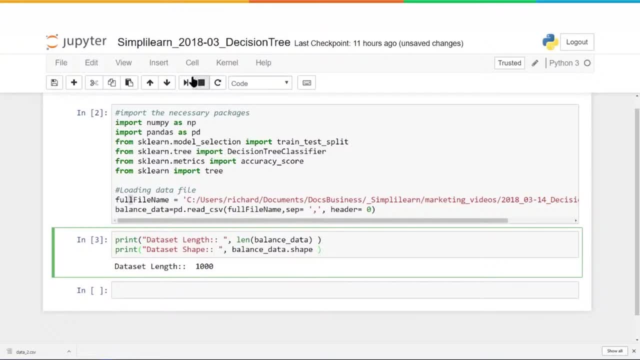 we can do a shape on it, And let's go ahead and run the shape and see what that looks like. What's nice about this shape is not only does it give me the length of the data- we have a thousand lines- it also tells me there's five columns. 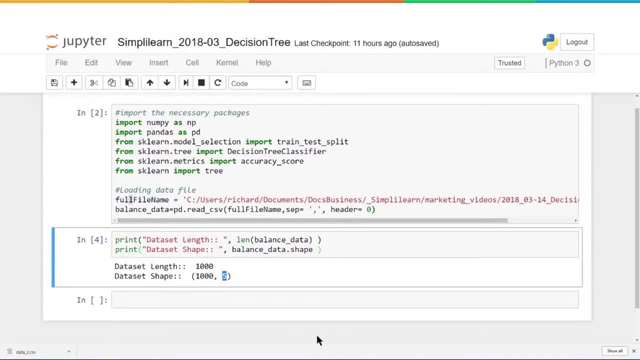 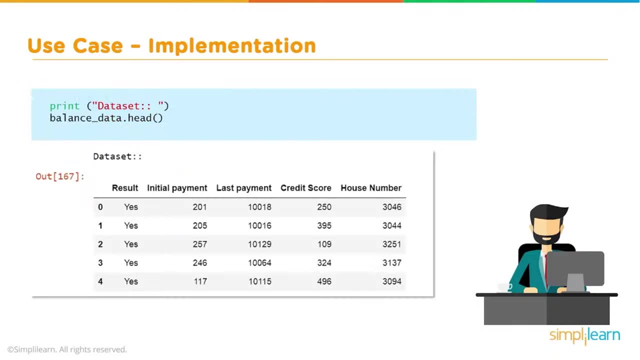 So when we were looking at the data, we had five columns of data. And then let's take one more step to explore the data using Python. Let's go ahead and use the Pandas module for head- Another beautiful thing in the data set that we can utilize. 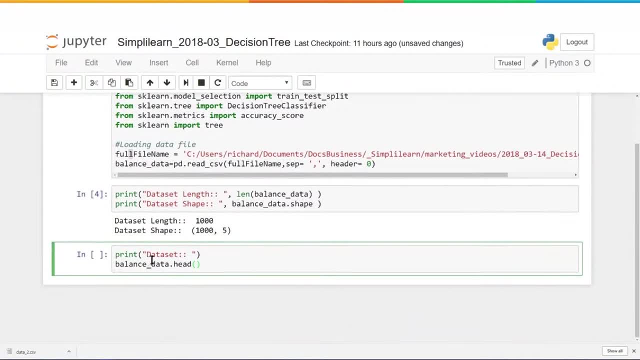 So let's put that on our sheet here. and we have print data set and balance data dot head. And this is a Pandas print statement of its own, So it has its own print feature in there. And then we went ahead and gave a label. 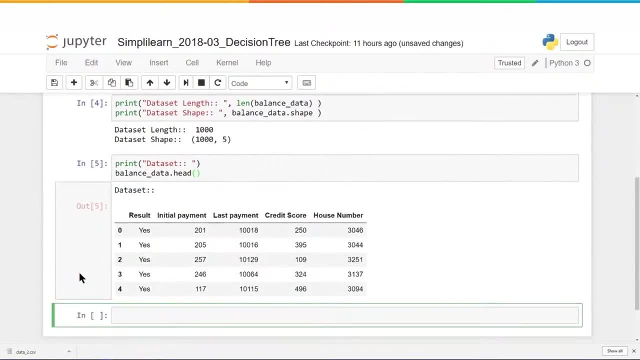 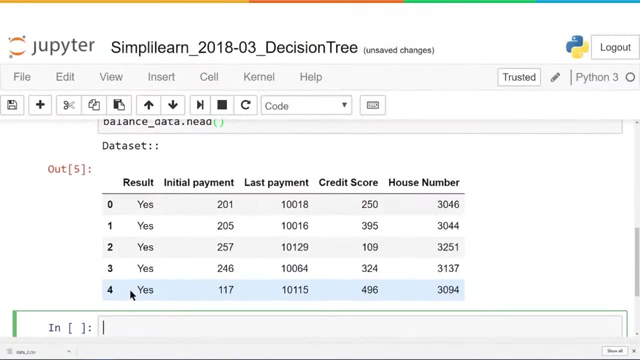 for our print job here of data set. Just a simple print statement, And when we run that let's just take a closer look at that. There we go. Pandas does such a wonderful job of making this a very clean, readable data set. 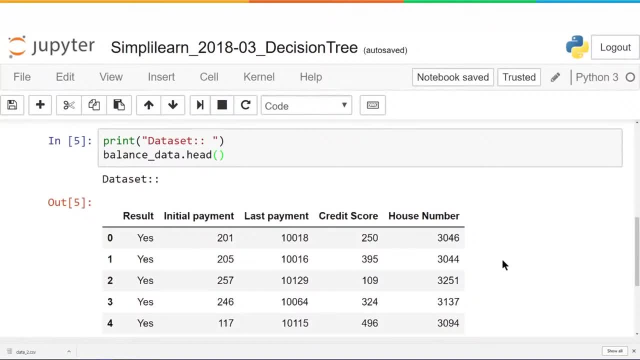 So you can look at the data, you can look at the column headers. you can have it when you put it as the head. it prints the first five lines of the data And we always start with zero. So we have five lines. we have zero one, two, three, four. 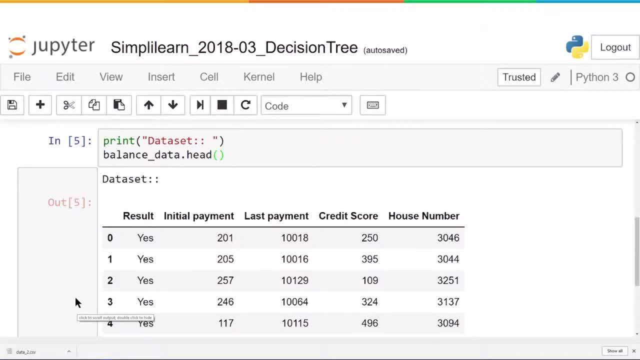 instead of one, two, three, four, five. That's a standard scripting and programming set as you want to start with the zero position, And that is what the data head does. It prints the first five rows of data, puts it in a nice format that you can look at. 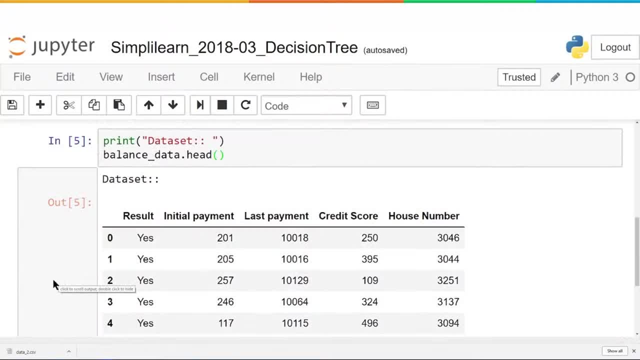 and view- Very powerful tool to view the data. So instead of having to flip and open up an Excel spreadsheet or open OfficeCal or trying to look at a Word doc where it's all scrunched together and hard to read, you can now get a nice. 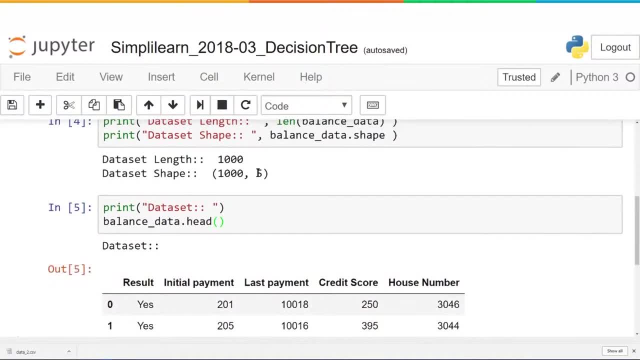 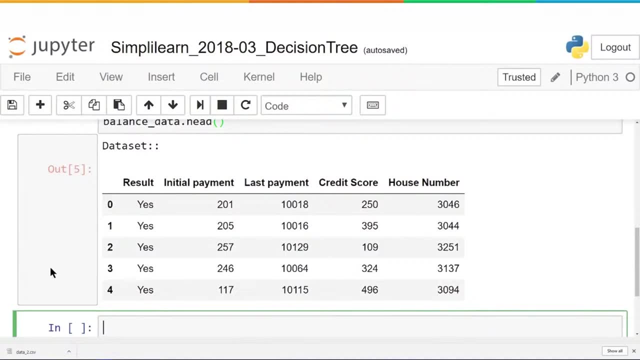 open view of what you're working with. We're working with a shape of a thousand long, five wide, so we have five columns and we do the full data head. you can actually see what this data looks like: The initial payment, last payment, credit scores, house number. 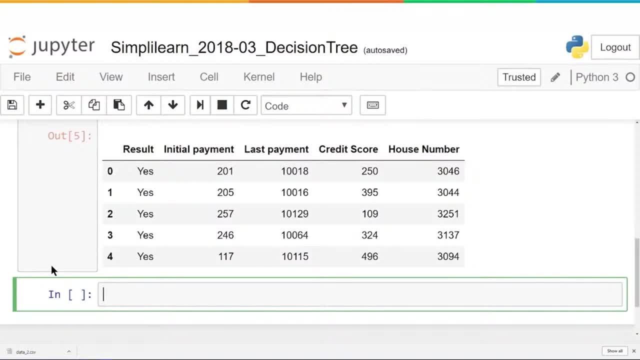 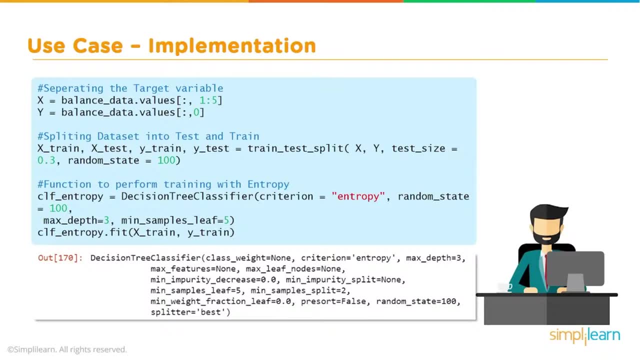 So let's take this, now that we've explored the data, and let's start digging into the decision tree. So in our next step, we're going to train and build our data tree, And to do that, we need to first separate the data out. 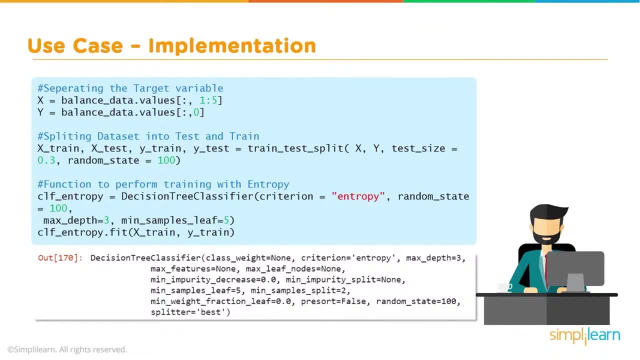 We're going to separate it into two groups so that we have something to actually train the data with and then we have some data on the side to test it, to see how good our model is. Remember, with any of the machine learning, you always want to have some kind of test set. 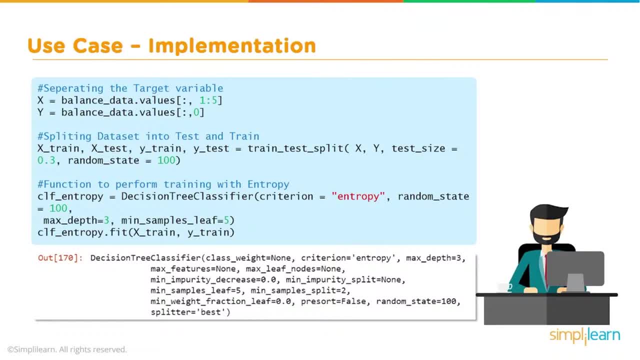 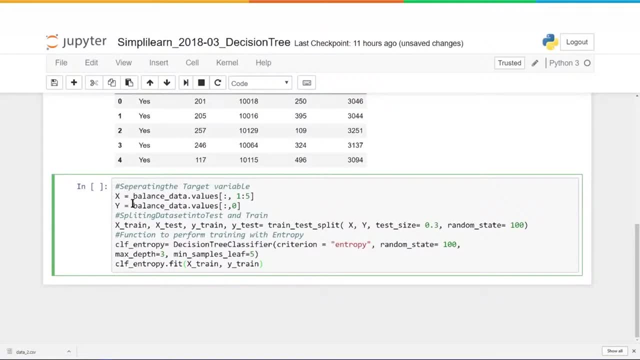 to weigh it against. so you know how good your model is when you distribute it. Let's go ahead and break this code down and look at it in pieces. So first we have our x and y. Where do x and y come from? Well, x is going to be. 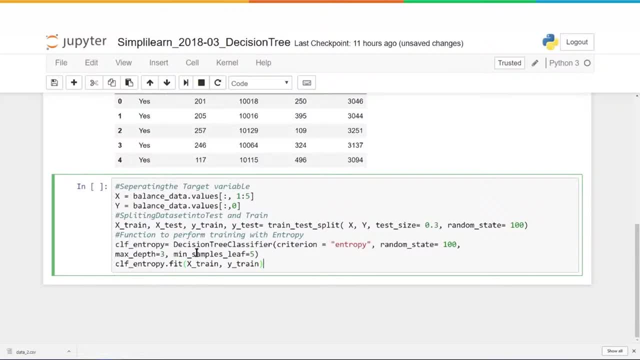 our data and y is going to be the answer or the target. You can look at it as source and target. In this case, we're using x and y to denote the data in and the data that we're actually trying to guess what the answer is going to be, And so to separate it. 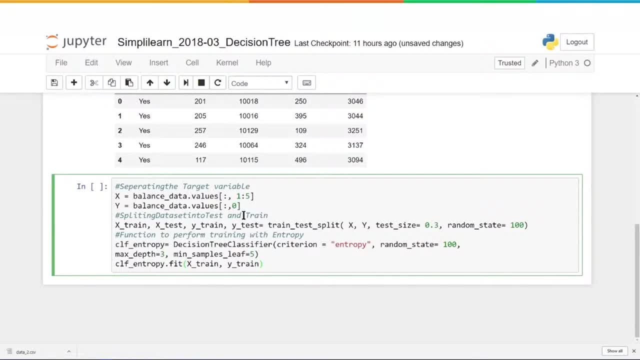 we can simply put in: x equals the balance of the data, dot values, and the first brackets means that we're going to select all the lines in the database. So it's all the data, And the second one says we're only going to look at. 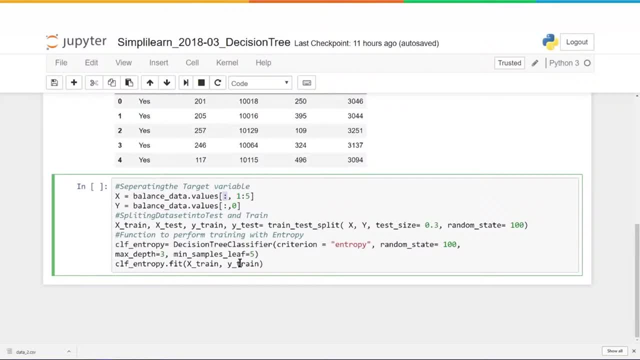 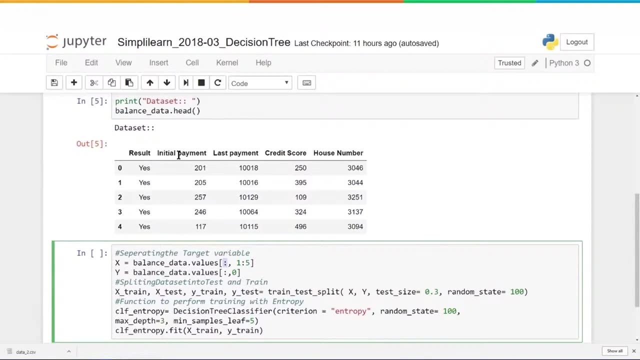 columns one through five. Remember, we always start with zero. Zero is a yes or no and that's whether the loan went default or not. So we want to start with one. If we go back up here, that's the initial payment and it goes all the way through. 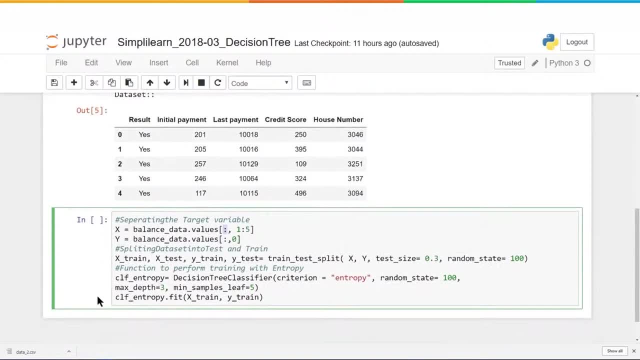 the house number. Well, if we want to look at one through five, we can do the same thing for y, which is the answer, and we're going to set that just equal to the zero row. So it's just the zero row, and then it's all rows going in there. 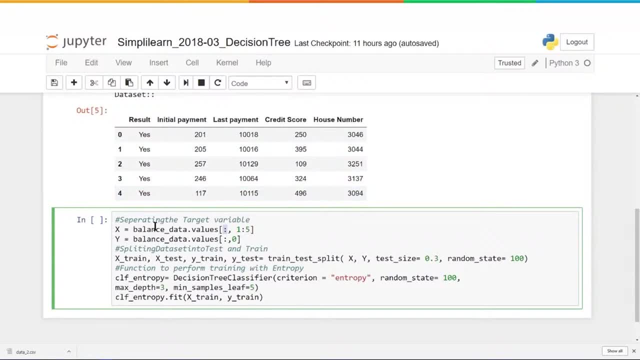 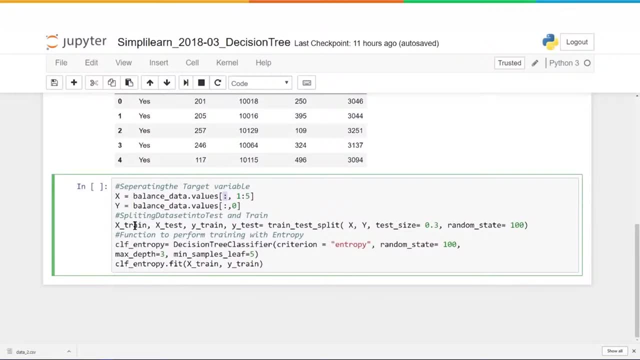 So now we've divided this into two different data sets, One of them with the data going in and one with the answers. Next we need to split the data, And here you'll see that we have it split into four different parts. The first one. 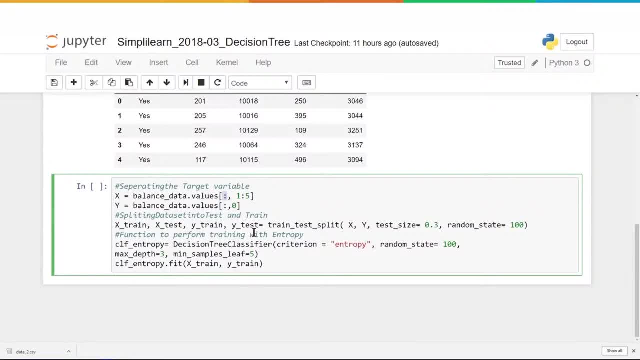 is your x training your x test? your y train your y test. Simply put, we have x going in where we're going to train it and we have to know the answer to train it with. And then we have x test where we're going to. 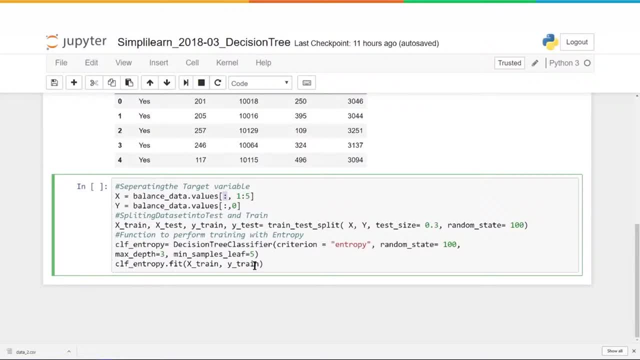 test that data And we have to know in the end what the y was supposed to be. And that's where this train test split comes in that we loaded earlier in the modules. This does it all for us And you can see. they set the test size equal to .3. 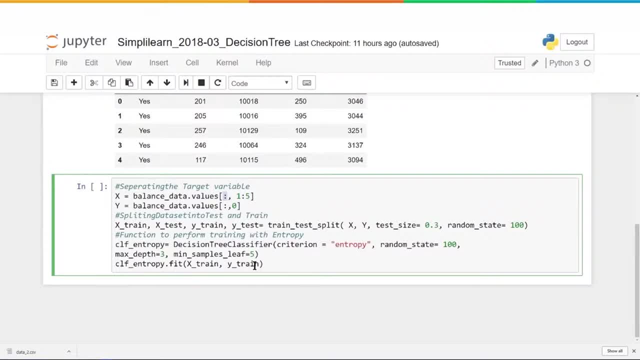 so that's roughly 30% will be used in the test. And then we use a random state, so it's completely random which rows it takes out of there, And then finally we get to actually build our decision tree. And they've called it here: clf. 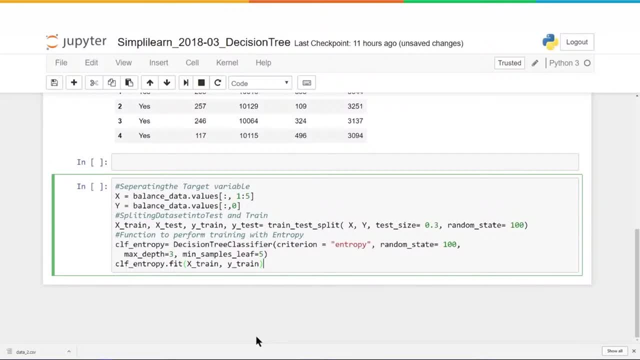 underscore entropy. That's the actual decision tree or decision tree classifier, And in here they've added a couple variables which we'll explore in just a minute, And then, finally, we need to fit the data to that. So we take our clf. 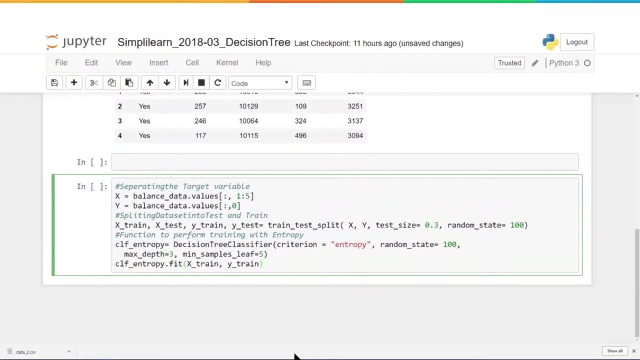 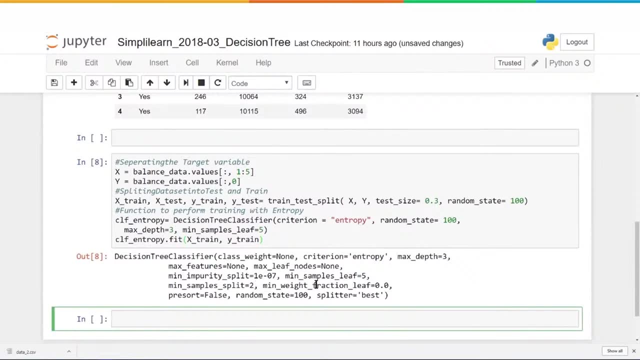 entropy that we created and we fit the x train and since we know the answers for x train are the y train, we go ahead and put those in And let's go ahead and run this And what most of these sklearn modules do. 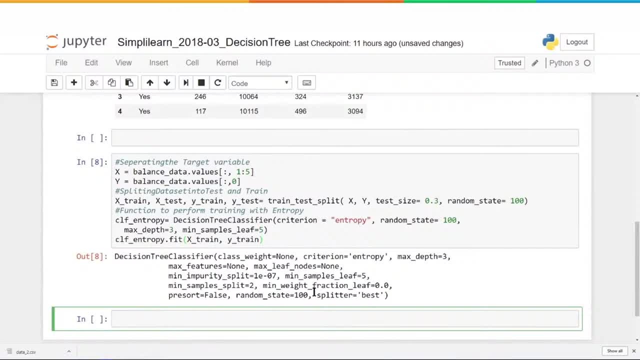 is when you set up the variable, in this case, when we set the clf entropy equal decision tree classifier, it automatically prints out what's in that decision tree. There's a lot of variables you can play with in here And it's quite beyond the scope of. 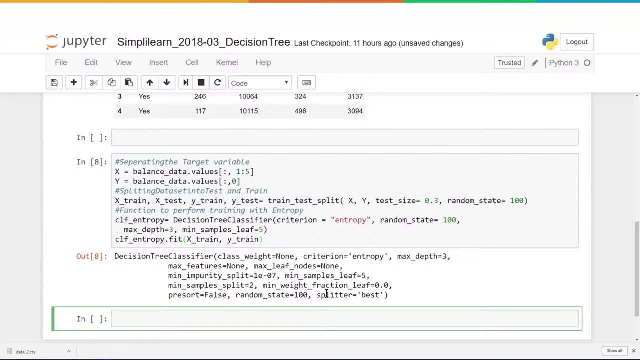 this tutorial to go through all of these and how they work. But we're working on entropy. that's one of the options. We've added that it's completely a random state of 100, so 100% And we have a max depth of 3.. 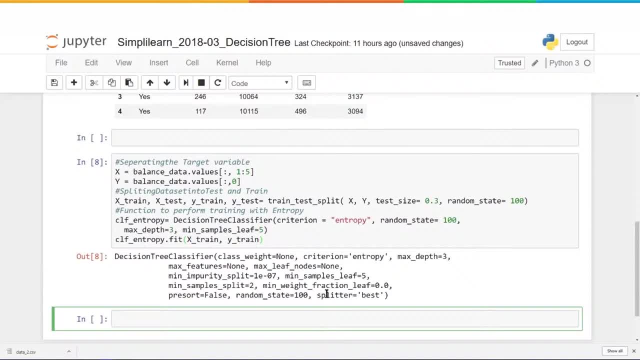 Now the max depth, if you remember above when we were doing the different graphs of animals, means it's only going to go down 3 layers before it stops, And then we have minimal samples of leaves as 5.. So it's going to have at least 5 leaves at the end. 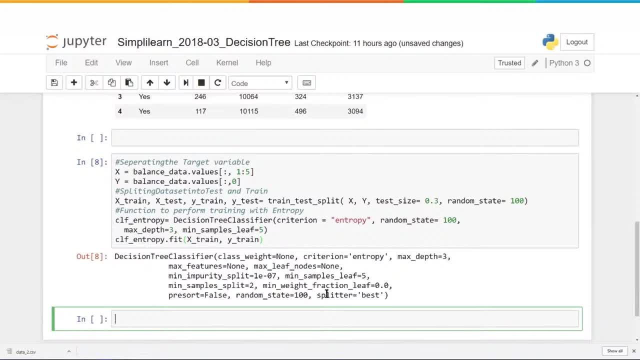 So it'll have at least 3 splits, it'll have no more than 3 layers and at least 5 end leaves, with the final result at the bottom, Now that we've created our decision tree classifier, not only created it, but trained it. 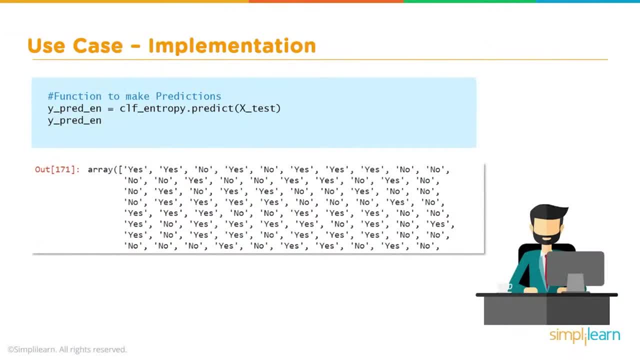 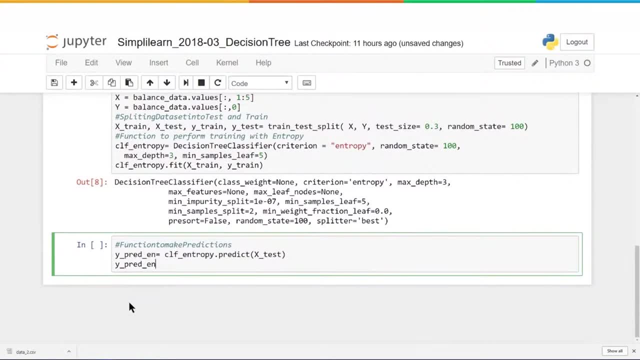 let's go ahead and apply it and see what that looks like. So let's go ahead and make a prediction and see what that looks like. We're going to paste our predict code in here And before we run it, let's just take a quick look at what. 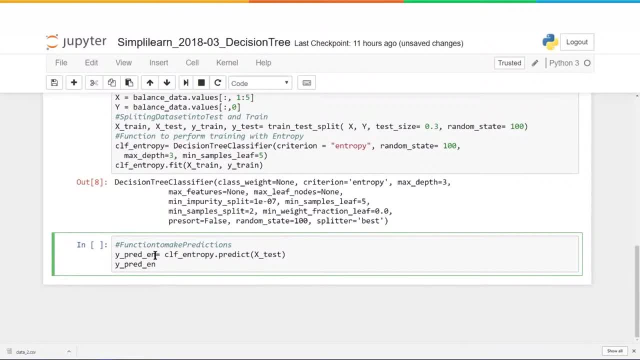 it's doing. here We have a variable, ypredict that we're going to do And we're going to use our variable clfentropy that we created And then you'll see predict. And it's very common in the sklearn modules that their different tools 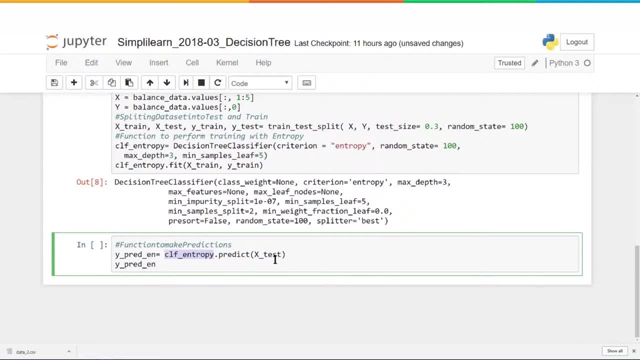 have the predict when you're actually running a prediction. In this case, we're going to put our xtest data in here. Now, if you delivered this for use- an actual commercial use- and distributed it, this would be the new loans you're putting in here, to guess. 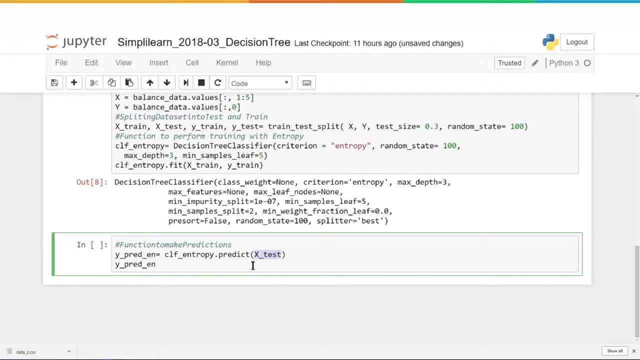 whether the person's going to be pay them back or not. In this case, though, we need to test out the data and just see how good our sample is, How good of our tree does at predicting the loan payments And finally, since Anaconda. 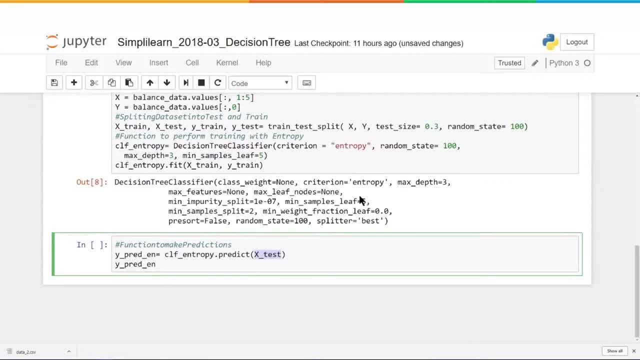 Jupyter Notebook works as a command line for Python. we can simply put the ypredicten to print it. I could just as easily have put the print and put brackets around ypredicten to print it out. We'll go ahead and do that. 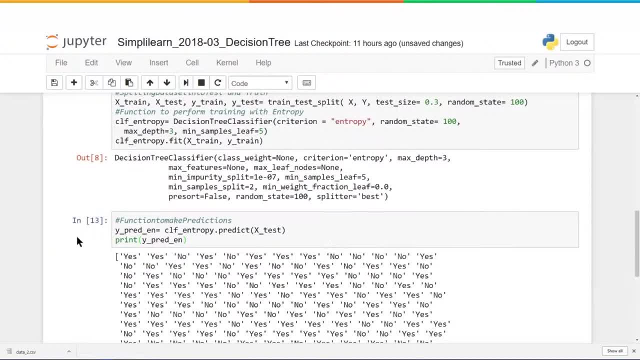 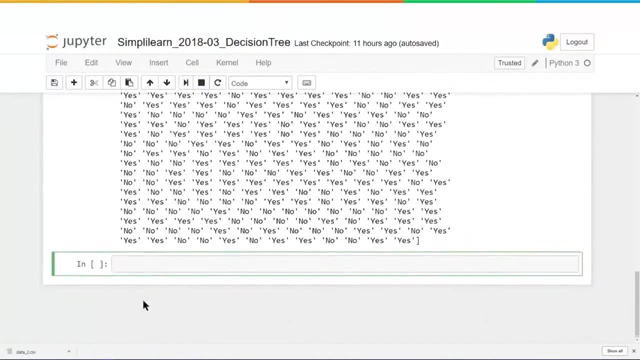 It doesn't matter which way you do it And you'll see right here that it runs a prediction. This is roughly 300 in here. Remember it's 30% of 1000, so you should have about 300 answers in here. 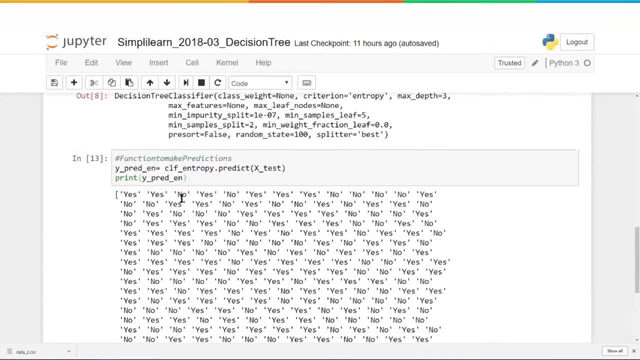 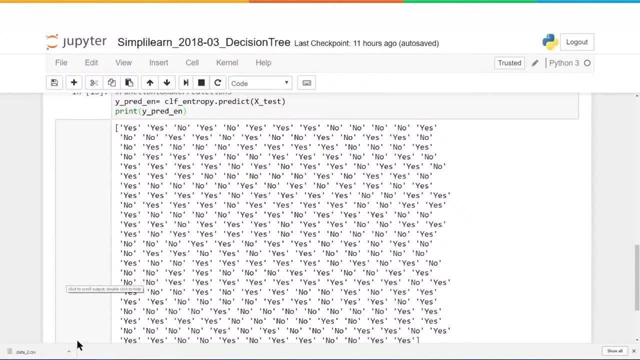 And this tells you which each one of those lines of our test went in there, And this is what our predict came out. So let's move on to the next step. We're going to take this data and try to figure out just how good a model we have. So here 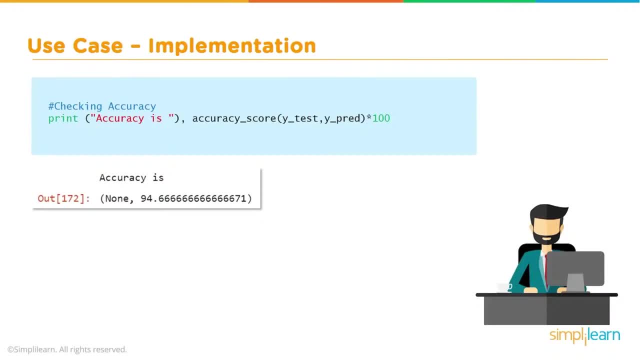 we go. Since sklearn does all the heavy lifting for you and all the math, we have a simple line of code to let us know what the accuracy is, And let's go ahead and go through that and see what that means and what that looks like. Let's go ahead and paste. 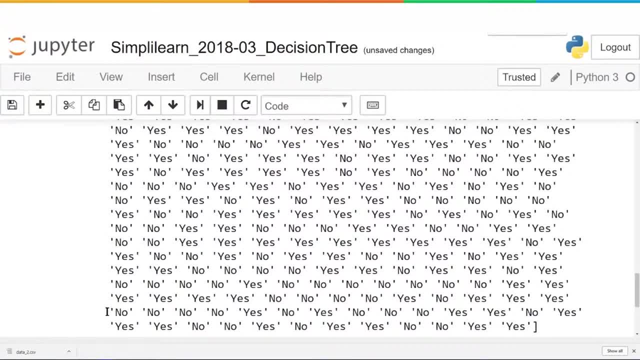 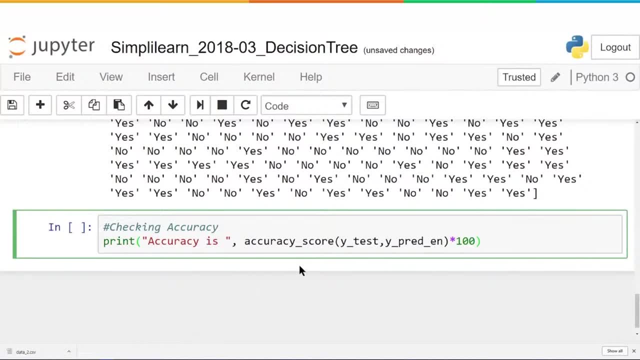 this in And let me zoom in a little bit. There we go, So you have a nice full picture And we'll see. here we're just going to do a print. accuracy is, And then we do the accuracy score, And this was. 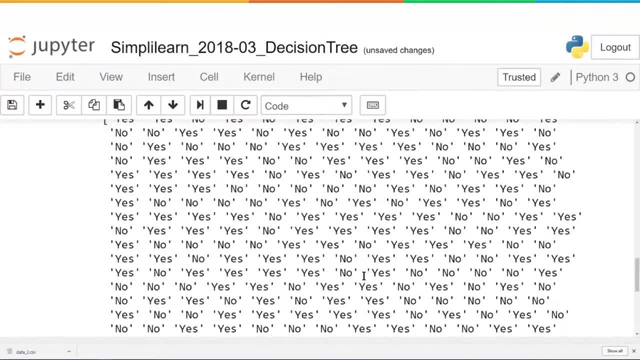 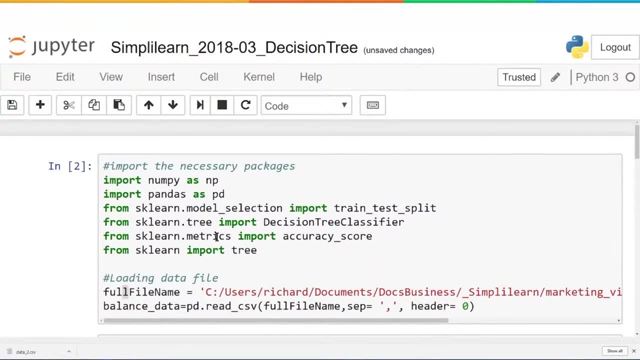 something we imported earlier, if you remember at the very beginning. Let me just scroll up there real quick so you can see where that's coming from. That's coming from here, down here, from sklearnmetrics import accuracy score, And you could probably run a script, make your own. 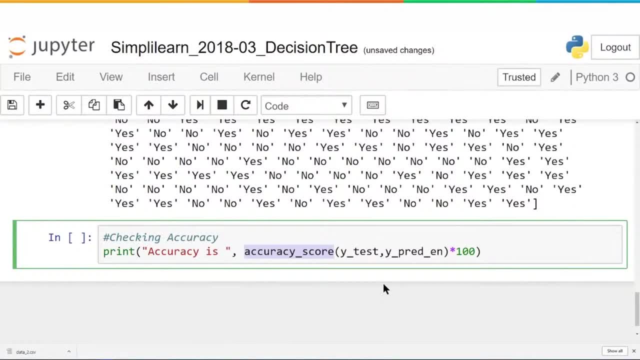 script to do this very easily. How accurate is it? How many out of 300 do we get right? And so we put in our y test- That's the one we ran the predict on. And then we put in our y predict en. That's the. 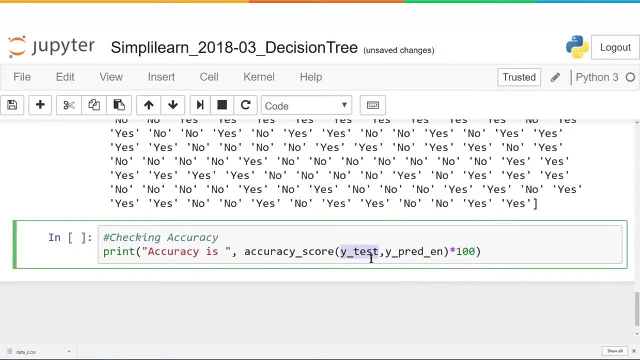 answers we got And we're just going to multiply that by 100.. Because this is just going to give us an answer as a decimal And we want to see it as a percentage And let's run that and see what it looks like. 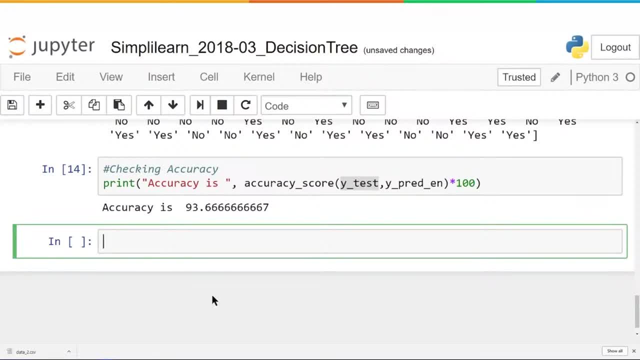 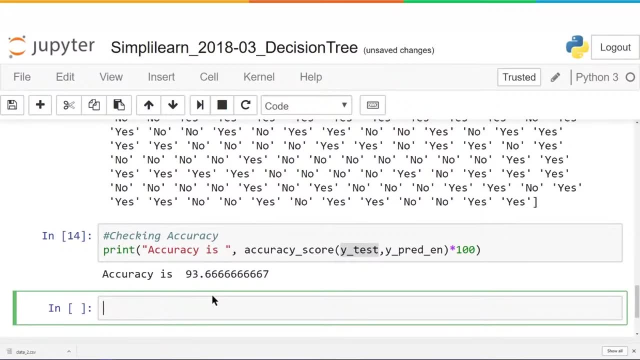 And if you see, here we got an accuracy of 93.66667.. So when we look at the number of loans and we look at how good our model fit, we can tell people it has about a 93.6 fitting to it. So just a quick. 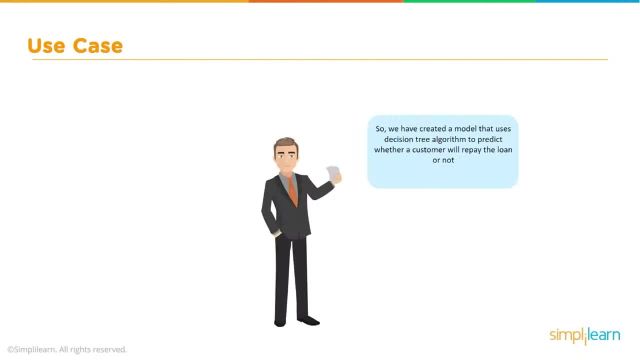 recap on that. We now have accuracy set up on here, And so we have created a model that uses the decision tree algorithm to predict whether a customer will repay the loan or not. The accuracy of the model is about 94.6%. The bank can now use. 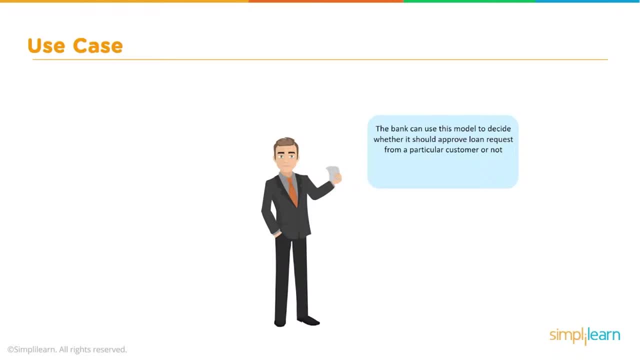 this model to decide whether it should approve the loan request from a particular customer or not, And so this information is really powerful. We may not be able to, as individuals, understand all these numbers, because they have thousands of numbers that come in, But you can see that this is a smart. 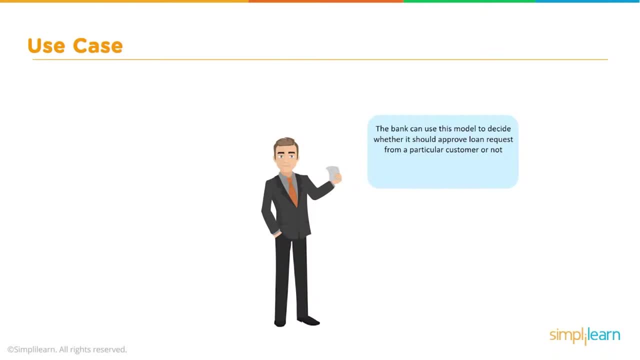 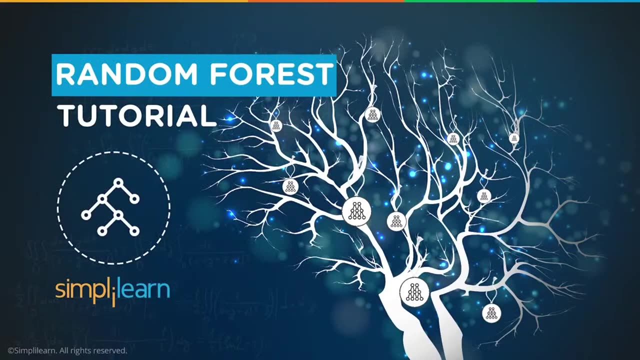 decision for the bank to use a tool like this to help them to predict how good their profit is going to be off of the loan balances and how many are going to default or not. We're going to be looking at Random Forest, one of the 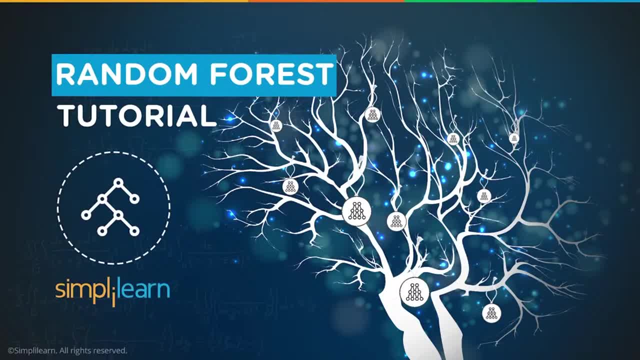 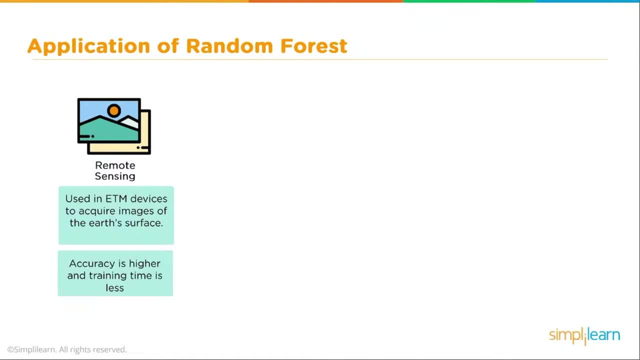 many powerful tools in the machine learning library. Before we dive into the topic, let's start by looking at a few of the uses for Random Forest Currently. today it's used in remote sensing, For example. they're used in the ETM devices If 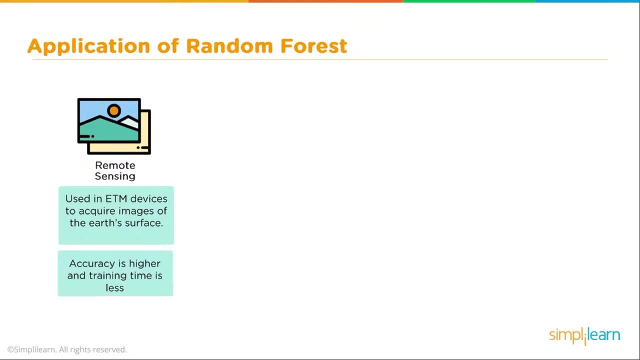 you're a space buff. that's the enhanced thermatic mapper they use on satellites which see far outside the human spectrum, for looking at land masses And they acquire images of the Earth's surface. The accuracy is higher and training time is less than many other machine. 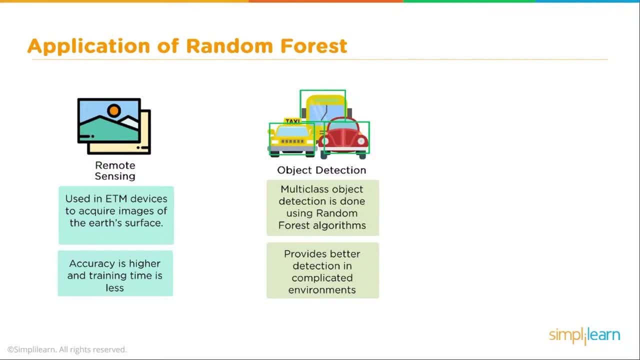 learning tools out there Also. object detection: multi-class object detection is done using Random Forest algorithms. A good example is traffic, where you try to sort out the different cars, buses and things, And it provides a better detection in complicated environments. They're very complicated up there And then we have 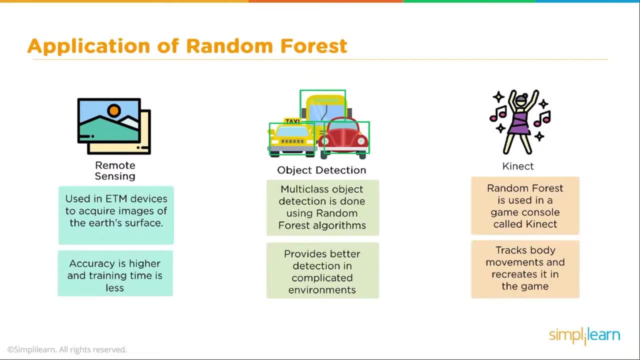 another example: Connect. And let's take a little closer look at Connect. Connect, they use the Random Forest as part of the game console And what it does is it tracks the body movements and it recreates it in the game. And let's see. 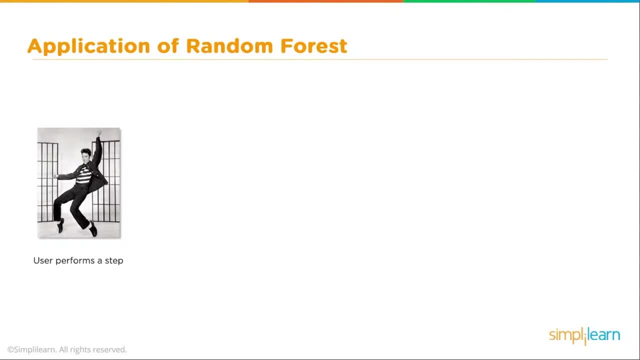 what that looks like. We have a user who performs a step- In this case it looks like Elvis Presley going there. That is then recorded so that Connect registers the movement, And then it marks the user based on accuracy And it looks like we have Prince going on. 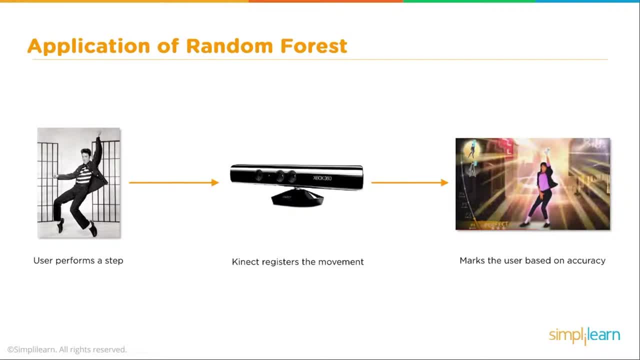 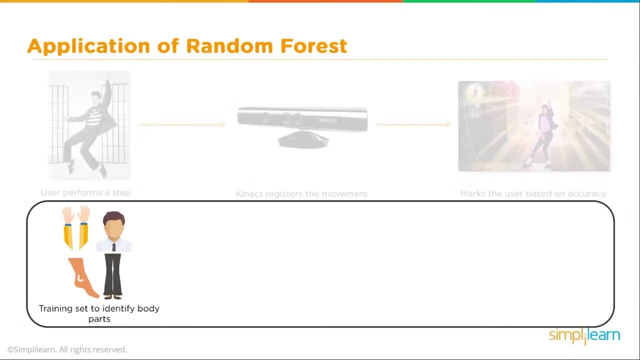 this one From Elvis Presley to Prince. It's great. So it marks the user based on the accuracy. If we look at that a little closer, we have a training set to identify body parts: Where are the hands, Where are the? 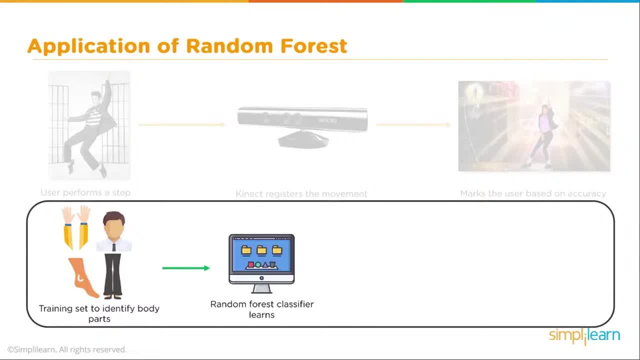 feet. What's going on with the body? That then goes into a Random Forest classifier that learns from it. Once we train the classifier, it then identifies the body parts while the person's dancing And it's able to represent that in a computer format And then based 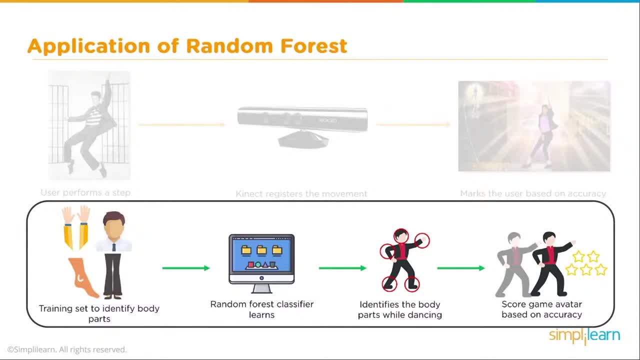 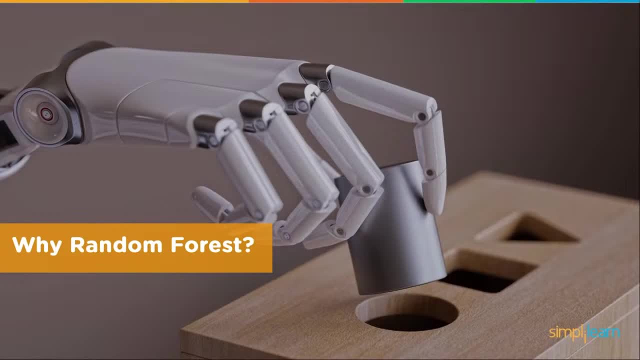 on that, it scores the game and how accurate you are as being Elvis Presley Or Prince and your dancing. So why Random Forest? It's always important to understand why we use this tool over the other ones. What are the benefits here? And so, with the 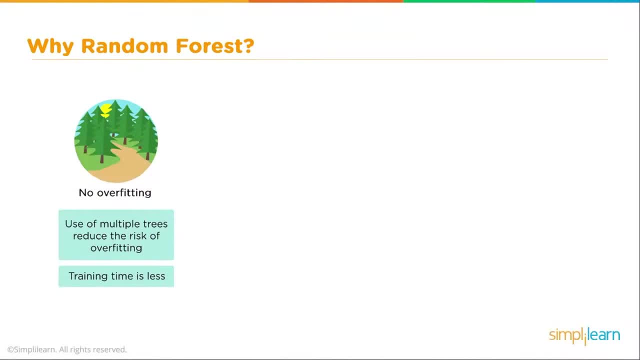 Random Forest. the first one is there's no overfitting. If you use of multiple trees, reduce the risk of overfitting. Training time is less Overfitting means that we have fit the data so close to what we have as our sample. 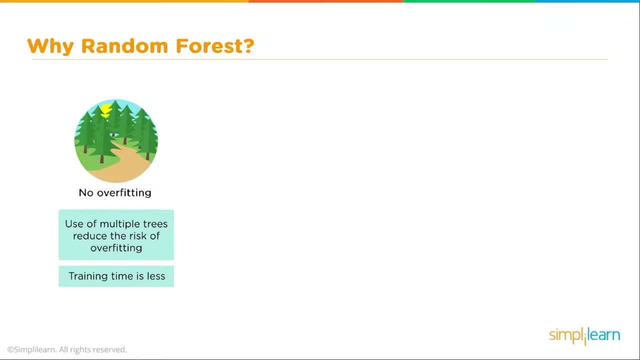 that we pick up on all the weird parts And, instead of predicting the overall data, you're predicting the weird stuff which you don't want. High accuracy Runs efficiently on large database For large data. it produces highly accurate predictions In today's world. 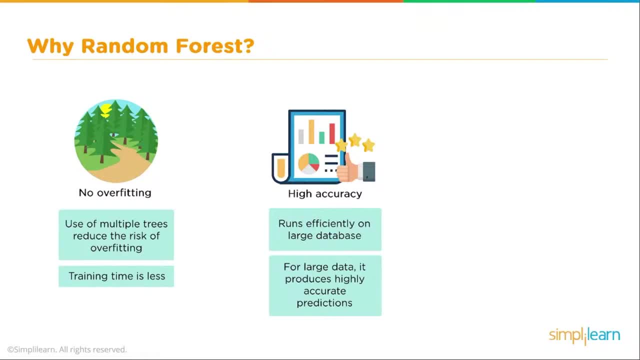 of big data. this is really important And this is probably where it really shines. This is where why Random Forest really comes in. It estimates missing data. Data in today's world is very messy, So when you have a Random Forest, it can. 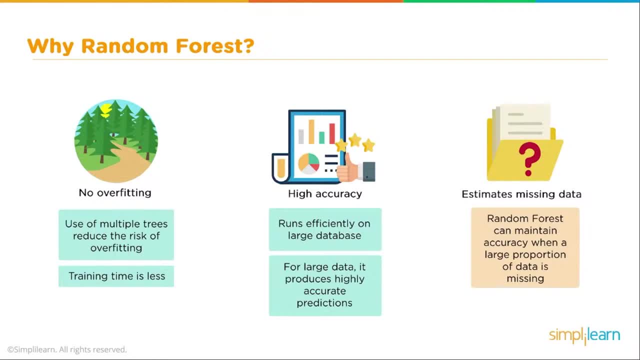 maintain the accuracy when a large proportion of the data is missing. What that means is if you have data that comes in from five or six different areas and maybe they took one set of statistics in one area and they took a slightly different set of statistics in the 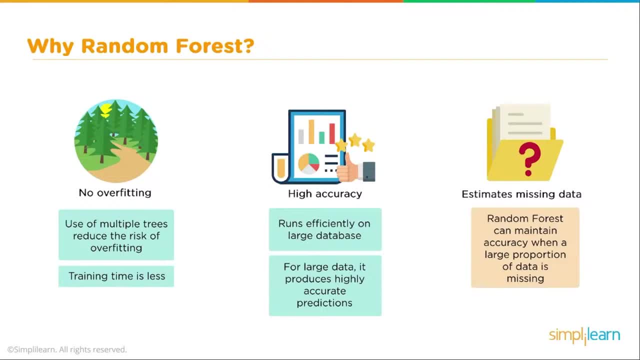 other. so they have some of the same shared data. but one is missing, like the number of children in the house, if you're doing something over demographics, And the other one is missing: the size of the house. It will look at both of those separately and build. 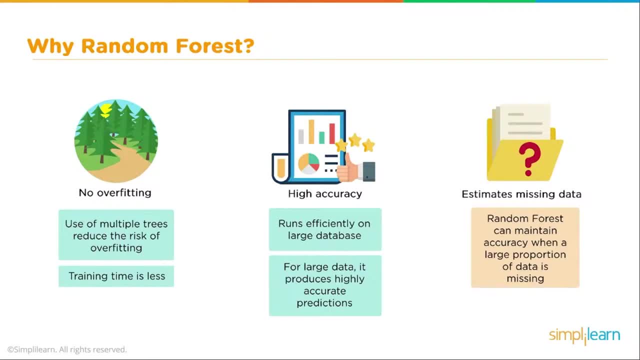 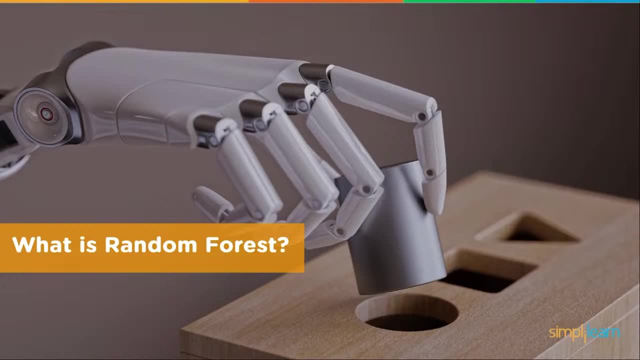 two different trees, and then it can do a very good job of guessing which one fits better, even though it's missing that data. Let us dig deep into the theory of exactly how it works, And let's look at what is Random Forest. 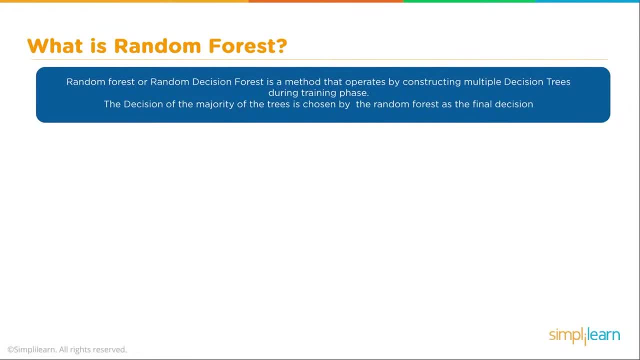 Random Forest or Random Decision Forest is a method that operates by constructing multiple decision trees. The decision of the majority of the trees is chosen by the Random Forest as the final decision. We have some nice graphics here. We have a decision tree and they actually use a real tree. 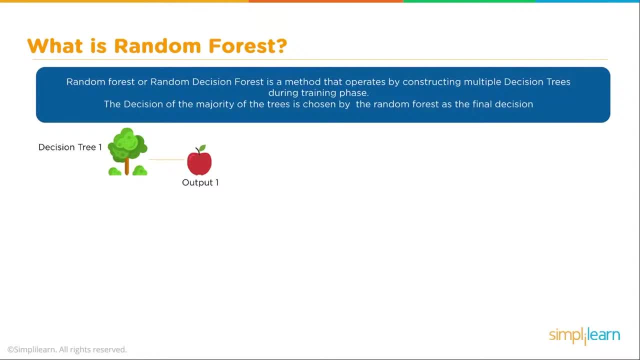 to denote the decision tree, which I love, And given a random, some kind of picture of a fruit, this decision tree decides that the output is it's an apple. And we have a decision tree two where we have that picture of the 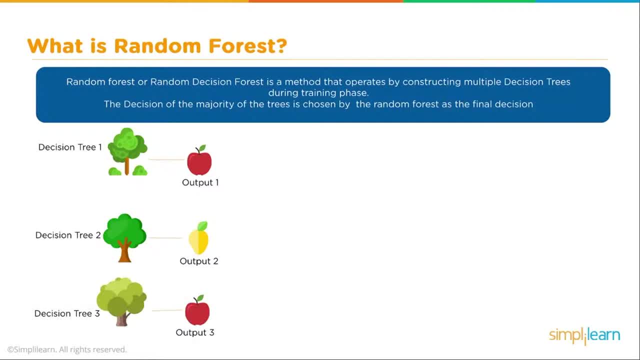 fruit goes in and this one decides that it's a lemon, And the decision tree three gets another image and it decides it's an apple. And then this all comes together in what they call the Random Forest, And this Random Forest then looks at it. 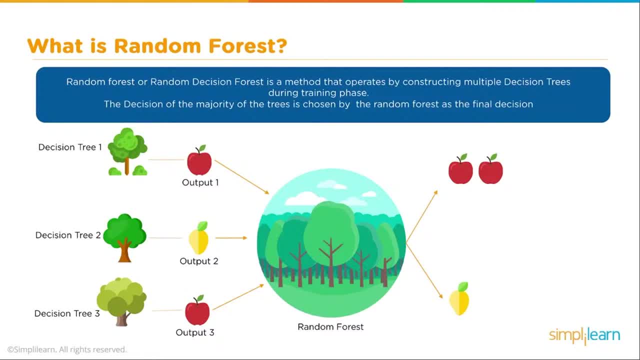 and says: okay, I got two votes for apple, one vote for lemon. the majority is apples, so the final decision is apples. To understand how the Random Forest works, we first need to dig a little deeper and take a look at the 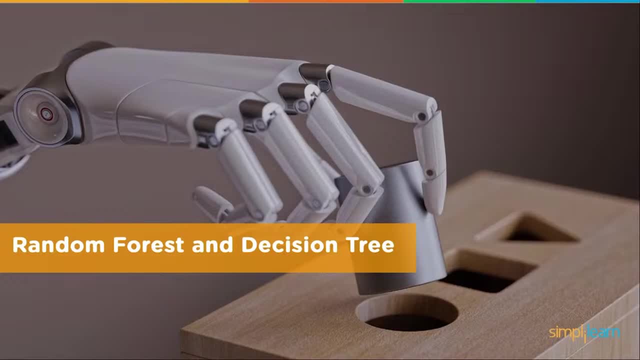 Random Forest and the actual decision tree and how it builds that decision tree. In looking closer at how the individual decision trees work, we'll go ahead and continue to use the fruit example, since we're talking about trees and forests. A decision tree is a tree. 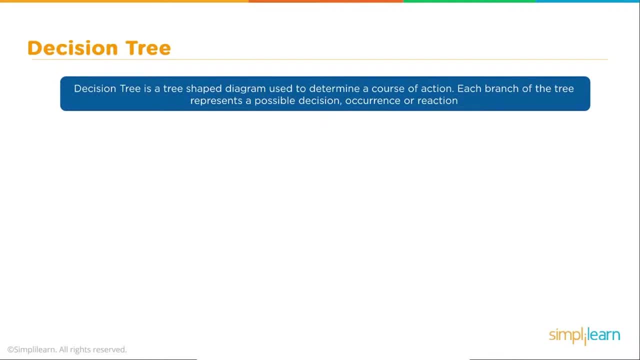 shaped diagram used to determine a course of action. Each branch of the tree represents a possible decision, occurrence or reaction. So in here we have a bowl of fruit and if you look at that, it looks like they switched from lemons to oranges. We have oranges. 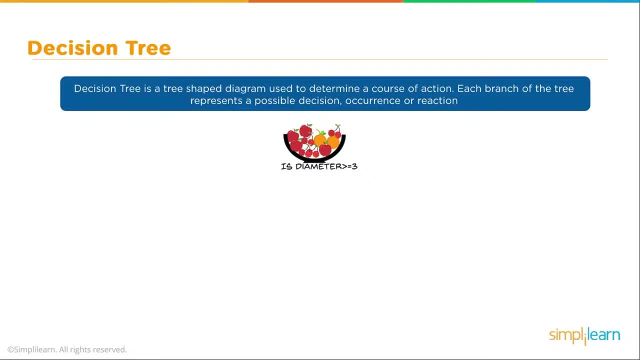 cherries and apples And the first decision of the decision tree might be: is the diameter greater than or equal to three? And if it says false, it knows that they're cherries, because everything else is bigger than that. So all the cherries fall. 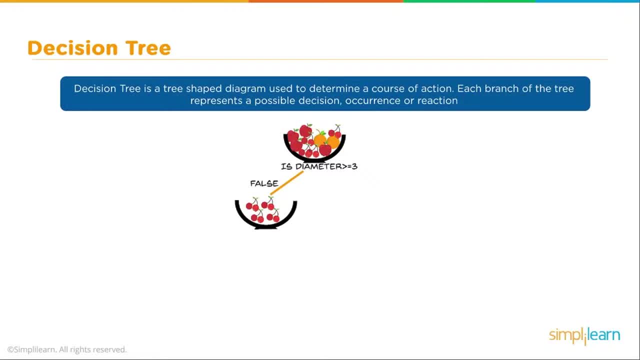 into that decision. So we have all that data we're training, we can look at that and we know that that's what's going to come up. Is the color orange? Well, it goes. hmm, orange or red? Well, if it's true, then it comes out. 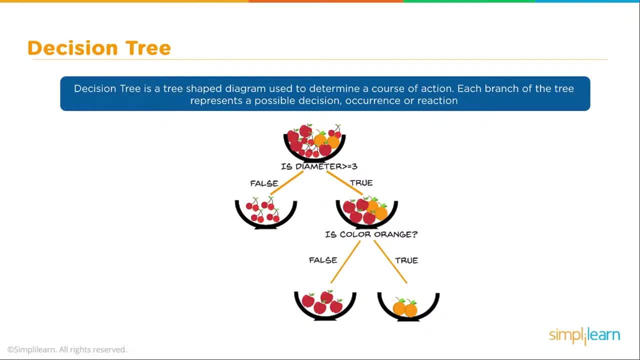 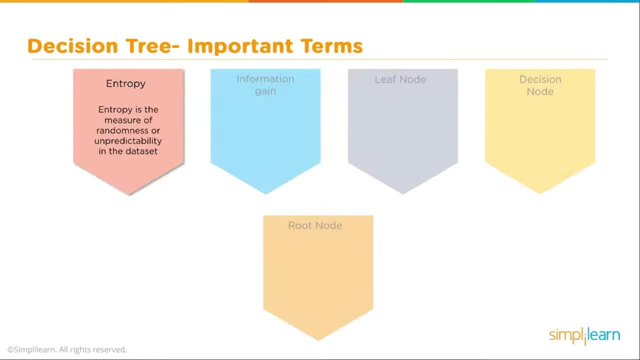 as the orange and if it's false, that leaves apples. So in this example, it sorts out the fruit in the bowl or the images of the fruit A decision tree. these are very important terms to know because these are very central to understanding the 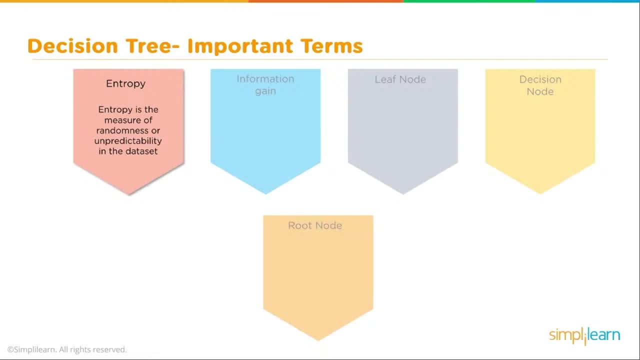 decision tree when working with them. The first is entropy. Everything on the decision tree and how it makes a decision is based on entropy. Entropy is a measure of randomness or unpredictability in the data set. Then they also have information gain- the leaf node, the decision. 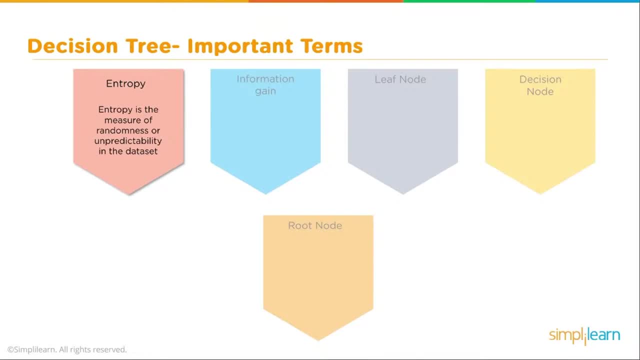 node and the root node. We'll cover these other four terms as we go down the tree, but let's start with entropy. So, starting with entropy, we have here a high amount of randomness. What that means is that whatever's coming out, 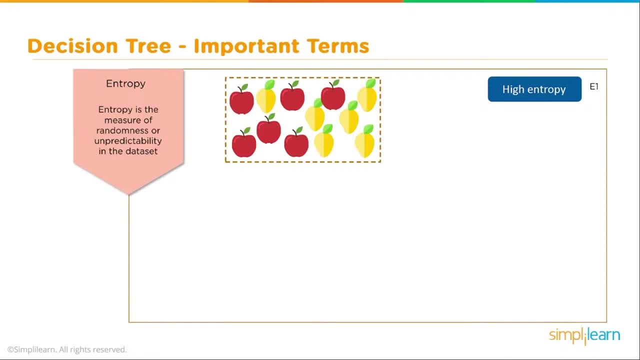 of this decision. if it was going to guess based on this data, it wouldn't be able to tell you whether it's a lemon or an apple. It would just say it's a fruit. So the first thing we want to do is we want 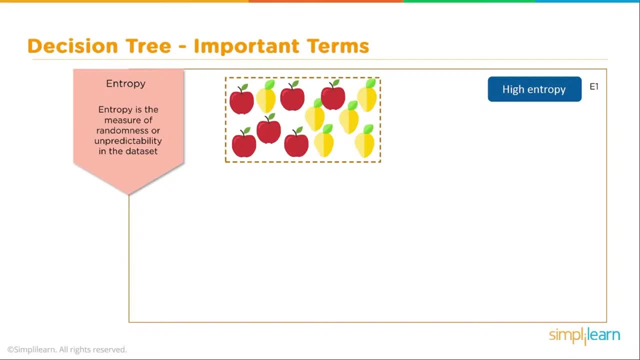 to split this apart and we take the initial data set and we're going to create a data set one and a data set two. We just split it in two And if you look at these new data sets after splitting them, the entropy of each 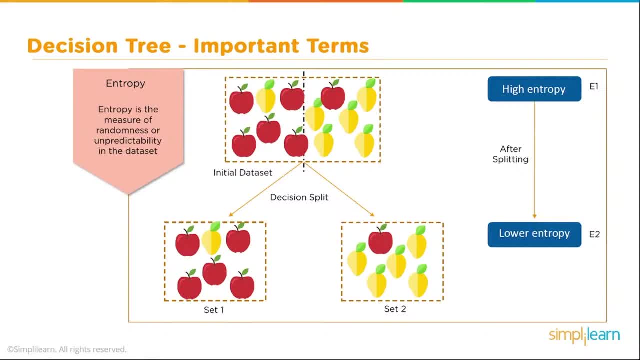 of those sets is much less So for the first one, whatever comes in there, it's going to sort that data and it's going to say, okay, if this data goes this direction, it's probably an apple, And if it goes into the other direction, it's. 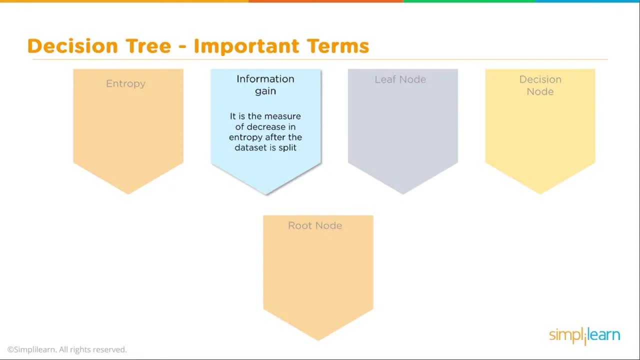 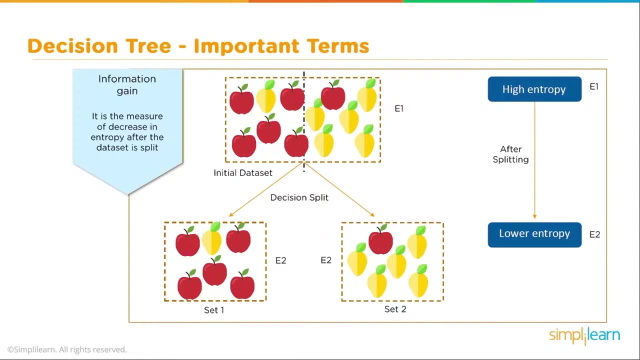 probably a lemon. So that brings us up to information gain. It is the measure of decrease in the entropy after the data set is split. What that means in here is that we've gone from one set which has a very high entropy to two lower sets of entropy. 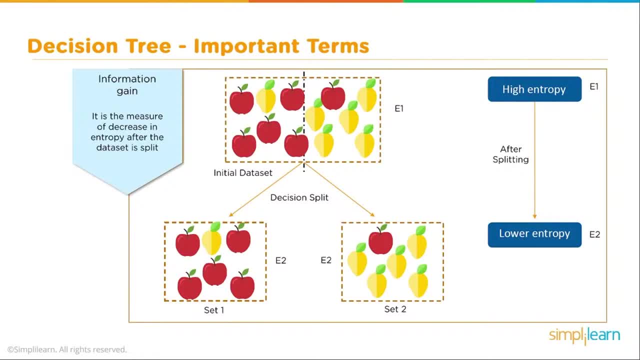 And we've added in the values of E1 for the first one and E2 for the second, two which are much lower, And so that information gain is increased greatly in this example, And so you can find that the information gain simply equals. 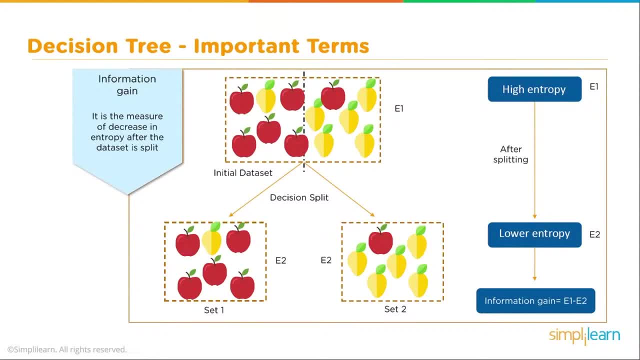 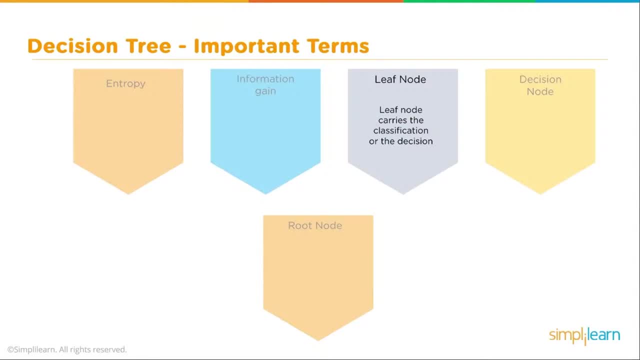 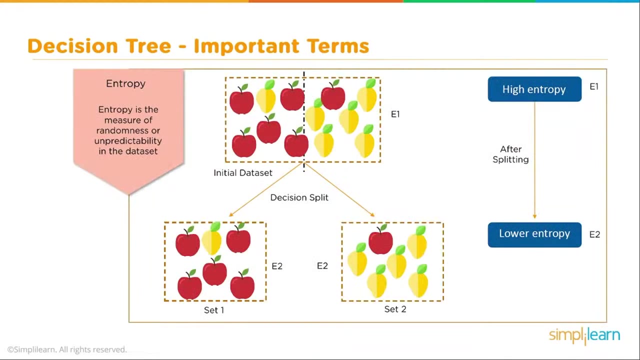 decision E1 minus E2.. As we're going down our list of definitions, we'll look at the leaf node, And the leaf node carries the classification or the decision. So we look down here to the leaf node. we finally get to our set one. 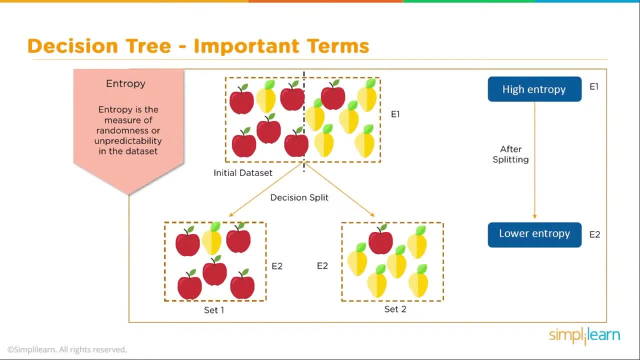 or our set two, When it comes down there and it says, okay, this object's gone into set one. if it's gone into set one, it's going to be split by some means and we'll either end up with apples on the leaf. 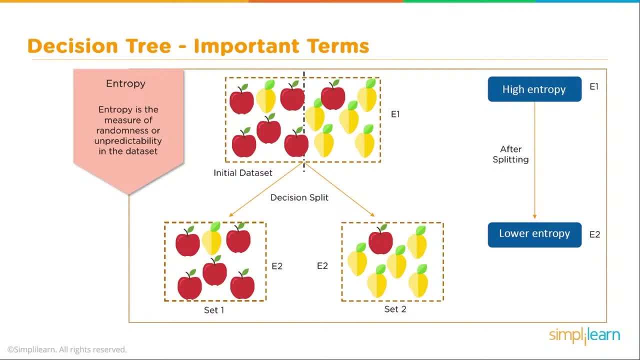 node or a lemon on the leaf node, and on the right it'll either be an apple or lemons. Those leaf nodes are those final decisions or classifications. That's the definition of leaf node in here. If we're going to have a final leaf, 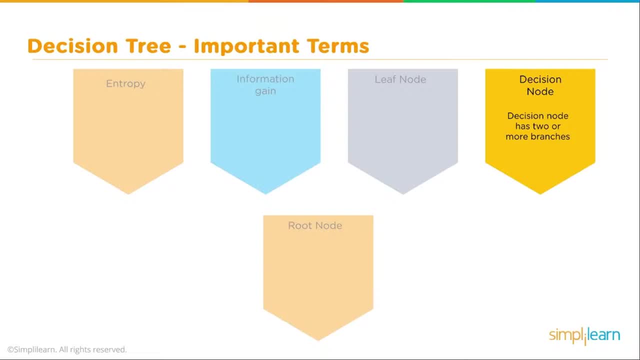 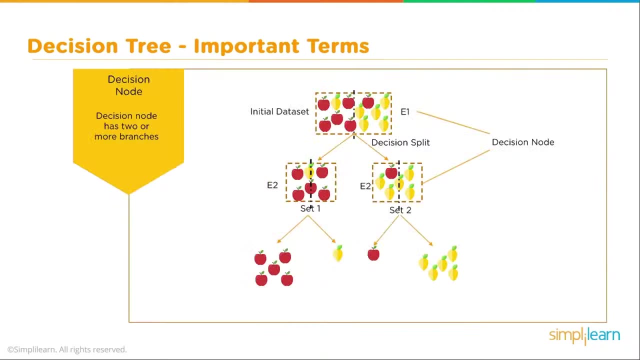 where we make the decision, we should have a name for the nodes above it and they call those decision nodes A decision node. a decision node has two or more branches And you can see here where we have the five apples and one lemon and in the other case the five. 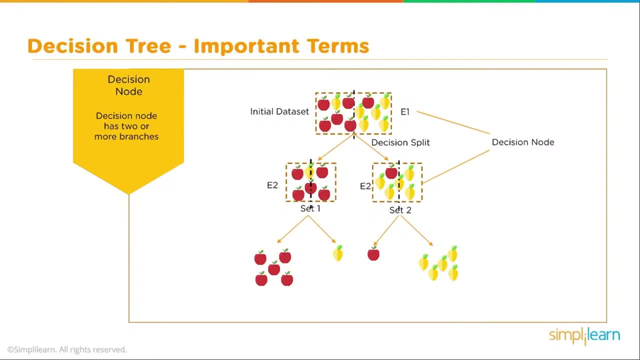 lemons and one apple. they have to make a choice of which tree it goes down, based on some kind of measurement or information given to the tree. And that brings us to our last definition. The root node, the top, most decision node, is known as: 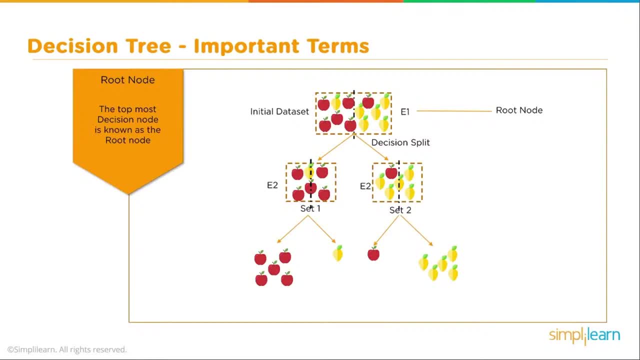 the root node And this is where you have all of your data and you have your first decision it has to make, or the first split in information. So far. we've looked at a very general image with the fruit being split. Let's look and. 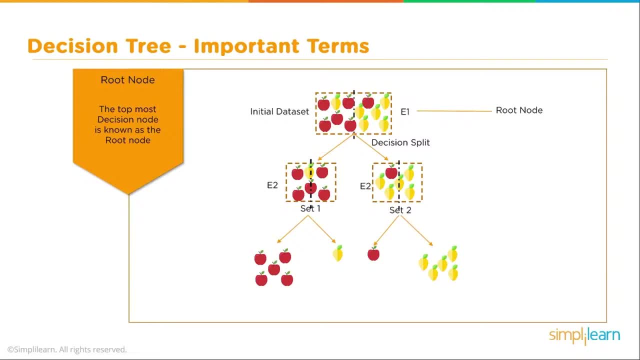 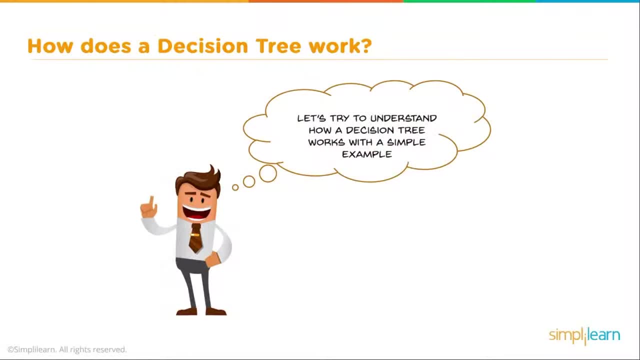 see exactly what that means to split the data and how do we make those decisions on there. Let's go in there and find out. how does a decision tree work. So let's try to understand this and let's use a simple example, and we'll stay with the fruit. 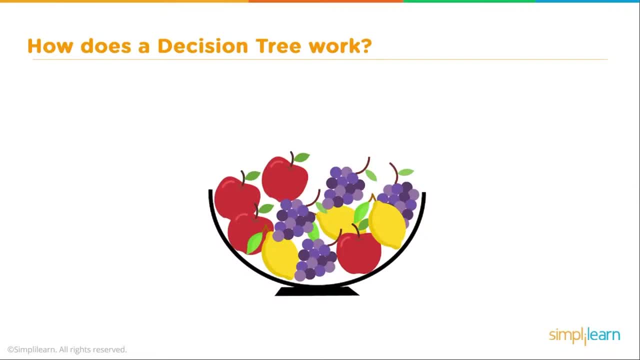 We have a bowl of fruit And so let's create a problem statement, and the problem is we want to classify the different types of fruits in the bowl based on different features. The data set in the bowl is looking quite messy and the entropy is high in this case. 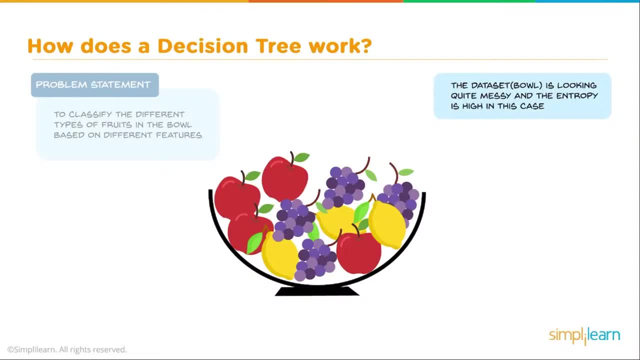 So if this bowl was our decision maker, it wouldn't know what choice to make. It has so many choices. Which one do you pick? apple, grape or lemons? And so we look in here we're going to start with a training set. So this is our data. 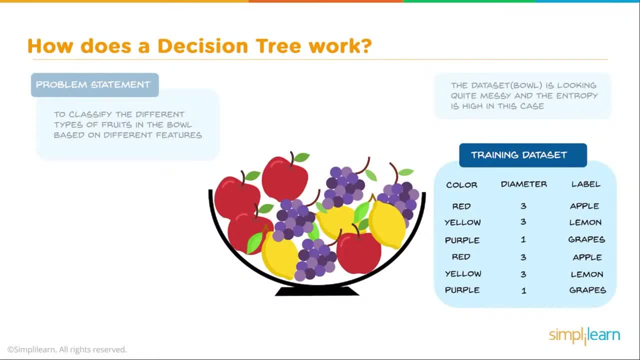 that we're training our data with And we have a number of options here. We have the color and under the color we have red, yellow, purple, We have a diameter 3-3-1-3-3-1 and we have a label. 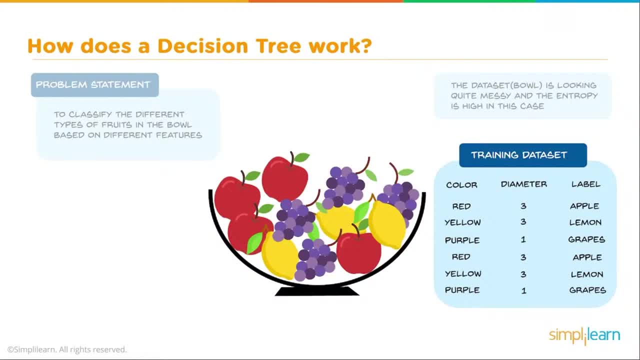 apple lemon grapes. apple lemon grapes. And how do we split the data? We have to frame the conditions to split the data in such a way that the information gain is the highest. It's very key to note that we're looking for the 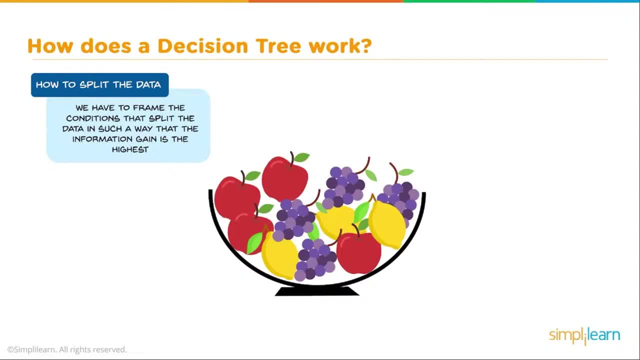 best gain. We don't want to just start sorting out the smallest piece in there. We want to split it the biggest way we can, And so we measure this decrease in entropy. that's what they call it entropy. there's our entropy after splitting. 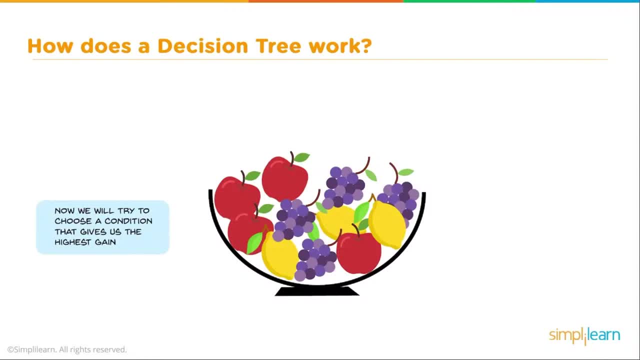 And now we'll try to choose a condition that gives us the highest gain. We will do that by splitting the data, using each condition and checking the gain that we get out of them. The conditions that give us the highest gain will be used to make. 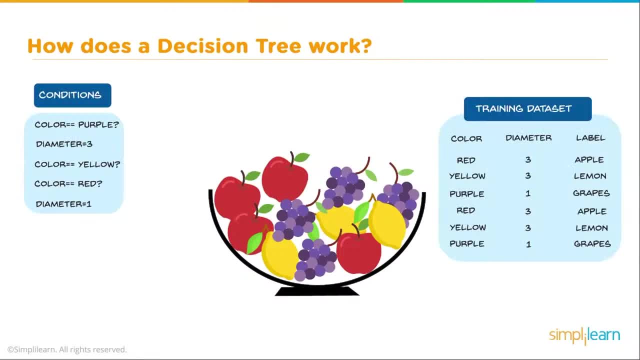 the first split. So let's take a look at these different conditions. We have color, we have diameter and if we look underneath that, we have a couple different values. We have: diameter equals 3,. color equals yellow, red. diameter equals 1.. 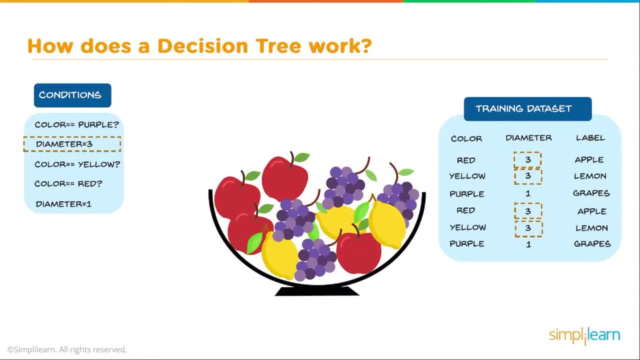 And when we look at that you'll see over here we have 1,, 2,, 3,, 4, 3's. That's a pretty hard selection. So let's say the condition gives us the maximum gain of 3.. 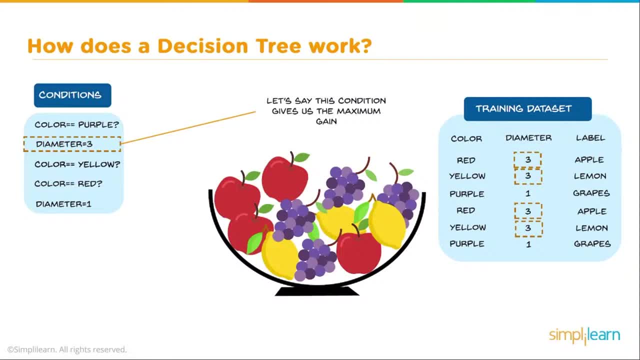 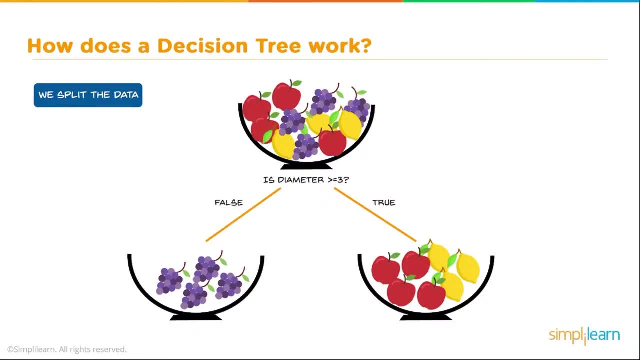 So we have the most pieces fall into that range. So our first split from our decision node is: we split the data based on the diameter. Is it greater than or equal to 3?? If it's not, that's false, it goes into the grape bowl. 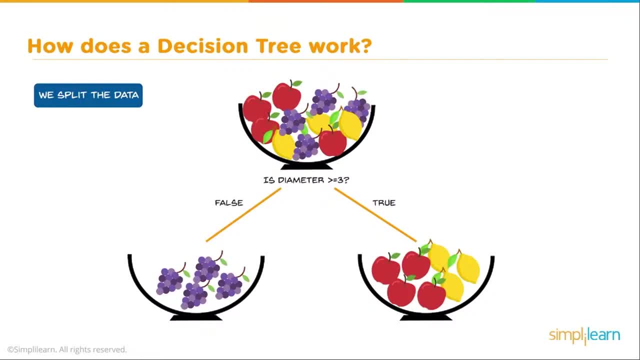 And if it's true, it goes into a bowl full of lemon and apples. The entropy after splitting has decreased considerably, So now we can make two decisions. if you look at, they're very much less chaos going on there. This node has already attained an entropy value of 0. 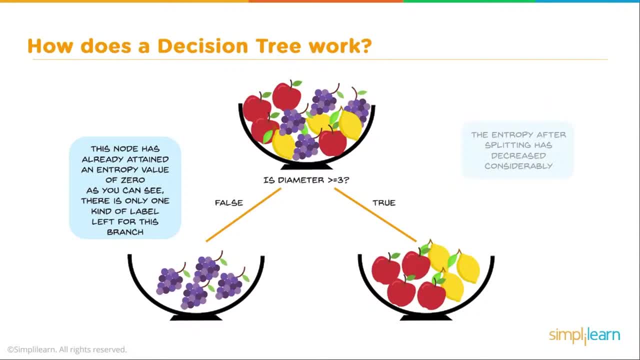 as you can see, There's only one kind of label left for this branch, So no further splitting is required for this node. However, this node on the right is still requires a split to decrease the entropy further. So we split the right node further based on color. 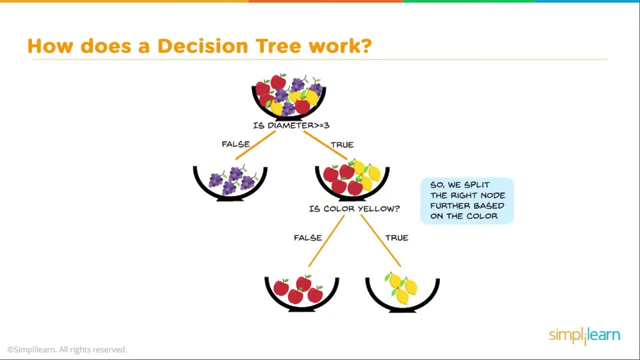 If you look at this, if I split it on color, that pretty much cuts it right down the middle. It's the only thing we have left in our choices of color and diameter too, And if the color is yellow, it's going to go to the right bowl. 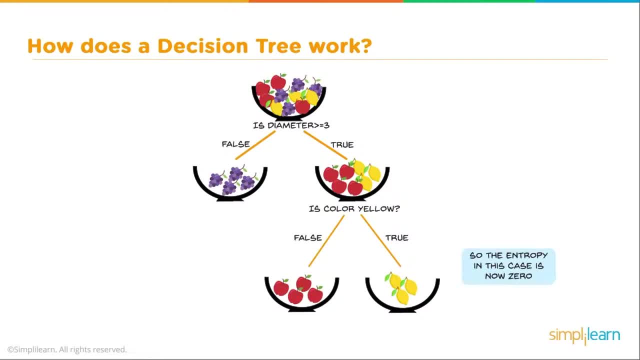 And if it's false, it's going to go to the left bowl. So the entropy in this case is now 0.. So now we have three bowls with 0 entropy. There's only one type of data in each one of those bowls. 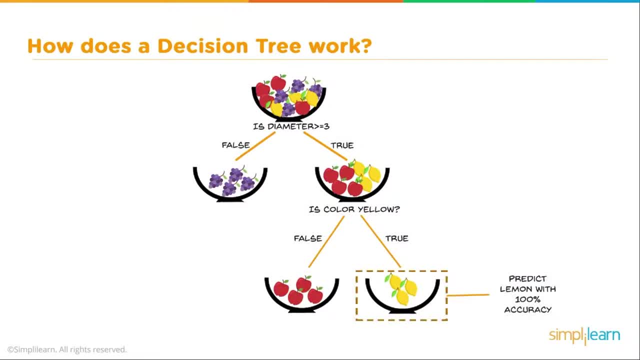 So we can predict a lemon with 100% accuracy And we can predict the apple also with 100% accuracy, along with our grapes up there. So we've looked at kind of a basic tree in our forest. but what we really want to know is how does a 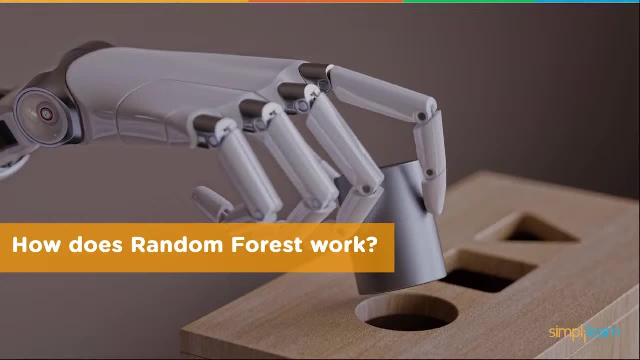 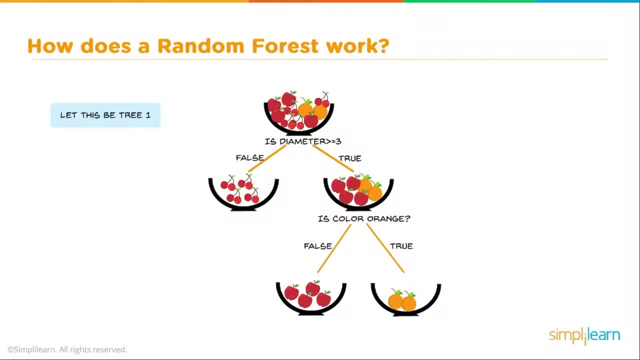 random forest work as a whole. So to begin our random forest classifier, let's say we already have built three trees And we're going to start with the first tree that looks like this, Just like we did in the example. this tree looks at the diameter If it's greater than. 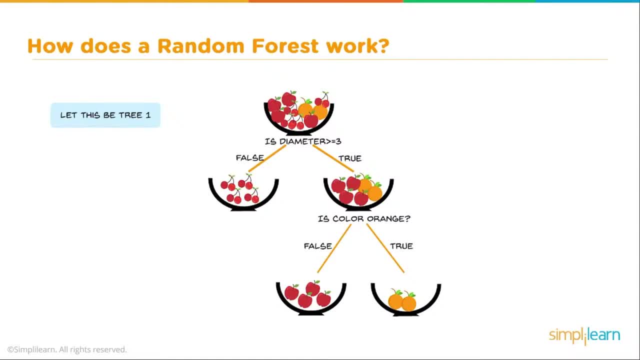 or equal to 3, it's true, Otherwise it's false. So one side goes to the smaller diameter, one side goes to the larger diameter, And if the color is orange it's going to go to the right, true. 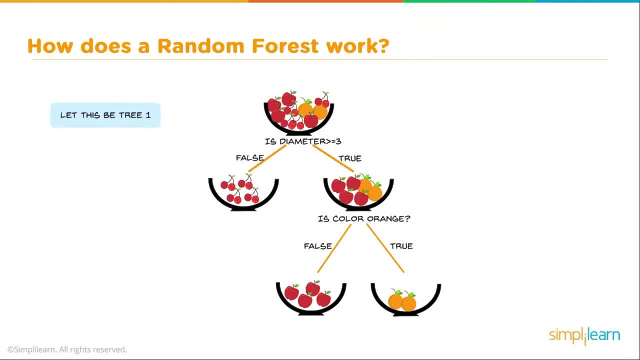 We're using oranges now instead of lemons, And if it's red it's going to go to the left- false. We build a second tree, very similar, but it's split differently. Instead of the first one being split by a diameter, this one- 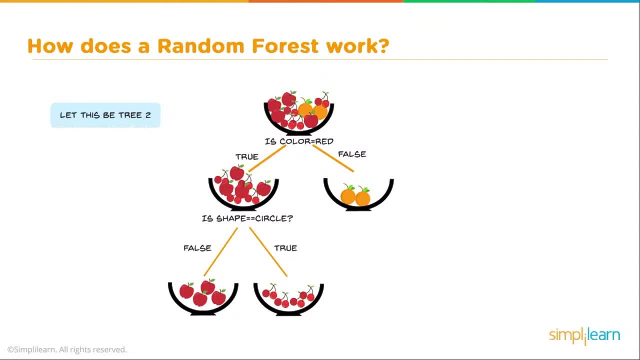 when they created it. if you look at that first bowl, it has a lot of red objects. So it says, is the color red? Because that's going to bring our entropy down the fastest. And so of course, if it's true, it goes to the left. 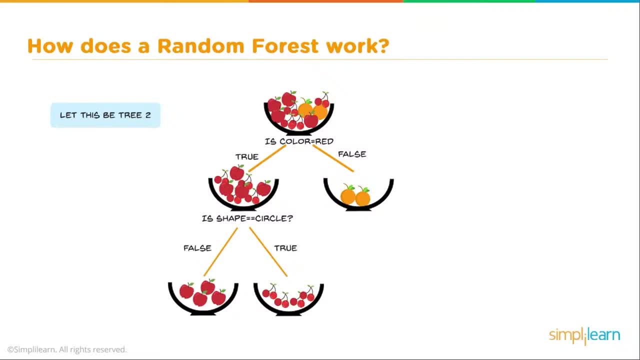 If it's false, it goes to the right And then it looks at the shape: false or true, and so on and so on. And tree 3, is the diameter equal to 1?? And it came up with this because there's a lot of cherries. 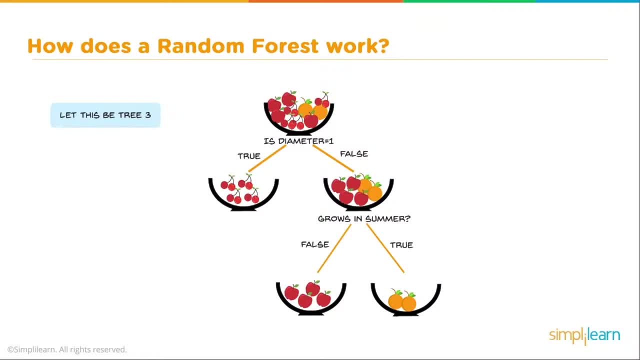 in this bowl, So that would be the biggest split on there. is the diameter equal to 1?? That's going to drop the entropy the quickest And, as you can see, it splits it into true if it goes false. and they've added another. 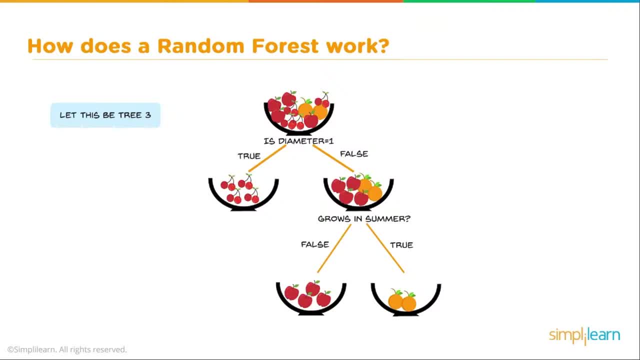 category: does it grow in the summer? And if it's false, it goes off to the left. If it's true, it goes off to the right. Let's go ahead and bring these three trees, so you can see them all in one image. 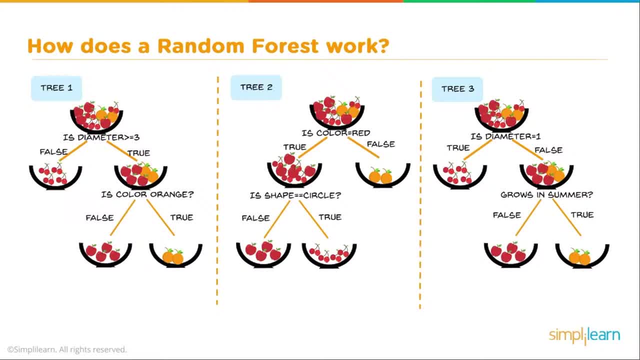 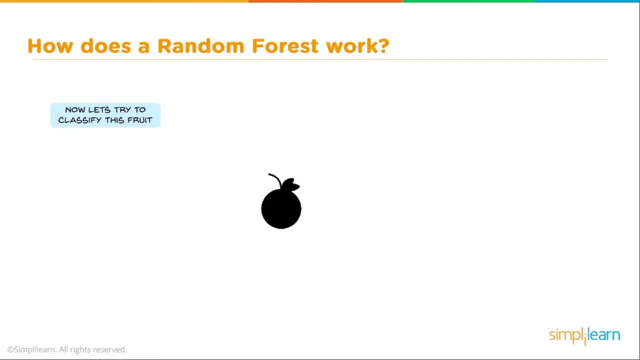 So this would be three completely different trees categorizing a fruit. And let's take a fruit. now let's try this and this fruit. if you look at it, we've blackened it out. You can't see the color on it. 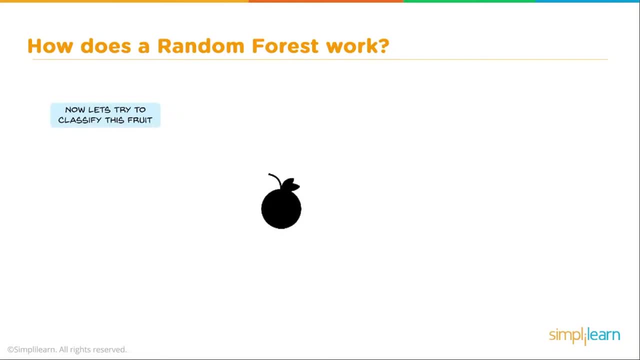 So it's missing data. Remember, one of the things we talked about earlier is that a random forest works really good if you're missing data, If you're missing pieces. So this fruit has an image, but maybe the person had a black and white camera when they took the picture. 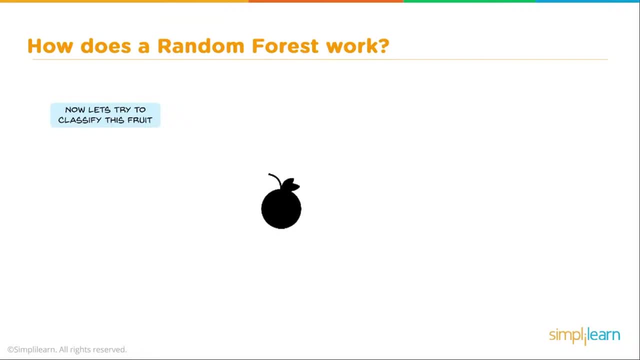 And we're going to take a look at this and it's going to have they put the color in there, so ignore the color down there. But the diameter equals 3, we find out it grows in the summer- equals yes. 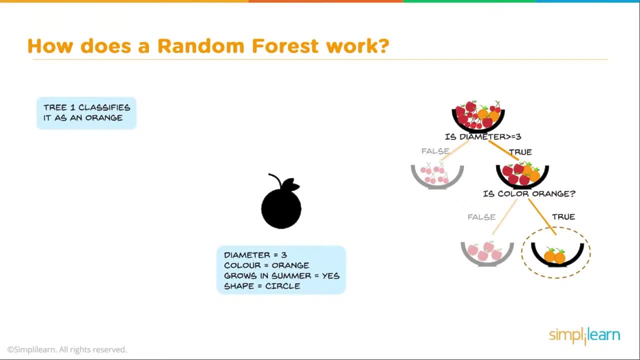 and the shape is a circle And if you go to the right you can look at what one of the decision trees did. this is the third one. Is the diameter greater than or equal to 3?? Is the color orange? Well, it doesn't really know. 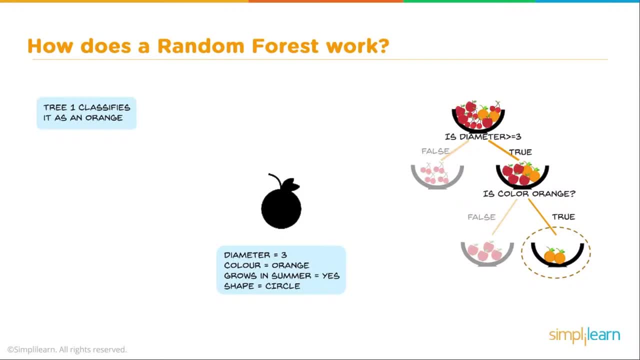 on this one. but if you look at the value, it'd say true and it'd go to the right Tree. 2 classifies it as: cherries. Is the color equal, red Is the shape- a circle? True, it is a circle. 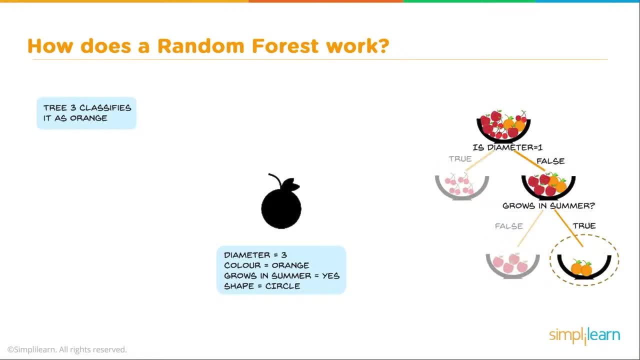 So this would look at it and say, oh, that's a cherry. And then we go to the other classifier and it says: is the diameter equal 1?? Well, that's false. Does it grow in the summer? True, So it goes down and looks at it as oranges. 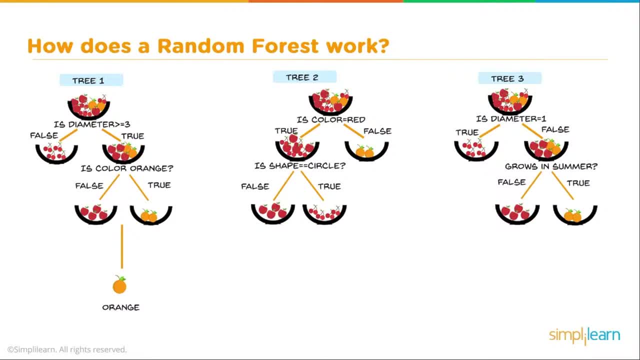 So how does this random forest work? The first one says it's an orange, The second one said it was a cherry And the third one says, hmm, it's an orange. And you can guess that if you have two oranges and one says 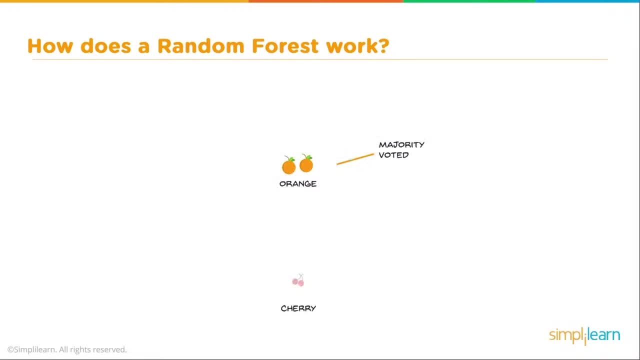 it's a cherry. when you add that all together, the majority of the vote says orange. So the answer is: it's classified as an orange, Even though we didn't know the color and we're missing data on it. I don't know about you. 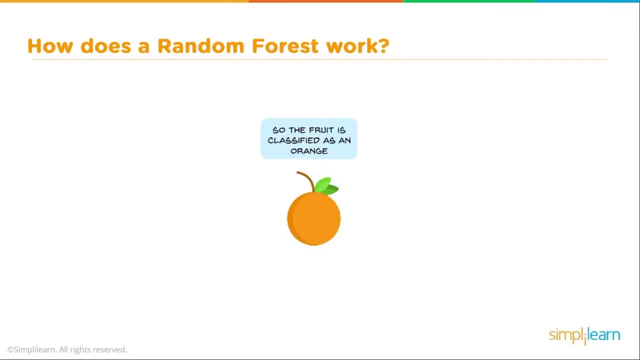 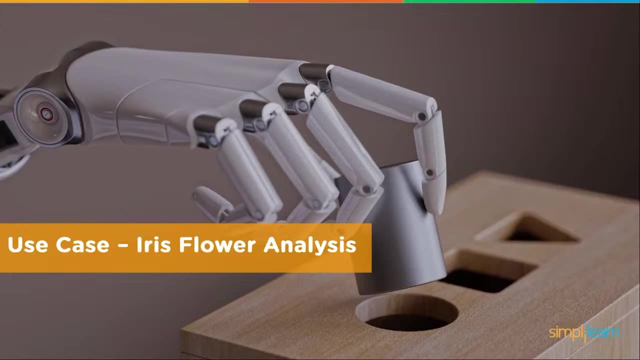 but I'm getting tired of fruit, So let's switch, and I did promise you we'd start looking at a case example and get into some Python coding. Today we're going to use the case the iris flower analysis. Ooh, this is the exciting part, as 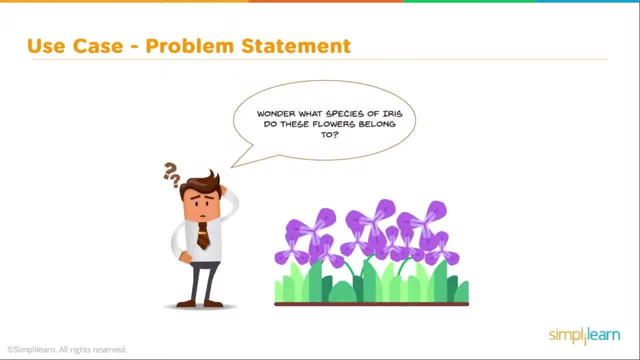 we roll up our sleeves and actually look at some Python coding. Before we start the Python coding, we need to go ahead and create a problem statement, Wonder: what species of iris do these flowers belong to? Let's try to predict the species of the flowers using machine. 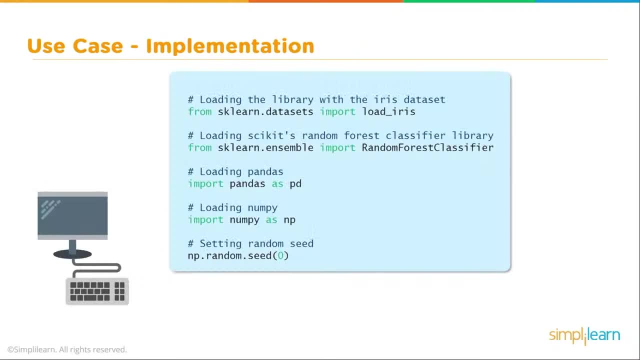 learning in Python. Let's see how it can be done. So here we begin to go ahead and implement our Python code, And you'll find that the first half of our implementation is all about organizing and exploring the data coming in. Let's go ahead and take this first. 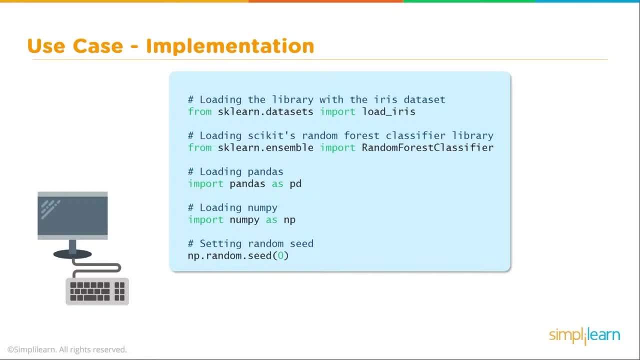 step, which is loading the different modules into Python, and let's go ahead and put that in our favorite editor. whatever your favorite editor is, In this case, I'm going to be using the Anaconda Jupyter Notebook, which is one of my favorites, Certainly. 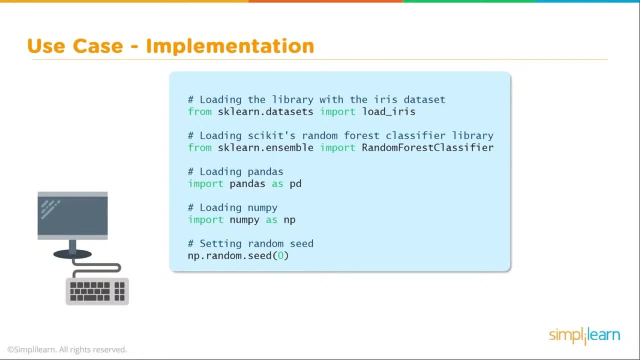 there's Notepad++ and Eclipse and dozens of others, or just even using the Python terminal window. Any of those will work just fine to go ahead and explore this Python coding. So here we go. let's go ahead and flip over to our Jupyter. 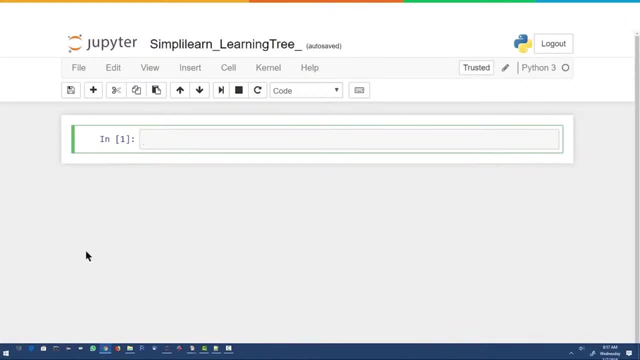 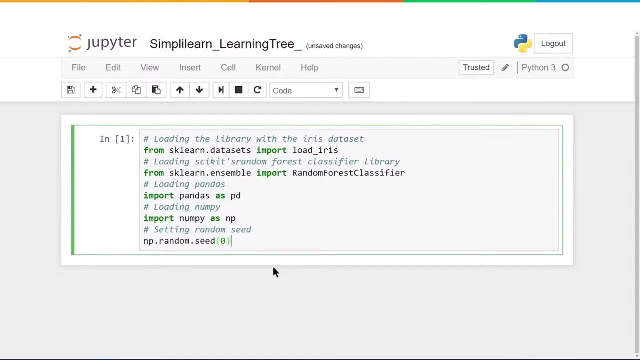 Notebook and I've already opened up a new page for Python 3 code and I'm just going to paste this right in there And let's take a look and see what we're bringing into our Python. The first thing we're going to do is, from the 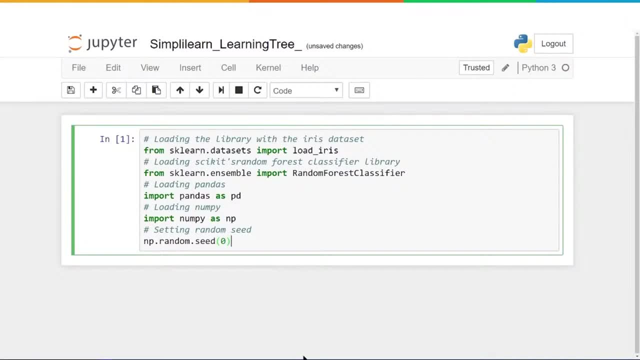 sklearndatasets import loadiris. Now, this isn't the actual data. this is just the module that allows us to bring in the data. the loadiris And the iris is so popular. it's been around since 1936, when Ronald Fisher published a paper on it. 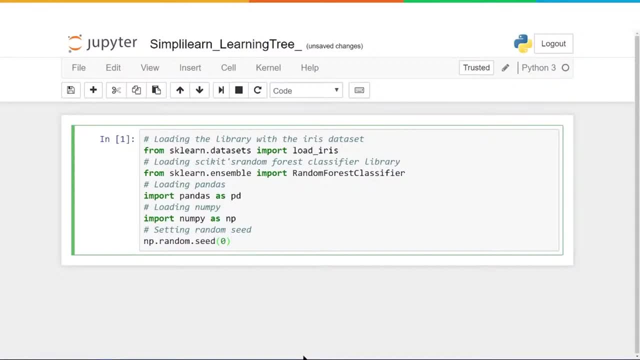 and they're measuring the different parts of the flower and, based on those measurements, predicting what kind of flower it is. And then, if we're going to do a random forest classifier, we need to go ahead and import a random forest classifier from the. 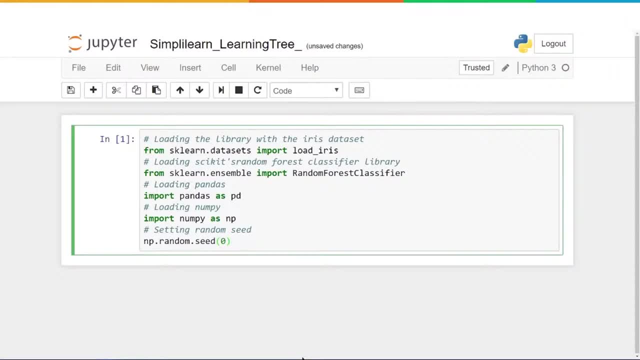 sklearn module, so sklearnensemble- import random forest classifier. and then we want to bring in two more modules, And these are probably the most commonly used modules in Python and data science. with any of the other modules that we bring in- And one is going to be pandas, so we're going to 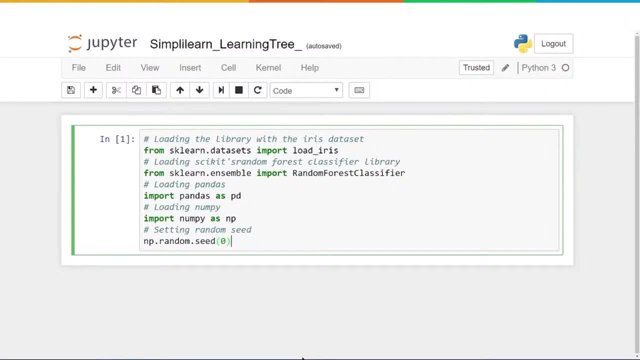 import pandas as pd. pd is the common term used for pandas, and pandas is basically a data format for us, where when you create a pandas data frame, it looks like an XScale spreadsheet And you'll see that in a minute when we start. 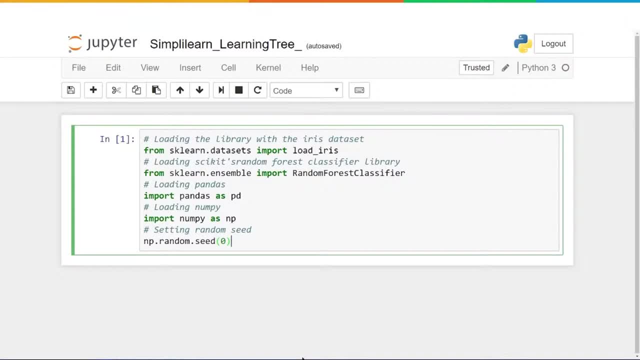 digging deeper into the code. Pandas is just wonderful because it plays nice with all the other modules in there. And then we have numpy, which is our numbers Python, and the numbers Python allows us to do different mathematical sets on here. We'll see. 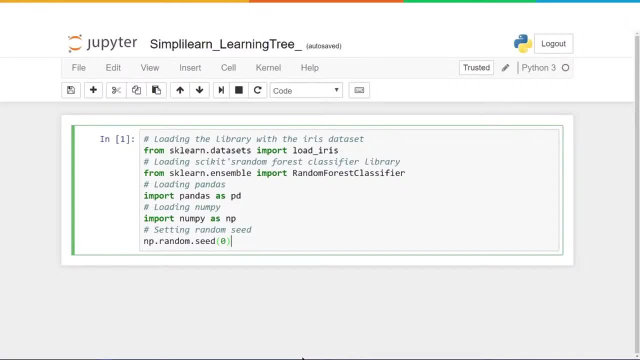 right off the bat. we're going to take our np and we're going to go ahead and seed the randomness with it with 0, so prandomseed because seeding that is 0. This code doesn't actually show anything. We're going to go ahead and run it. 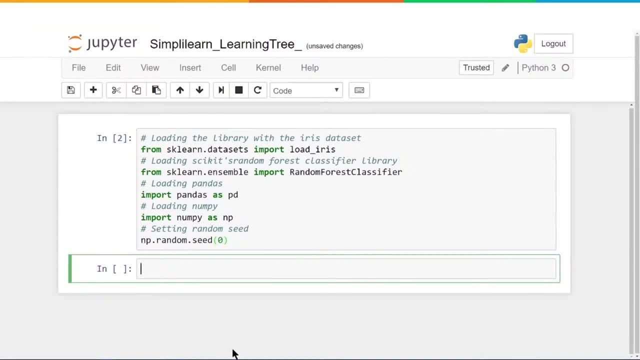 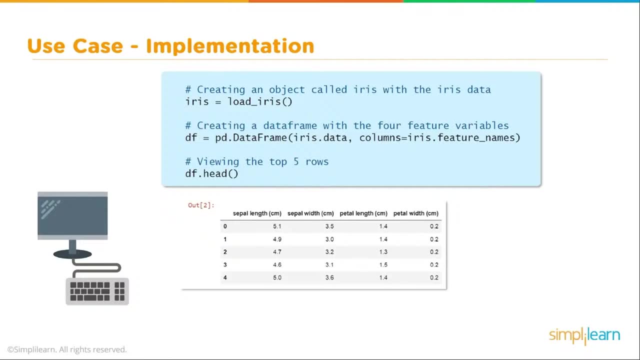 because I need to make sure I have all those loaded. And then let's take a look at the next module on here. The next six slides, including this one, are all about exploring the data. Remember I told you half of this is about 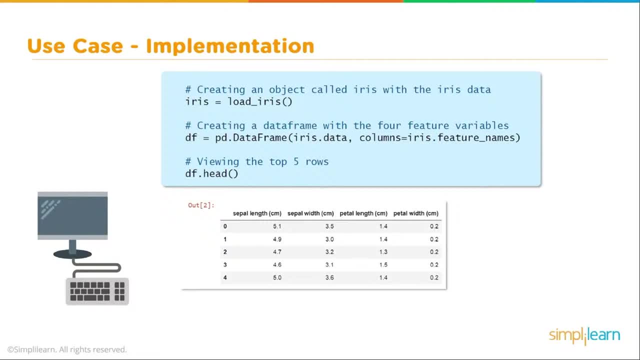 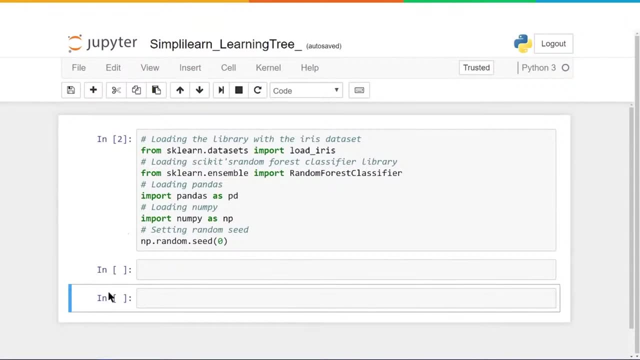 looking at the data and getting it all set. So let's go ahead and take this code right here, the script, and let's get that over into our Jupyter notebook. And here we go. we've gone ahead and run the imports and I'm going to paste the code down here. 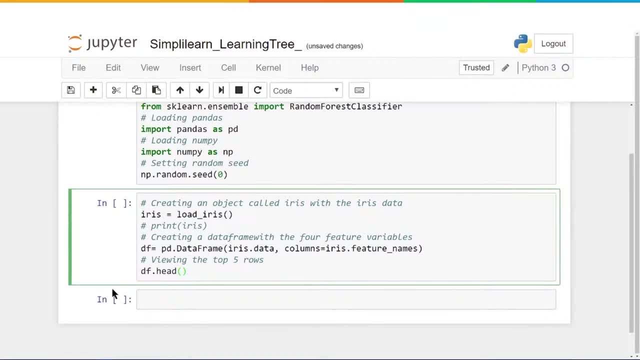 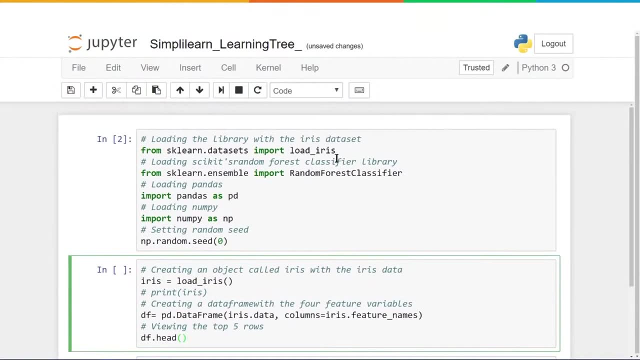 And let's take a look and see what's going on. The first thing we're doing is we're actually loading the iris data And, if you remember, up here we loaded the module that tells it how to get the iris data. Now we're actually assigning that data. 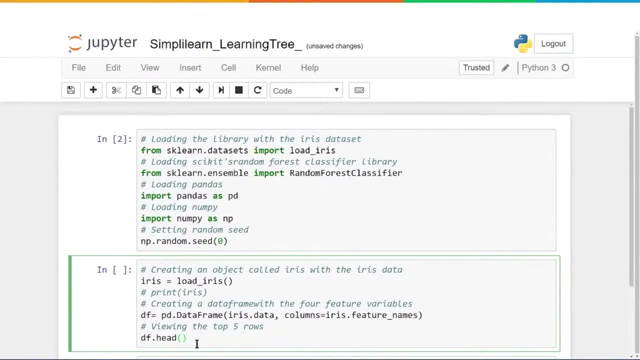 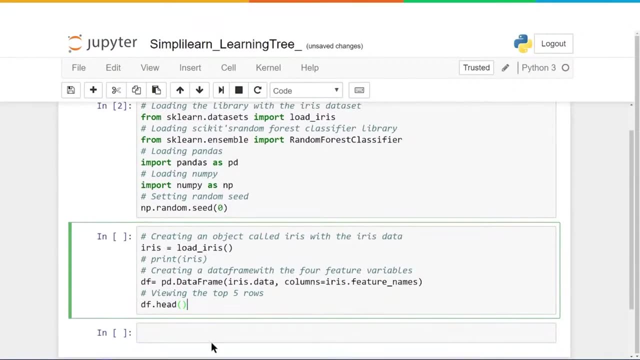 to the variable iris. And then we're going to go ahead and use the df to define data frame And that's going to equal pd and if you remember, that's pandas as pd. So that's our pandas And panda data frame. and then we're 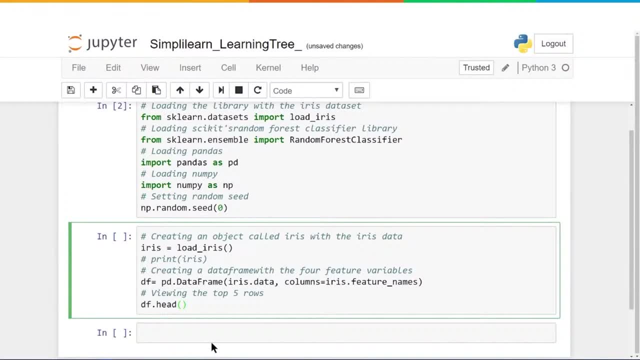 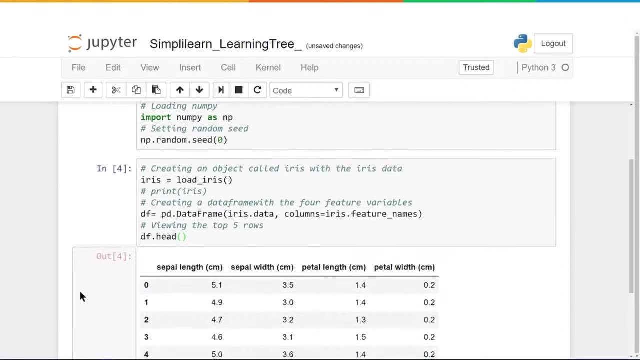 looking at iris data and columns equals iris feature names, And we're going to do the df head And let's run this so you can understand what's going on here. The first thing you want to notice is that our df has created what looks like an 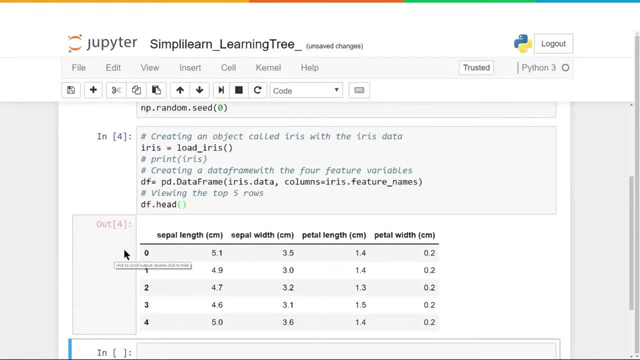 Excel spreadsheet And in this Excel spreadsheet we have set the columns. So up on the top you can see the four different columns, And then we have the data- irisdata- down below. It's a little confusing, without knowing where this data is coming from. 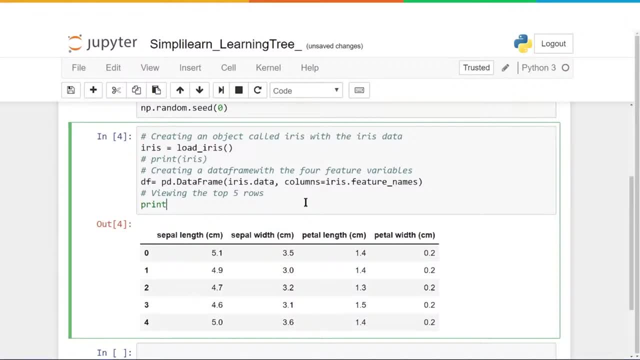 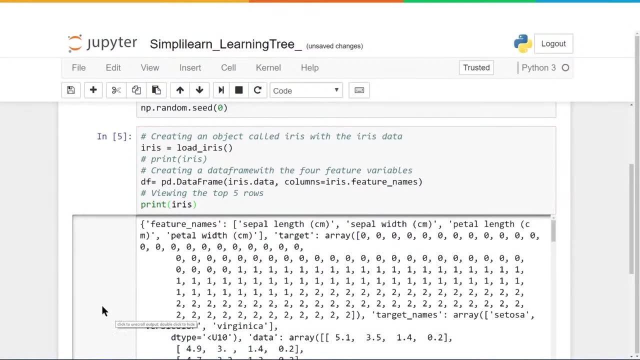 So let's look at the bigger picture And I'm going to go print- I'm just going to change this for a moment- And we're going to print all of iris and see what that looks like. So when I print all of iris, I get this long. 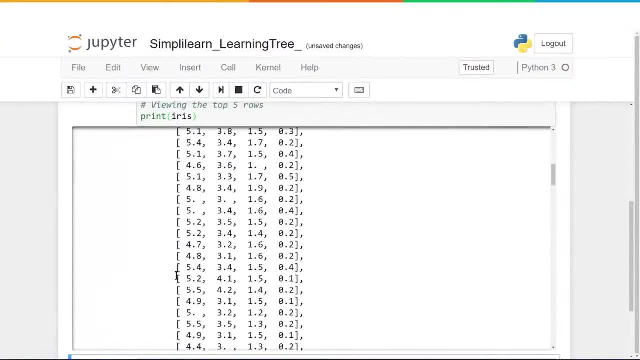 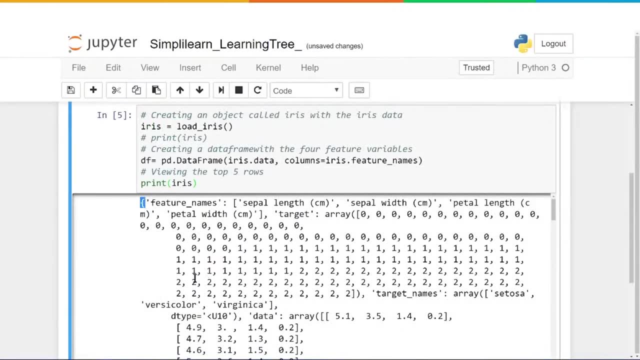 list of information And you can scroll through here and see all the different titles on there. What's important to notice is that, first off, there's brackets at the beginning. So this is a Python dictionary, And in a Python dictionary you'll have: 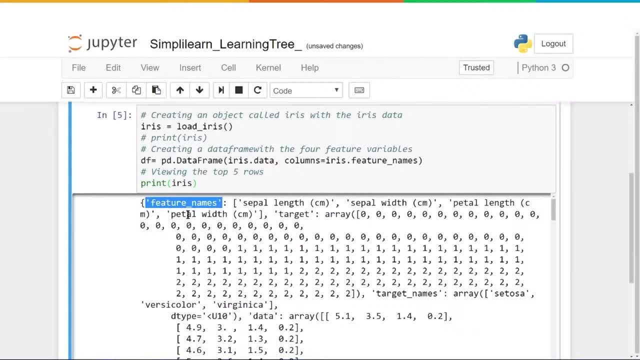 a key or a label, And this label pulls up whatever information comes after it. So feature names, which we actually used over here under columns, is equal to an array of sepal length, sepal width, petal length, petal width. These are the 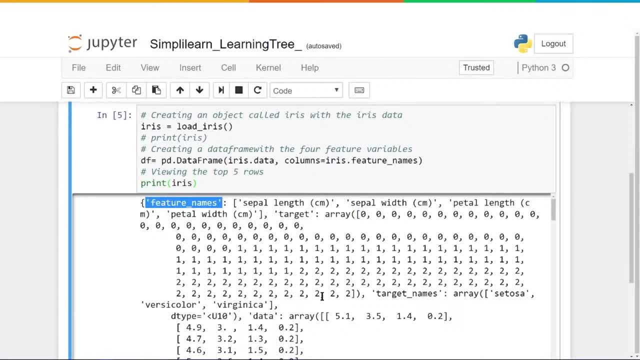 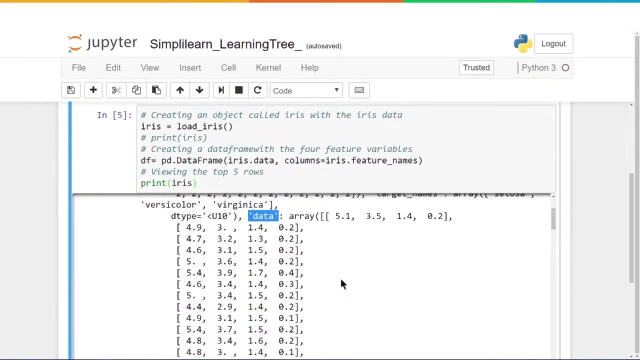 different names they have for the four different columns And if you scroll down far enough, you'll also see data down here. Oh goodness, it came up right towards the top And data is equal to the different data we're looking at Now. there's a lot of other things in. 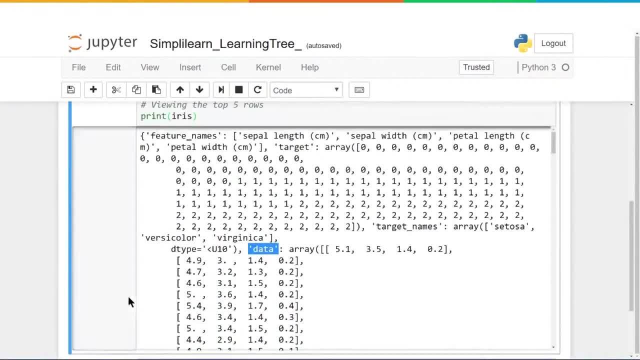 here like target. We're going to be pulling that up in a minute And there's also the names, the target names, which is further down, And we'll show you that also in a minute. Let's go ahead and set that back. 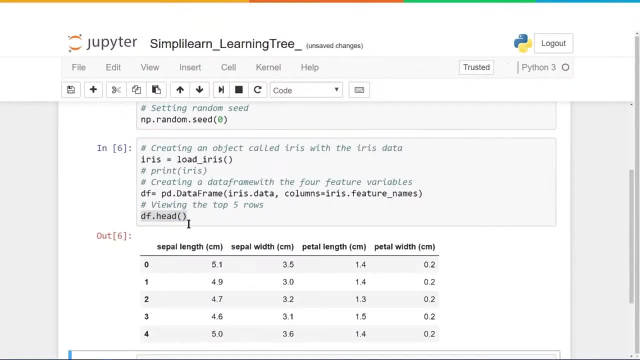 to the head, And this is one of the neat features of pandas and panda dataframes is, when you do dfhead or the panda dataframehead, it'll print the first five lines of the dataset in there, Along with the headers, if you have. 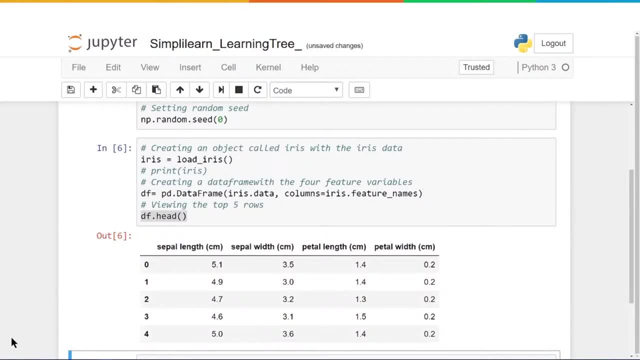 it. In this case we have the column headers set to iris features And in here you'll see that we have 0,, 1,, 2,, 3, 4.. In Python, most arrays always start at 0.. 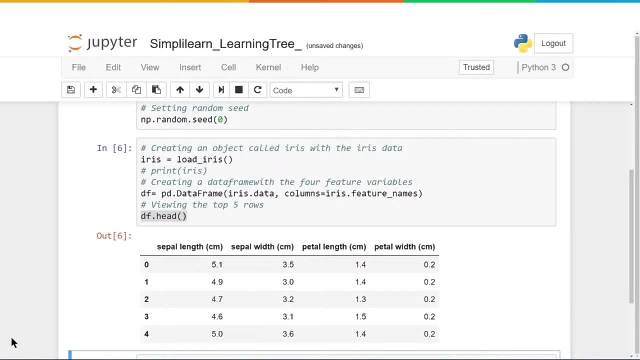 So when you look at the first five, it's going to be 0,, 1,, 2, 3, 4,, not 1, 2, 3, 4, 5.. So now we've got our iris data imported into. 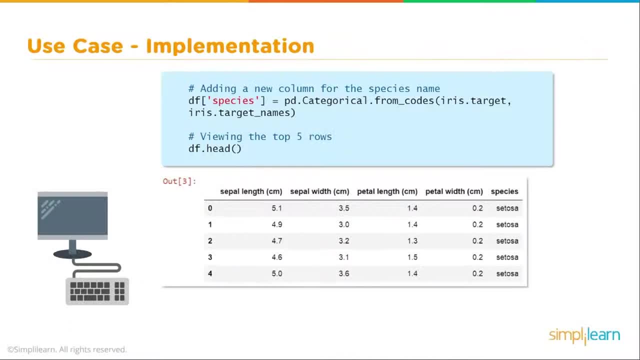 a dataframe. Let's take a look at the next piece of code in here, And so in this section here of the code, we're going to take a look at the target And let's go ahead and get this into our notebook, this piece of code. 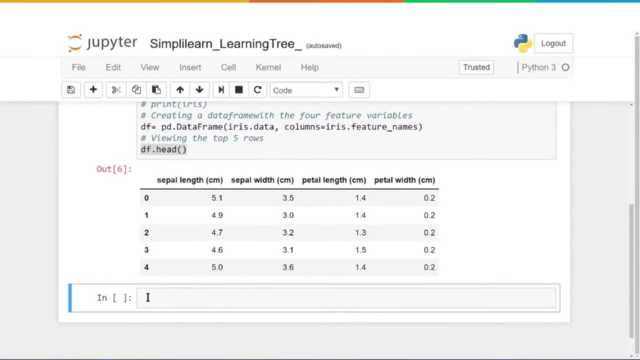 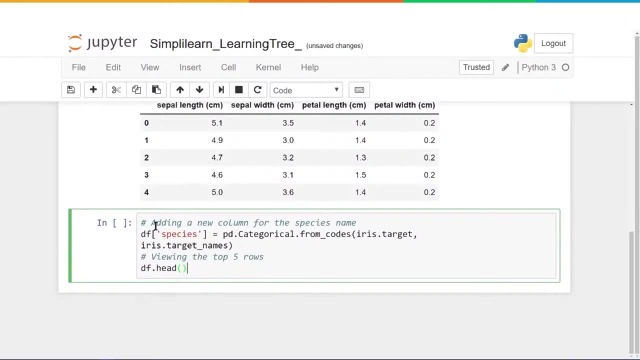 so we can discuss it a little bit more in detail. So here we are in our Jupyter notebook. I'm going to put the code in here And before I run it I want to look at a couple things going on. So we have df. 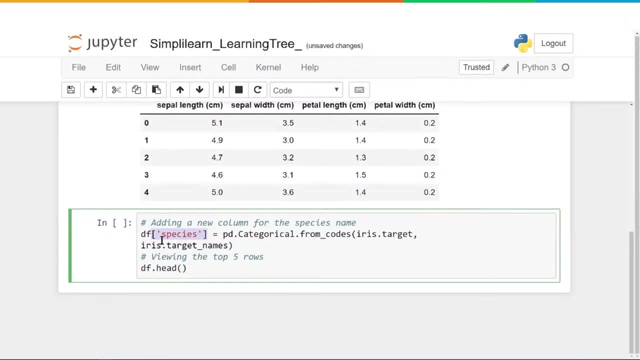 species. And this is interesting because right here you'll see where I have df species in brackets, which is the key code for creating another column, And here we have iristarget. Now these are both in the pandas setup on here, So in pandas we can do either one. 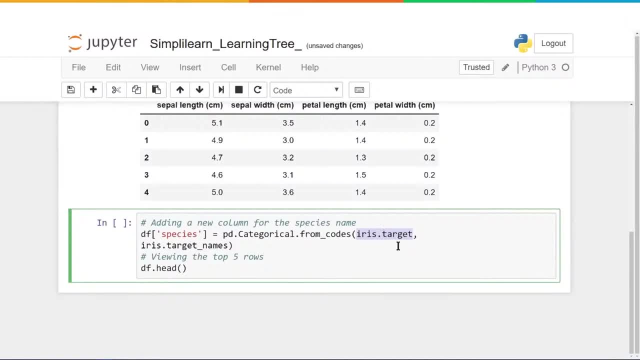 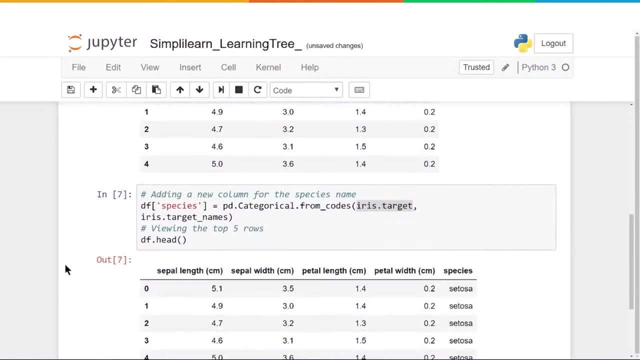 I could have just as easily done iris and then, in brackets, target. depending on what I'm working on, Both are acceptable. Let's go ahead and run this code and see how this changes, And what we've done is we've added the target. 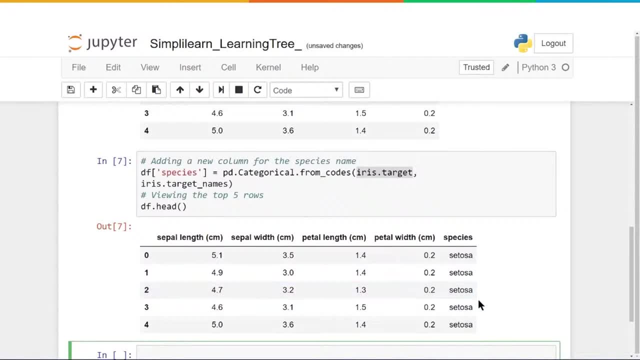 from the iris dataset as another column on the end. Now, what species is? this is what we're trying to predict. So we have our data, which tells us the answer for all these different pieces, And then we've added a column with the answer. That way, when we do, 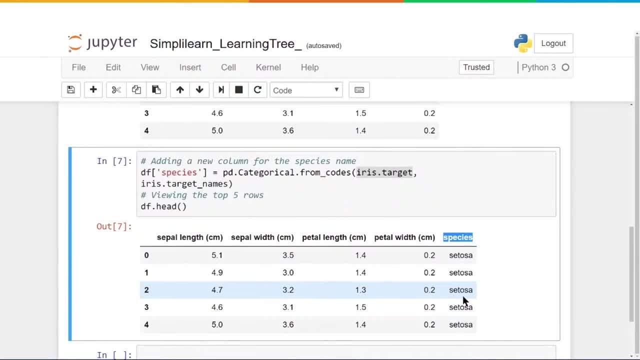 our final setup, we'll have the ability to program our neural network to look for this different data and know what a cetosa is, or a vericolor, which we'll see in just a minute, or virginica. Those are the three that are in there, And now we're going to add: 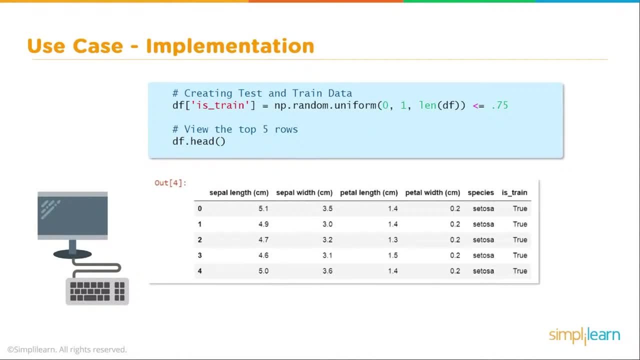 one more column. I know we're organizing all this data over and over again. It's kind of fun. There's a lot of ways to organize it. What's nice about putting everything onto one data frame is I can then do a printout. 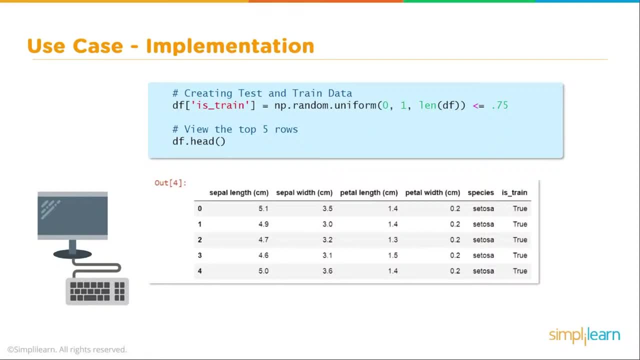 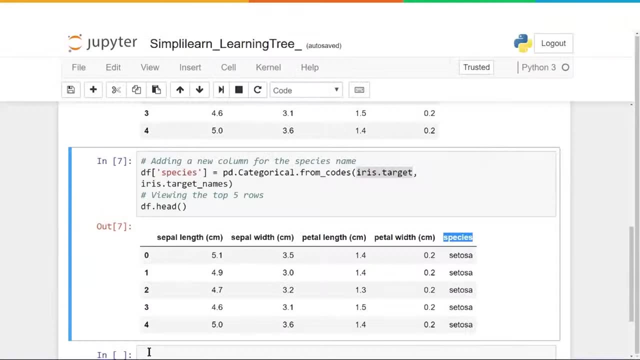 and it shows me exactly what I'm looking at And I'll show you where that's different, Where you can alter that and do it slightly differently. But let's go ahead and put this into our script up to that now. And here we go, We're going to put that. 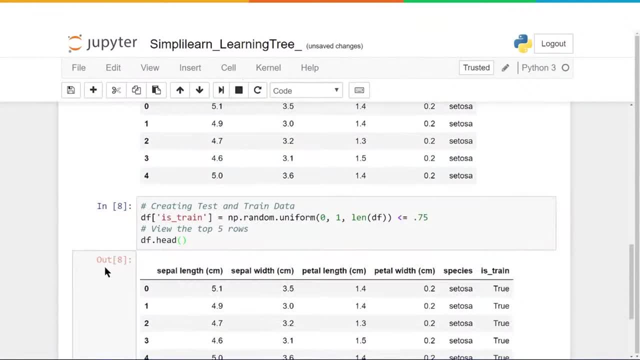 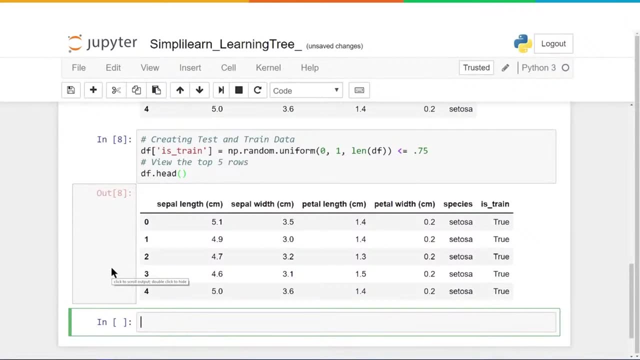 down here And we're going to run that, And let's talk a little bit about what we're doing Now. we're exploring data and one of the challenges is knowing how good your model is. Did your model work? And to do this, we need to split. 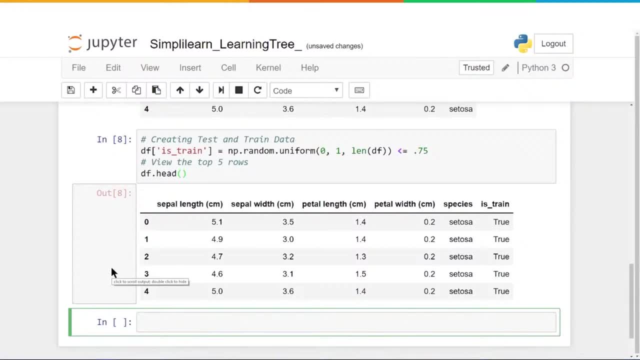 the data And we split it into two different parts. They usually call it the training and the testing, And so in here we're going to go ahead and put that in our database so you can see it clearly, And we've set it df. 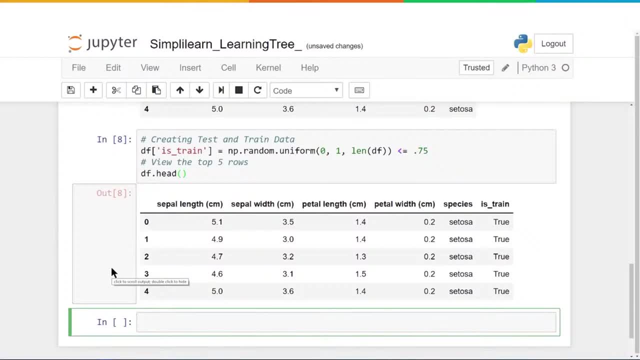 and remember you can put brackets. This is creating another column Is trained, So we're going to use part of it for training. And this equals np. Remember that stands for numpy, randomuniform, So we're generating a random number between 0 and 1.. 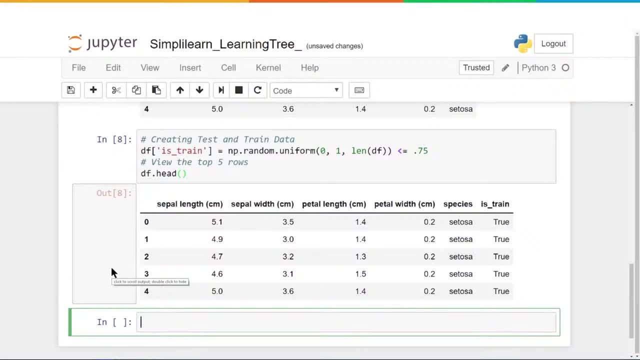 And we're going to do it for each of the rows. That's where the length df comes from. So each row gets a generated number, And if it's less than .75, it's true, And if it's greater than .75, it's false. This means we're. 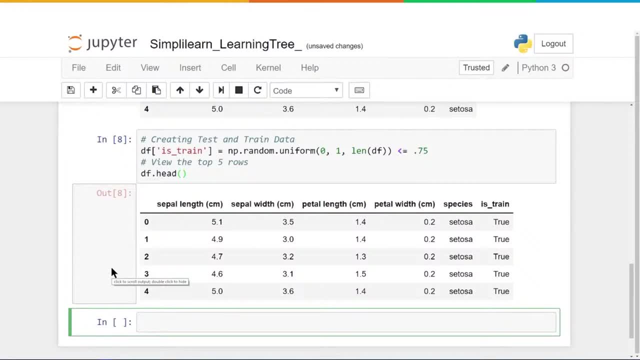 going to take 75% of the data roughly, because there's a randomness involved And we're going to use that to train it, And then the other 25% we're going to hold off to the side and use that to test it later on. 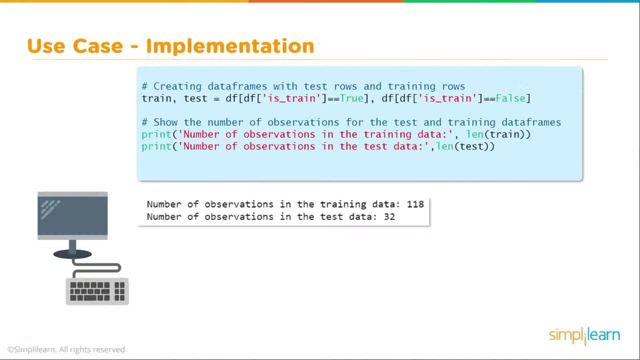 So let's flip back out over and see what the next step is. So, now that we've labeled our database for which is training and which is testing, let's go ahead and sort that into two different variables, Train and test. And let's take this code and let's 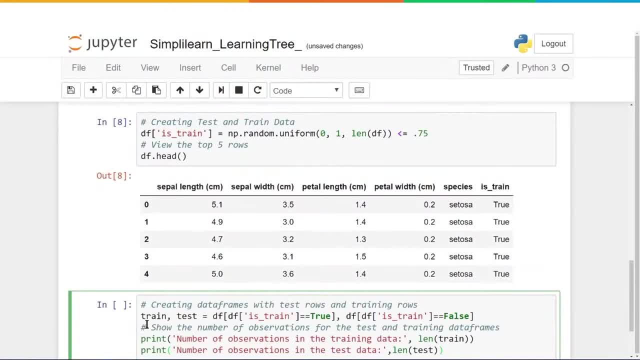 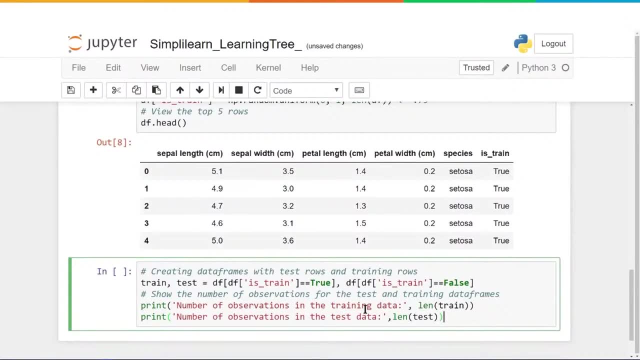 bring it into our project. And here we go, Let's paste it on down here. And before I run this, let's just take a quick look at what's going on here. We have up above, we created, remember there's our 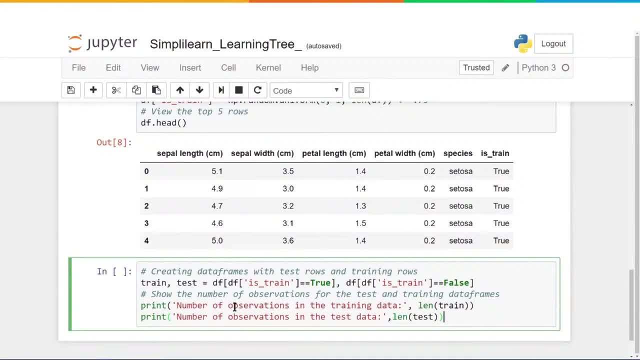 defhead which prints the first five rows, And we've added a column: is train at the end, And so we're going to take that and we're going to create two variables. We're going to create two new data frames: One's called train, One's called 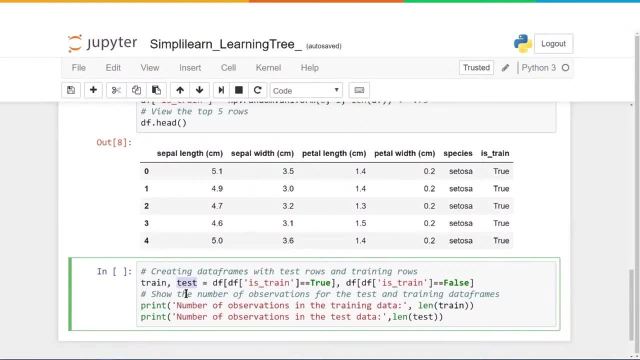 test: 75% in train, 25% in test- And then to sort that out, we're going to do that by doing df, our original data frame, with the iris data in it, And if df is train equals true, that's going to go in the train. 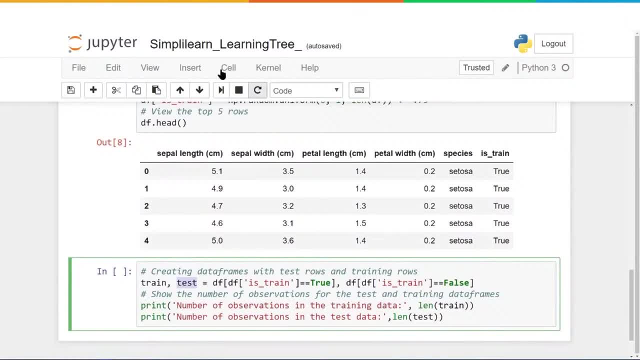 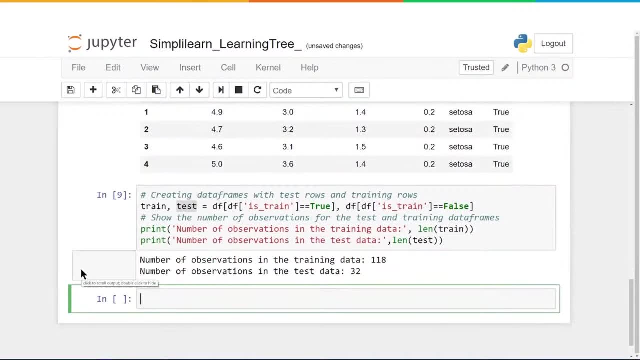 And if df is train equals false, it goes in the test, And so when I run this, we're going to print out the number in each one. Let's see what that looks like, And you'll see that it puts 118 in the. 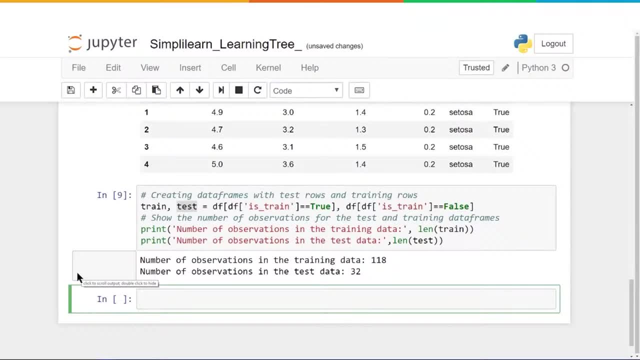 training module And it puts 32 in the testing module, Which lets us know that there was 150 lines of data in here. So if you went and looked at the original data, you could see that there's 150 lines And that's roughly 75% in one. 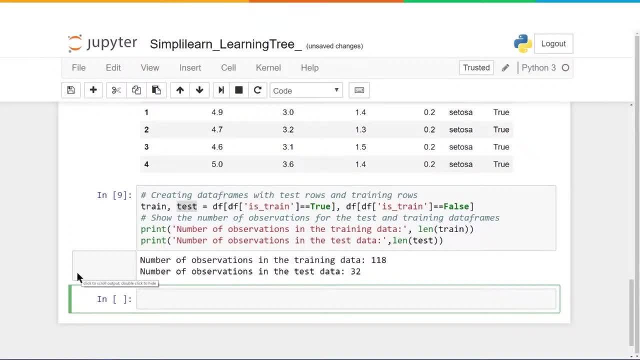 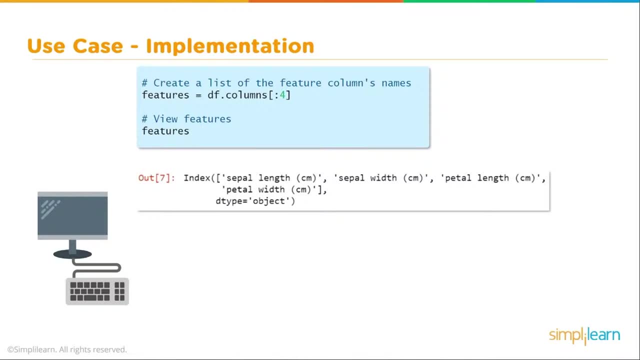 and 25% for us to test our model on afterward. So let's jump back to our code and see where this goes. In the next two steps, we want to do one more thing with our data, And that's make it readable to humans. 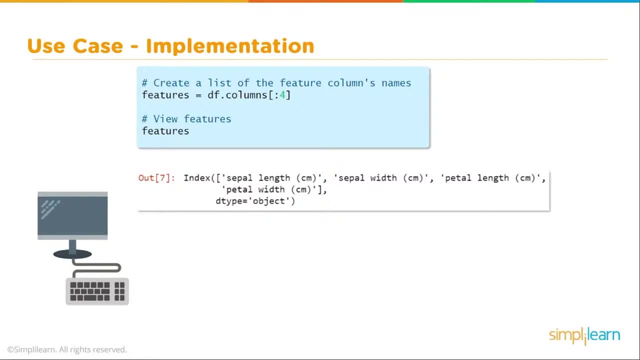 I don't know about you, but I hate looking at zeros and ones. So let's start with the features And let's go ahead and take those and make those readable to humans And let's put that in our code. Let's see, here we go, paste it in. 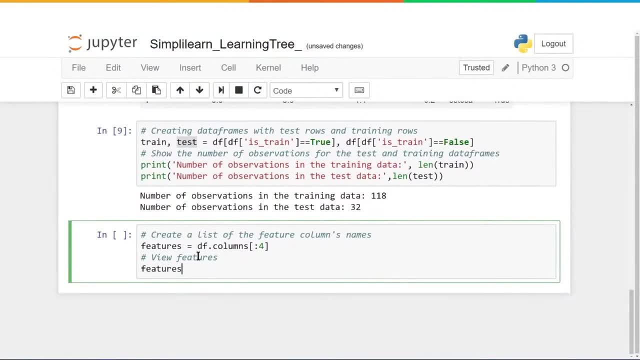 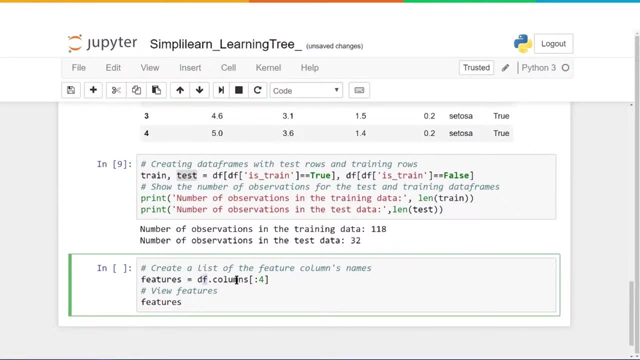 And you'll see here we've done a couple very basic things. We know that the columns in our data frame- again this is a panda thing- the DF columns, And we know the first four of them: 0,, 1,, 2, 3, that'd be the first. 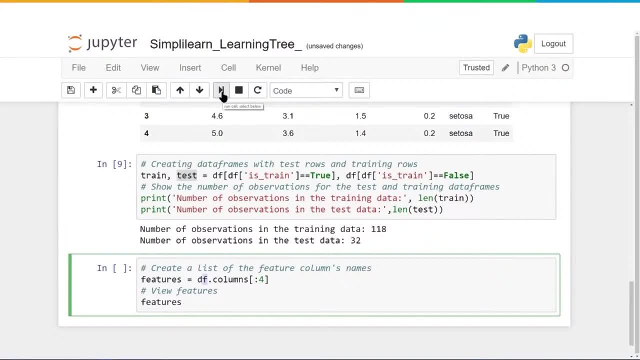 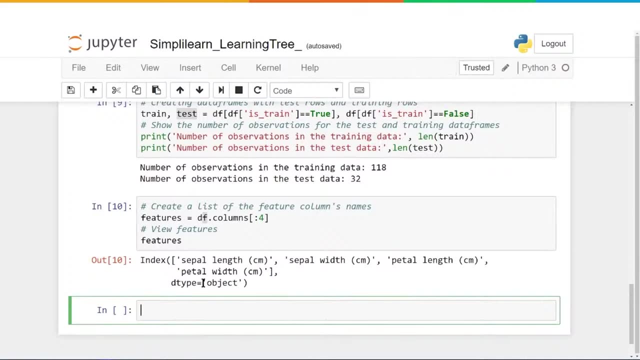 four are going to be the features or the titles of those columns, And so when I run this, you'll see down here that it creates an index: SEPA length, SEPA width, petal length and petal width. And this should be familiar because if you look up here, 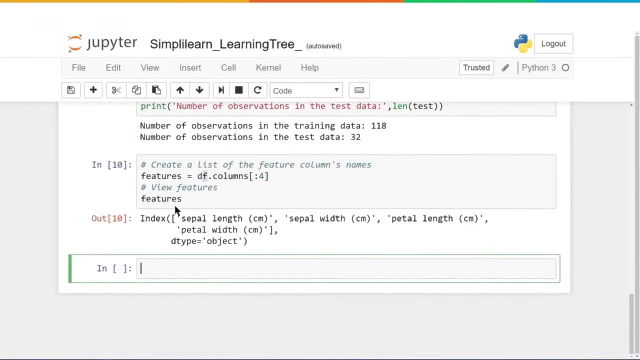 here's our column titles going across, and here's the first four. One thing I want you to notice here is that when you're in a command line- whether it's Jupyter Notebook, or you're running command line in the terminal window. 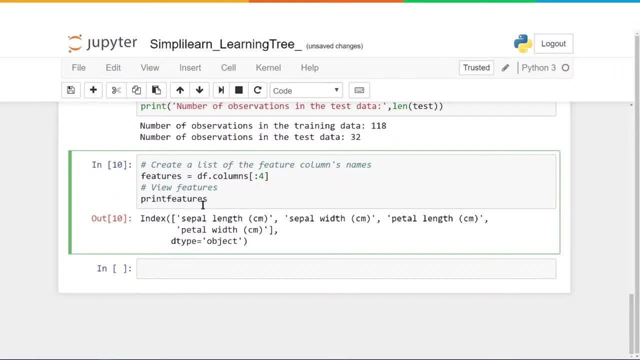 if you just put the name of it, it'll print it out. This is the same as doing print features And the shorthand is you just put features in here If you're actually writing a code and saving the script and running it. 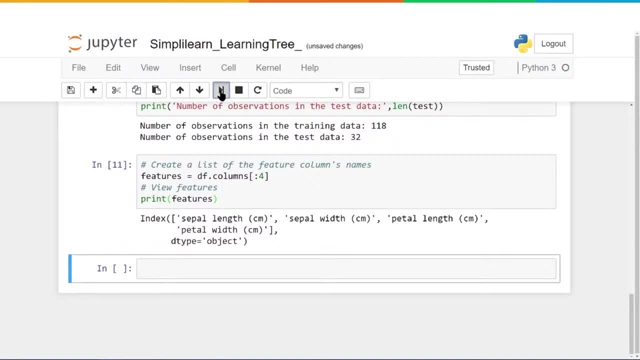 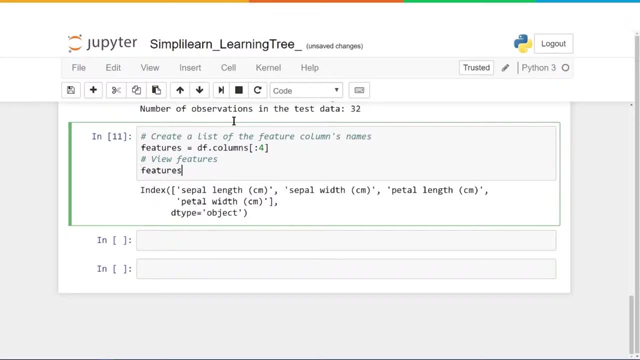 by remote, you really need to put the print in there. But for this, when I run it, you'll see it gives me the same thing. But for this we want to go ahead and we'll just leave it as features because it doesn't really matter. And this is. 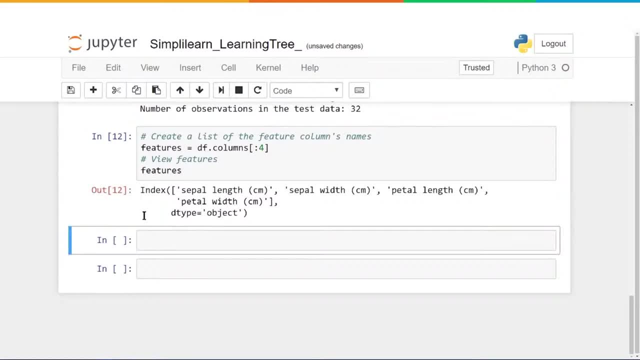 one of the fun things about Jupyter Notebooks is I'm just building the code as we go, And then we need to go ahead and create the labels for the other part. So let's take a look and see what that looks like. 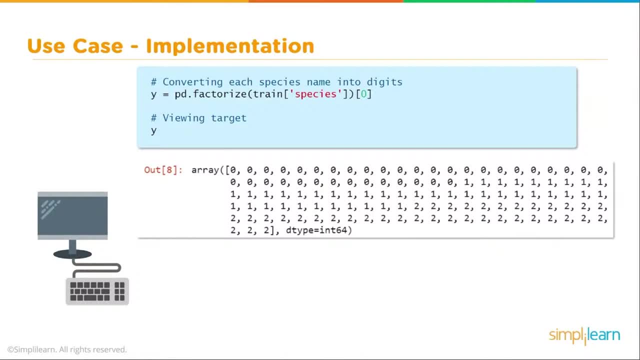 For our final step in prepping our data before we actually start running the training and the testing, is we're going to go ahead and convert the species on here into something the computer understands. So let's put this code into our script and see where that takes us. 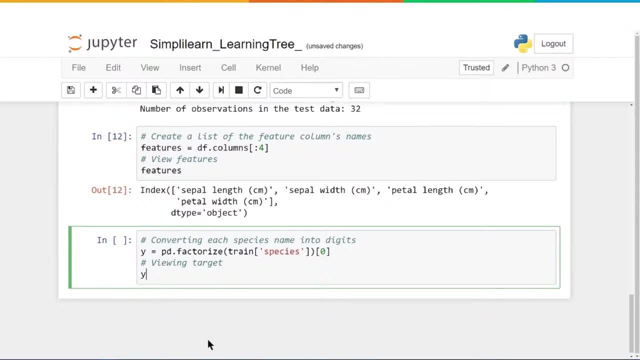 Alright, here we go. We've set y equal to pd. dot factorize- train species of zero. So let's break this down just a little bit. We have our pandas right here. pd factorize- What's factorize doing? I'm going to come back to that in just. 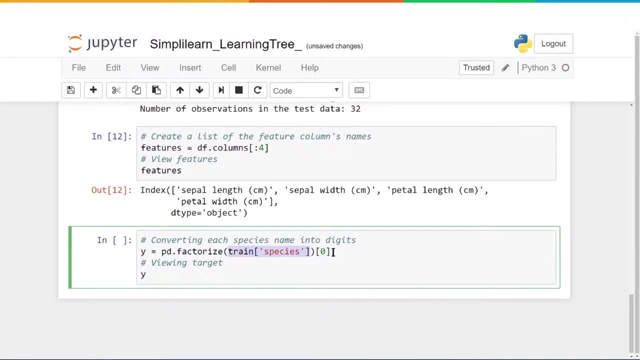 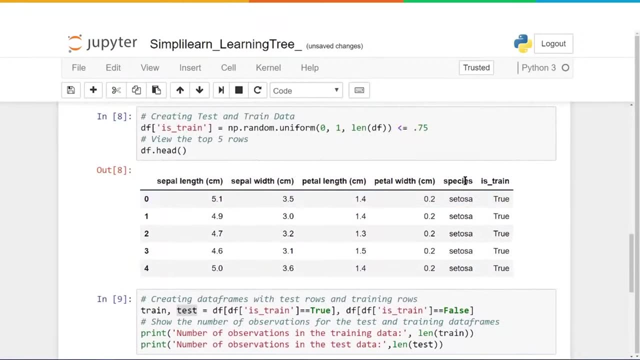 a second. Let's look at what train species is and why. we're looking at the group zero on there And let's go up here, and here is our species. Remember this: We created this whole column here for species And then it has setosa, setosa. 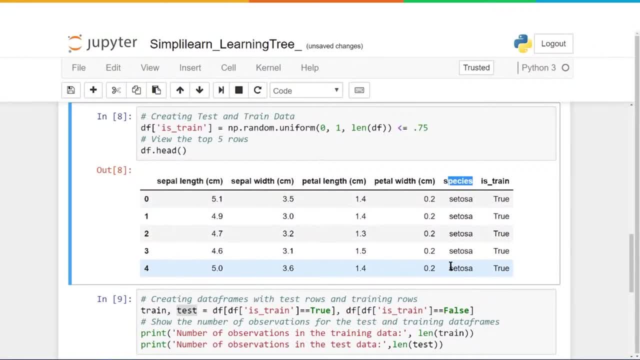 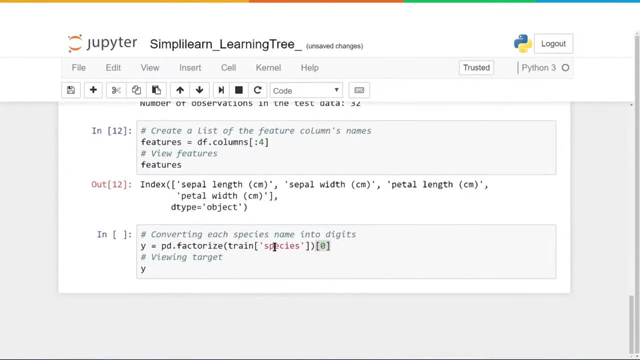 setosa, setosa, and if you scroll down enough, you'd also see virginica and vericolor. We need to convert that into something the computer understands: Zeros and ones, So the train species of zero, because this is in the format of a. 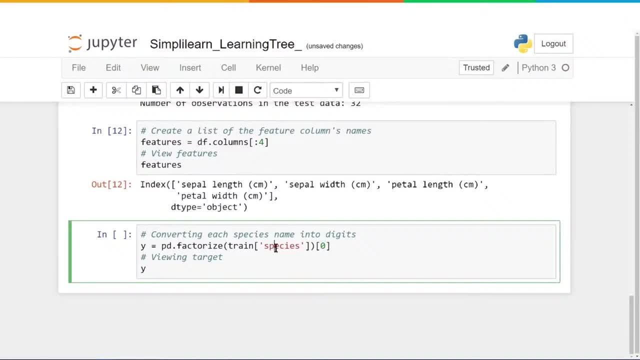 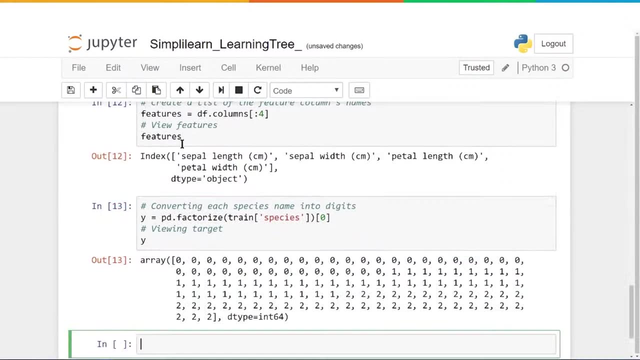 array of arrays, so you have to have the zero on the end. And then species is just that column Factorize goes in there and looks at the fact that there's only three of them. So when I run this you'll see that y generates. 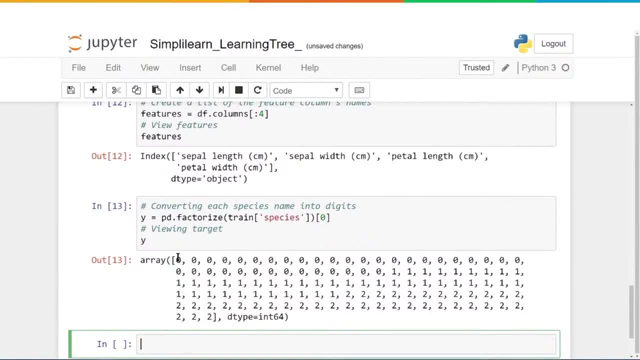 an array that's equal to- in this case it's the training set and it's zeros, ones and twos, representing the three different kinds of flowers we have. So now we have something the computer understands and we have a nice table that we can read. 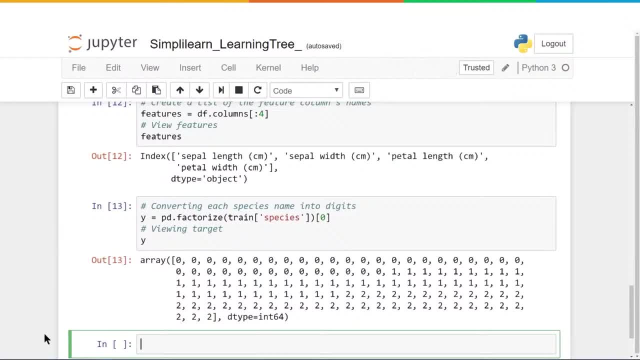 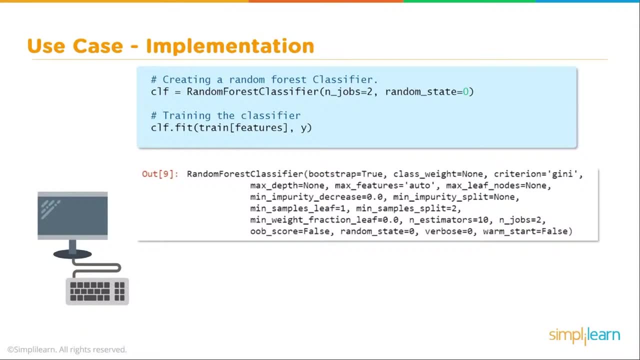 and understand, And now we get to actually start doing the predicting. So here we go. We have two lines of code. Oh my goodness, that was a lot of work to get to two lines of code, But there is a lot in these two lines of. 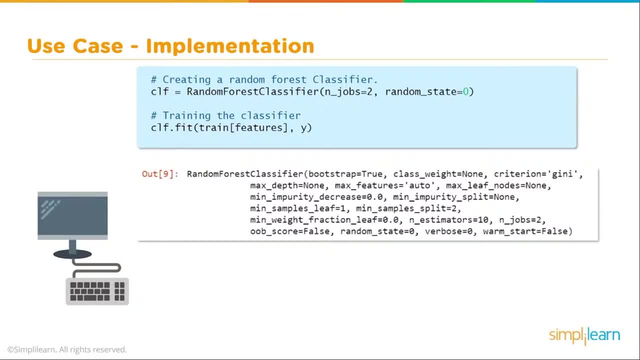 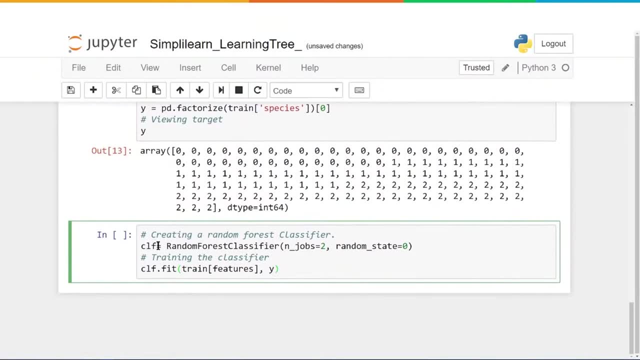 code. So let's take a look and see what's going on here. Put this into our full script that we're running. Let's paste this in here And let's take a look and see what this is We have. we're creating a. 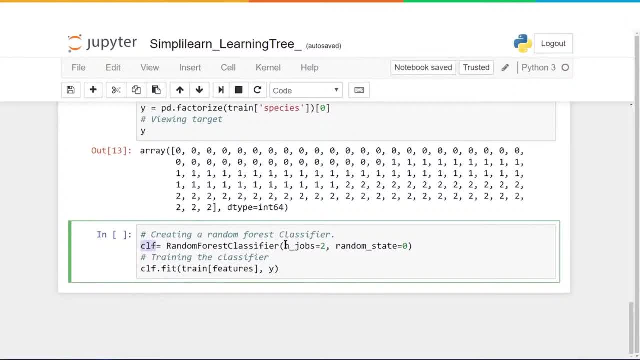 variable clf and we're going to set this equal to the random forest classifier And we're passing two variables in here And there's a lot of variables you can play with. As far as these two are concerned, they're very standard. 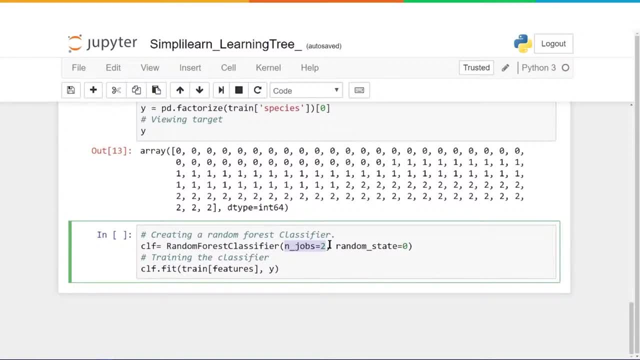 njobs. all that does is to prioritize it, Not something to really worry about. Usually, when you're doing this on your own computer, you do: njobs equals two. If you're working in a larger or big data and you need to prioritize it differently, this is. 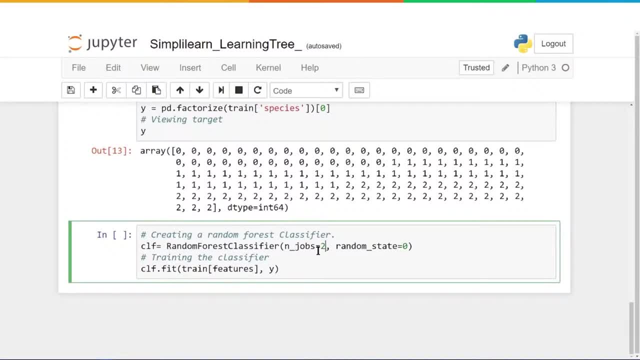 what that number does is it changes your priorities and how it's going to run across the system and things like that, And then the random state is just how it starts. Zero is fine for here, But let's go ahead and run this. 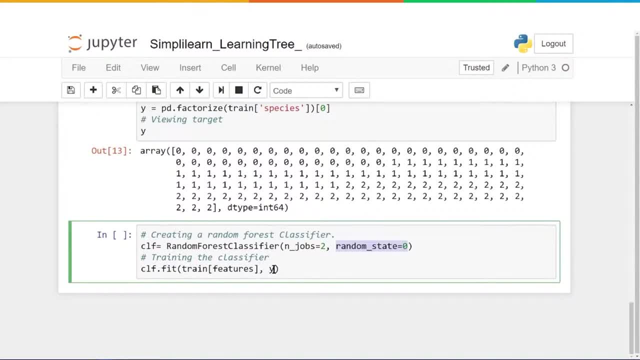 We also have clffit. train features comma y And before we run it, let's talk about this a little bit. more. clffit, So we're fitting, we're training it. We are actually creating our random forest classifier right here. This is the code. 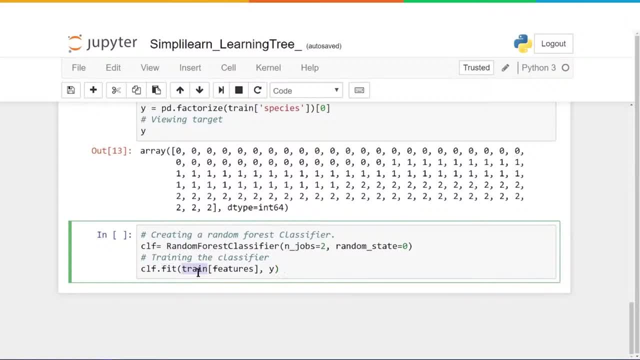 that does everything. And we're going to take our training set- remember, we kept our test off to the side- and we're going to take our training set with the features and then we're going to go ahead and put that in. And here's our target: the y. 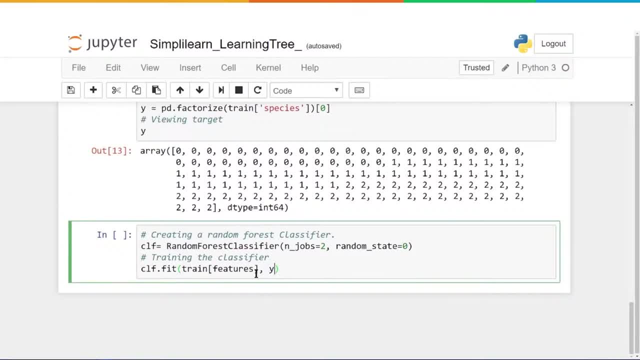 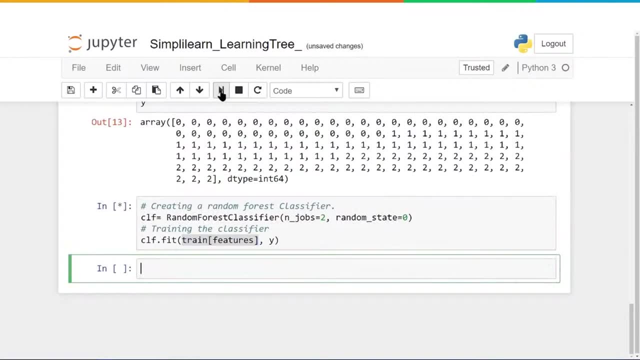 So the y is zero, one and two that we just created And the features is the actual data going in that we put into the training set And let's go ahead and run that. And this is kind of an interesting thing because it printed out the random. 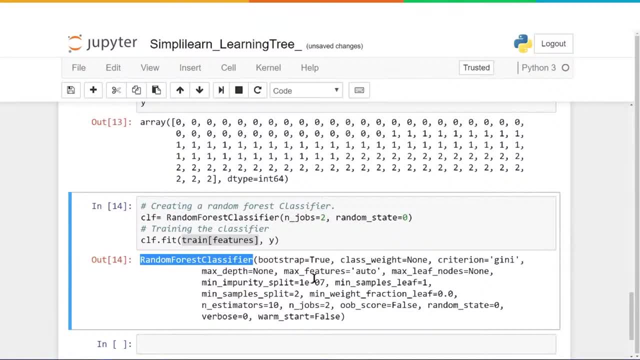 forest classifier and everything around it, And so when you're running this in your terminal window or in a script like this, this automatically treats this, just like when we were up here and I typed in y and it printed out y instead of print y. 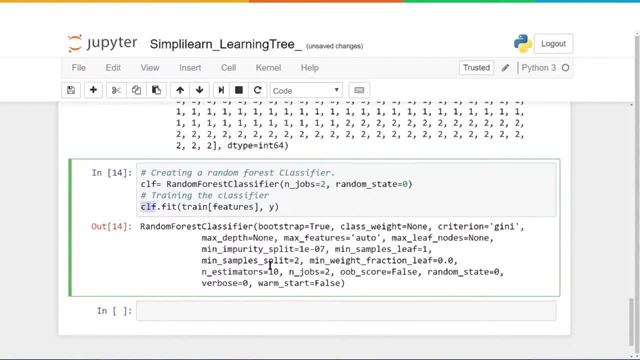 This does the same thing. It treats this as a variable and prints it out. But if you were actually running your code, that wouldn't be the case. And what it's printed out is: it shows us all the different variables we can change, And if we go down here, 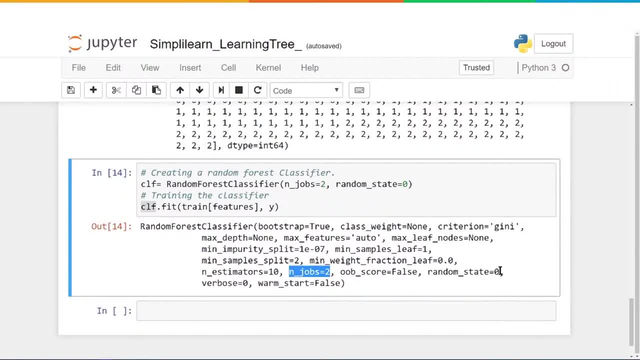 you can actually see njobs equals two. You can see the random state equals zero. Those are the two that we sent in there. You would really have to dig deep to find out all these different meanings of all these different settings on here. Some of them are self-explanatory. 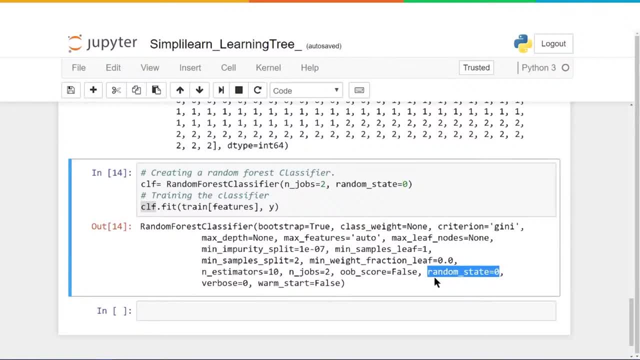 if you kind of think about it a little bit like, max features is auto, So all the features that we're putting in there is just going to automatically take all four of them. Whatever we send it, it'll take. Some of them might have so many. 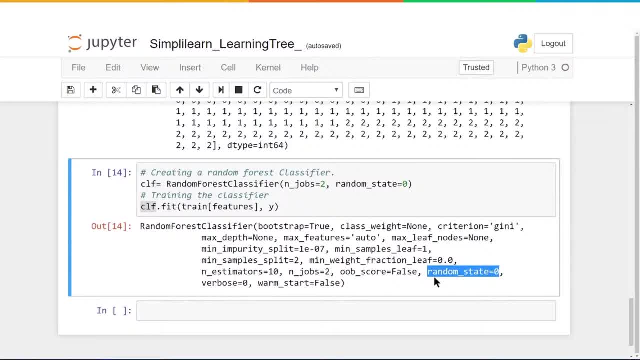 features because you're processing words. there might be like 1.4 million features in there because you're doing legal documents and that's how many different words are in there. At that point you probably want to limit the maximum features that you're going. 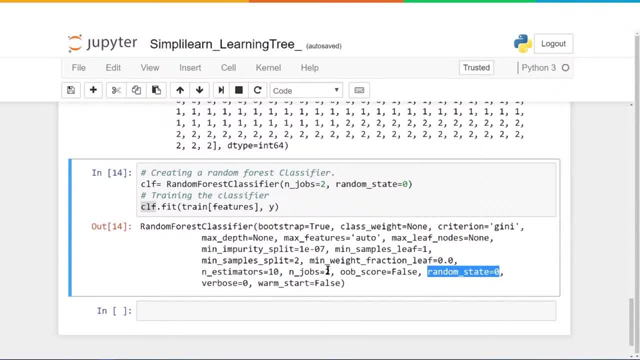 to process And leaf nodes. that's the end nodes. Remember we had the fruit and we're talking about the leaf nodes. Like I said, there's a lot in this. We're looking at a lot of stuff here, So you might have in this. 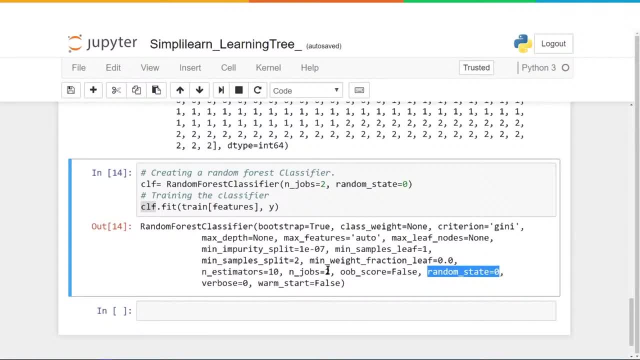 case, there's probably only, I think, three leaf nodes, maybe four. You might have thousands of leaf nodes, at which point you do need to put a cap on that and say, okay, you can only go so far, and then we're going to use all of our resources. 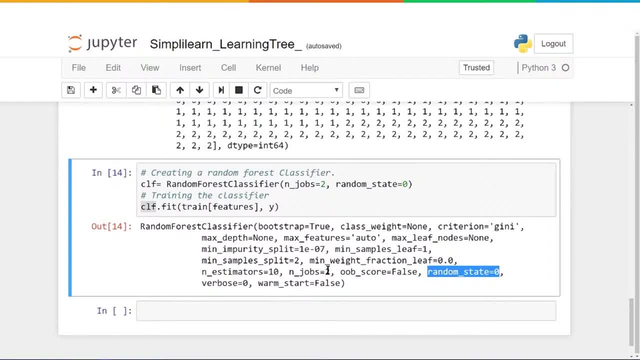 on processing this, And that really is what most of these are about is limiting the process and making sure we don't overwhelm a system. And there's some other settings in here. Again, we're not going to go over all of them. Warm start equals. 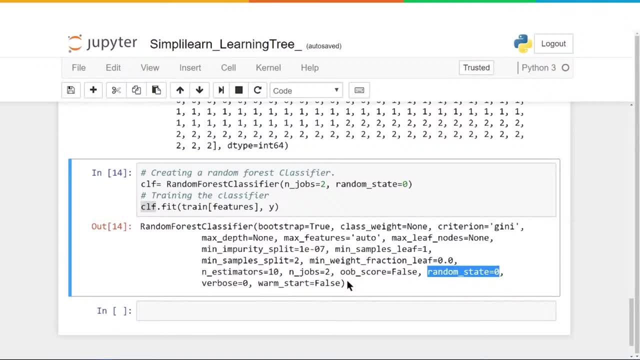 false Warm start is if you're programming it one piece at a time externally, Since we're not, we're not going to continually train this particular learning tree And again, like I said, there's a lot of things in here that you'll want to. 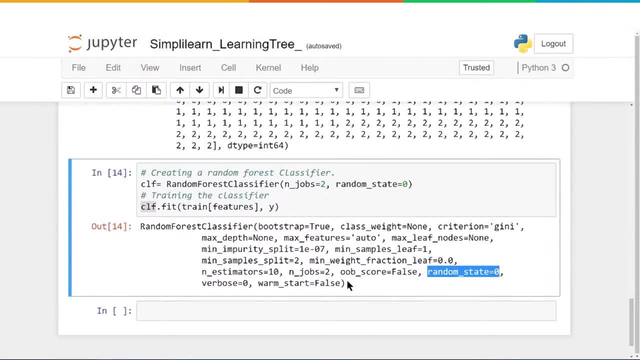 look up more detail from the sklearn and if you're digging in deep and running a major project on here. For today, though, all we need to do is fit or train our features and our target Y, So now we have our training model. what's? 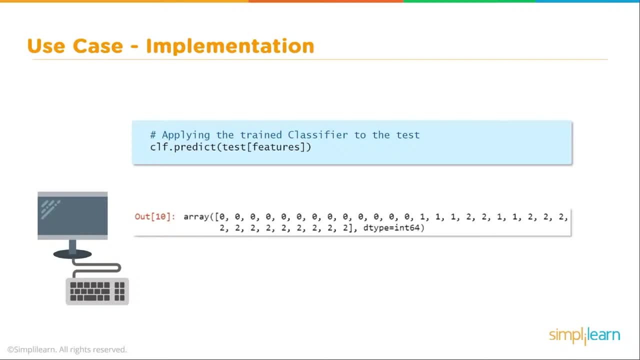 next, If we're going to create a model, we now need to test it. Remember, we set aside the test feature, test group- 25% of the data. So let's go ahead and take this code and let's put it into our 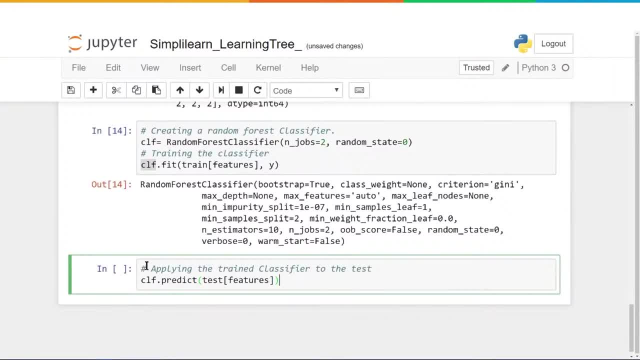 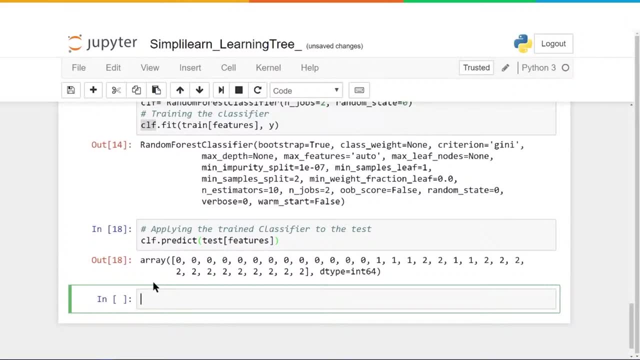 script and see what that looks like. Okay, here we go And we're going to run this and it's going to come out with a bunch of zeros, ones and twos, which represents the three type of flowers: The setosa, the. 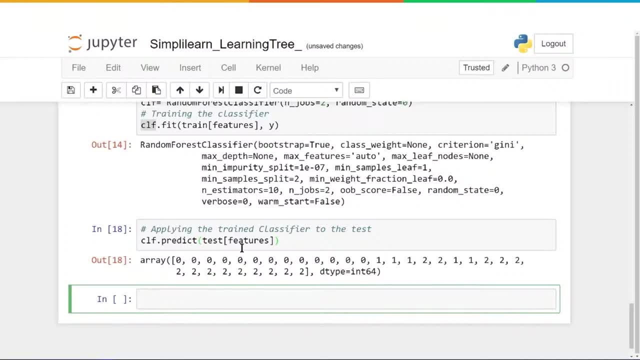 virginica and the versicolor, And what we're putting into our predict is the test features, and I always kind of like to know what it is I am looking at. So, real quick, we're going to do test features And remember features is an. 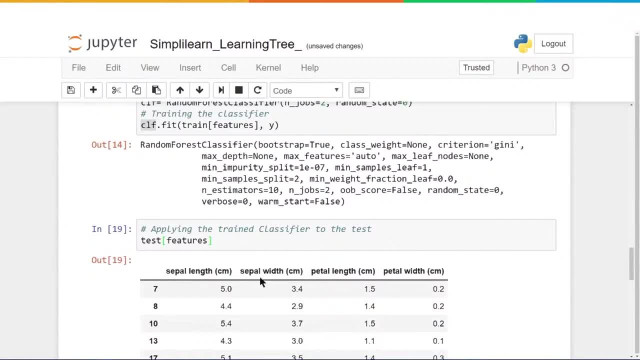 array of sepal length, sepal width, petal length, petal width. So when we put it in this way, it actually loads all these different columns that we loaded into features. So if we did just features, let me just do features in here so we can see what features looks. 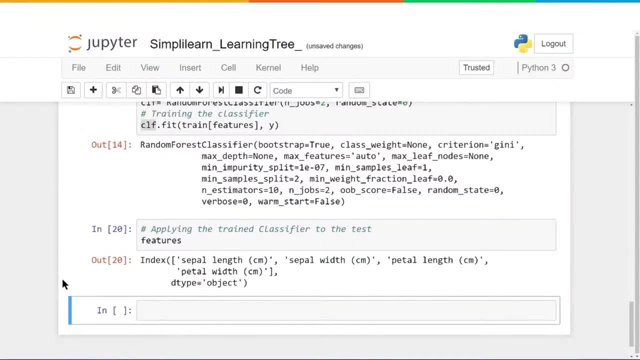 like This is just playing with Panda's data frames, You'll see that it's an index. So when you put an index in like this into test features, into test, it then takes those columns and creates a Panda data frames from those columns And in this, 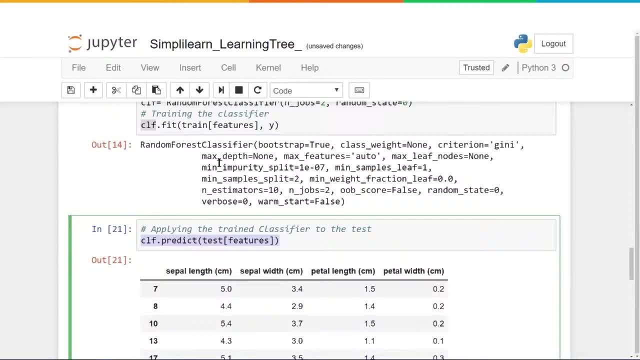 case, we're going to go ahead and put those into our predict. So we're going to put each one of these lines of data- the 5.0,, 3.4,, 1.5,, .2, and we're going to put those. 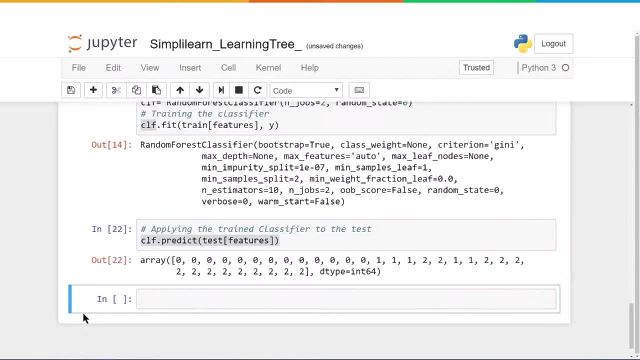 in and we're going to predict what our new forest classifier is going to come up with, And this is what it predicts. It predicts 0, 0, 0, 1, 2, 1, 1, 2,, 2,, 2, and. 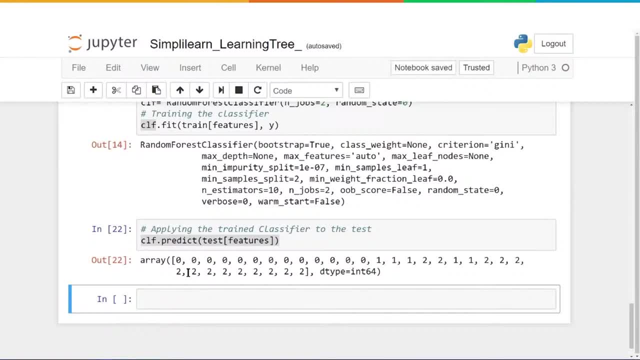 again, this is the flower type: setosa, virginica and versicolor. So now that we've taken our test features, let's explore that. Let's see exactly what that data means to us. So the first thing we can do with our predicts is: 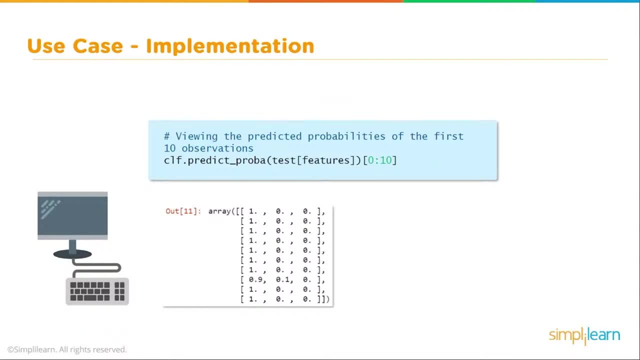 we can actually generate a different prediction model. When we say different, we're going to view it differently. It's not that the data itself is different. So let's take this next piece of code and put it into our script. So we're pasting it in here. 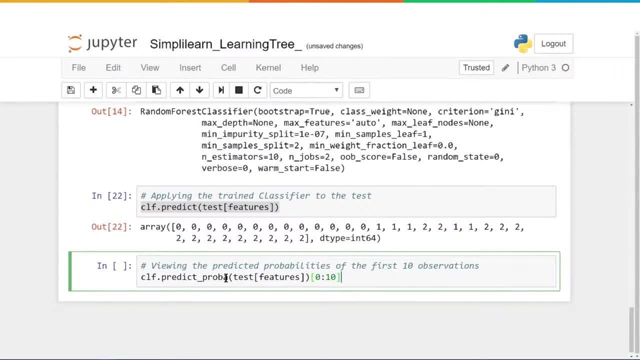 and you'll see that we're doing predict and we've added underscore proba for probability. So there's our clfpredict probability. So we're running it just like we ran it up here, but this time, with this, we're going to get a slightly different result. 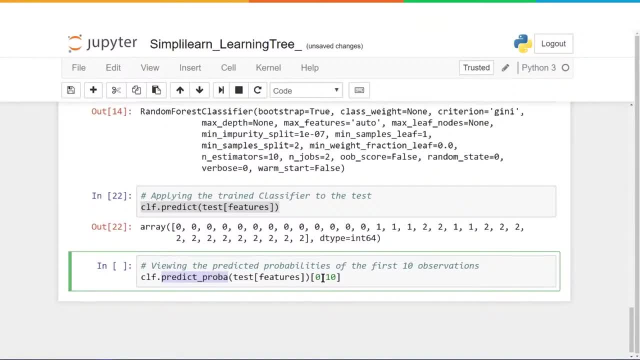 And we're only going to look at the first 10.. So you'll see down here, instead of looking at all of them, which was what? 27,? you'll see right down here that this generates a much larger field on the probability. 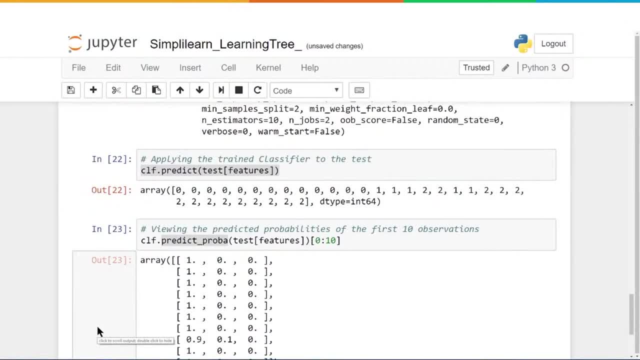 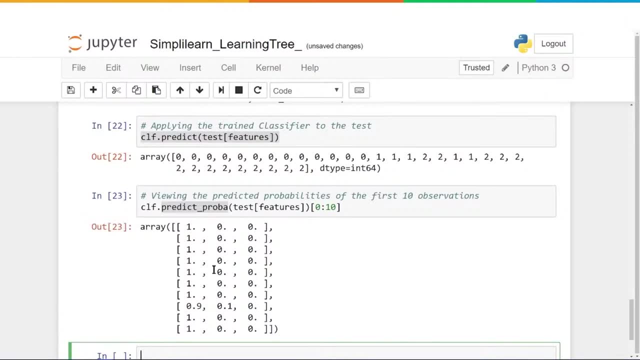 And let's take a look and see what that looks like and what that means. So when we do the predict underscore, proba for probability, it generates three numbers. So we had three leaf nodes at the end And if you remember, from all the theory we 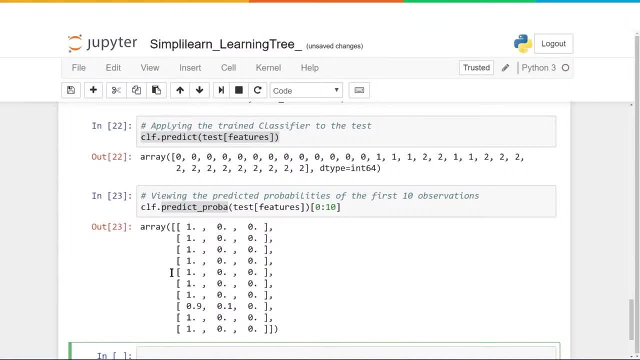 did. this is the predictors. The first one is predicting a 1 for setosa, it predicts a 0 for virginica, and it predicts a 0 for versicolor, and so on, and so on, and so on, And let's. 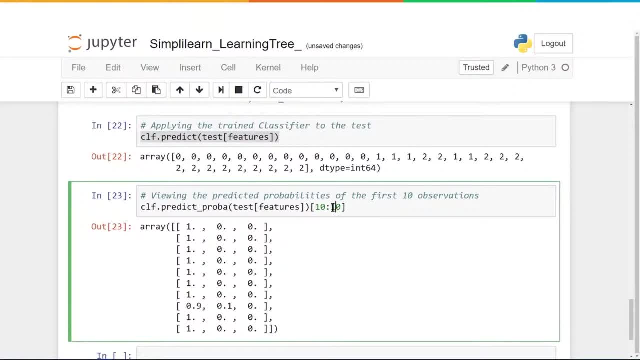 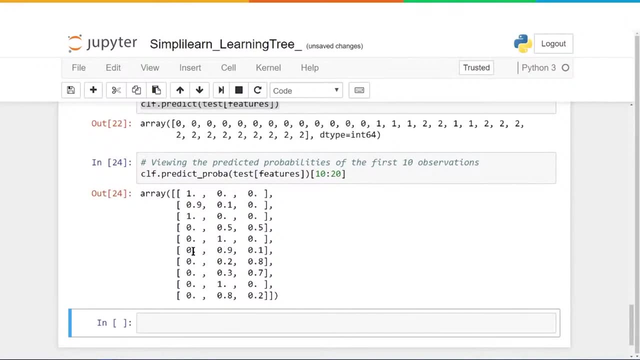 you know what? I'm going to change this just a little bit. Let's look at 10 to 20, just because we can And we start to get in a little different of data, and you'll see right down here, it gets to this one, this line, right. 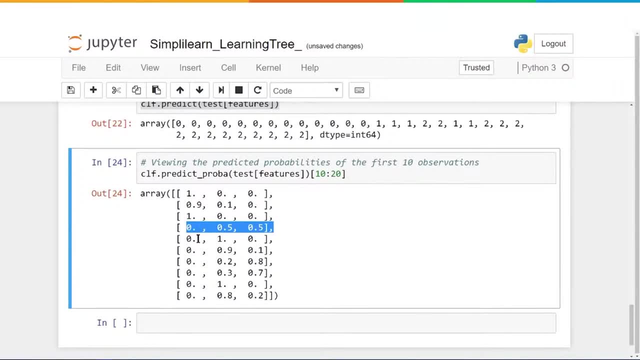 here And this line has 0,, 0.5,, 0.5. And so if we're going to vote and we have two equal votes, it's going to go with the first one. So it says setosa gets 0. 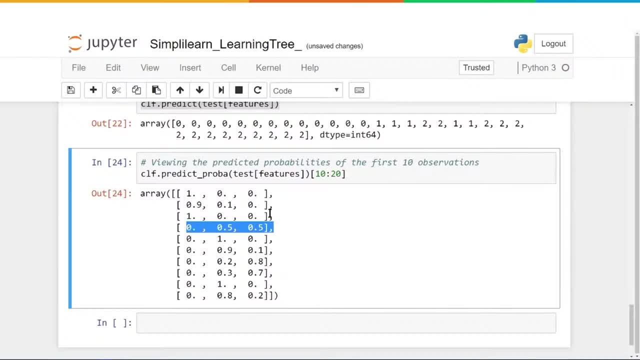 votes. virginica gets 0.5 votes, versicolor gets 0.5 votes, but let's just go with the virginica, since these two are equal, and so on and so on. down the list, You can see how they vary on here. 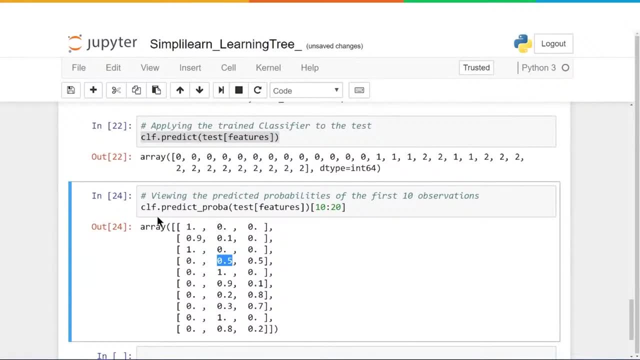 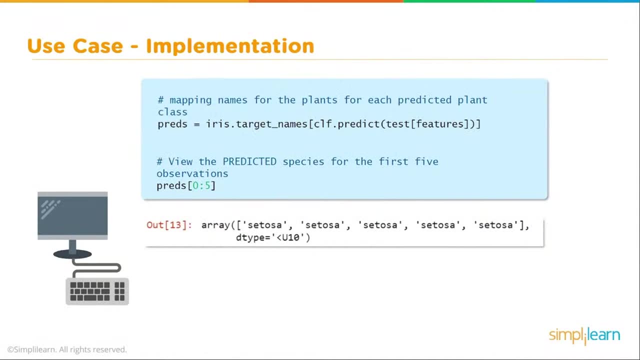 So now we've looked at both how to do a basic predict of the features and we've looked at the predict probability. Let's see what's next on here. So now we want to go ahead and start mapping names for the plants. We want to attach names. so 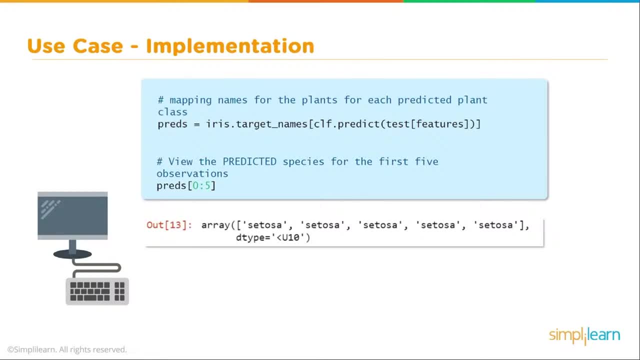 that it makes a little more sense for us, And that's what we're going to do in these next two steps. We're going to start by setting up our predictions and mapping them to the names, So let's see what that looks like. 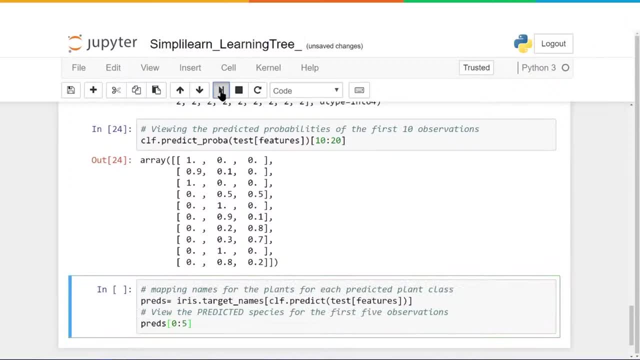 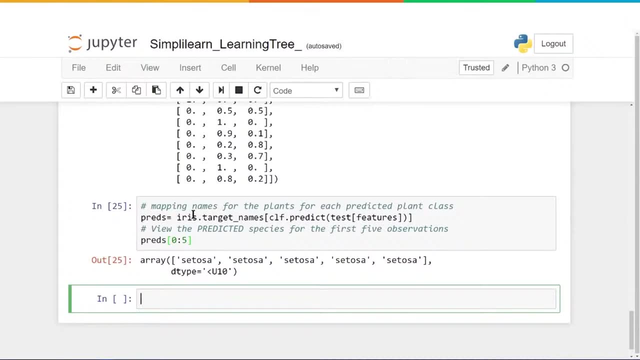 And let's go ahead and paste that code in here and run it, And this goes along with the next piece of code. So we'll skip through this quickly and then come back to it a little bit. So here's iris dot target names. 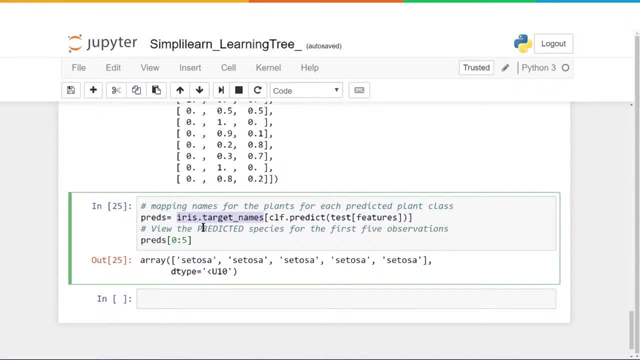 And, if you remember correctly, this was the names that we've been talking about this whole time: The setosa virginica versicolor. And then we're going to go ahead and do the prediction again. We could have just set a variable equal to this instead of re-running. 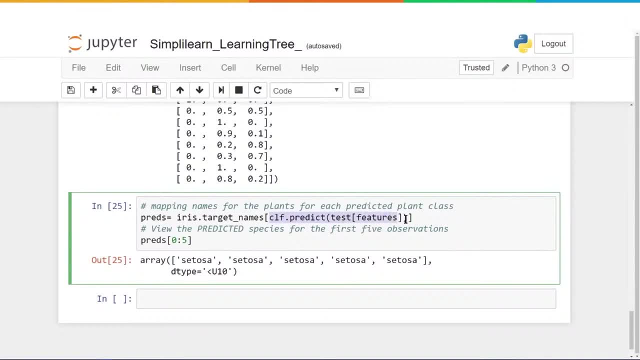 it each time, But we're going to go ahead and run it again. clf dot- predict test features. Remember that returns the zeros, the ones and the twos, And then we're going to set that equal to predictions. So this time we're actually putting it in a 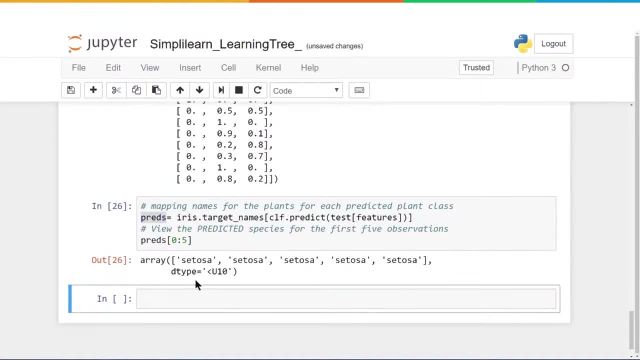 variable And when I run this it distributes and it comes out as an array And the array is: setosa, setosa, setosa, setosa, setosa. We're only looking at the first five We could actually do. let's do the first. 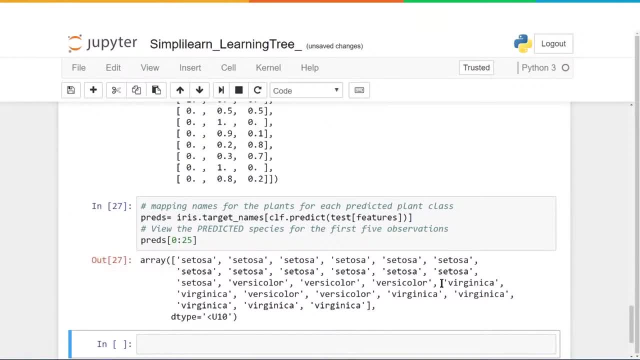 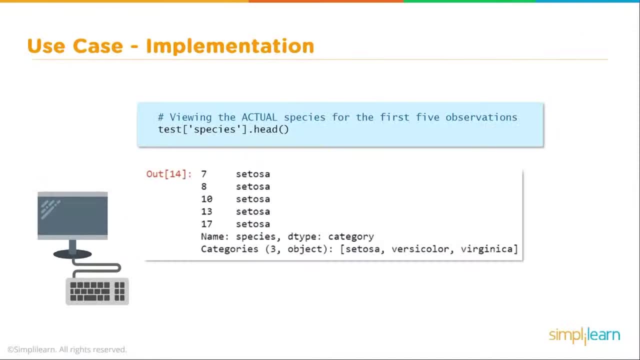 25, just so we can see a little bit more on there. And you'll see that it starts mapping it to all the different flower types- The versicolor and the virginica in there- And let's see how this goes with the next one. So let's take a look at. 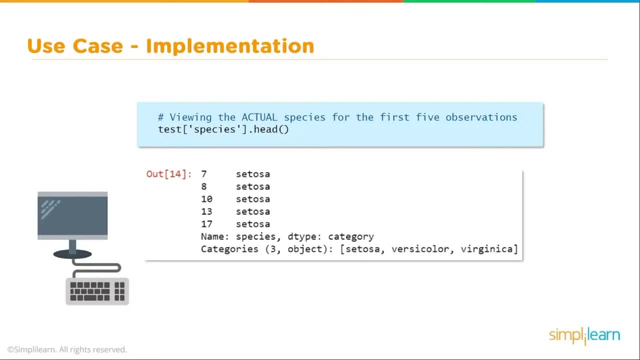 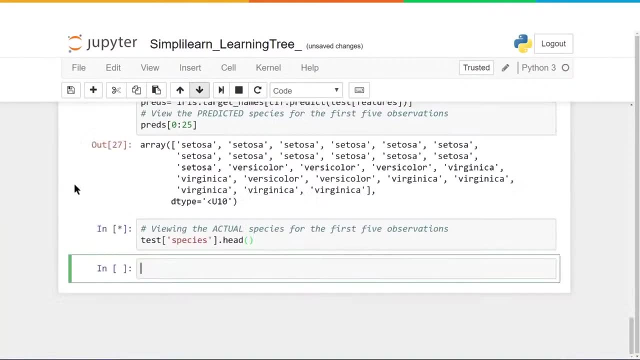 the top part of our species in here, And we'll take this code and put it in our script And let's put that down here and paste it. There we go And we'll go ahead and run it And let's talk about both these sections of code here. 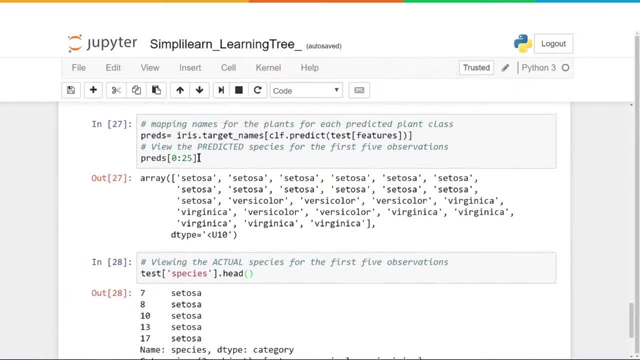 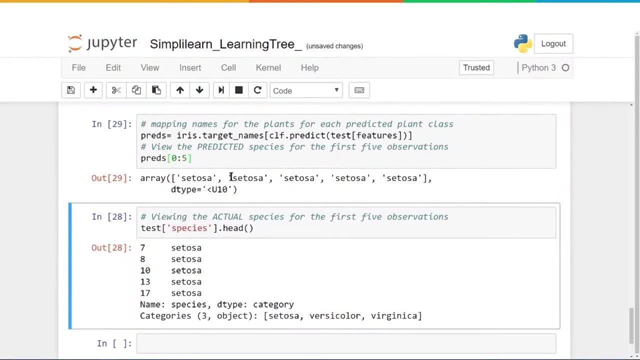 And how they go together. The first one is our predictions, And I went ahead and did predictions through 25.. Let's just do 5. And so we have setosa, setosa, setosa, setosa. That's what we're predicting from. 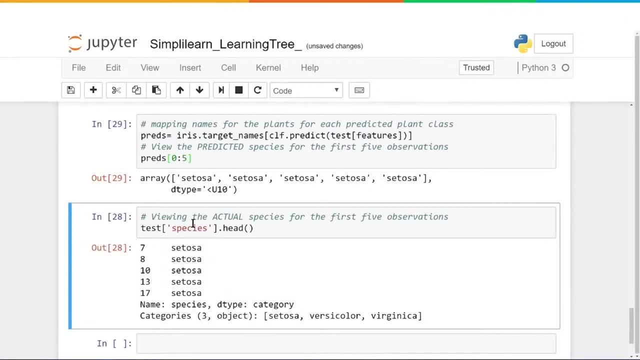 our test model. And then we come down here and we look at test species And remember I could have just done testspecieshead And you'll see, it says setosa, setosa, setosa, setosa And they match. So the first 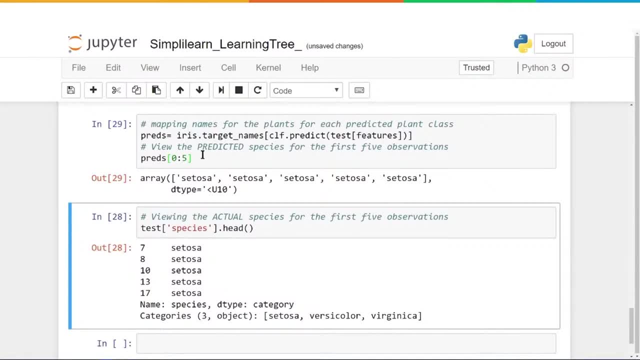 one is what our forest is doing, And the second one is what the actual data is. Now we need to combine these so that we can understand what that means. We need to know how good our forest is, How good it is at predicting the features, So that's where we come up to the 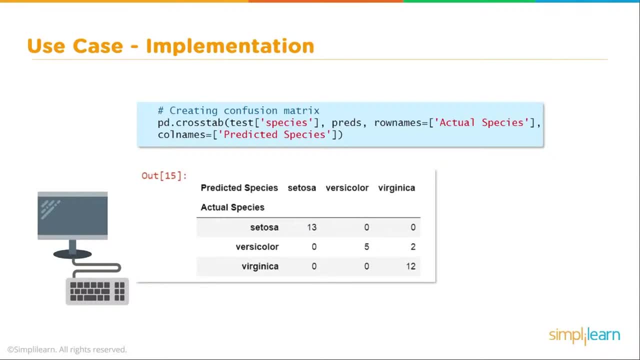 next step, Which is lots of fun- We're going to use a single line of code to combine our predictions and our actuals, So we have a nice chart to look at, And let's go ahead and put that in our script, in our 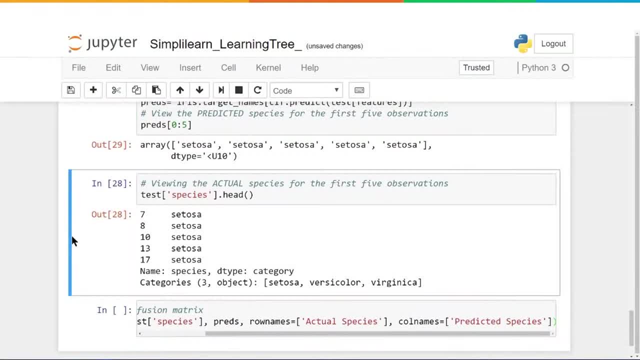 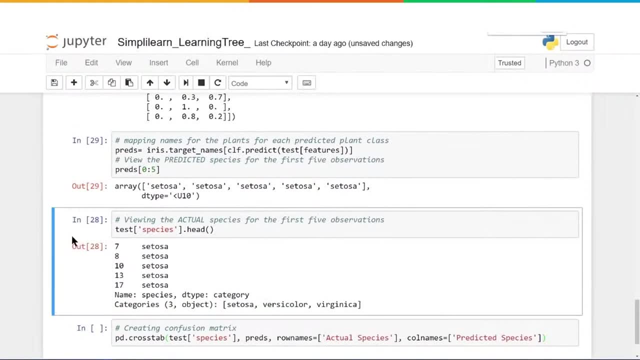 Jupyter notebook here. Let's go ahead and paste that in, Because I'm on the Jupyter notebook. I can do a control minus. You can see the whole line there. There we go, Resize it And let's take a look and see what's. 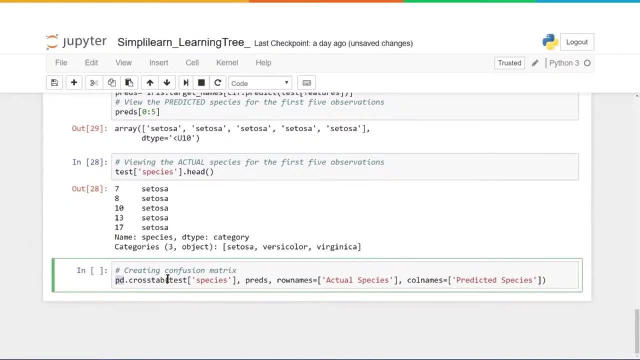 going on here. We're going to create in pandas- Remember, PD stands for pandas And we're doing a crosstab. This function takes two sets of data and creates a chart out of them, So when I run it, you'll get a nice. 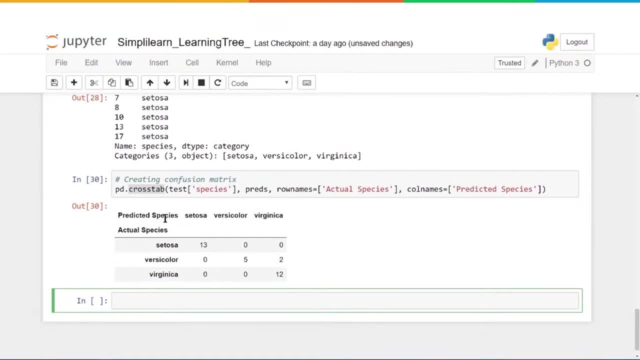 chart down here And we have the predicted species. so across the top you'll see the Cetosa versicolor virginica and the actual species, Cetosa versicolor virginica. And so the way to read this chart and let's go ahead and take a look on how to. 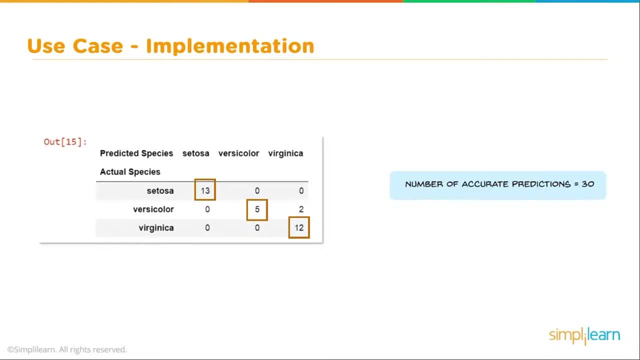 read this chart here. When you read this chart, you have Cetosa where they meet, You have versicolor where they meet, And you have virginica where they meet, And they're meeting where the actual and the predicted agree. So this is the number of accurate. 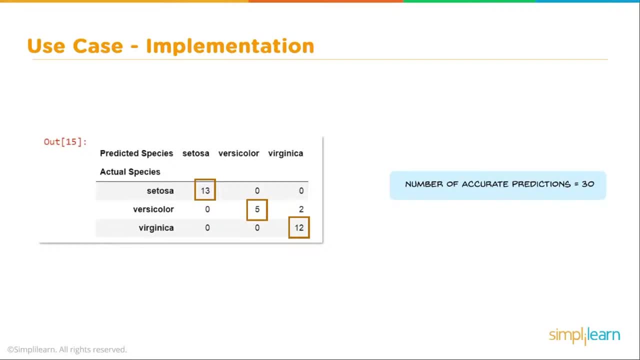 predictions. So in this case it equals 30. If you had 30 plus 5 plus 12, you get 30. And then we notice here where it says virginica, but it was supposed to be versicolor. This is inaccurate. So 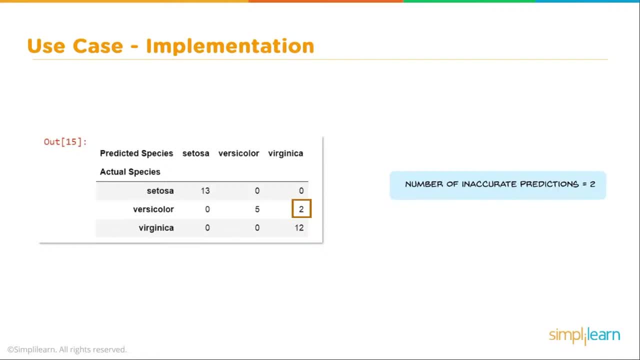 now we have two: Two inaccurate predictions and 30 accurate predictions. So we'll say that the model accuracy is 93. That's just 30 divided by 32. And if we multiply it by 100, we can say that it is 93% accurate. So we have a. 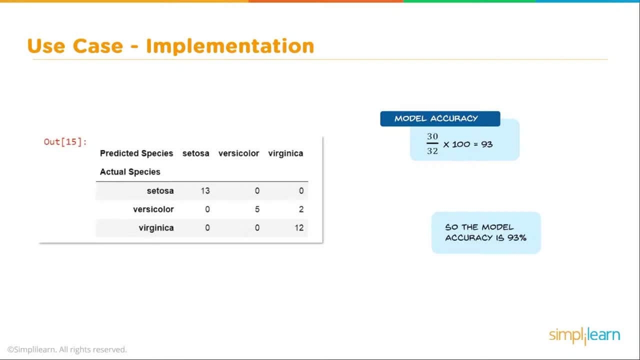 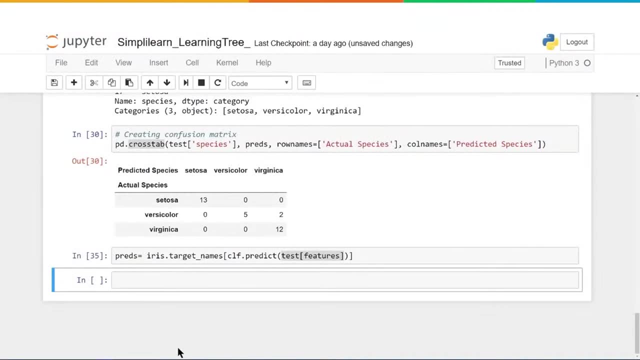 93% accuracy with our model. I did want to add one more quick thing in here on our scripting before we wrap it up, So let's flip back on over to my script In here. we're going to take this line of code from up above: 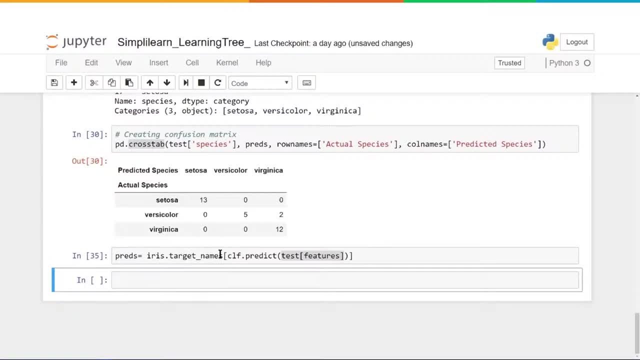 I don't know if you remember it, but predicts equals the iris dot target underscore names. So we're going to map it to the names And we're going to run the prediction And we read it on test features. But you know, we're not just testing it, We want to actually deploy it. 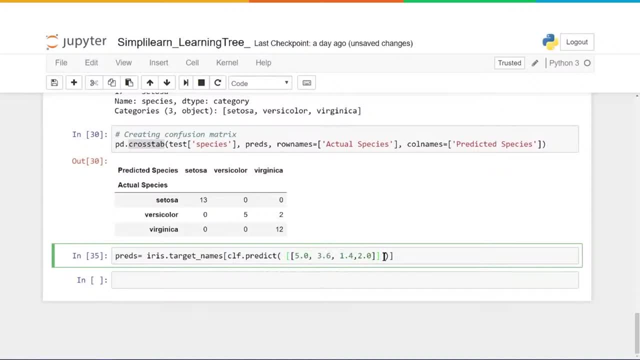 So at this point I would go ahead and change this, And this is an array of arrays. It's really important when you're running these to know that. So you need the double brackets And I could actually create data. maybe let's just do two flowers. 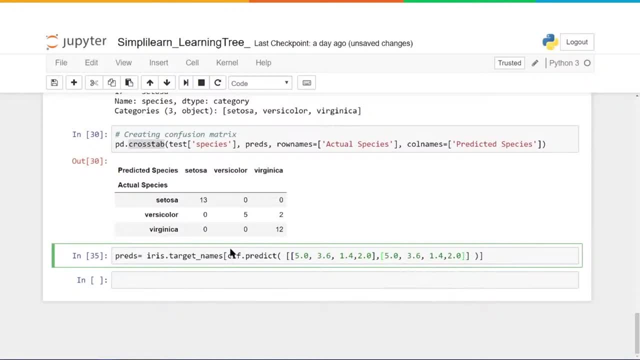 So maybe I'm processing more data coming in And we'll put two flowers in here, And then I actually want to see what the answer is. So let's go ahead and type in preds and print that out, And when I run this you'll see that I've now predicted two flowers. 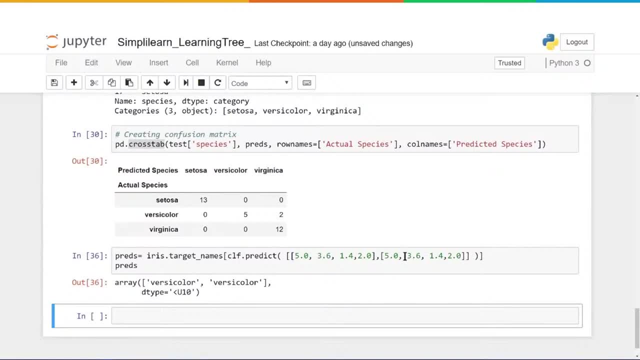 that maybe I measured in my front yard as versicolor and versicolor. Not surprising, since I put the same data in for each one. This would be the actual end product going out to be used on data that you don't know the answer for. 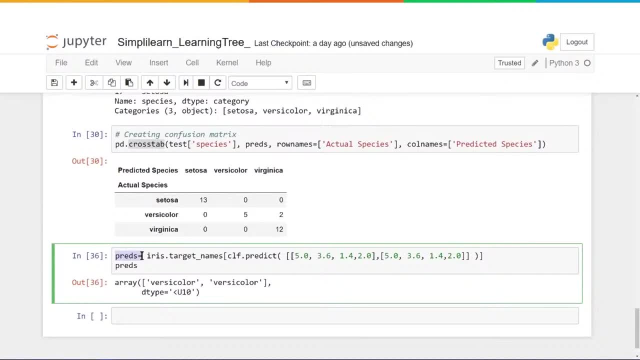 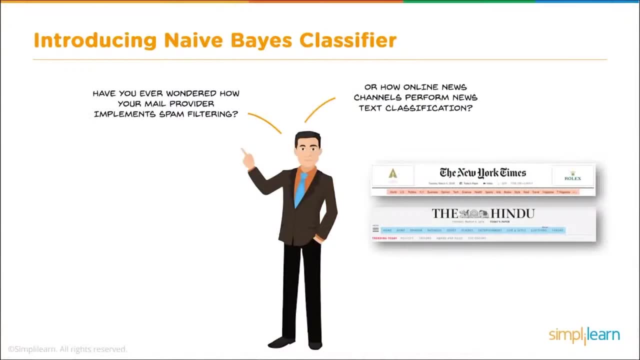 So that's going to conclude our scripting part of this Introducing Naive Bayes Classifier. Have you ever wondered how your mail provider implements spam filtering, Or how online news channels perform news text classification, Or how companies perform sentimental analysis of their audience? 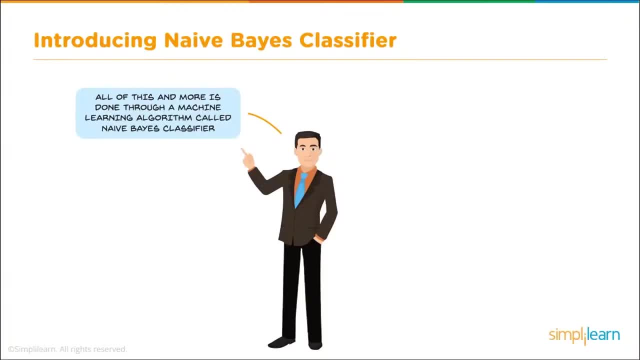 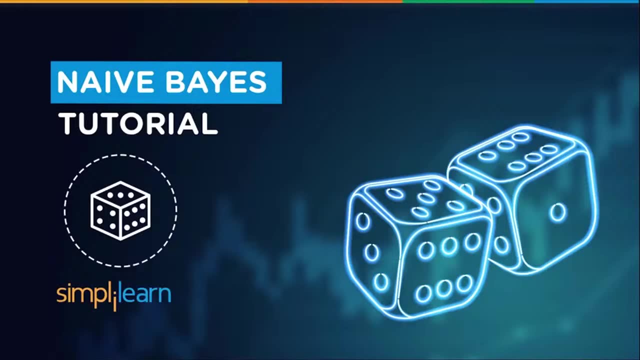 on social media. All of this and more is done through a machine learning algorithm called Naive Bayes Classifier. Welcome to Naive Bayes Tutorial. My name is Richard Kirschner. I'm with the Simply Learn team. That's wwwsimplylearncom. 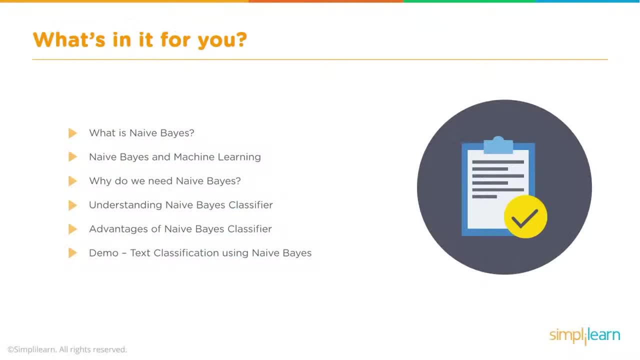 Get certified, Get ahead. What's in it for you? We'll start with what is Naive Bayes: A basic overview of how it works. We'll get into Naive Bayes and machine learning Where it fits in with our other machine learning tools. 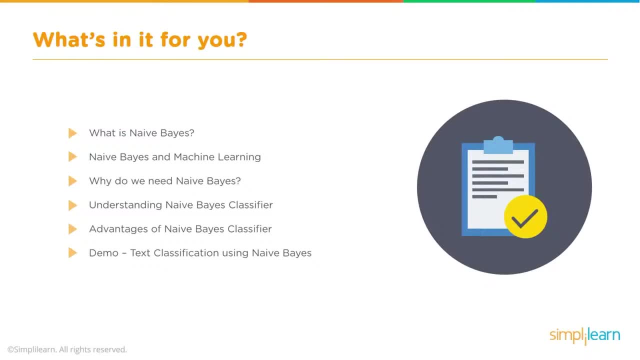 Why do we need Naive Bayes And understanding Naive Bayes Classifier a much more in-depth of how the math works in the background. Finally, we'll get into the advantages of the Naive Bayes Classifier in the machine learning setup, And then we'll roll up our sleeves. 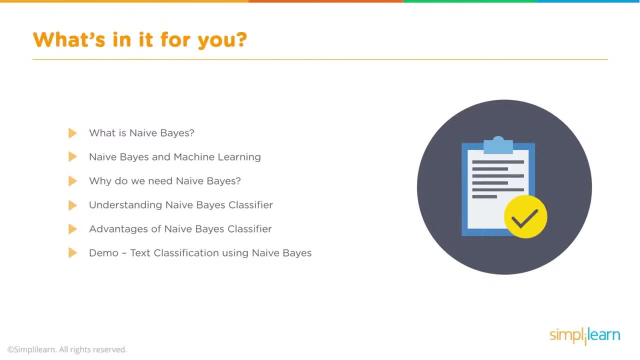 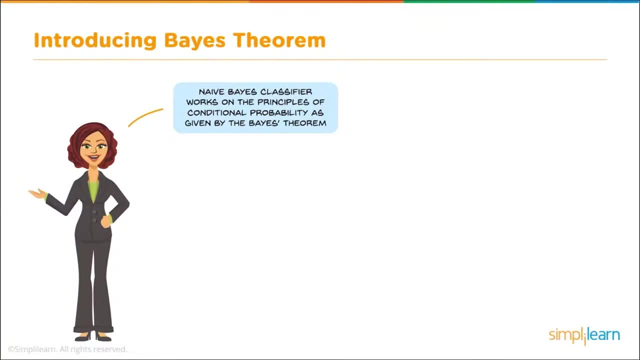 and do my favorite part. We'll actually do some Python coding and do some text classification using the Naive Bayes. What is Naive Bayes? Let's start with a basic introduction to the Bayes Theorem, Named after Thomas Bayes from the 1700's. 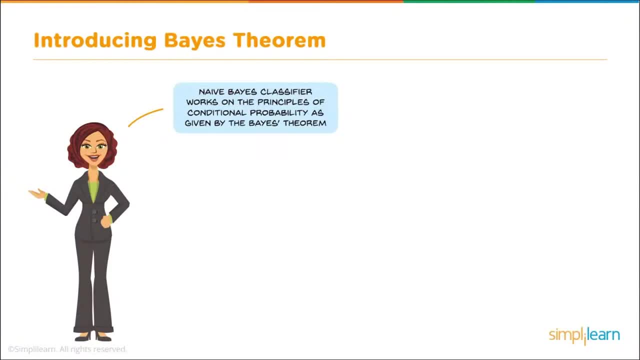 who first coined this in the western literature, Naive Bayes Classifier works on the principle of conditional probability as given by the Bayes Theorem. Before we move ahead, let us go through some of the simple concepts and the probability that we will be using. Let us consider the 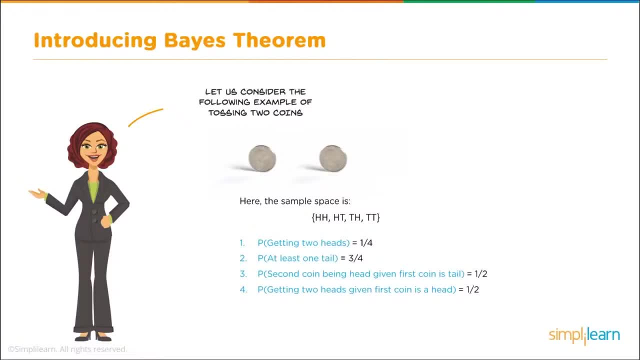 following example of tossing two coins: Here we have two quarters and if we look at all the different possibilities of what they can come up as we get that, they can come up as head heads, come up as head, tell, tell, head and tell, tell. 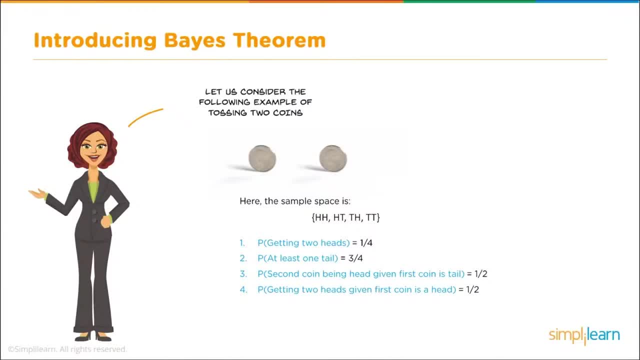 When doing the math on probability, we usually denote probability as a P, a capital P. So the probability of getting two heads equals one fourth. You can see on our data set: we have two heads and this occurs once out of the four possibilities. And then the probability of at least one tell. 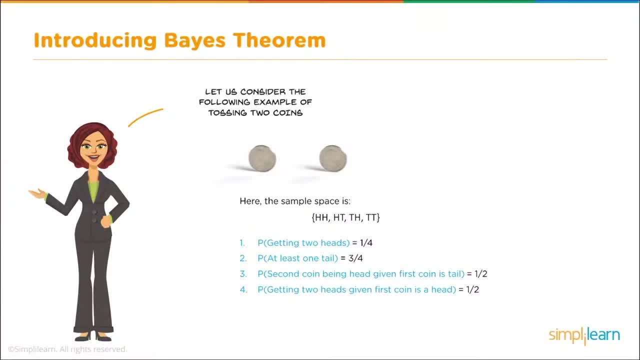 occurs three quarters of the time. You'll see on three of the coin tosses we have tells in them And out of four that's three fourths. And then the probability of the second coin being head, given the first coin is tell is one half And the probability of getting 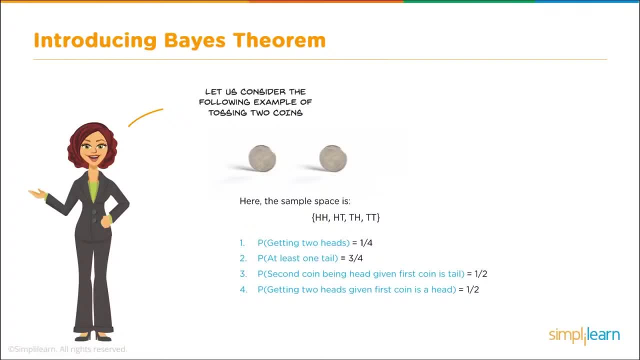 two heads. given the first coin is a head is one half. We'll demonstrate that in just a minute and show you how that math works. Now, when we're doing it with two coins, it's easy to see, But when you have something more complex, you can see where these 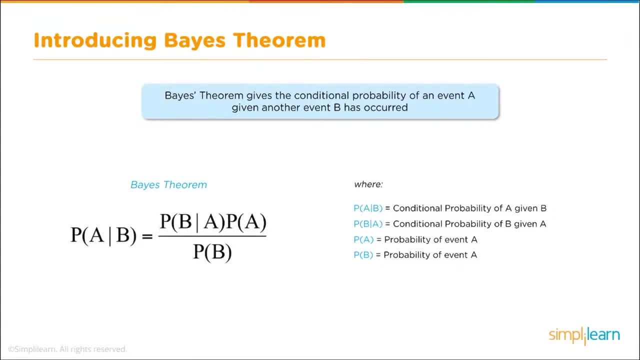 formulas really come in and work. So the Bayes Theorem gives us the conditional probability of an event A given another event B has occurred. In this case, the first coin toss will be B and the second coin toss A. This could be confusing, because we've actually 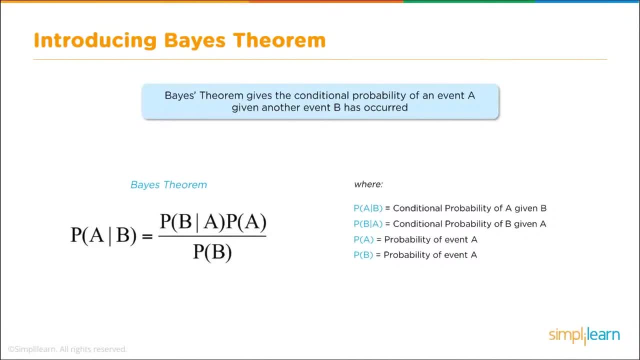 reversed the order of them and go from B to A instead of A to B. You'll see this a lot when you work in probabilities. The reason is we're looking for event A. We want to know what that is, So we're going to label that A, since that's our 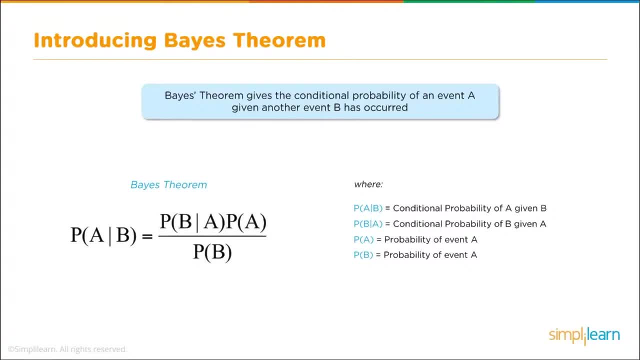 focus And then, given another event, B has occurred. In the Bayes Theorem, as you can see on the left, the probability of A occurring, given B has occurred, equals the probability of B occurring, given A has occurred, times the probability of A over the probability of B. 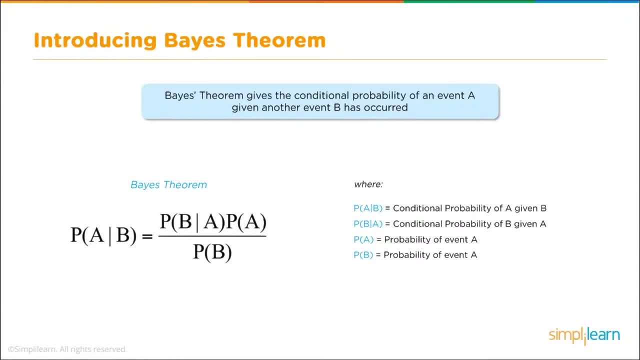 This simple formula can be moved around just like any algebra formula And we could do. the probability of A after a given B times probability of B equals the probability of B given A times probability of A. You can easily move that around and apply it and divide it out. 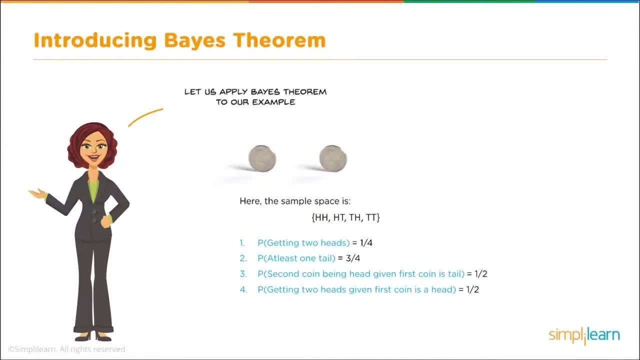 Let us apply Bayes Theorem to our example. Here we have our two quarters and we'll notice that the first two probabilities of getting two heads and at least one tail we compute directly off the data. So you can easily see that we have one example. 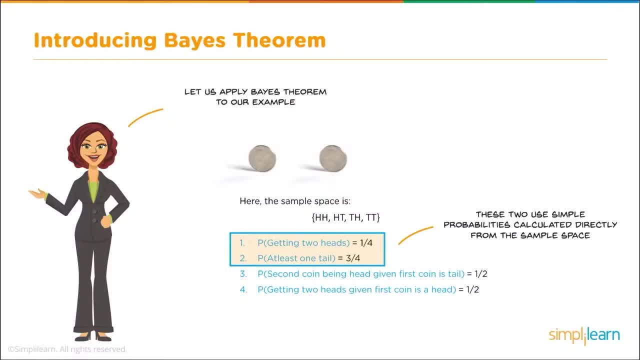 HH out of four, one fourth, and we have three with tails in them, giving us three quarters or three fourths, 75%. The second condition, the second set, three and four. we're going to explore a little bit more in detail. Let's stick to a simple example with two coins. 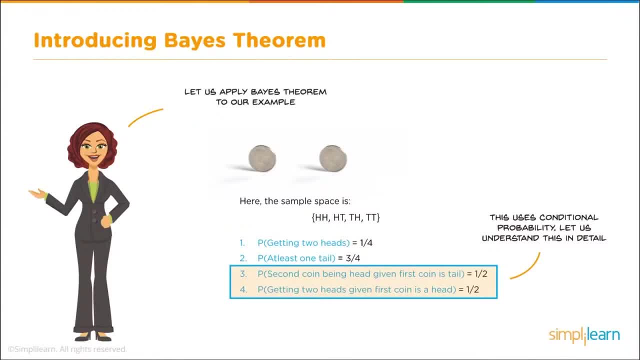 because you can easily understand the math. The probability of throwing a tail doesn't matter what comes before it, and the same with the head. So it's still going to be 50% or one half. But when that probability gets more complicated, let's say you have a D6 dice or some- 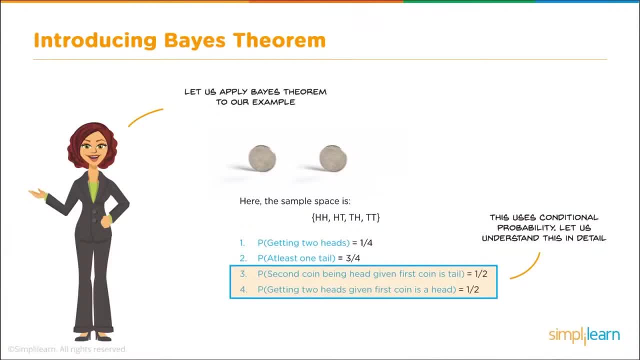 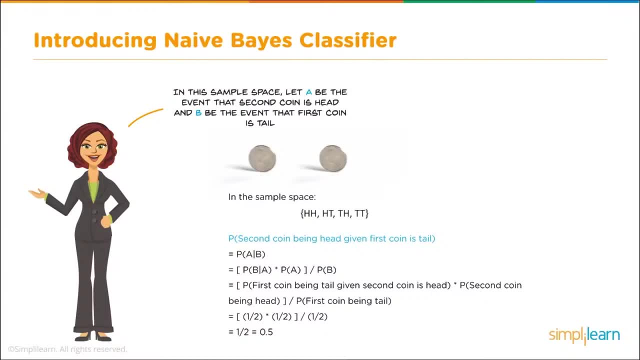 other instance, then this formula really comes in handy. But let's stick to the simple example for now. In this sample space, let A be the event that the second coin is head and B be the event that the first coin is tails. Again, we reversed it because we want to know what the second 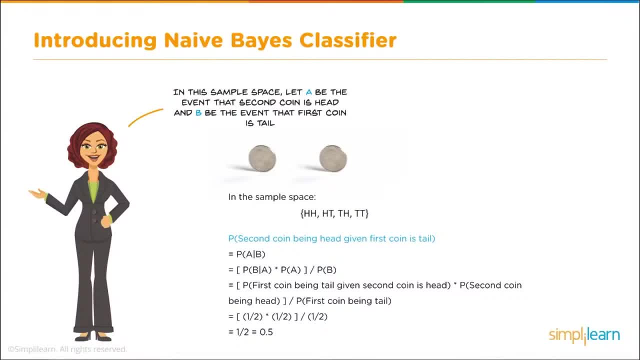 coin is going to be. So we're going to be focusing on A And we write that out as the probability of A given B, And we know this from our formula: that that equals the probability of B given A times the probability of A over. 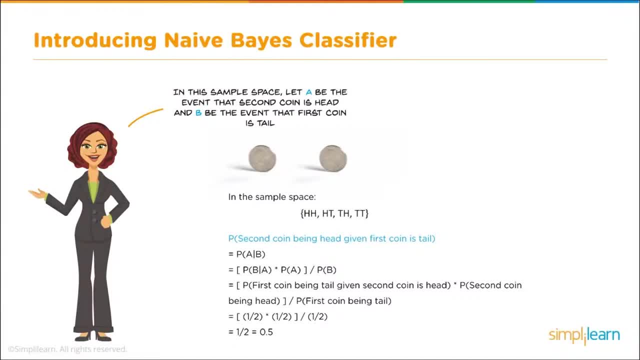 the probability of B, And when we plug that in, we plug in the probability of the first coin being tails, given the second coin is heads, and the probability of the second coin being heads, given the first coin being over the probability of the first coin being tails. When we plug that data. 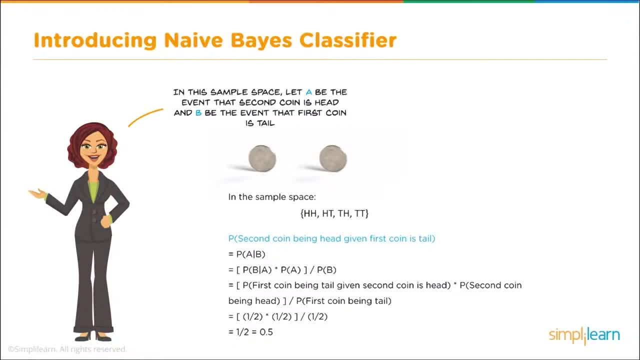 in and we have the probability of the first coin being tails, given the second coin is heads times the probability of the second coin being heads over the probability of the first coin being tails. You can see, it's a simple formula to calculate. We have one half times one half. 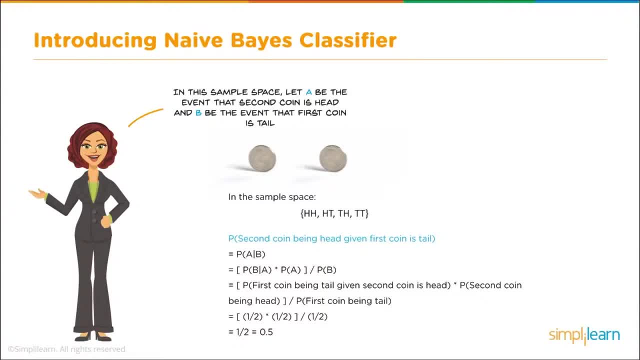 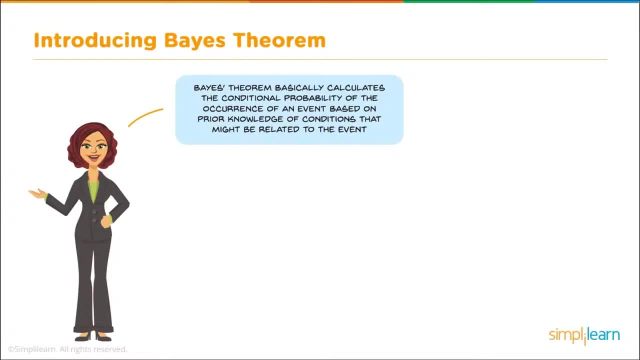 over one half, or one half equals point five or one fourth. So the Bayes theorem basically calculates the conditional probability of the occurrence of an event based on prior knowledge of conditions that might be related to the event. We will explore this in detail when we take up an example of online shopping. 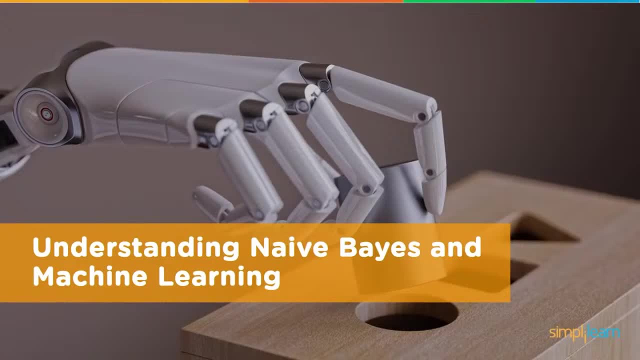 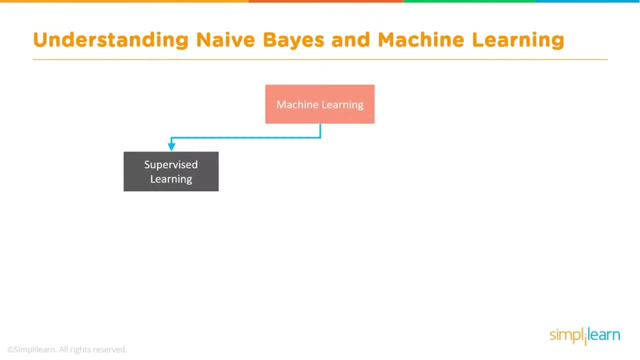 further in this tutorial Understanding naive Bayes and machine learning. Like with any of our other machine learning tools, it's important to understand where the naive Bayes fits in the hierarchy. So under the machine learning, we have supervised learning and there is other things. 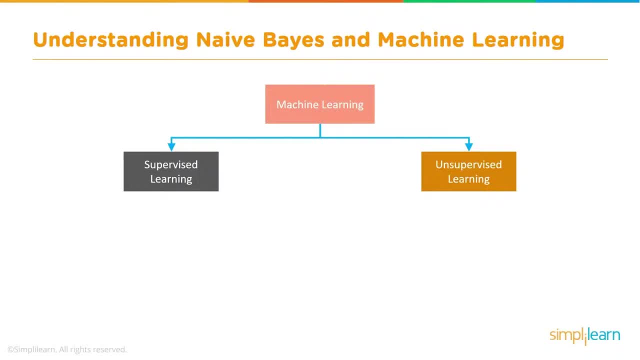 like unsupervised learning. There's also reward system. This falls under the supervised learning. And then under the supervised learning there's classification. There's also regression, But we're going to be in the classification side. And then under classification. is your naive Bayes? 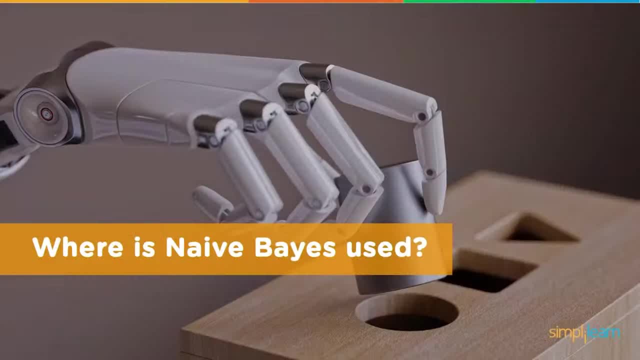 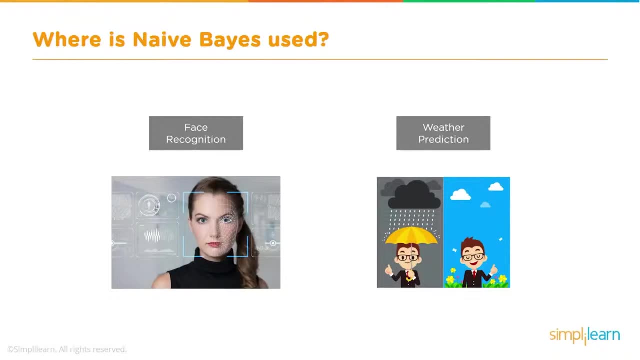 Let's go ahead and glance into where is naive Bayes used. Let's look at some of the used scenarios for it. As a classifier. we use it in face recognition- Is this Cindy, Or is it not Cindy? Or whoever? Or it might be used to identify parts. 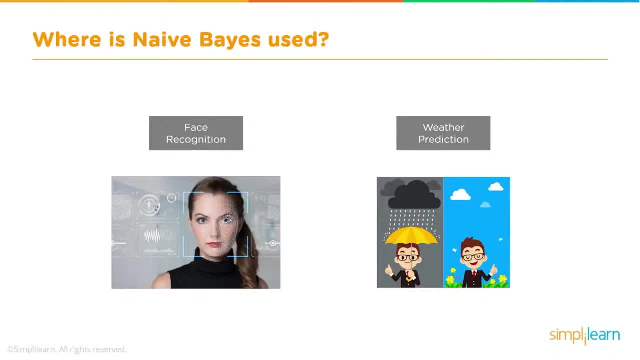 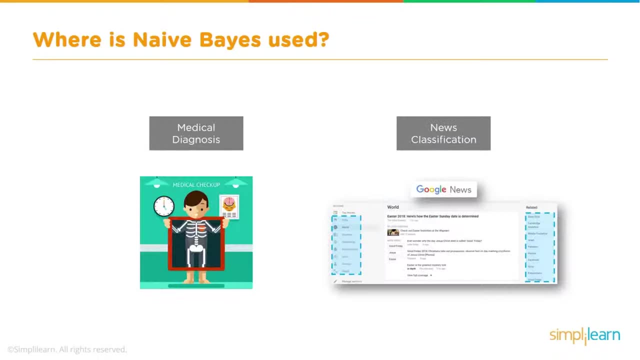 of the face that they then feed into another part of the face recognition program. This is the eye, This is the nose, This is the mouth. Weather prediction: Is it going to be rainy or sunny? Medical recognition News prediction. It's also used. 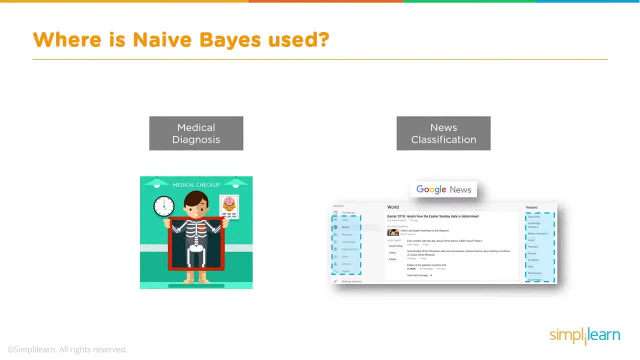 in medical diagnosis We might diagnose somebody as either as high risk or not as high risk for cancer or heart disease Or other ailments, And news classification. You look at the Google News and it says: well, is this political Or is this world news? 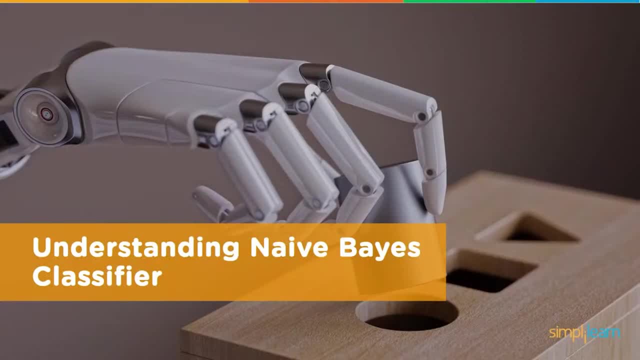 Or a lot of. that's all done with the naive Bayes Understanding naive Bayes classifier. Now we already went through a basic understanding with the coins and the two heads and two tells and head, tell, tell, heads etc. We're going to do just a quick. 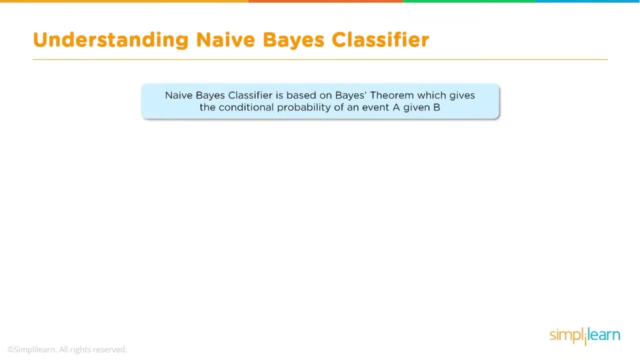 review on that And remind you that the naive Bayes classifier is based on the Bayes theorem, which gives a conditional probability of event A given event B, And that's where the probability of A given B equals the probability of B given A times probability. 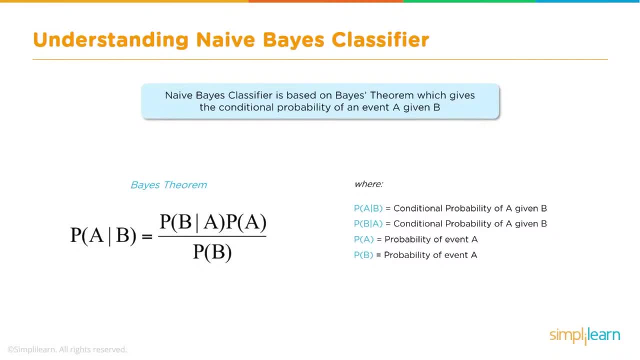 of A over probability of B. Remember, this is an algebraic function so we can move these different entities around. We can multiply by the probability of B, So it goes to the left hand side, And then we can divide by the probability of A given B. And just as 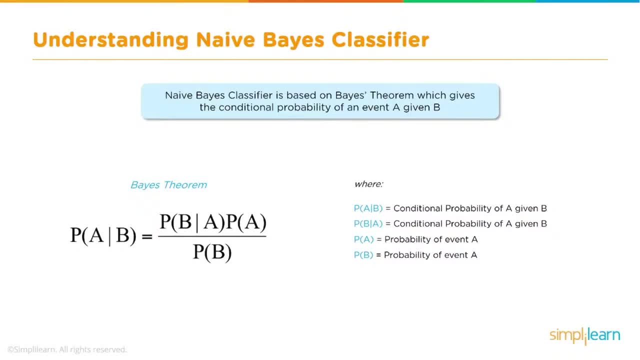 easily come up with a new formula for the probability of B. To me, staring at these algebraic functions kind of gives me a slight headache. It's a lot better to see if we can actually understand how this data fits together in a table, And let's go ahead and start applying it to some. 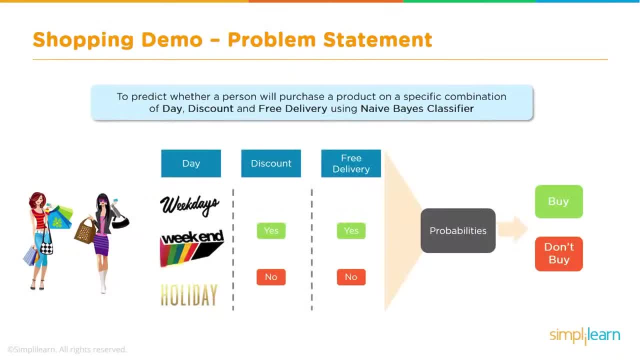 actual data so you can see what that looks like. So we're going to start with the shopping demo problem statement And remember we're going to solve this first in table form so you can see what the math looks like, And then we're going to solve it in Python. 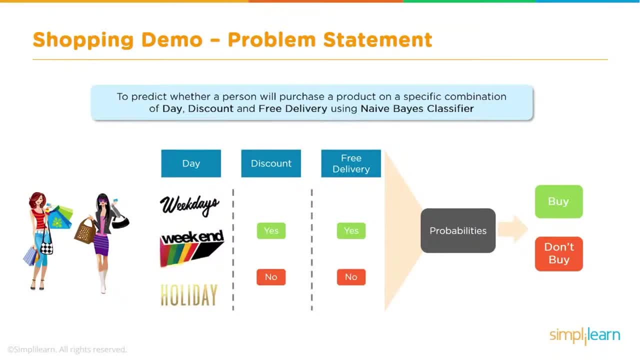 And in here we want to predict whether the person will purchase a product. Are they going to buy or don't buy? Very important: if you're running a business, you want to know how to maximize your profits or at least maximize the purchase of the people coming into your store. 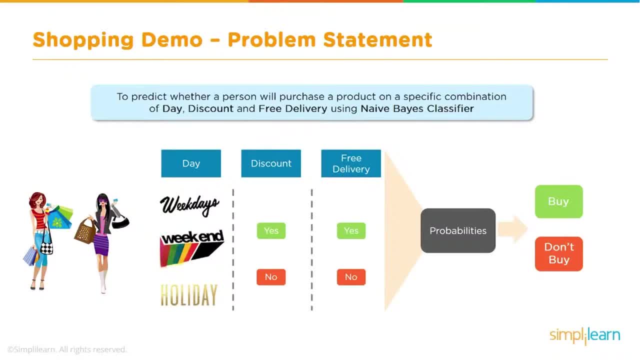 We're going to look at a specific combination of different variables. In this case we're going to look at the day, the discount and the free delivery And you can see here under the day. we want to know whether it's on the weekday, you know somebody's working. 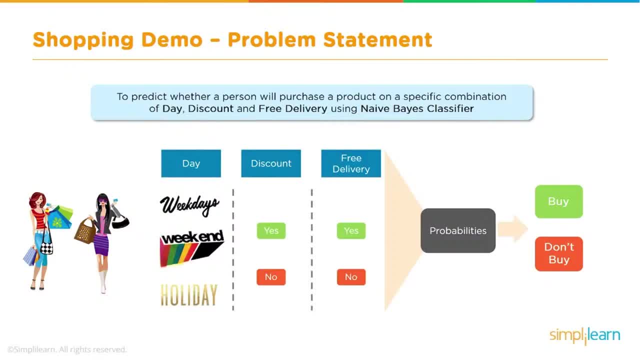 they come in after work, or maybe they don't work Weekend. you can see the bright colors coming down there celebrating not being in work or holiday. And did we offer a discount that day, Yes or no? Did we offer free delivery that day? Yes or no? 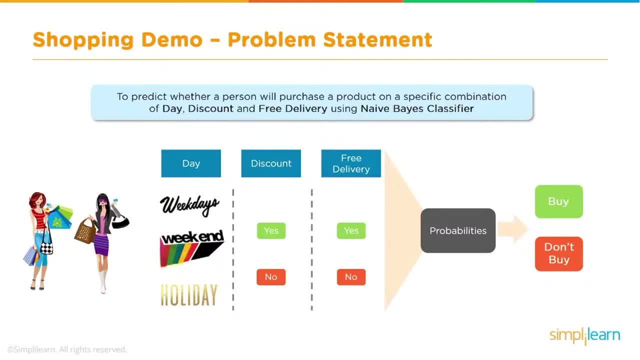 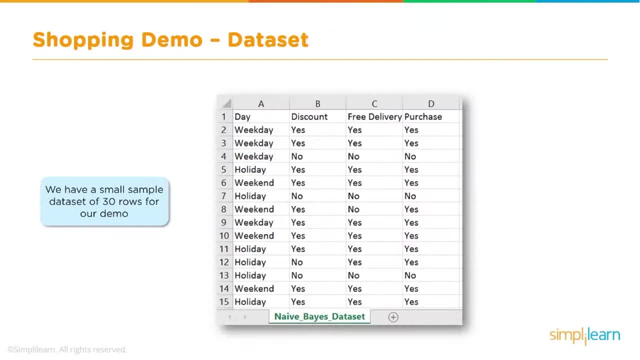 And from this we want to know whether the person's going to buy based on these traits, so we can maximize them and find out the best for getting somebody to come in and purchase our goods and products from our store. Now, having a nice visual is great, but we do. 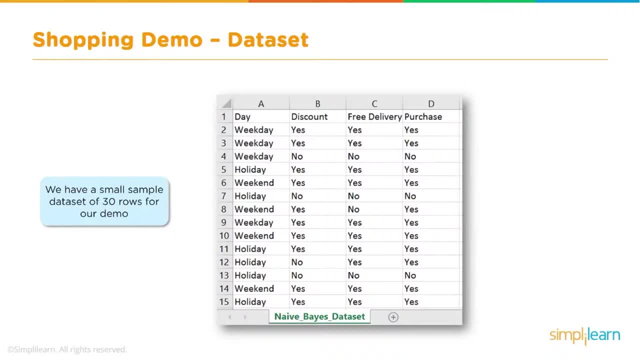 need to dig into the data. So let's go ahead and take a look at the data set. We have a small sample data set of 30 rows. We're showing you the first 15 of those rows for this demo. Now the actual data file you can request. 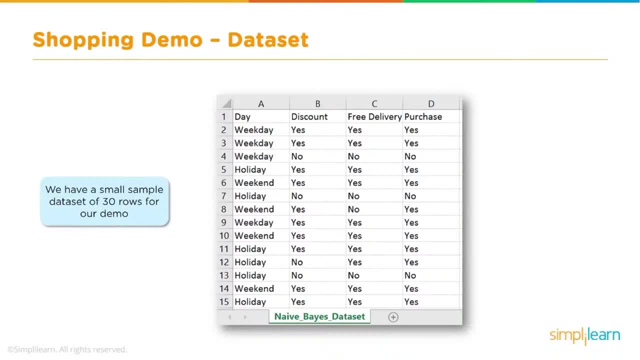 just type in below under the comments on the YouTube video and we'll send you some more information and send you that file. As you can see here, the file is very simple: columns and rows. We have the day, the discount, the free delivery, and did the person purchase or not? 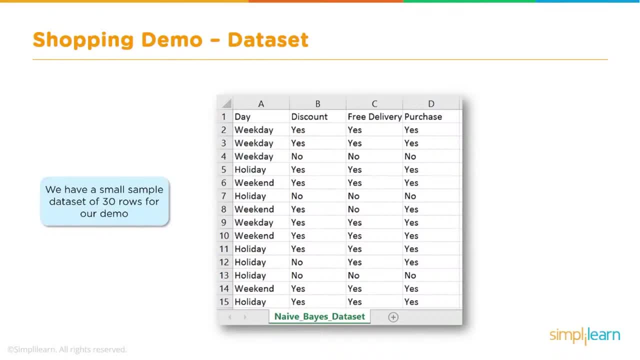 And then we have under the day whether it was a weekday, a holiday, was it the weekend? This is a pretty simple set of data and long before computers, people used to look at this data and calculate this all by hand. So let's go ahead and walk through this. 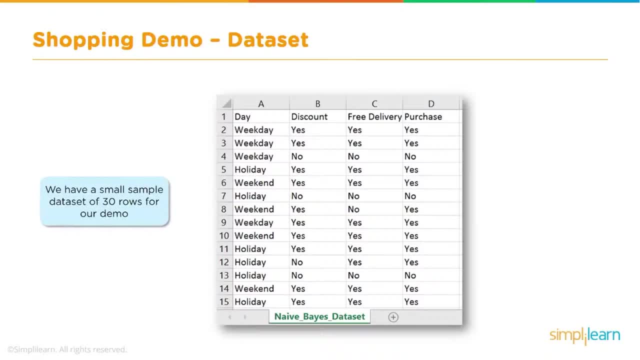 and see what that looks like when we put that into tables. Also note: in today's world we're not usually looking at three different variables in 30 rows. Nowadays, because we're able to collect data so much, we're usually looking at 27,. 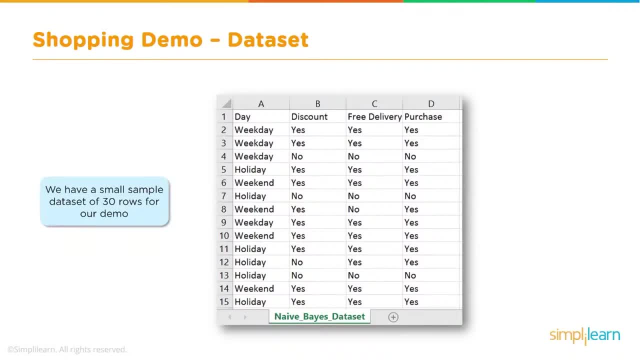 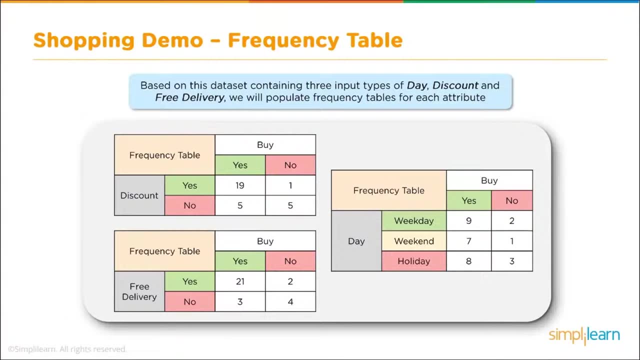 30 variables across hundreds of rows. The first thing we want to do is we're going to take this data and, based on the data set containing our three inputs- day discount and free delivery- we're going to go ahead and populate that to frequency tables. 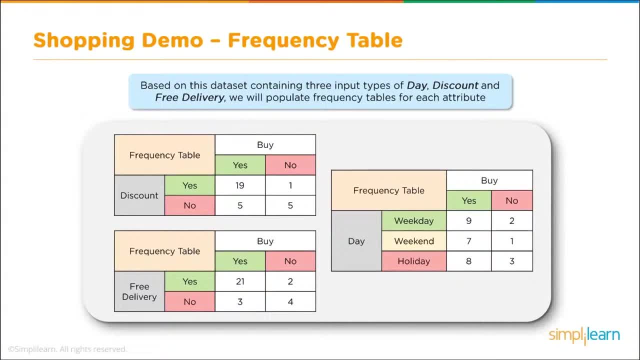 for each attribute. So we want to know if they had a discount. how many people buy and did not buy. did they have a discount, yes or no? do we have a free delivery, yes or no? on those days, how many people made a purchase and how many people didn't? 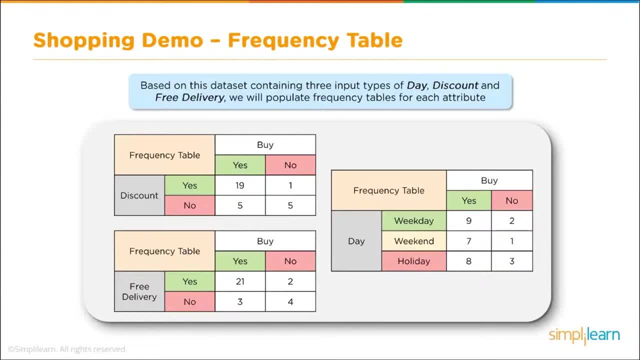 And the same with the three days of the week. Was it a weekday, a weekend, a holiday? and did they buy, yes or no? As we dig in deeper to this table for our Bayes Theorem, let the event buy be A. 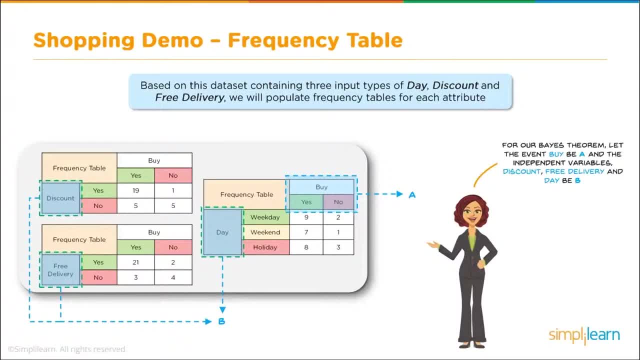 Now remember when we looked at the coins I said we really want to know what the outcome is. Did the person buy or not? And that's usually event A is what you're looking for And the independent variables discount, free delivery and day be B. 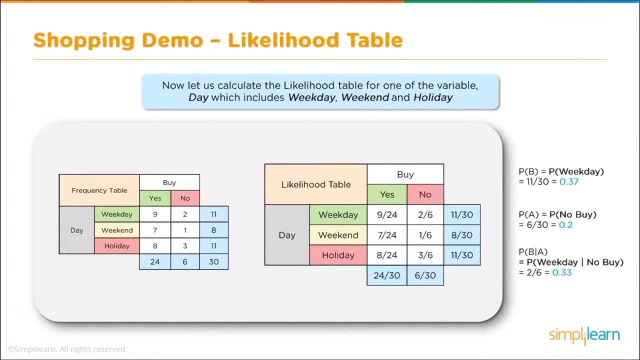 So we'll call that probability of B. Now let us calculate the likelihood table for one of the variables. Let's start with day, which includes weekday, weekend and holiday, And let us start by summing all of our rows so we have the weekday. 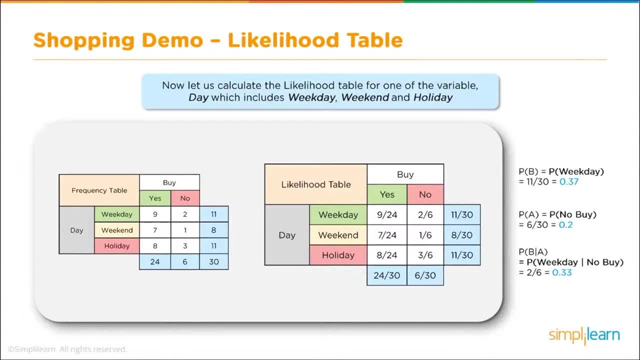 row, and out of the weekdays there's 9 plus 2, so it's 11 weekdays. There's 8 weekend days and 11 holidays. Wow, that's a lot of holidays. And then we want to sum up the total number of days, So we're looking at a total of 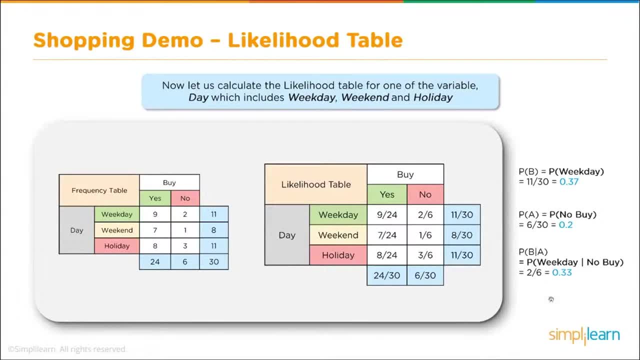 30 days. Let's start pulling some information from our chart and see where that takes us. And when we fill in the chart on the right, you can see that 9 out of 24 purchases are made on the weekday, 7 out of 24 purchases on the. 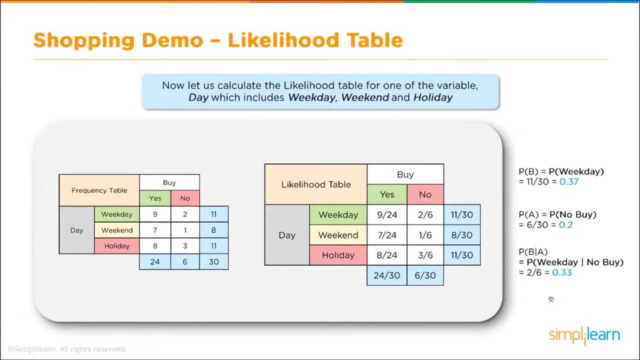 weekend and 8 out of 24 purchases on a holiday And out of all the people who come in, 24 out of 30 purchase. You can also see how many people do not purchase On the weekday: it's 2 out of 6 didn't purchase and so 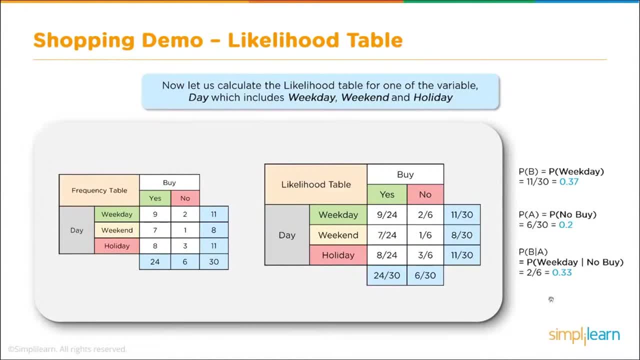 on and so on. We can also look at the totals and you'll see. on the right we put together some of the formulas. The probability of making a purchase on the weekend comes out at 11 out of 30. So, out of the 30 people who came into the store, 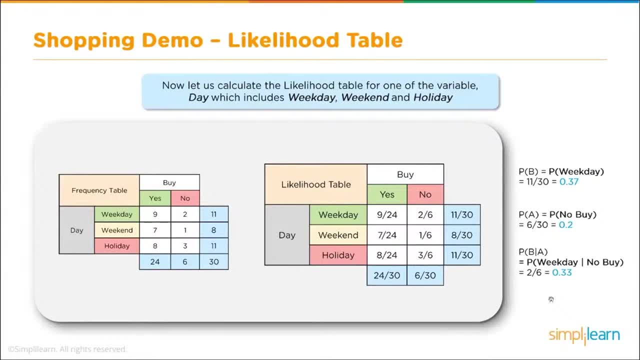 throughout the weekend, weekday and holiday. 11 of those purchases were made on the weekday, And then you can also see the probability of them not making a purchase, And this is done for it doesn't matter which day of the week. So we call that probability of. 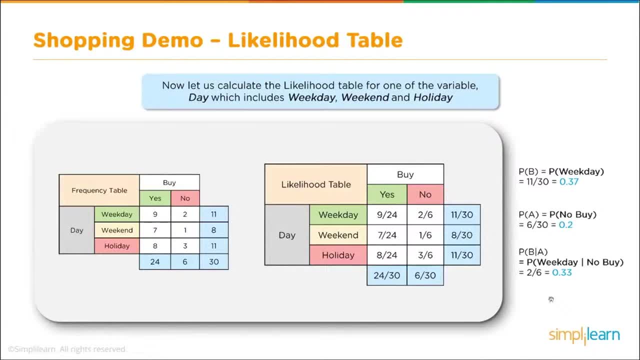 no buy would be 6 over 30 or .2.. So there's a 20% chance that they're not going to make a purchase, no matter what day of the week it is. And finally, we look at the probability of B of A In this case. we're going to look at 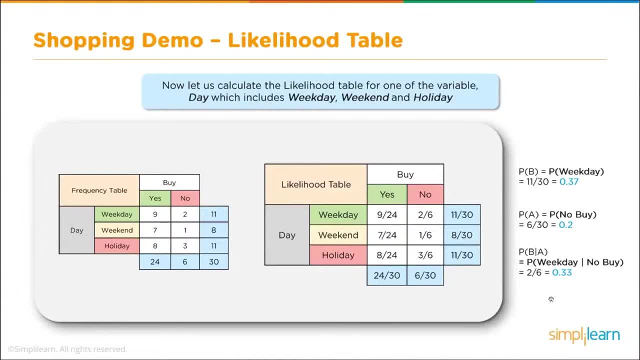 the probability of the weekday and not buying, 2 of the no buys were done out of the weekend out of the 6 people who did not make purchases. So when we look at that, probability of the weekday without a purchase is going to be. 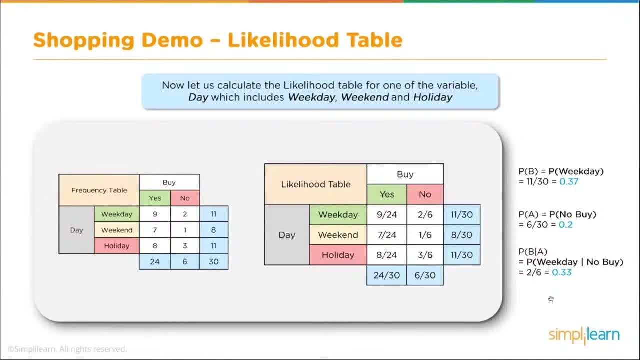 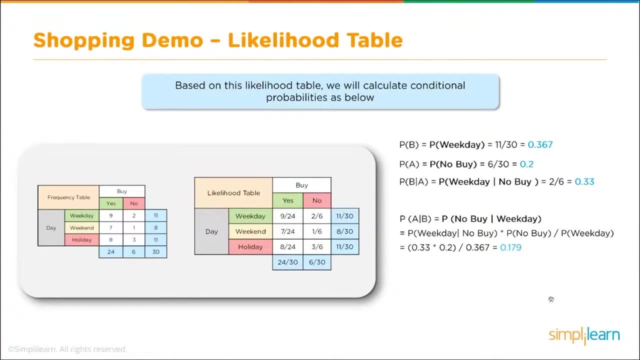 .33 or 33%. Let's take a look at this, at different probabilities, And, based on this likelihood table, let's go ahead and calculate conditional probabilities as below The first three we just did, the probability of making a purchase on the weekday. 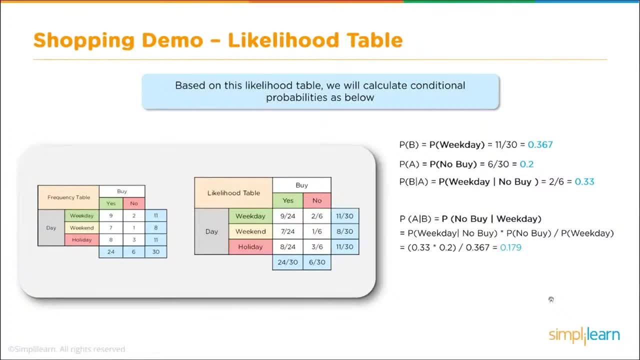 is 11 out of 30, or roughly 36 or 37%, .367.. The probability of not making a purchase at all, doesn't matter what day of the week, is roughly .2 or 20%, And the probability of a weekday no purchase. 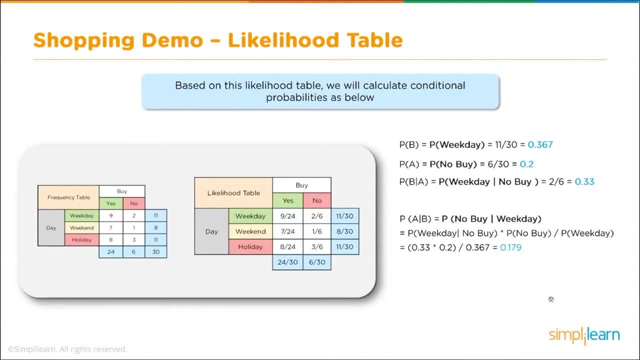 is roughly 2 out of 6.. So 2 out of 6 of our no purchases were made on the weekday. And then, finally, we take our P of AB and if you look, we've kept the symbols up there- We've got probability of B. 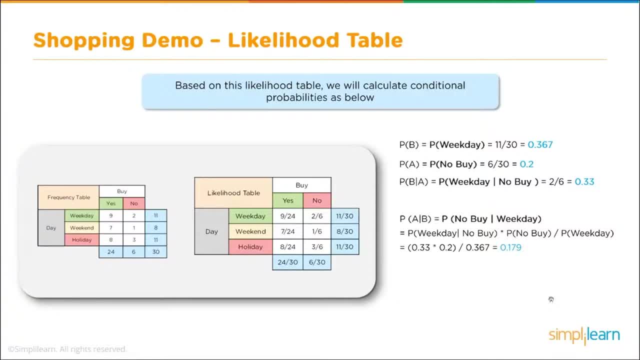 probability of A. probability of B if A. We should remember that the probability of A if B is equal to the first one times the probability of no buys over the probability of the weekday. So we could calculate it both off the table we created. we can also calculate. 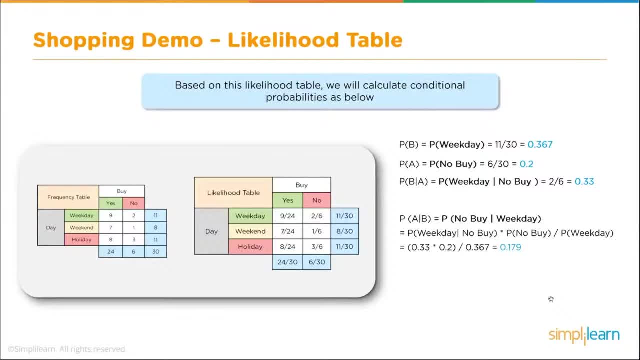 this by the formula and we get the .367, which equals, or .33 times .2 over .367, which equals .179, or roughly 17 to 18%. And that would be the probability of no purchase done on the weekday. And this is important because 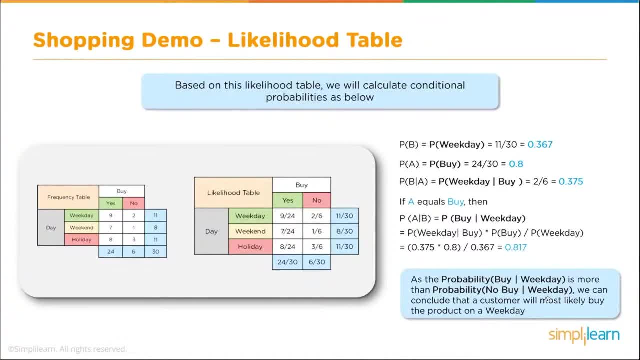 we can look at this and say: as the probability of buying on the weekday is more than the probability of not buying on the weekday, we can conclude that customers will most likely buy the product on a weekday. Now we've kept our chart simple and we're only looking at one aspect. 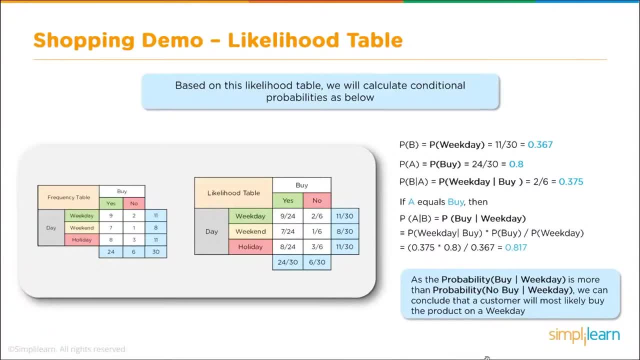 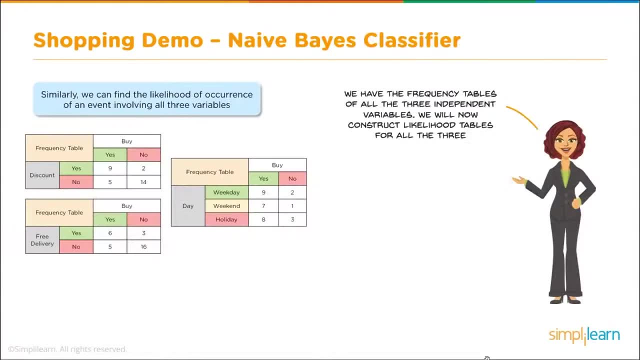 So you should be able to look at the table and come up with the same information or the same conclusion. That should be kind of intuitive at this point. Next, we can take the same setup. We have the frequency tables of all three independent variables. 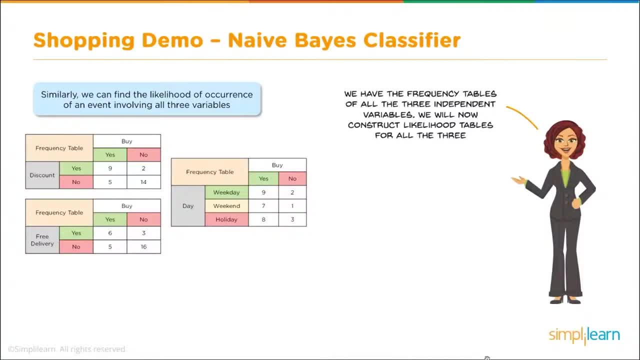 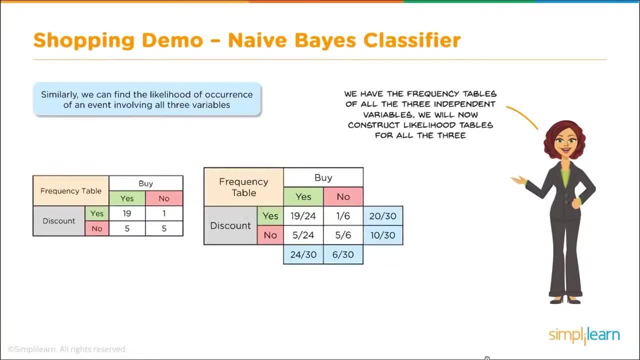 Now we can construct the likelihood tables for all three of the variables we're working with. We can take our day like we did before- We have weekday, weekend and holiday and we filled in this table And then we can come in and also do that. 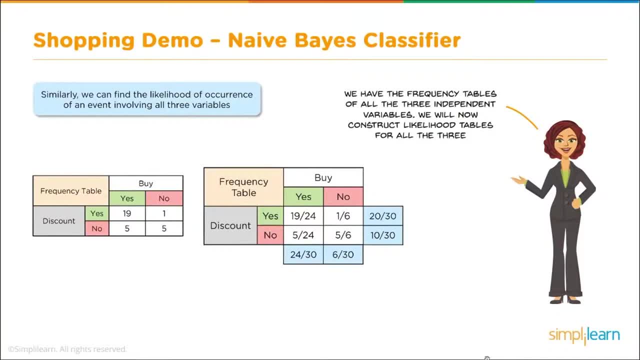 for the discount, yes or no? Did they buy Yes or no? And we fill in that full table. So now we have our probabilities for a discount and whether the discount leads to a purchase or not, And the probability for free delivery. 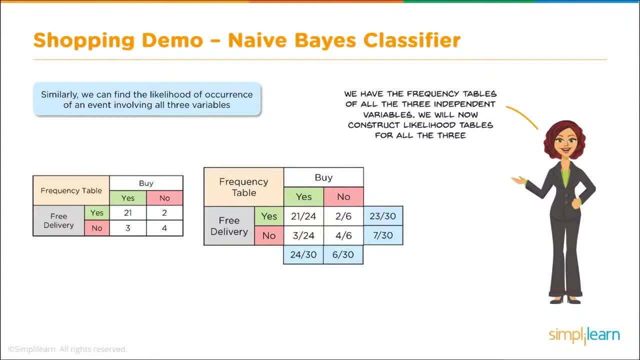 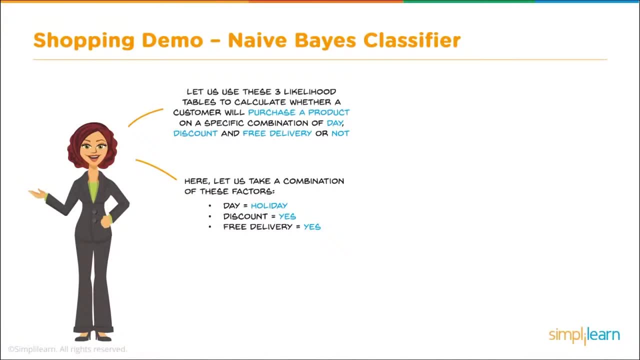 Does that lead to a purchase or not? And this is where it starts getting really exciting. Let us use these three likelihood tables to calculate whether a customer will purchase a product on a specific combination of day discount and free delivery, or not purchase. 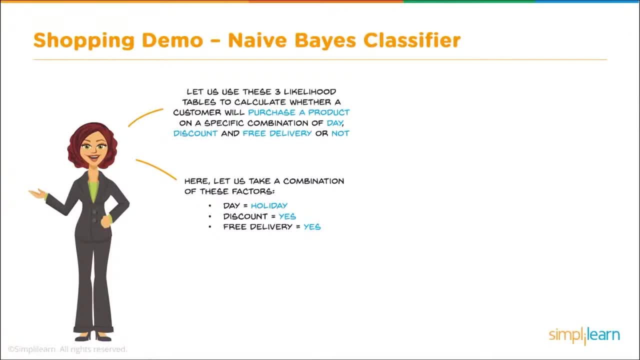 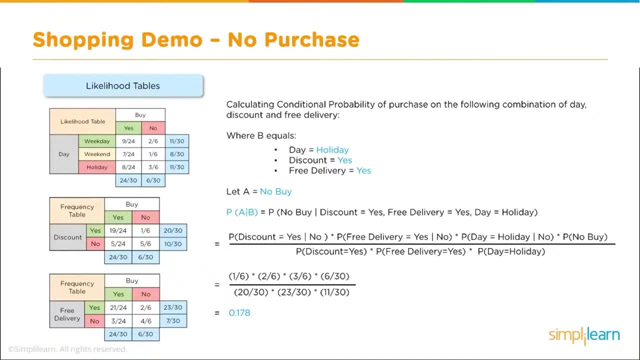 Here, let us take a combination of these factors: Day equals holiday Discount equals yes, Free delivery equals yes. Let's dig deeper into the math and actually see what this looks like, And we're going to start with looking for the probability of them. 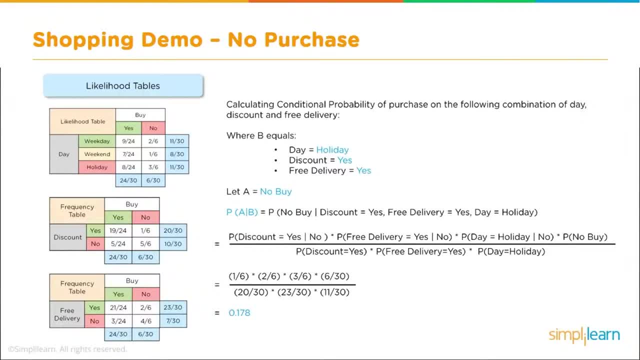 not purchasing. on the following combinations of days, We are actually looking for the probability of A equal- no buy, no purchase, And our probability of B we're going to set equal to. is it a holiday? Did they get a discount? Yes, And was. 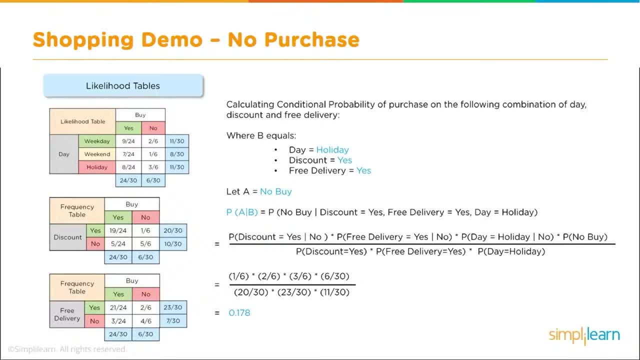 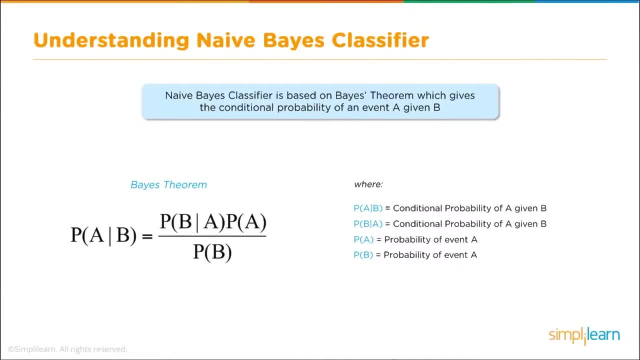 it a free delivery? Yes, Before we go further, let's look at the original equation: The probability of A if B equals the probability of B, given the condition, A times the probability of A over the probability of B occurring Now. this is basic. 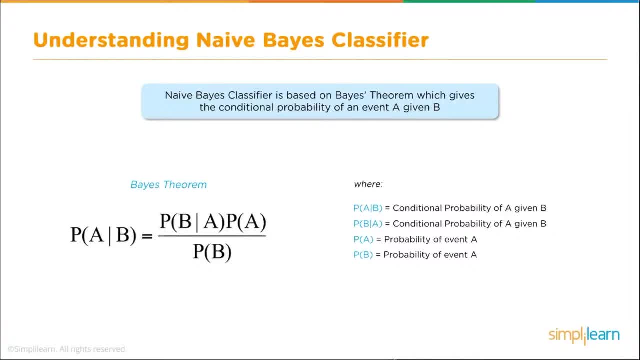 algebra so we can multiply this information together. So when you see the probability of A given B, in this case the condition is B, C and D, or the three different variables we're looking at, And when you see the probability of B, that would be the. 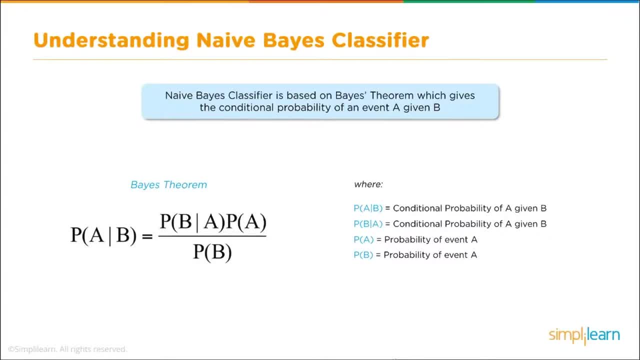 conditions. We're actually going to multiply those three separate conditions out: Probability of. you'll see that in just a second in the formula times the full probability of A over the full probability of B. So here we are, back to this and we're going. 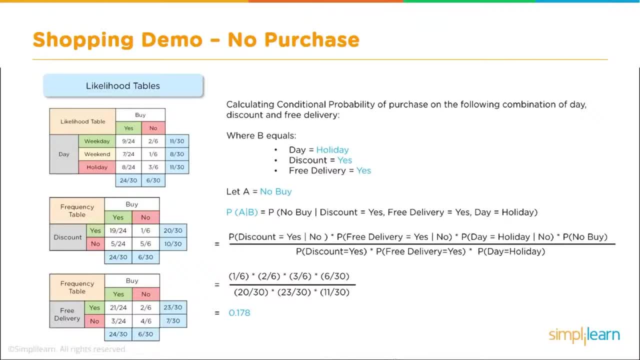 to have let A equal no purchase and we're looking for the probability of B on the condition A, where A sets for three different things. Remember that equals the probability of A given the condition B And in this case we just multiply those three different variables together. So we have 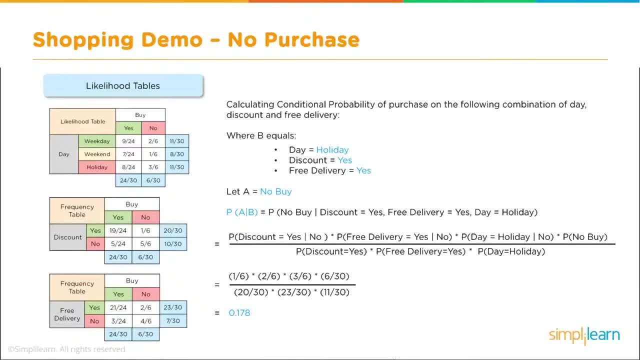 the probability of the discount times, the probability of free delivery times, the probability is the day equal a holiday. Those are our three variables of the probability of A, if B, And then that is going to be multiplied by the probability of them not making a purchase. And then we want to divide. 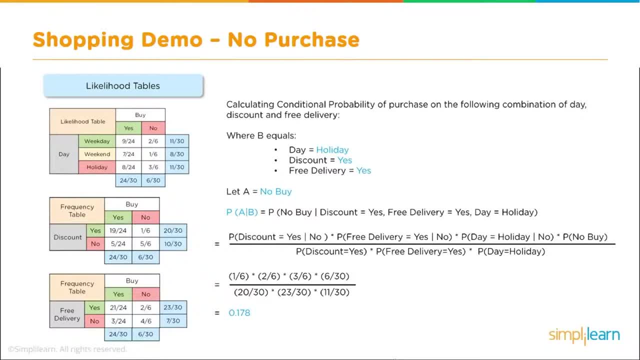 that by the total probabilities and they're multiplied together. So we have the probability of a discount, the probability of a free delivery and the probability of it being on a holiday. When we plug those numbers in, we see that one out of six were no purchase. 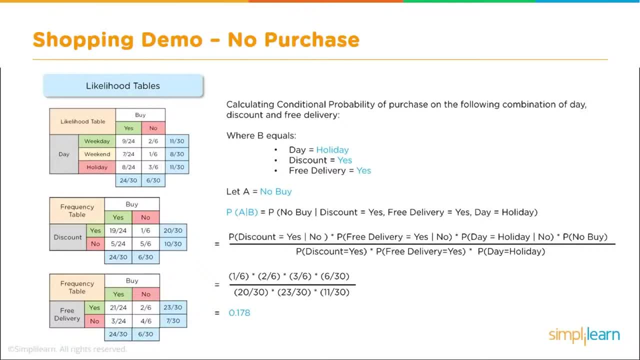 on a discounted day, Two out of six were a no purchase on a free delivery day And three out of six were a no purchase on a holiday. Those are our three probabilities of A if B multiplied out, And then that has to be multiplied by the probability of a no. 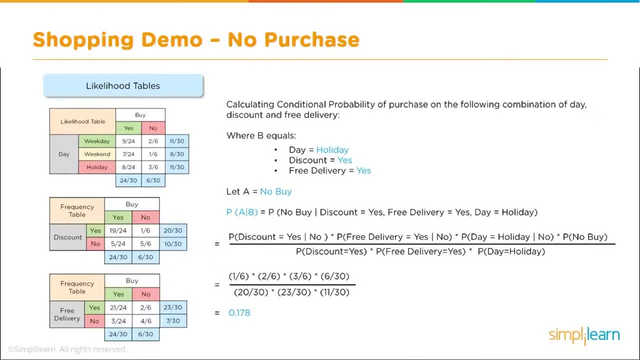 purchase And remember the probability of a no buy is across all the data. So that's where we get the six out of thirty. We divide that out by the probability of each category over the total number, So we get the twenty out of thirty had a discount. 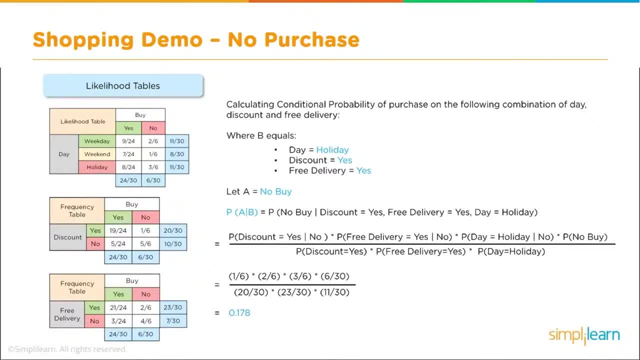 twenty-three out of thirty had a yes for free delivery and eleven out of thirty were on a holiday. We plug all those numbers in, we get point one, seven, eight. So in our probability math we have a point one, seven, eight, if it's. 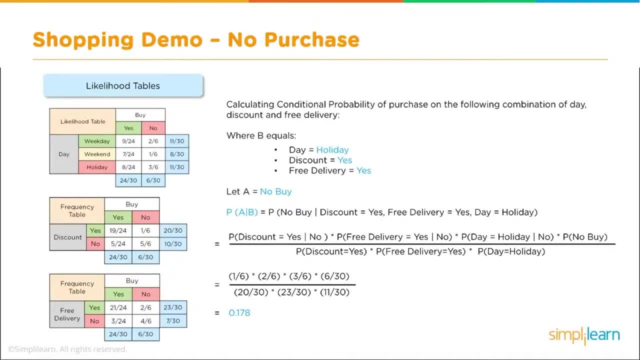 a no buy for a holiday, a discount and a free delivery. Let's turn that around and see what that looks like if we have a purchase. I promise this is the last page of math before we dig into the Python script. So here we're calculating. 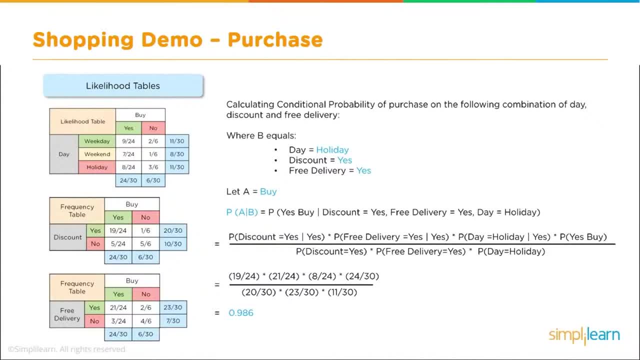 the probability of the purchase, using the same math we did to find out if they didn't buy. Now we want to know if they did buy. And again we're going to go by the day equals a holiday discount equals yes. free delivery equals yes. and let A equal buy. 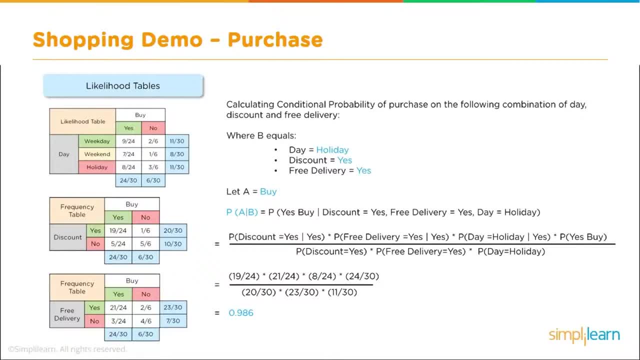 Now, right about now, you might be asking: why are we doing both calculations? Why would we want to know the no buys and buys for the same data going in? Well, we're going to show you that in just a moment, but we have to have both of those pieces of. 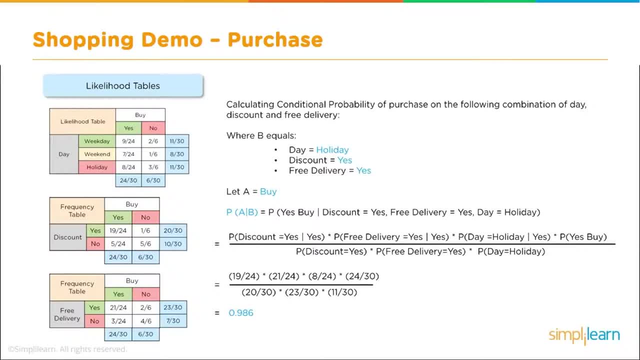 information so that we can figure it out as a percentage as opposed to a probability equation, And we'll get to that finalization here in just a moment. Let's go ahead and walk through this calculation And, as you can see here, the probability of A. 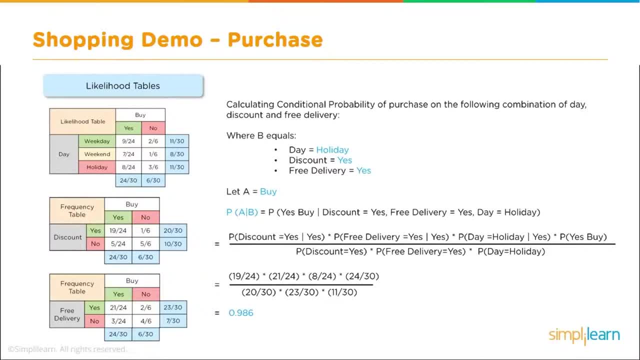 on the condition of B, B being all three categories. did we have a discount with a purchase? do we have a free delivery with a purchase? and is the day equal to holiday? And when we plug this all into that formula and multiply it all out, 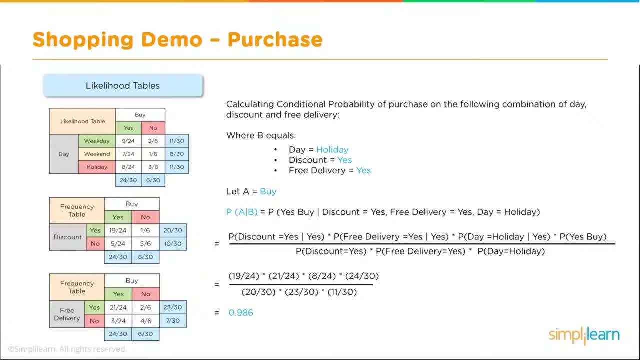 we get our probability of a discount, probability of a free delivery, probability of the day being a holiday times, the overall probability of it being a purchase divided by again multiplying the three variables out the full probability of there being a discount, the full. 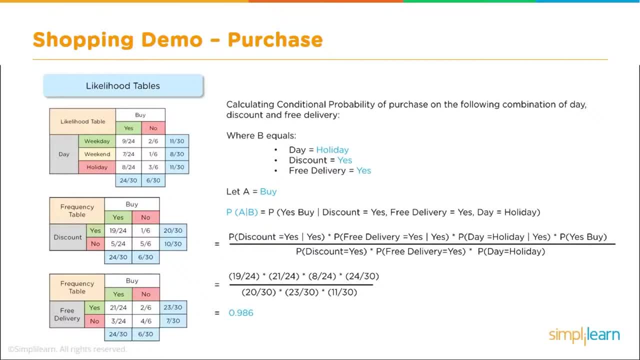 probability of being a free delivery and the full probability of there being a day equal holiday, And that's where we get this: 19 over 24, times, 21 over 24, times, 8 over 24, times the P of A. 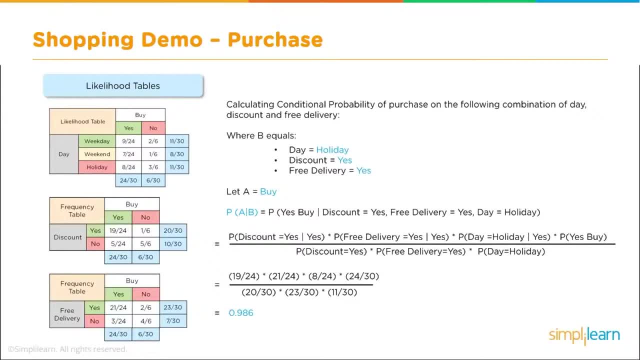 24 over 30, divided by the probability of the discount, the free delivery times the day, or 20 over 30,, 23 over 30, times 11 over 30, and that gives us our 0.986.. 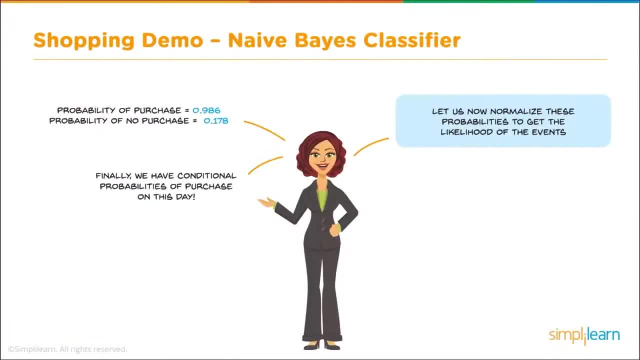 So what are we going to do with these two pieces of data we just generated? Well, let's go ahead and go over them. We have a probability of purchase equals 0.986.. We have a probability of no purchase equals 0.178. 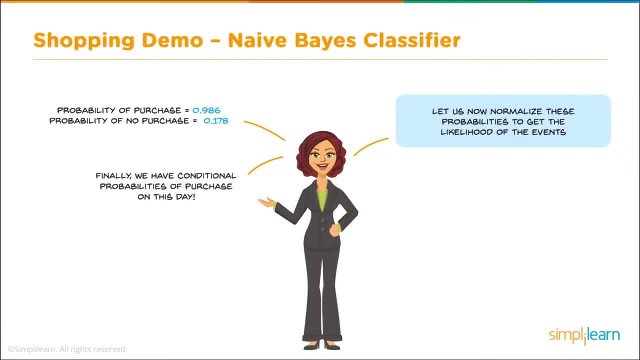 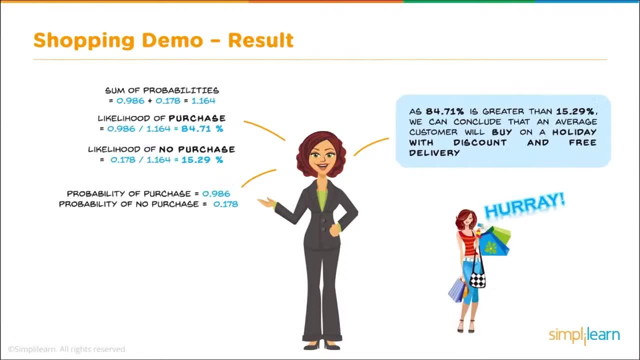 So, finally, we have a conditional probabilities of purchase on this day. Let us take that. we're going to normalize it and we're going to take these probabilities and turn them into percentages. This is simply done by taking the sum of probabilities, which equals. 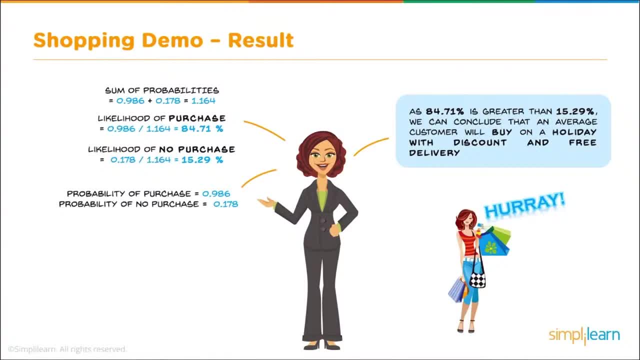 0.98686 plus 0.178, and that equals the 1.164.. If we divide each probability by the sum, we get the percentage, And so the likelihood of a purchase is 84.71% and the likelihood of no purchase is. 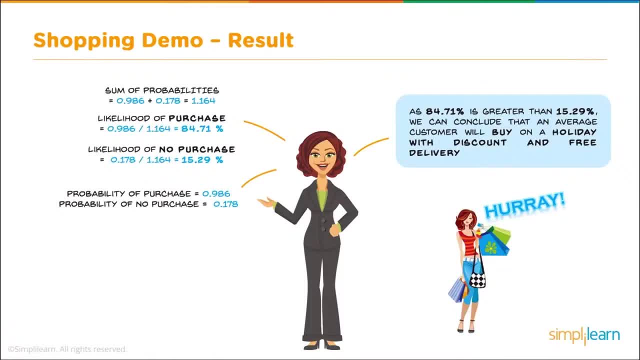 15.29%, given these three different variables. So if it's on a holiday, if it's with a discount and has free delivery, then there's an 84.71% chance that the customer is going to come in and make a purchase. Hooray. 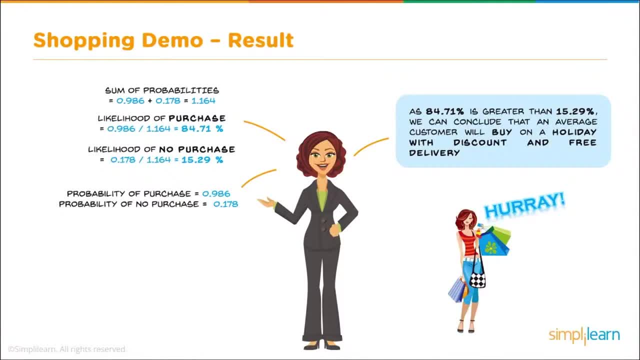 We purchased our stuff, We're making money. If you're owning a shop, that is the bottom line- is you want to make some money so you can keep your shop open and have a living. Now I promised you that we were going to be finishing up the math here. 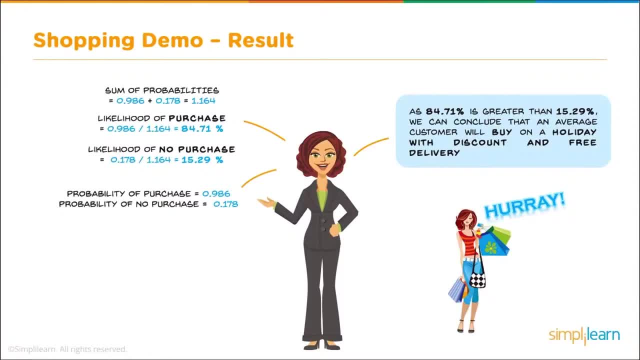 with a few pages. So we're going to move on and we're going to do two steps. The first step is: I want you to understand why you want to use the naive Bayes. What are the advantages of naive Bayes? 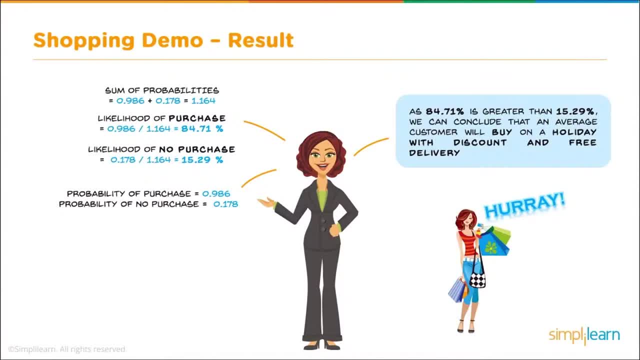 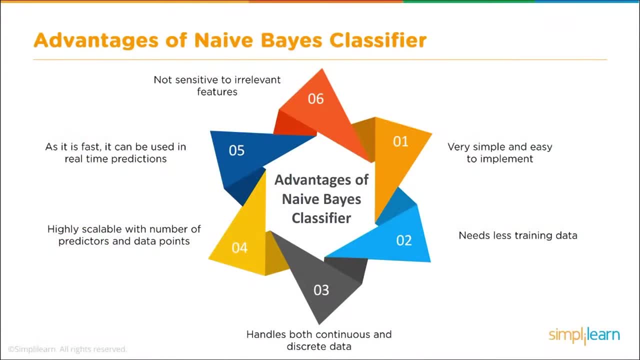 And then once we understand those advantages, we'll just look at that briefly. then we're going to dive in and do some Python coding. Advantages of naive Bayes classifier. So let's take a look at the six advantages of the naive Bayes classifier. 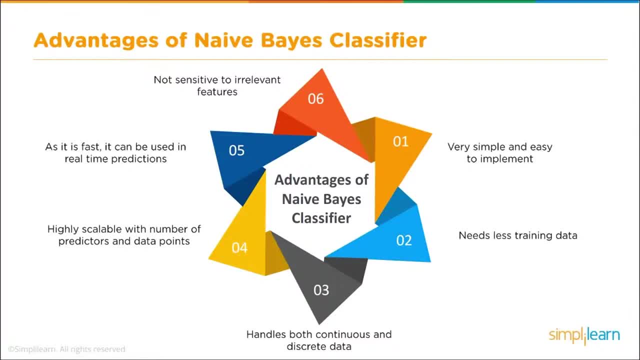 And we're going to walk around this lovely wheel. It looks like an origami folded paper. The first one is very simple and easy to implement. Certainly you could walk through the tables and do this by hand. You've got to be a little careful, because 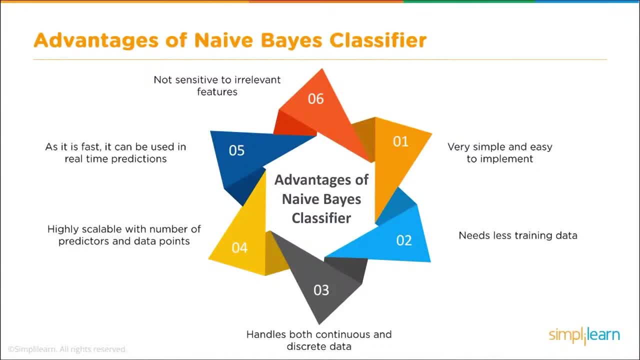 the notations can get confusing. You have all these different probabilities and I certainly mess those up as I put them on. you know, is it on the top or the bottom? You've got to really pay close attention to that. When you put it into Python, it's really nice. 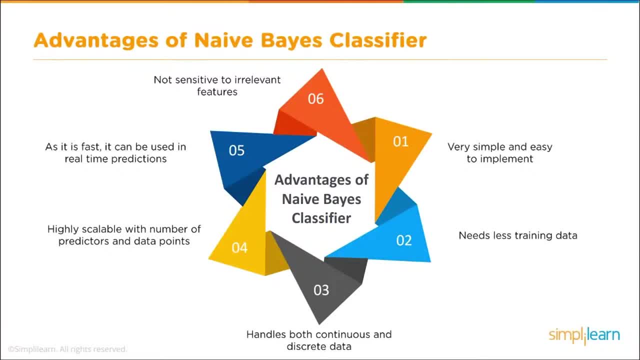 because you don't have to worry about any of that. You let the Python handle that, the Python module. But understanding it, you can put it on a table and you can easily see how it works. and it's a simple algebraic function. 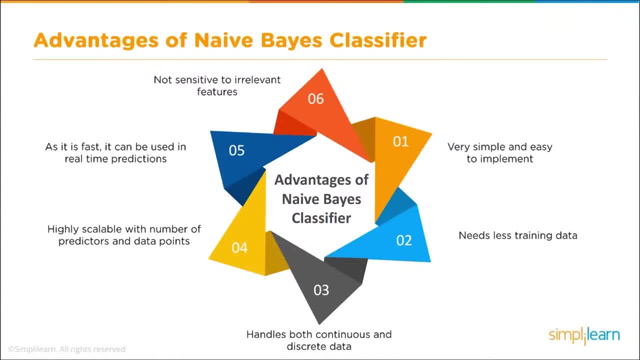 It needs less training data, So if you have smaller amounts of data, this is a great powerful tool for that. It handles both continuous and discrete data. It's highly scalable with number of predictors and data points, So, as you can see, you can just keep multiplying. 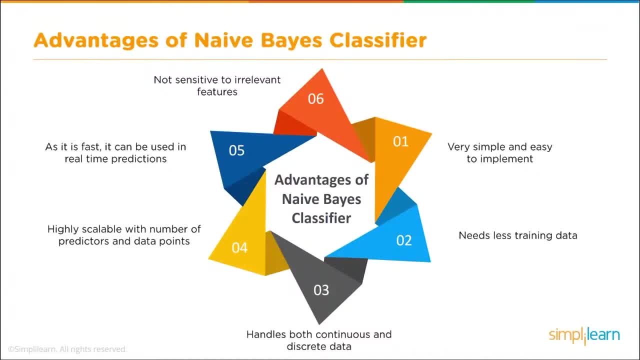 different probabilities in there and you can cover not just three different variables or sets. You can now expand this to even more categories. Number five: it's fast. It can be used in real-time predictions. This is so important. This is why it's used in a lot of our predictions. 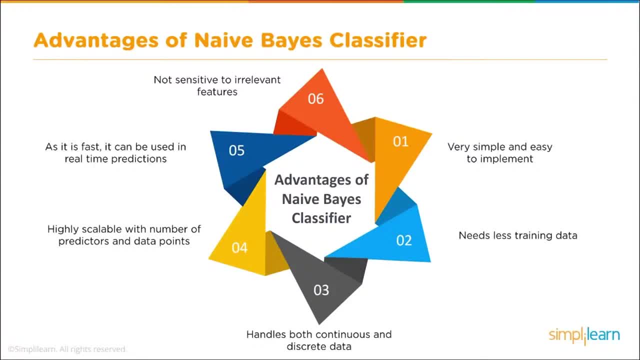 on online shopping carts, referrals, spam filters- is because there's no time delay, as it has to go through and figure out a neural network or one of the other mini setups where you're doing classification, And certainly there's a lot of other tools out there. 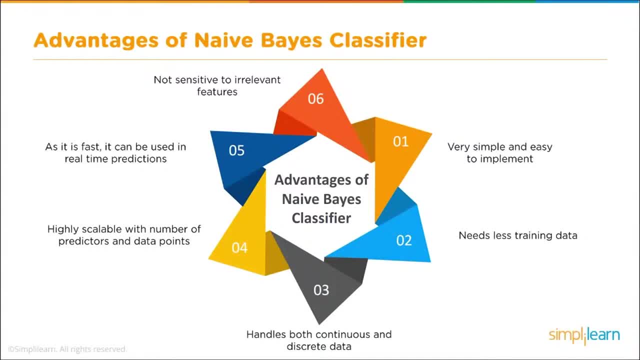 in the machine learning that can handle these, but most of them are not as fast as the Naive Bayes. And then, finally, it's not sensitive to relevant features. So it picks up on your different probabilities and, if you're short on data, on one probability. 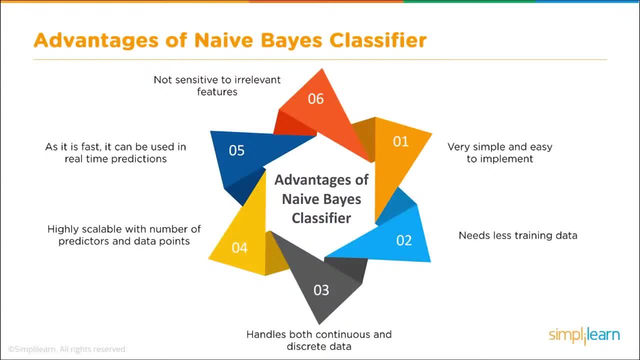 you can kind of automatically adjust for that. Those formulas are very automatic and so you can still get a very solid predictability, even if you're missing data or you have overlapping data for two completely different areas. We see that a lot in doing census and studying of people and habits. 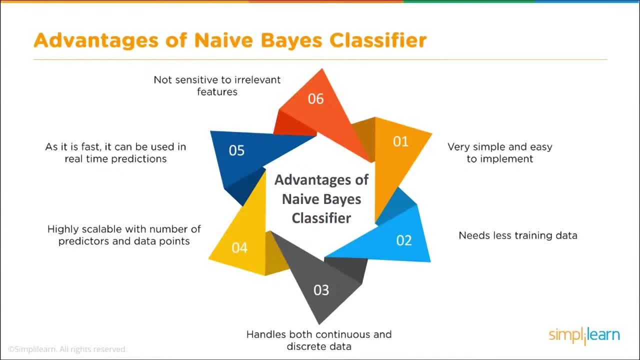 where they might have one study that covers one aspect and another one that overlaps, and because the two overlap, they can then predict the unknown for the group that they haven't done the second study on, or vice versa. So it's very powerful in that it is not sensitive. 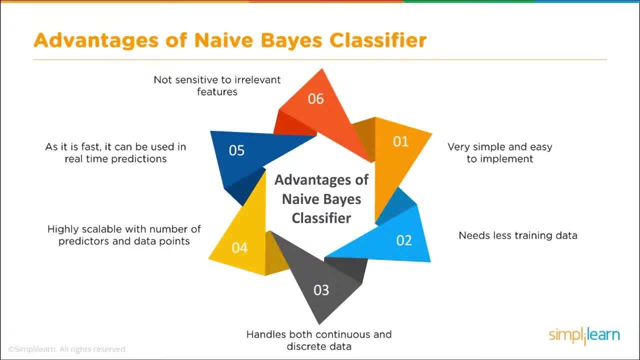 to the irrelevant features and, in fact, you can use it to help predict features that aren't even in there. So now we're down to my favorite part. We're going to roll up our sleeves and do some actual programming. We're going to do the use case text classification. 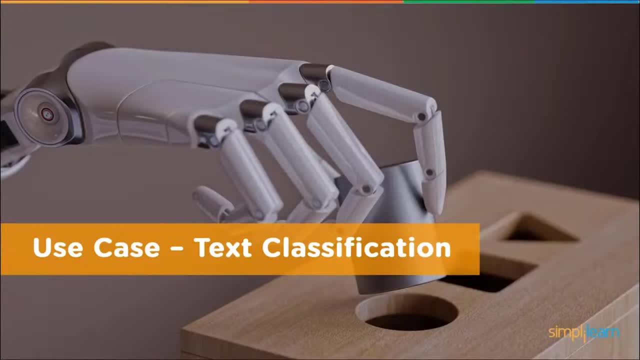 Now I would challenge you to go back and send us a note on the notes below underneath the video and request the data for the shopping cart so you can plug that in to Python code and do that on your own time so you can walk through it, since we walked through all the information on it. 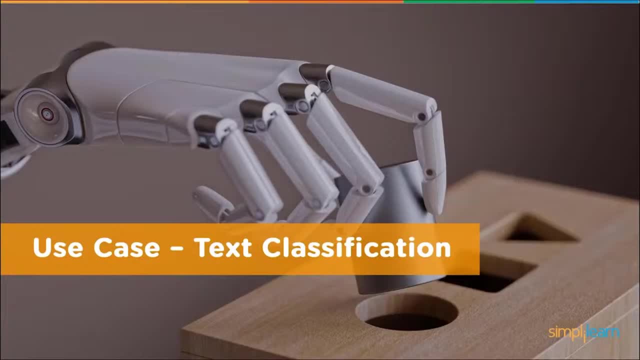 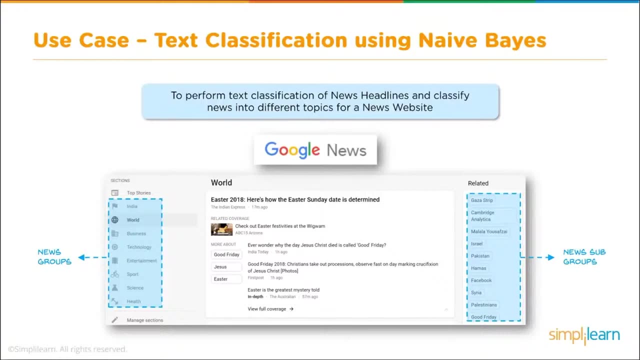 But we're going to do a Python code doing text classification- Very popular for doing the naive bays. So we're going to use our new tool to perform a text classification of news headlines and classify news into different topics for a news website. As you can see, here we have a nice image. 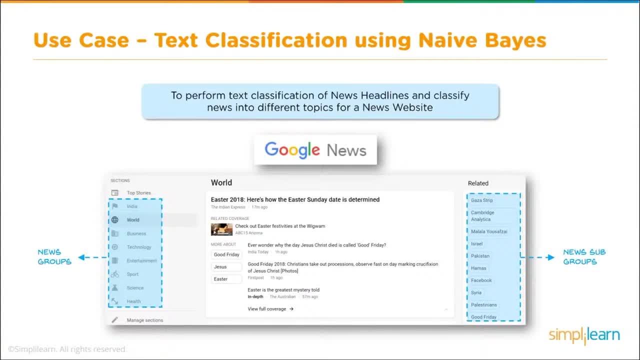 of the Google News and then related on the right subgroups. I'm not sure where they actually pulled the actual data we're going to use from. We're going to use the standard sets, But certainly this can be used on any of our. 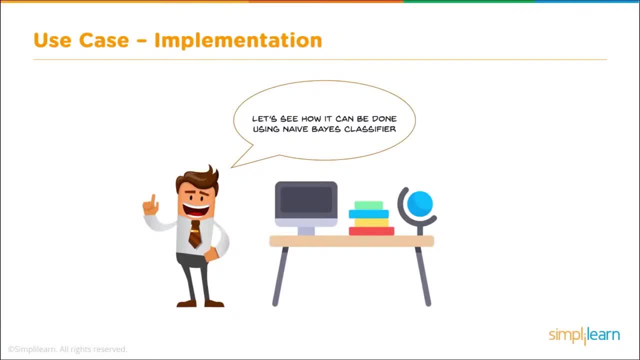 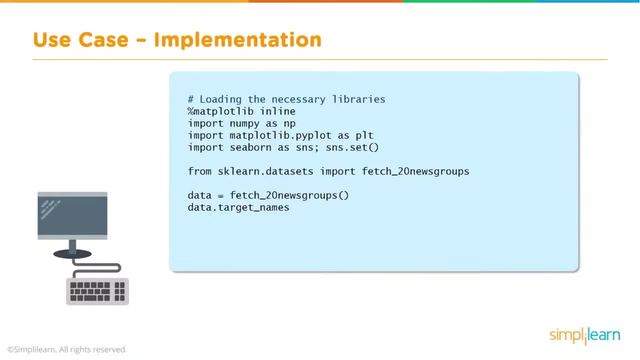 news headlines and classification. So let's see how it can be done using the naive bays classifier. Now we're at my favorite part. We're actually going to write some Python script, Roll up our sleeves And we're going to start by doing our imports. 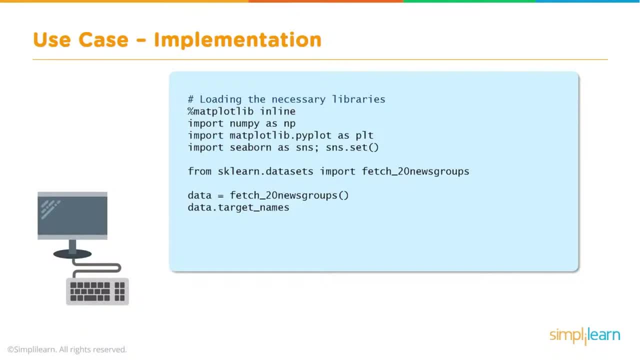 These are very basic imports, including our news group. We'll take a quick glance at the target names. Then we're going to go ahead and start training our data set and putting it together. We'll put together a nice graph, because it's always good to have a graph. 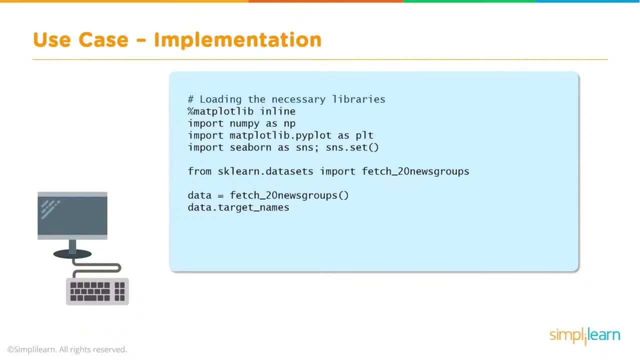 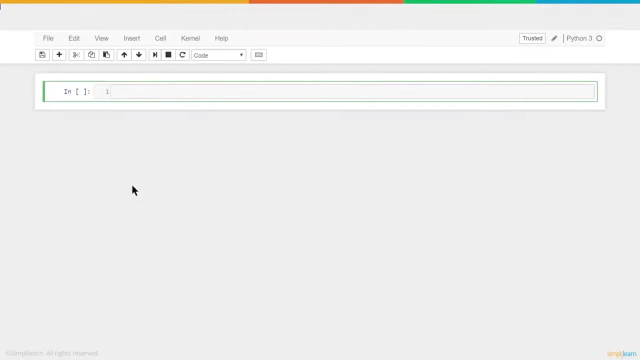 and once we've trained it and we've shown you a graph of what's going on, then we're going to explore how to use it and see what that looks like. Now I'm going to open up my favorite editor, or inline editor for Python. 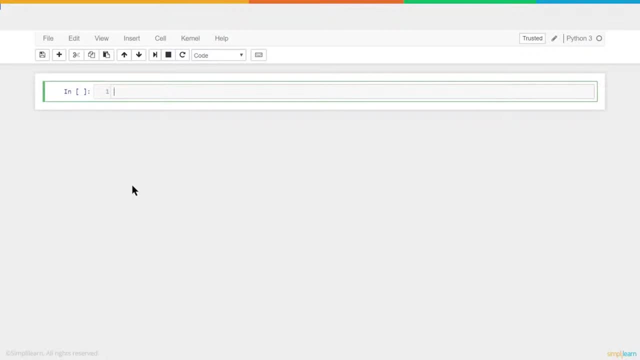 You don't have to use this. You can use whatever your editor that you like, Whatever interface IDE you want. This just happens to be the Anaconda Jupyter Notebook And I'm going to paste that first piece of code in here so we can walk through it. 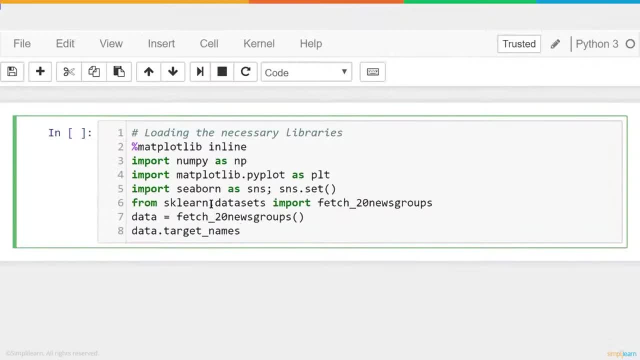 Let's make it a little bigger on the screen so you have a nice view of what's going on. And we're using Python 3. So this would work in any of your 3x. If you have it set up correctly, it should also work in a lot of the 2x. 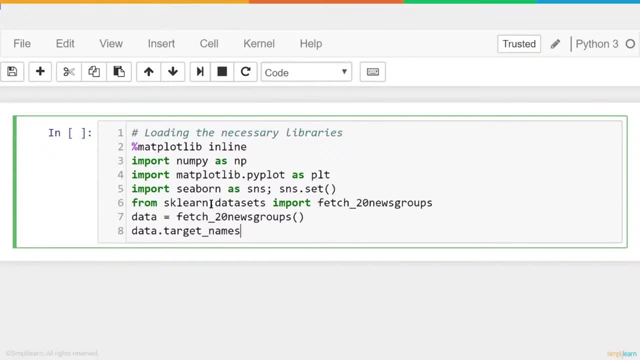 You just have to make sure all of the versions of the modules match your Python version, And in here you'll notice. the first line is your percentage matplot library inline. Now three of these lines of code are all about plotting the graph. This one lets the notebook notes. 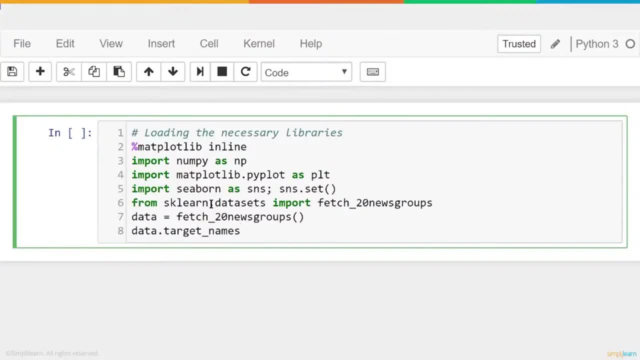 and this is the inline setup that we want the graphs to show up on this page. Without it, in a notebook like this and an explorer interface, it won't show up. Now, a lot of IDEs don't require that. A lot of them like if I'm working on one of my other setups. 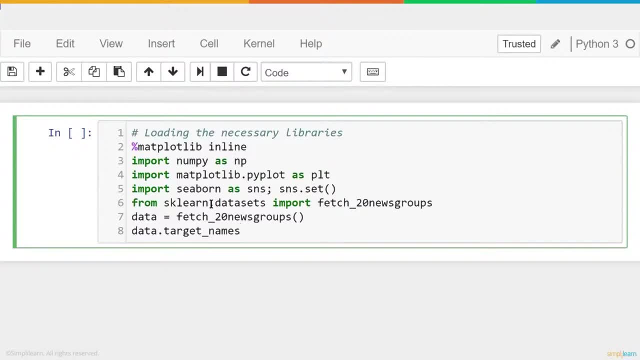 it just has a popup and the graph pops up on there. So you have that setup also. But for this we want the matplot library inline. And then we're going to import numpy as np, that's number Python, which has a lot of different formulas in it. 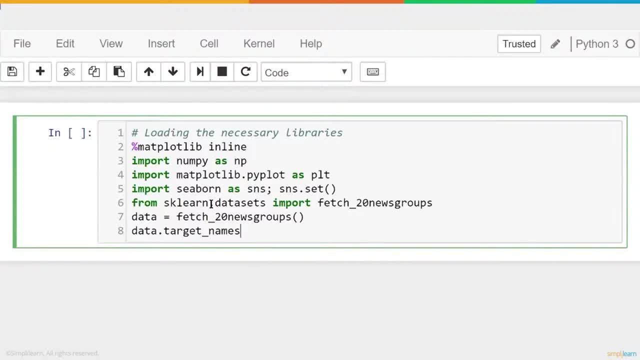 that we use for both of our sklearn module And we also use it for any of the upper math functions in Python. It's very common to see that as np, The next two lines are all about our graphing. Remember I said three of these were about graphing. 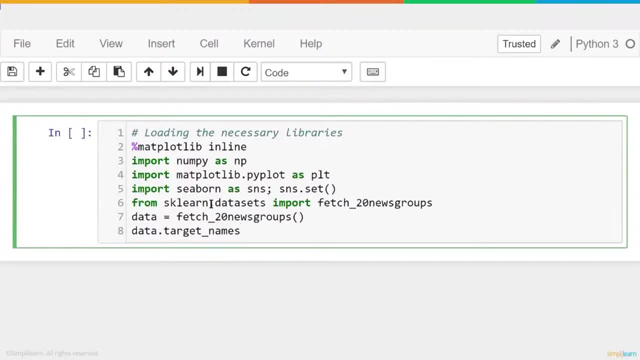 Well, we need our matplot library, pyplot, as plt, and you'll see that plt is a very common setup, as is the sns and just like the np, And we're going to import sklearn as sns and we're going to do the snsset. 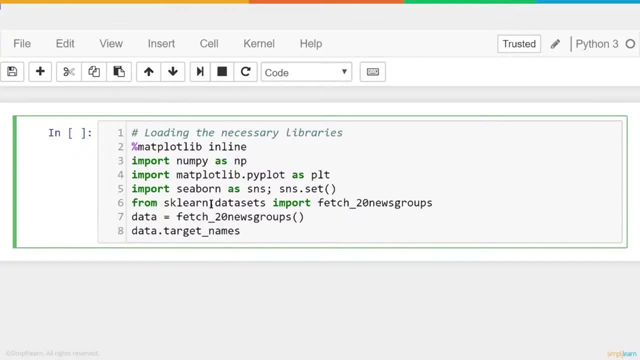 Now sklearn sits on top of pyplot and it just makes a really nice heatmap. It's really good for heatmaps And if you're not familiar with heatmaps, that just means we give it a color scale. The term comes from the brighter red it is, the hotter it is. 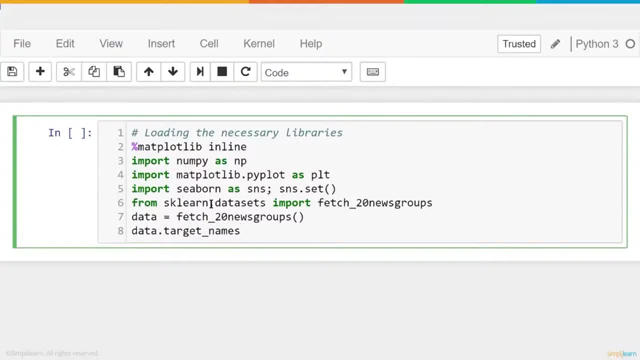 in some form of data And you can set it to whatever you want, And we'll see that later on. So you'll see that those three lines of code here are just importing the graph function so we can graph it And as a data scientist, you always want to. 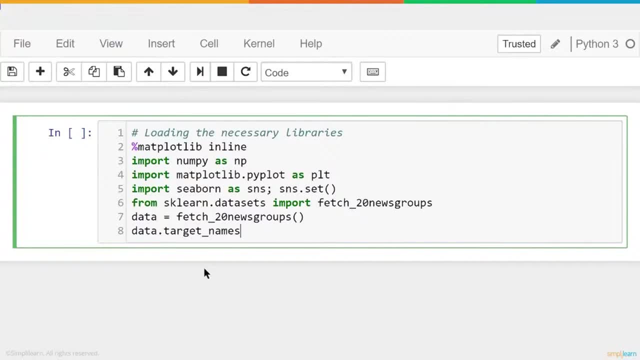 graph your data and have some kind of visual. It's really hard just to shove numbers in front of people and they look at it and it doesn't mean anything. And then from the sklearndatasets we're going to import the fetch20 newsgroups. 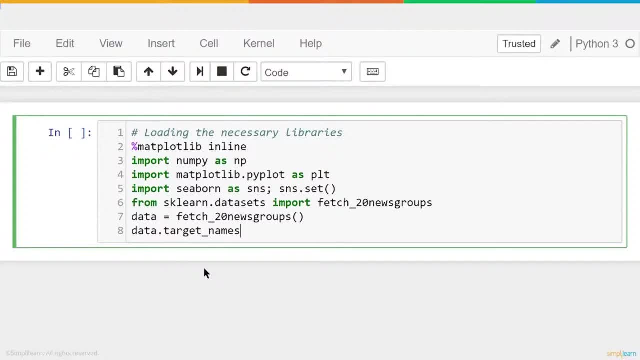 Very common one for analyzing, tokenizing words and setting them up and exploring how the words work and how do you categorize different things when you're dealing with documents. And then we set our data equal to fetch20 newsgroups, So our data variable will have the data in it. 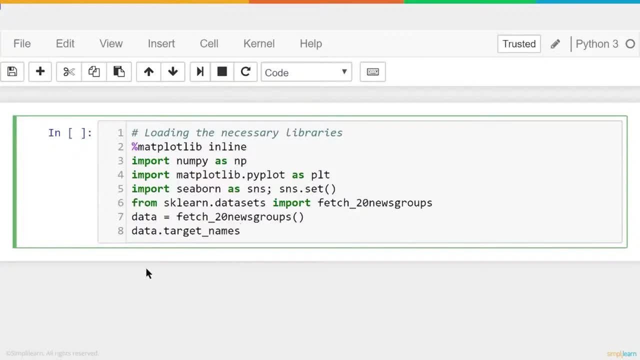 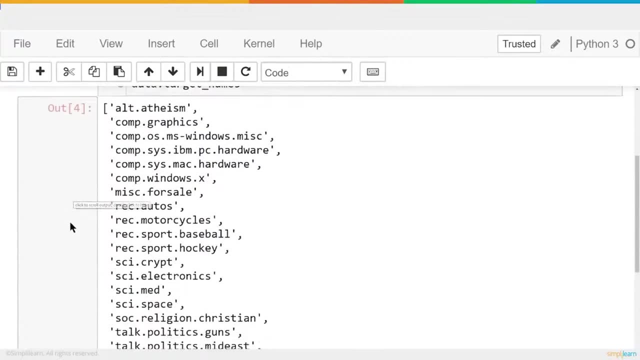 And we're going to go ahead and just print the target names, datatargetnames, And let's see what that looks like And you'll see. here we have alt atheism, comp graphics, comp os, ms windows, miscellaneous, And it goes all the. 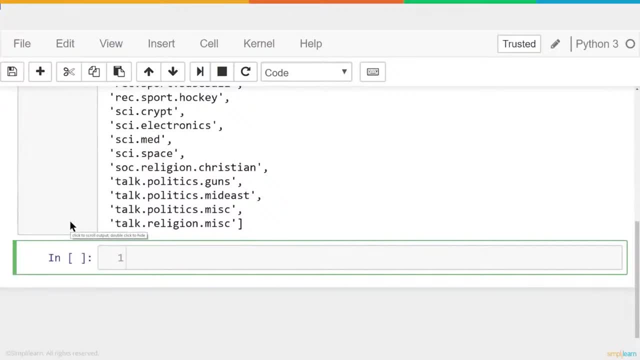 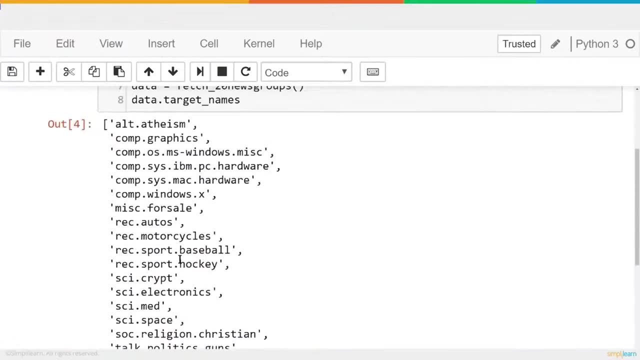 way down to talk politics- miscellaneous. talk religion- miscellaneous. These are the categories they've already assigned to this newsgroup And it's called fetch20 because you'll see, I believe there's 20 different topics in here, or 20 different categories. 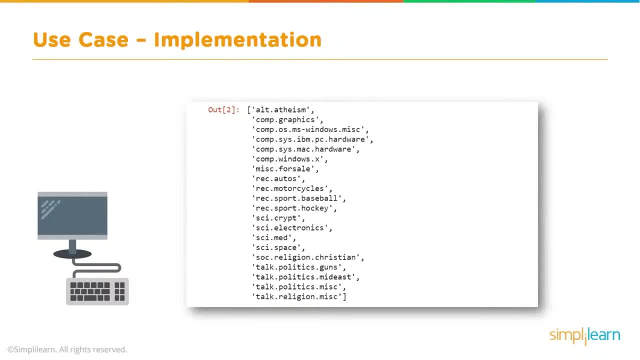 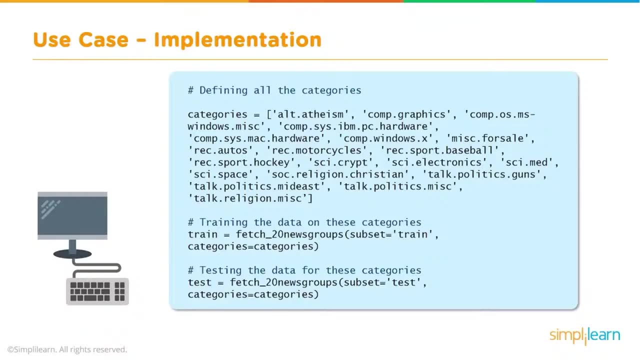 as we scroll down. Now we've gone through the 20 different categories and we're going to go ahead and start defining all the categories and set up our data. So we're actually going to go ahead and get the data all set up and take a look at our data And let's 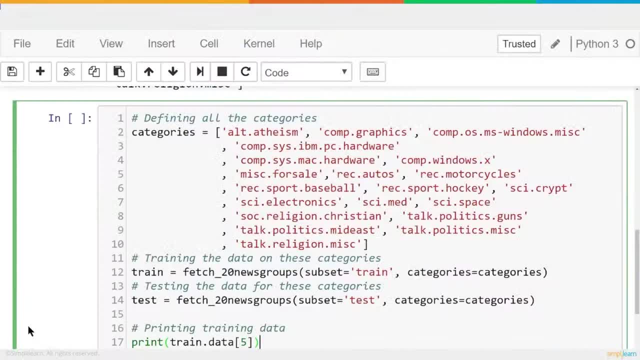 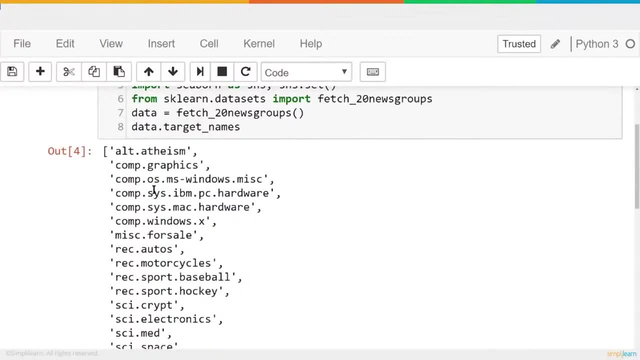 move this over to our Jupyter notebook and let's see what this code does. First, we're going to set our categories. Now, if you noticed up here, I could have just as easily set this equal to datatarget underscore names, because it's the same. 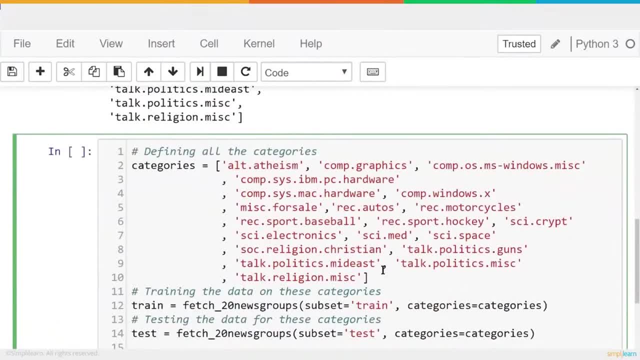 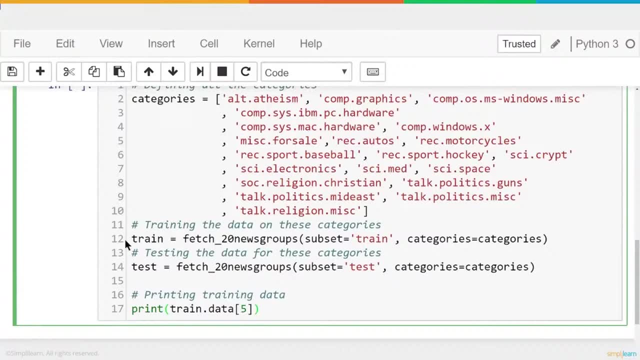 thing, But we want to kind of spell it out for you so you can see the different categories. It kind of makes it more visual so you can see what your data is looking like in the background. Once we've created the categories, we're going to open up a train. 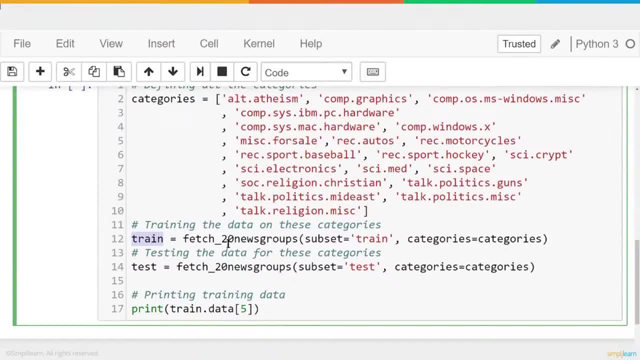 set. So this training set of data is going to go into fetch20 newsgroups and it's a subset in there called train, and categories equals categories. So we're pulling out those categories that match And then if you have a train set, you should also have. 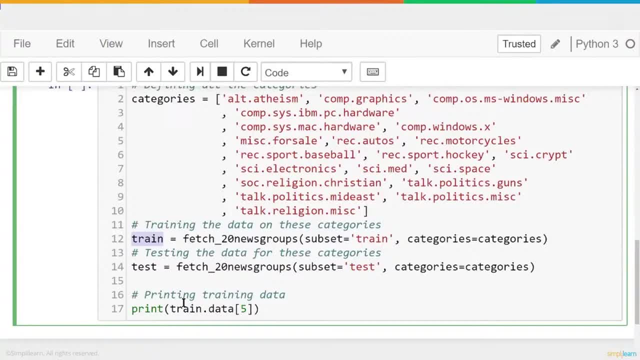 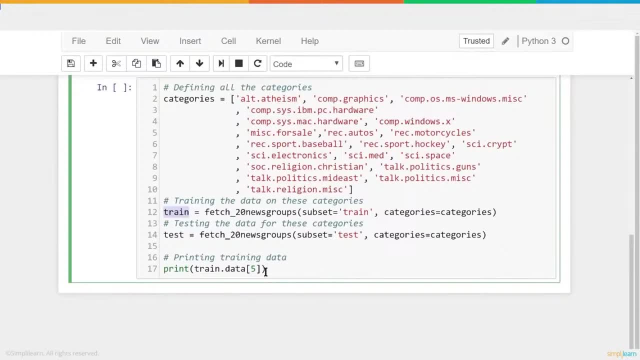 the testing set. We have test equals fetch20, newsgroups, subset equals test and categories equals categories. Let's go down one size so it all fits on my screen. There we go, And just so we can really see what's going on. let's see what happens. 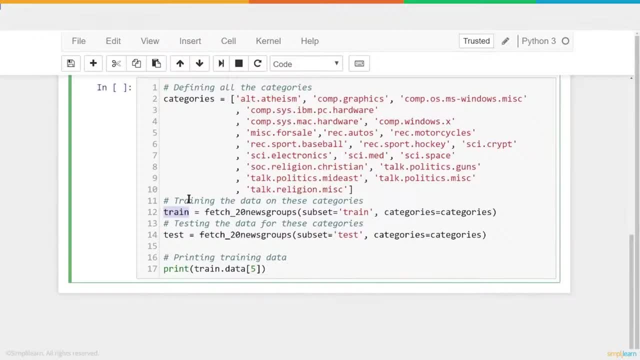 when we print out one part of that data. So it creates train and under train it creates traindata. and we're just going to look at data piece number five And let's go ahead and run that and see what that looks like. And you can see when I print traindata. 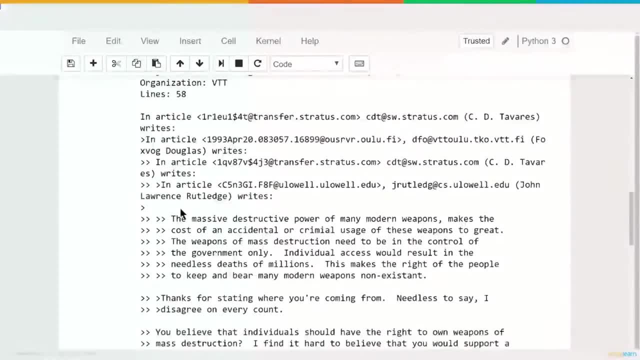 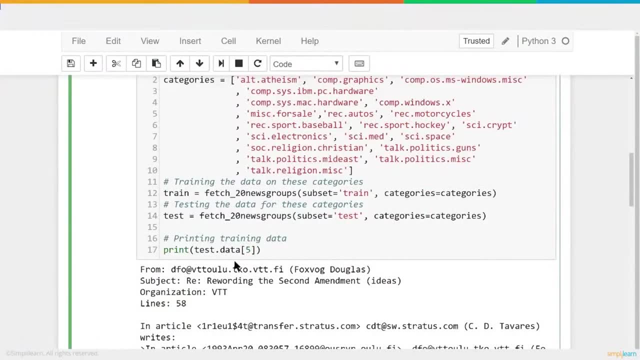 number five. under train it prints out one of the articles. This is article number five. You can go through and read it on there And we can also go in here and change this to test, which should look identical because it's splitting the data up into different groups. 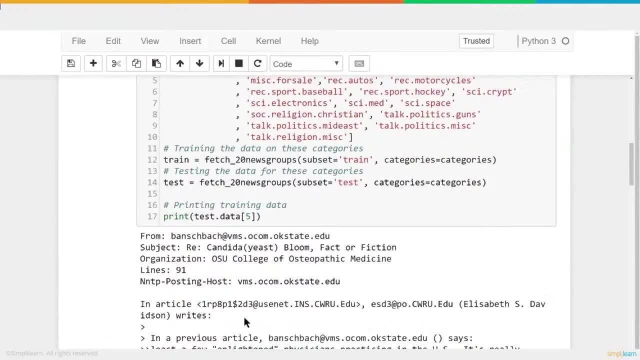 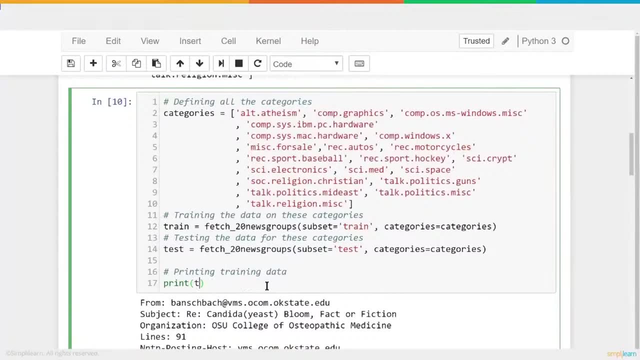 Train and test And we'll see. test number five is a different article but it's another article in here And maybe you're curious and you want to see just how many articles are in here. We could do links of traindata and if we run that, 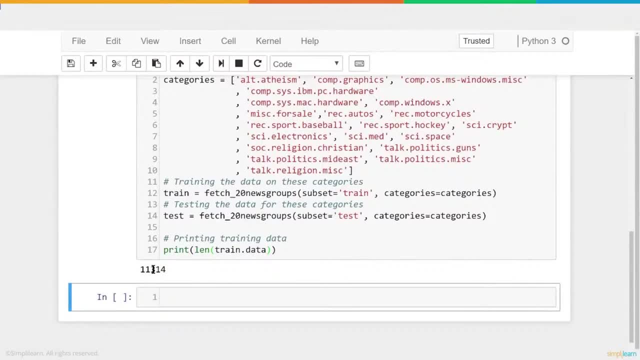 you'll see that the training data has 11,314 articles, So we're not going to go through all those articles. That's a lot of articles, But we can look at one of them just so you can see what kind of information is coming out of it and what we're looking at, And we'll 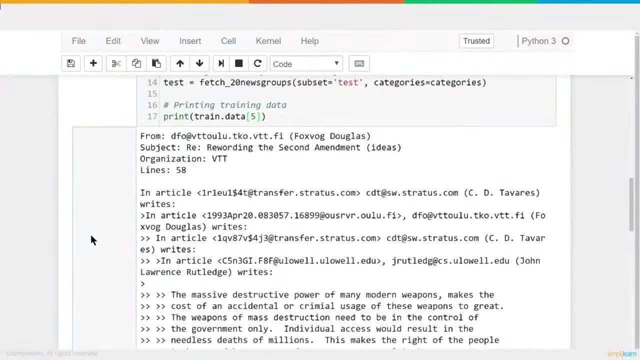 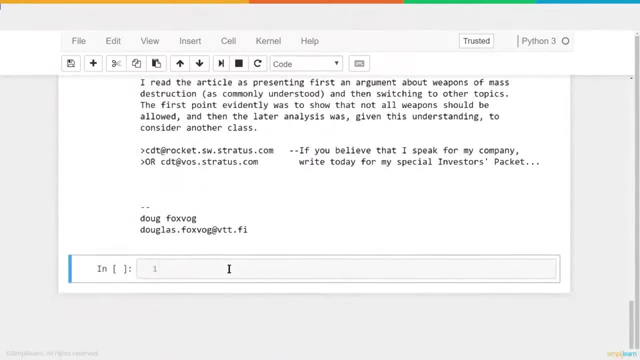 just look at number five for today And here we have it, Rewording the second amendment, IDs VTT, line 58, lines 58 in article, etc. And you can scroll all the way down and see all the different parts to there. Now we've looked at it and that's pretty complicated. 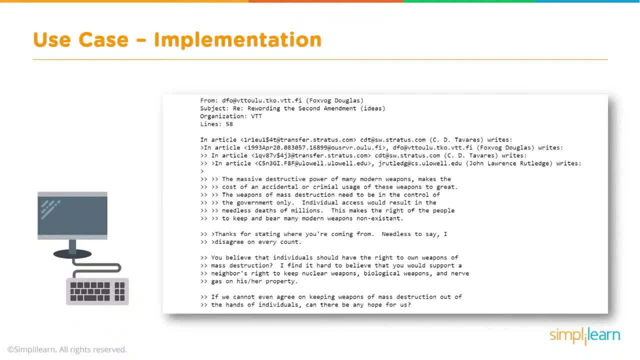 when you look at one of these articles to try to figure out, how do you weight this. If you look down here, we have different words and maybe the word from, Well from- is probably in all the articles, so it's not going to have a lot of meaning as far. 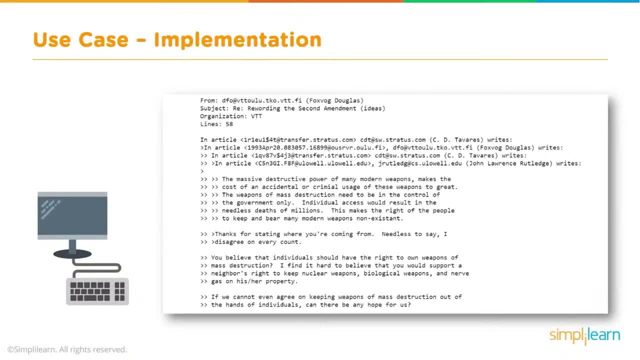 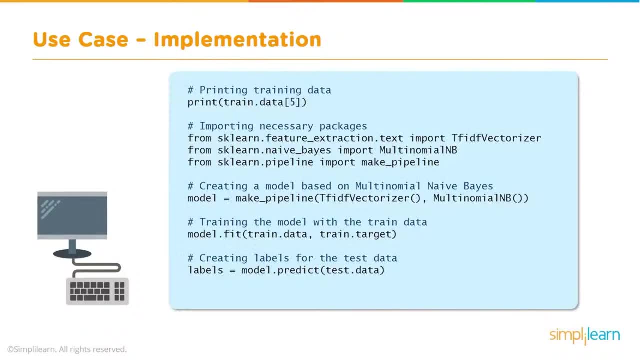 as trying to figure out whether this article fits one of the categories or not. So trying to figure out which category it fits in based on these words is where the challenge comes in. Now that we've viewed our data, we're going to dive in and do the actual. 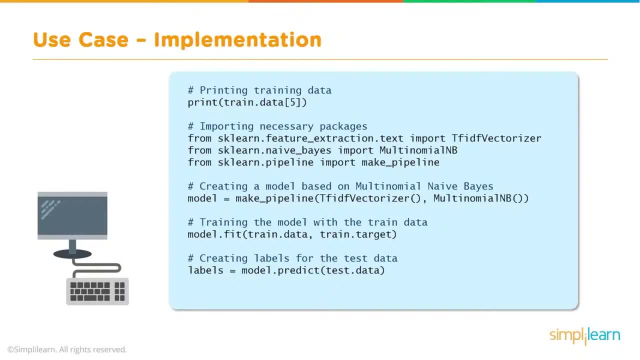 predictions. This is the actual naive base And we're going to throw another model at you or another module at you here in just a second. We can't go into too much detail, but it deals specifically working with words and text and what they call tokenizing those words. 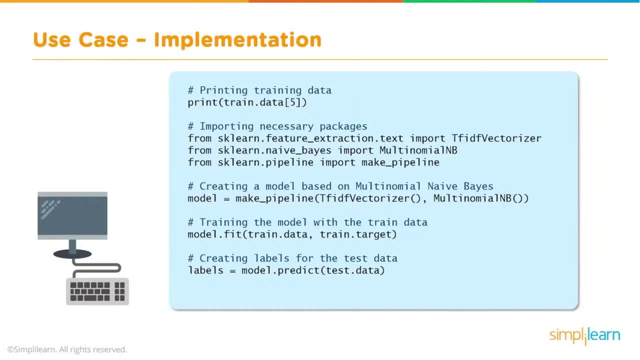 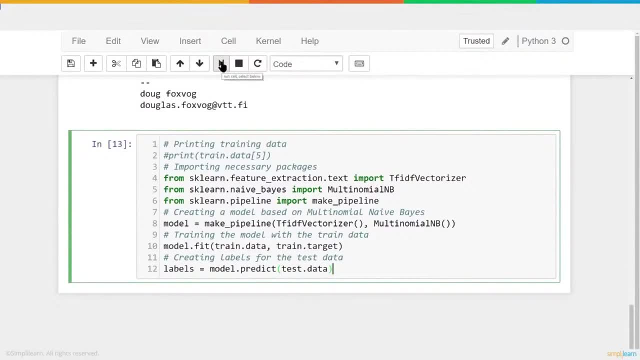 So let's take this code and let's skip on over to our Jupyter notebook and walk through it And here we are in our Jupyter notebook. Let's paste that in there And I can run this code right off the bat. It's not actually going to display. 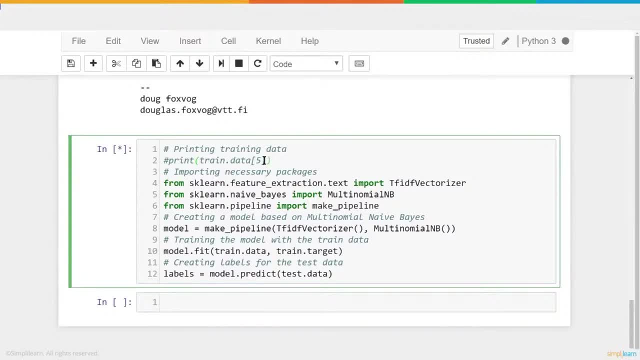 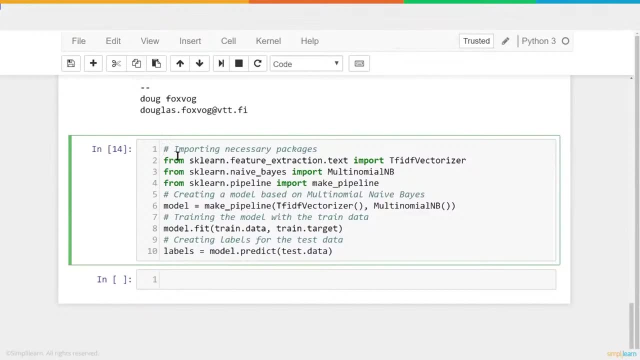 anything yet, But it has a lot going on in here. So at the top we have the print module from the earlier one. I didn't know why that was in there. So let's start by importing our necessary packages And from the sklearnfeaturesextractiontxt. 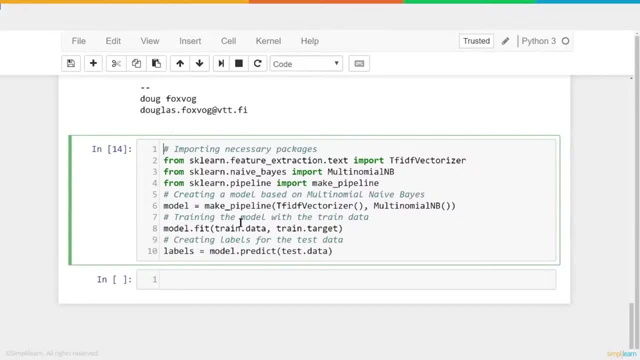 we're going to import tfidfvectorizer. I told you we're going to throw a module at you. We can't go too much into the math behind this or how it works. You can look it up. The notation for the math is usually tfidf. 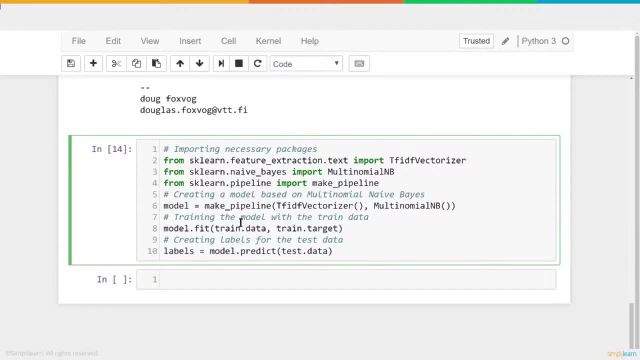 And that's just a way of weighing the words, And it weighs the words based on how many times they're used in a document, how many times or how many documents they're used in, And it's a well-used formula. It's been around for a while. It's a little. 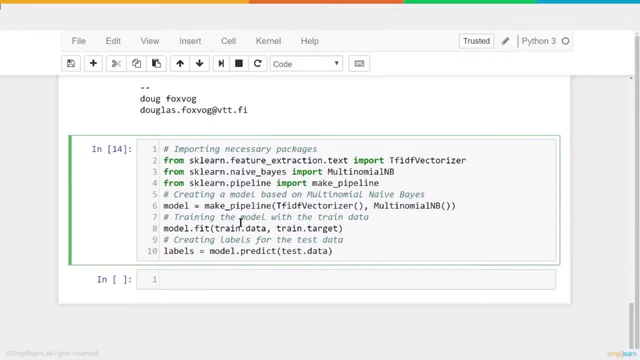 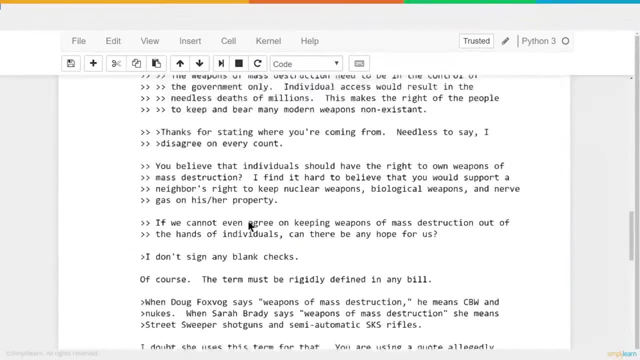 confusing to put this in here, But let's let her know that it just goes in there and weights the different words in the document for us. That way we don't have to wait And if you put a weight on it- if you remember, I was talking about that up here earlier. 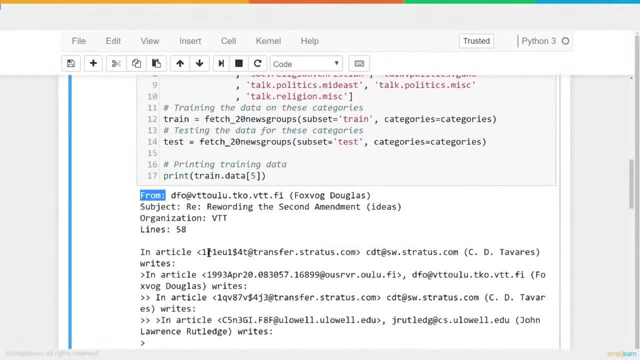 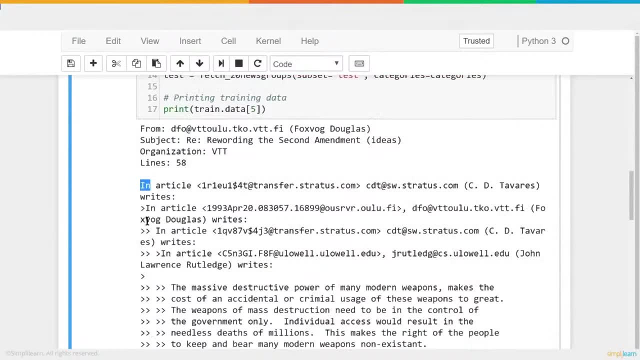 if these are all emails, they probably all have the word from in them. From probably has a very low weight. It has very little value in telling you what this document's about. Same with words like in, in article, in articles, in. 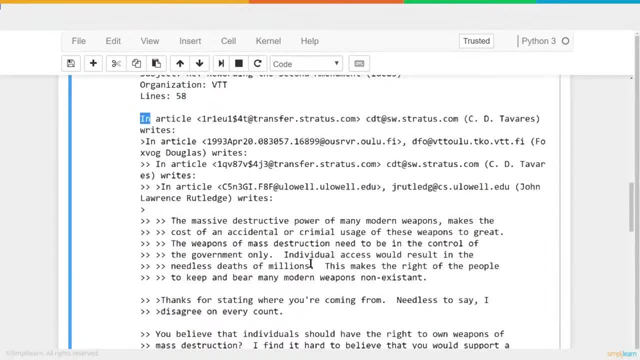 cost of un, maybe cost, might, or where words like criminal weapons, destruction. these might have a heavier weight because they describe a little bit more what the article's doing. Well, how do you figure out all those weights in the different articles? 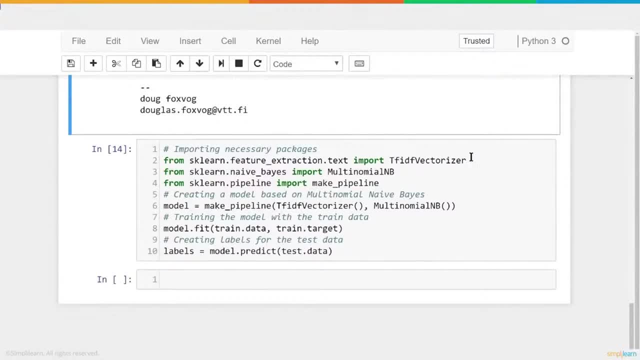 That's what this module does, That's what the TF-IDF vectorizer is going to do for us, And then we're going to import our sklearnnaivebase and that's our multinomial NB, Multinomial naive base. Pretty easy. 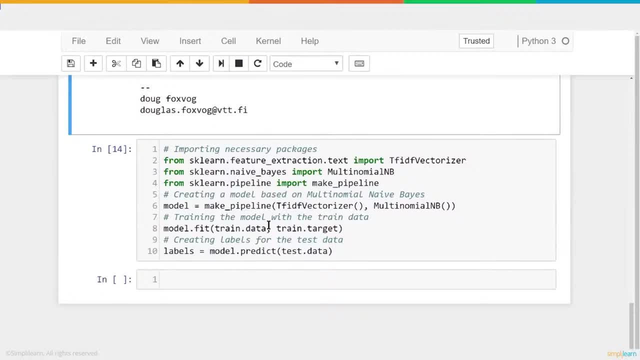 to understand that, where that comes from. And then, finally, we have the sklearn pipeline, import make pipeline. Now, the make pipeline is just a cool piece of code, because we're going to take the information we get from the TF-IDF vectorizer and we're going to pump that. 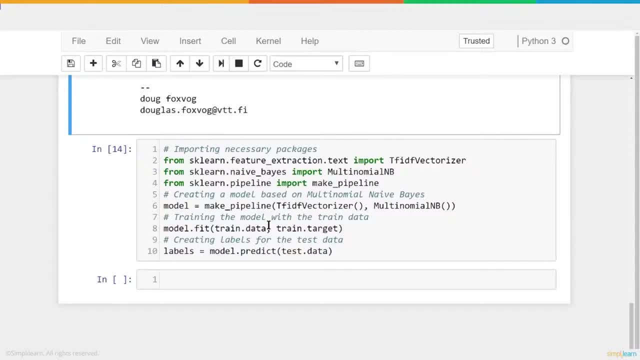 into the multinomial NB. So a pipeline is just a way of organizing how things flow. It's used commonly- you probably already guessed what it is- if you've done any businesses. They talk about the sales pipeline If you're on a work crew or project. 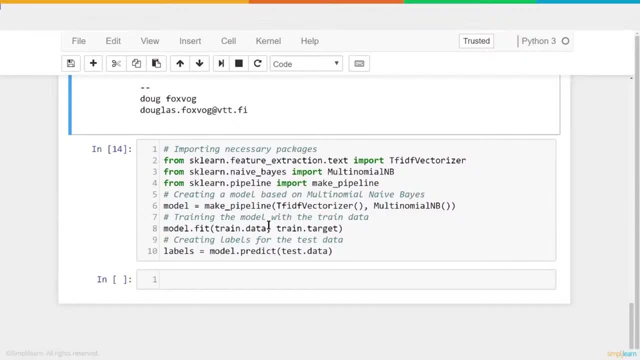 manager, you have your pipeline of information that's going through or your projects and what has to be done, in what order That's all this pipeline is. We're going to take the TF-ID vectorizer and then we're going to push that into the. 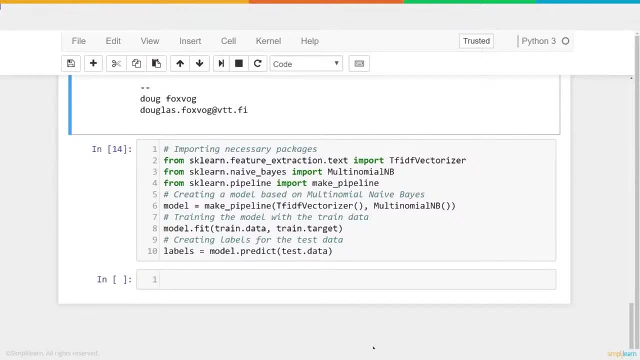 multinomial NB. Now we've designated that as the variable model. We have our pipeline model And we're going to take that model. and this is just so elegant. this is done in just a couple lines of code- Modelfit, and we're going to fit the data. and first, 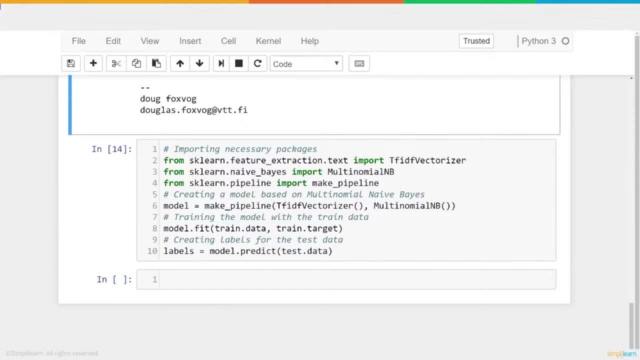 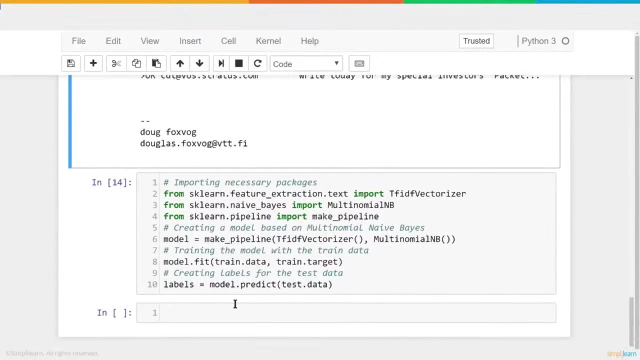 the train data and then the train target. Now the train data has the different articles in it- You can see the one we were just looking at- And the traintarget is what category they already categorized that particular article as, And what's happening here is the train data. 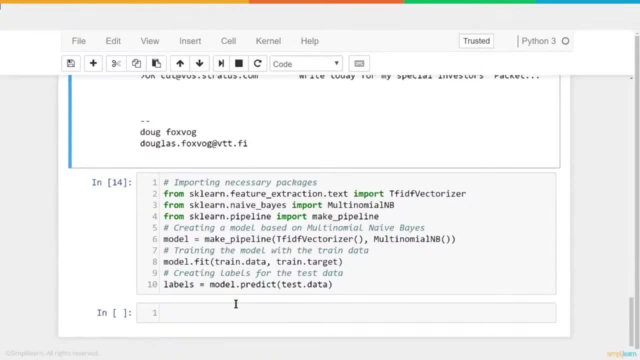 is going into the TF-ID vectorizer. So when you have one of these articles that goes in there, it weights all the words in there. So there's thousands of words with different weights on them. I remember once running a model on this and I literally had 2.4. 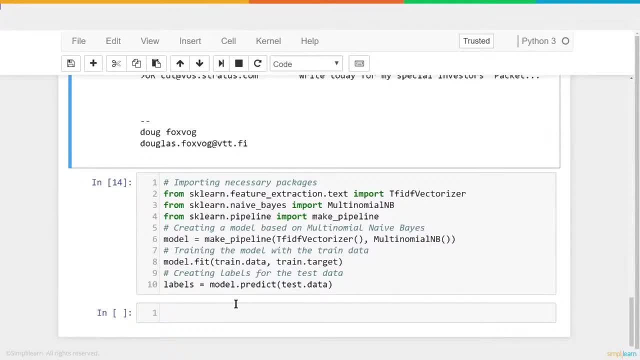 million tokens go into this. So when you're dealing with large document bases, you can have a huge number of different words. It then takes those words, gives them a weight and then based on that weight, based on the words and the weights- and then puts that into the multinomial. 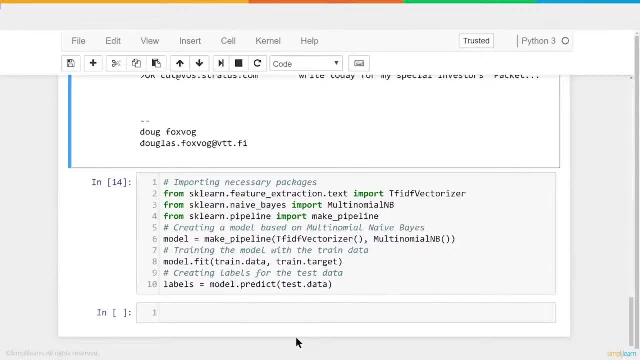 NB, And once we go into our naive base, we want to put the train target in there. So the train data that's been mapped to the TF-ID vectorizer is now going through the multinomial NB, and then we're telling it: well, these are the answers. These are the answers. 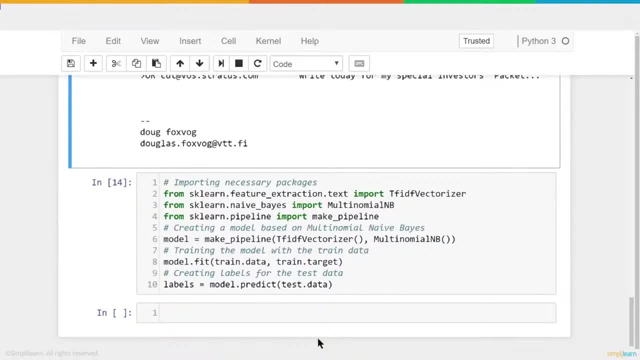 to the different documents. So this document that has all these words, with these different weights from the first part is going to be, whatever category it comes out of- Maybe it's the talk show or the article on religion- miscellaneous. Once we fit that model, we can then take. 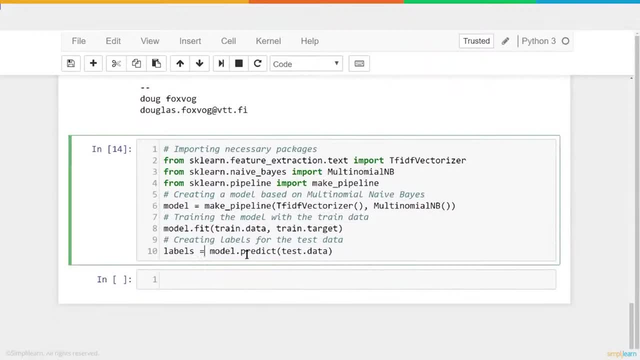 labels and we're going to set that equal to modelpredict. Most of the sklearn use the term predict to let us know that we've now trained the model and now we want to get some answers And we're going to put our test data in there, because 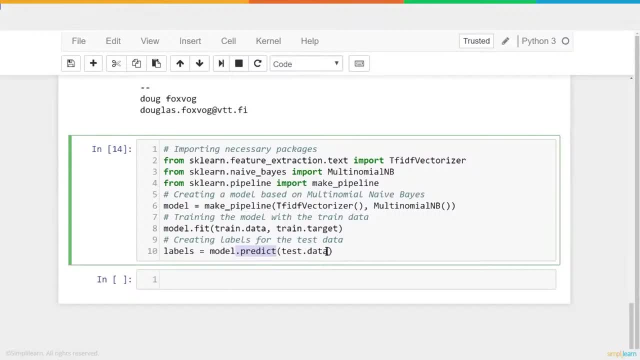 our test data is the stuff we held off to the side. We didn't train it on there and we don't know what's going to come up out of it. and we just want to find out how good our labels are. Do they match what they should be? 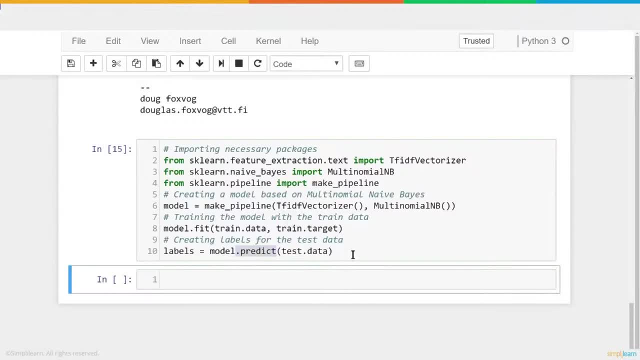 Now, I've already run this through. There's no actual output to it to show. This is just setting it all up. This is just training our model, creating the labels so we can see how good it is, and then we move on to the next step, to find out. 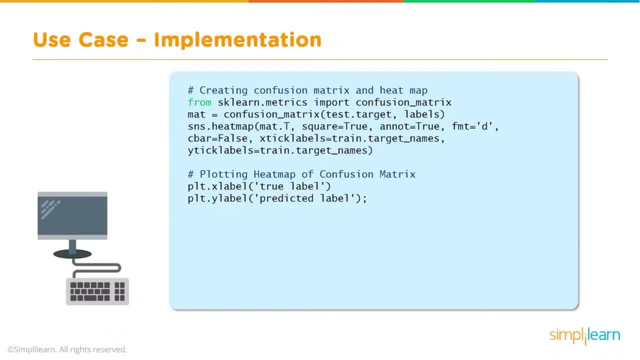 what happened To do this? we're going to go ahead and create a confusion matrix and a heat map. So the confusion matrix, which is confusing just by its very name, is basically going to ask: how confused is our answer? Did it get it correct? 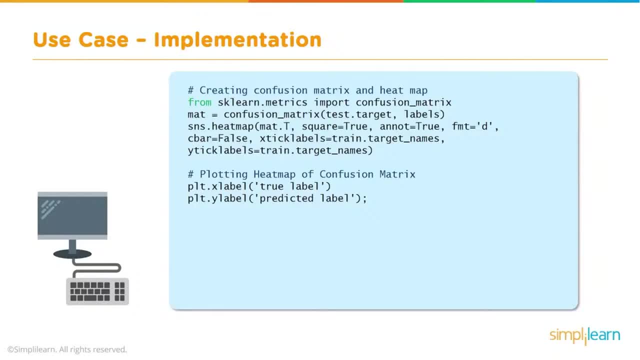 or did it miss some things in there or have some missed labels, And then we're going to put that on a heat map, so we'll have some nice colors to look at to see how that plots out. Let's go ahead and take this code. 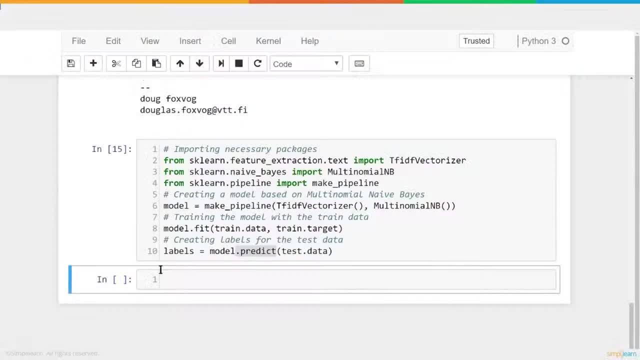 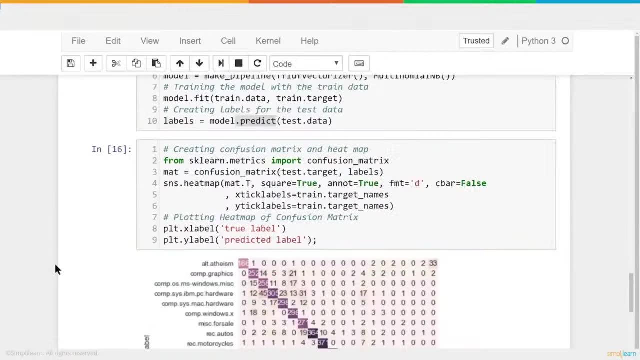 and see how that. take a walk through it and see what that looks like. So back to our Jupyter notebook. I'm going to put the code in there and let's go ahead and run that code. Take it just a moment and remember we had the inline that way, my graph. 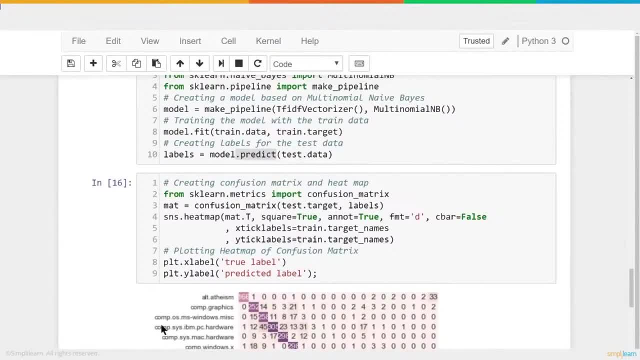 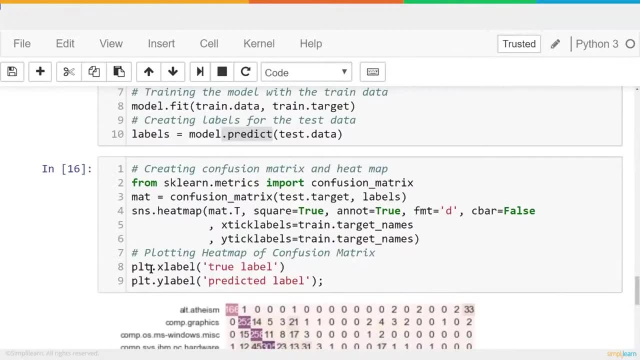 shows up on the inline here And let's walk through the code and then we'll look at this and see what that means. So let me make it a little bit bigger. There we go. No reason not to use the whole screen Too big. So we have here. 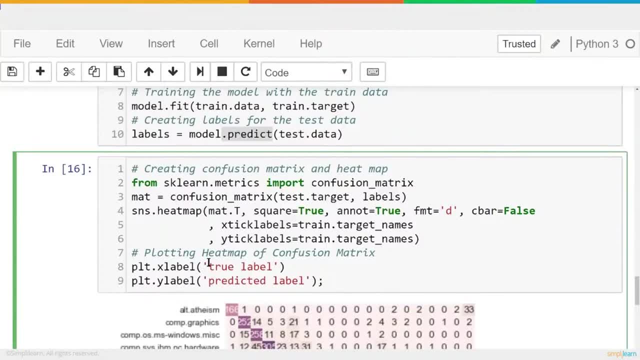 from sklearnmetrics import confusion matrix, And that's just going to generate a set of data that says the prediction was such the actual truth was either agreed with it or something different- And it's going to add up those numbers so we can take a look and 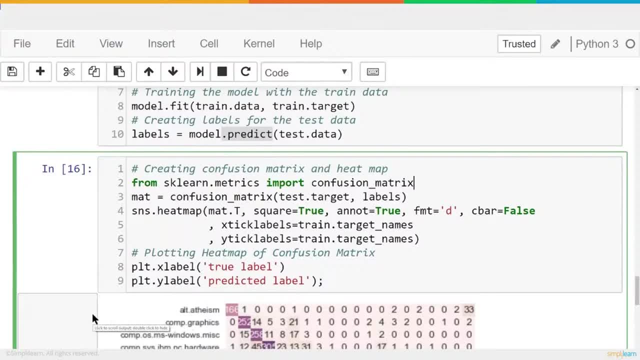 see how well it worked And we're going to set a variable mat equal to confusion matrix. We have our test target, our test data. that was not part of the training- Very important in data science. we always keep our test data separate. 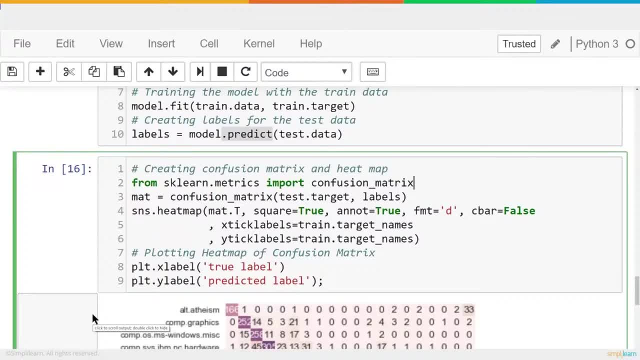 Otherwise it's not a valid model if we can't properly test it with new data. And this is the labels we created from that test data. These are the ones that we predict it's going to be. So we go in and we create our sn-heatmap. 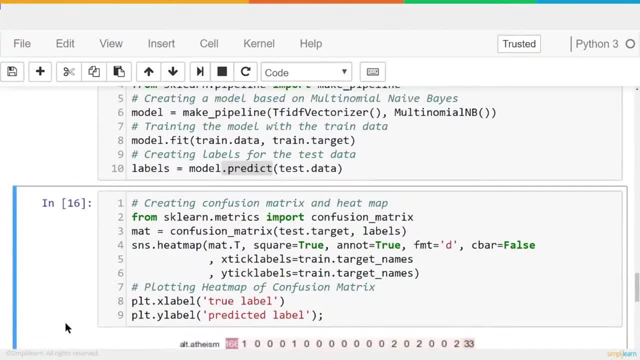 The sns is our seaborn, which sits on top of the pi plot. So when we create a snsheatmap we take our confusion matrix and it's going to be matt, and then we have other variables that go into the snsheatmap. We're not going to go into detail. 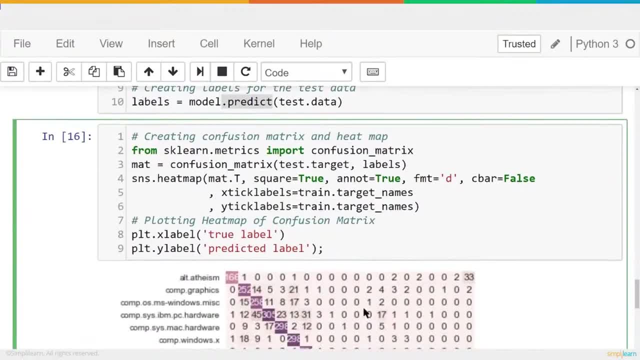 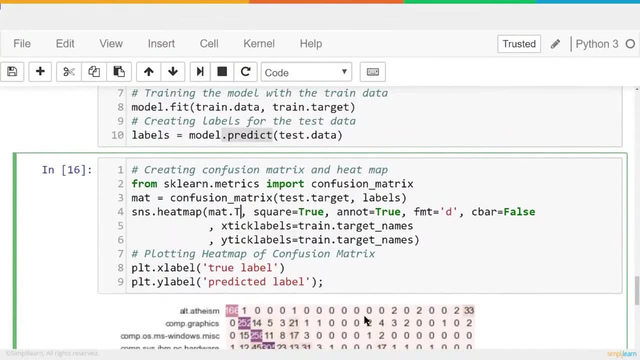 what all the variables mean. The annotation equals true. that's what tells it to put the numbers here. So you have the 166, the 1, the 0001 format. d and cbar equals false. have to do with the format. If you take those out, you'll 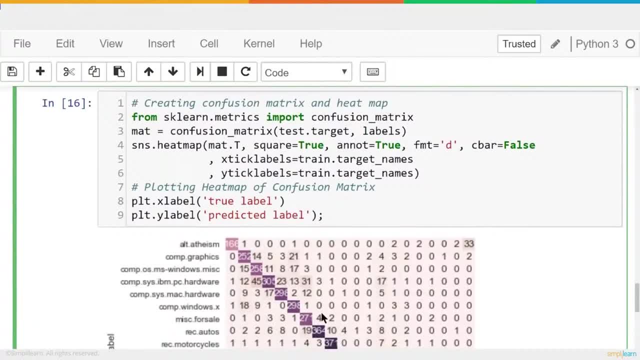 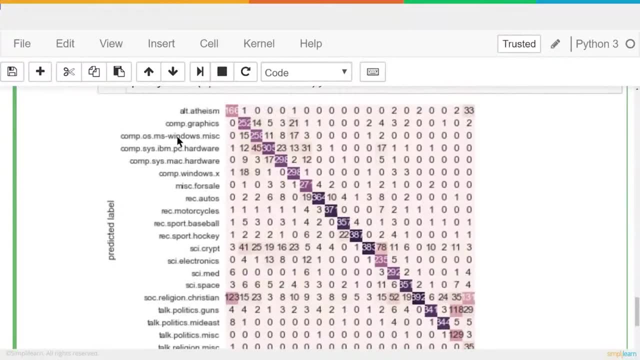 see that some things disappear. And then the s tick labels and the y tick labels. those are our target names And you can see right here: that's the alt atheism, comp, graphics, comp, os, ms, windows, dot, miscellaneous. And then finally we have our plt dot x label. 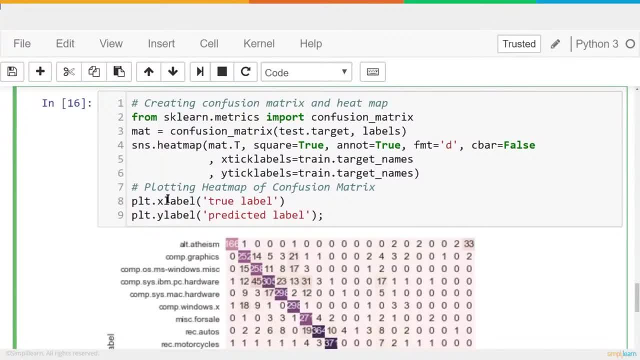 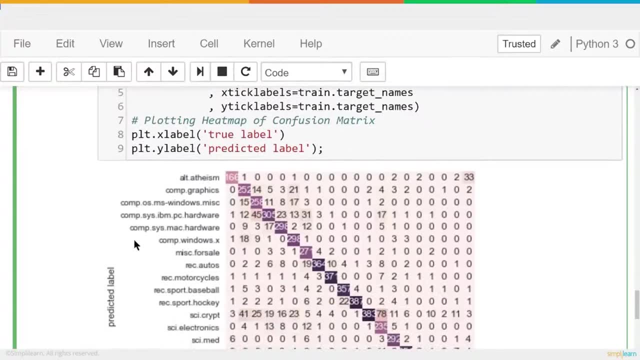 remember the sns or the seaborn sits on top of our matplot library, our plt, And so we want to just tell it: x label equals a, true is true, The labels are true, and then the y label is prediction label. So when we say a 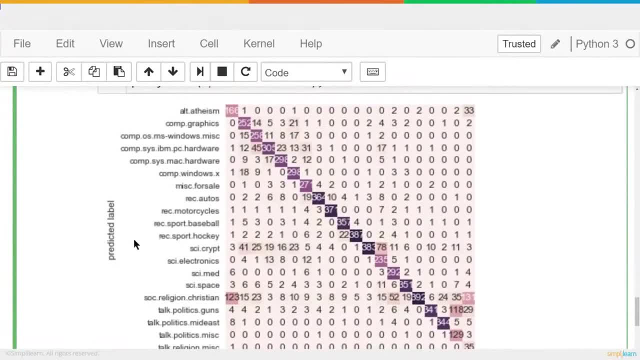 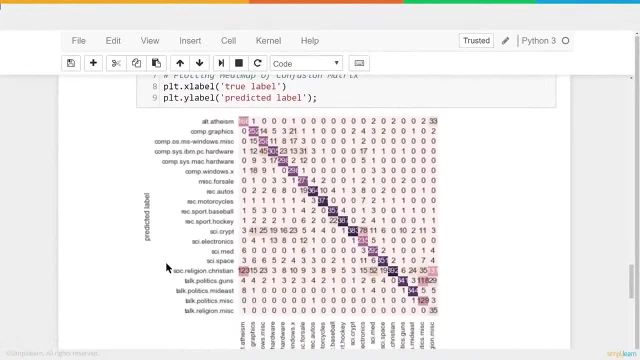 true, this is what it actually is, and the prediction is what we predicted. And let's look at this graph, because that's probably a little confusing the way we rattled through it, And what I'm going to do is I'm going to go ahead and flip back to 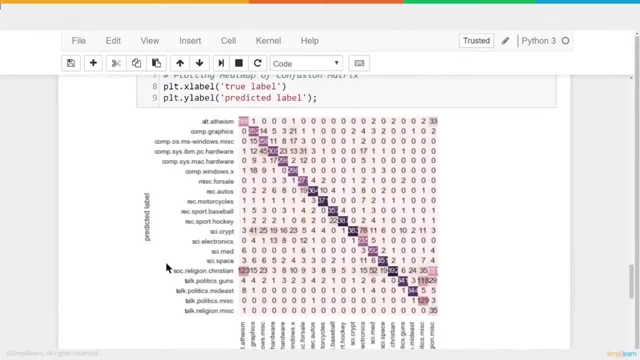 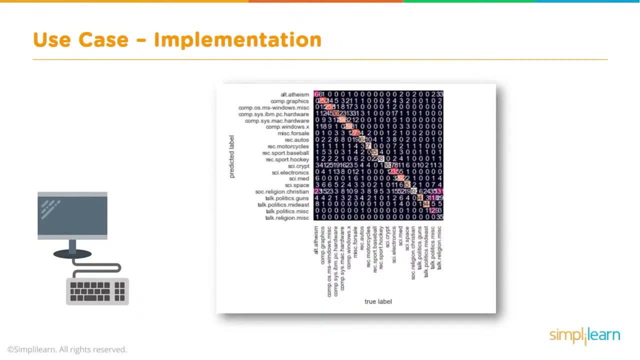 the slides because they have a black background they put in there. that helps it shine a little bit better so you can see the graph a little bit easier. So in reading this graph, what we want to look at is how the color scheme has come out. 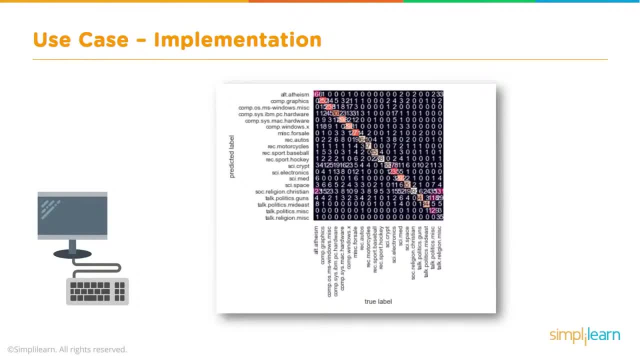 And you'll see a line right down the middle, diagonally from upper left to bottom right. What that is is, if you look at the labels, we have our predicted label on the left and our true label on the right. Those are the numbers where the prediction 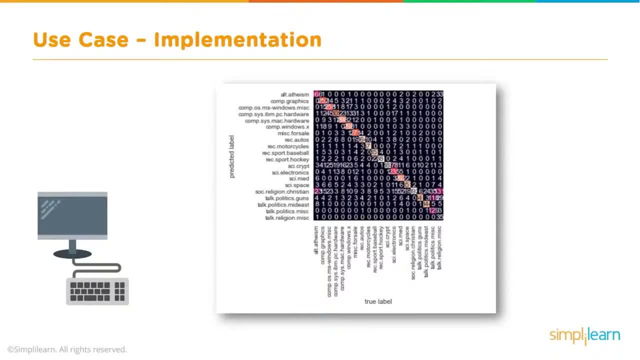 and the true come together, And this is what we want to see is we want to see those lit up. That's what that heat map does, As you can see that it did a good job of finding those data, And you'll notice that. 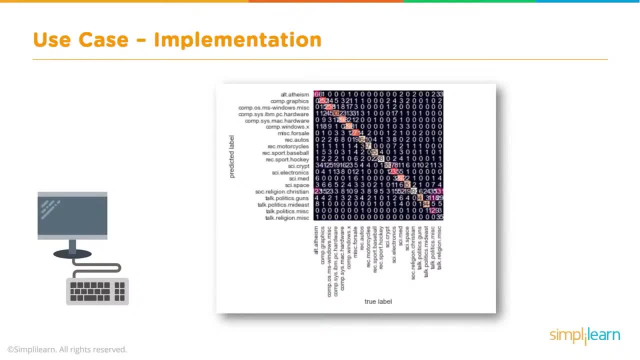 there's a couple of red spots on there where it missed. You know it's a little confused when we talk about talk religion, miscellaneous versus talk politics, miscellaneous social religion, Christian versus alt atheism. It mislabeled some of those And those are very similar topics. 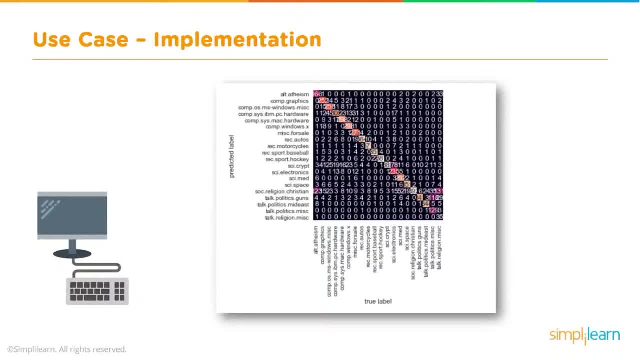 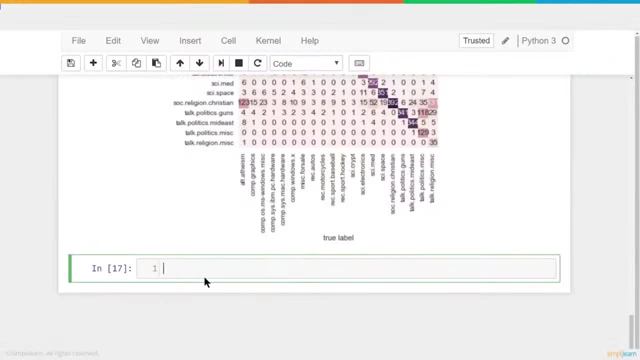 so you could understand why it might mislabel them, But overall it did a pretty good job. If we're going to create these models, we want to go ahead and be able to use them, So let's see what that looks like To do this. let's go ahead and create. 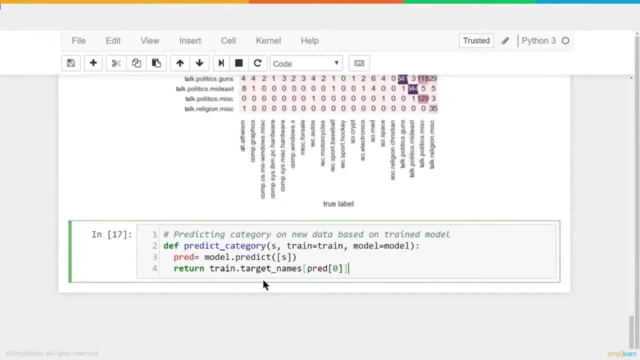 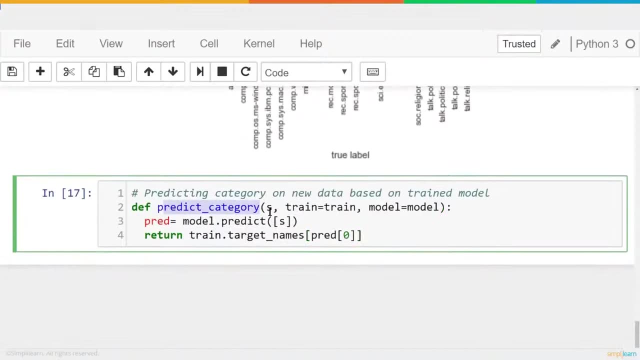 a definition, a function to run, And we're going to call this function. let me just expand that just a notch here. There we go. I like mine in big letters: Predict categories. We want to predict the category We're going to send it. 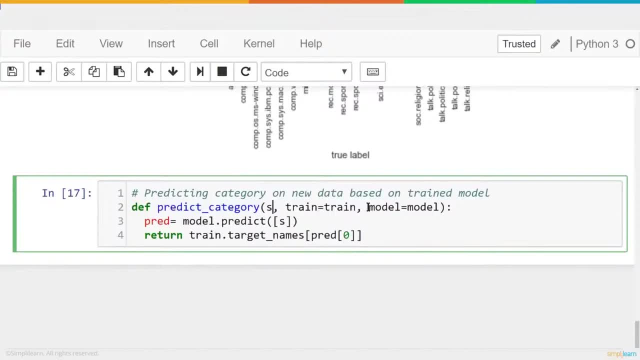 s a string and then we're sending it train equals train. we have our training model and then we have our pipeline Model equals model. This way we don't have to resend these variables each time. The definition knows that. because I said train equals train. 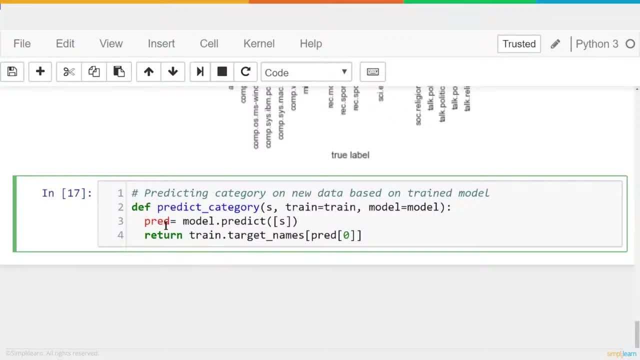 and I put the equal for model And then we're going to set the prediction equal to the model dot predict s. So it's going to send whatever string we send to it. It's going to push that string through the pipeline, the model pipeline. 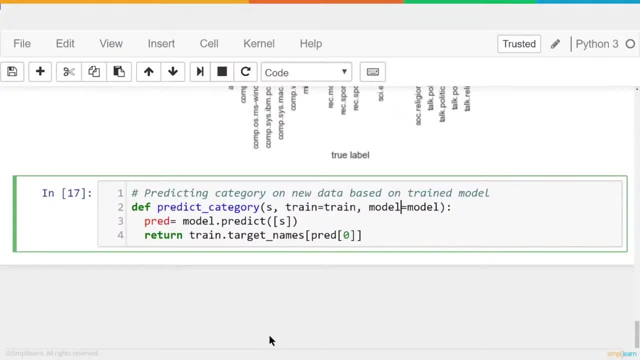 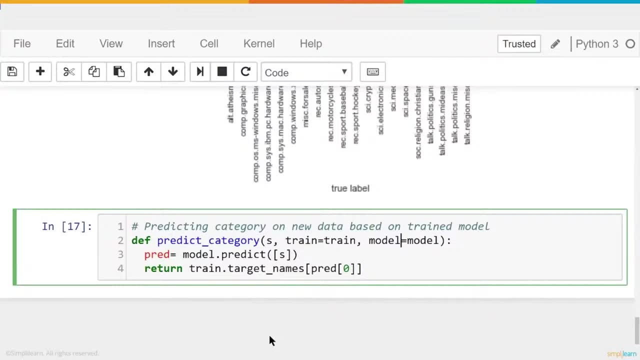 It's going to go through and tokenize it and put it through the tf, idf, convert that into numbers and weights for all the different documents and words, and then it'll put that through our naive bays And from it we'll go ahead and get our 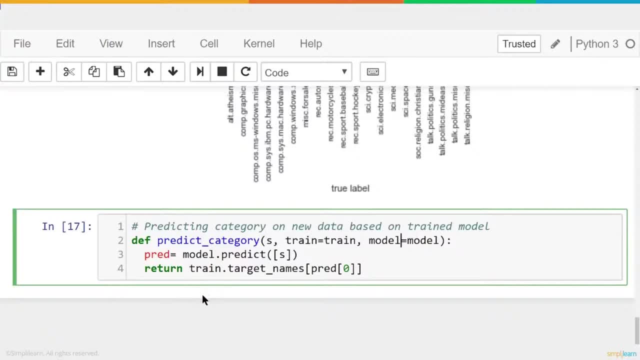 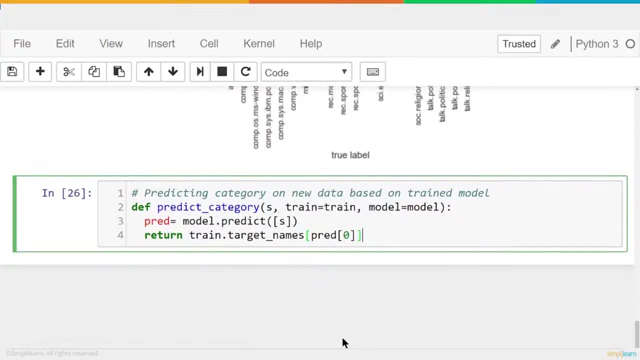 prediction. We're going to predict what value it is, And so we're going to return train dot target names- predict of zero. And remember that the train dot target names, that's just categories. I could have just as easily put categories in there. dot- predict of zero. 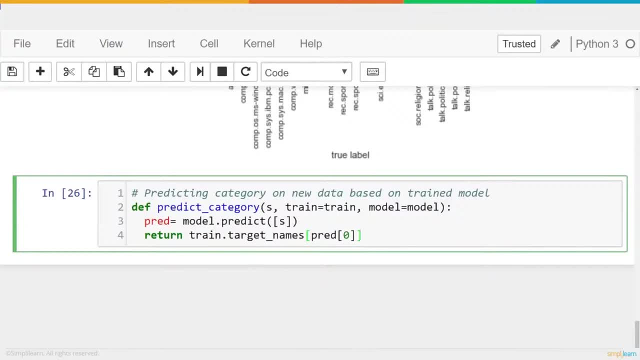 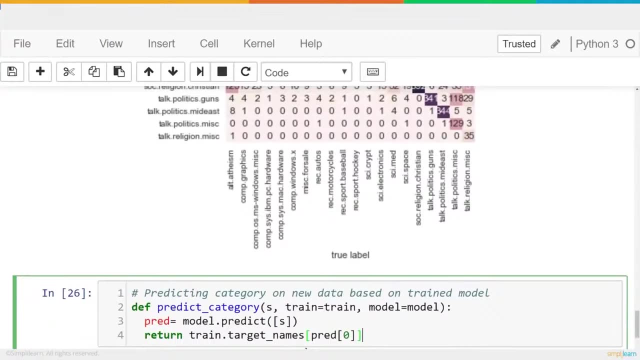 So we're taking the prediction, which is a number, and we're converting it to an actual category. We're converting it from. I don't know what the actual numbers are, but let's say, zero equals alt atheism. So we're going to convert that zero to the word. 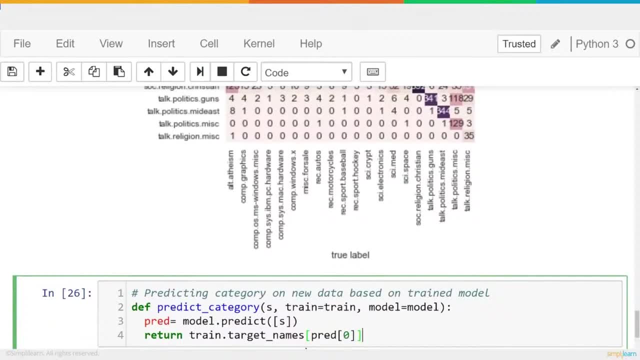 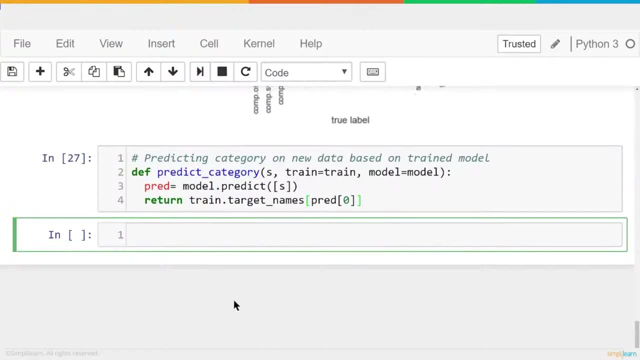 or one. maybe it equals comp graphics. So we're going to convert number one into comp graphics. That's all that is. And then we got to go ahead and and then we need to go ahead and run this, So I load that up and then, once I run that, 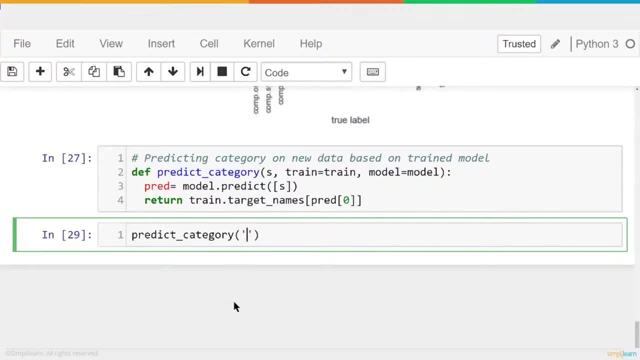 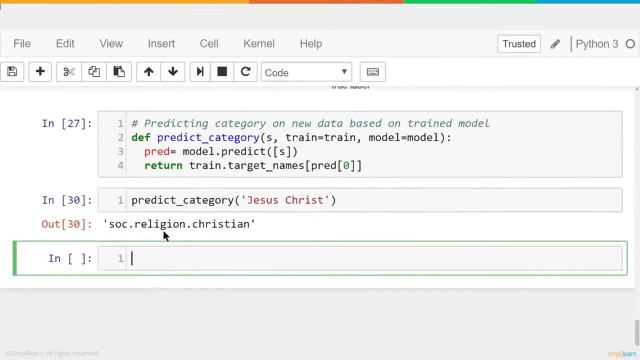 we can start doing some predictions. I'm going to go ahead and type in predict category and let's just do predict category Jesus Christ And it comes back and says it's social religion Christian. That's pretty good. Now note: I didn't put print on this. 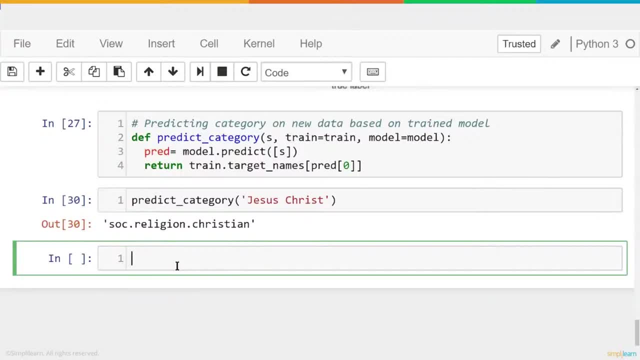 One of the nice things about the Jupiter notebook editor and a lot of inline editors is if you just put the name of the variable out as returning the variable train dot target underscore names, it'll automatically print that for you In your own ID you might have to put: 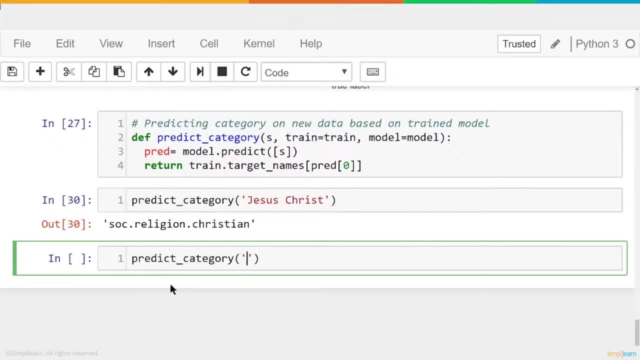 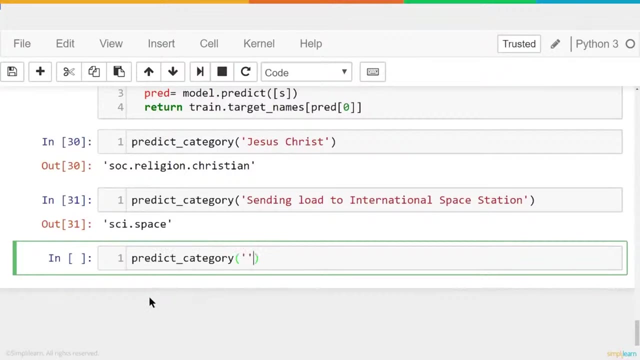 in print. Let's see where else we can take this. And maybe you're a space science buff, So how about sending load to international space station? And if we run that, we get science space. Or maybe you're a automobile buff And let's do. 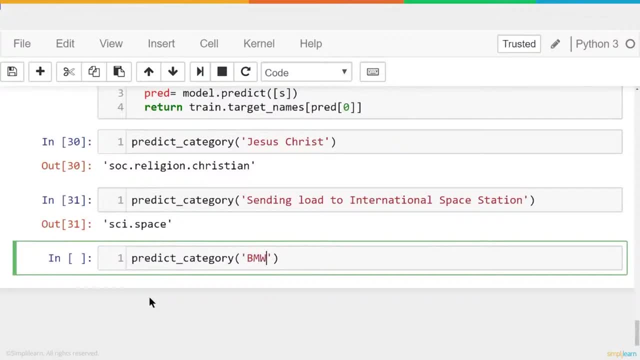 they were going to tell me Audi is better than BMW. but I'm going to do: BMW is better than an Audi. So maybe you're a car buff And we run that and you'll see. it says recreational. I'm assuming that's what REC. 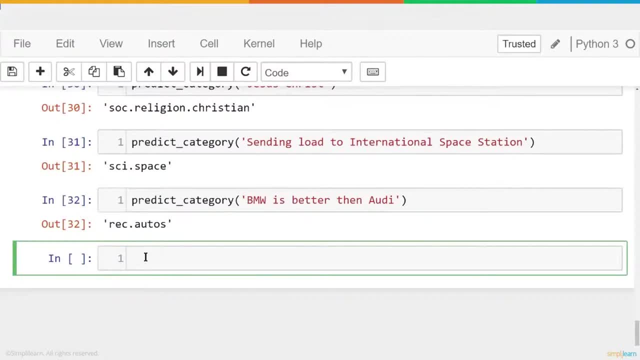 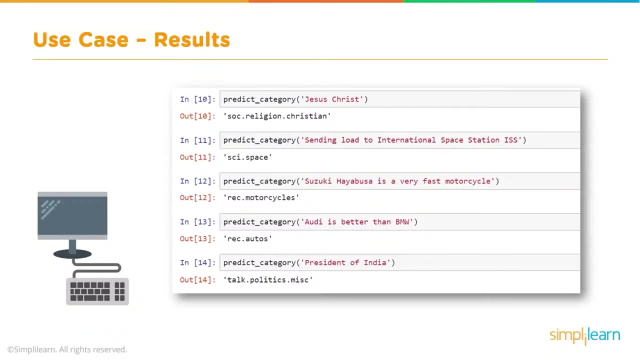 stands for Autos, So I did a pretty good job labeling that one. How about if we have something like the caption running through there, President of India. And if we run that it comes up and says: talk politics miscellaneous. So when we take our definition or our function, 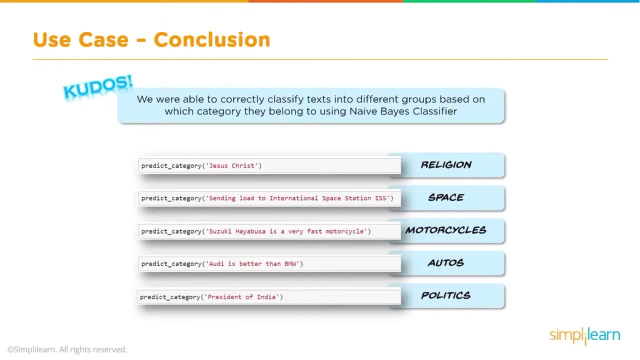 and we run all these things through kudos. we made it. We were able to correctly classify text into different groups, based on which category they belong to, using the naive base classifier. Now we did throw in the pipeline the TF idea vectorizer. we threw in the graphs. Those are 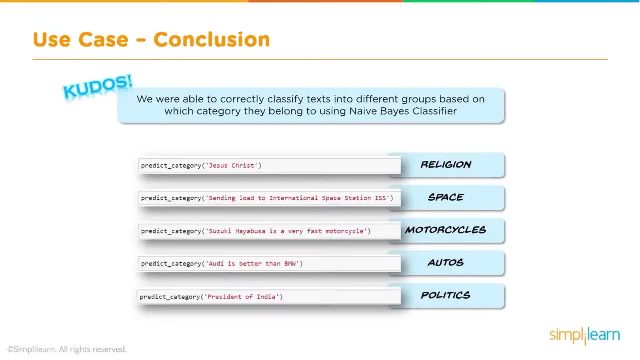 all things that you don't necessarily have to know to understand the naive base setup or classifier, But they're important to know. One of the main uses for the naive base is with the TF, IDF tokenizer or vectorizer, where it tokenizes a word and has labels And 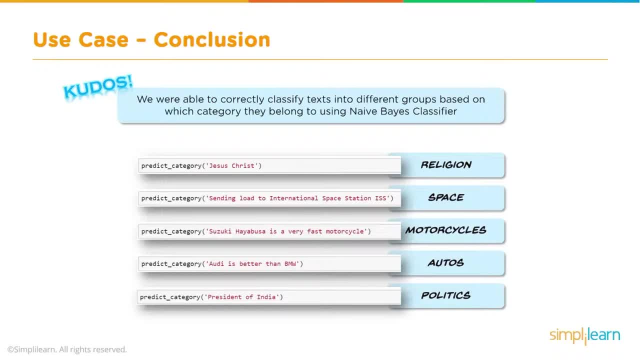 we use the pipeline because you need to push all that data through and it makes it really easy and fast. You don't have to know those to understand naive base, but they certainly help for understanding the industry and data science And we can see our categorizer. 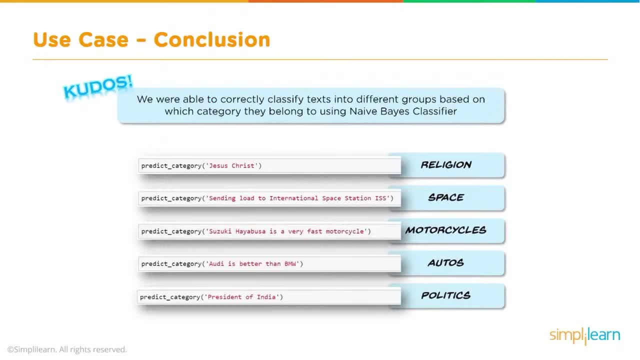 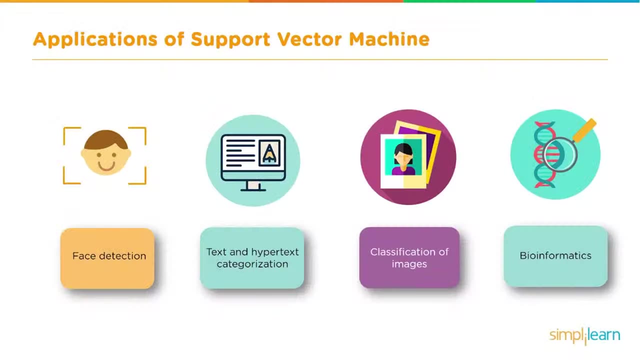 or naive base classifier. We were able to predict the category- religion, space, motorcycles, autos, politics- and properly classify all these different things. we pushed into our prediction and our trained model. Before we dive into the SVM, let's take a look at applications of the support vector. 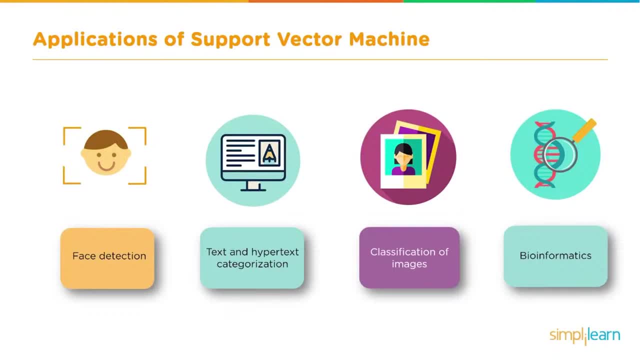 machine, At least some general ones that are commonly used with it: Face detection, text and hypertext categorization, classification of images and bioinformatics. These are only but a few of those that are used with this SVM. As we go through this lesson, see if 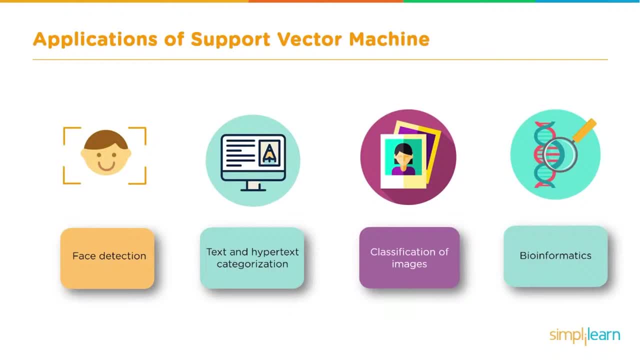 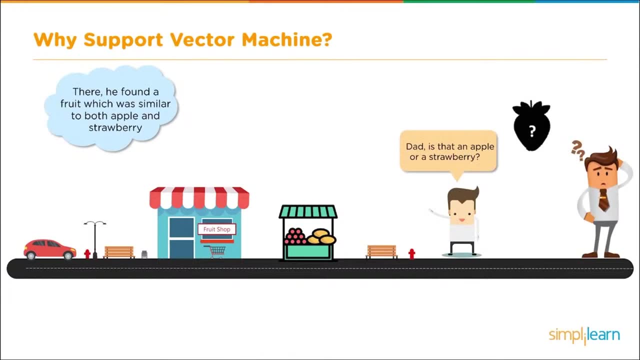 you can figure out what other ones you can apply it to, and also what you would want to use some other tools for. So in this example, last week my son and I visited a fruit shop. Dad, is that an apple or a strawberry? So the question comes up: 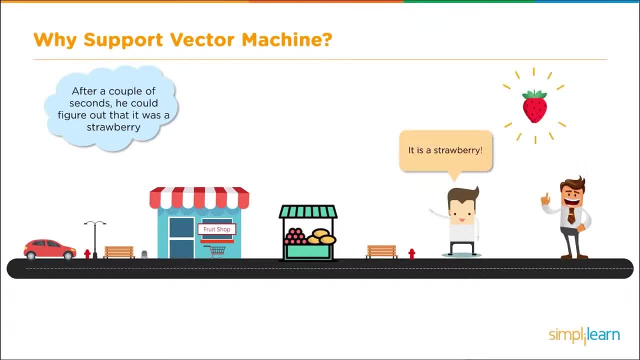 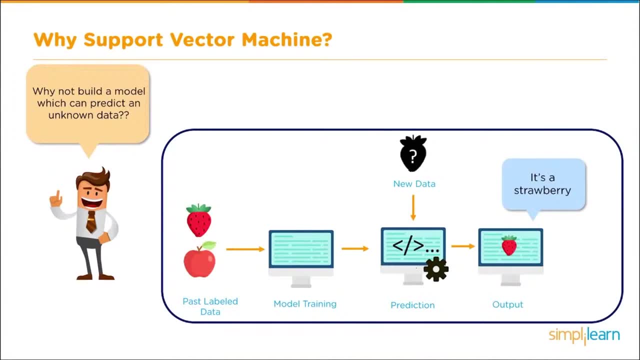 what fruit did I just pick up from the fruit stand? After a couple of seconds, you can figure out that it was a strawberry. So let's take this model a step further and let's- why not? build a model which can predict an unknown data. 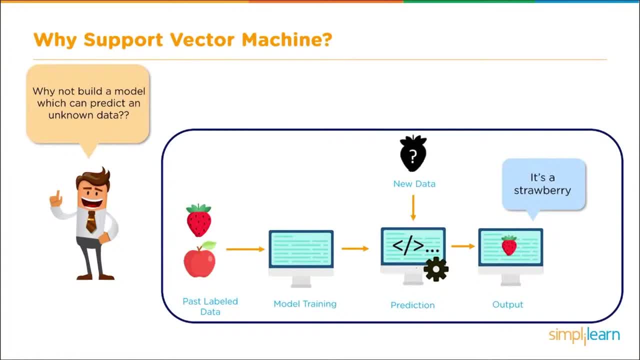 And in this we're going to be looking at some sweet strawberries or crispy apples. We want it to be able to label those two and decide what the fruit is, And we do that by having data already put in. So we already have a bunch of strawberries. 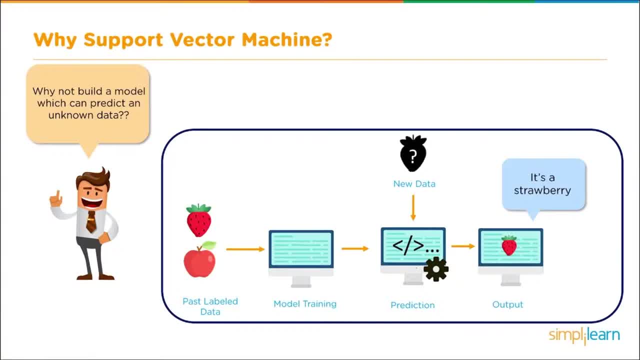 we know are strawberries and they're already labeled as such. We already have a bunch of apples we know are apples and are labeled as such. Then, once we train our model, that model then can be given the new data. and the new data is this image: In this case, you can see a 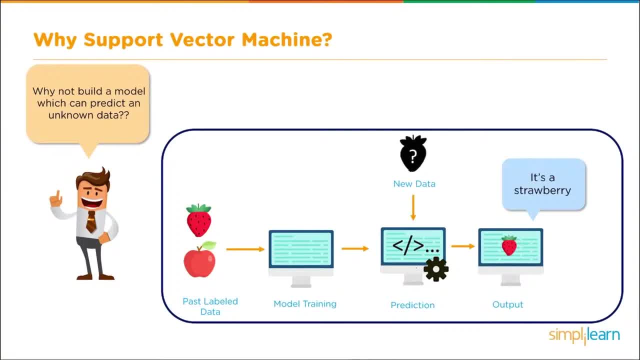 question mark on it and it comes through and goes. it's a strawberry. In this case we're using the support vector machine model. SVM is a super revised learning method that looks at data and sorts it into one of two categories, And in this case we're sorting the strawberry into. 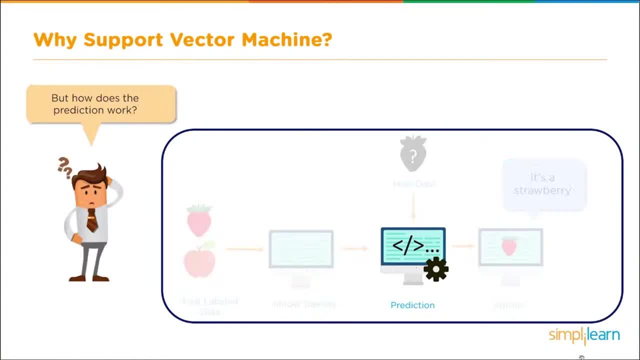 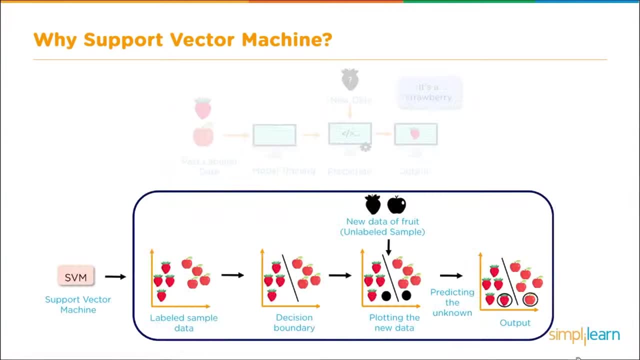 the strawberry side. At this point you should be asking the question: how does the prediction work? Before we dig into an example with numbers, let's apply this to our fruit scenario. We have our support vector machine, We've taken it and we've taken labeled. 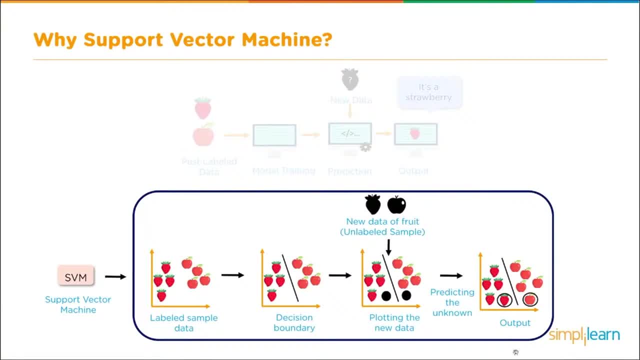 sample of data- strawberries and apples- and we've drawn a line down the middle between the two groups. This split now allows us to take new data, in this case an apple and a strawberry, and place them in the appropriate group based on which side of the line. 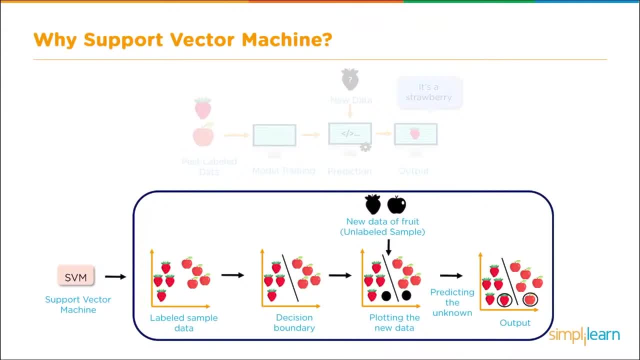 they fall in, And that way we can predict the unknown. As colorful and tasty as the fruit example is, let's take a look at another example with some numbers involved, And we can take a closer look at how the math works In this example. 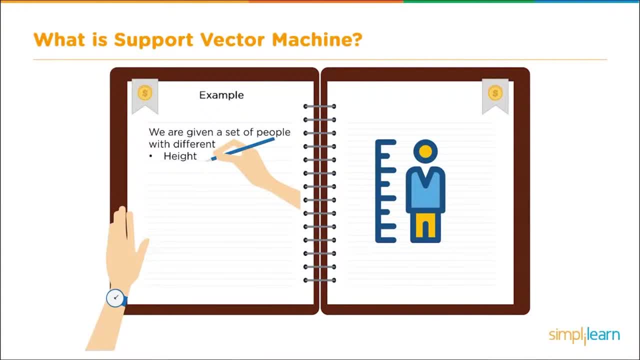 we're going to be classifying men and women And we're going to start with a set of people with a different height and a different weight, And to make this work, we'll have to have a sample data set of female, where you have their height. 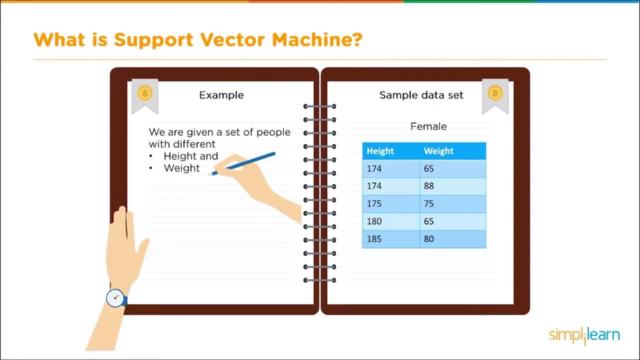 and weight: 174,, 65,, 174,, 88, and so on, And we'll need a sample data set of the male. They have a height 179,, 90,, 180, to 80, and so on. Let's go ahead. 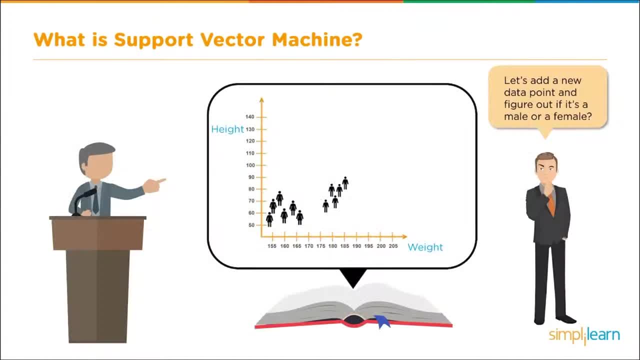 and put this on a graph so we have a nice visual. So you can see, here we have two groups based on the height versus the weight, And on the left side we're going to have the women, on the right side we're going to have the men. Now, if we're going to create a 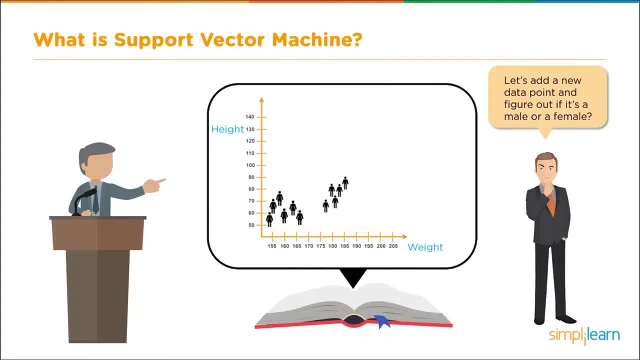 classifier, let's add a new data point and figure out if it's male or female. So before we can do that, we need to split our data first. We can split our data by choosing any of these lines. In this case, we've drawn two lines through the data in the 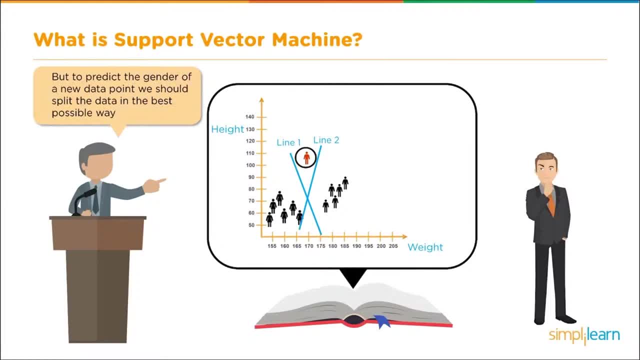 middle that separates the men from the women. But to predict the gender of a new data point, we should split the data in the best possible way. And we say the best possible way because this line has a maximum space that separates the two classes. 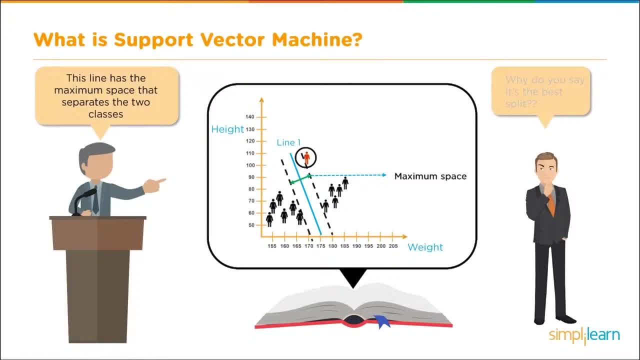 Here you can see there's a clear split between the two different classes, And in this one there's not so much a clear split. This doesn't have the maximum space that separates the two. That is why this line best splits the data. We don't want to just do. 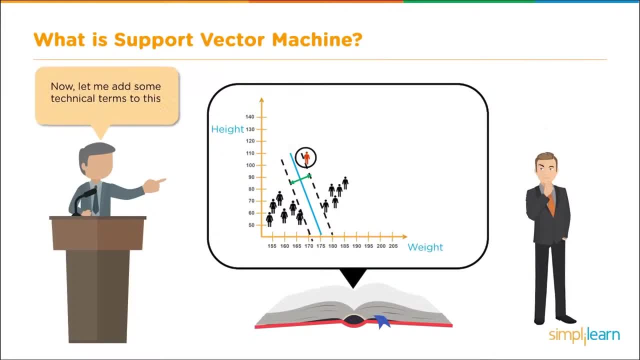 this by eyeballing it, And before we go further, we need to add some technical terms to this. We can also say that the distance between the points in the line should be as far as possible. In technical terms we can say the distance between the support. 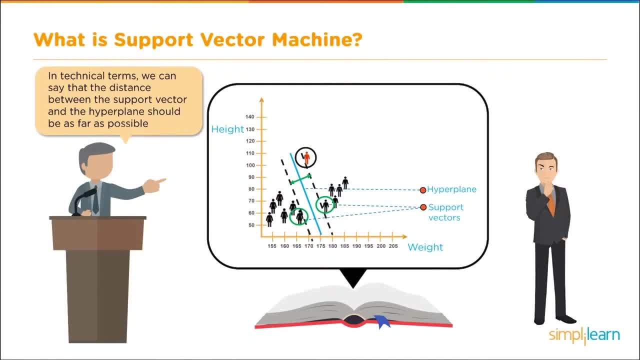 vector and the hyperplane should be as far as possible And this is where the support vectors are the extreme points in the data set. And if you look at this data set, they have circled two points which seem to be right on the outskirts of the women and one on the 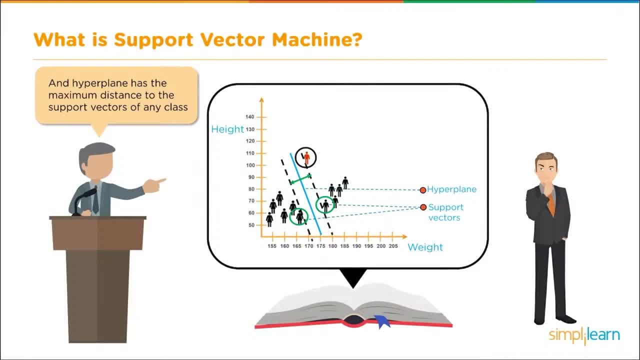 outskirts of the men And hyperplane has a maximum distance to the support vectors of any class. Now you'll see the line down the middle And we call this the hyperplane, because when you're dealing with multiple dimensions, it's really not just a line but a plane of intersections. 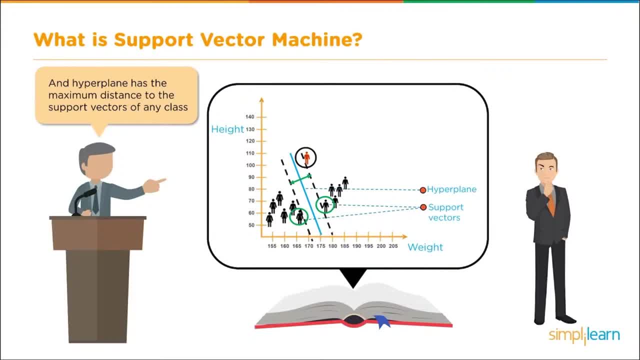 And you can see here where the support vectors have been drawn in dashed lines. The math behind this is very simple. We take D plus, the shortest distance to the closest positive point, which would be on the men's side, and D minus is the shortest distance to the closest negative. 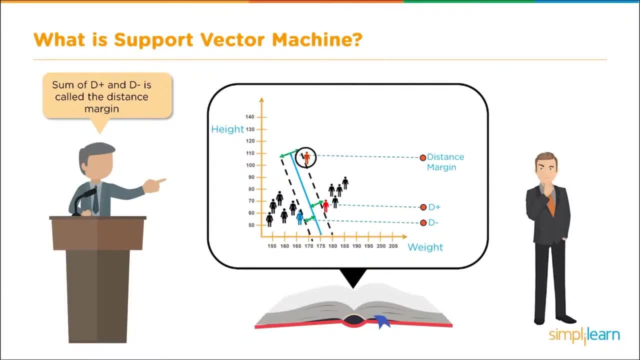 point, which is on the women's side. The sum of D plus and D minus is called the distance margin, or the distance between the two support vectors that are shown in the dashed lines, And then by finding the largest distance margin, we can. 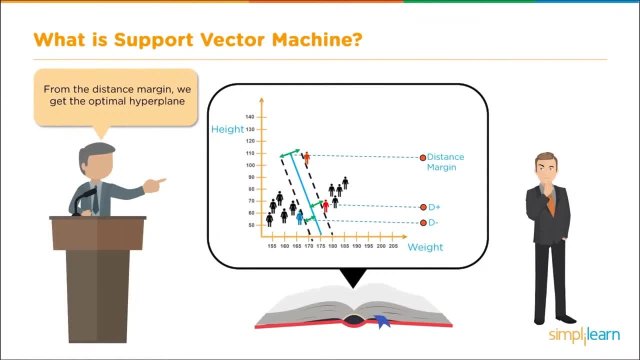 get the optimal hyperplane. Once we've created an optimal hyperplane, we can easily see which side the new data fits in And, based on the hyperplane, we can say the new data point belongs to the male gender. Hopefully that's clear. 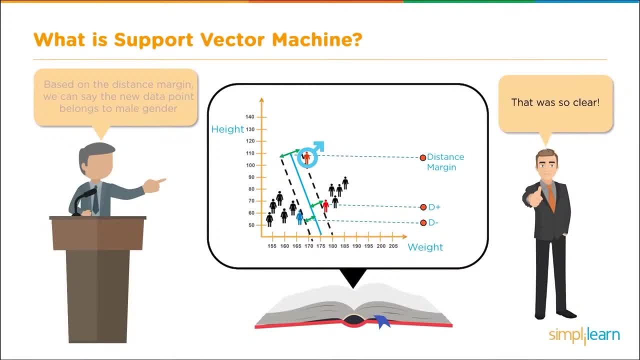 how that works on a visual level. As a data scientist, you should also be asking what happens if the hyperplane is not optimal. If we select a hyperplane having low margin, then there is a high chance of misclassification. This particular SVM. 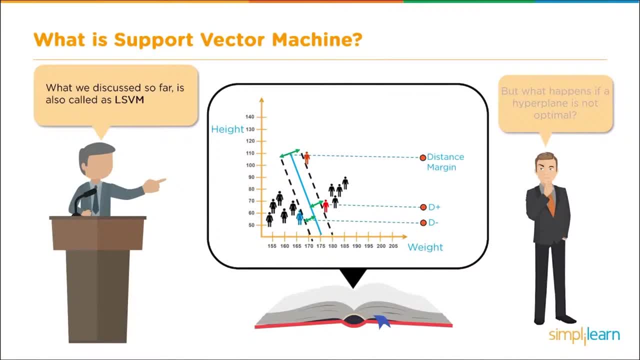 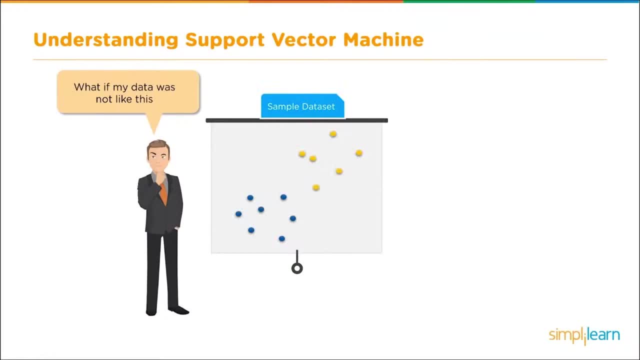 model, the one we discussed so far, is also called or referred to as the LSVM. So far, so clear. but a question should be coming up. We have our sample data set, but instead of looking like this, what if it looked like? 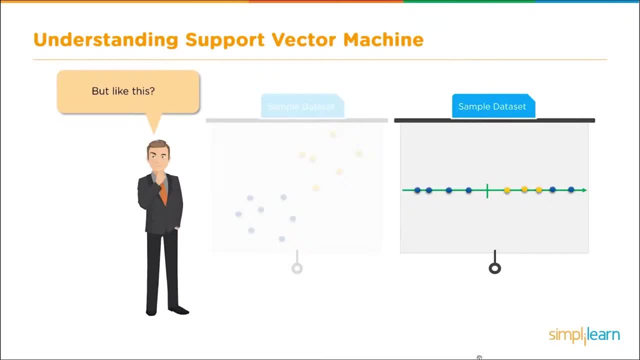 this where we have two sets of data but one of them occurs in the middle of another set. You can see here where we have the blue and the yellow and then blue again on the other side of our data line In this data set. 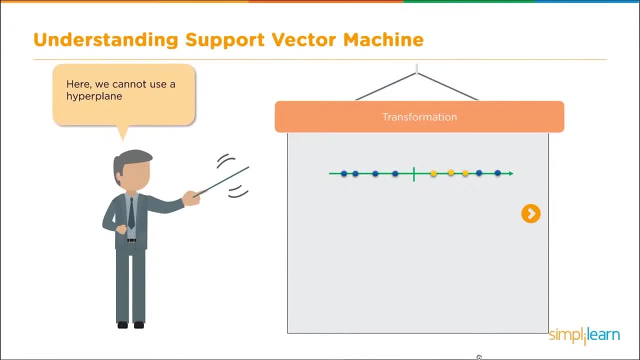 we can't use a hyperplane. So when you see data like this, it's necessary to move away from a 1D view of the data to a two-dimensional view of the data, And for the transformation we use what's called a kernel. 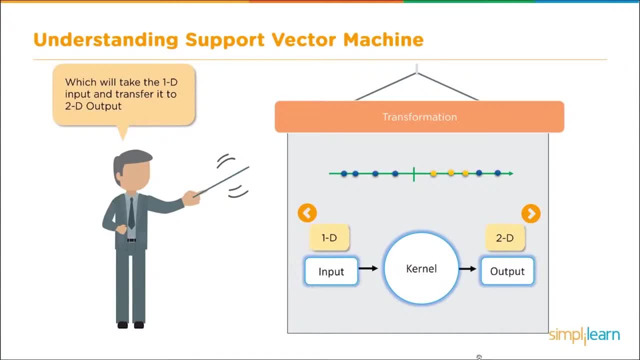 function, The kernel function, will take the 1D input and transfer it to a two-dimensional output. As you can see in this picture here, the 1D when transferred to a two-dimensional makes it very easy to draw a line between the two. 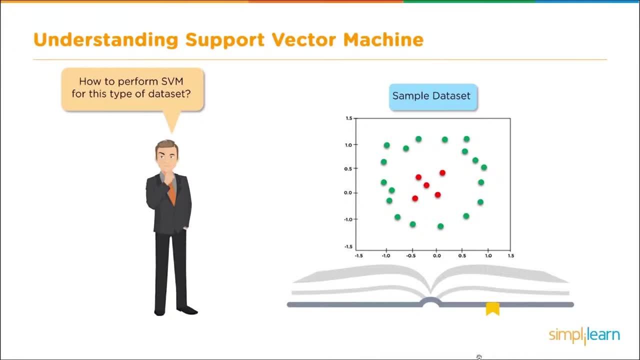 data sets. What if we make it even more complicated? How do we perform an SVM for this type of data set? Here you can see we have a two-dimensional data set where the data is in the middle surrounded by the green data on the outside. In this case, we're going. 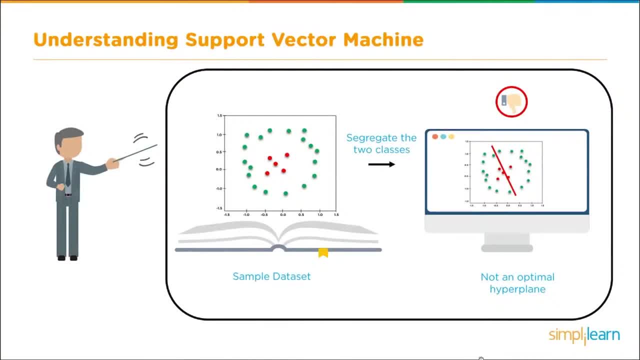 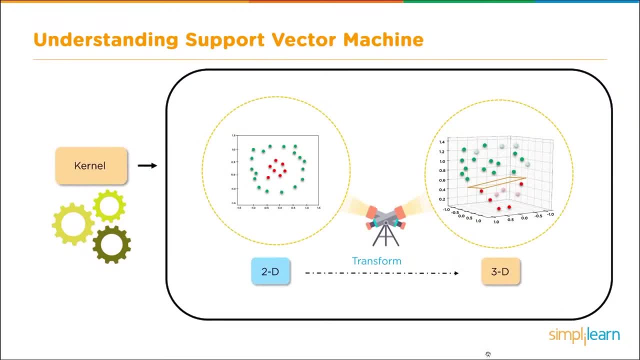 to segregate the two classes. We have our sample data set and if you draw a line through it's obviously not an optimal hyperplane in there. So to do that, we need to transfer the 2D to a 3D array And we need to. 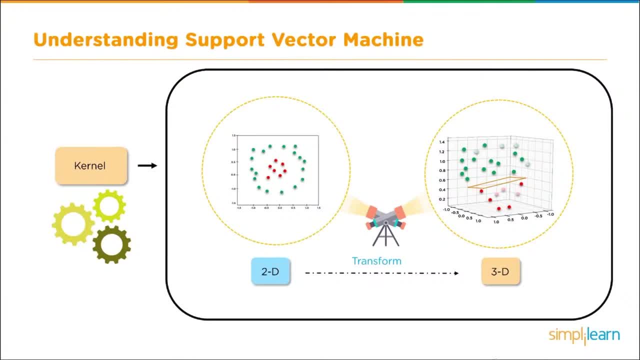 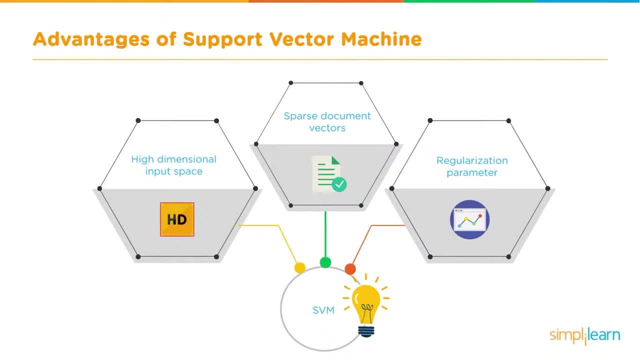 translate it into a three-dimensional array using the kernel. You can see where you can place a hyperplane right through it and easily split the data. Before we start looking at a programming example and dive into the script, let's look at the advantage of the support vector machine. We'll start. 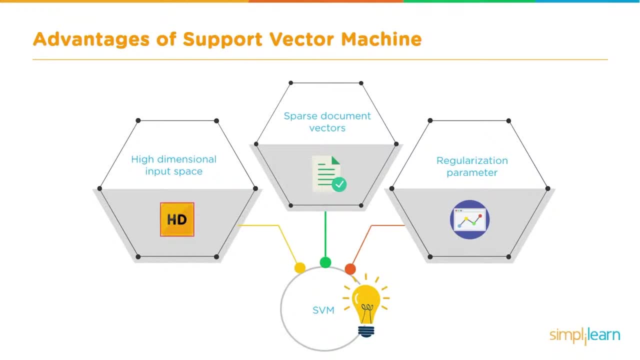 with high-dimensional input space, or sometimes referred to as the curse of dimensionality, We looked at earlier one-dimension, two-dimension, three-dimension. When you get to a thousand dimensions a lot of problems start occurring with most algorithms that have to be adjusted for The SVM. 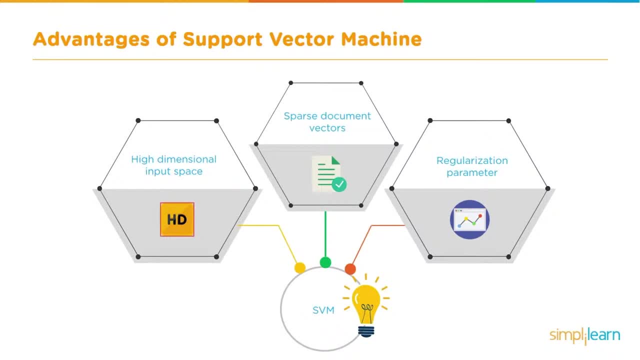 automatically does that in high-dimensional space. One of the high-dimensional space, one high-dimensional space that we work on, is sparse document vectors. This is where we tokenize the words and documents so we can run our machine learning algorithms over them. I've seen. 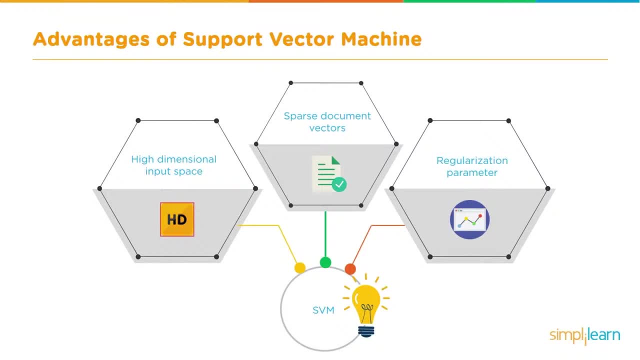 ones get as high as 2.4 million different tokens. That's a lot of vectors to look at. And finally, we have regularization parameter. The regularization parameter, or lambda, is a parameter that helps figure out whether we're going to have a bias. 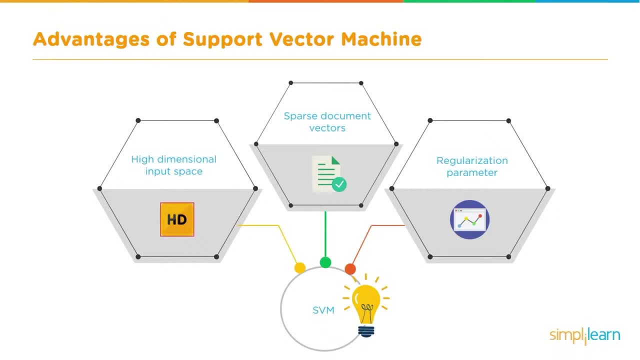 or overfitting of the data, Whether it's going to be overfitted to a very specific instance or it's going to be biased to a high or low value. With the SVM, it naturally avoids the overfitting and bias problems that we see. 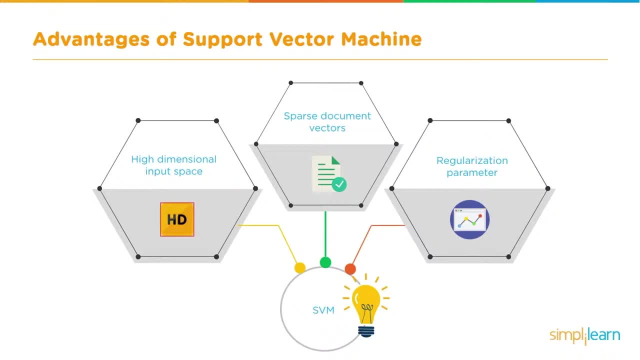 in many other algorithms. These three advantages of the support vector machine make it a very powerful tool to add to your repertoire of machine learning tools. Now, we did promise you a use case study. We're actually going to dive in to some Python programming, And so we're going to 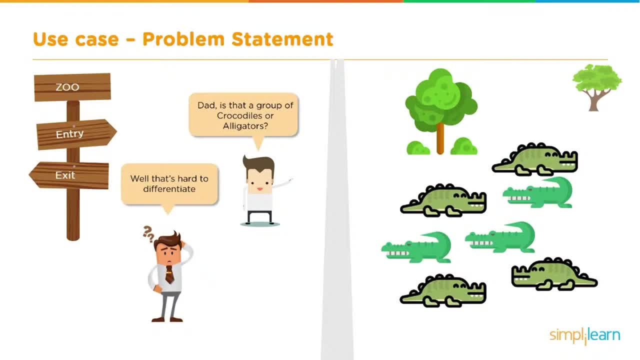 go into a problem statement and start off with the zoo. So in the zoo example we have family members going to the zoo And we have the young child going Dad, is that a group of crocodiles or alligators? Well, that's hard to. 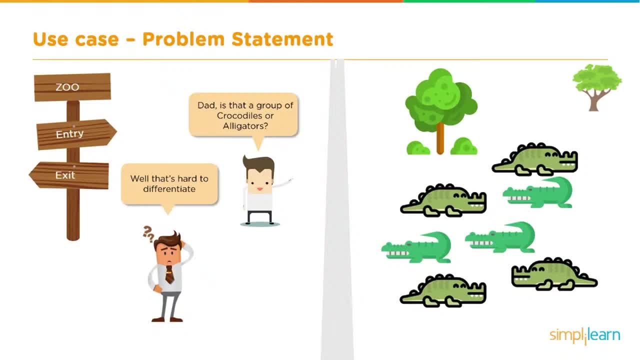 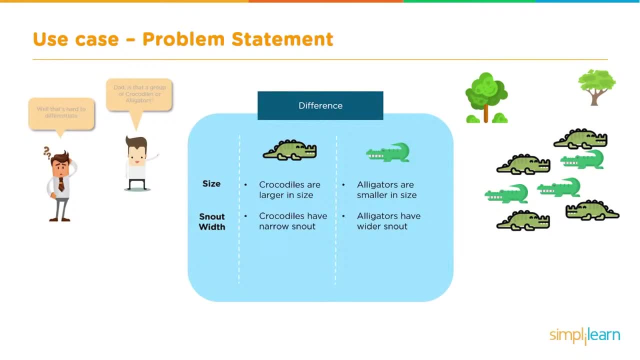 differentiate, And zoos are a great place to start looking at science and understanding how things work, especially as a young child. And so we can see the parents sitting here thinking, well, what is the difference between a crocodile and an alligator? Well, one. 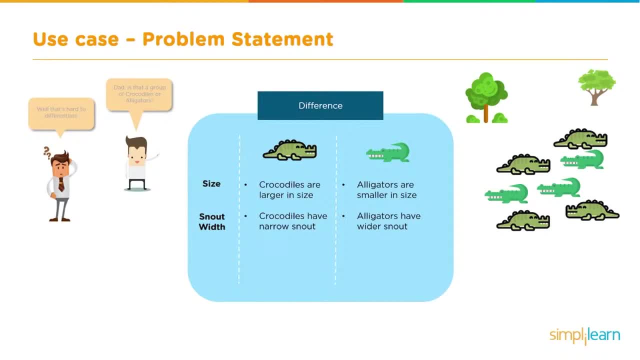 crocodiles are larger in size, alligators are smaller in size. snout width: the crocodiles have a narrow snout and alligators have a wider snout. And, of course, in the modern day and age, the father is sitting here thinking: how can I? 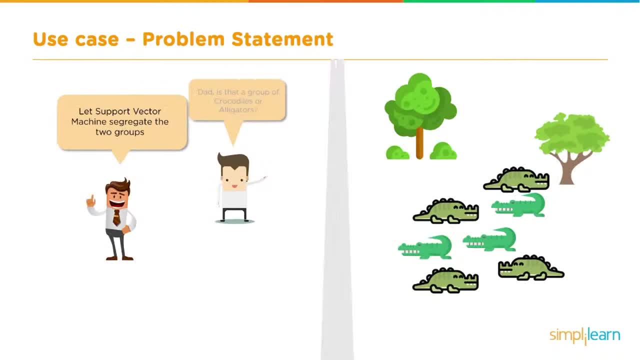 turn this into a lesson for my son And he goes let a support vector machine segregate the two groups. I don't know if my dad ever told me that, but that would be funny. Now, in this example, we're not going. 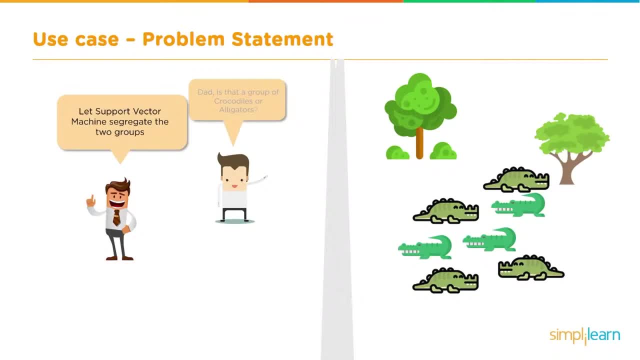 to use actual measurements and data. We're just using that for imagery And that's very common in a lot of machine learning algorithms and setting them up. But let's roll up our sleeves and we'll talk about that more in just a moment as we break into our Python. 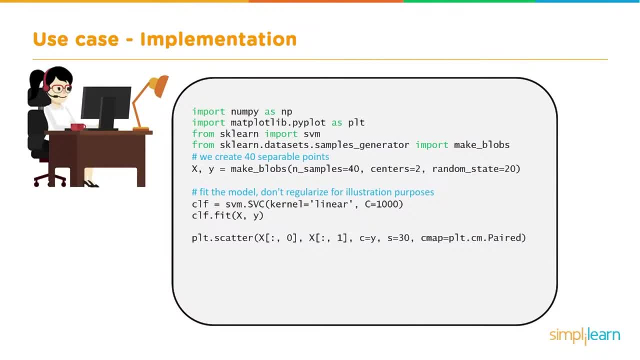 script. So here we arrive in our actual coding, And I'm going to move this into a Python editor in just a moment. But let's talk a little bit about what we're going to cover First. we're going to cover in the 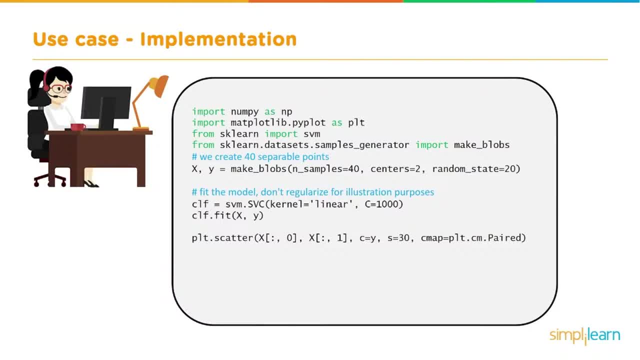 code, the setup, How to actually create our SVM, And you're going to find that there's only two lines of code that actually create it, and the rest of it is done so quick and fast that it's all here in the first page And we'll show you what that looks. 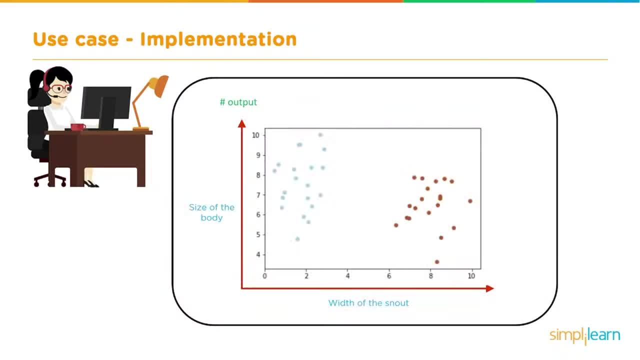 like, as far as our data, We're going to create some data. I talked about creating data just a minute ago, And so we'll get into the creating data here and you'll see this nice correction of our two blobs And we'll go through that in just a second. 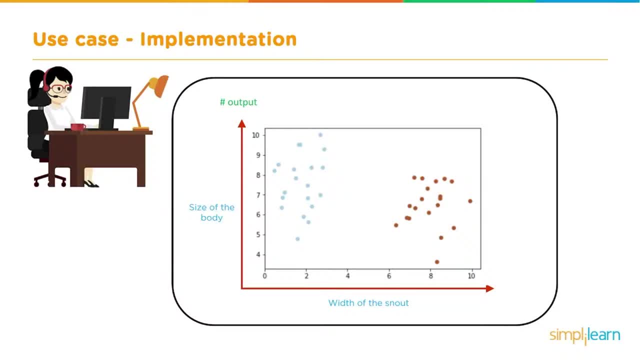 And then the second part is: we're going to take this and we're going to bump it up a notch. We're going to show you what it looks like behind the scenes, But let's start with actually creating our setup. I like to use the 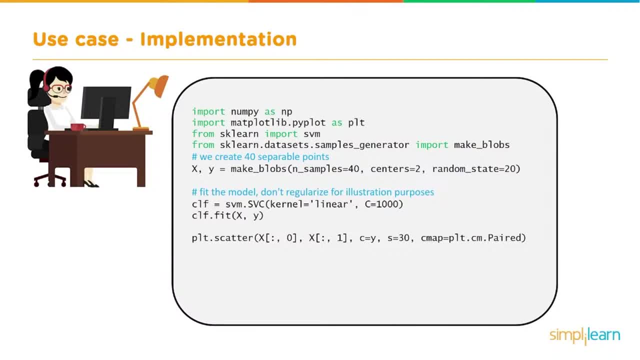 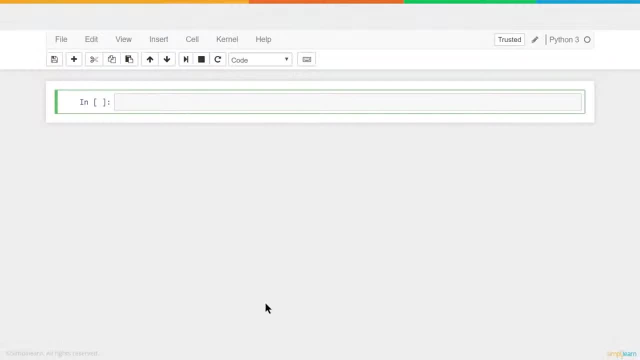 Anaconda Jupyter Notebook because it's very easy to use. But you can use any of your favorite Python editors or setups and go in there, But let's go ahead and switch over there and see what that looks like. So here we are in the 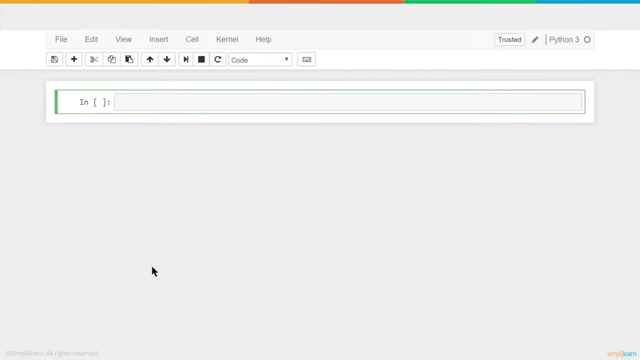 Anaconda Python Notebook or Anaconda Jupyter Notebook. with Python, We're using Python 3.. I believe this is 3.5, but it should work in any of your 3x versions And you'd have to look at the sklearn and make sure if you're using 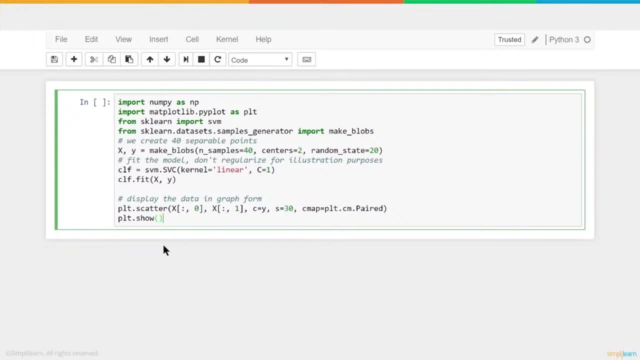 a 2x version or an earlier version. Now let's go ahead and put our code in there, And one of the things I like about the Jupyter Notebook is I can go up to view and I'm going to go ahead and toggle the line numbers on to make it. 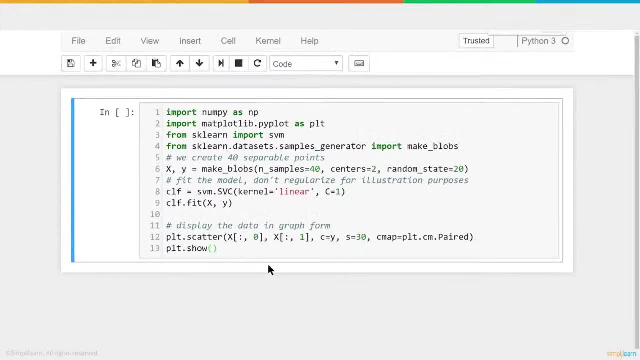 a little bit easier to talk about, And we can even increase the size, because this is edited in. in this case, I'm using Google Chrome Explorer and that's how it opens up for the editor, Although anyone, like I said, any editor will work. 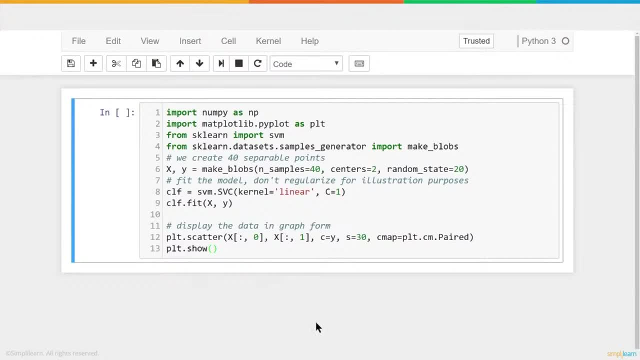 Now the first step is going to be our imports, And we're going to import four different parts. The first two I want you to look at are line 1 and line 2 are numpy as np and matplotlibrarypyplot as plt. Now, these are very standardized. 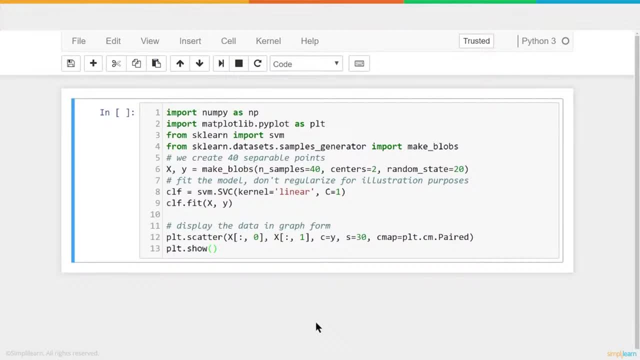 imports when you're doing work. The first one is the numbers Python. We need that because part of the platform we're using uses that for the numpy array, And I'll talk about that in a minute so you can understand why we want to use a numpy array versus a standard. 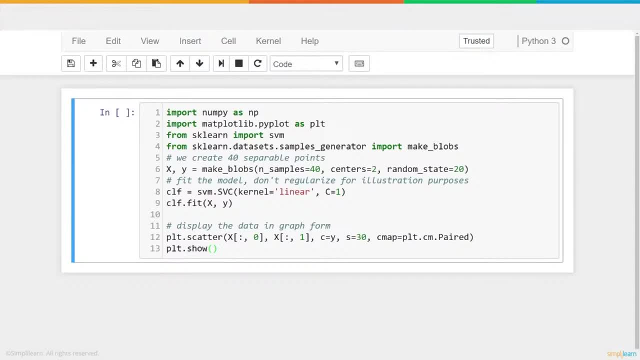 Python array And normally it's pretty standard setup to use np for numpy. The matplotlibrary is how we're going to view our data, So this has. you do need the np for the sklearn module, But the matplotlibrary is purely for our use. 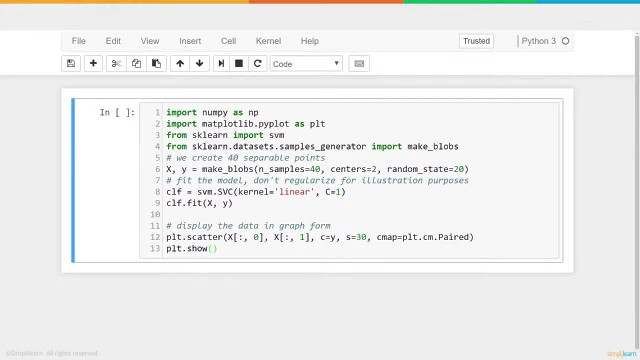 for visualization, And so you really don't need that for the SVM, But we're going to put it there so you have a nice visual aid and we can show you what it looks like. That's really important at the end when you finish everything. So you have a. 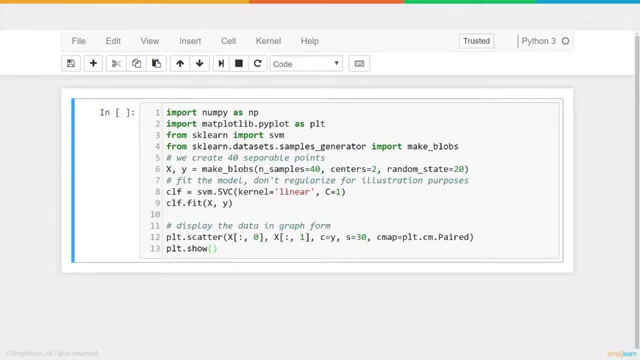 nice display for everybody to look at. And then, finally, we're going to- I'm going to jump one ahead- to line number 4.. That's the sklearndatasetssamplesgenerator import makeblobs. And I told you that we were going to make up data. 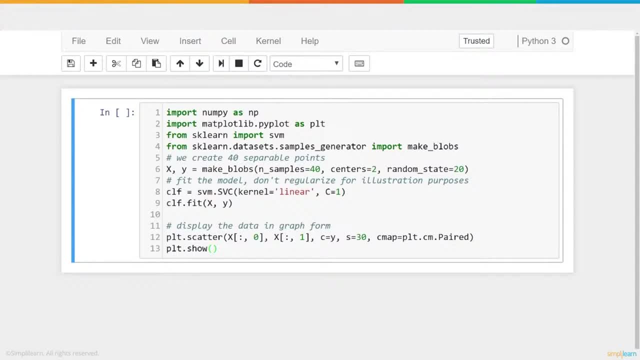 And this is a tool that's in the sklearn to make up data. I personally don't want to go to the zoo, get in trouble for jumping over the fence and probably get eaten by the crocodiles or alligators as I work on measuring. 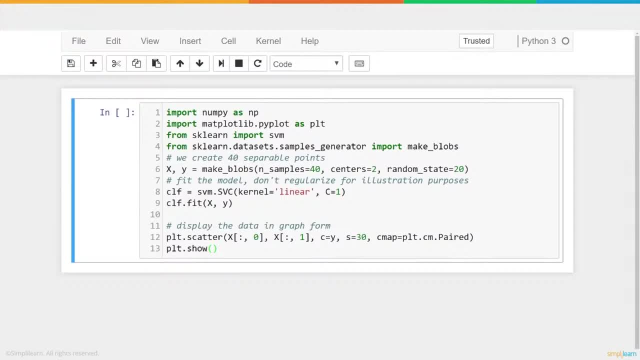 their snouts and width and length. Instead, we're just going to make up some data, And that's what that makeblobs is. It's a wonderful tool if you're ready to test your setup and you're not sure about what data you're going to put in there. 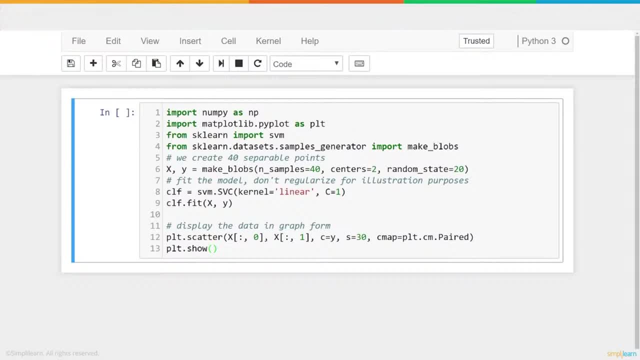 You can create this blob and it makes it real easy to use. And finally, we have our actual SVM, The sklearn import SVM on line 3.. So that covers all our imports. We're going to create- remember I used the makeblobs to create data And we're going to. 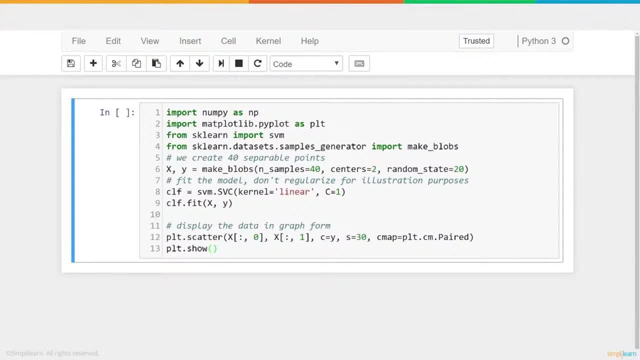 create a capital X and a lower case Y equals makeblobs in samples equals 40. So we're going to make 40 lines of data. It's going to have two centers with a random state equals 20.. So each group is going to have 20 different pieces of. 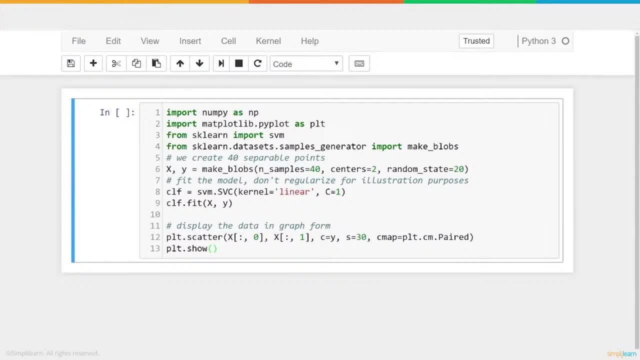 data in it, And the way that looks is that we'll have under X an XY plane. So I'll have two numbers under X, And Y will be 0 or 1.. That's the two different centers. So we have yes or 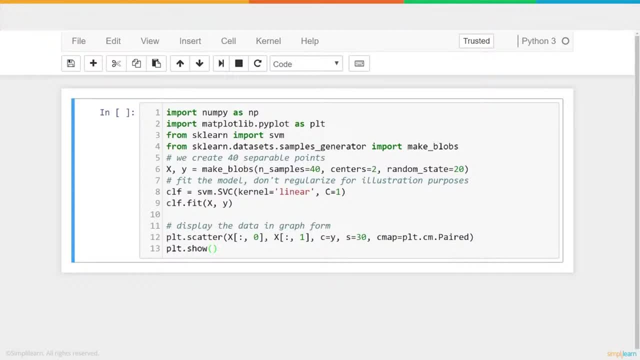 no, In this case alligator or crocodile, That's what that represents. And then I told you that the actual sklearn, or the SVM, is in two lines of code, And we see it right here with: CLF equals SVM, dot, SVC, kernel equals linear, And I set C equal to. 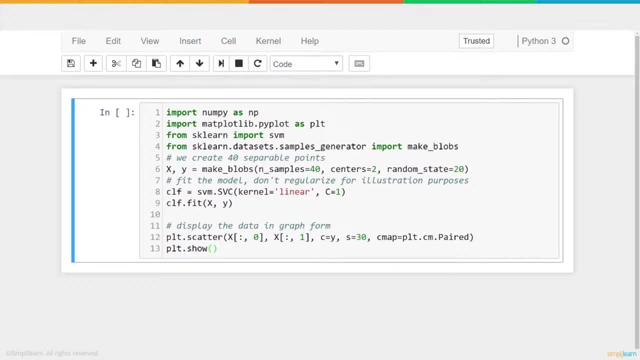 1. Although in this example, since we are not regularizing the data because we want it to be very clear and easy to see, I went ahead. you can set it to 1000 a lot of times when you're not doing that. 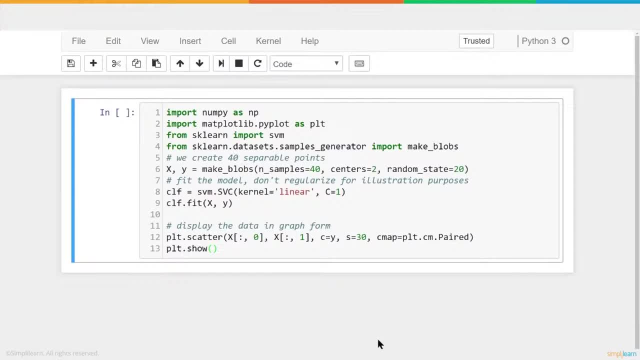 But for this thing- linear, because it's a very simple linear example. We only have the two dimensions and it'll be a nice linear hyper plane. It'll be a nice linear line instead of a full plane, So we're not dealing with a huge amount of data. 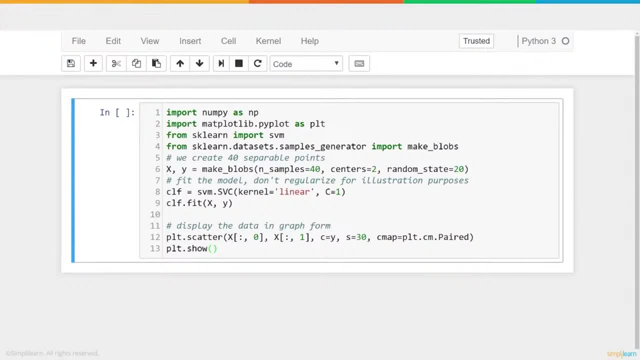 And then all we have to do is do CLF dot fit X, comma Y, And that's it. CLF has been created, And then we're going to go ahead and display it, And I'm going to talk about this display here in just a second, But let me go. 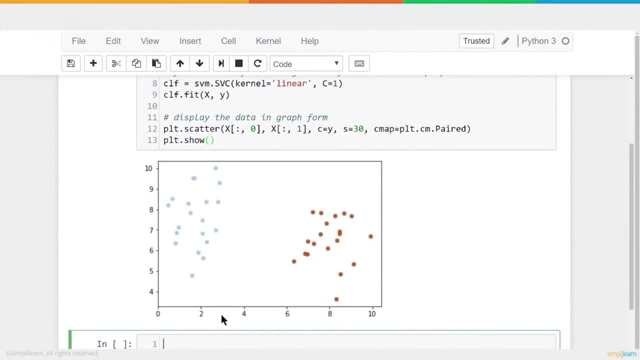 ahead and run this code- And this is what we've done- is we've created two blobs. You'll see the blue on the side and then kind of an orangeish on the other side. That's our two sets of data They represent- one represents crocodiles. 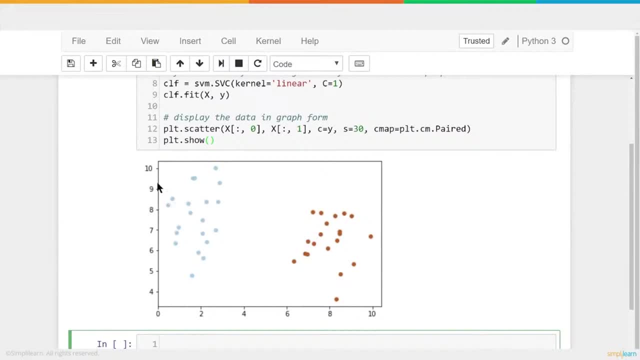 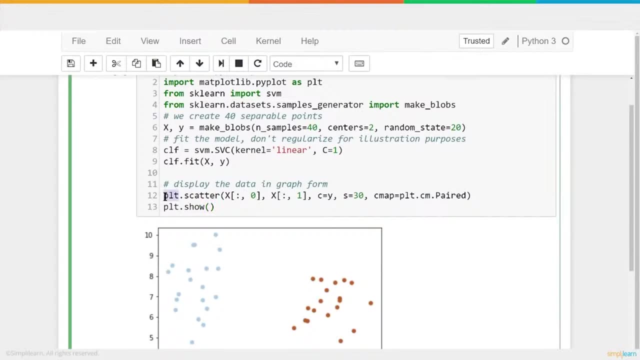 and one represents alligators. And then we have our measurements. In this case we have like the width and length of the snout, And I did say I was going to come up here and talk just a little bit about our plot And you'll see, PLT, That's what we. 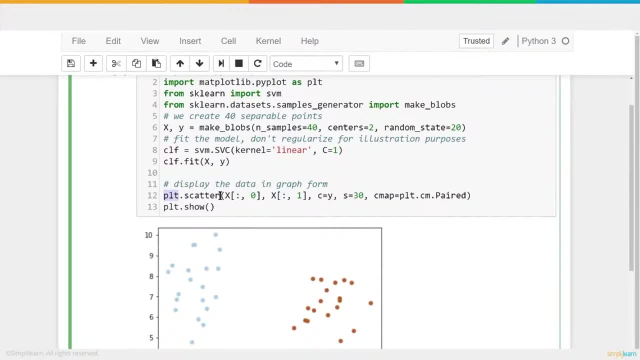 imported. We're going to do a scatter plot. That means we're just putting dots on there. And then look at this notation: I have the capital X and then in brackets I have a colon, comma zero. That's from NumPy, If you did. 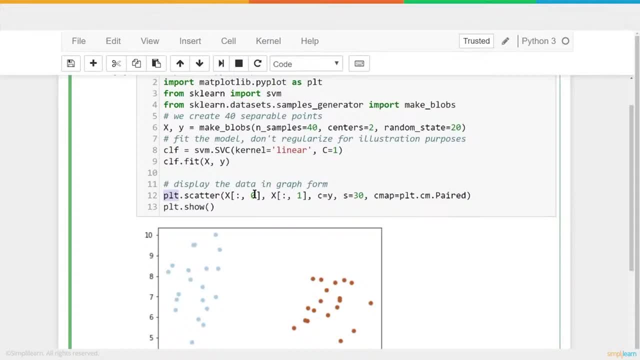 that in a regular array, you'll get an error. in a Python array You have to have that in a NumPy array. It turns out that our make blobs returns a NumPy array, And this notation is great, because what it means is the first part. 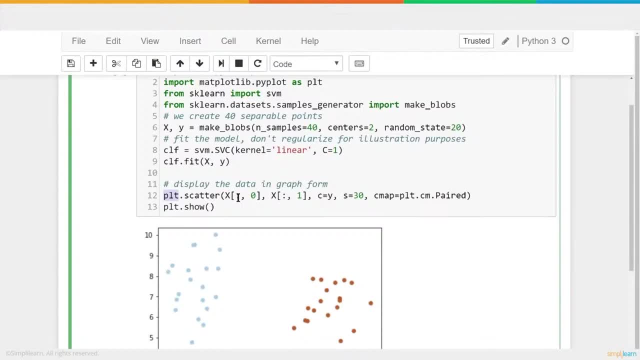 is the colon. It means we're going to do all the rows. That's all the data in our blob. we created under capital X, And then the second part has a comma zero. We're only going to take the first value And then, if you notice, 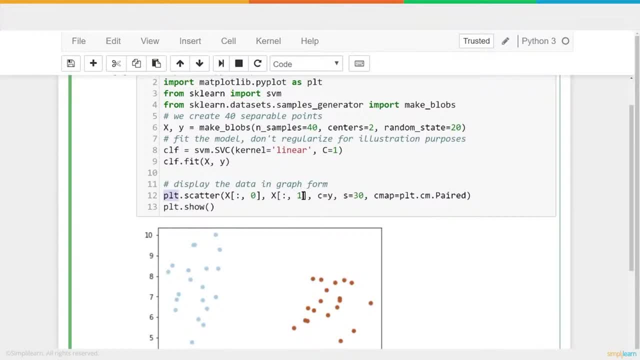 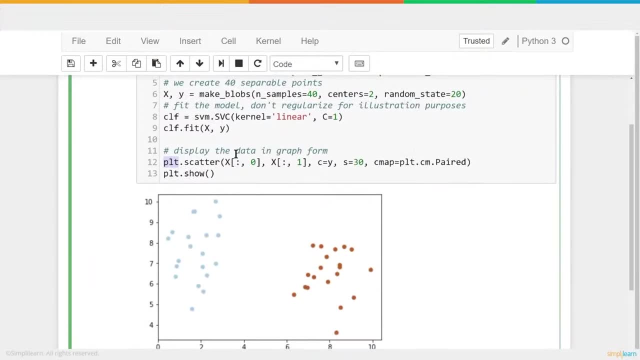 we do the same thing, but we're going to take the second value. Remember we always start with zero and then one. So we have columns zero and column one, And you can look at this as our X- Y plots. The first one is the X. 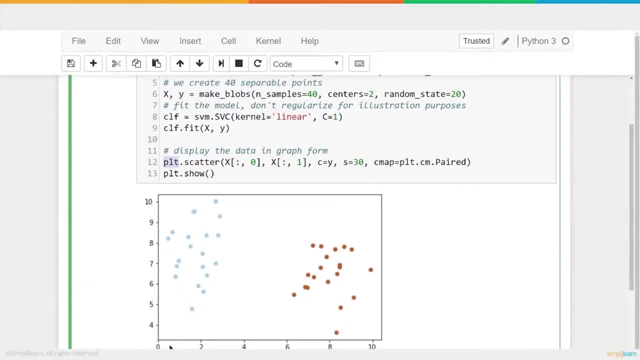 plot and the second one is the Y plot. So the first one is on the bottom Zero, two, four, six, eight and ten, And then the second one, X of the one, is the four, five, six, seven, eight, nine, ten going up the. 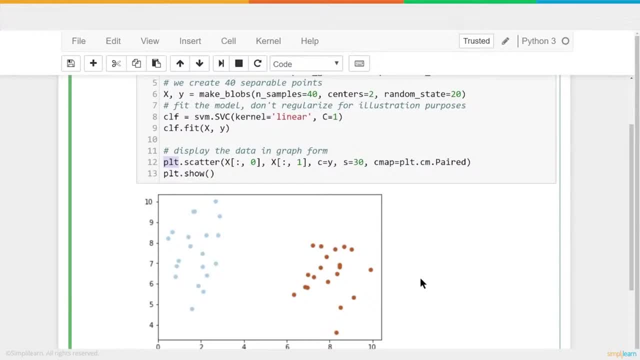 left hand side. S equals thirty is just the size of the dots. We can see them. It says real tiny dots And then CMAP equals PLT dot, CM dot paired And you'll also see the C equals Y. That's the color We're using, two colors. 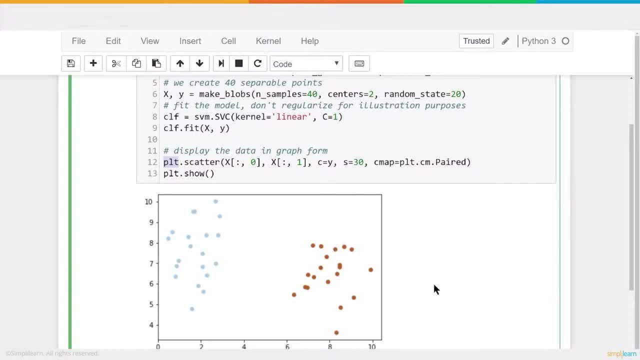 Zero one, And that's why we get the nice blue and the two different colors for the alligator and the crocodile. Now you can see here that we did this. the actual fit was done in two lines of code. A lot of times it'll be. 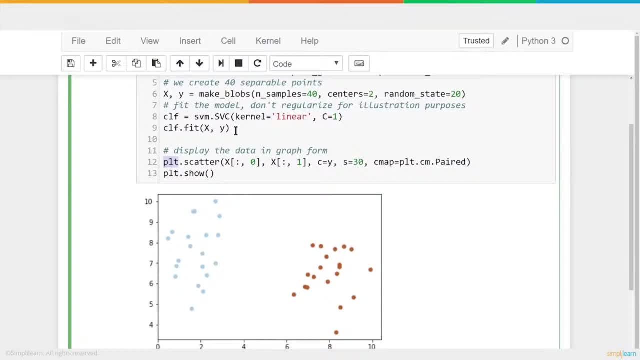 a third line where we regularize the data. We set it between like minus one and one And we reshape it. But for this it's not necessary And it's also kind of nice because you can actually see what's going on. And then, if we wanted, 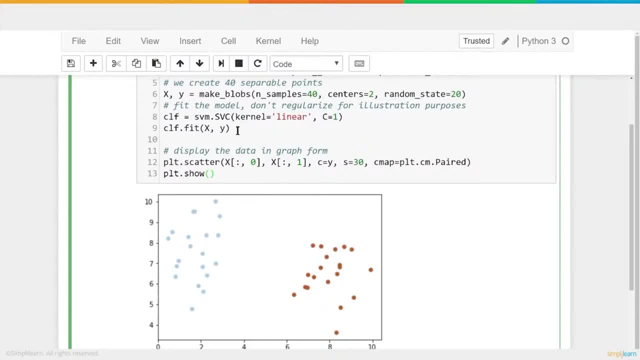 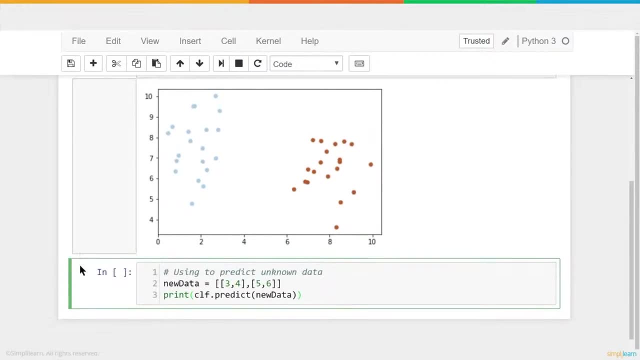 to. we wanted to actually run a prediction- Let's take a look and see what that looks like- And to predict some new data, and we'll show this again as we get towards the end of digging in deep. You can simply assign your new data. 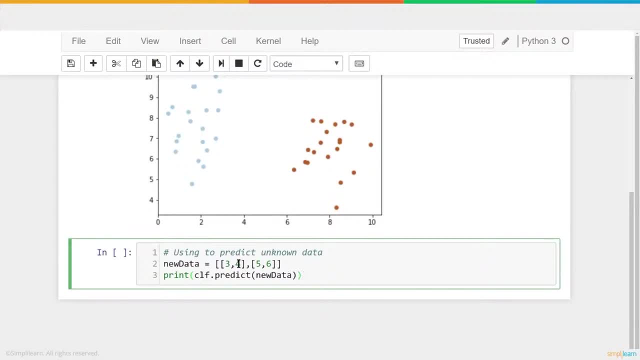 In this case, I am giving it a width and length three, four, and a width and length five, six, And note that I put the data as a set of brackets and then I have the brackets inside. And the reason I do that is because when we're looking, 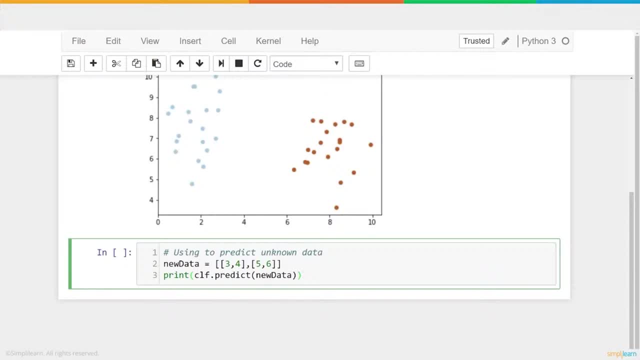 at data. it's designed to process a large amount of data coming in. We don't want to just process one line at a time, And so in this case I'm processing two lines And then I'm just going to print And you'll see: clfpredict new data. 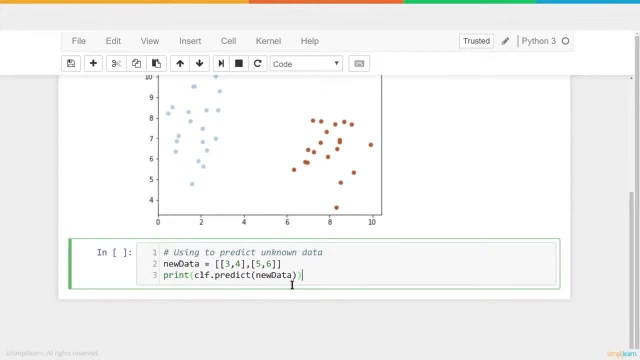 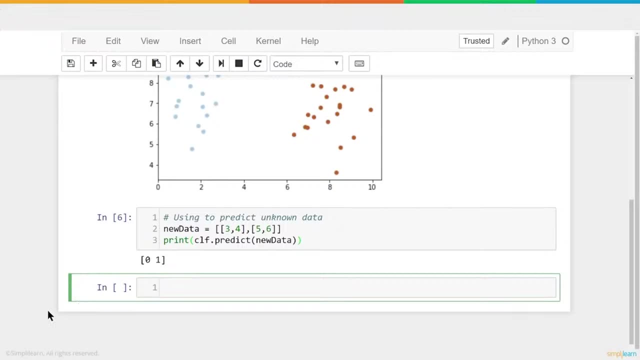 So the clf and the dot predict part is going to give us an answer And let's see what that looks like And you'll see zero one. So predicted the first one, the three, four is going to be on the one side and the five- six is going. 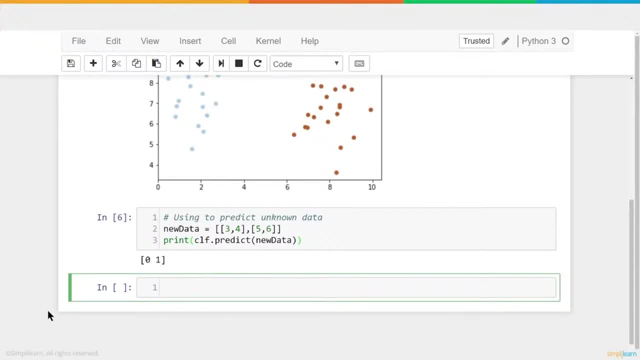 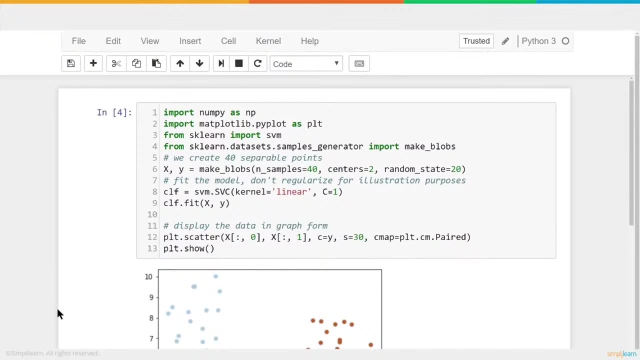 to be on the other side. So one came out as an alligator and one came out as a crocodile. Now, that's a pretty short explanation for this setup, But really we want to dig in and see what's going on behind the scenes. And let's see what that. 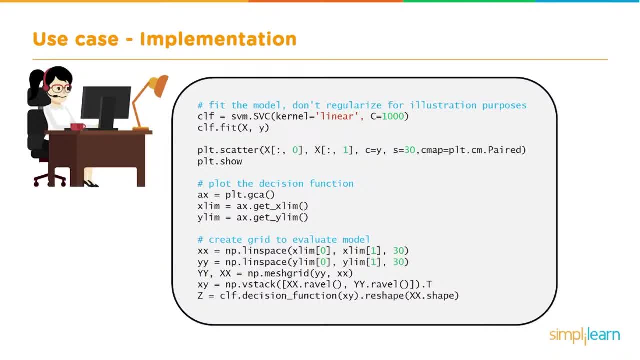 looks like. So the next step is to dig in deep and find out what's going on behind the scenes And also put that in a nice pretty graph. We're going to spend more work on this than we did actually generating the original model, And you'll see here. 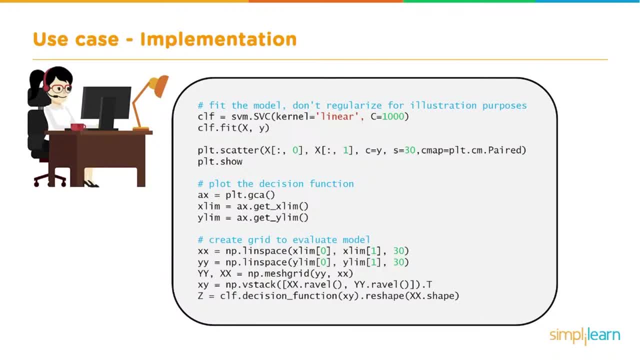 that we go through a few steps. I'll move this over to our editor in just a second. We come in, We create our original data. It's exactly identical to the first part And I'll explain why we redid that and show you how not to redo that. 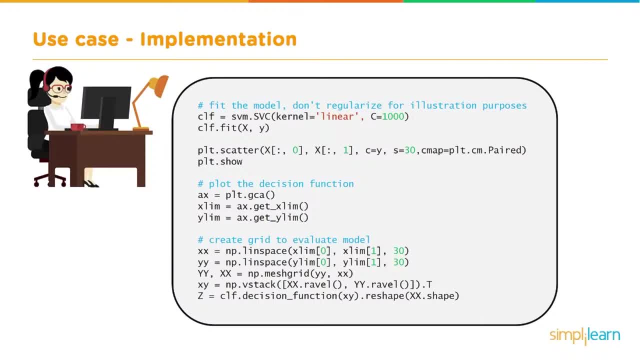 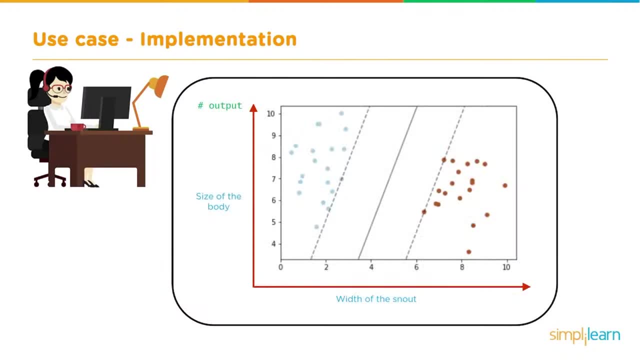 And then we're going to go in there and add in those lines. We're going to see what those lines look like and how to set those up, And finally we're going to plot all that on here and show it And you'll get a nice graph with the. 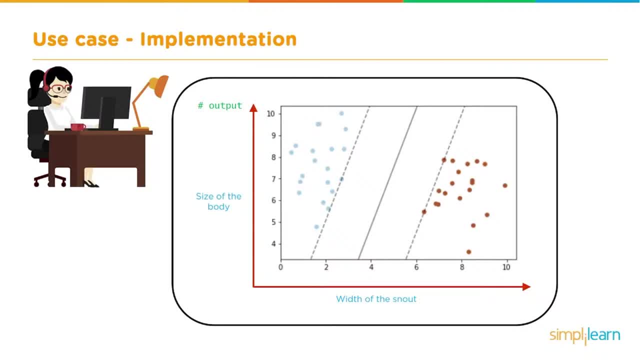 what we saw earlier when we were going through the theory behind this, where it shows the support vectors and the hyperplane And those are done, where you can see the support vectors as the dash lines and the solid line, which is the hyperplane. Let's get that into our. 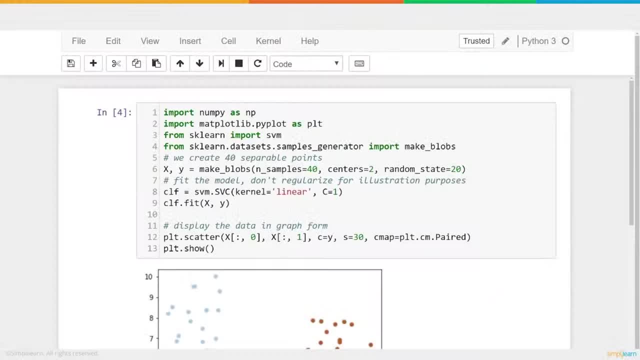 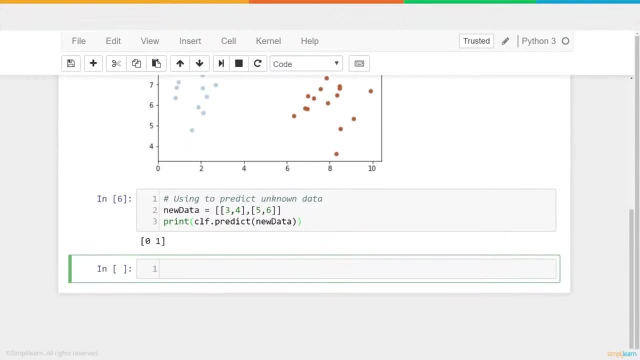 Jupyter notebook. Before I scroll down to a new line, I want you to notice line 13.. It has plot show And we're going to talk about that here in just a second. Let's scroll down to a new line down here. 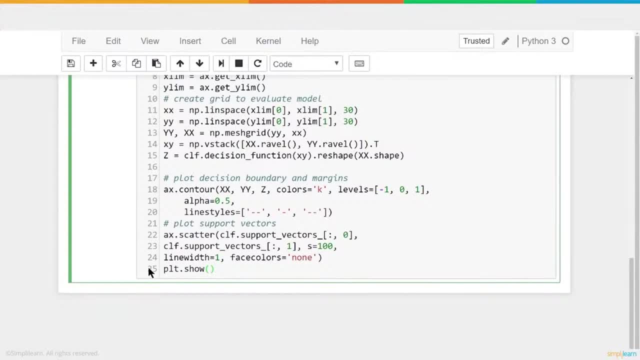 And I'm going to paste that code in And you'll see that the plot show has moved down below. Let's scroll up a little bit And if you look at the top here of our new section, 1,, 2,, 3,- 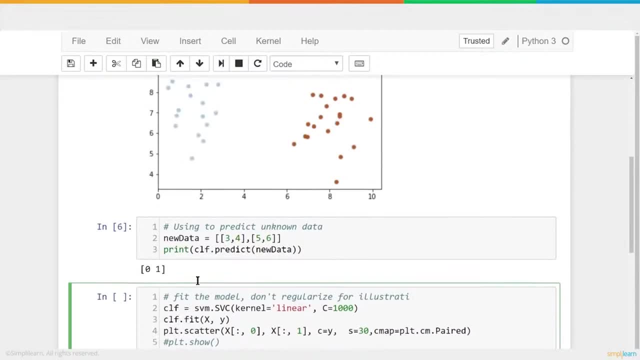 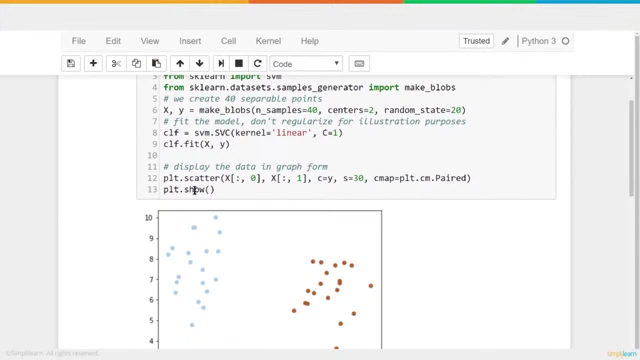 and 4 is the same code we had before, And let's go back up here and take a look at that. We're going to fit the values on our SVM and then we're going to plot scatter it and then we're going to do a plot show. 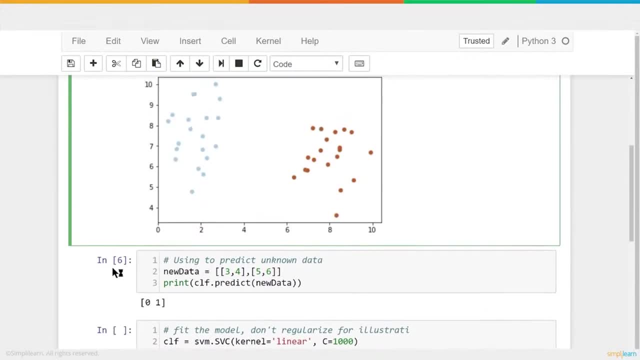 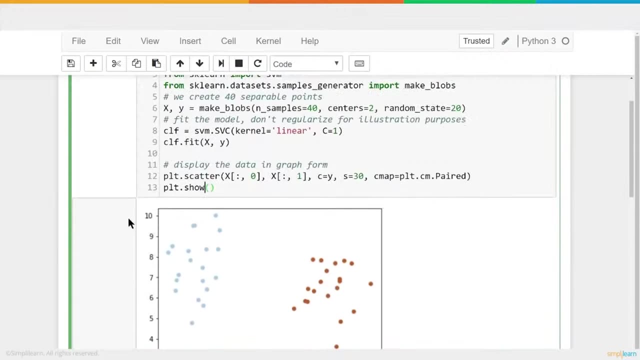 So you should be asking: why are we redoing the same code? Well, when you do the plot show, that blanks out what's in the plot. So once I've done this plot show, I have to reload that data. Now we could do this simply by removing it up here. 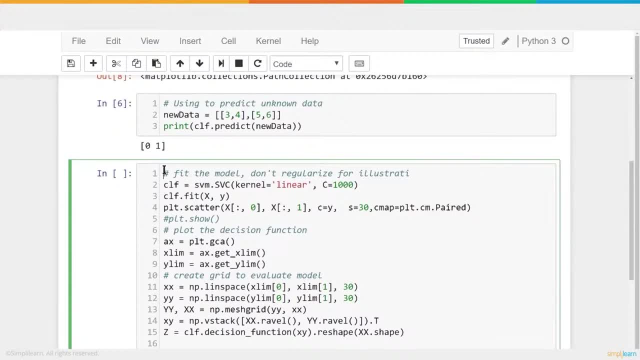 re-running it and then coming down here, and then we wouldn't have to re-run these first four lines of code. Now in this it doesn't matter too much, and you'll see the plot show is down here and then removed right there on line 5.. 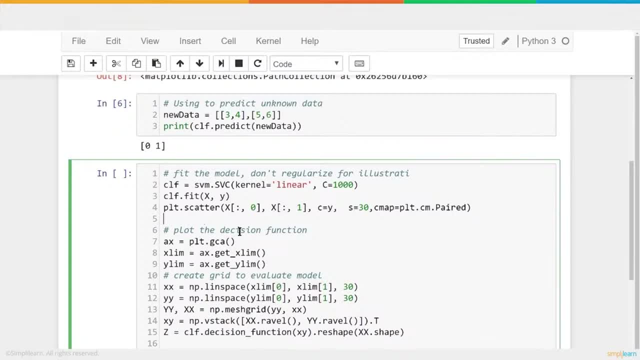 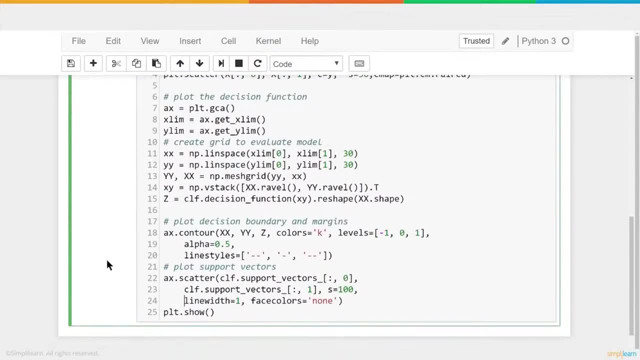 I'll go ahead and just delete that out of there, Because we don't want to blank out our screen, We want to move on to the next setup. So we can go ahead and just skip the first four lines, because we did that before, And let's take a look at the. 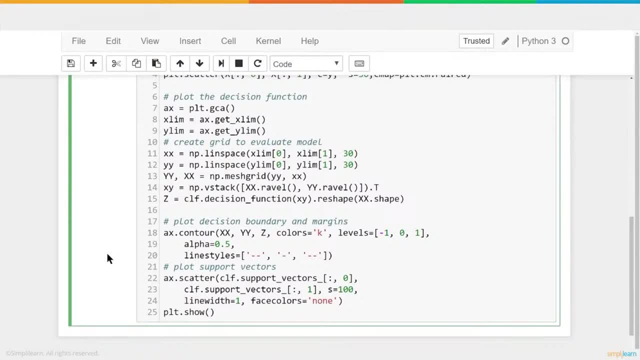 ax equals pltgca. Now, right now, we're actually spending a lot of time just graphing. That's all we're doing here. So this is how we display a nice graph with our results and our data. Ax is a very standard used variable when you're talking about. 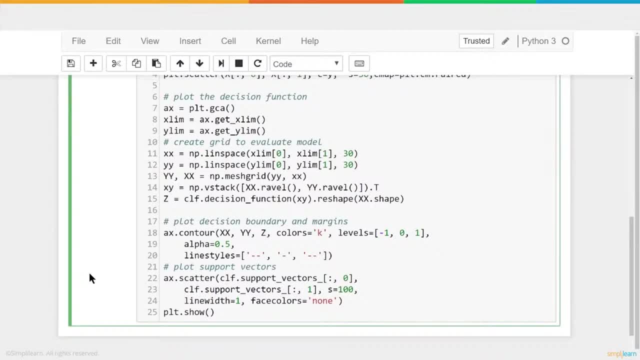 plt And it's just setting it to that axis, the last axis in the plt. It can get very confusing if you're working with many different layers of data on the same graph And this makes it very easy to reference the ax. So this reference is looking at. 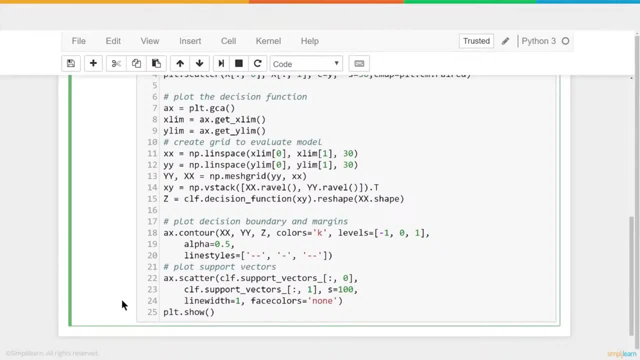 the plt that we created and we already mapped out our two blobs on. And then we want to know the limits, So we want to know how big the graph is. We can find out the x limit and the y limit simply with the get x limit. 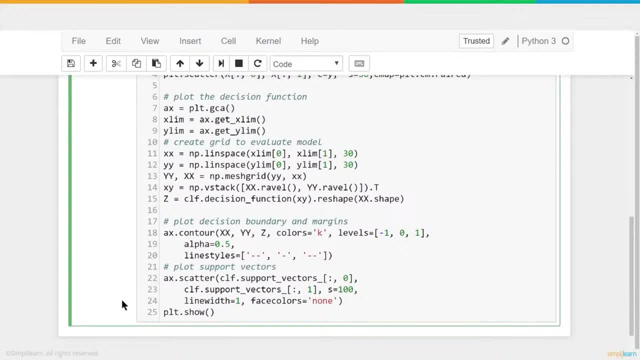 and get y limit commands, which is part of our matplot library, And then we're going to create a grid And you'll see down here we have. we've set the variable xx equal to nplinespace. xlimit 0,. xlimit 1, 30. 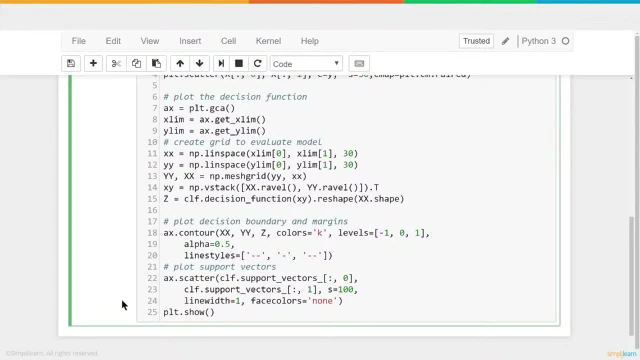 And we've done the same thing for the y space. And then we're going to go in here and we create a mesh grid And this is a numpy command. So we're back to our numbers, python. Let's go through what these numpy commands mean with the 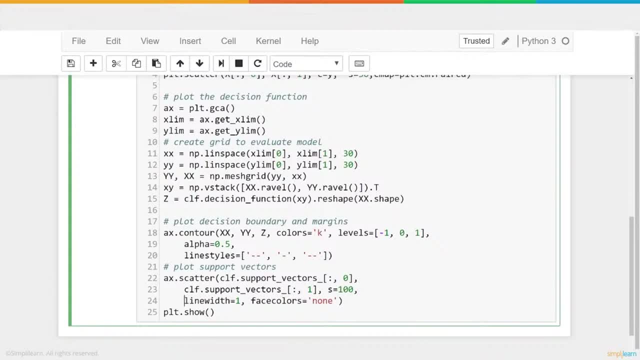 linespace and the mesh grid. We've taken xx- small xx equals nplinespace, and we have our xlimit 0 and our xlimit 1 and we're going to create 30 points on it And we're going to do the same thing for the y axis. 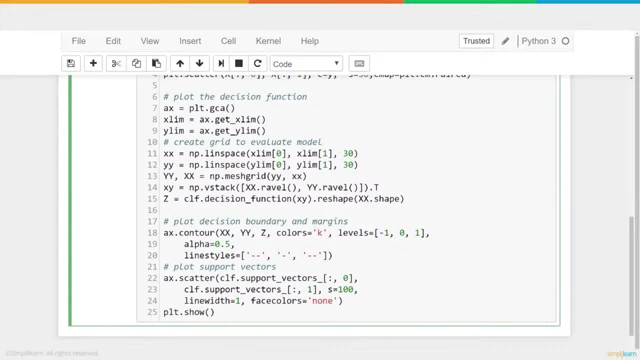 Now, this has nothing to do with our evaluation. It's all we're doing is we're creating a grid of data, And so we're creating a set of points between 0 and the xlimit. We're creating 30 points, And the same thing with the y And then the mesh. 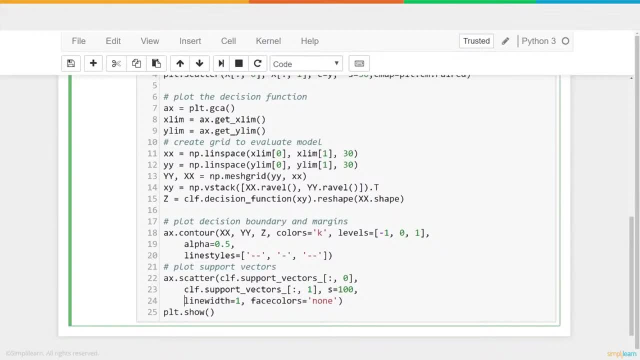 grid loops those all together, so it forms a nice grid. So if we were going to do this, say between the limit 0 and 10, and do 10 points, we would have a 0, 0, 1, 1, 0, 1, 0, 2, 0, 3. 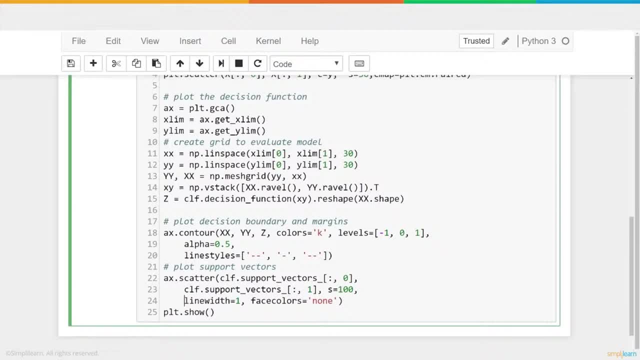 0,, 4 to 10 and so on. You can just imagine a point at each corner of one of those boxes And the mesh grid combines them all. So we take the yy and the xx we created and creates the full grid. 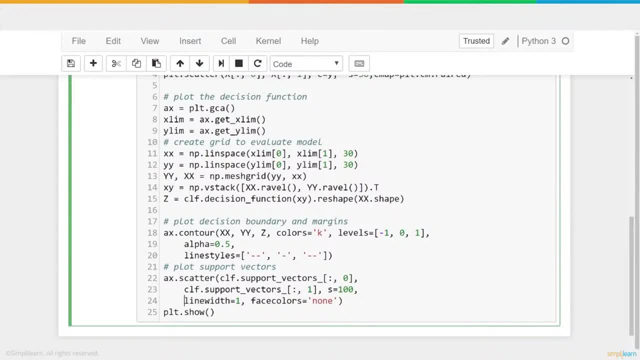 And we've set that grid into the yy coordinates and the xx coordinates. Now, remember we're working with Numbi and Python. We like to separate those We like to have instead of it being x comma 1, x comma y and then x2 comma y2. 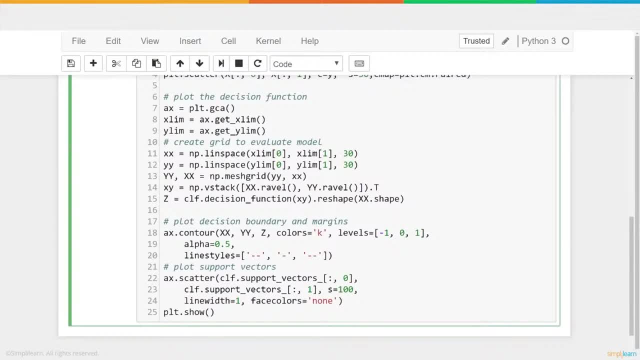 and in the next set of data it would be a column of x's and a column of y's, And that's what we have here is, we have a column of y's, and we put it as a capital yy, and a column of x's, Capital xx, With all. 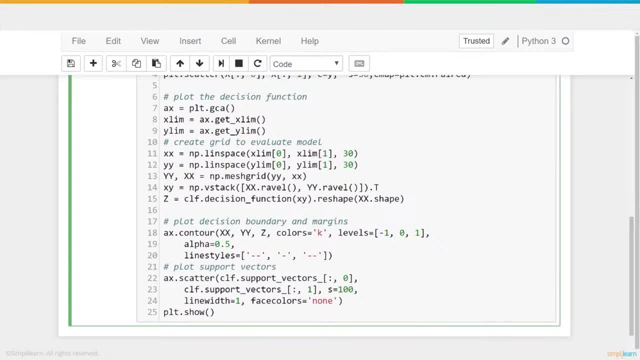 those different points being listed And finally, we get down to the Numbi vstack. Just as we created those in the mesh grid, we're now going to put them all into one array, xy array, Now that we've created the stack of data. 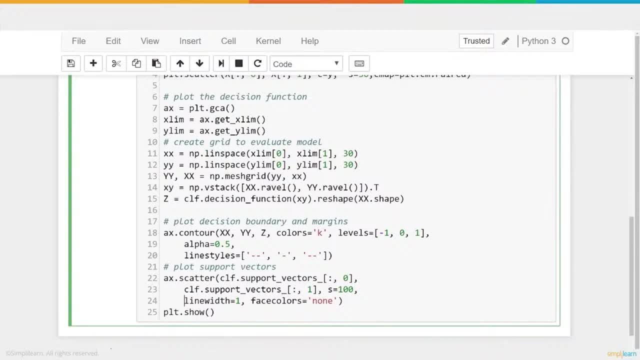 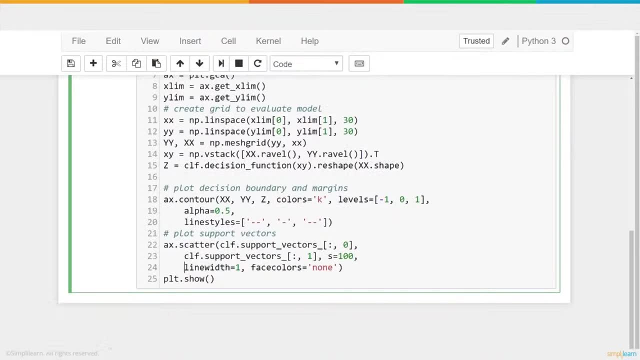 points. we're going to do something interesting here. We're going to create a value, z, And the z equals the clf. That's our support vector machine. we created And we've already trained And we have a dot decision function And we're going to put the xy in there. 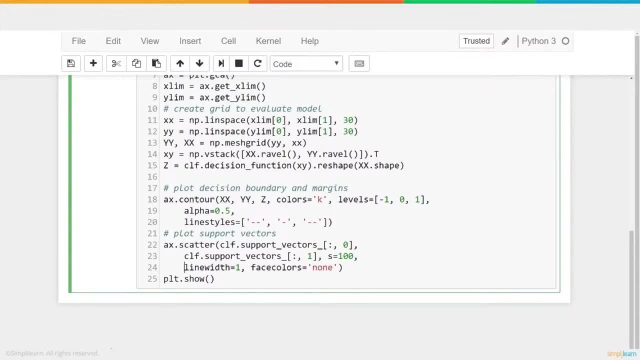 So here we have all this data. We're going to put that xy in there, That data, And we're going to reshape it And you'll see that we have the xx dot shape in here. This literally takes the xx, resets it up connected. 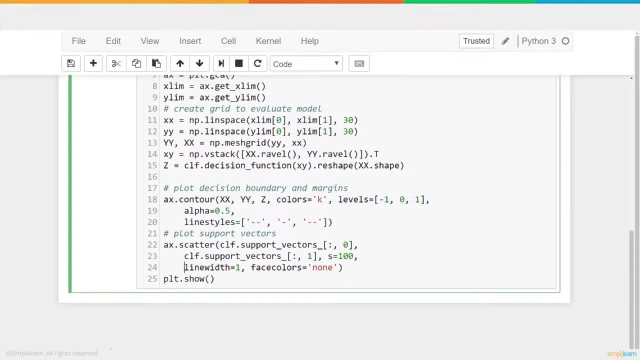 to the y And the z value lets us know whether it is the left hand side. It's going to generate three different values. The z value does, And it'll tell us whether that data is a support vector to the left. the hyperplane. 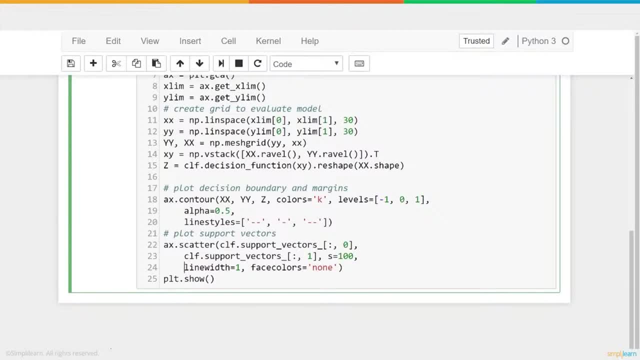 in the middle or the support vector to the right. So it generates three different values for each of those points And those points have been reshaped so that they're right on the line, On those three different lines. So we've set all of our data. 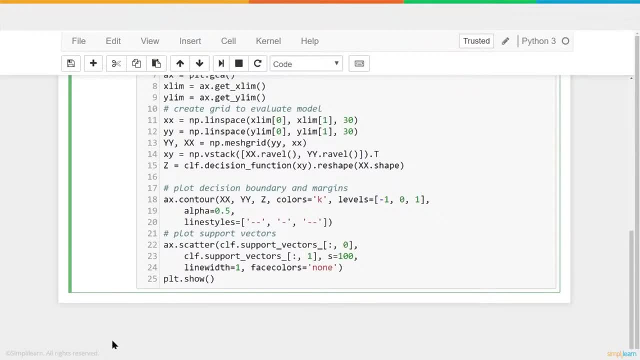 up, We've labeled it to three different areas And we've reshaped it And we've just taken thirty points in each direction. If you do the math, you have thirty times thirty, So that's nine hundred points of data And we've separated it between the three lines. 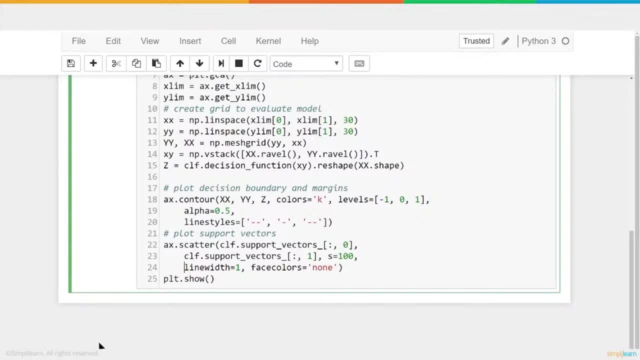 and reshaped it to fit those three lines. We can then go back to our map plot library. We've created the ax And we're going to create a contour, And you'll see, here we have contour xx, capital yy. These have been reshaped to fit those lines. 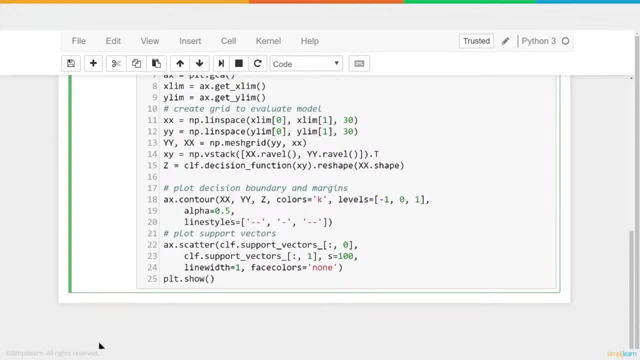 Z is the labels. So now we have the three different points with the labels in there And we can set the colors. equals k And I told you we had three different labels But we have three levels of data. The alpha just makes it kind of see-through. 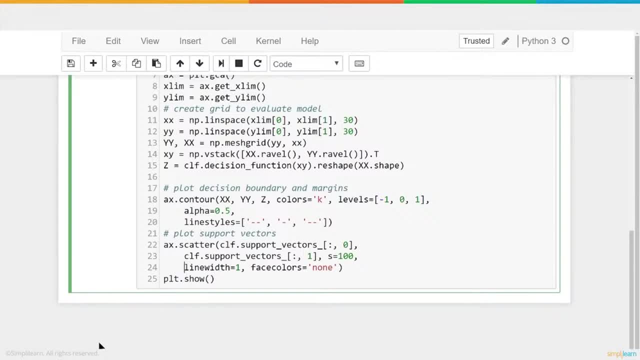 So it's only .5 of the value in there. So when we graph it, the data will show up from behind it wherever the lines go. And finally, the line styles. This is where we set the two support vectors to be dash, dash lines And then a single one. 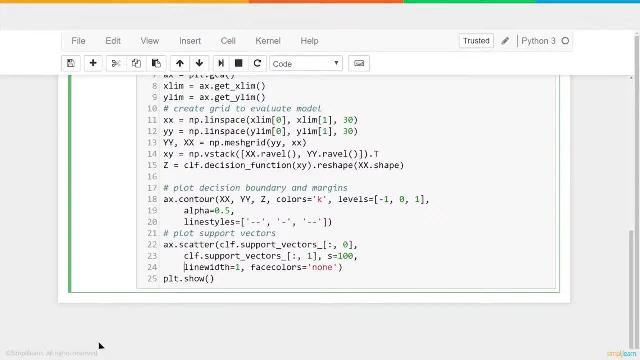 is just a straight line. That's what all that setup does. And then, finally, we take our axscatter. We're going to go ahead and plot the support vectors, But we've programmed it in there so that they look nice Like the dash, dash line and the dash line. 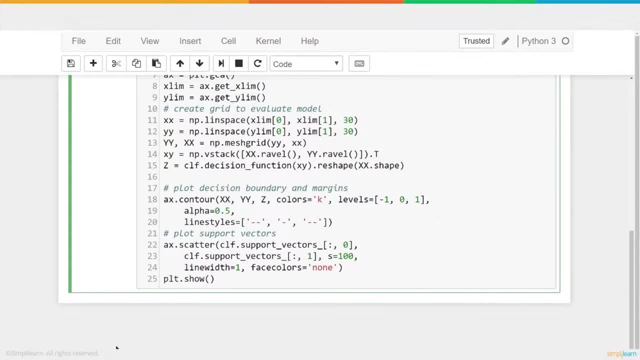 on that grid And you can see here, when we do the clfsupport vectors, we are looking at column 0 and column 1.. And then again we have the s equals 100.. So we're going to make them larger And the line width equals 1.. 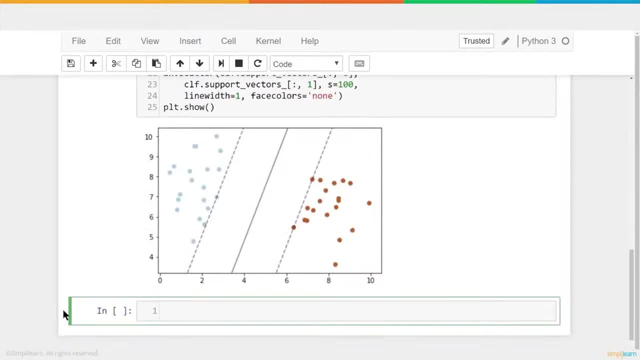 And the colors equals none. Let's take a look and see what that looks like when we show it And you can see when we get down to our end result. it creates a really nice graph. We have our two support vectors and dash lines, And they have. 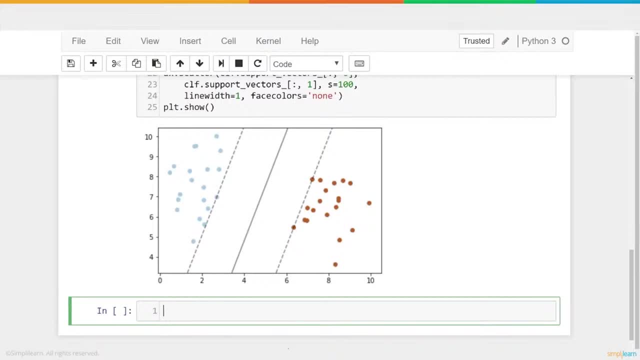 the near data, So you can see those two points, or in this case the four points where those lines nicely cleave the data, And then you have your hyperplane down the middle, which is as far from the two different points as possible, creating the maximum. 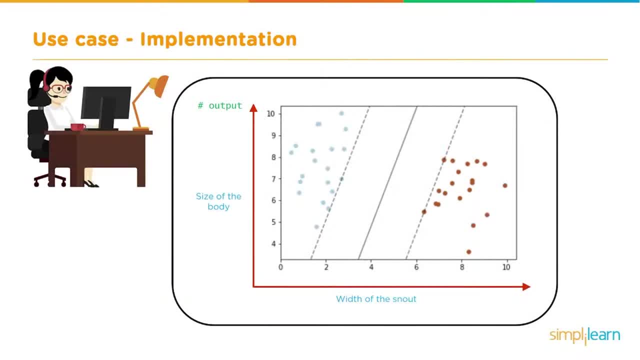 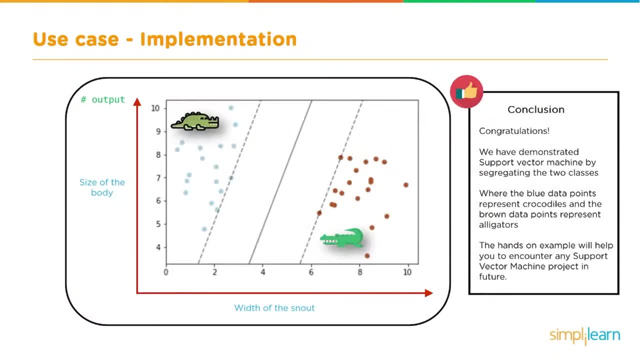 distance. So you can see that we have our nice output for the size of the body and the width of the snout, and we've easily separated the two groups of crocodile and alligator. Congratulations, You've done it, We've made it. 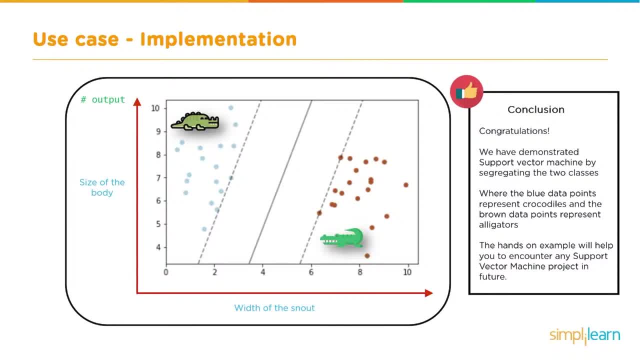 Of course, these are pretend data for our crocodiles and alligators, But this hands-on example will help you to encounter any support vector machine projects in the future And you can see how easy they are to set up and look at in depth. We're going to cover 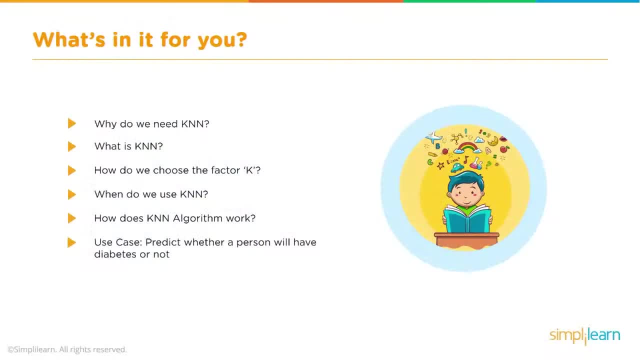 the k-nearest neighbors, a lot referred to as knn, And knn is really a fundamental place to start in the machine learning. It's the basis of a lot of other things. just the logic behind it is easy to understand and incorporated in other. 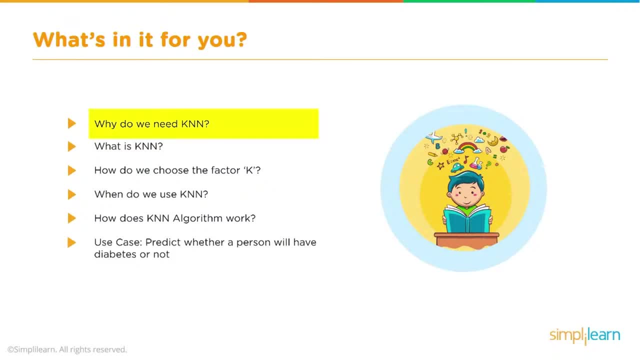 forms of machine learning. So, today, what's in it for you? Why do we need knn? What is knn? How do we choose the factor k? When do we use knn? How does knn algorithm work? And then we'll. 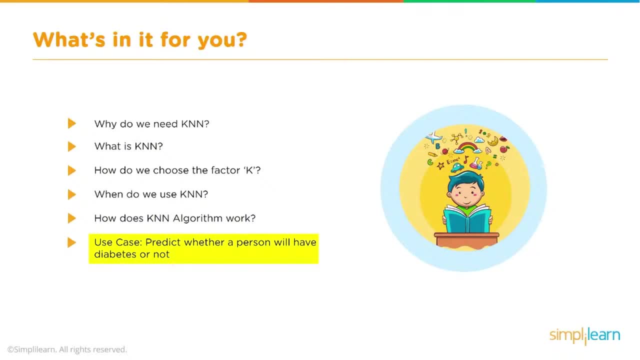 dive into my favorite part, the use case Predict whether a person will have diabetes or not. That is a very common and popular used data set. as far as testing out models and learning how to use the different models in machine learning, By now we all 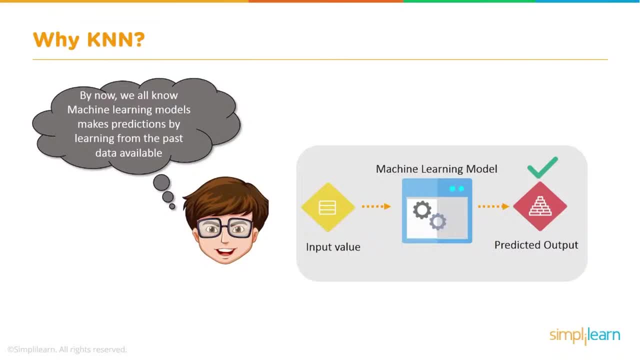 know. machine learning models make predictions by learning from the past data available. So we have our input values. our machine learning model builds on those inputs of what we already know and then we use that to create a predicted output. Is that a dog? Little kid looking? 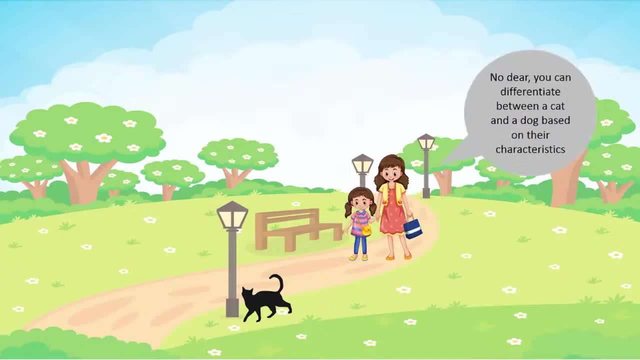 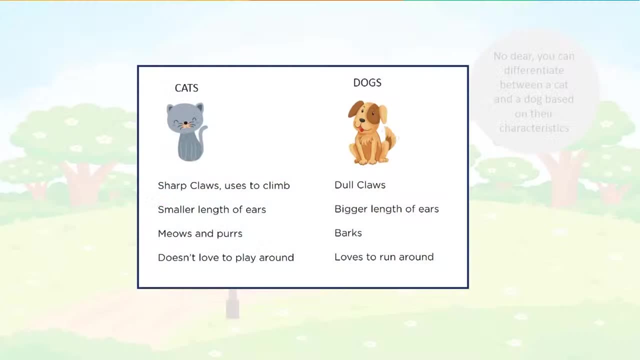 over there watching the black cat cross their path. No dear, you can differentiate between a cat and a dog based on their characteristics: Cats: Cats have sharp claws, uses to climb, smaller length of ears, meows and purrs. doesn't love to play around. 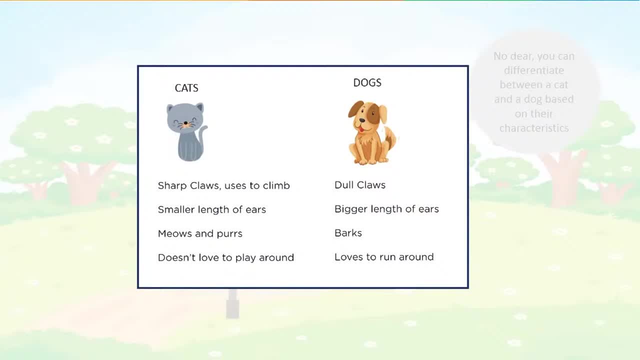 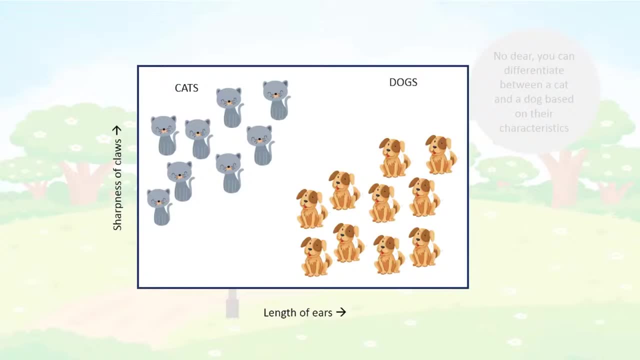 Dogs have dull claws, bigger length of ears, barks, loves to run around. You usually don't see a cat running around people, although I do have a cat that does that where dogs do, And we can look at these and say we can evaluate. 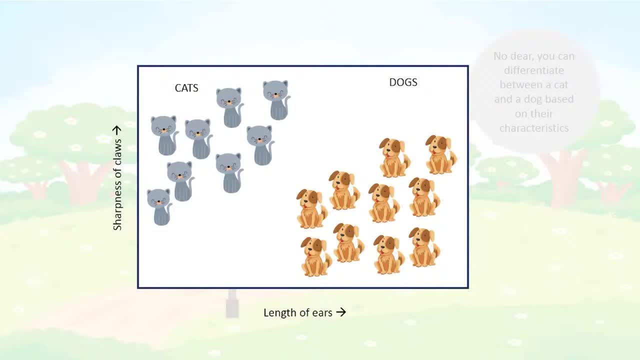 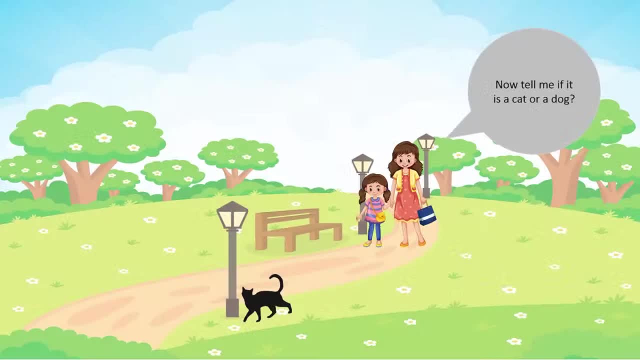 the sharpness of the claws. how sharp are their claws? and we can evaluate the length of the ears and we can usually sort out cats from dogs based on even those two characteristics. Now tell me if it is a cat or a dog. An odd question usually. 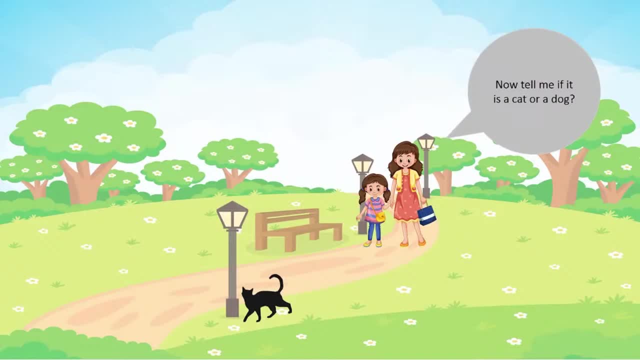 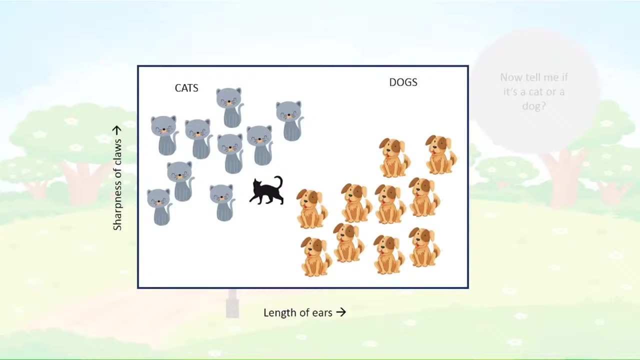 little kids know cats and dogs by now, Unless they live in a place where there's not many cats or dogs. So if we look at the sharpness of the claws, the length of the ears and we can see that the cat has smaller ears and sharper claws. 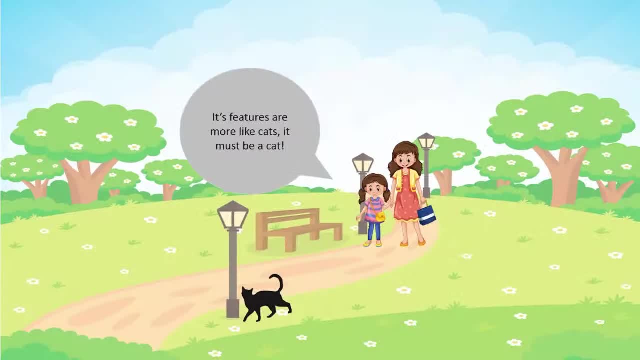 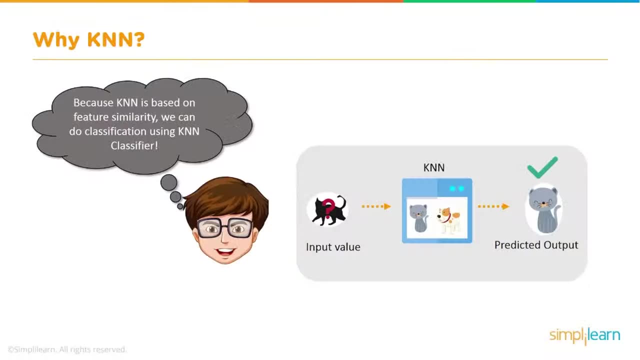 than the other animals. Its features are more like cats. it must be a cat- Sharp claws, length of ears- and it goes in the cat group. Because KNN is based on feature similarity, we can do classification using KNN classifier. So we have our 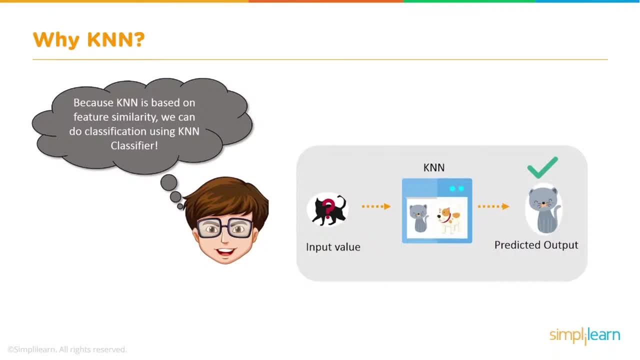 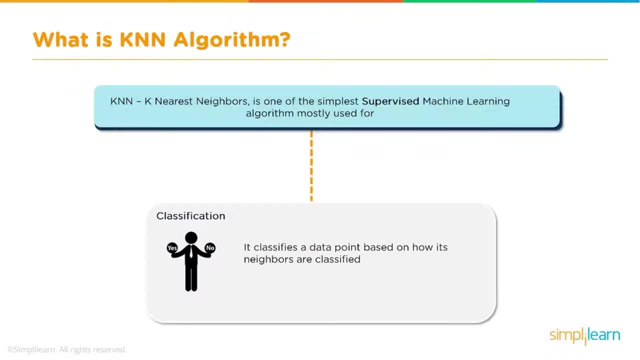 input value, the picture of the black cat. it goes into our trained model and it predicts that this is a cat coming out. So what is KNN? What is the KNN algorithm? K nearest neighbors is what that stands for. It's one of the simplest supervised. 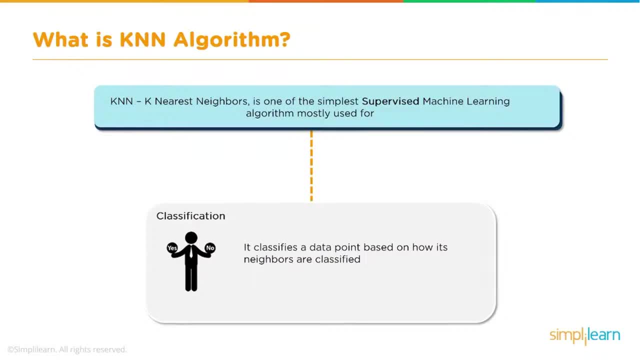 machine learning algorithms mostly used for classification. So we want to know: is this a dog or is it not a dog? Is it a cat or not a cat? It classifies a data point based on how its neighbors are classified. KNN stores. 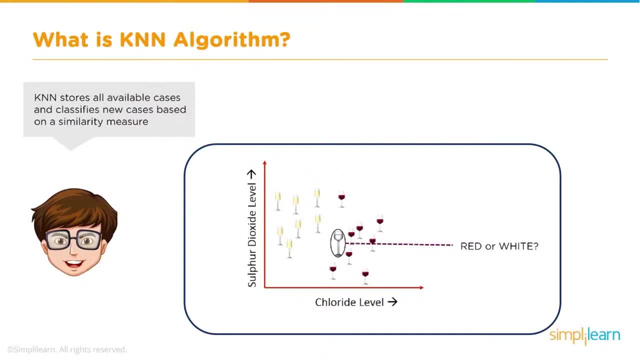 all available cases and classifies new cases based on a similarity measure. And here we've gone from cats and dogs right into wine. another favorite of mine, KNN, stores all available cases and classifies new cases based on a similarity measure. And here you see, we have a measurement. 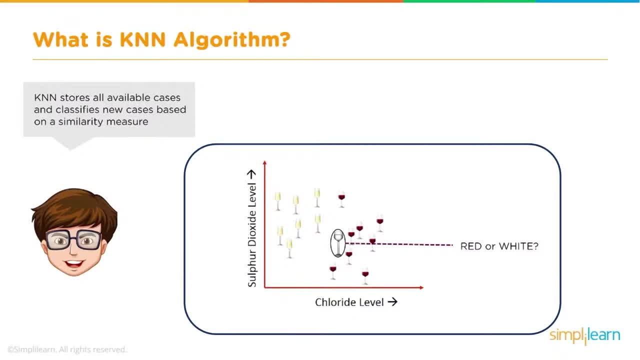 of sulfur dioxide versus the chloride level and then the different wines they've tested and where they fall on that graph based on how much sulfur dioxide and how much chloride. K and KNN is a perimeter that refers to the number of nearest neighbors to include in the majority. 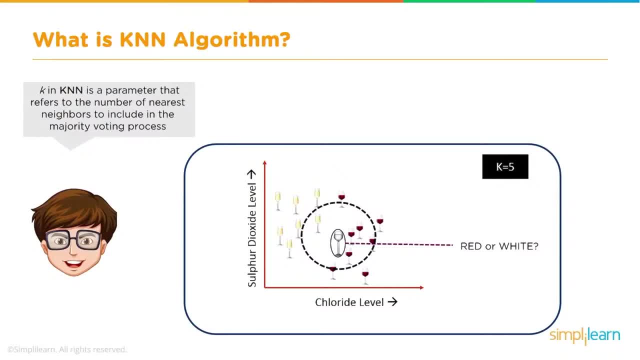 of the voting process, And so if we had a new glass of wine there, red or white- we want to know what the neighbors are. In this case, we're going to put K equals five. We'll talk about K in just a minute. A data point is classified. 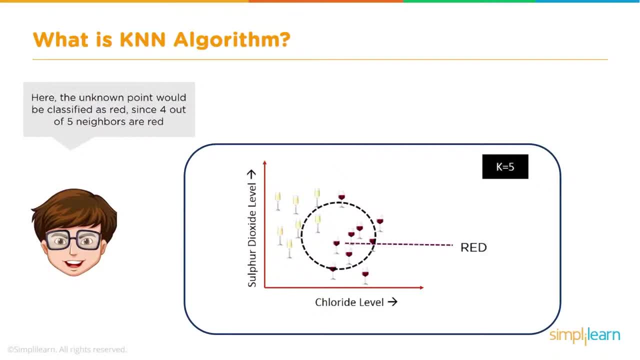 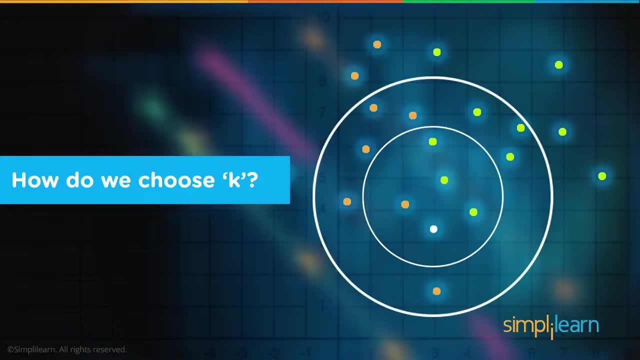 by the majority of votes from its five nearest neighbors. Here the unknown point would be classified as red, since four out of five neighbors are red. So how do we choose K? How do we know K equals five? I mean, that's what is the value we put in. 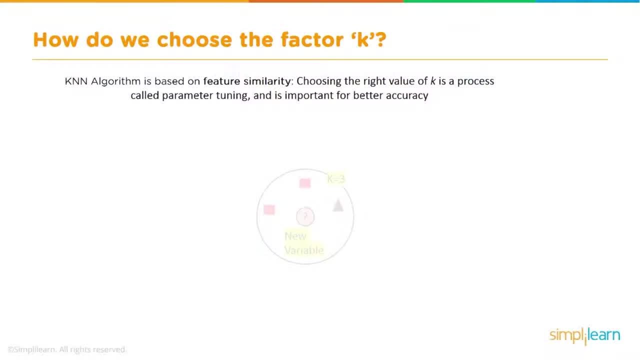 so we're going to talk about it. How do we choose the factor K? KNN algorithm is based on feature similarity. Choosing the right value of K is a process called parameter tuning and is important for better accuracy. So at K equals three, we can classify. we have a question. 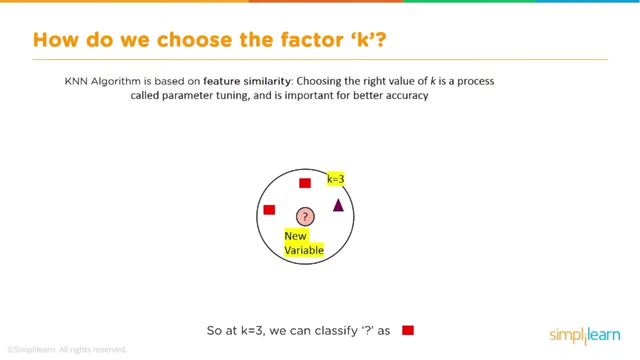 mark in the middle as either a square or not. Is it a square or is it, in this case, a triangle? And so if we set K equals to three, we're going to look at the three nearest neighbors. we're going to say: 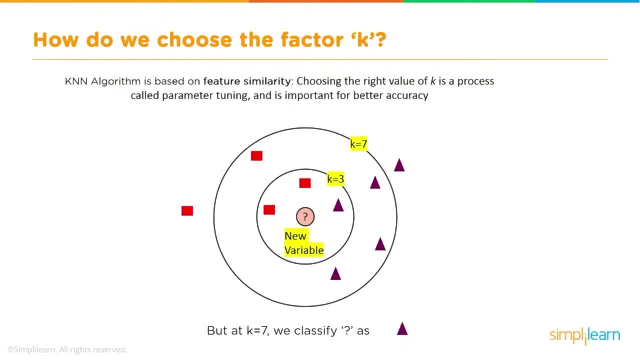 this is a square And if we put K equals to seven, we classify as a triangle depending on what the other data is around it And you can see as the K changes depending on where that point is. that drastically changes your answer. 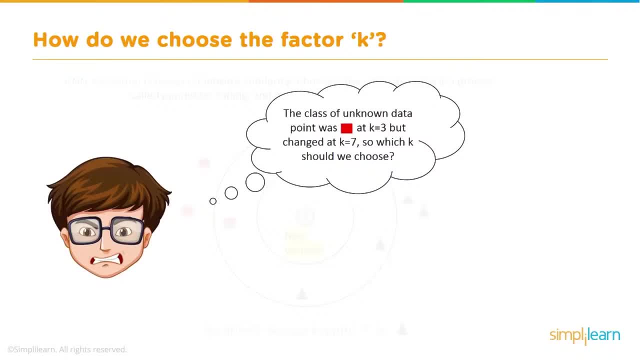 And we jump here and we go. how do we choose the factor of K? You'll find this in all machine learning: Choosing these factors, that's the face you get. It's like: oh my gosh, did I choose the right K, Did I? 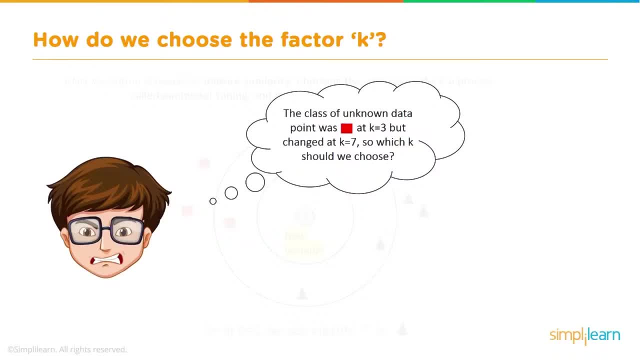 set it right my values in whatever machine learning tool you're looking at, so that you don't have a huge bias in one direction or the other. And in terms of KNN, the number of K, if you choose it too low, the bias. 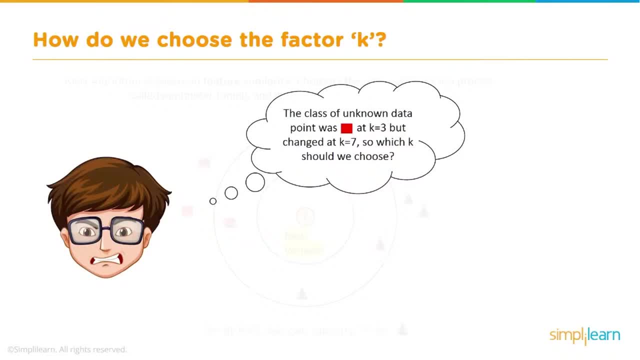 is based on. it's just too noisy. It's right next to a couple things and it's going to pick those things and you might get a skewed answer And if your K is too big then it's going to take forever to process. So you're going to run. 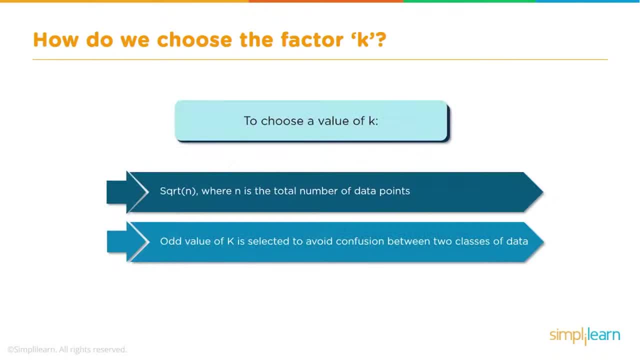 into processing issues and resource issues. So what we do, the most common use- and there's other options for choosing K- is to use the square root of N. So N is the total number of values you have. you take the square root of it. 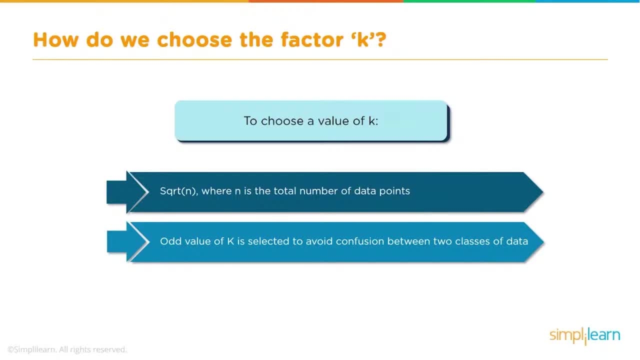 In most cases you also if it's an even number. so if you're using, like in this case, squares and triangles, if it's even, you want to make your K value odd. That helps it select better. So, in other words, you're not. 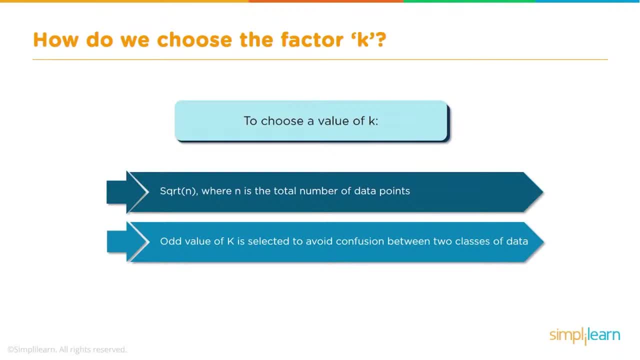 going to have a balance between two different factors that are equal. So usually take the square root of N and, if it's even you add one to it or subtract one from it, and that's where you get the K value from. That is the most common use and it's pretty solid. 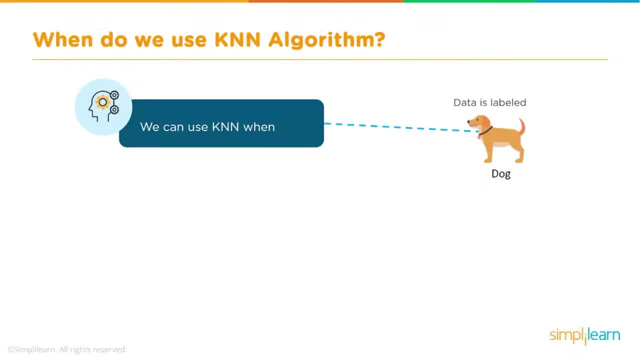 It works very well. When do we use KNN? We can use KNN when data is labeled, So you need a label on it. We know we have a group of pictures with dogs, dogs, cats, cats. Data is noise free And so you can see. 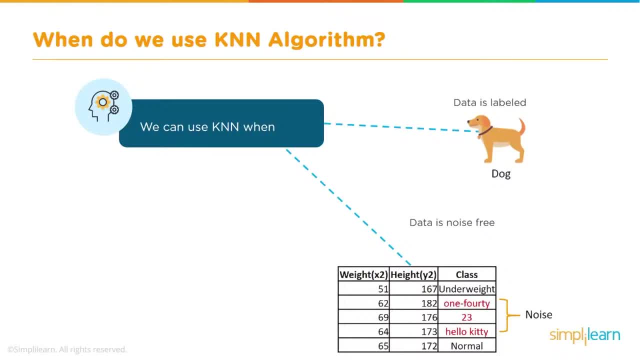 here when we have a class and we have, like, underweight 140,, 23,, hello kitty, normal, that's pretty confusing. We have a high variety of data coming in, So it's very noisy And that would cause an issue. 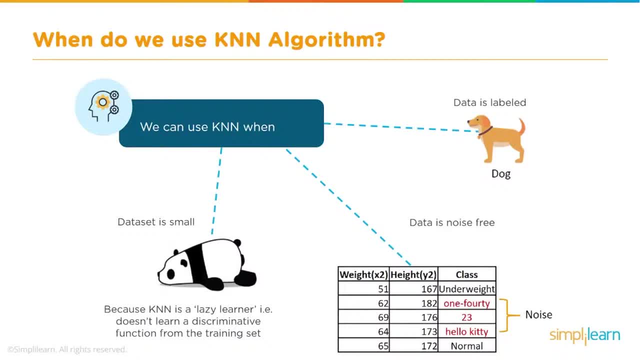 Data set is small, So we're usually working with smaller data sets where you might get into a gig of data if it's really clean, doesn't have a lot of noise, Because KNN is a lazy learner, ie it doesn't learn a. 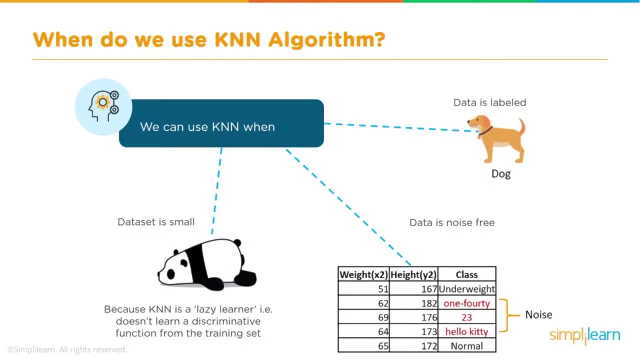 discriminative function from the training set, So it's very lazy. So if you have very complicated data and you have a large amount of it, you're not going to use the KNN, But it's really great to get a place to start. 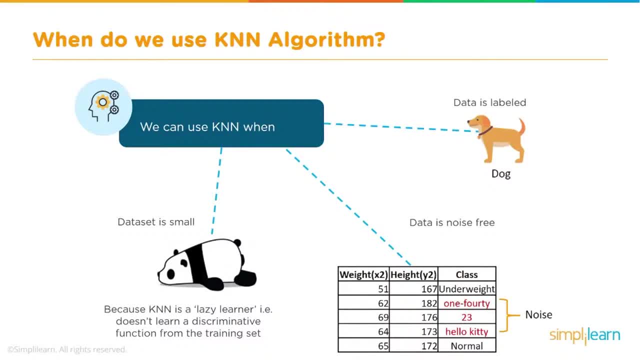 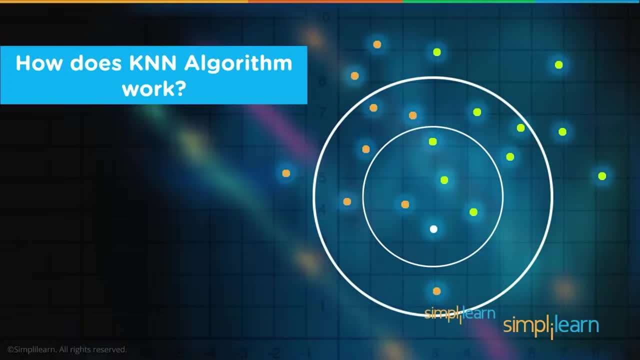 Even with large data, you can sort out a small sample and get an idea of what that looks like. using the KNN And also just using for smaller data sets, KNN works really good. How does a KNN algorithm work? Consider a data set having. 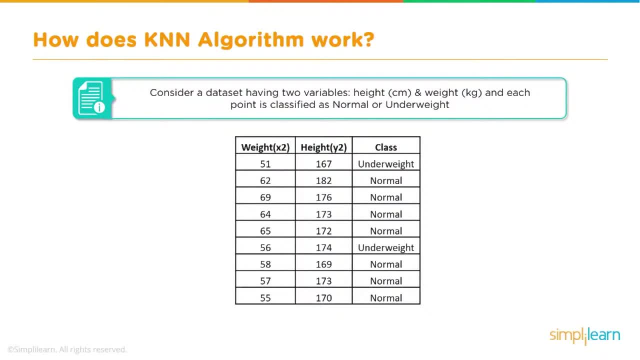 two variables: Height in centimeters and weight in kilograms, And each point is classified as normal or underweight. So we can see, right here we have two variables. You know, true, false, They're either normal or they're not. They're underweight. 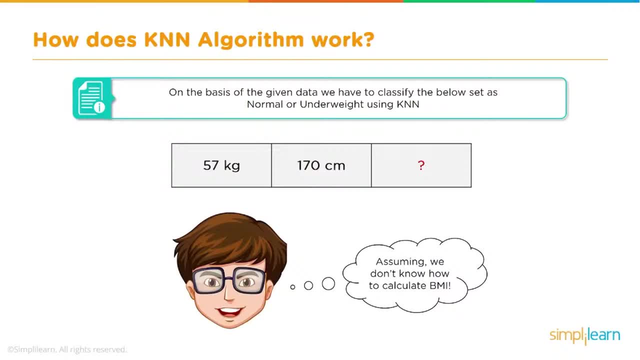 On the basis of the given data, we have to classify the below set as normal or underweight using KNN. So if we have new data coming in that says 57 kilograms and 177 centimeters, is that going to be normal or underweight? 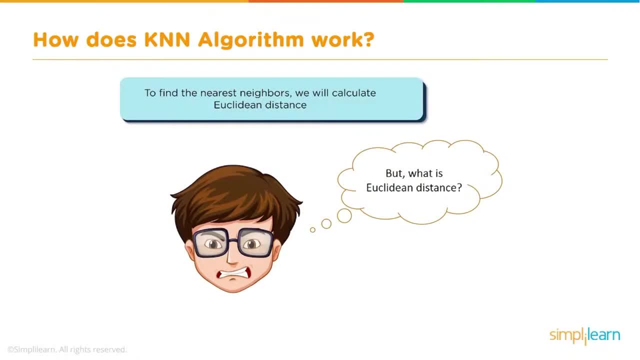 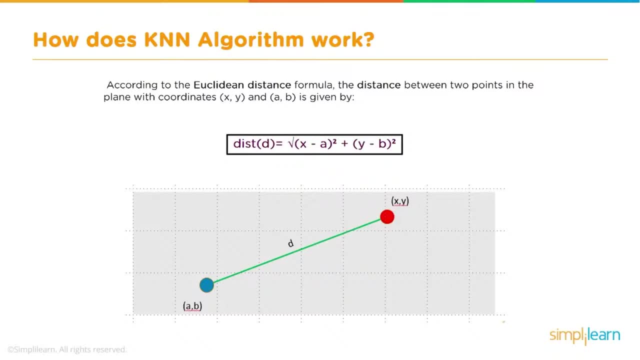 To find the nearest neighbors, we'll calculate the Euclidean distance According to the Euclidean distance formula. the distance between two points in the plane with the coordinates is given by distance. d equals the square root of x minus a squared, plus y minus b squared. 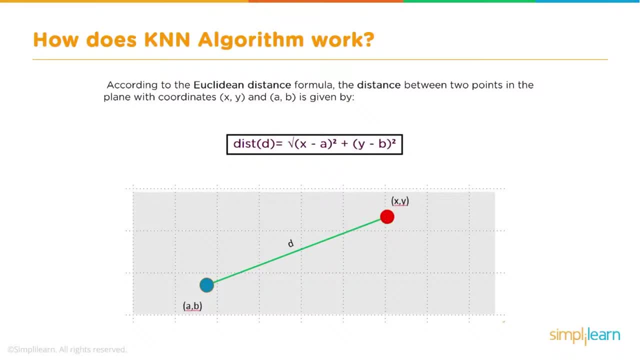 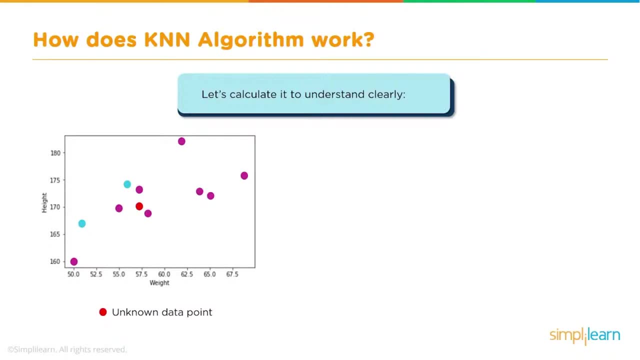 And you can remember that from the two edges of a triangle We're computing the third edge. since we know the x side and the y side, Let's calculate it to understand clearly. So we have our unknown point, We placed it there in red And we have. 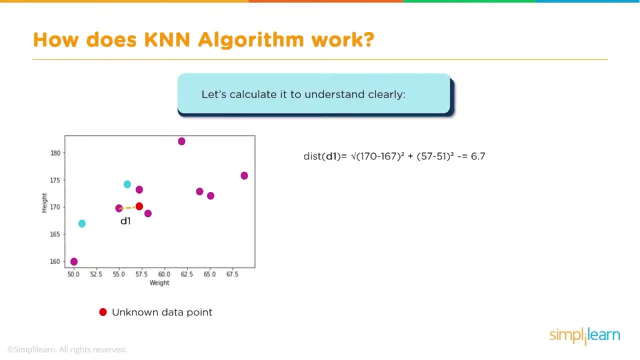 our other points where the data is scattered around. The distance d1 is the square root of 70 minus 167 squared, plus 57 minus 51 squared, which is about 6.7.. And distance 2 is about 13.. And distance 3 is about 13.4.. 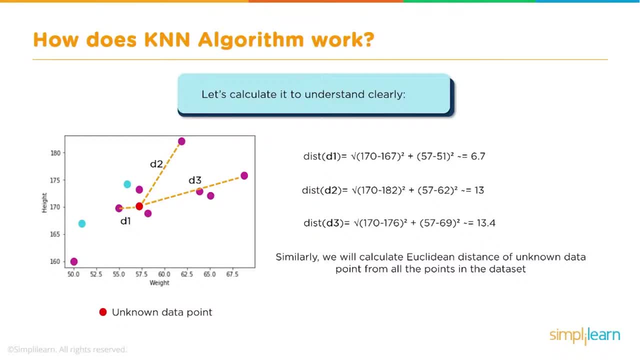 Similarly we will calculate the Euclidean distance of unknown data point from all the points in the data set And because we're dealing with small amount of data, that's not that hard to do. It's actually pretty quick for a computer And it's not really complicated math. So you can just see. 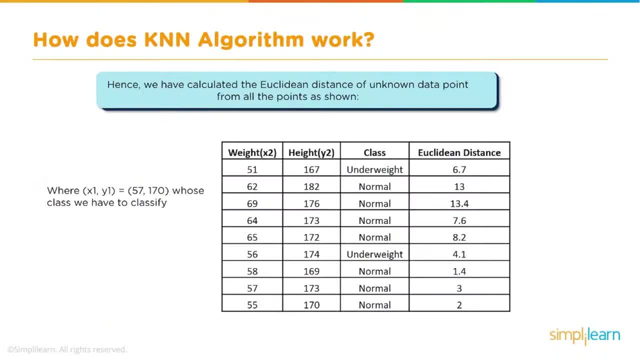 how close is the data based on the Euclidean distance. Hence we have calculated the Euclidean distance of unknown data point from all the points as shown, where x1 and y1 equal 57 and 170, whose class we have to classify. So now we're looking at that and we're saying 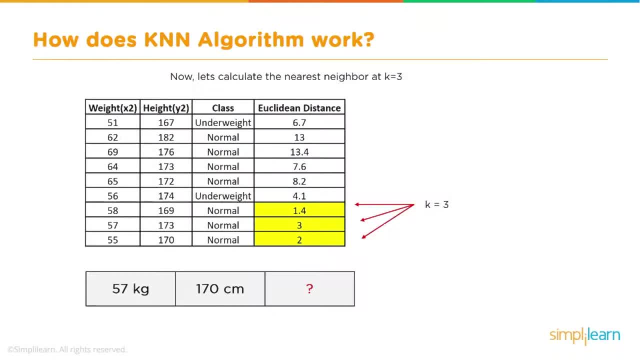 well, here's the Euclidean distance. Who's going to be their closest neighbors? Now, let's calculate the nearest neighbor at k equals 3. And we can see the three closest neighbors. puts them at normal And that's pretty self-evident. 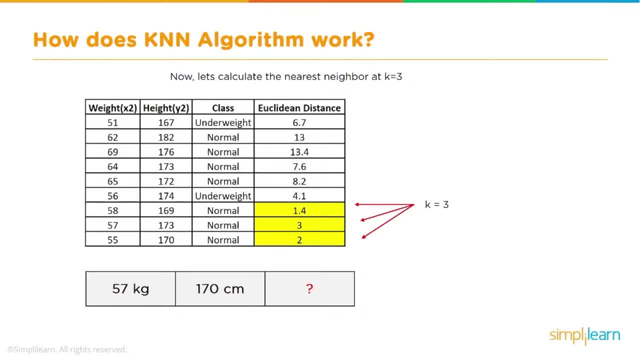 When you look at this graph, it's pretty easy to say: okay, we're just voting Normal, normal, normal. Three votes for normal. This is going to be a normal weight. So majority of neighbors are pointing towards normal Hence. 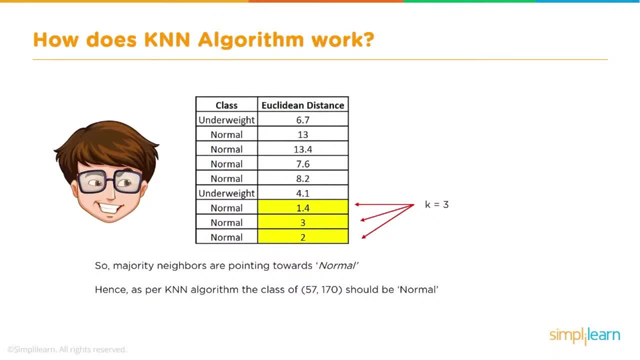 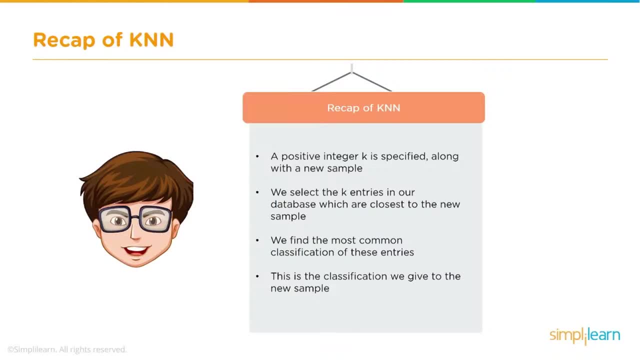 as per KNN algorithm, the class of 57 and 170 should be normal. So a recap of KNN Positive integer k is specified along with a new sample. We select the k entries in our database which are closest to the new sample. 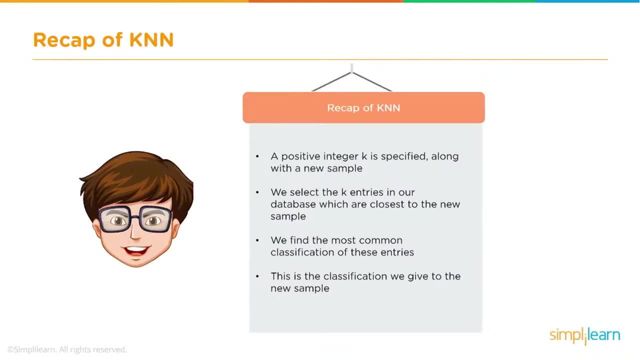 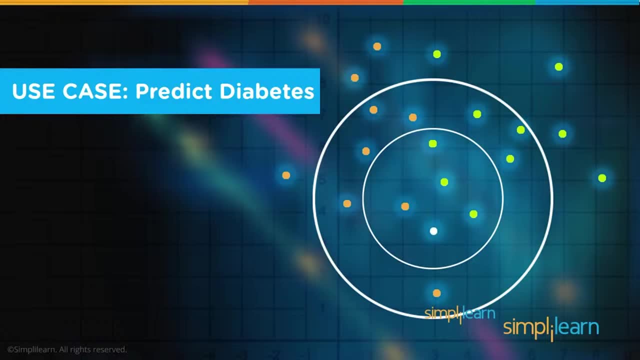 We find the most common classification of these entries. This is the classification we give to the new sample. So, as you can see, it's pretty straightforward. We're just looking for the closest things that match what we got. So let's take a look and see what that 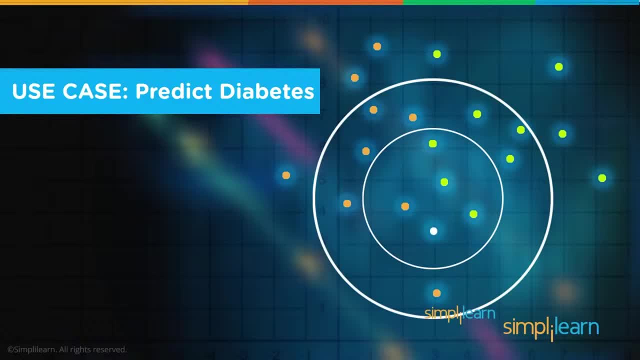 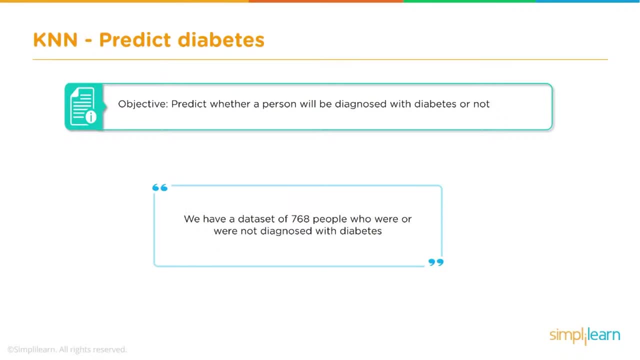 looks like in a use case in Python. So let's dive into the predict diabetes use case. So use case: predict diabetes. The objective: predict whether a person will be diagnosed with diabetes or not. We have a data set of 768 people who were or were. 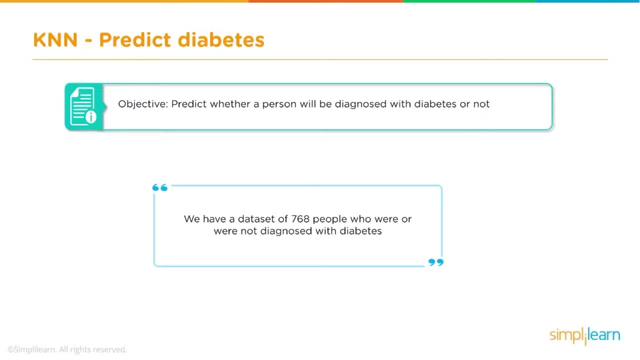 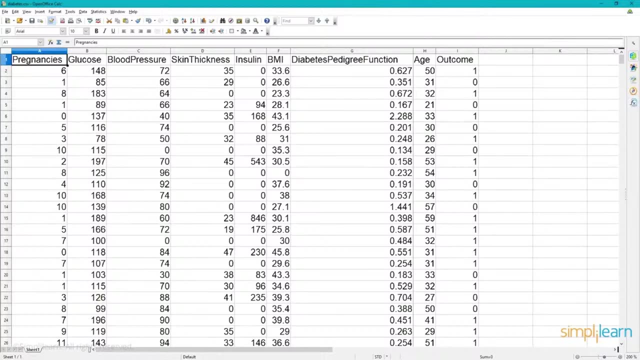 not diagnosed with diabetes. And let's go ahead and open that file and just take a look at that data. And this is in a simple spreadsheet format. The data itself is comma separated- Very common set of data And it's also a very common way to get the data. 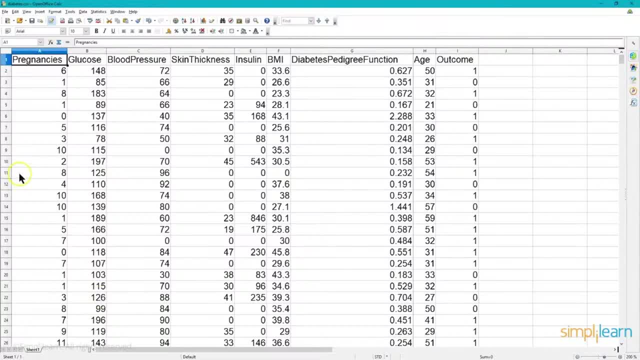 And you can see, here we have columns A through I. That's what: 1, 2, 3, 4, 5, 6,, 7, 8. Eight columns with a particular attribute, And then the ninth column. 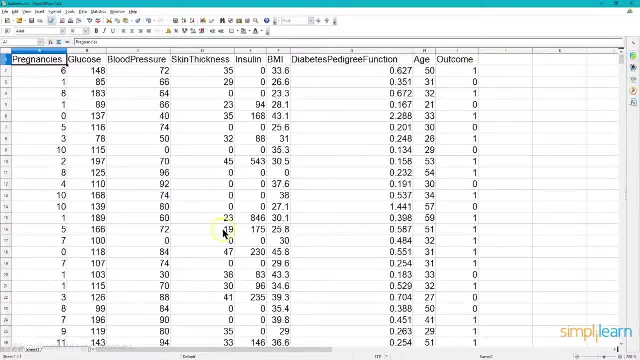 which is the outcome is whether they have diabetes. As a data scientist, the first thing you should be looking at is insulin. Well, you know, if someone has insulin, they have diabetes because that's why they're taking it, And that could cause issue in some of the machine learning. 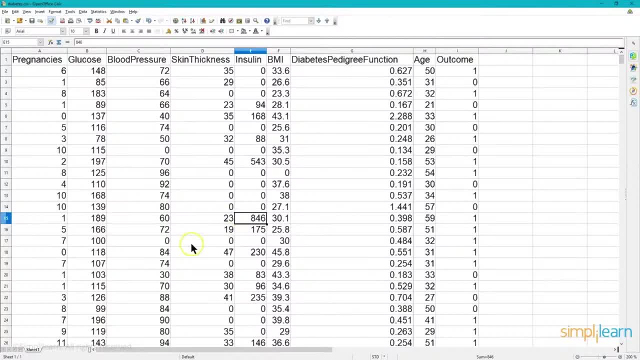 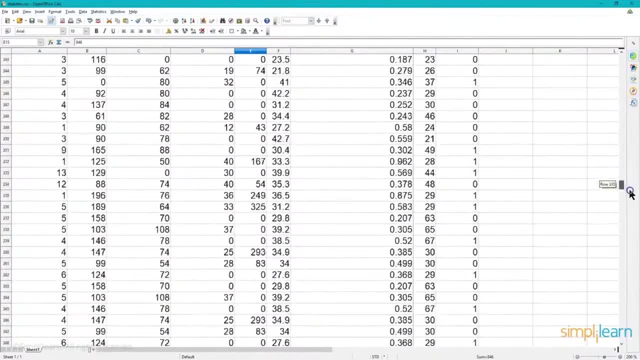 packages, But for a very basic setup. this works fine for doing the KNN And the next thing you notice is it didn't take very much to open it up. I can scroll down to the bottom of the data. There's 768.. 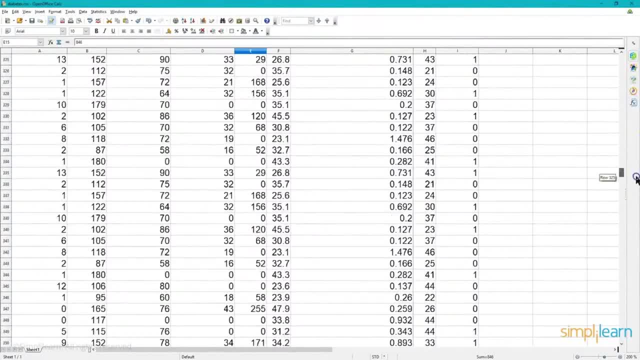 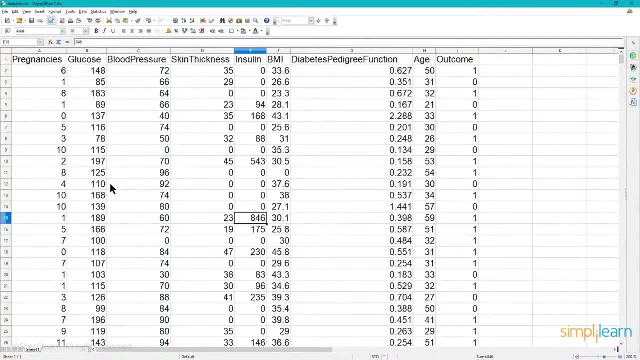 It's pretty much a small data set. You know, at 769. I can easily fit this into my RAM on my computer. I can look at it, I can manipulate it And it's not going to really tax, just a regular desktop computer. You don't even need an enterprise. 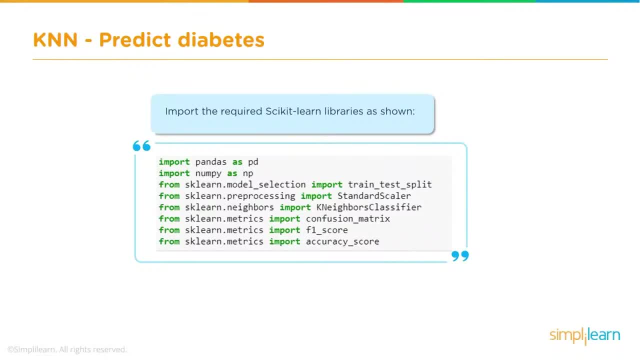 version to run a lot of this. So let's start with importing all the tools we need, And before that, of course, we need to discuss what IDE I'm using. Certainly, you can use any particular editor for Python, But I like to use for doing very basic. 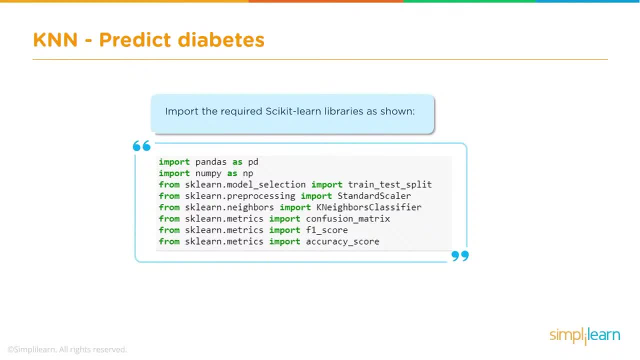 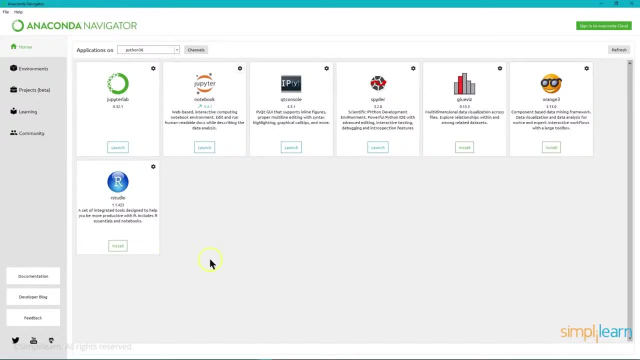 visual stuff: the Anaconda, which is great for doing demos with the Jupyter Notebook, And just a quick view of the Anaconda Navigator, which is the new release out there, which is really nice. You can see under home. I can choose my application. We're going to be using Python 3.6.. 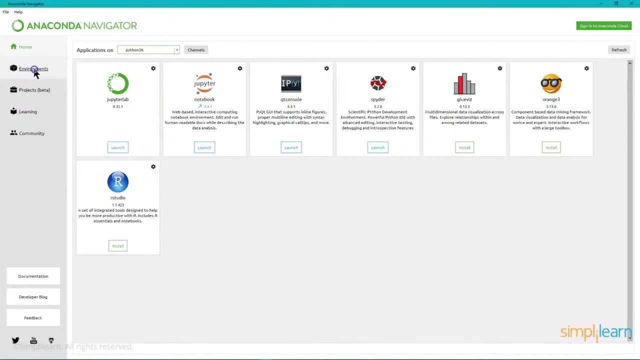 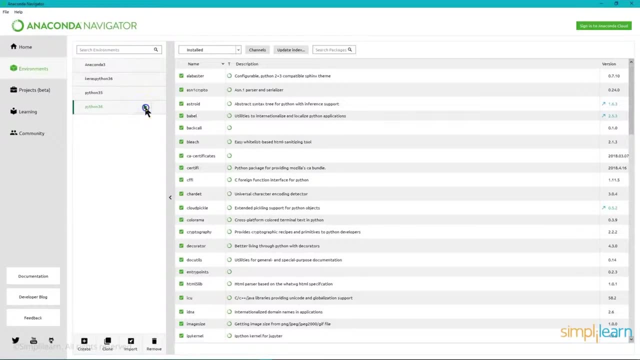 I have a couple different versions on this particular machine. If I go under environments, I can create a unique environment for each one, which is nice, And there's even a little button there where I can install different packages. So if I click on that button and open the, 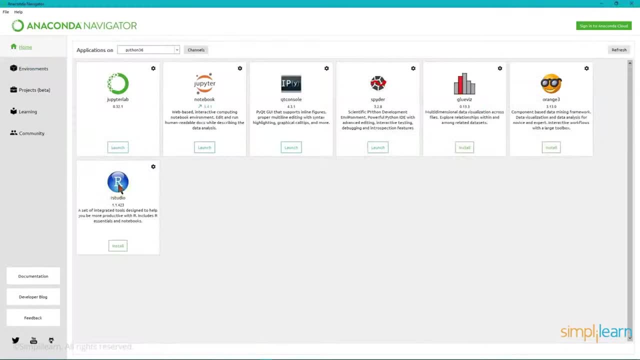 terminal. I can then use a simple pip install to install different packages I'm working with. Let's go ahead and go back under home and we're going to launch our notebook And I've already kind of like the old cooking shows. I've already 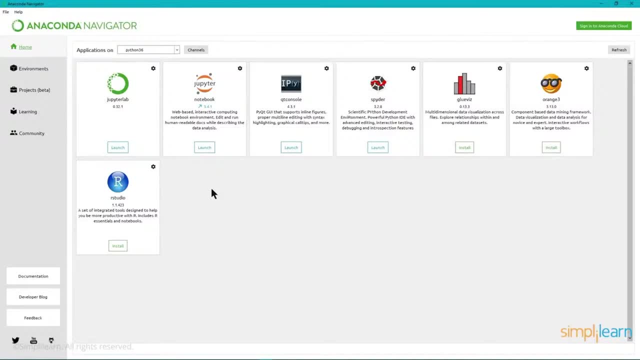 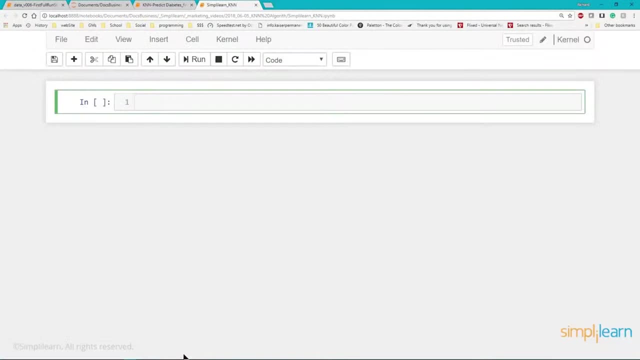 prepared a lot of my stuff, so we don't have to wait for it to launch, because it takes a few minutes for it to open up a browser window. In this case, I'm going to open up Chrome because that's my default that I use And since the script is pre-done. 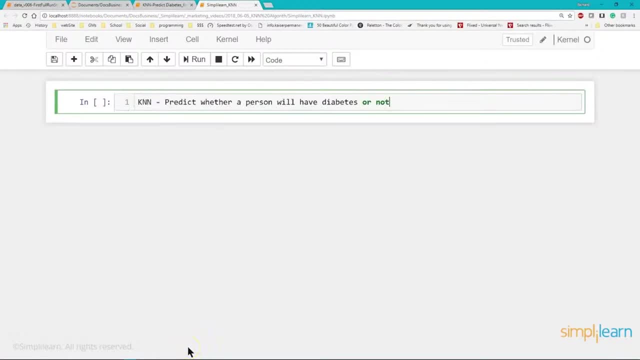 we're working in And since we're working on the KNN predict whether a person will have diabetes or not, let's go ahead and put that title in there, And I'm also going to go up here and click on cell. Actually, we want to go ahead. 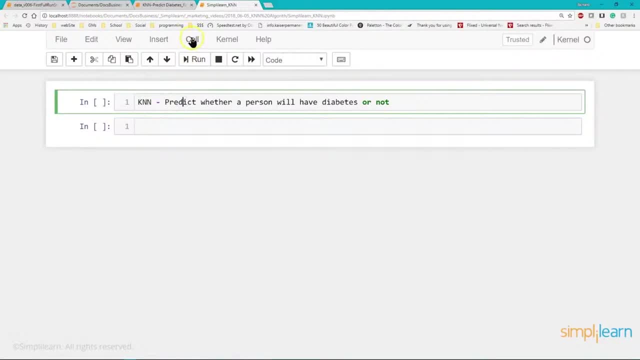 and first insert a cell below And then I'm going to go back up to the top cell and I'm going to change the cell type to markdown. That means this is not going to run as Python. It's a markdown language, So if I run this first one, it 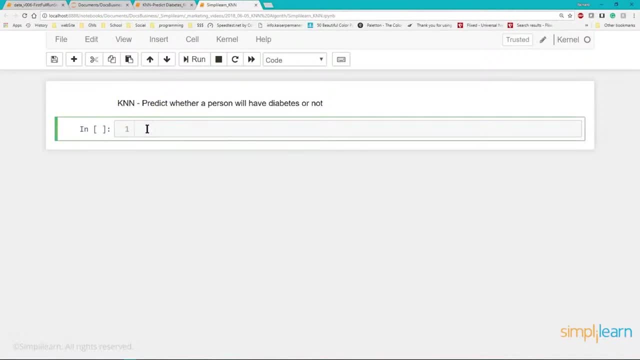 comes up in nice big letters, which is kind of nice, Reminds us what we're working on And by now you should be familiar with doing all of our imports. We're going to import the pandas as pd Import numpy, as np. Pandas is the pandas. 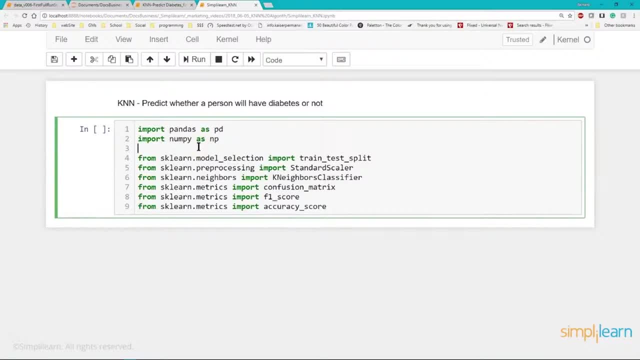 data frame and numpy is the number array, Very powerful tools to use in here. So we have our imports, So we've brought in our pandas, our numpy, our two general Python tools, And then you can see over here we have our train test split. 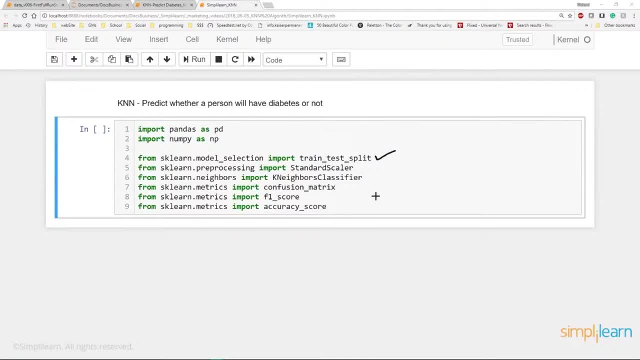 By now you should be familiar with splitting the data. We want to split part of it for training our thing and then training our particular model, And then we want to go ahead and test the remaining data to see how good it is Pre-processing a standard scalar pre-processor. 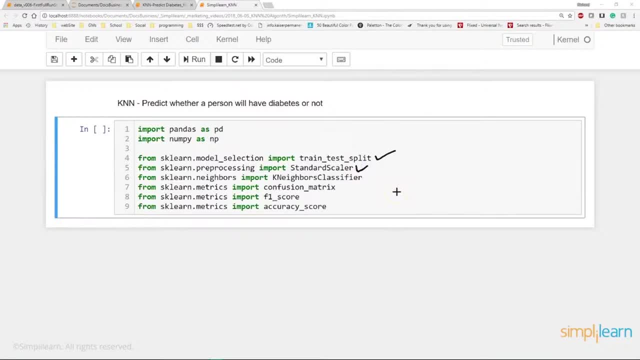 so we don't have a bias of really large numbers. Remember, in the data we had like number of pregnancies isn't going to get very large, where the amount of insulin they take can get up to 256. So 256 versus 6, that will skew results. So we 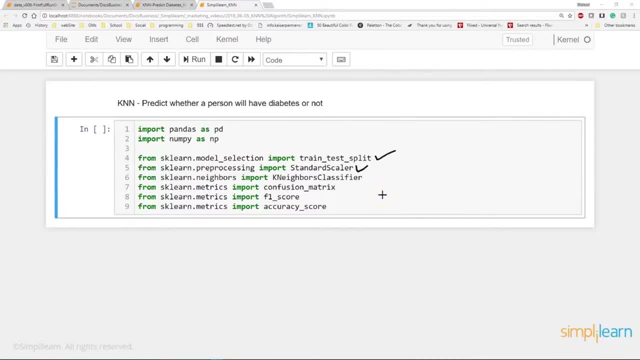 want to go ahead and change that so that they're all uniform between minus 1 and 1.. And then the actual tool. This is the k-neighbors classifier we're going to use. And finally, the last three are three tools to test. All about testing our 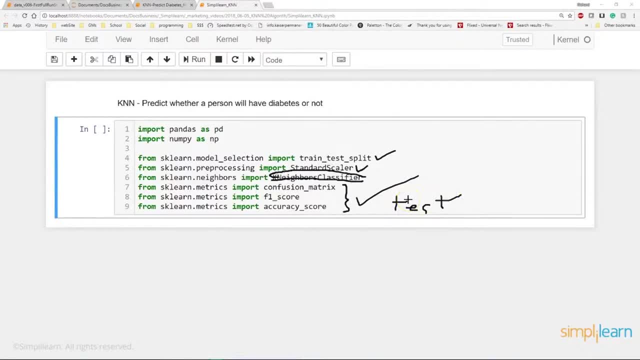 model. How good is it? Let me just put down test on there. And we have our confusion matrix, our F1 score and our accuracy. So we have our two general Python modules we're importing and then we have our six modules specific from the sklearn. 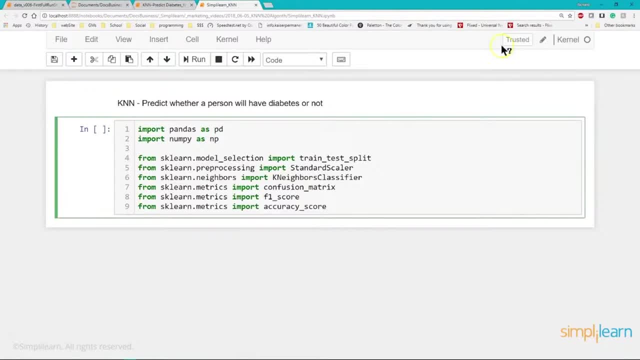 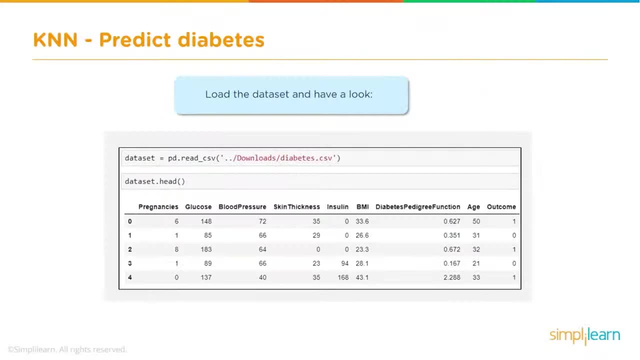 setup And then we do need to go ahead and run this so that these are actually imported. There we go And then move on to the next step, And so in this set we're going to go ahead and load the database We're going to use. 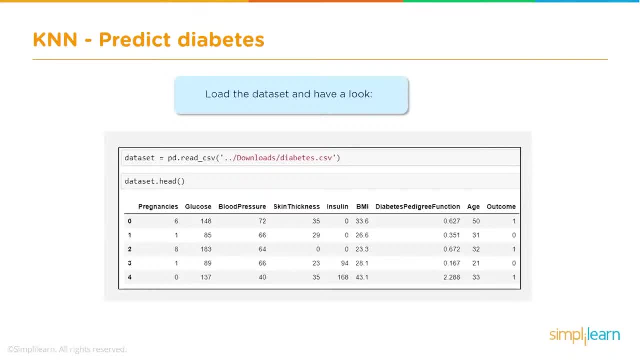 pandas. Remember, pandas is pd, And we'll take a look at the data in Python. We looked at it in a simple spreadsheet, But usually I like to also pull it up so that we can see what we're doing. So here's our 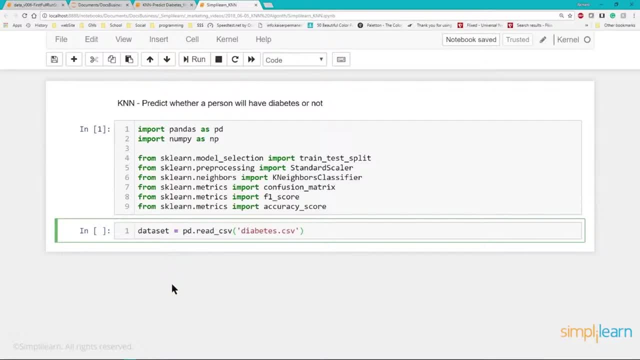 dataset equals pd dot. read csv. That's a pandas command. And the diabetes folder I just put in the same folder where my IPython script is. If you put it in a different folder you'd need the full length on there. We can also do a quick length. 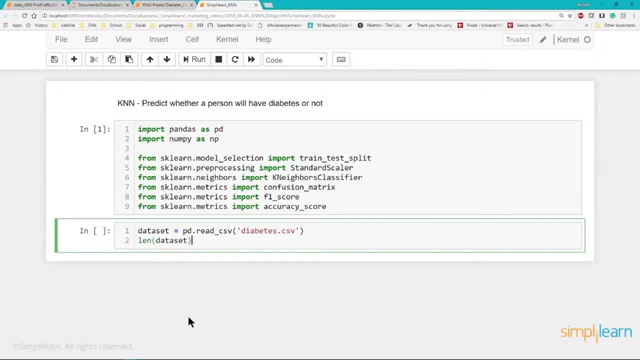 of the dataset. That is a simple Python command. Again, for length, We might even let's go ahead and print that We'll go print And if you do it on its own line length dot dataset in the Jupyter Notebook, it'll automatically. 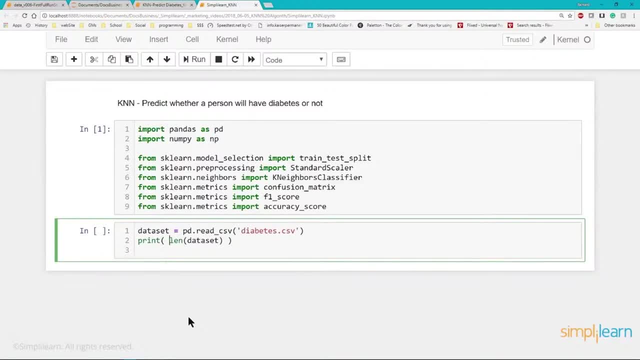 print it, But when you're in most of your different setups, you want to do the print in front of there, And then we want to take a look at the actual dataset And since we're in pandas, we can simply do dataset head And again. 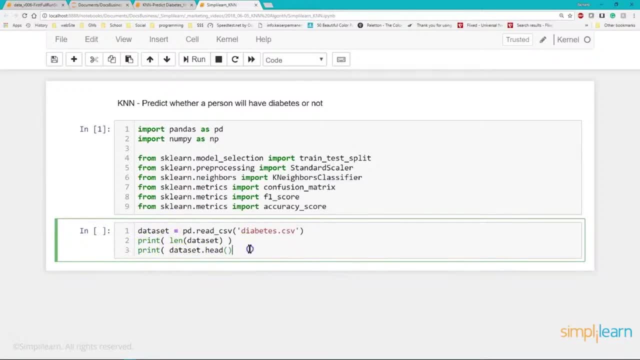 let's go ahead and add the print in there. If you put a bunch of these in a row, you know the dataset one head, dataset two head. it only prints out the last one. So I usually always like to keep the print statement in there. But 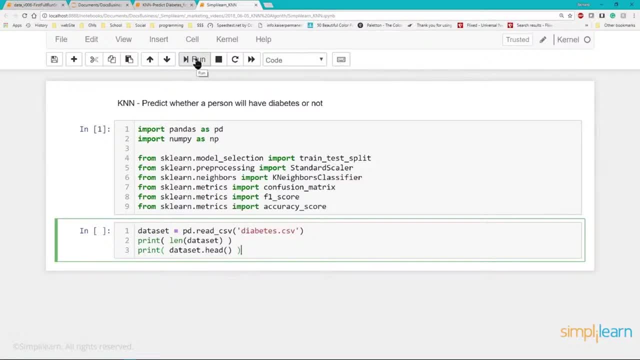 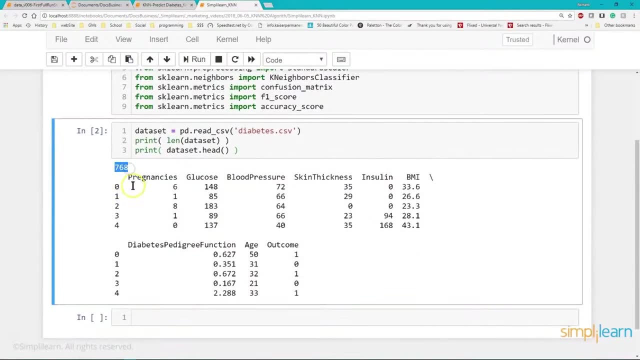 because most projects only use one data frame, pandas data frame. doing it this way doesn't really matter. The other way works just fine And you can see when we hit the run button we have the 768 lines which we knew And we have our 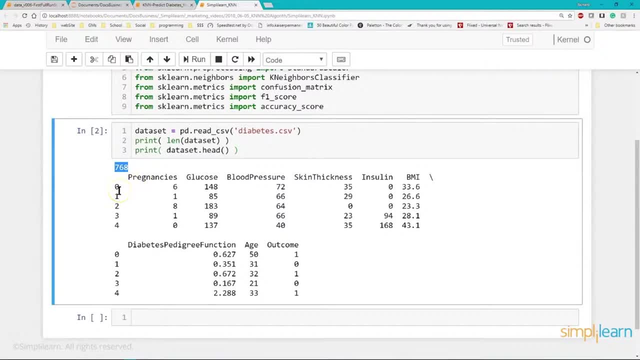 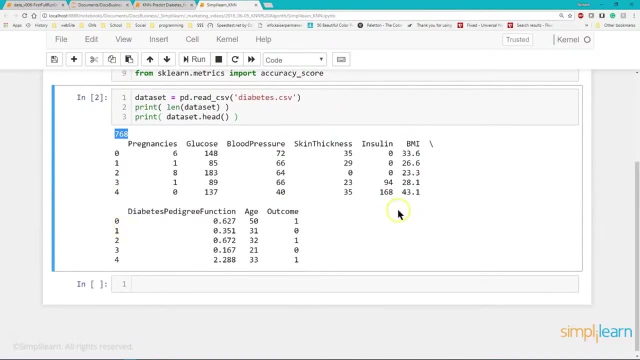 pregnancies It's automatically given a label on the left. Remember, the head only shows the first five lines, So we have zero through four And just a quick look at the data you can see it matches what we looked at before We have pregnancy. 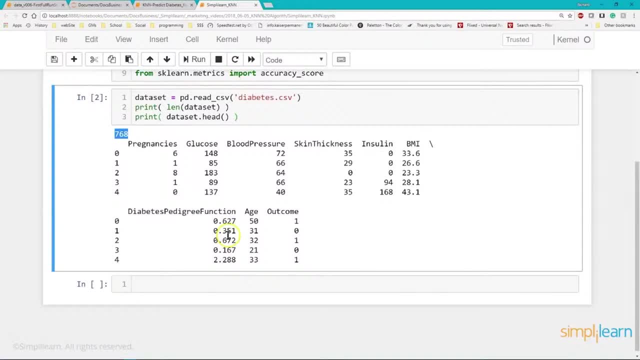 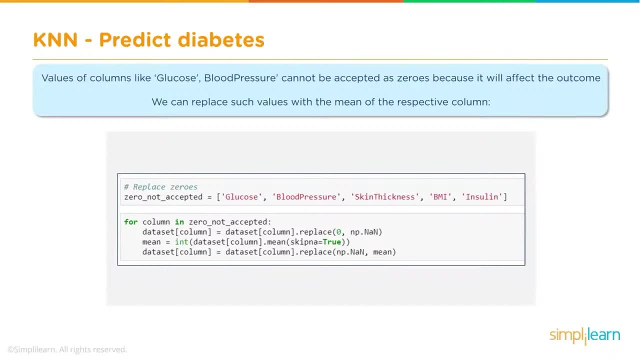 glucose blood pressure all the way to age, And then the outcome on the end. And we're going to do a couple things in this next step. We're going to create a list of columns where we can't have zero. There's no such thing as zero skin thickness. 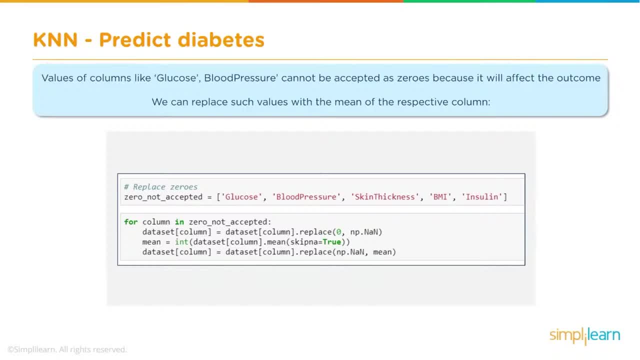 or zero blood pressure, zero glucose- Any of those you'd be dead, So not a really good factor. if they have a zero in there because they didn't have the data- And we'll take a look at that because we're going to start replacing that- 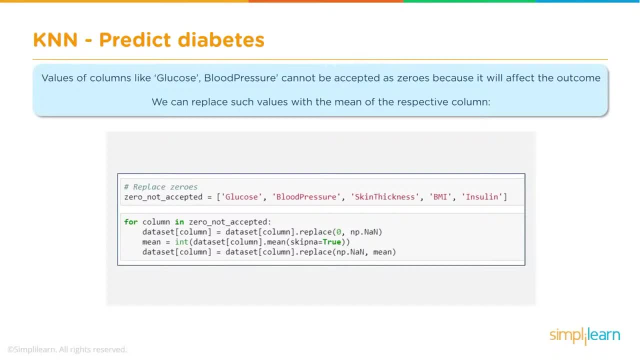 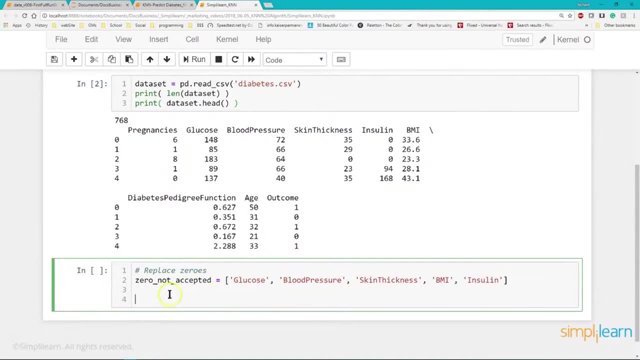 information with a couple of different things, And let's see what that looks like. So first, we create a nice list. as you can see, We have the values we talked about- glucose, blood pressure, skin thickness- And this is a nice way. 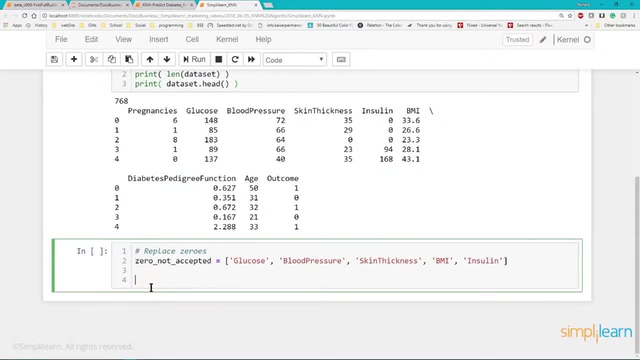 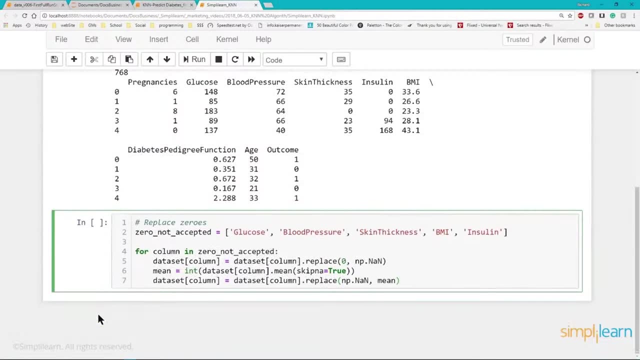 when you're working with columns is to list the columns. you need to do some kind of transformation on A very common thing to do, And then, for this particular setup, we certainly could use the. there's some panda tools that will do a lot of this. 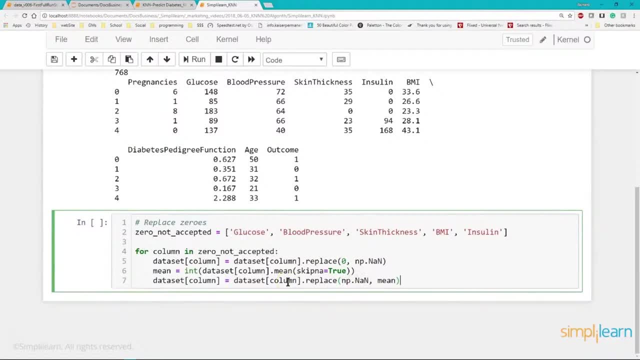 where we can replace the NA, But we're going to go ahead and do it as a data set column equals data set column dot replace. This is still pandas. You can do it direct. There's also one that you look for your NAN. A lot of different options. 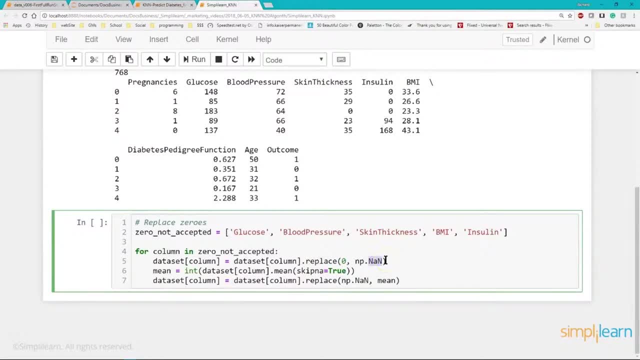 in here. But the NAN- numpy- NAN is what that stands for- is none- doesn't exist. So the first thing we're doing here is we're replacing the zero with a numpy none. There's no data there. That's what that says. That's what this is saying right here. 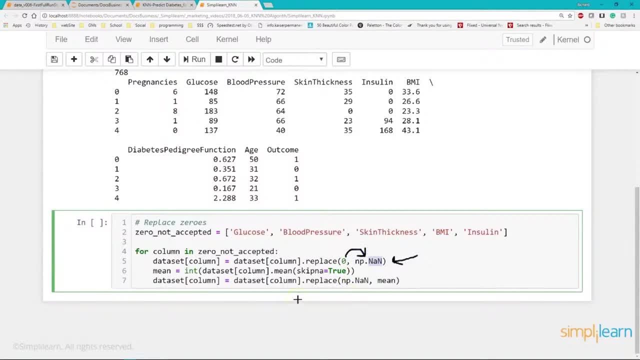 So put the zero in and we're going to replace zeros with no data. So if it's a zero, that means the person's well, hopefully, not dead. Hopefully, they just didn't get the data. The next thing we want to do is we're. 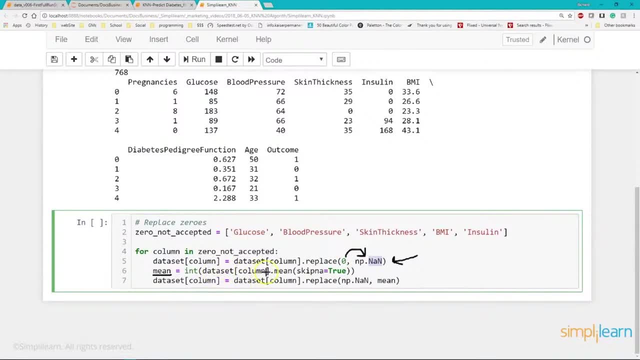 going to create the mean, which is the integer from the data set, from the column dot mean where we skip NAs. We can do that. That is a pandas command there, the skip NA. So we're going to figure out the mean of that data set And then we're going to take 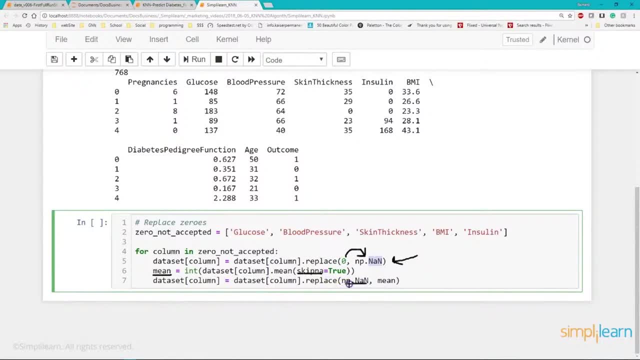 that data set column and we're going to replace all the NPNAN with the means. Why did we do that? We could have actually just taken this step and gone right down here and just replaced zero and skip anything where except you could actually. 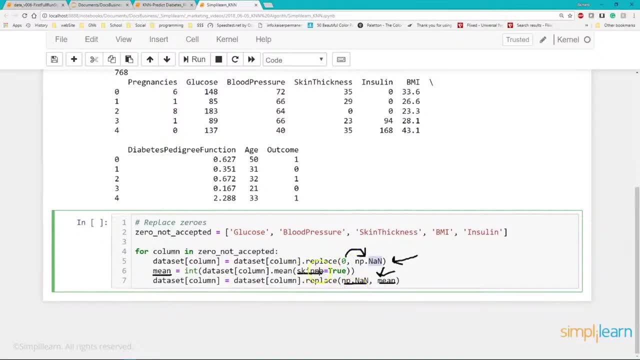 there's a way to skip zeros and then just replace all the zeros, But in this case we want to go ahead and do it this way, So you can see that we're switching this to a non-existent value. Then we're going to create the mean. 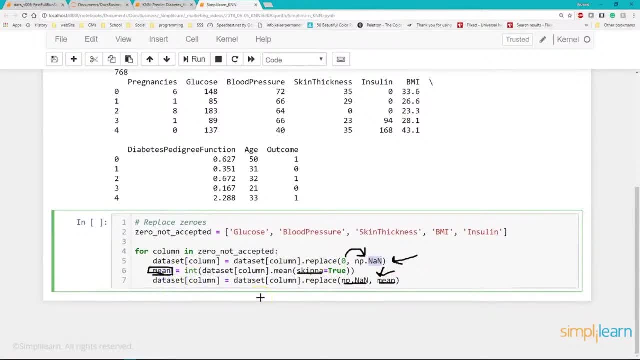 Well, this is the average person. So if we don't know what it is, if they did not get the data and the data's missing, one of the tricks is you replace it with the average- What is the most common data for that. This way, you can still. 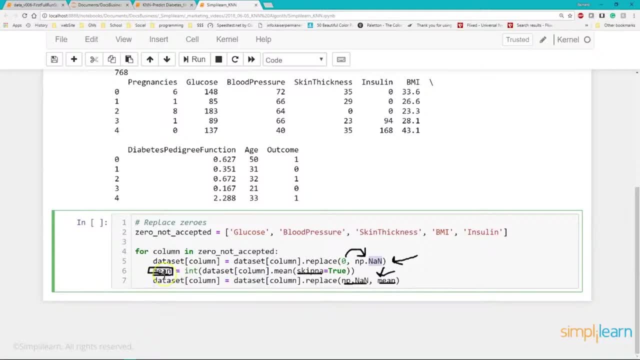 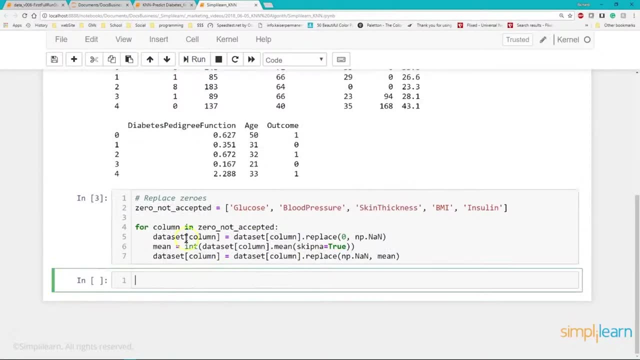 use the rest of those values to do your computation and it kind of just brings that particular value, those missing values, out of the equation. Let's go ahead and take this and we'll go ahead and run it. It doesn't actually do anything, so we're still. 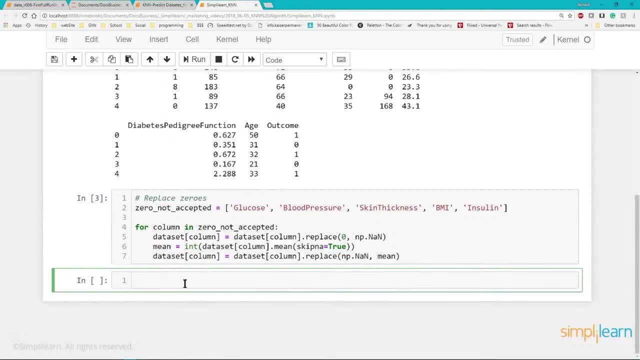 preparing our data. If you wanted to see what that looks like, we don't have anything in the first few lines, so it's not going to show up, But we certainly could look at a row. Let's do that. Let's go into. 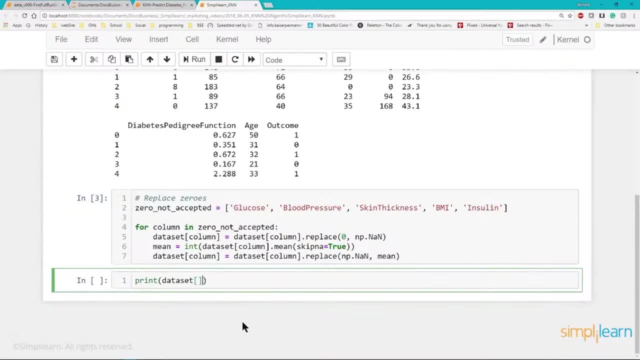 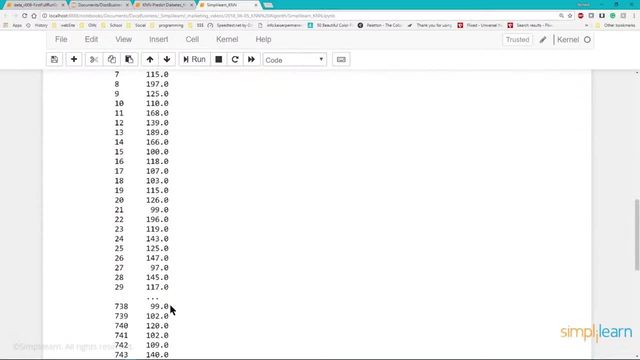 our data set. Let's print a data set And let's pick- in this case let's just do glucose- And if I run this, this is going to print all the different glucose levels going down And we, thankfully, don't see anything. 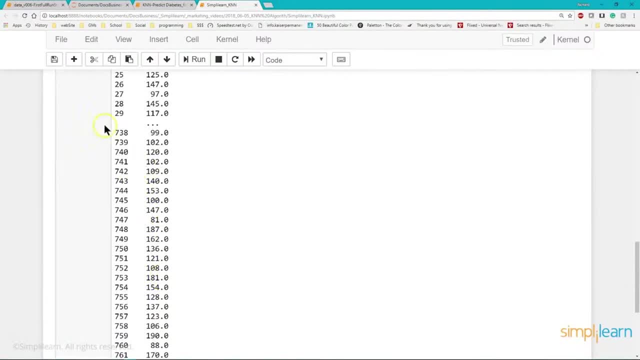 in here. that looks like missing data. At least on the ones it shows You can see it's left a bunch in the middle, Because that's what it does. If you have too many lines in Jupyter Notebook, it'll skip a few and go on to the next. 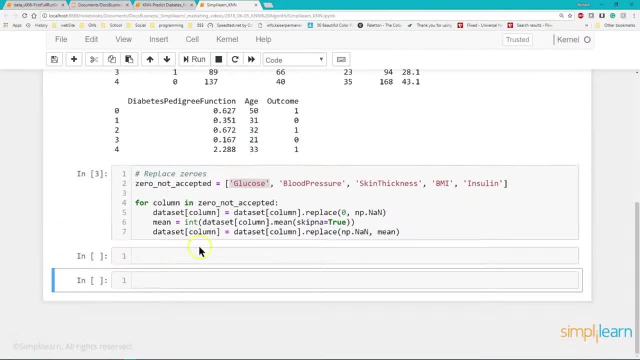 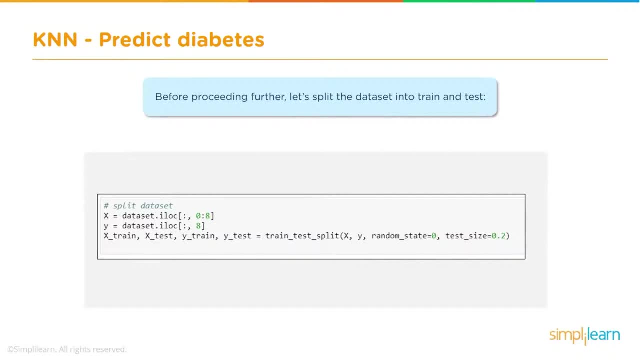 in a data set. Let me go ahead and remove this And we'll just zero out that. And, of course, before we do any processing, before proceeding any further, we need to split the data set into our train and testing data. That way we have. 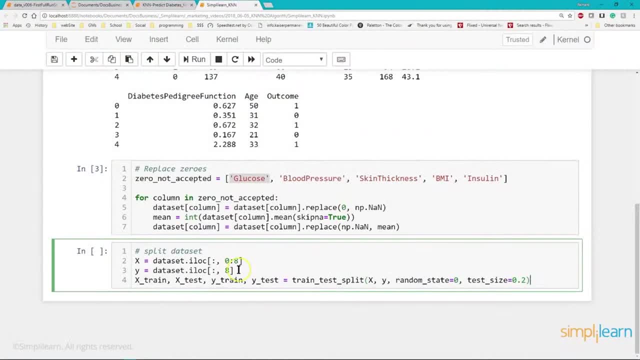 something to train it with and something to test it on. And you're going to notice we did a little something here with the Pandas database code. There we go, my drawing tool. We've added in this right here off the data set. 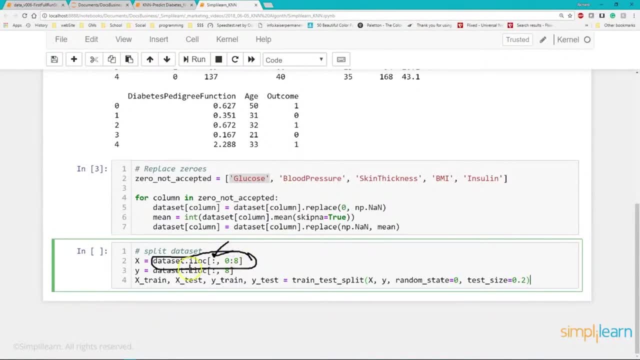 And what this says is that the first one in Pandas- this is from the PD Pandas- it's going to say, within the data set, we want to look at the I location and it is all rows. That's what that says. So we're going to keep. 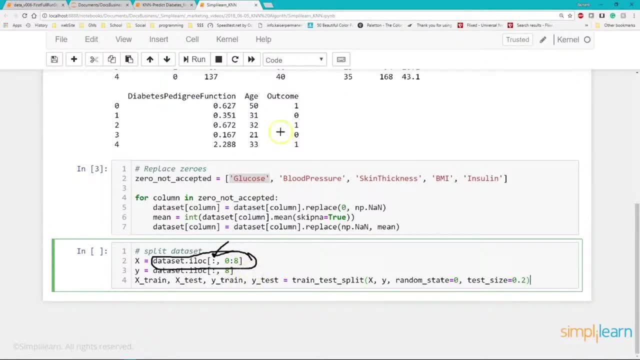 all the rows, But we're only looking at zero, column zero to eight. Remember column nine? here it is, right up here, we printed it in. here is outcome. Well, that's not part of the training data, that's part of the 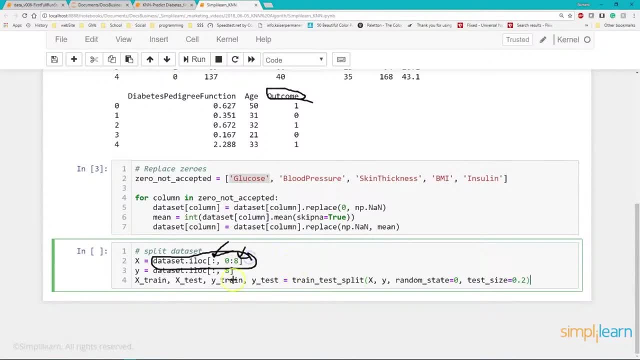 answer: Yes, column nine, but it's listed as eight number eight. So zero to eight is nine columns, So eight is the value And when you see it in here, zero. this is actually zero to seven. It doesn't include 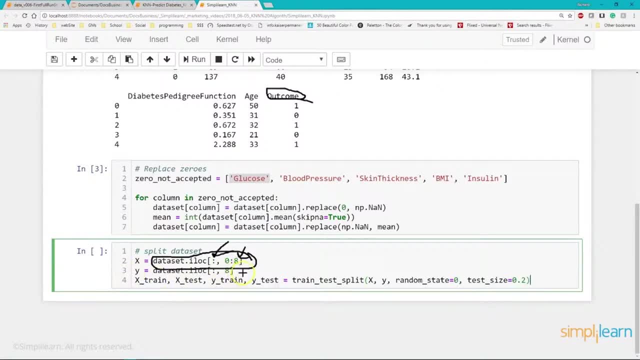 the last one, And then we go down here to y, which is our answer, and we want just the last one, Just column eight, And you can do it this way with this particular notation. And then, if you remember, we imported the train. 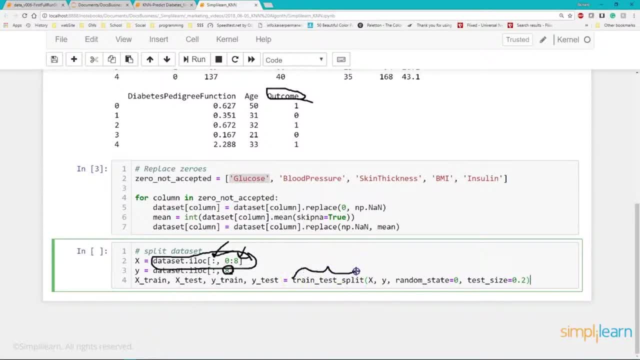 test split. That's part of the sklearn right there And we simply put in our x and our y. We're going to do random. state equals zero. You don't have to necessarily seed it. That's a seed number, I think the default. 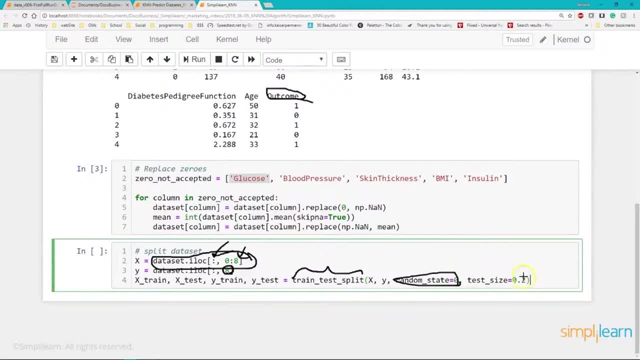 is one when you seed it. I'd have to look that up. And then the test size. Test size is .2.. That simply means we're going to take 20% of the data and put it aside so that we can test it later. 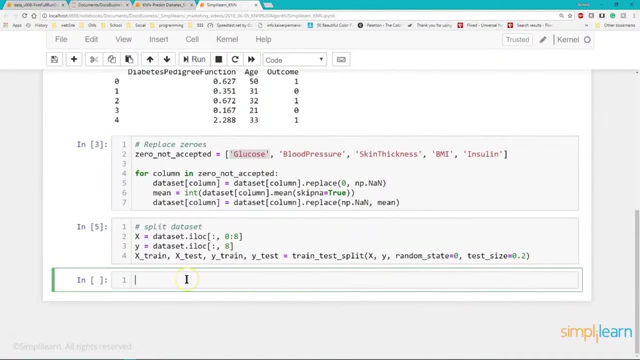 That's all that is, And again we're going to run it. Not very exciting. So far we haven't had any printout other than to look at the data, But that is a lot of. this is prepping this data Once you prep. 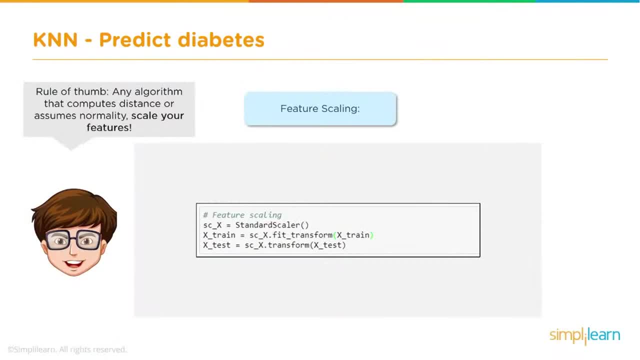 it. the actual lines of code are quick and easy And we're almost there with the actual running of our KNN. We need to go ahead and do a scale the data. If you remember correctly, we're fitting the data in a standard scaler, which means 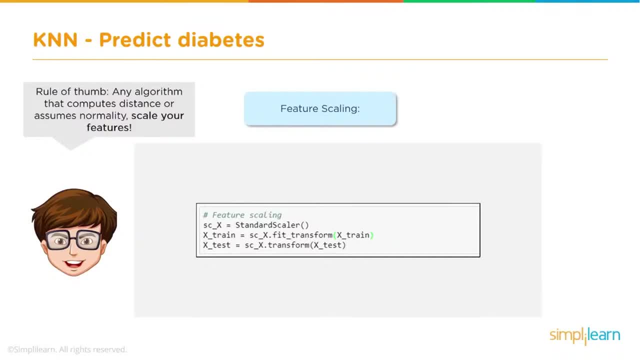 instead of the data being from 5 to 303 in one column and the next column is 1 to 6, we're going to set that all so that all the data is between minus 1 and 1.. That's what that. 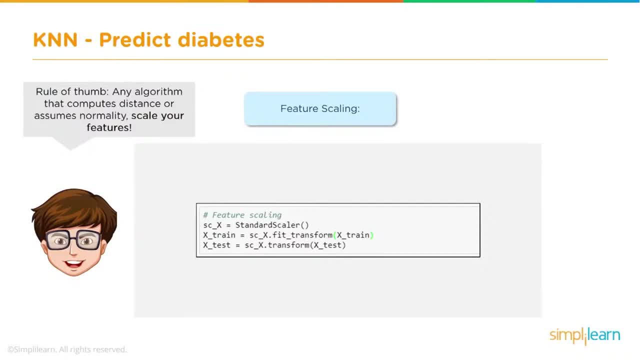 standard scaler does, Keeps it standardized, And we only want to fit the scaler with the training set. but we want to make sure the testing set is the xtest going in is also transformed, So it's processing it the same. So here we go with our standard. 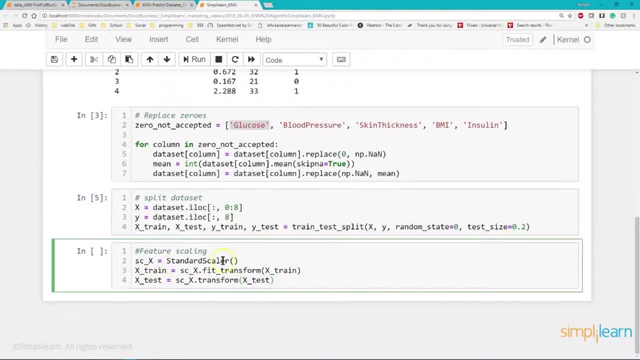 scaler. We're going to call it sc x for the scaler and we're going to import the standard scaler into this variable and then our xtrain equals sc, underscore x, dot fit transform. So we're creating the scaler on the xtrain variable And then our xtest. 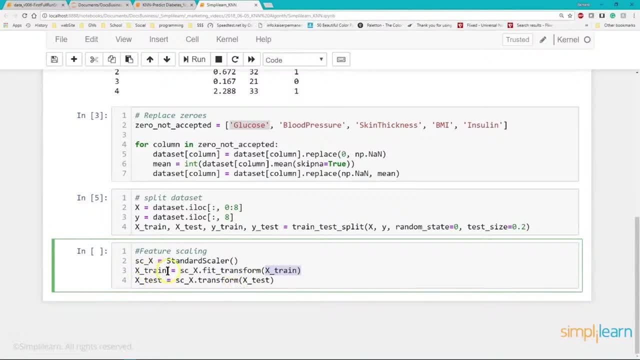 we're also going to transform it. So we've trained and transformed the xtrain and then the xtest isn't part of that training. It isn't part of training the transformer. It just gets transformed. That's all it does. And again, we're going to go ahead and run this. 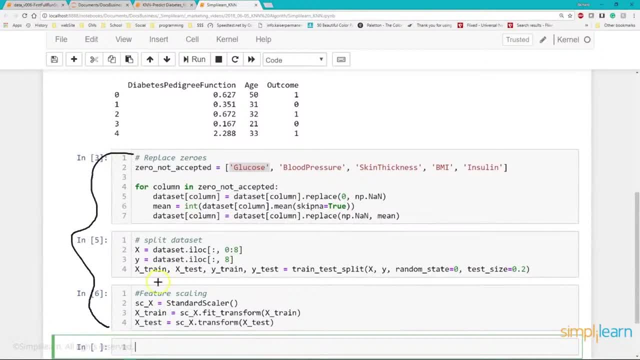 And if you look at this, we've now gone through these steps, all three of them. We've taken care of replacing our zeros for key columns that shouldn't be zero And we've replaced that with the means of those columns, That way that they fit right. 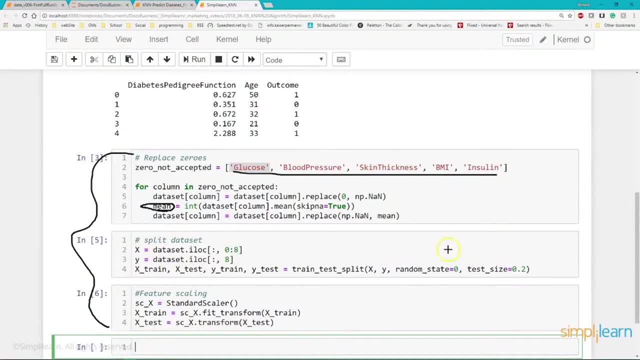 in with our data models. We've come down here and we've split the data. So now we have our test data and our training data, And then we've taken and we've scaled the data. So all of our data going in Now. no, we don't. 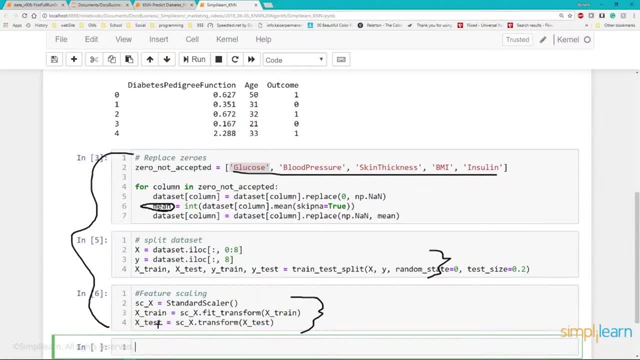 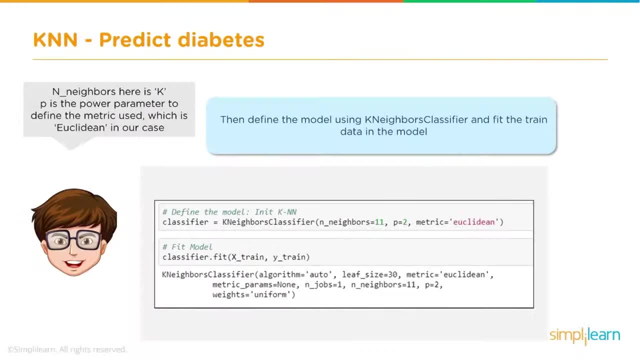 train the y part, the y train and y test. That never has to be trained, It's only the data going in. That's what we want to train in there. Then define the model using kNeighborsClassifier and fit the trained data in the. 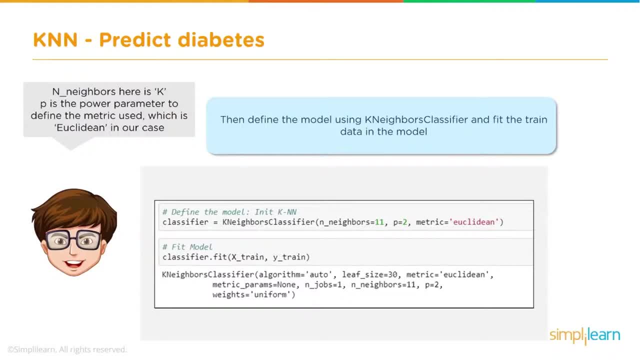 model. So we do all that data prep and you can see down here we're only going to have a couple lines of code where we're actually building our model and training it. That's one of the cool things about Python and how far we've come. 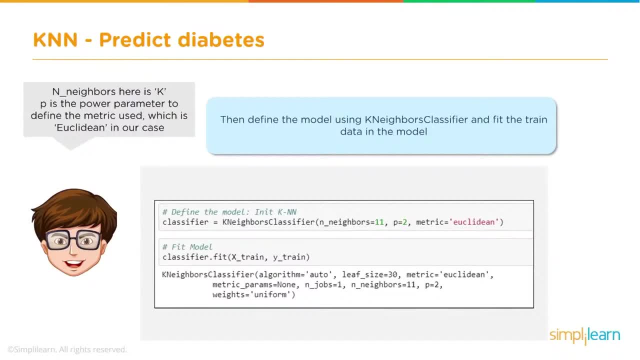 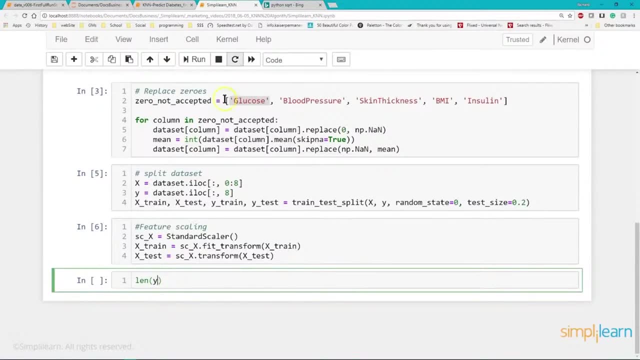 It's such an exciting time to be in machine learning because there's so many automated tools. Let's see, before we do this, let's do a quick length of and let's do y We want. let's just do length of y. 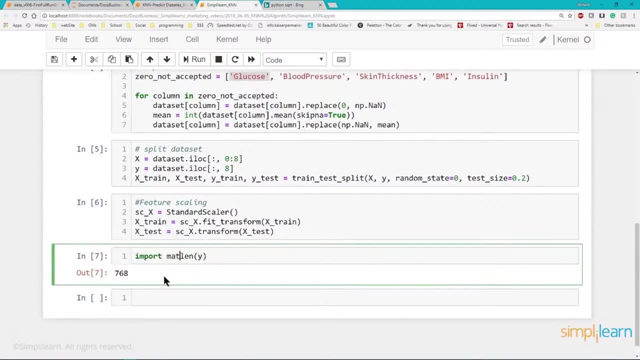 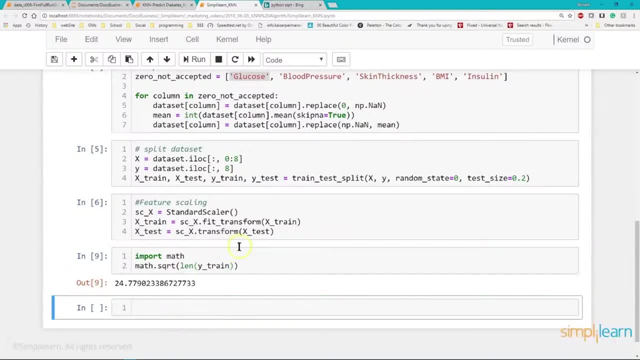 And we get 768.. And if we import math, we do math dot square root. Let's do y train. There we go. It's actually supposed to be x train. Before we do this, let's go ahead and do import math. 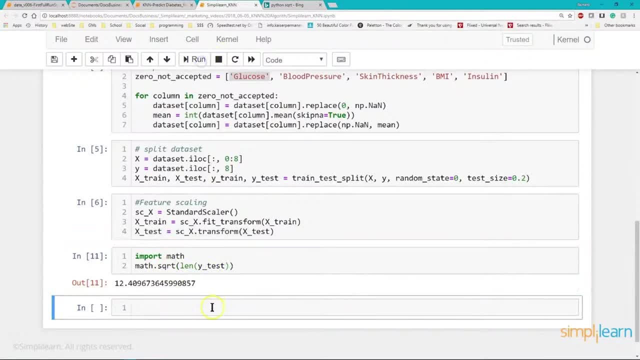 and do math- square root length of y test- And when I run that we get 12.409.. I wanted to show you where this number comes from. we're about to use 12 is an even number, So if you know if you're ever voting. 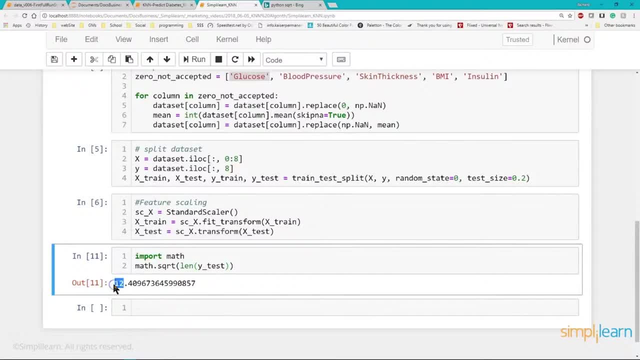 on things. remember the neighbors all vote don't want to have an even number of neighbors voting, So we want to do something odd And let's just take one away and we'll make it 11.. Let me delete this out of here. That's one of the reasons. 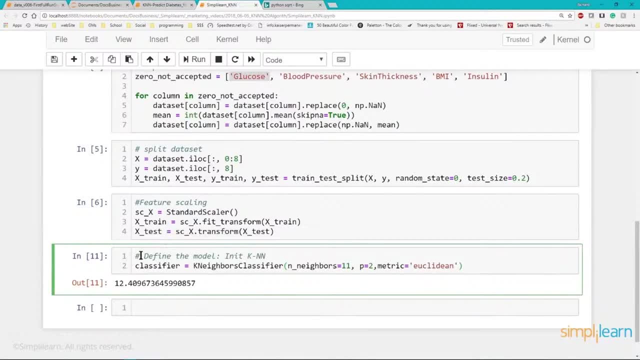 I love Jupyter Notebook because you can flip around and do all kinds of things on the fly. So we'll go ahead and put in our classifier. We're creating our classifier now And it's going to be the kNeighbors classifier: nNeighbors equals 11.. Remember we did. 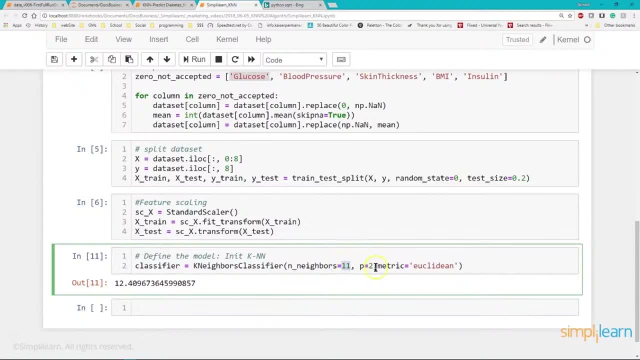 12 minus 1 for 11.. So we have an odd number of neighbors. p equals 2, because we're looking for is it- are they diabetic or not? And we're using the Euclidean metric. There are other means of measuring the distance. You could do like square. 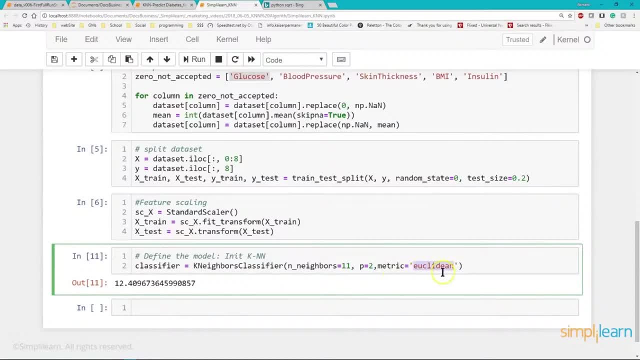 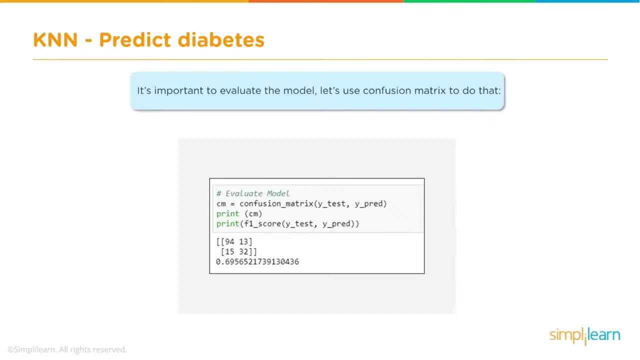 square means value. There's all kinds of ways to measure this, But the Euclidean's the most common one and it works quite well. It's important to evaluate the model. Let's use the confusion matrix to do that, And we're going to use the. 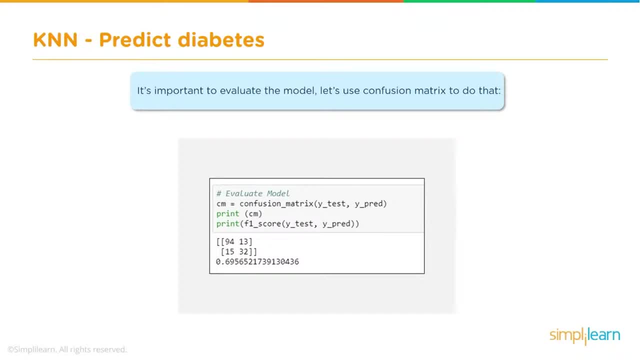 confusion matrix- Wonderful tool- And then we'll jump into the F1 score. And finally, accuracy score, which is probably the most commonly used quoted number when you go into a meeting or something like that. So let's go ahead and paste that in there And we'll set the cm. 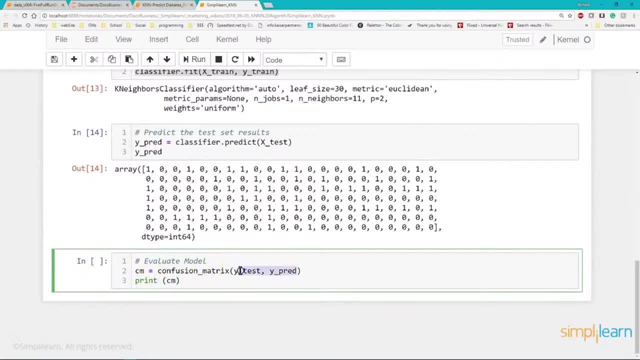 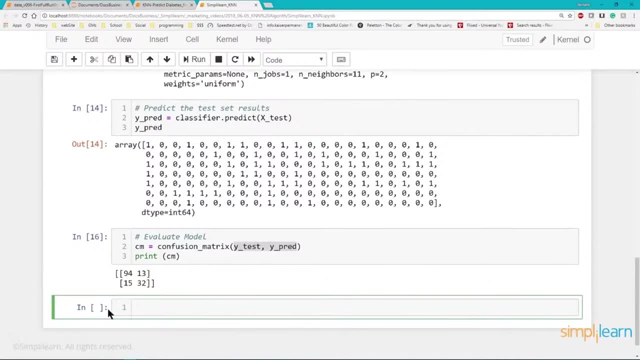 equal to confusion. matrix y test: y predict. So those are the two values we're going to put in there And let me go ahead and run that and print it out. And the way you interpret this is: you have the y predicted, which would be your. 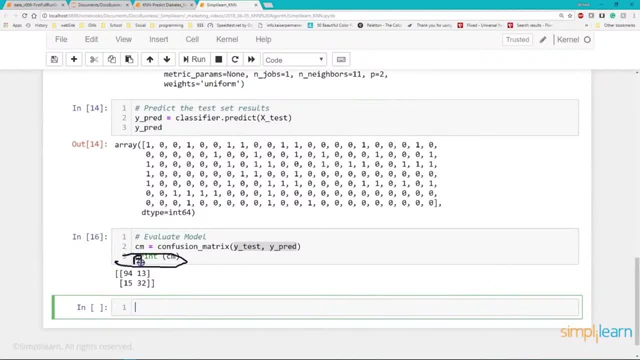 title up here We could do. let's just do pred Predicted across the top And actual going down. Actual. Always hard to write in here, Actual. That means that this column here down the middle that's the important column And it means that our 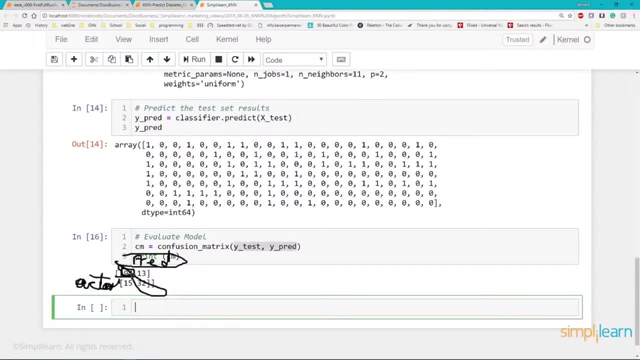 prediction said 94 and prediction and the actual agreed on 94 and 32.. This number here, the 13 and the 15, those are what was wrong. So you could have like three different if you're looking at this across three different variables. 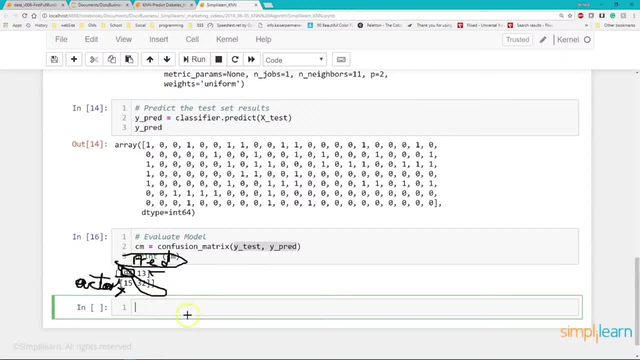 instead of just two. you'd end up with the third row down here and the column going down the middle. So in the first case we have the and I believe the zero is the 94, people who don't have diabetes. The prediction: 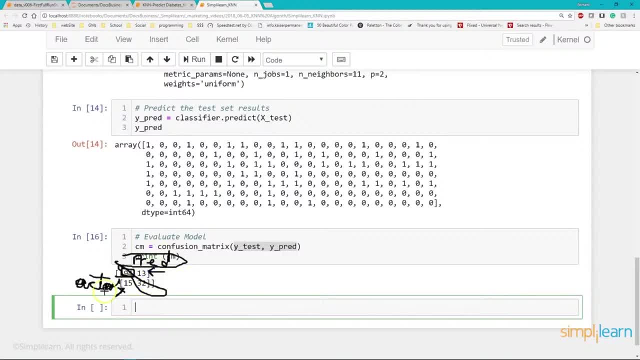 said that 13 of those people did have diabetes and were at high risk And the 32 that had diabetes it had correct, But our prediction said another 15. out of that 15 it classified as incorrect, So you can see where that classification comes. 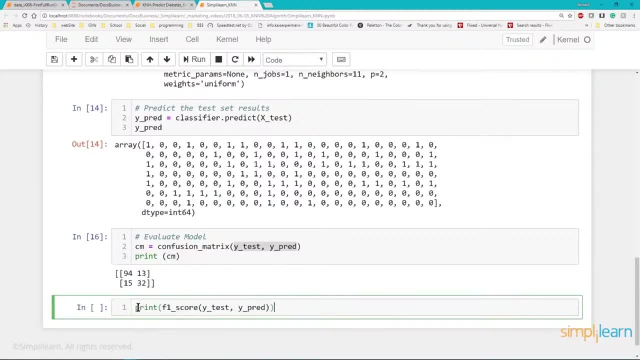 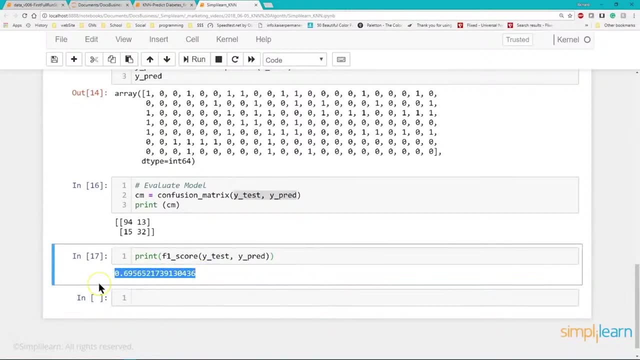 in and how that works on the confusion matrix, Then we're going to go ahead and print the F1 score. Let me just run that. You see, we get a .69 in our F1 score. The F1 takes into account both sides of the. 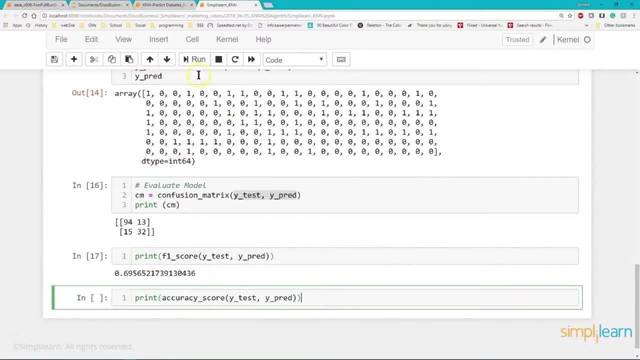 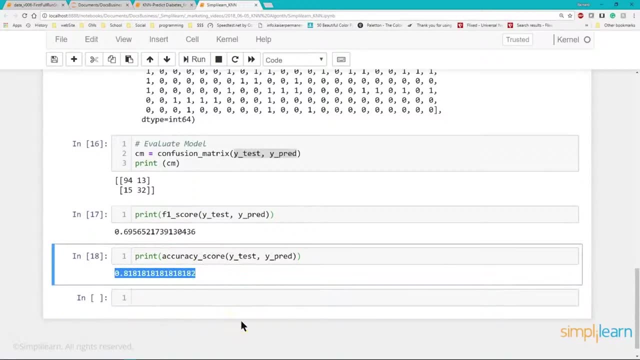 balance of false positives Where, if we go ahead and just do the accuracy account- and that's what most people think of is, it looks at just how many we got right out of how many we got wrong. So a lot of people, when you're a data scientist and 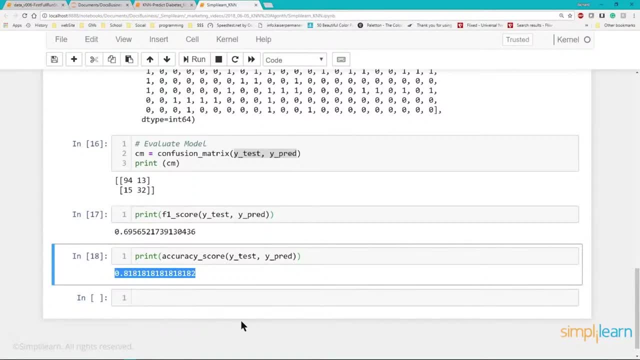 you're talking to other data scientists, they're going to ask you what the F1 score, the F score, is. If you're talking to the general public or the decision makers in the business, they're going to ask what the accuracy is, And the accuracy is always. 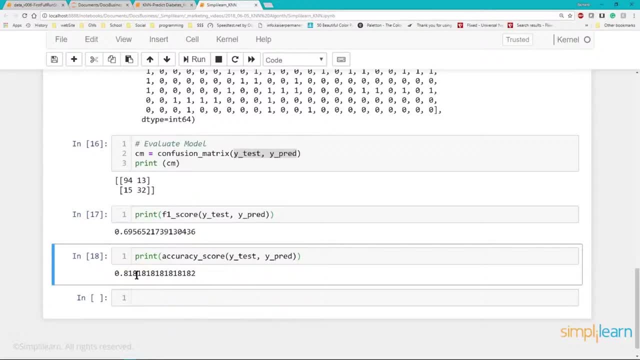 better than the F1 score, But the F1 score is more telling. It lets us know that there's more false positives than we would like on here. But 82%, not too bad for a quick flash. look at people's different statistics and running an sklearn and running. 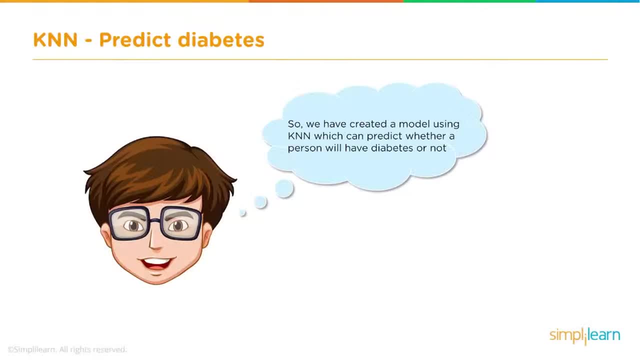 the KNN, the K nearest neighbor on it. So we have created a model using KNN which can predict whether a person will have diabetes or not Or, at the very least, whether they should go get a checkup and have their glucose checked regularly or not. 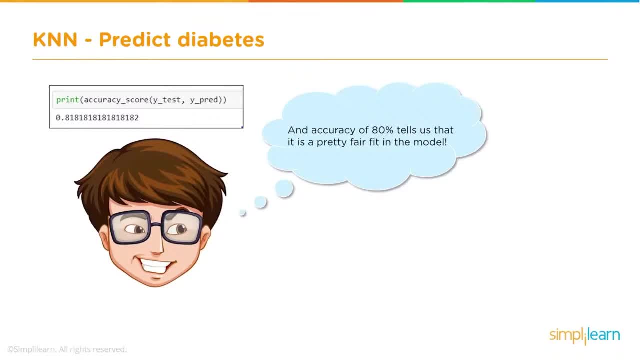 The print accuracy score. we got the .818, was pretty close to what we got And we can pretty much round that off and just say we have an accuracy. of 80% Tells us it is a pretty fair fit in the model. So 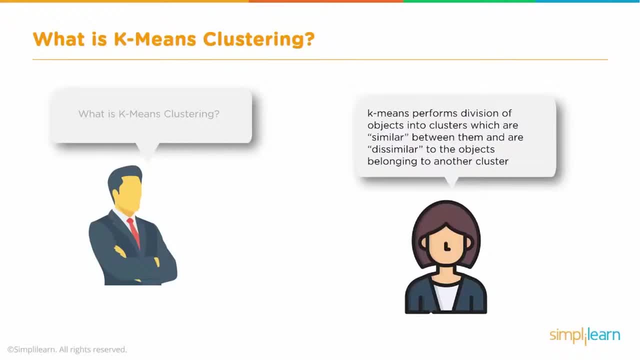 what is K-means clustering? K-means clustering is an unsupervised learning algorithm. In this case, you don't have labeled data, unlike in supervised learning. So you have a set of data and you want to group them And, as the name suggests, you want to put them. 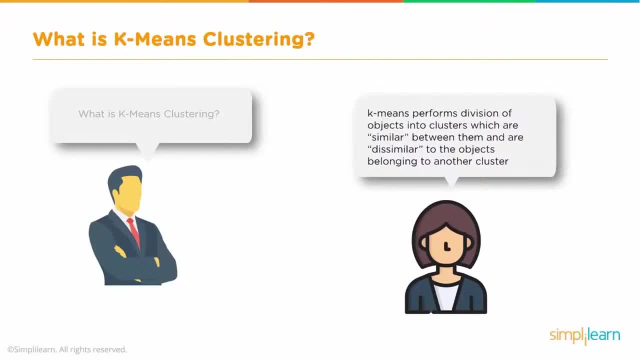 into clusters, which means objects that are similar in nature, similar in characteristics, need to be put together. So that's what K-means clustering is all about. The term K is basically is a number, So we need to tell the system how many clusters we need to. 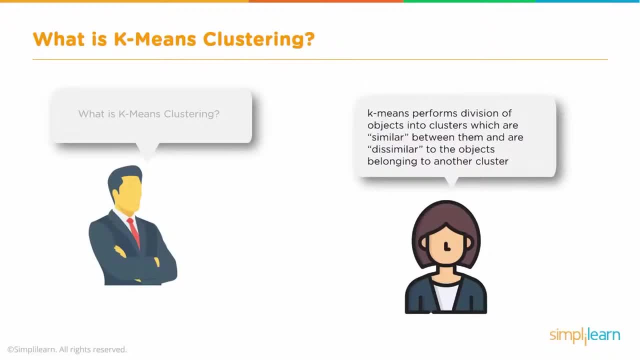 perform. So if K is equal to 2, there will be 2 clusters, If K is equal to 3, 3 clusters, and so on and so forth. That's what the K stands for, And of course there is a way of finding out. 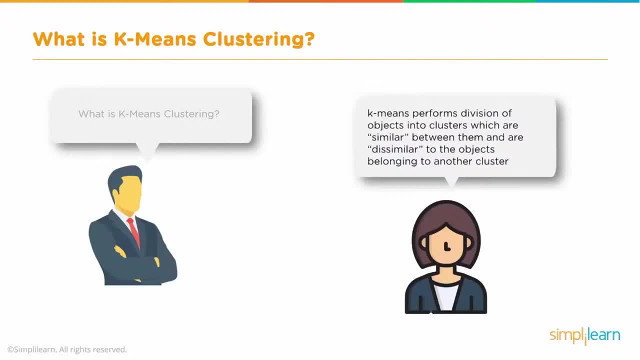 what is the best or optimum value of K for a given data? We will look at that. So that is K-means clustering. So let's take an example. K-means clustering is used in many, many scenarios, but let's take an example of cricket. 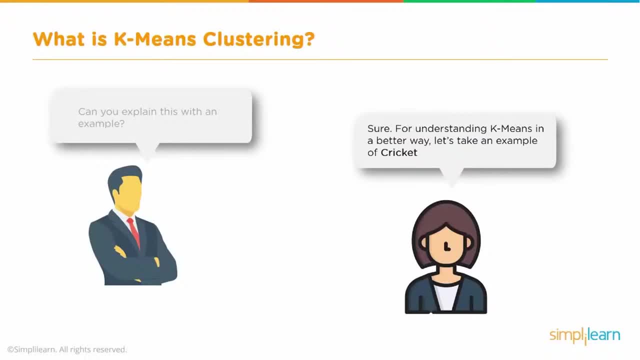 the game of cricket. Let's say, you received data of a lot of players from maybe all over the country or all over the world, And this data has information about the runs scored by the people or by the player and the wickets taken by the player. 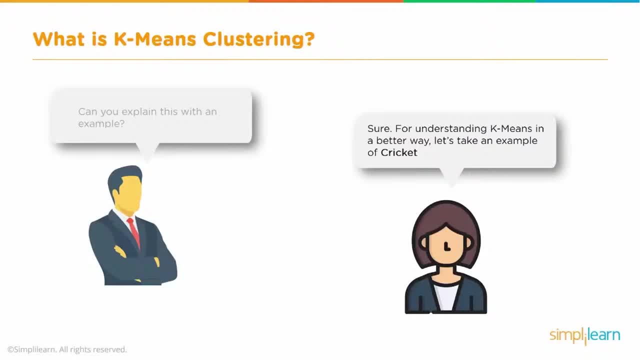 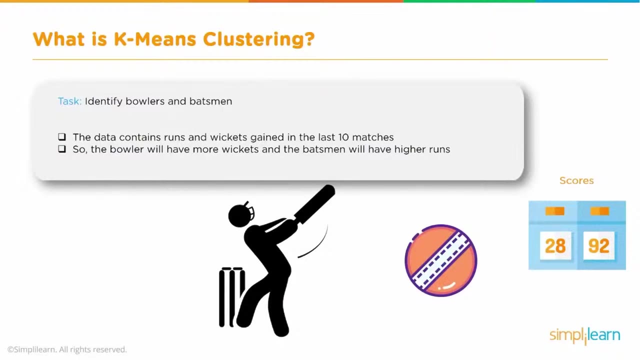 And, based on this information, we need to cluster this data into 2 clusters: batsmen and bowlers. So this is an interesting example. Let's see how we can perform this. So we have the data, which consists of primarily 2 characteristics. 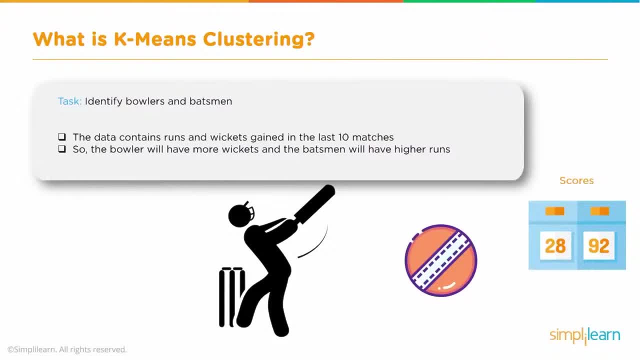 which is the runs and the wickets. So the bowlers basically take wickets and the batsmen score runs. There will be, of course, a few bowlers who can score some runs and similarly, there will be some batsmen who would have taken a few wickets. 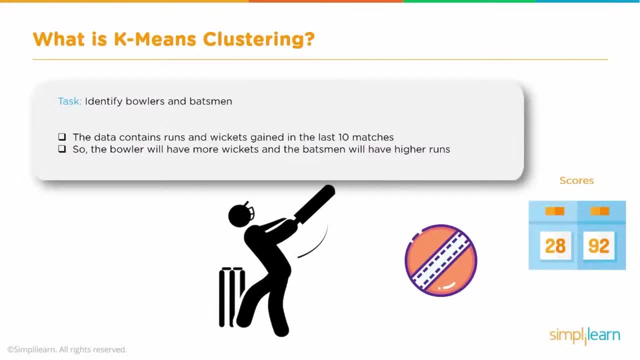 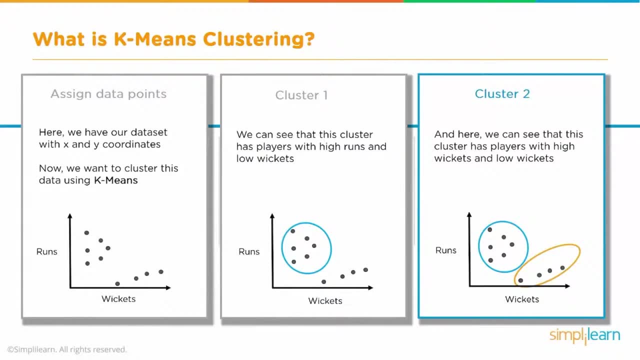 But with this information, we want to cluster these players into batsmen and bowlers. So how does this work? Let's say this is how the data is. So there are information. there is information on the y-axis about the runs scored and on the 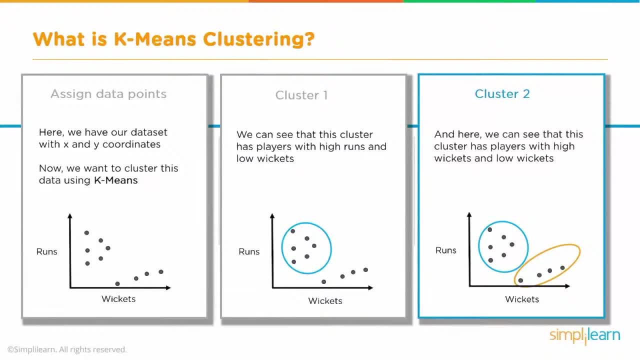 x-axis about the wickets taken by the players. So if we do a quick plot, this is how it would look, and when we do the clustering, we need to have the clusters, like shown in the third diagram, out here. So we need to have a cluster which consists of people. 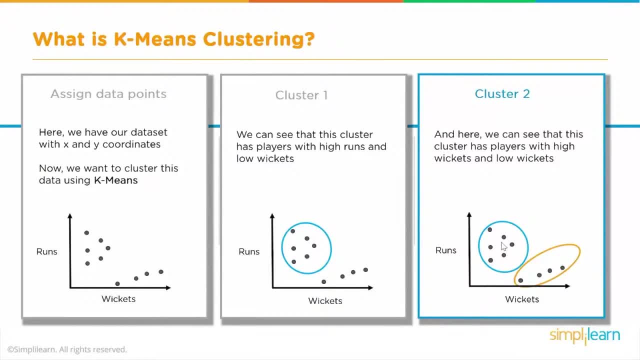 who have scored high runs, which is basically the batsmen, and then we need a cluster with people who have taken a lot of wickets, which is typically the bowlers. There may be a certain amount of overlap, but we will not talk about it right now. So with K-means, 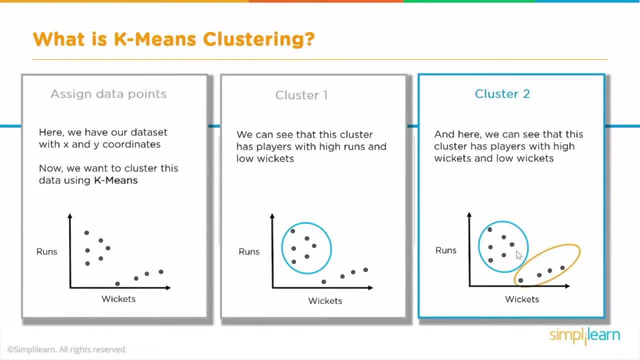 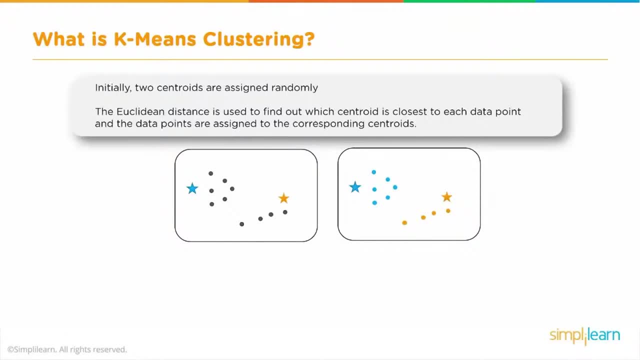 clustering we will have here. that means K is equal to 2 and we will have two clusters, which is batsmen and bowlers. So how does this work? The way it works is: the first step in K-means clustering is the allocation of two centroids randomly. 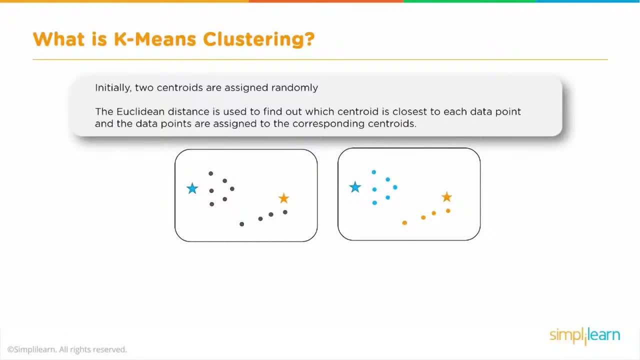 So two points are assigned as so called centroids. So in this case we want two clusters, which means K is equal to 2.. So two points have been randomly assigned as centroids. Keep in mind, these points can be anywhere. There are random points. They are not. 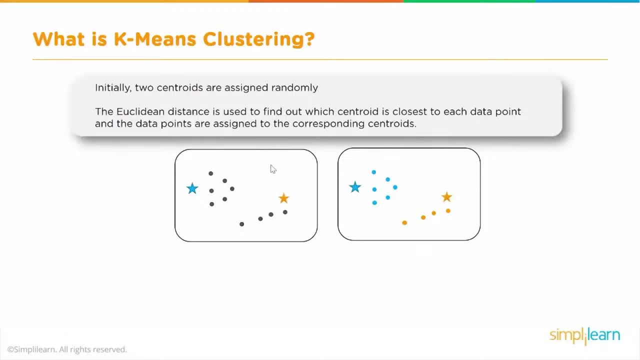 initially, they are not really the centroids. Centroid means it's a central point of a given data set, but in this case, when it starts off, it's not really the centroid. So these points, though in our presentation here, we have shown them one point closer to these. 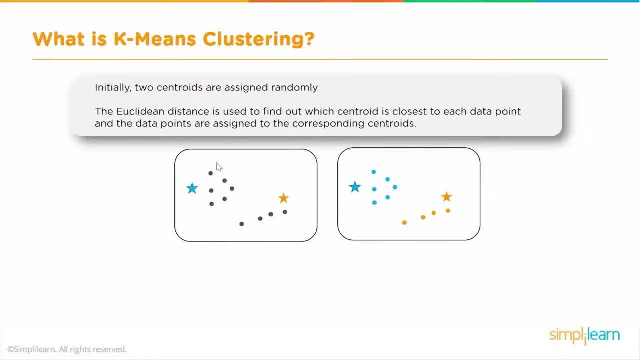 data points and another closer to these data points. they can be assigned randomly anywhere. So that's the first step. The next step is to determine the distance of each of the data points from each of the randomly assigned centroids. So, for example, we take this point and find: 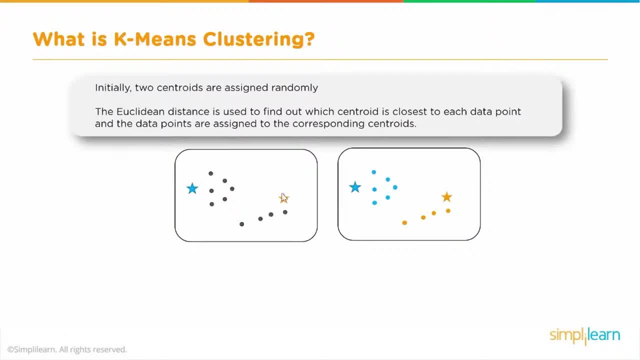 the distance from this centroid and the distance from this centroid. This point is taken and the distance is found from this centroid and this centroid, and so on and so forth. So for every point the distance is measured from both the centroids and then whichever distance is less. 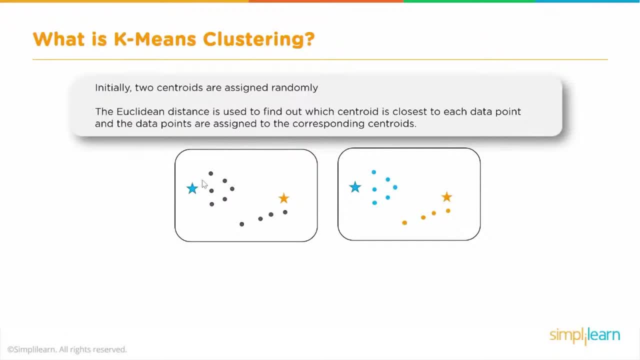 that point is assigned to that centroid. So, for example, in this case, visually it is very obvious that all these data points are assigned to this centroid and all these data points are assigned to this centroid. And that's what is represented here in blue color and in this yellow color. The next: 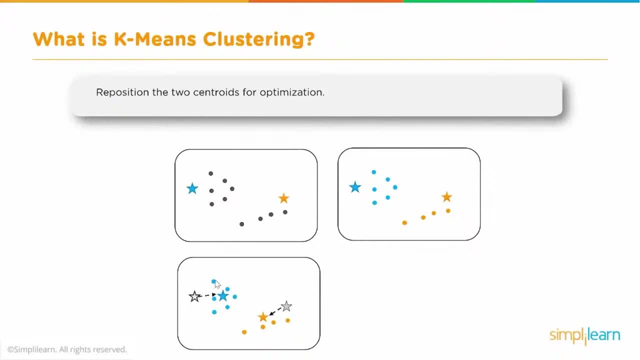 step is to actually determine the central point or the actual centroid for these two clusters. So we have this one initial cluster, this one initial cluster, but, as you can see, these points are not really the centroid. Centroid means it should be the central position. 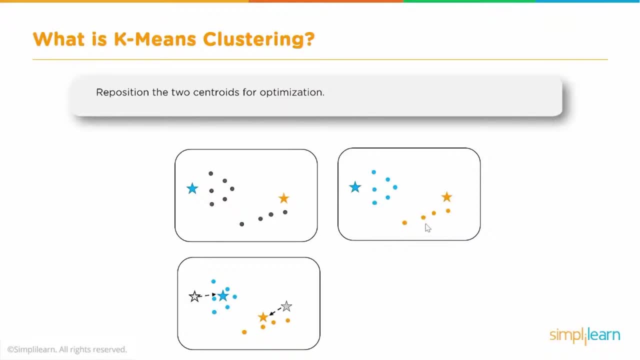 of this data set, Central position of this data set. So that is what needs to be determined as the next step. So the central point or the actual centroid is determined and the original randomly allocated centroid is repositioned to the actual centroid of these. 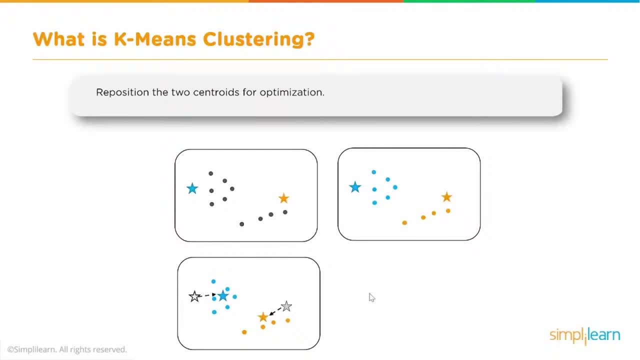 new clusters, And this point process is actually repeated. Now what might happen is some of these points may get reallocated In our example. that is not happening, probably, But it may so happen that the distance is found between each of these data points once again with these centroids. 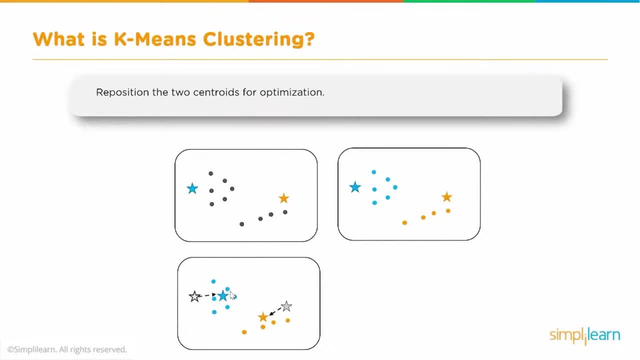 And if it is required, some points may be reallocated. We will see that in a later example, But for now we will keep it simple. So this process is continued till the centroid repositioning stops And that is our final cluster. So 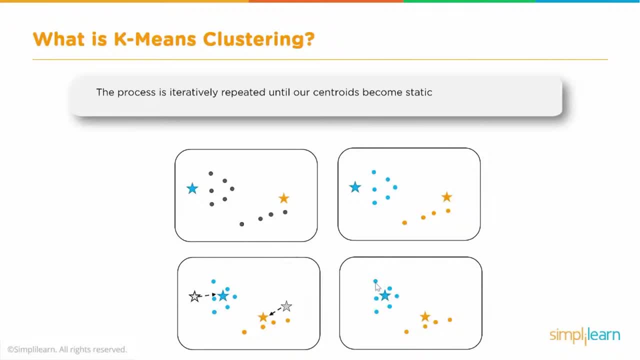 this is our. so, after iteration, we come to this position, this situation where the centroid doesn't need any more repositioning And that means our algorithm has converged, Convergence has occurred and we have the cluster, Two clusters, We have the clusters. 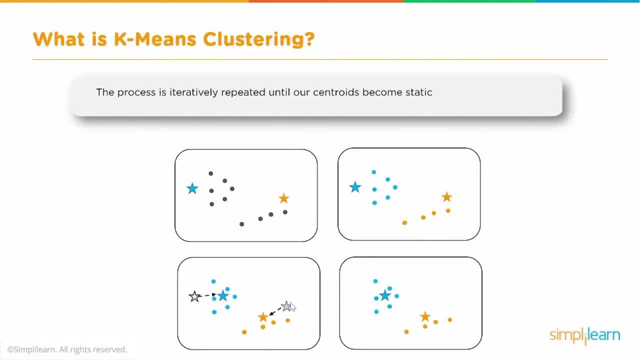 with a centroid, So this process is repeated. The process of calculating the distance and repositioning the centroid is repeated till the repositioning stops, Which means that the algorithm has converged And we have the final cluster with the data points and the centroids. 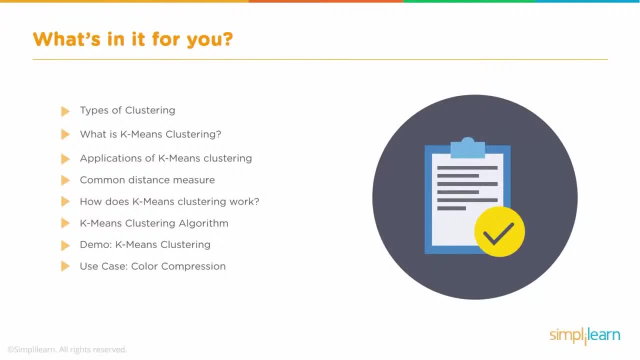 So this is what you are going to learn from this session. We will talk about the types of clustering. What is k-means clustering? Application of k-means clustering? K-means clustering is done using distance measure, So we will talk about 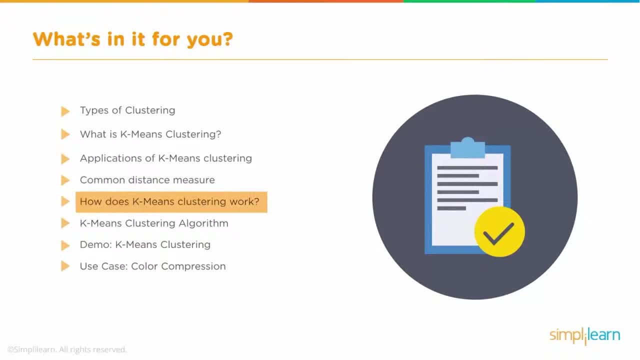 the common distance measures, And then we will talk about how k-means clustering works And go into the details of k-means clustering algorithm, And then we will end with a demo and a use case for k-means clustering. So let's begin First of all. 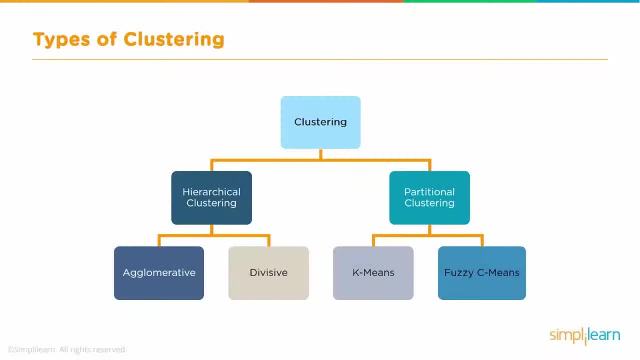 what are the types of clustering? There are primarily two categories of clustering: Hierarchical clustering and then partitional clustering, And each of these categories are further subdivided into agglomerative and divisive clustering and k-means and fuzzy k-means clustering. Let's take a quick. 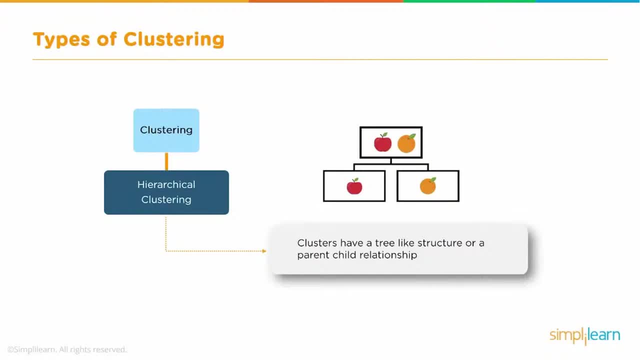 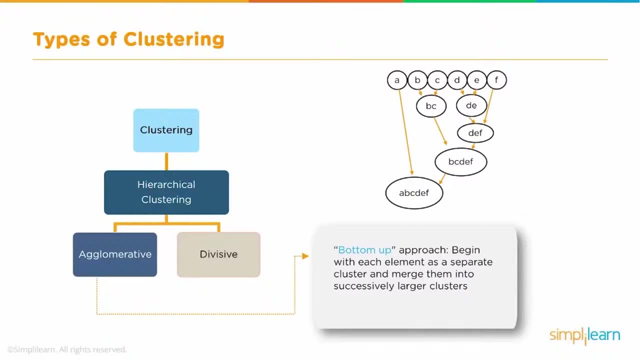 look at what each of these types of clustering are. In hierarchical clustering, the clusters have a tree-like structure, and hierarchical clustering is further divided into agglomerative and divisive. Agglomerative clustering is a bottom-up approach. We begin with each element as a separate cluster. 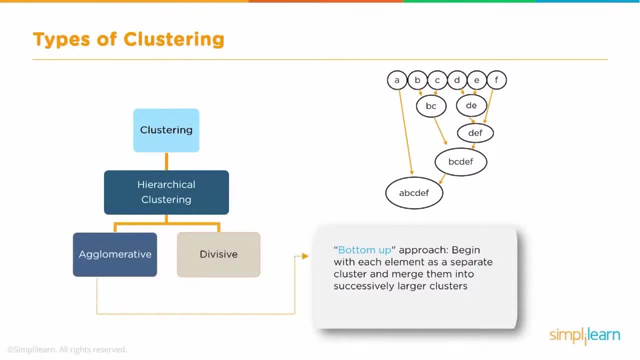 and merge them into successively larger clusters. So for example, we have A, B, C, D, E, F. We start by combining B and C form one cluster, D and E form one more. then we combine D, E and F one. 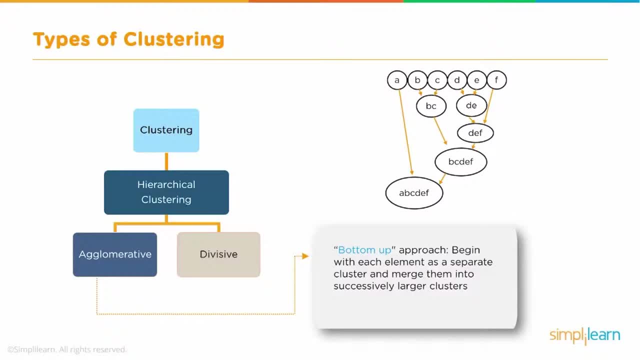 more bigger cluster and then add B, C to that and then finally A to it. Compared to that, divisive clustering, or divisive clustering is a top-down approach. We begin with the whole set and proceed to divide it into successively smaller clusters. So we have A, B, C. 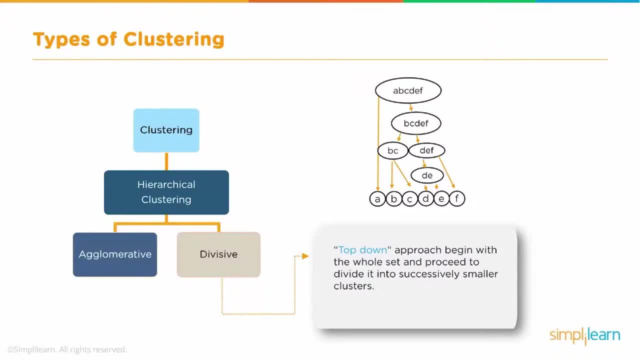 D, E, F. We first take that as a single cluster and then break it down into A, B, C, D, E and F. Then we have partitional clustering, split into two subtypes: K-means clustering and fuzzy C-means. In K-means, 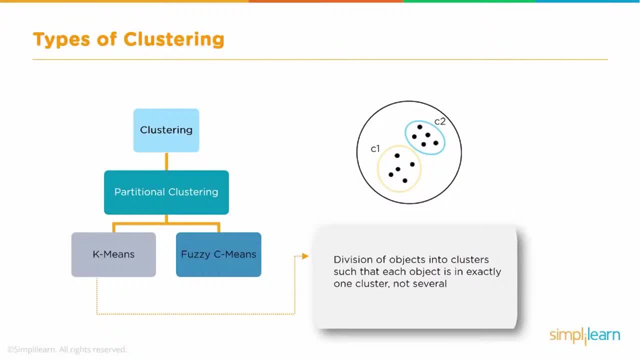 clustering. the objects are divided into the number of clusters mentioned by the number K. That's where the K comes from. So if we say K is equal to 2, the objects are divided into two clusters, C1 and C2. and the way it is. 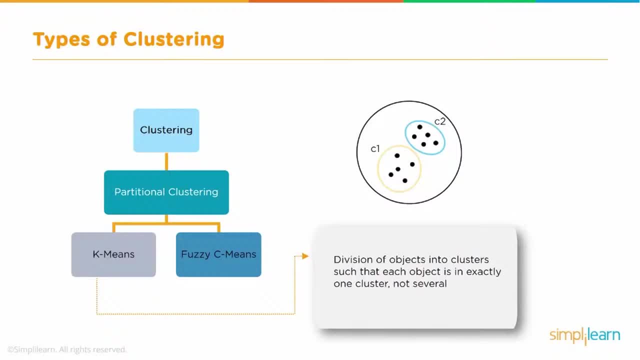 done is the features or characteristics are compared and all objects having similar characteristics are clubbed together. So that's how K-means clustering is done. We will see it in more detail as we move forward. And fuzzy C-means is very similar to. 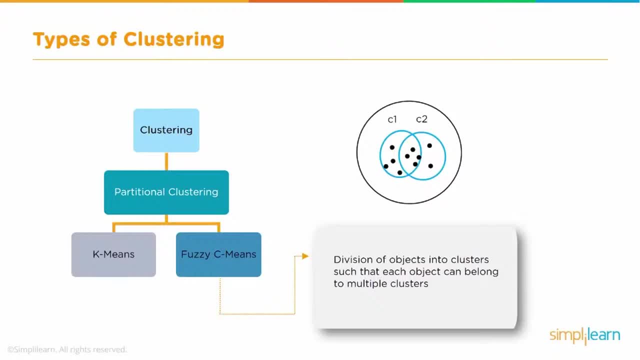 K-means in the sense that it clubs objects that have similar characteristics together. but while in K-means clustering two objects cannot belong to or any object, a single object cannot belong to two different clusters. in C-means objects can belong to more than one cluster. So 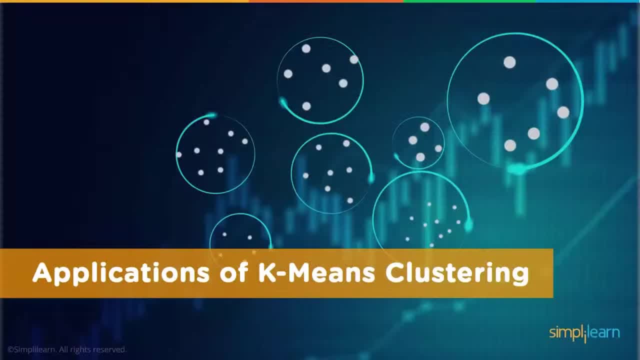 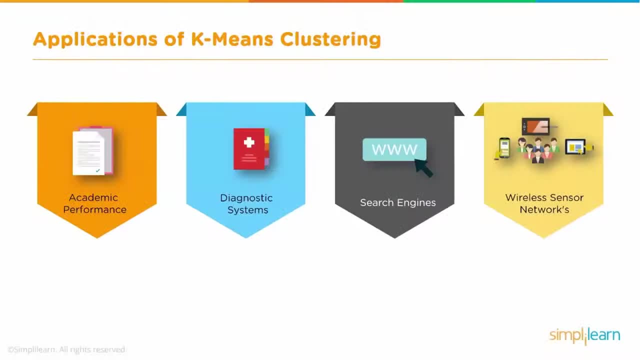 that is the primary difference between K-means and fuzzy C-means. So what are some of the applications of K-means clustering? K-means clustering is used in a variety of examples or variety of business cases in real life, starting from academic performance diagnostic systems. 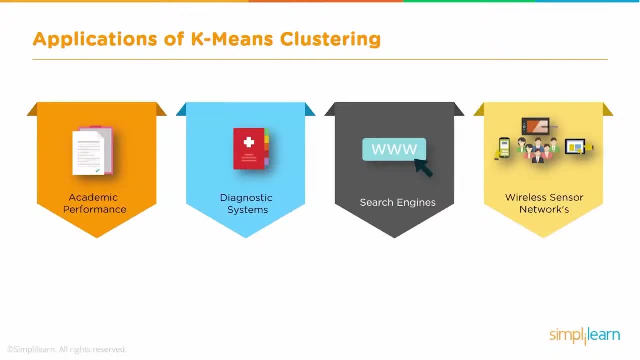 search engines and wireless sensor networks, and many more. So let us take a little deeper look at each of these examples. Academic performance, so, based on the scores of the students, students are categorized into A, B, C, and so on. Clustering forms. 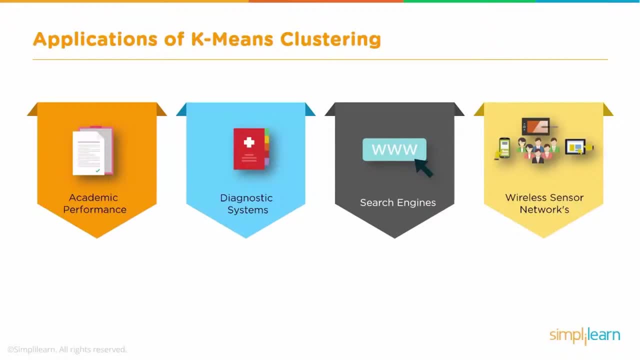 a backbone of search engines. When a search is performed, the search results need to be grouped together. The search engines very often use clustering to do this And, similarly, in case of wireless sensor networks, the clustering algorithm plays the role of finding the 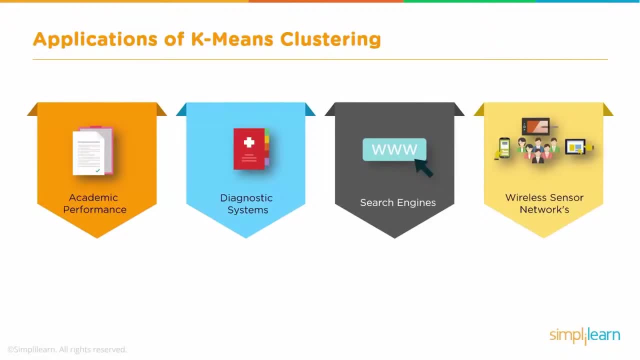 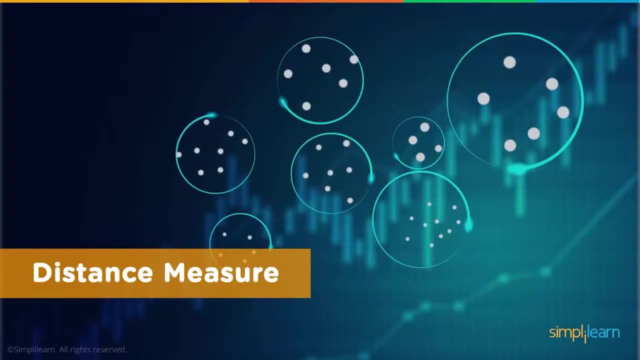 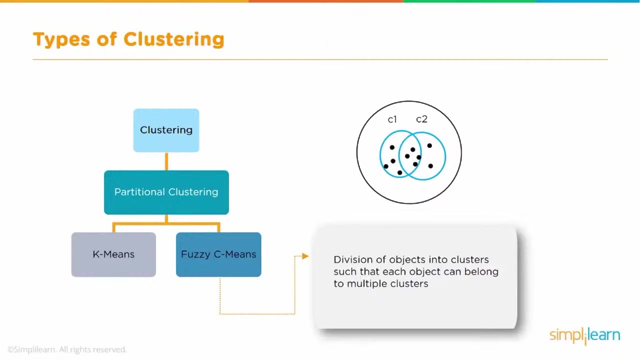 cluster heads, which collects all the data in its respective cluster. So clustering, especially K-means clustering, uses distance measure, So let us take a look at what is distance measure. So, while these are the different types of clustering in this video, we will focus on 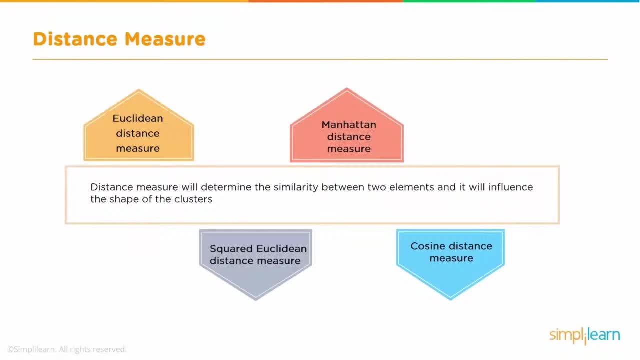 K-means clustering. So distance measure tells how similar some objects are. So the similarity is measured using what is known as distance measure. And what are the various types of distance measures? There is Euclidean distance, there is Manhattan distance, then we have squared Euclidean distance. 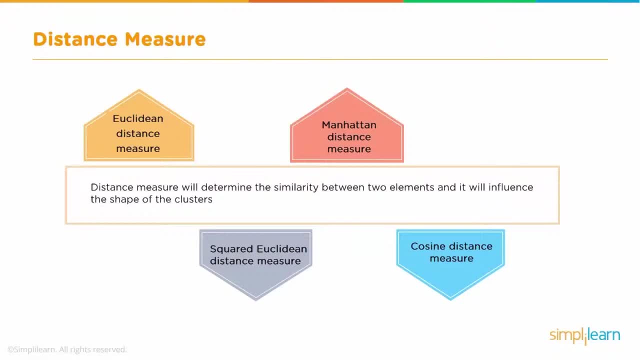 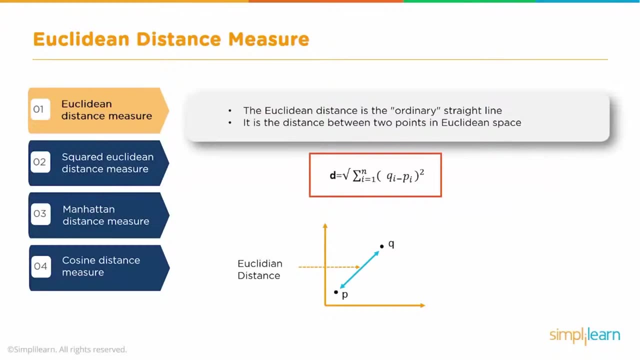 measure and cosine distance measure. These are some of the distance measures supported by K-means clustering. Let us take a look at each of these. What is Euclidean distance measure? This is nothing but the distance between two points. So we have learnt in high school. 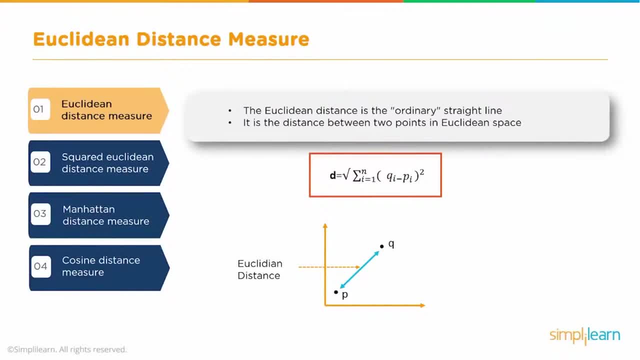 how to find the distance between two points. This is a little sophisticated formula for that, but we know a simpler one is square root of y2 minus y1 whole square plus x2 minus x1 whole square. So this is an extension of that. 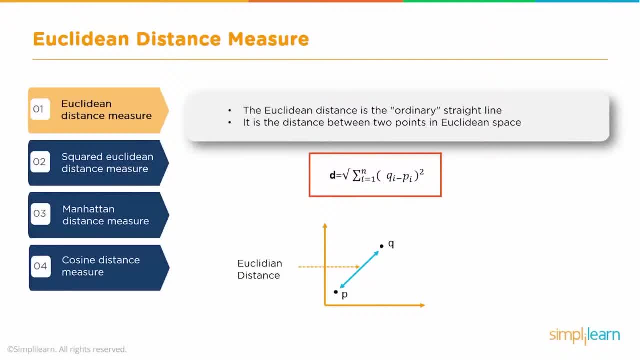 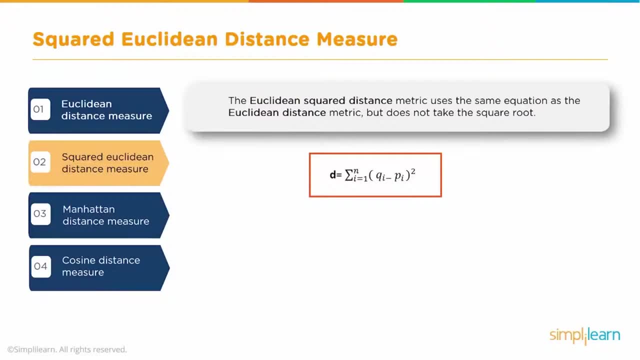 formula. So that is the Euclidean distance between two points. What is the squared Euclidean distance measure? It is nothing but the square of the Euclidean distance, as the name suggests. So instead of taking the square root, we leave the square as. 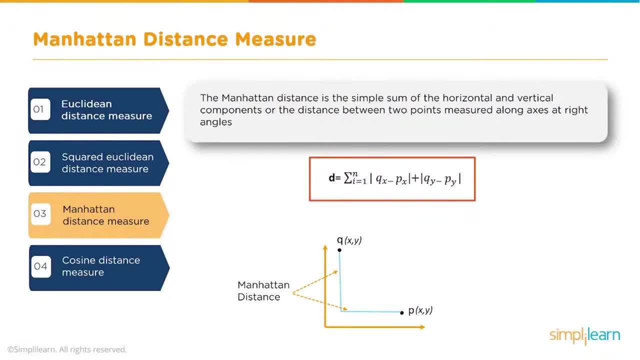 it is. And then we have Manhattan distance measure. In case of Manhattan distance, it is the sum of the distances across the x-axis and the y-axis, And note that we are taking the absolute value so that the negative values don't come into. 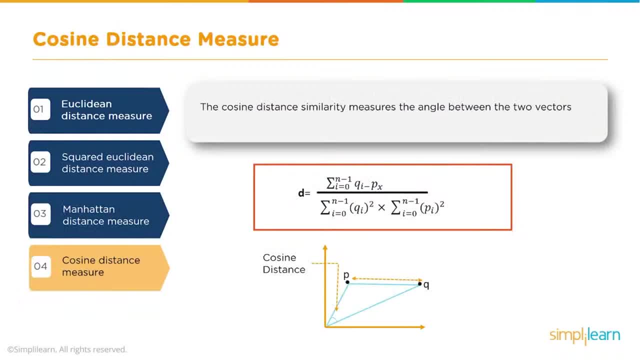 play. So that is the Manhattan distance measure. Then we have cosine distance measure. In this case we take the angle between the two vectors formed by joining the points from the origin. So that is the cosine distance measure. Okay, so that was a quick. 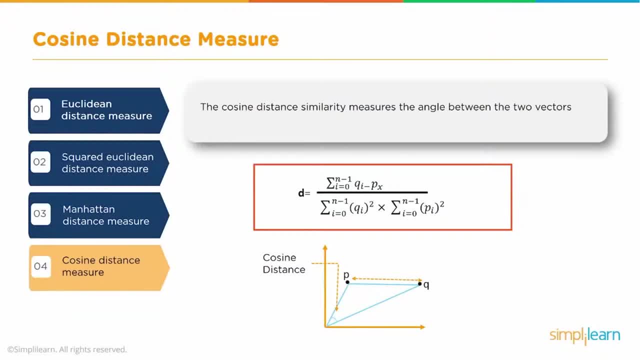 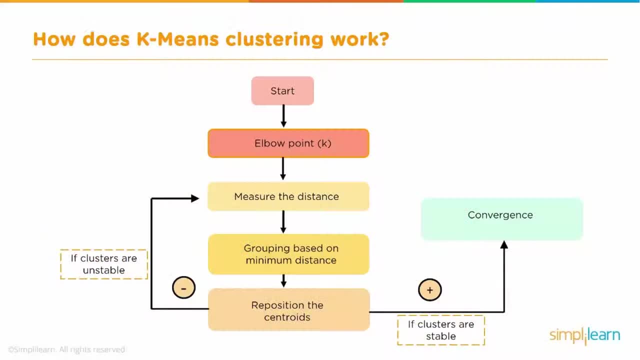 overview about the various distance measures that are supported by k-means. Now let's go and check how exactly k-means clustering works. Okay, so this is how k-means clustering works. This is like a flow chart of the whole process. There is a 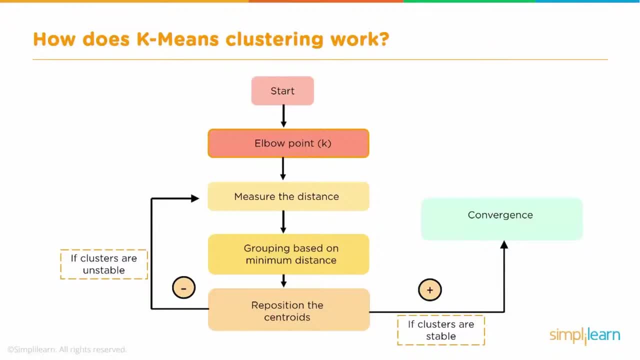 starting point, and then we specify the number of clusters that we want. Now there are a couple of ways of doing this. We can do by trial and error. So we specify a certain number- maybe k is equal to 3 or 4 or 5 to start with, And then 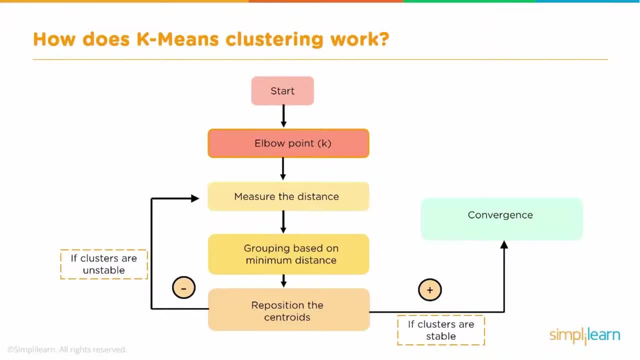 as we progress, we keep changing until we get the best number of clusters. or there is a technique called ELBO technique, whereby we can determine the value of k. what should be the best value of k? how many clusters should be formed? So once we have 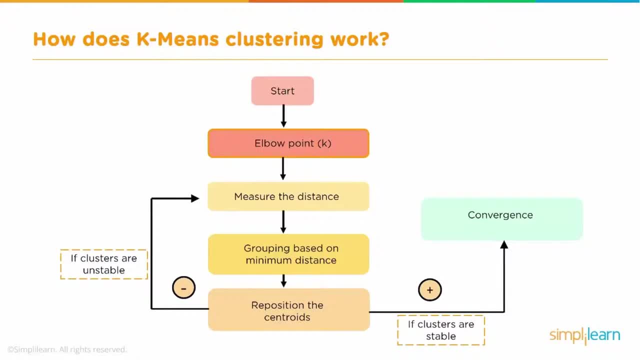 the value of k, we specify that and then the system will assign that many centroids. So it picks randomly that to start with, randomly that many points that are considered to be the centroids of these clusters, And then it measures the distance of each of the data points from. 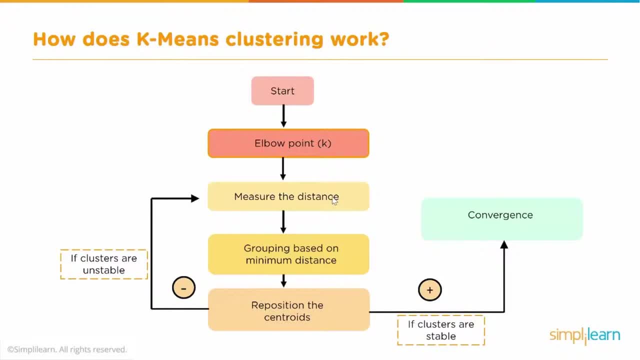 these centroids and assigns those points to the corresponding centroid from which the distance is minimum. So each data point will be assigned to the centroid which is closest to it, And thereby we have k number of initial clusters. However, this is not the final clusters. 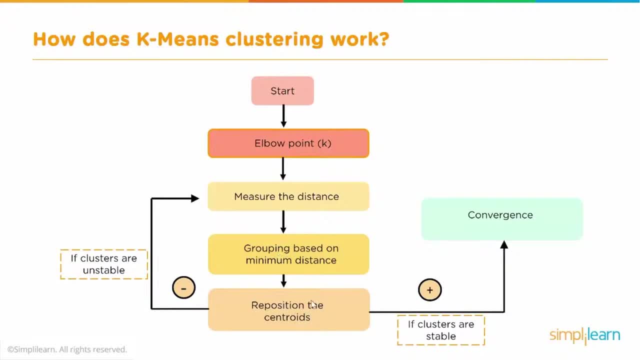 The next step it does is for the new groups, for the clusters that have been formed. it calculates the mean position, thereby calculates the new centroid position. The position of the centroid moves compared to the randomly allocated one, So it's an iterative process. Once again, 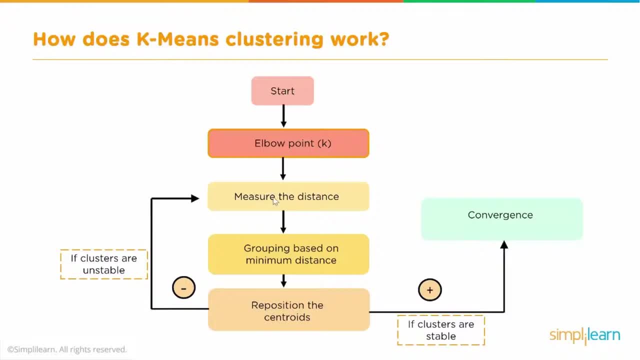 the distance of each point is measured from this new centroid point And, if required, the data points are reallocated to the new centroids and the mean position or the new centroid is calculated once again. If the centroid moves, then the iteration continues, Which means the convergence has not. 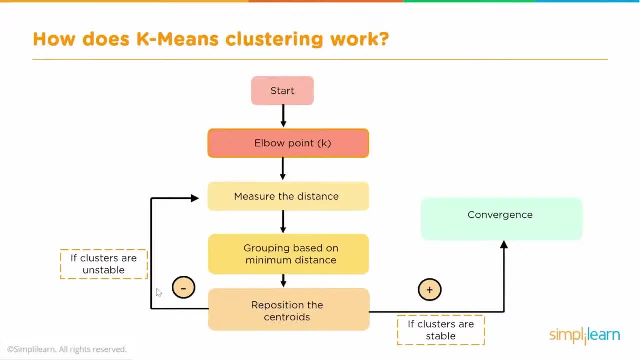 happened, The clustering has not converged. So as long as there is a movement of the centroid, this iteration keeps happening. But once the centroid stops moving- which means that the cluster has converged or the clustering process has converged- that will be the end result. So now we have 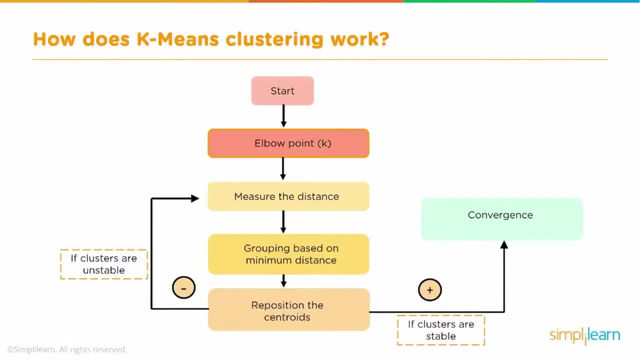 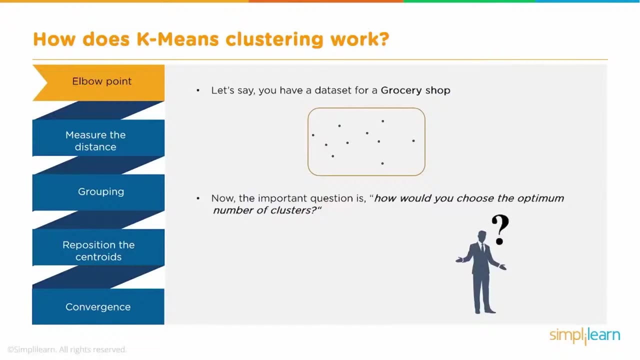 the final position of the centroid and the data points are allocated according to the closest centroid. I know it's a little difficult to understand from this simple flow chart, So let's do a little bit of visualization and see if we can explain it better. 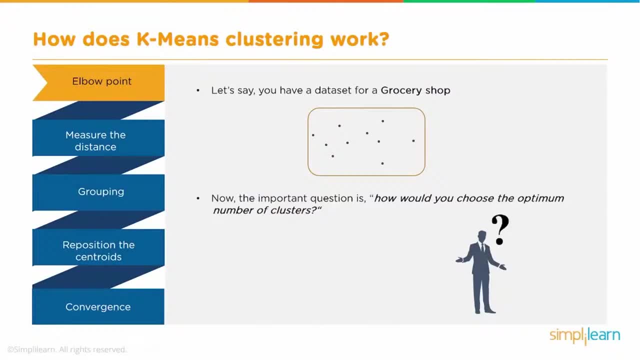 Let's take an example. If we have a data set for a grocery shop. So let's say we have a data set for a grocery shop and now we want to find out how many clusters this has to be spread across. So how do we find the optimum? 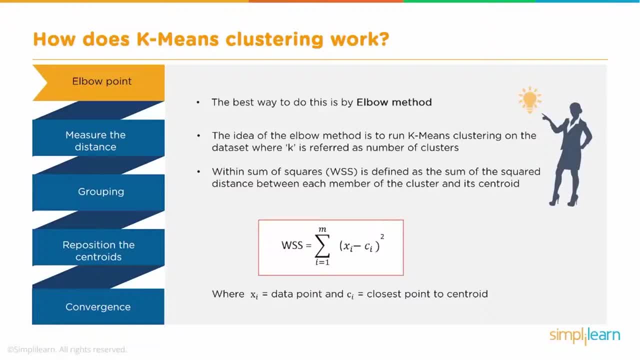 number of clusters. There is a technique called the Elbow method. So when these clusters are formed, there is a parameter called within sum of squares, And the lower this value is, the better the cluster is. That means all these points are very close to each other. 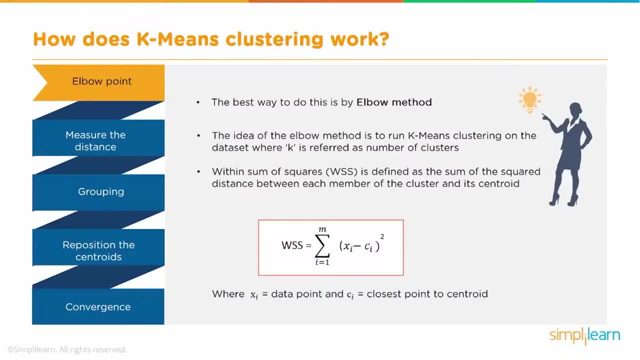 So we use this within sum of squares as a measure to find the optimum number of clusters that can be formed for a given data set. So we create clusters, or we let the system create clusters of a variety of numbers, maybe of 10 clusters. 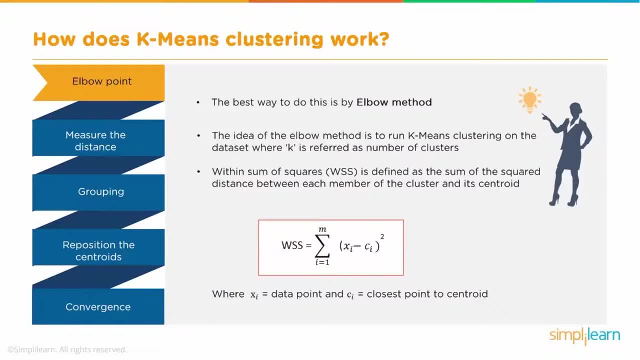 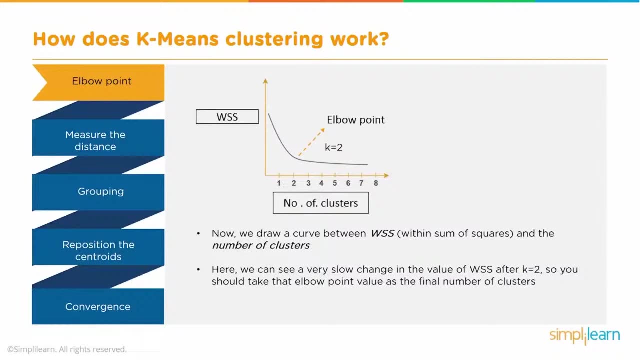 And for each value of k the within ss is measured and the value of k which has the least amount of within ss or wss, that is taken as the optimum value of k. So this is the diagrammatic representation So we have on the y-axis. 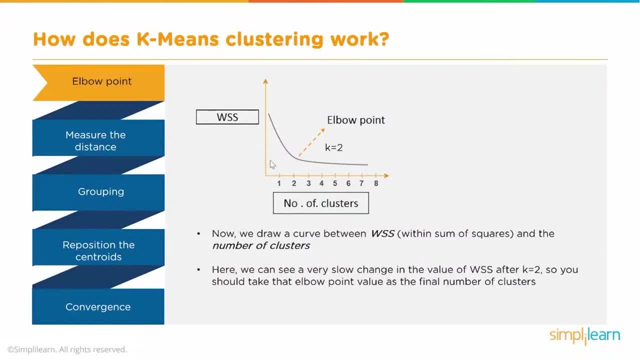 the within sum of squares, or wss, and on the x-axis we have the number of clusters. So, as you can imagine, if you have, k is equal to 1, which means all the data points are in a single cluster, the within ss value will be very high. 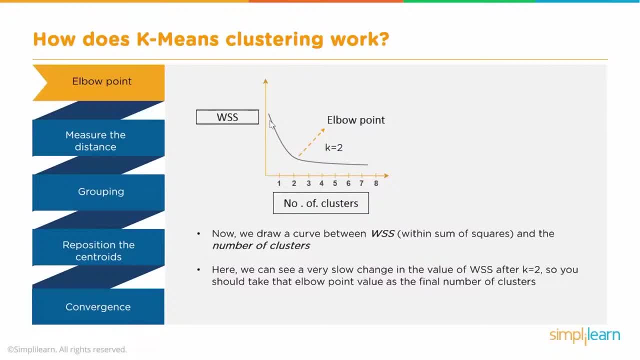 because they are probably scattered all over. The moment you split it into two, there will be a drastic fall in the within ss value. That's what is represented here. But then, as the value of k increases, the decrease, the rate of decrease will not be so. 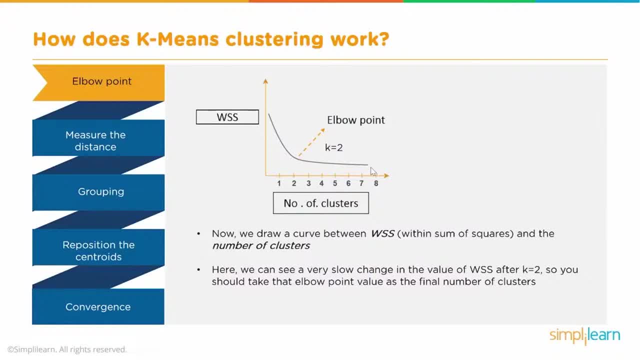 high. It will continue to decrease, but probably the rate of decrease will not be high. So that gives us an idea. So from here we get an idea. for example, the optimum value of k should be either 2 or 3 or, at the most, 4.. 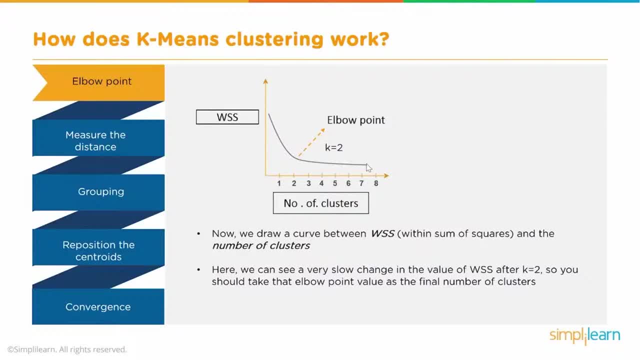 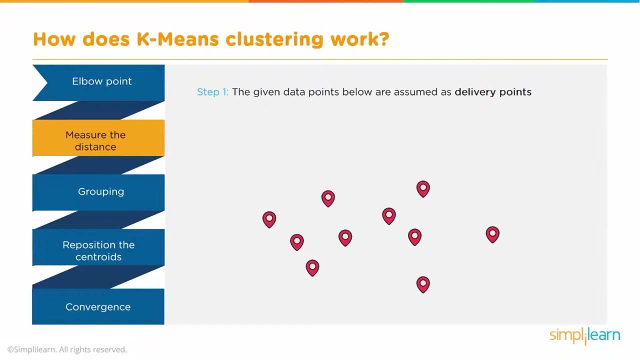 But beyond that, increasing the number of clusters is not dramatically changing the value in wss, because that pretty much gets stabilized. Okay, now that we have got the value of k, and let's assume that these are our delivery points, the next step is basically to 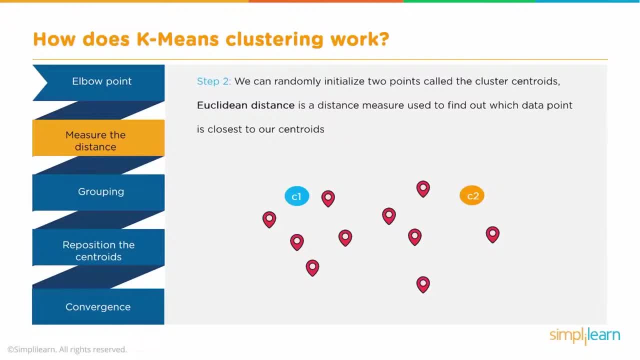 assign two centroids randomly. So let's say c1 and c2 are the centroids assigned randomly. Now the distance of each location from the centroid is measured and each point is assigned to the centroid which is closest to it. So, for example, these points are very obvious that these are. 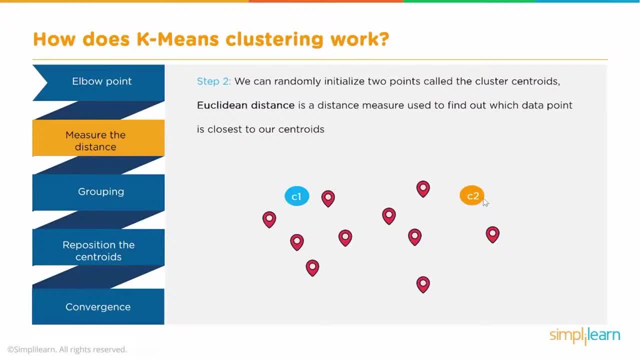 closest to c1, whereas this point is far away from c2.. So these points will be assigned: which are close to c1 will be assigned to c1, and these points or locations which are close to c2 will be assigned to c2.. And then so this: 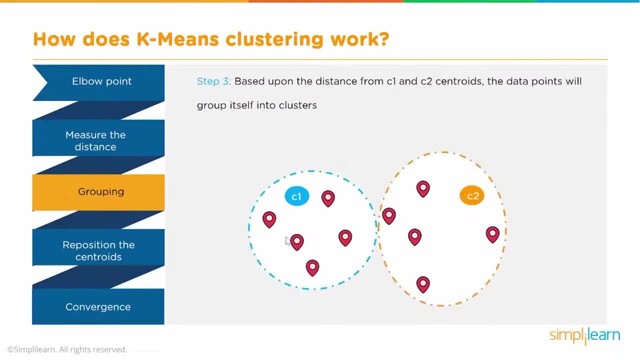 is how the initial grouping is done: This is part of c1 and this is part of c2.. Then the next step is to calculate the actual centroid of this data, because, remember, c1 and c2 are not the centroids, They have been randomly. 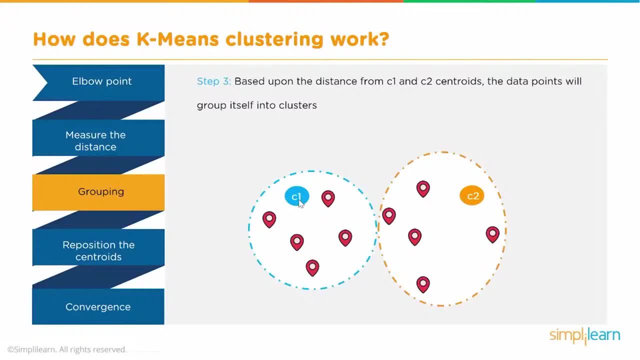 assigned points, and only thing that has been done was the data points which are closest to them have been assigned. But now, in this step, the actual centroid will be calculated, which may be for each of these data sets somewhere in the middle. So that's like the 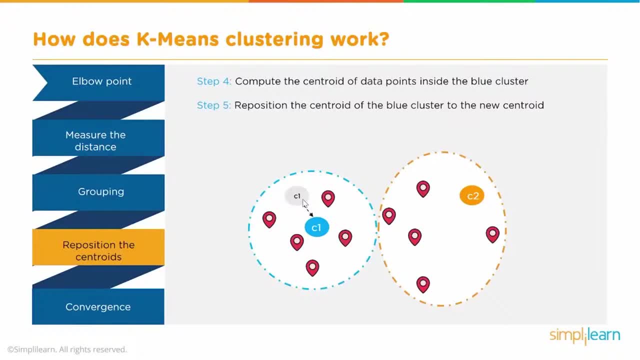 mean point. that will be calculated and the centroid will actually be positioned or repositioned there Same with c2.. So the new centroid for this group is c2, in this new position and c1 is in this new position Once again, the distance of each of the data. 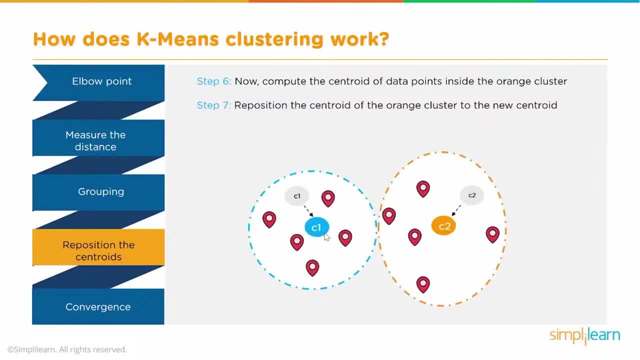 points is calculated from these centroids. Now remember, it's not necessary that the distance still remains the or each of these data points still remain in the same group. By recalculating the distance, it may be possible that some points get reallocated like, so See this: 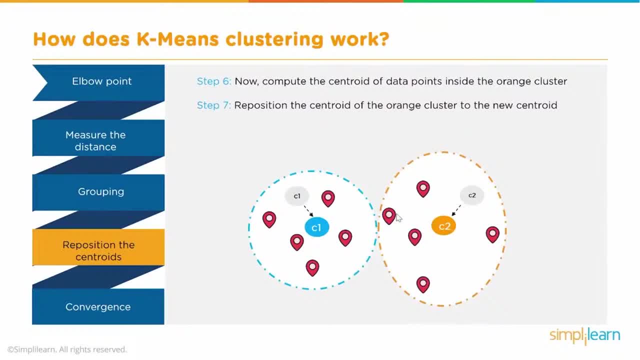 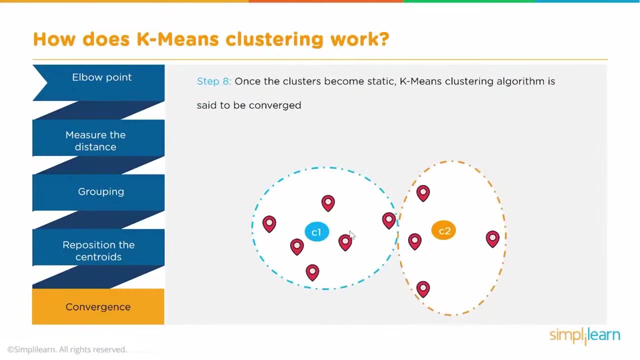 So this point earlier was closer to c2 because c2 was here. but after recalculating repositioning it is observed that this is closer to c1 than c2.. So this is the new grouping. So some points will be reassigned and 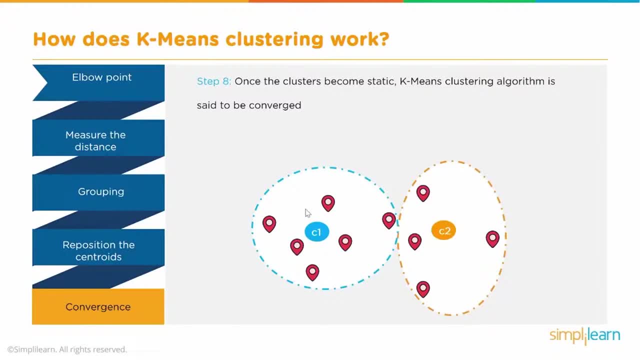 again, the centroid will be calculated. and if the centroid doesn't change, so that is a repetitive process, iterative process- and if the centroid doesn't change, once the centroid stops changing, that means the algorithm has converged. and this is our final cluster, With this as the 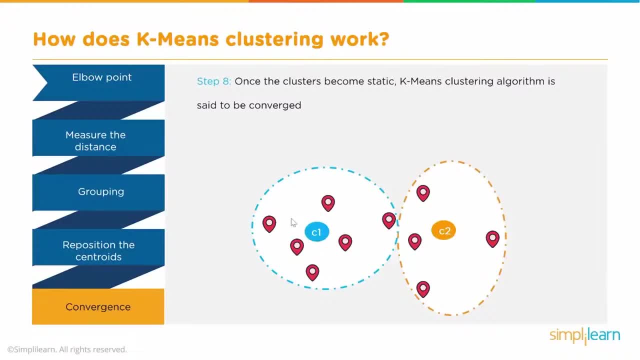 centroid c1 and c2 as the centroids. these data points as a part of each cluster. So I hope this helps in understanding the whole process. iterative process of k-means clustering. So let's take a look at the k-means clustering algorithm. 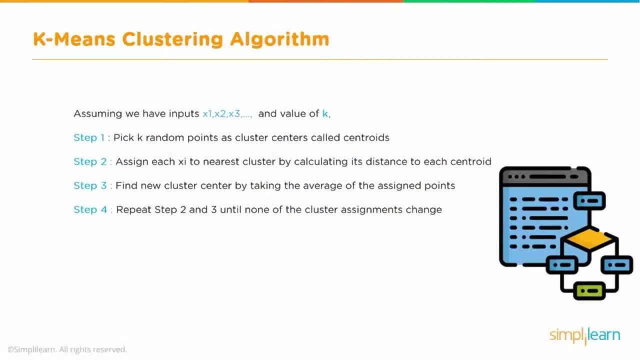 Let's say we have x1,, x2, x3- n number of points as our inputs and we want to split this into k clusters or we want to create k clusters. So the first step is to randomly pick k points and call them centroids. 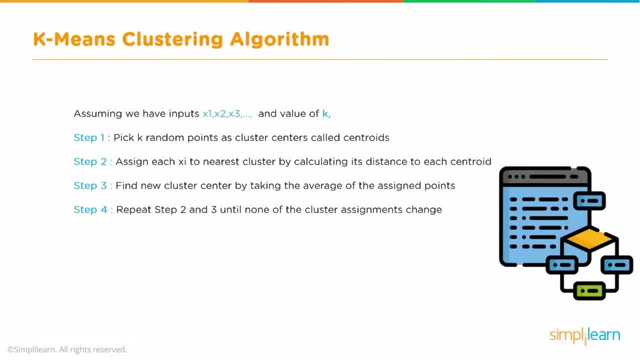 They are not real centroids, because centroid is supposed to be a center point, but they are just called centroids and we calculate the distance of each and every input point from each of the centroids. So the distance of x1 from c1, from c2, c3. 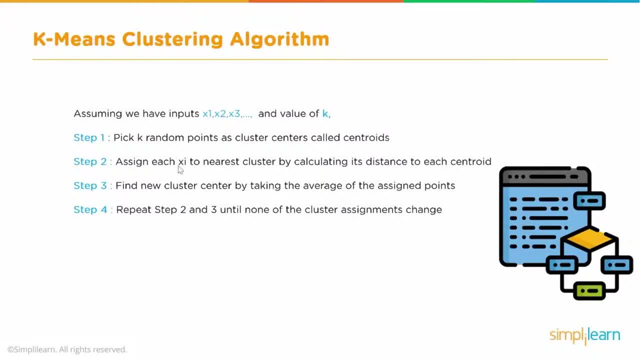 each of the distances we calculate and then find out which distance is the lowest and assign x1 to that particular random centroid. Repeat that process for x2.. Calculate its distance from each of the centroids c1,, c2, c3 to ck and find which is the lowest distance. 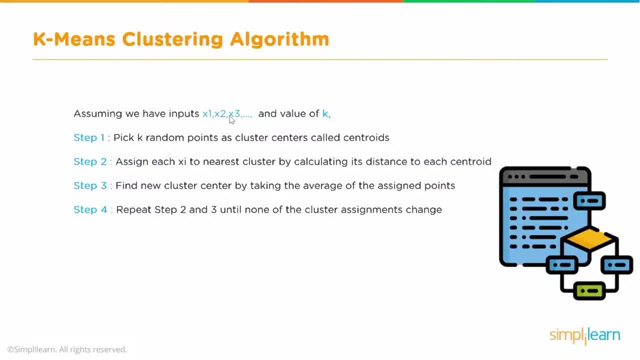 and assign x2 to that particular centroid, Same with x3, and so on. So that is the first round of assignment that is done. Now we have k groups, because there are. we have assigned the value of k, so there are k centroids, and so there are. 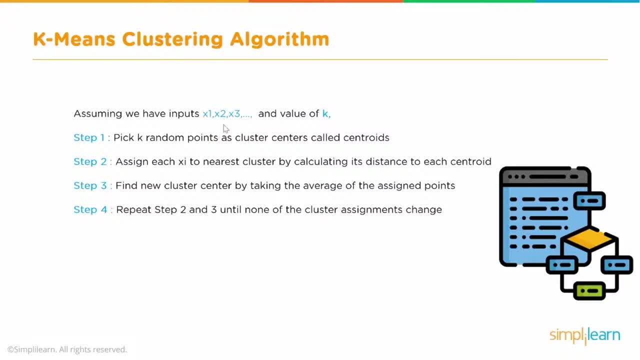 k groups. All these inputs have been split into k groups. However, remember we picked the centroids randomly, so they are not real centroids. So now what we have to do? we have to calculate the actual centroids for each of these groups, which is like the mean position, Which means that 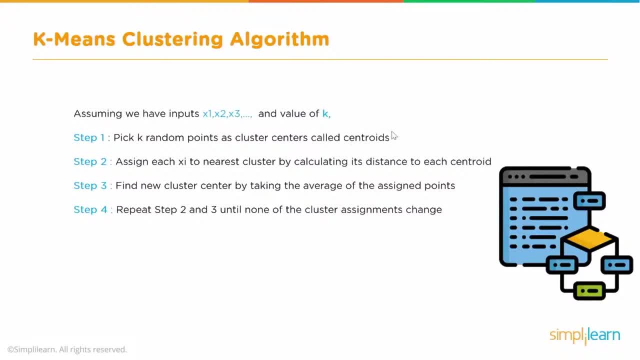 the position of the randomly selected centroids will now change and they will be the mean positions of these newly formed k groups, And once that is done, we once again repeat this process of calculating the distance. So this is what we are doing as a part of 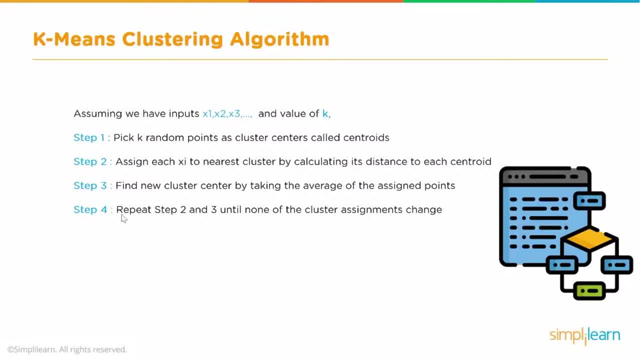 step 4.. We repeat step 2 and 3. So we again calculate the distance of x1 from the centroid c1,, c2,, c3 and then c, which is the lowest value, and assign x1 to that, Calculate the distance of x2 from. 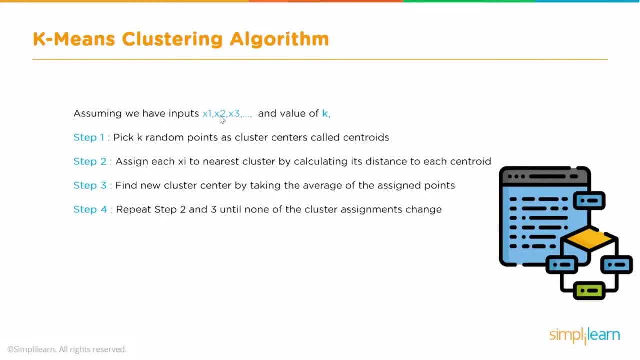 c1, c2, c3 or whatever up to ck and find whichever is the lowest distance and assign x2 to that centroid and so on. In this process there may be some reassignment. x1 was probably assigned to cluster c2 and after. 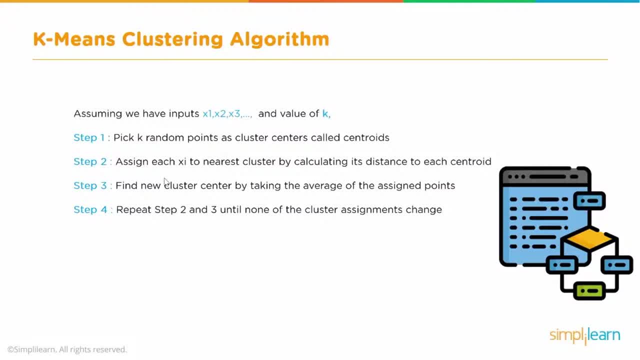 doing this calculation. maybe now x1 is assigned to c1. So that kind of reallocation may happen. So we repeat steps 2 and 3 till the position of the centroids. don't change or stop changing, and that's when we have convergence. 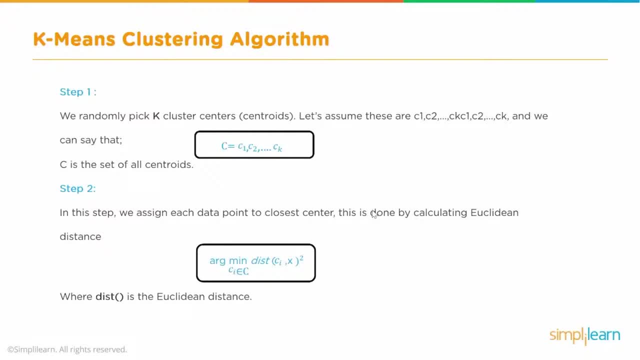 So let's take a detailed look at each of these steps. So we randomly pick k cluster centers. We call them centroids because they are not initially. they are not really the centroids, So we let us name them c1, c2, up to ck, and 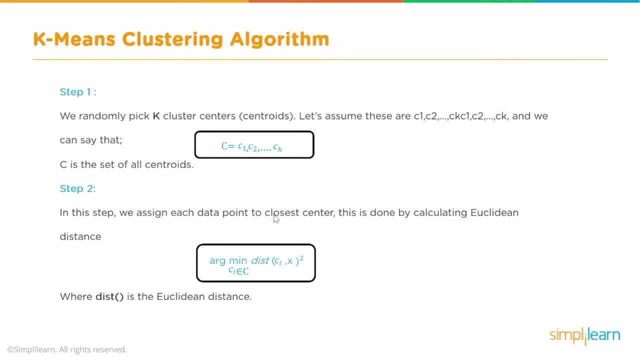 then step 2: we assign each data point to the closest center. So what we do? we calculate the distance of each x value from each c value. So the distance between x1, c1.. Distance between x1, c2, x1, c3, and then 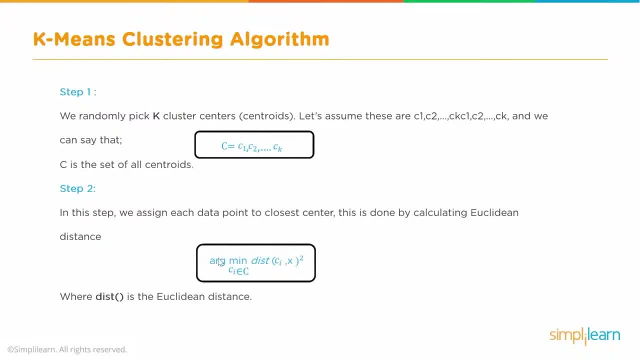 we find which is the lowest value and that's the minimum value. we find and assign x1 to that particular centroid. Then we go next to x2, find the distance of x2 from c1, x2 from c2, x2 from c3 and so on. 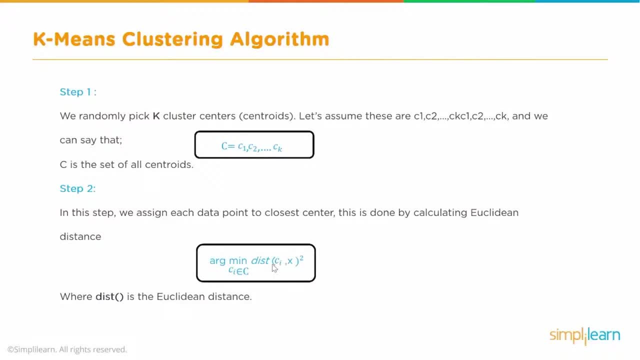 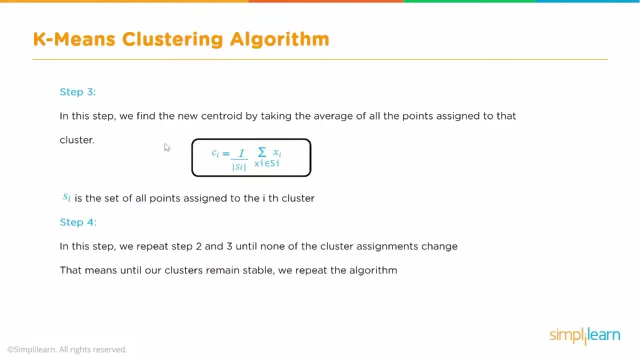 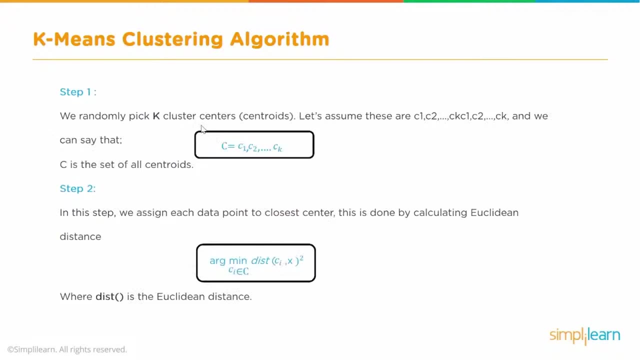 up to ck and then assign it to the point of the centroid which has the lowest value, and so on. So that is step number 2.. In step number 3 we now find the actual centroid for each group. So what has happened as a part of step number 2? 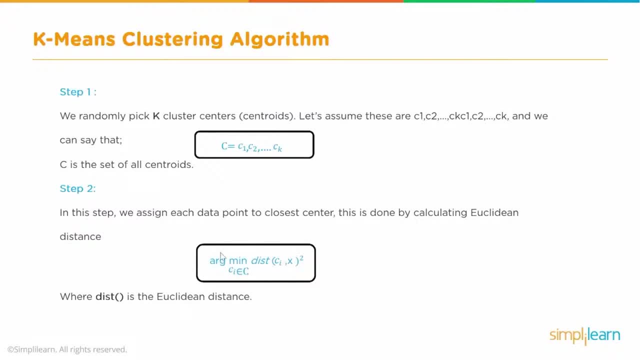 we now have all the points, all the data points, grouped into k groups because we wanted to create k clusters. So we have k groups, Each one may be having a certain number of input values. They need not be equal, distributed by the way Based. 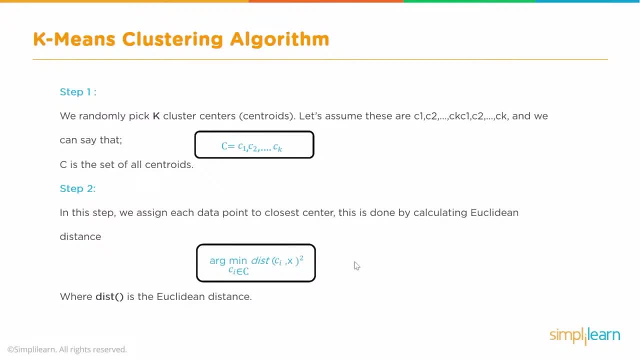 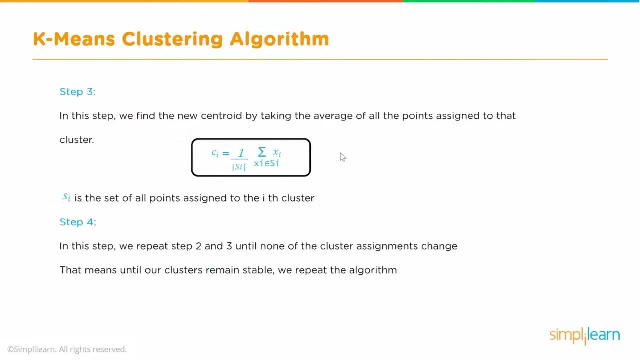 on the distance. we will have k groups, But remember, the initial values of the c1, c2 were not really the centroids of these groups. We assigned them randomly. So now in step 3 we actually calculate the centroid of each group, which means the original. 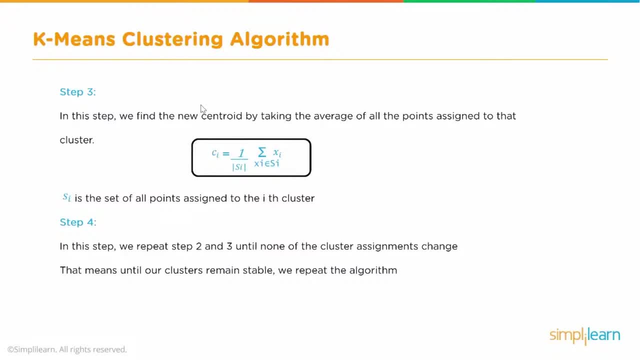 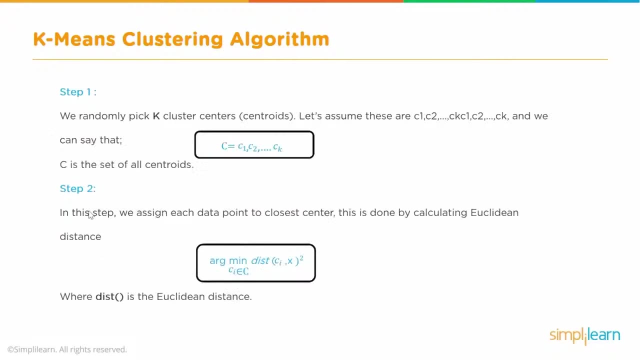 point which we thought was the centroid, will shift to the new position, which is the actual centroid for each of these groups, And we again calculate the distance. So we go back to step 2, which is what We calculate again, the distance of each of these points from the newly. 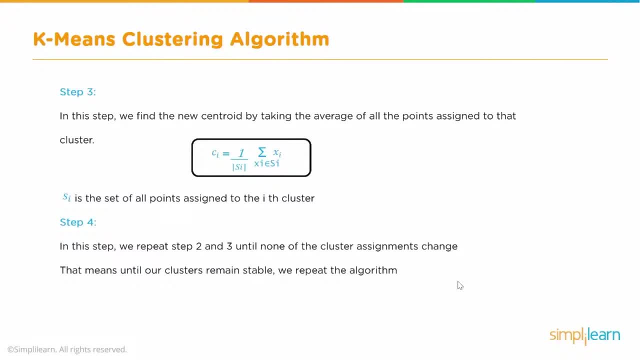 positioned centroids and, if required, we reassign these points to the new centroids. So, as I said earlier, there may be a reallocation. So we now have a new set or a new group. We still have k groups, but the number of items and the actual assignment may be. 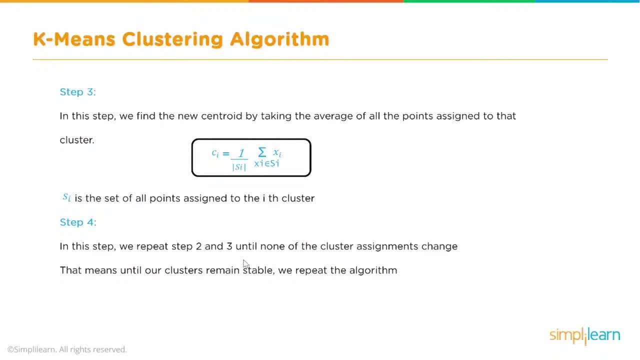 different from what was in step 2 here, So that might change. Then we perform step 3 once again to find the new centroid of this new group. So we have again a new set of clusters, new centroids and new assignments. We repeat this. 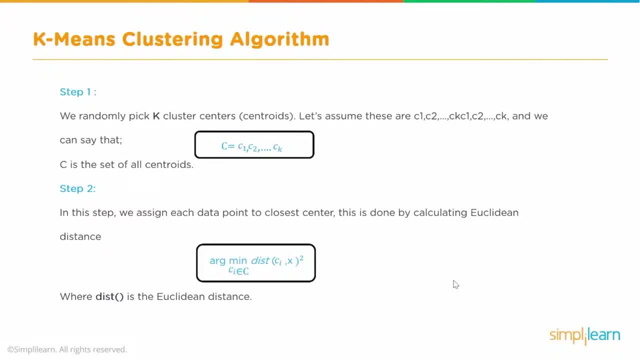 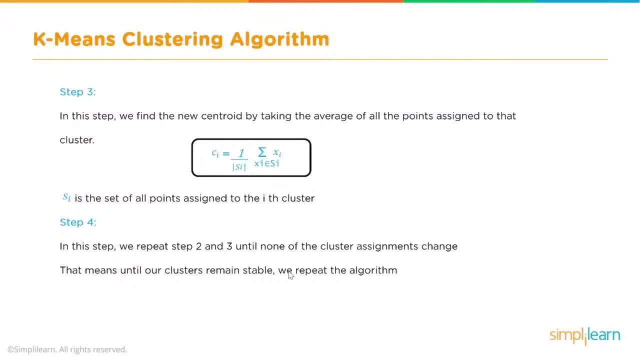 step 2, again. Once again, we find, and then it is possible that after iterating through 3 or 4 or 5 times, the centroid will stop moving, In the sense that when you calculate the new value of the centroid, that will be same as the original value, or 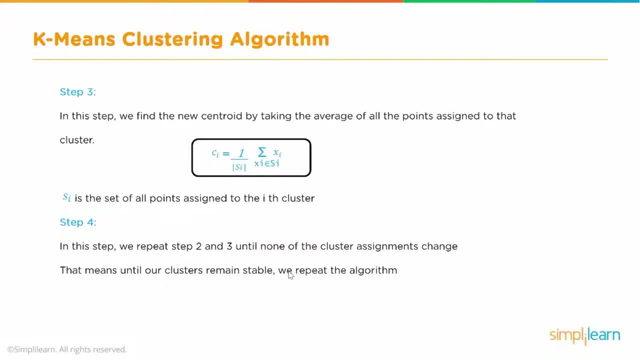 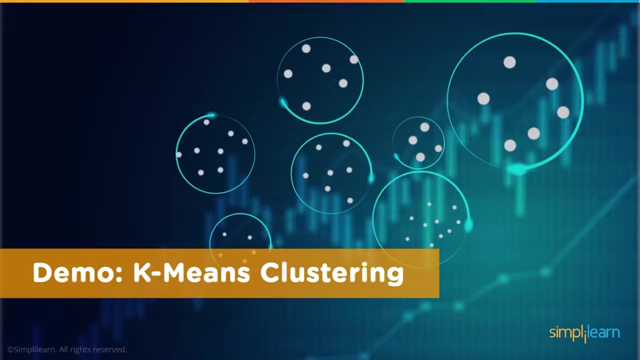 there will be very marginal change. So that is when we say convergence has occurred and that is our final cluster. That is the formation of the final cluster. Alright, so let's see a couple of demos of k-means clustering. We will actually see some. 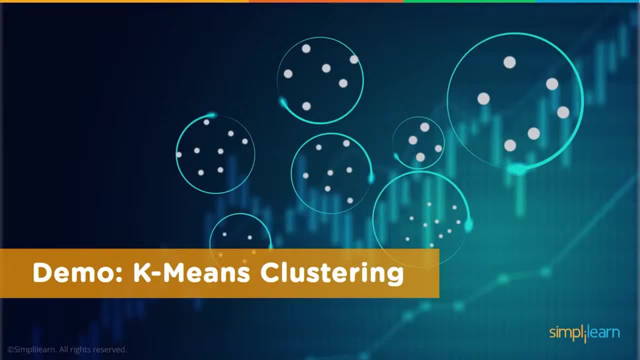 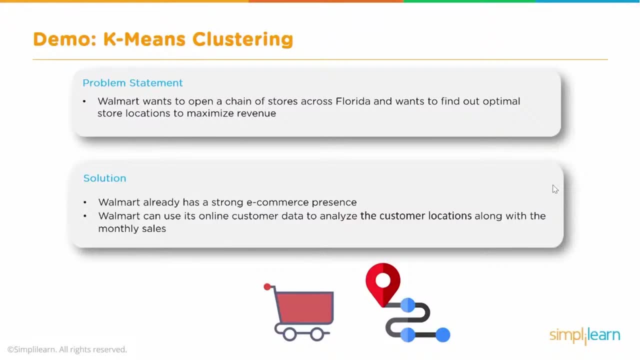 live demos in Python Notebook using Python Notebook. But before that, let's find out what's the problem that we are trying to solve. The problem statement is: let's say, Walmart wants to open a chain of stores across the state of Florida and it wants to find the optimal. 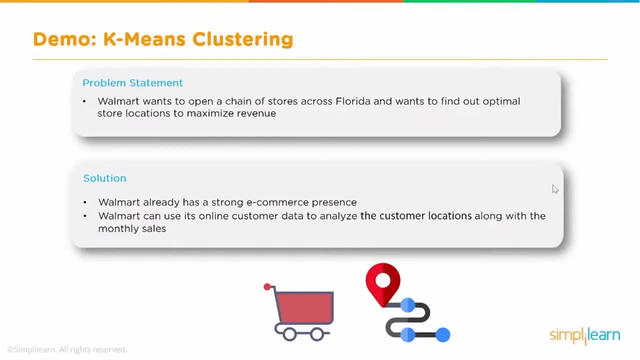 store locations. Now the issue here is: if they open too many stores close to each other, obviously they will not make profit, But if the stores are too far apart, then they will not have enough sales. So how do they optimize this Now for an organization like Walmart? 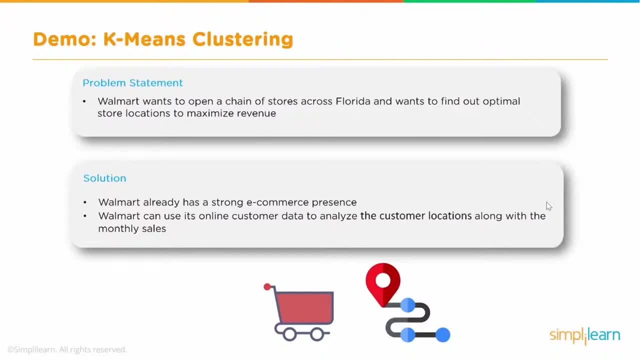 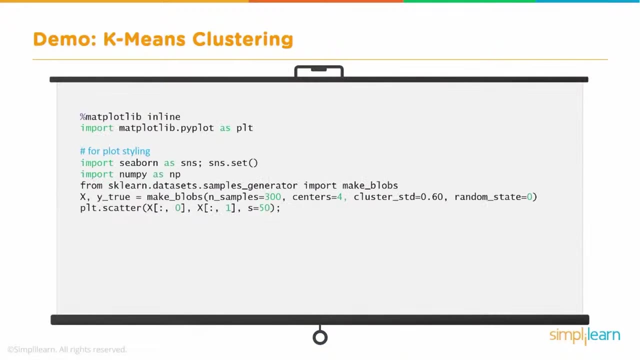 which is an e-commerce giant. they already have the addresses of their customers in their database, So they can actually use this information or this data, and use k-means clustering to find the optimal location. Now, before we go into the Python Notebook and show you the 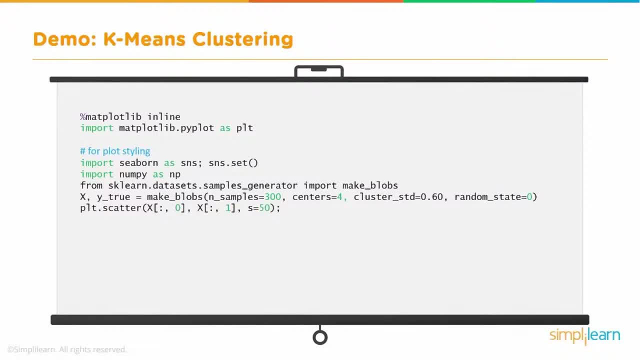 live code. I wanted to take you through very quickly a summary of the code in the slides and then we will go into the Python Notebook. So in this block we are basically importing all the required libraries like numpy, matplotlib and so on, And we are loading the 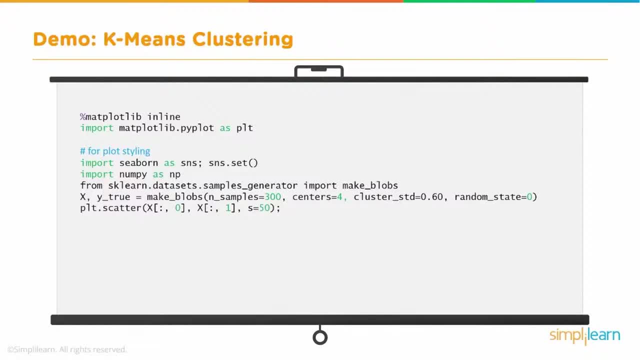 data that is available in the form of, let's say, the addresses. for simplicity sake, we will just take them as some data points. Then the next thing we do is quickly do a scatter plot to see how they are related to each other with respect to each other. So in the scatter, 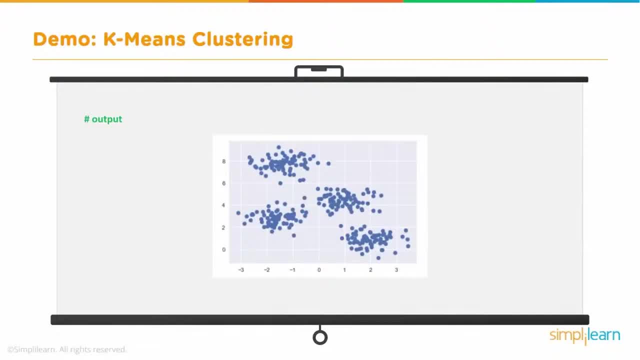 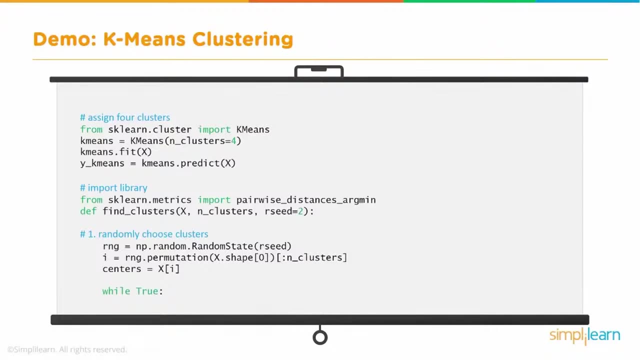 plot we see that there are a few distinct groups already being formed, So you can actually get an idea about how the cluster would look and how many clusters, what is the optimal number of clusters? And then starts the actual k-means clustering process. So we 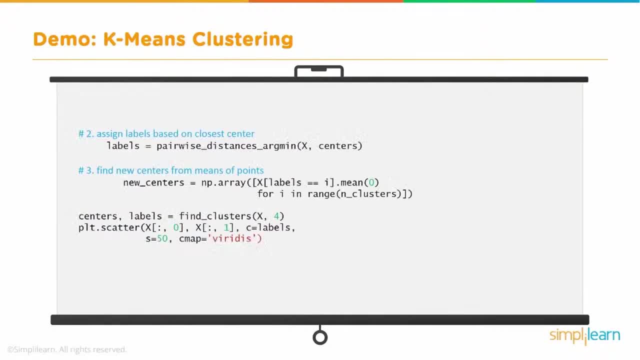 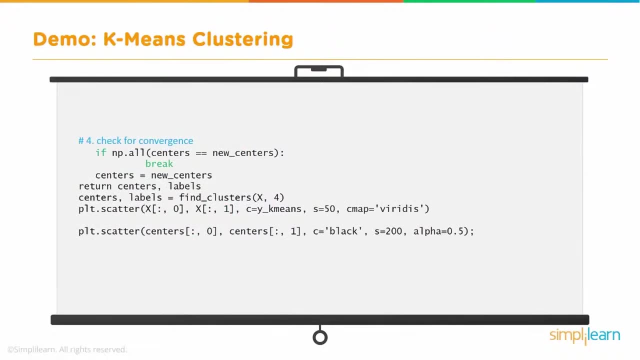 will assign each of these points to the centroids and then check whether they are the optimal distance, which is the shortest distance, and assign each of the points- data points- to the centroids and then go through this iterative process till the whole process converges And finally we get an. 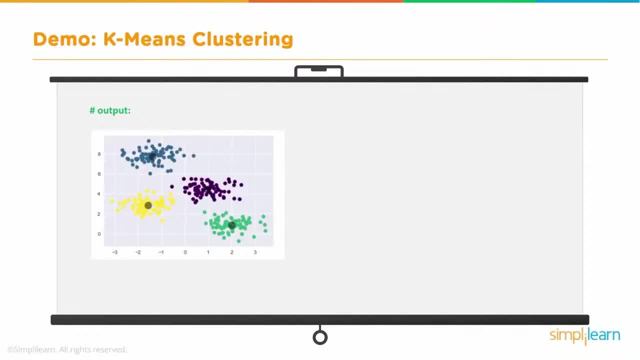 output like this. So we have four distinct clusters and which is? we can say that this is how the population is probably distributed across Florida state, and the centroids are like the location where the store should be, The optimum location where the store should be. So 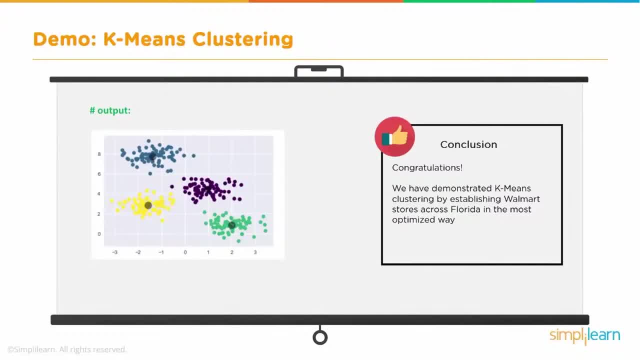 that's the way we determine the best locations for the store and that's how we can help Walmart find the best locations for their stores in Florida. So now let's take this into Python notebook. Let's see how this looks when we are running the code live. 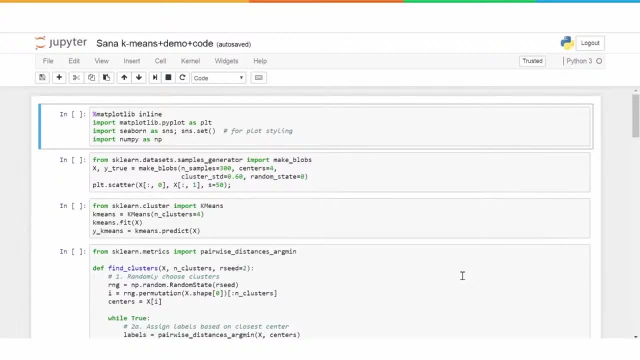 Alright, so this is the code for k-means clustering in Jupyter Notebook. We have a few examples here which we will demonstrate how k-means clustering is used, and even there is a small implementation of k-means clustering as well. Okay, so let's get started. 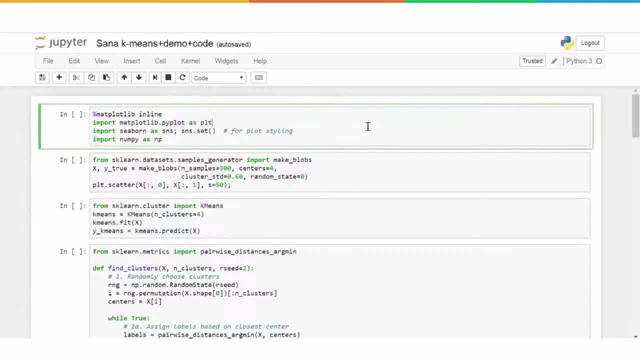 Okay, so this block is basically importing the various libraries that are required, like matplotlib and numpy and so on and so forth, which would be used as a part of the code. Then we are going and creating blobs which are similar to clusters. Now, this is a very 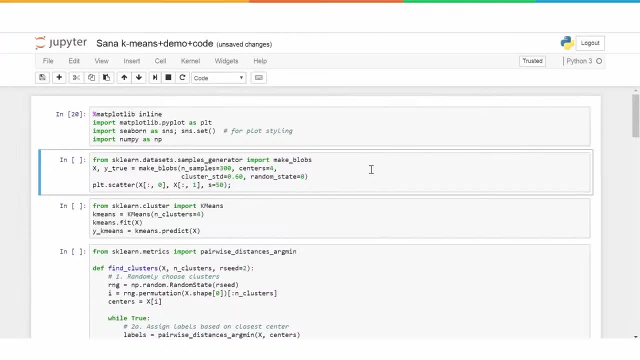 neat feature which is available in scikit-learn. Make blobs is a nice feature which creates clusters of datasets, So that's a wonderful functionality that is readily available for us to create some test data kind of thing. Okay, so that's exactly what we are doing here. We 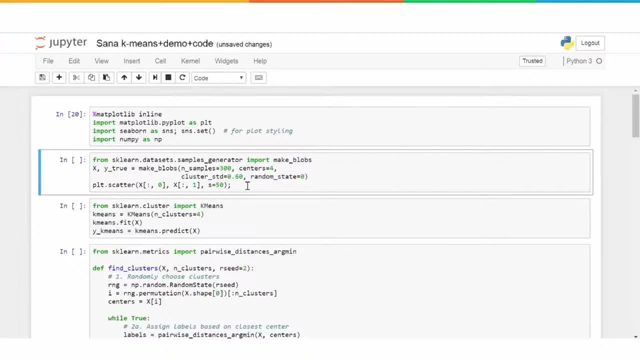 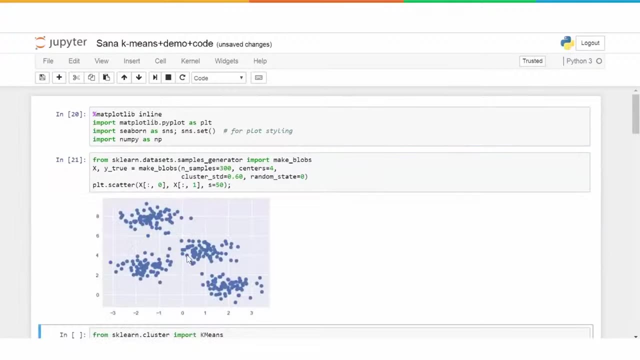 are using, make blobs and we can specify how many clusters we want. So centers we are mentioning here, So it will go ahead, and so we just mentioned four. so it will go ahead and create some test data for us and this is how it looks, as you can see Visually. 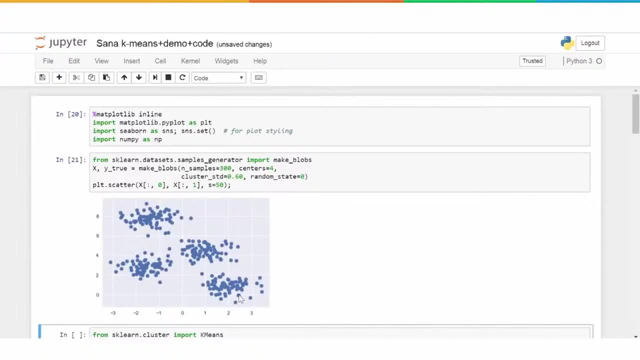 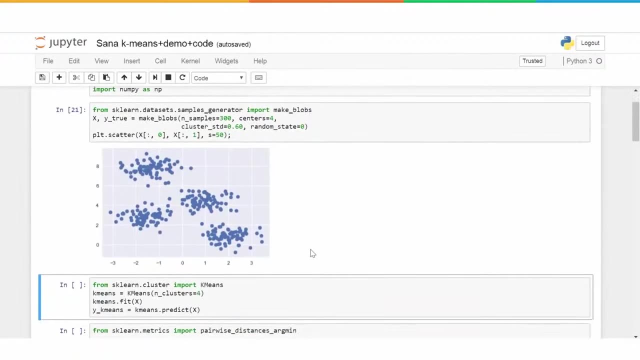 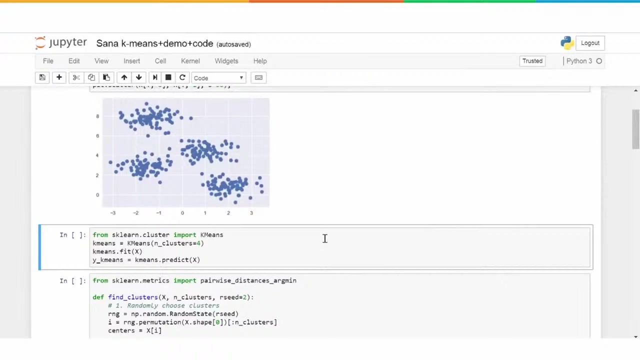 also, we can figure out that there are four distinct classes or clusters in this dataset, and that is what make blobs actually provides. Now, from here onwards, we will basically run the standard k-means functionality that is readily available, So we really don't have to implement. 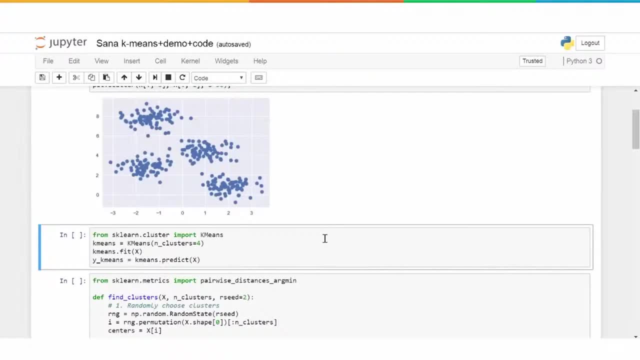 k-means itself. The k-means functionality or the function is readily available. You just need to feed the data and create the clusters. So this is the code for that: We import k-means and then we create an instance of k-means. 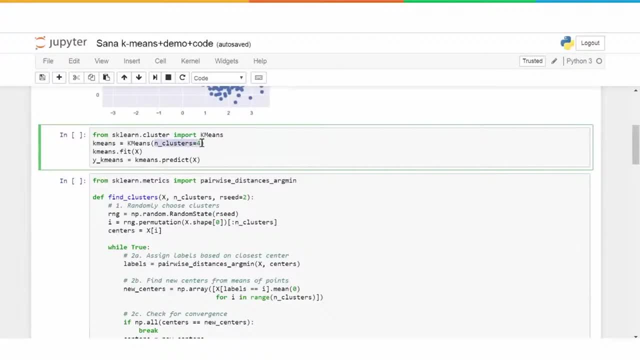 and we specify the value of k. This n underscore clusters- is the value of k, Remember k-means and k-means. k is basically the number of clusters that you want to create and it is an integer value. So this is where we are specifying that. So 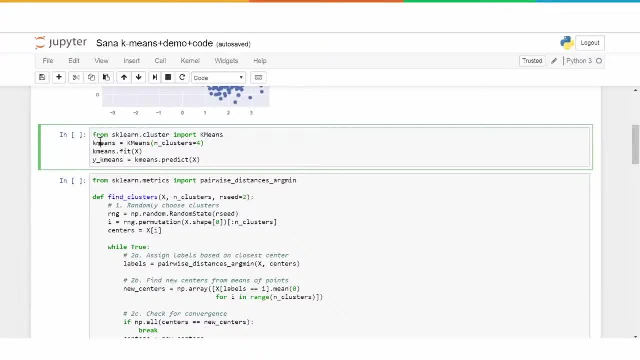 we have, k is equal to four, and so that instance is created. We take that instance and, as with any other machine learning functionality, fit is what we use, The function or the method. rather, fit is what we use to train the model. Here there is no real training. 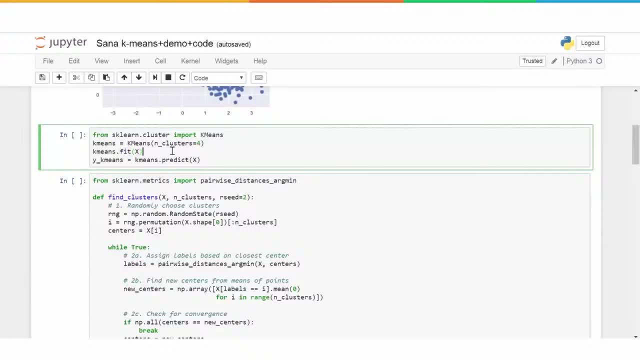 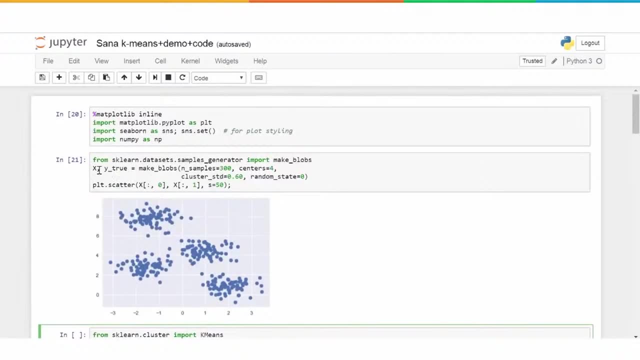 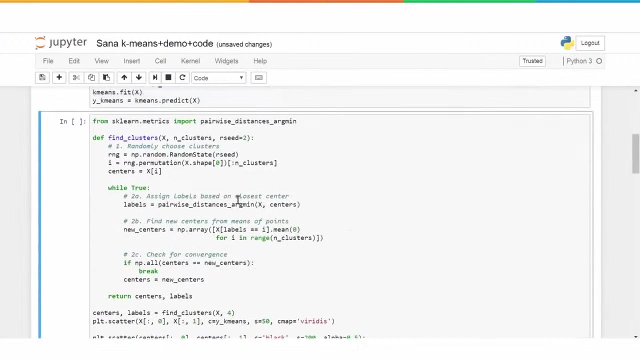 kind of thing. but that is the call, So we are calling fit and what we are doing here. we are just passing the data, So x has these values, the data that has been created. So that is what we are passing here and this will go ahead and create. 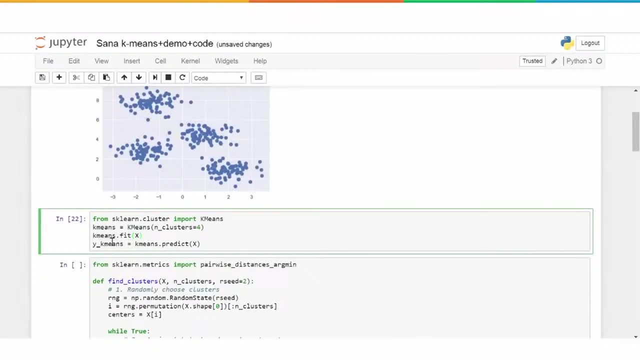 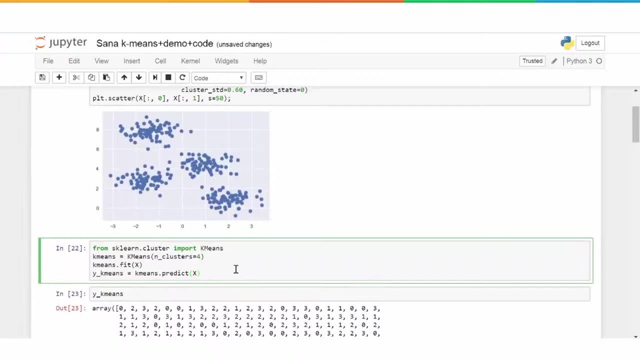 the clusters and then we are using, after doing fit, we run the predict, which basically assigns for each of these observations which cluster it belongs to. So it will name the clusters. maybe this is cluster 1, this is 2,, 3 and so on, or 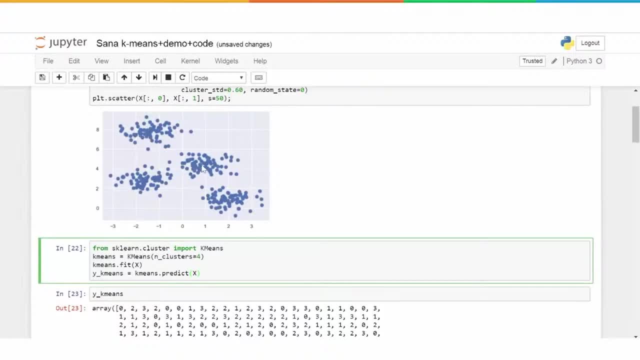 it will actually start from 0 cluster 0,, 1,, 2 and 3 maybe, and then for each of the observations it will assign, based on which cluster it belongs to, it will assign a value. So that is stored in y, underscore k means. 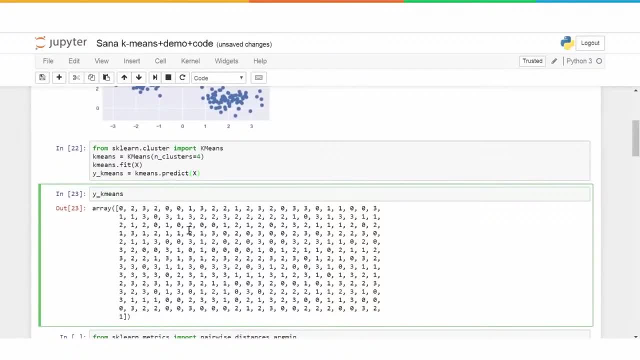 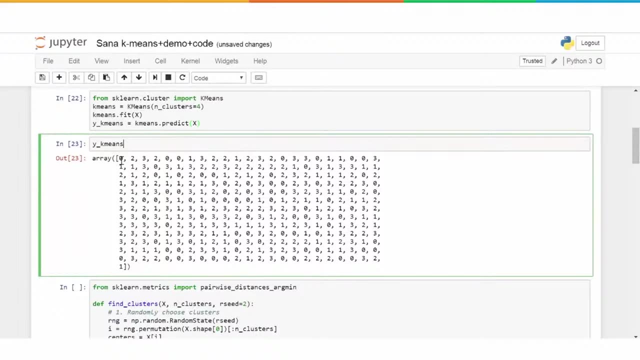 when we call predict, that is what it does, and we can take a quick look at these y underscore, k means or the cluster numbers that have been assigned for each observation. So this is the cluster number assigned for observation 1. maybe this is for observation 2, observation 3 and so. 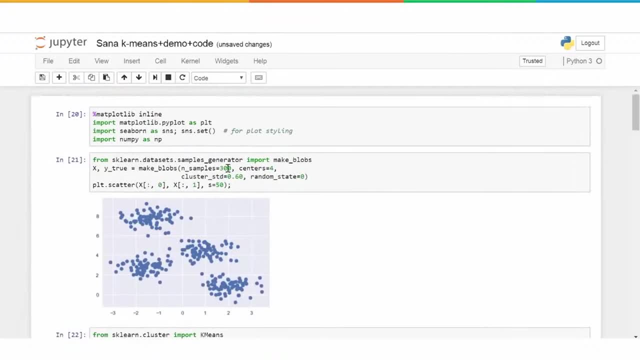 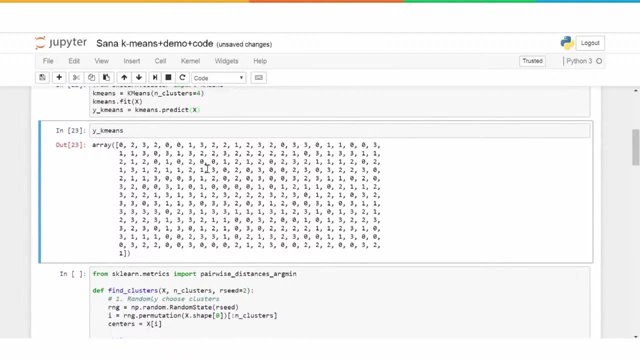 on. so we have how many about? I think, 300 samples, right? so all the 300 samples. there are 300 values here. Each of them the cluster number is given and the cluster number goes from 0 to 3.. So there are 4 clusters. 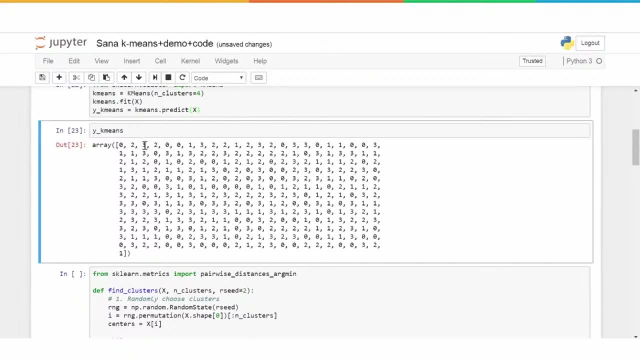 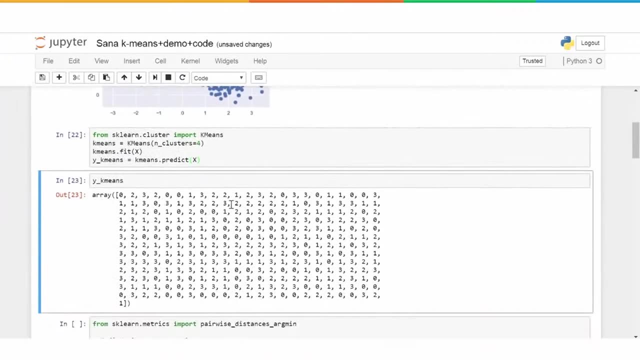 so the numbers go from 0, 1,, 2, 3. so that is what is seen here. Okay now. so this was a quick example of generating some dummy data and then clustering that. okay, and this can be applied. if you have proper data, you can just load it. 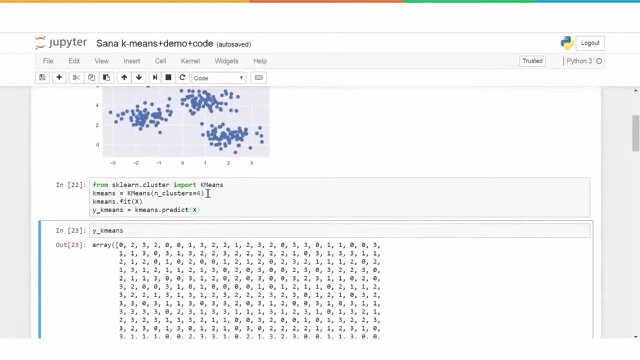 up into x, for example here, and then run the k means. So this is the central part of the k means, clustering program example. so you basically create an instance and you mention how many clusters you want by specifying this parameter: n underscore clusters and that is also the value of k. 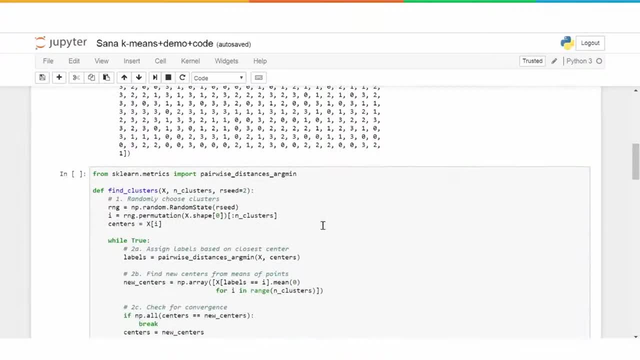 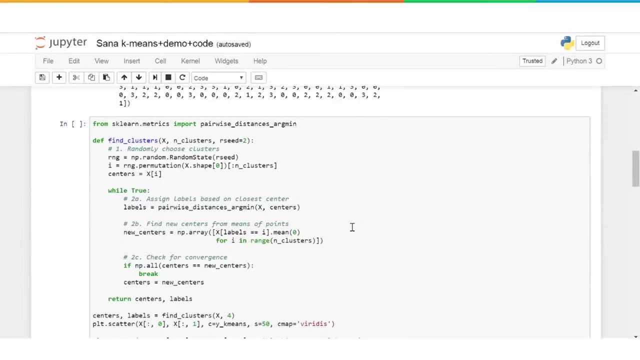 and then pass the data to get the value values. Now the next section of this code is the implementation of a k means. Now, this is kind of a rough implementation of the k means algorithm, so we will just walk you through. I will walk you through the code. 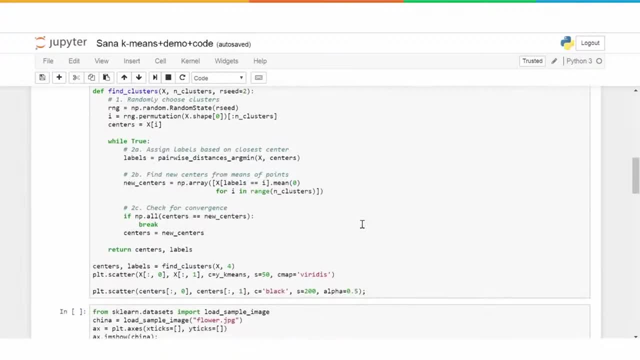 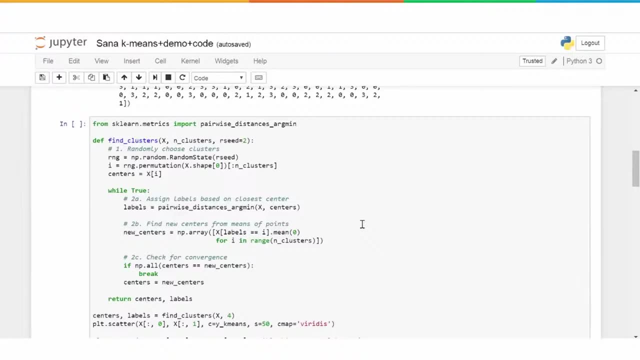 at each step what it is doing, and then we will see a couple of more examples of how k means clustering can be used in maybe some real life examples, real life use cases. alright, So in this case, here what we are doing is basically implementing k means clustering, and 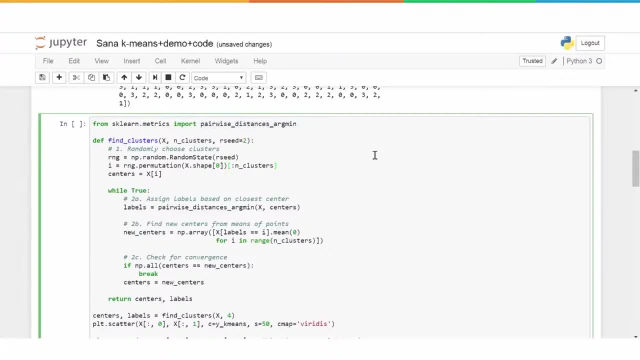 there is a function for a library that calculates for a given two pairs of points. it will calculate the distance between them and see which one is the closest, and so on. so this is like. this is pretty much like what k means does, right? so it calculates the distance of each. 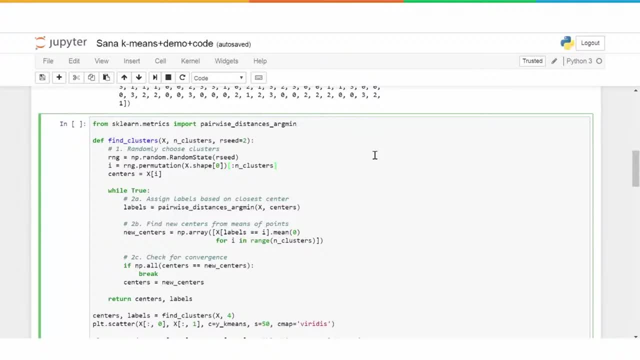 point or each data set from predefined centroid and then, based on whichever is the lowest, this particular data point is assigned to that centroid. so that is basically available as a standard function and we will be using that here. so, as explained in the slides, the first step, that is 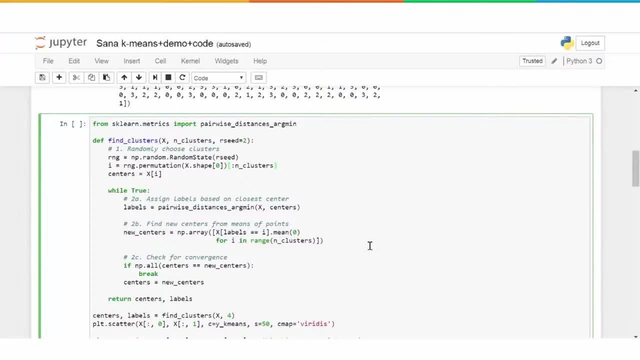 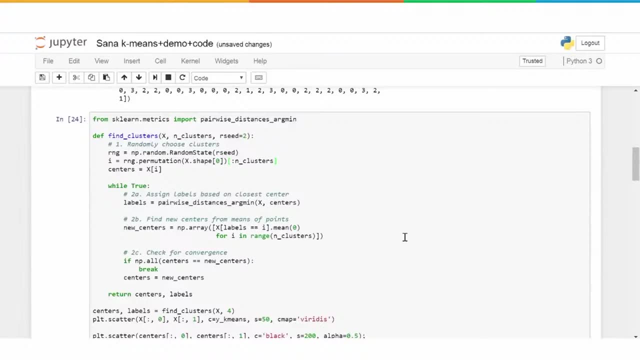 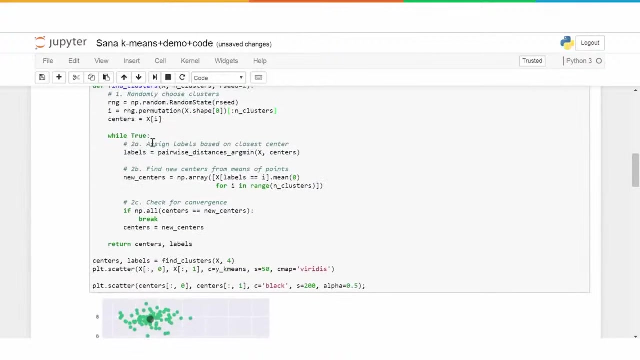 done in case of k means clustering is to randomly assign some centroids. so as a first step we randomly allocate a couple of centroids which we call here we are calling as centers, and then we put this in a loop and we take it through an iterative process for each of the data points we 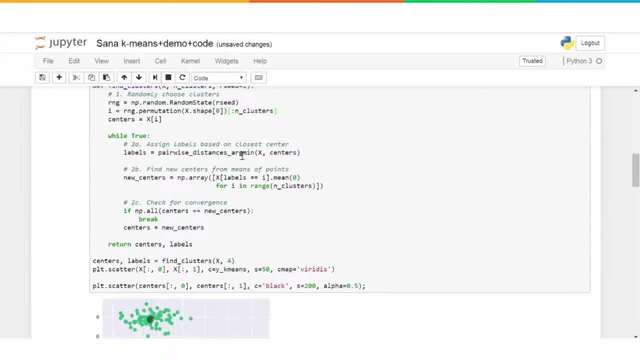 first find out using this function, pairwise distance argument for each of the points we find out which one, which center or which randomly selected centroid is the closest and accordingly we assign that data or the data point to that particular centroid or cluster. and once that is done for all the data points, 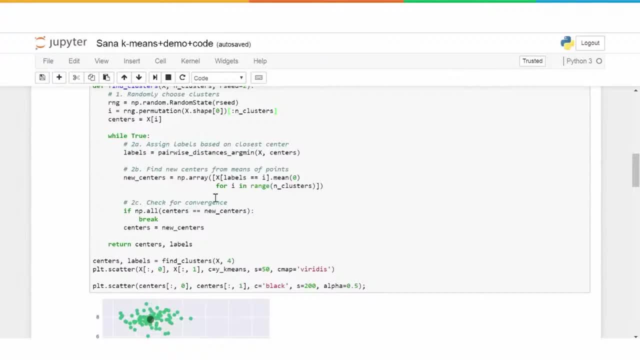 we calculate the new centroid by finding out the mean position, which is the center position, right? so we calculate the new centroid and then we check if the new centroid is the coordinates or the position is the same as the previous centroid. the positions we will compare and if it is the same, 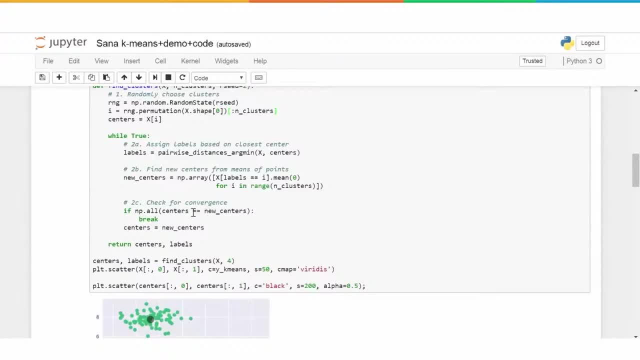 that means the process has converged. so remember, we do this process till the centroid or the centroid doesn't move anymore, right, so the centroid gets relocated each time this relocation is done. so the moment it doesn't change anymore, the position of the centroid doesn't change anymore. we know. 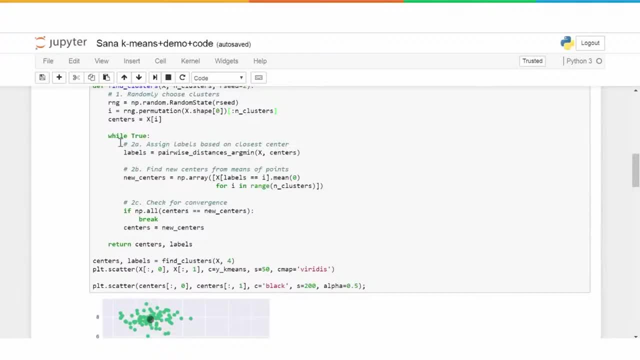 that convergence has occurred. so till then. so you see here this is like an infinite loop. while true is an infinite loop, it only breaks when the centers are the same, the new center and old center positions are the same, and once that is done, we return the centers and the labels. now, of course, 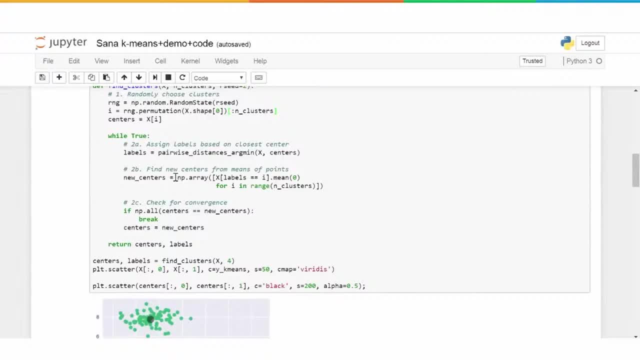 as explained, this is not a very sophisticated and advanced implementation, very basic implementation, because one of the flaws in this is that sometimes what happens is the centroid, the position, will keep moving, but in the change will be very minor. so in that case also, that is actually convergence. 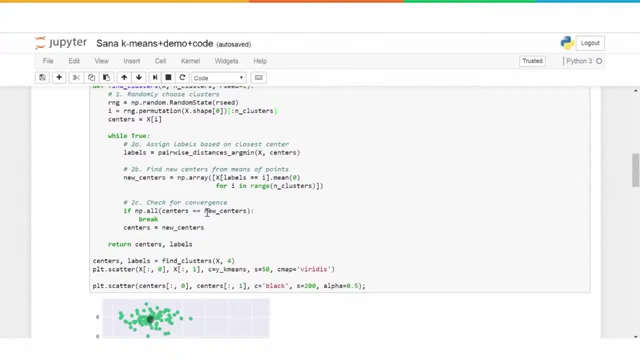 right. so, for example, the change is 0.0001. we can consider that as convergence. otherwise what will happen is this will either take forever or it will be never ending. so that's a small flaw here. so that is something. additional checks may have to be added here, but again, as mentioned, 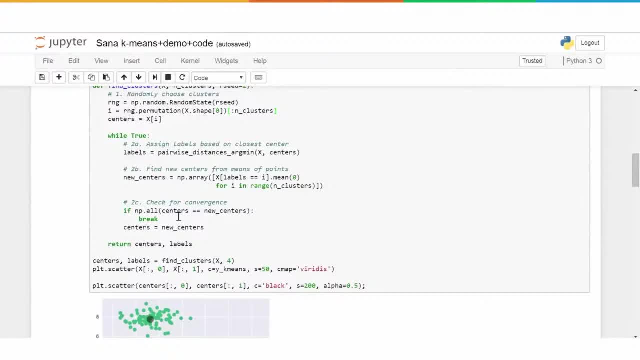 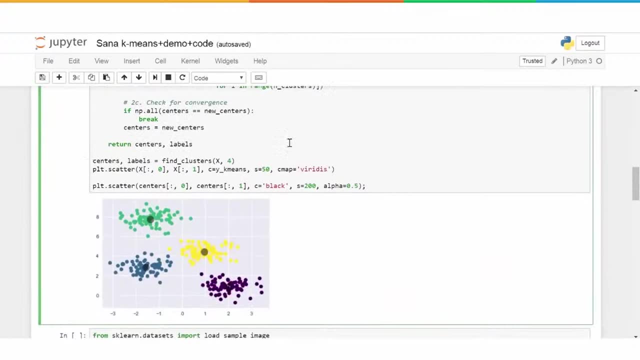 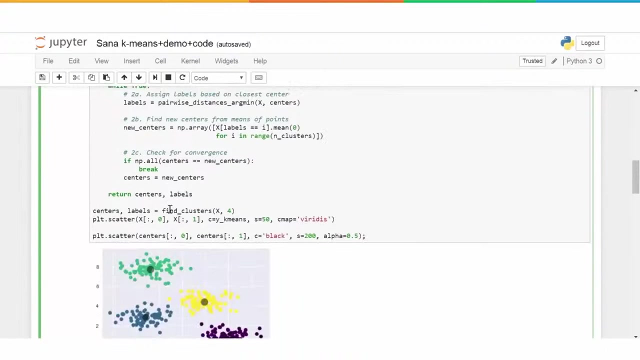 this is not the most sophisticated implementation. this is like a kind of a rough implementation of the k-means clustering. okay, so if we execute this code, this is what we get as the output. so this is the definition of this particular function, and then we call that find underscore clusters and we 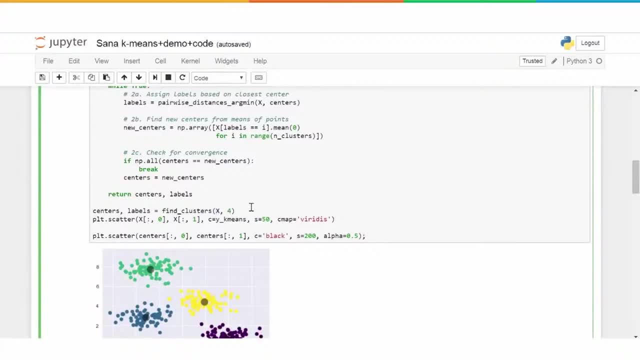 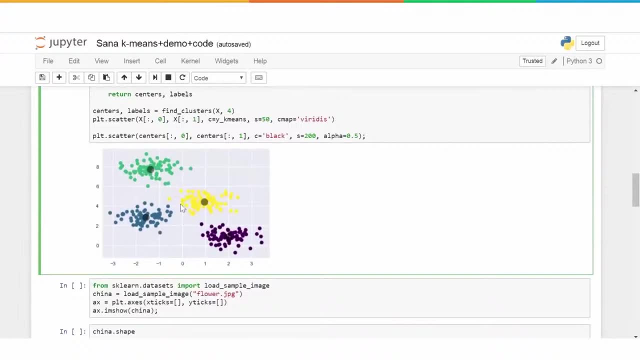 pass our data x and the number of clusters, which is 4, and if we run that and plot it, this is the output that we get. so this is of course. each cluster is represented by a different color, so we have a cluster in green color, yellow color and so on and so forth, and 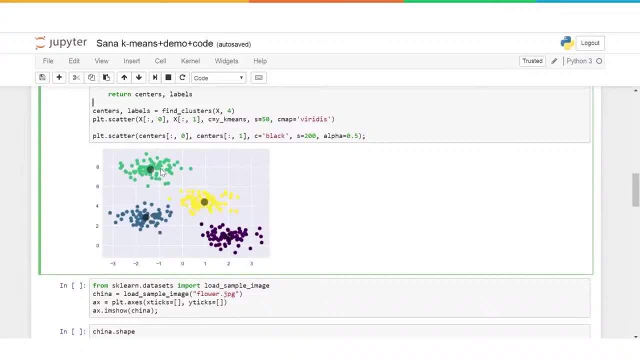 these big points here. these are the centroids. this is the final position of the centroids and, as you can see, visually also, this appears like a kind of a center of all these points here, right. similarly, this is like the center of all these points here, and so on. so 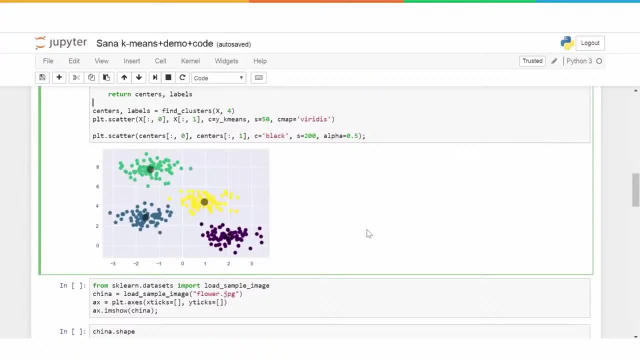 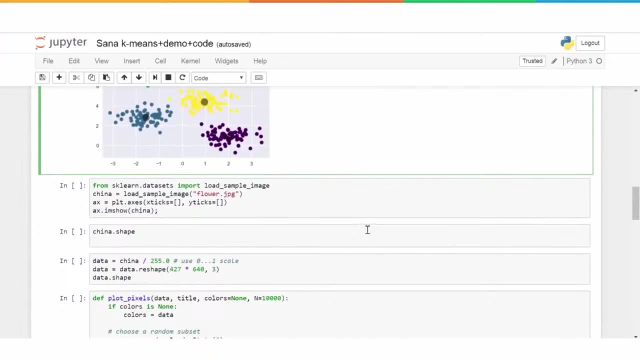 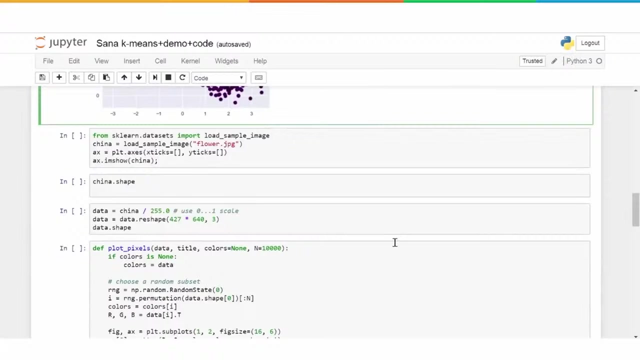 this is the example, or this is an example of a implementation of k-means clustering, and next we will move on to see a couple of examples of how k-means clustering is used in maybe some real life scenarios or use cases. in the next example or demo. 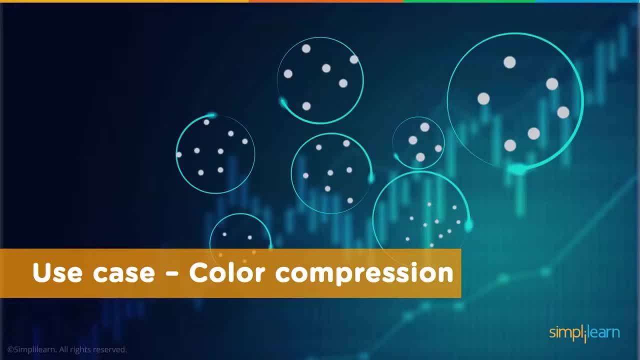 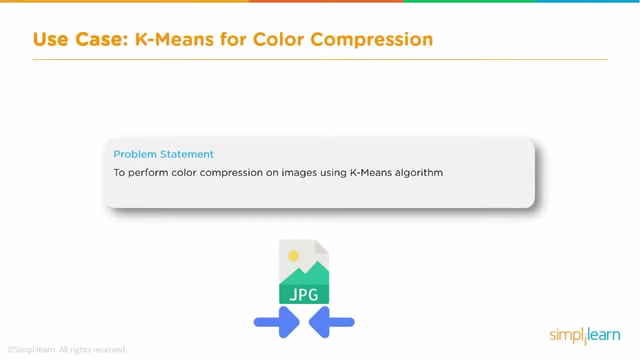 we are going to see how we can use k-means clustering to perform color compression. we will take a couple of images, so there will be two examples, and we will try to use k-means clustering to compress the colors. this is a common situation in image processing. 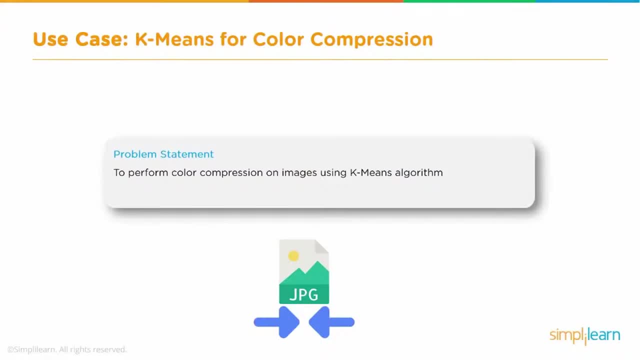 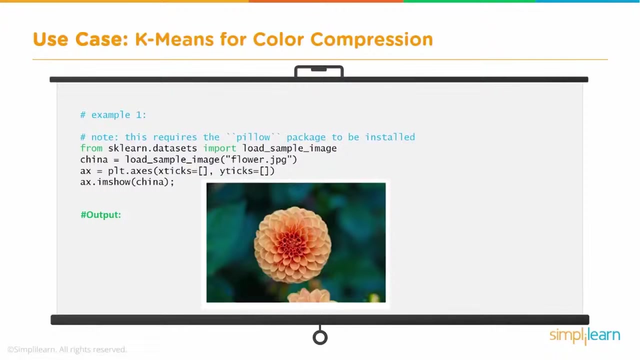 when you have an image with millions of colors, but then you cannot render it on some devices which may not have enough memory. so that is the scenario where something like this can be used. so before again we go into the python notebook, let's take a look at quickly. 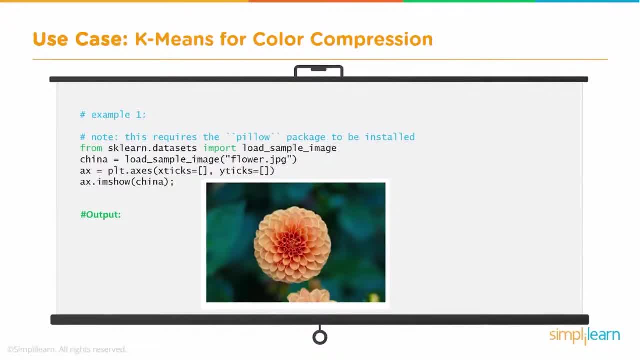 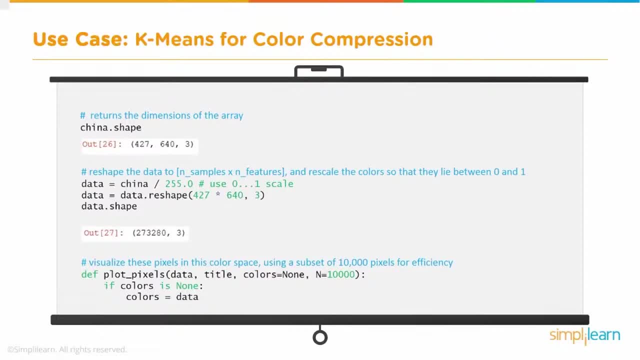 the code. as usual, we import the libraries and then we import the image and then we will flatten it. so the reshaping is basically: we have the image, information is stored in the form of pixels, and if the image is like, for example, 427 by 640, and it has 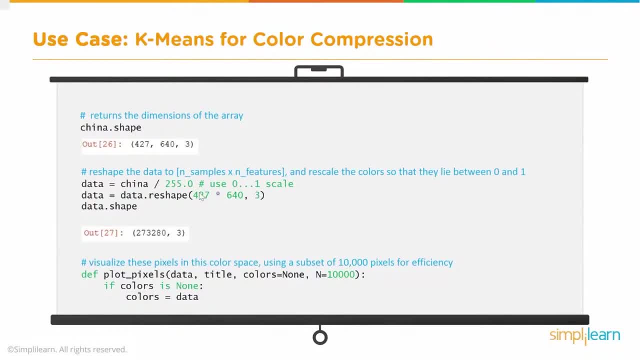 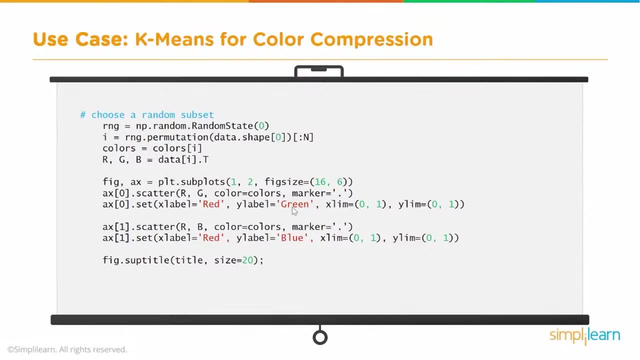 three colors. so that is the overall dimension of the initial image. we just reshape it and then feed this to our algorithm, and this will then create clusters of only 16 clusters. so these colors, there are millions of colors, and now we need to bring it down to 16 colors. 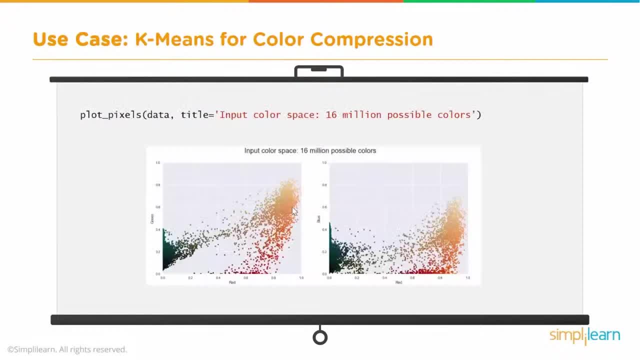 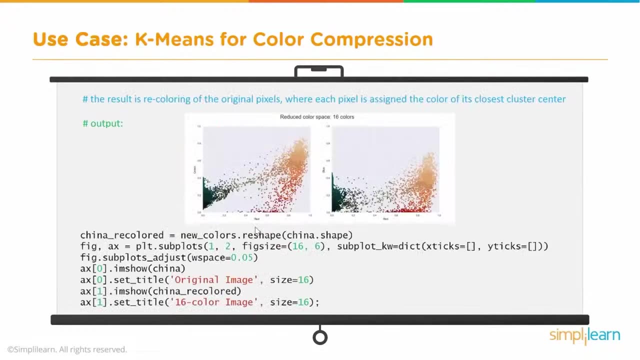 so we use k is equal to 16 and this is how. when we visualize, this is how it looks. these are all about 16 million possible colors. the input color space has 16 million possible colors and we just sub, compress it to 16 colors. so this is how it would look. 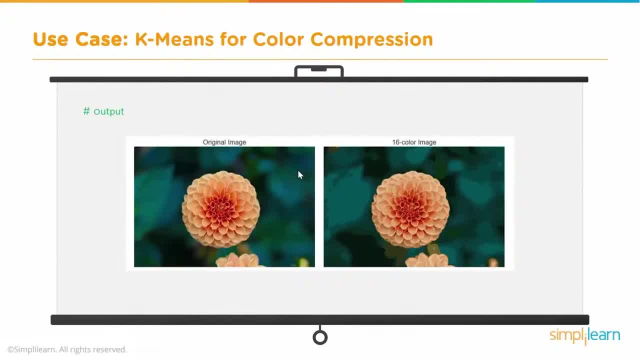 when we compress it to 16 colors, and this is how the original image looks, and after compression to 16 colors, this is how the new image looks. as you can see, there is not a lot of information that has been lost, though the image quality is definitely. 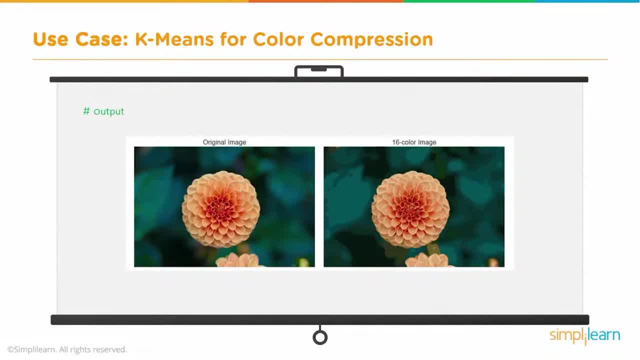 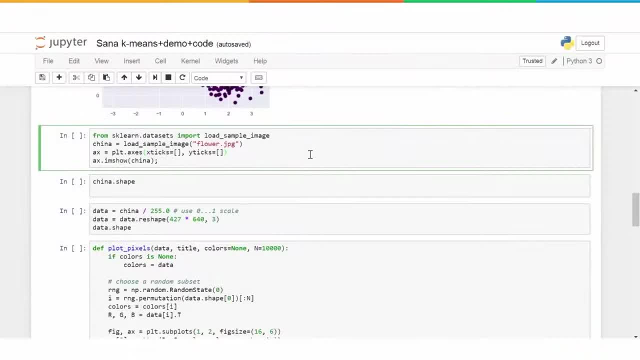 reduced a little bit. so this is an example which we are going to now see in python. let's go into the python and once again, as always, we will import some libraries and load this image called flower dot jpg. ok, so let me load that and this is how it looks. 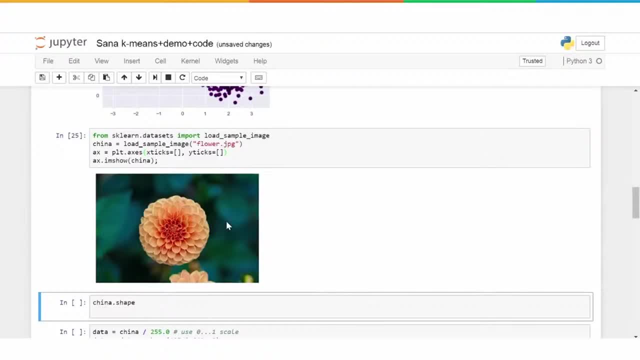 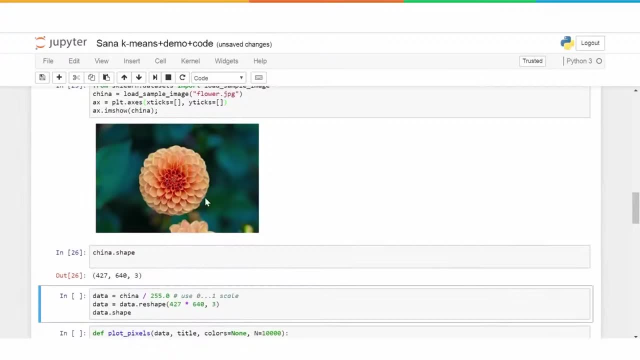 this is the original image, which has, i think, 16 million colors, and this is the shape of this image, which is basically what is? the shape is nothing but the overall size, right? so this is 427 pixel by 640 pixel, and then there are three layers, which is: 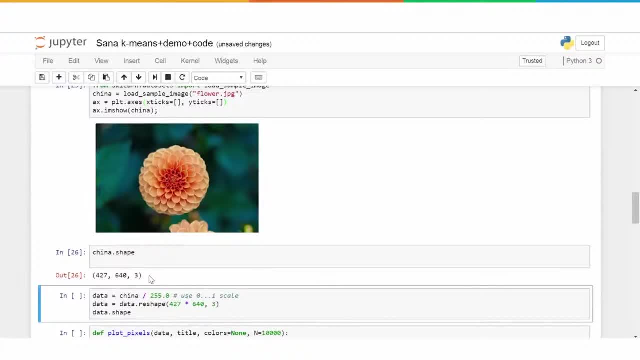 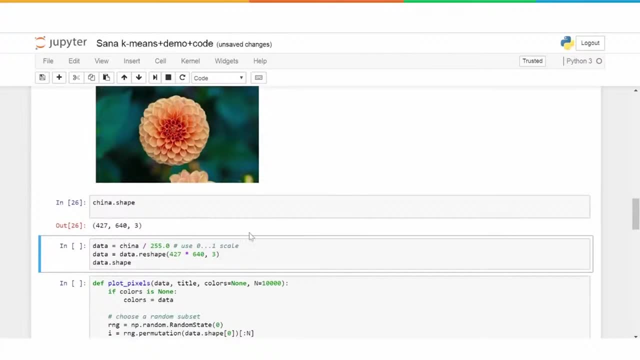 this three basically is for rgb, which is red, green, blue, so color image will have that right. so that is the shape of this. now what we need to do is data. let's take a look at how data is looking. so let me just create a new cell and show you. 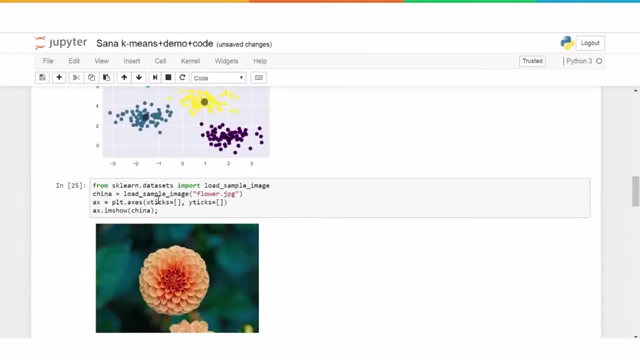 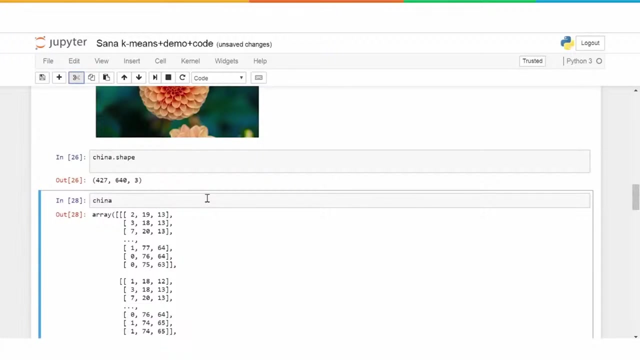 what is in data? basically, we have captured this information, so data is what. let me just show you here. alright, so let's take a look at china. what are the values in china? and if we see here, this is how the data is stored. this is nothing but. 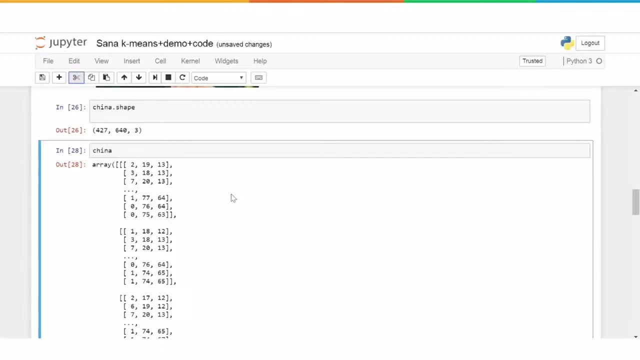 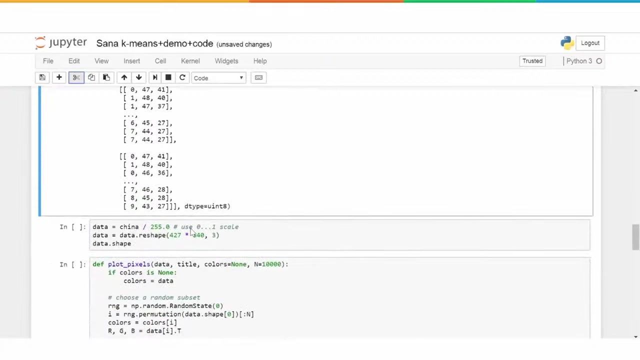 the pixel values. ok, so this is like a matrix and each one has about for this, 427 by 640 pixels. alright, so this is how it looks. now the issue here is: these values are large, the numbers are large, so we need to normalize them to between 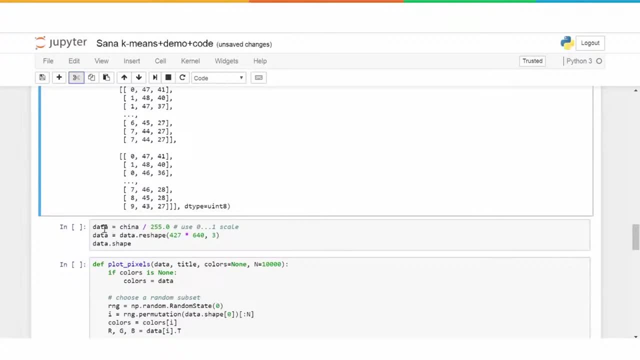 0 and 1, right. so that's why we will basically create one more variable, which is data, which will contain the values between 0 and 1, and the way to do that is divide by 255. so we divide china by 255 and we get the new values in. 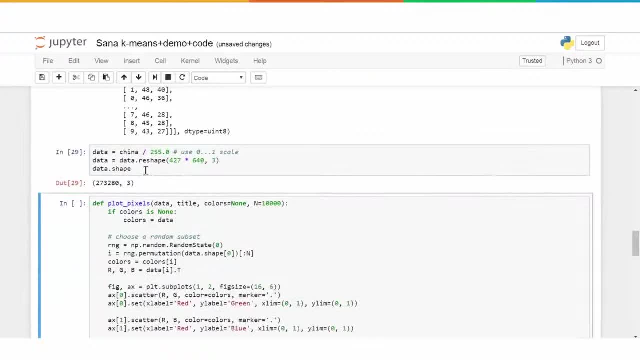 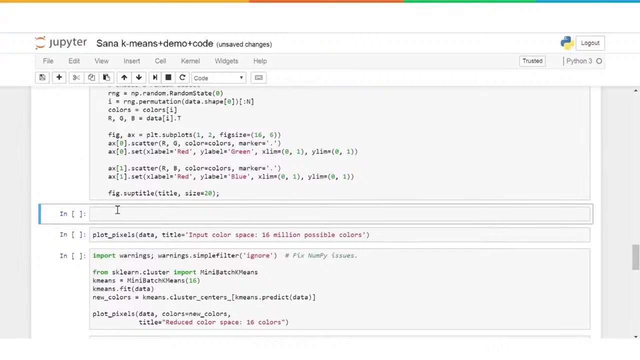 data. so let's just run this piece of code and this is the shape so we now have also. yeah, what we have done is we changed, using reshape, we converted into the three dimensional, into a two dimensional data set. and let us also take a look at how. 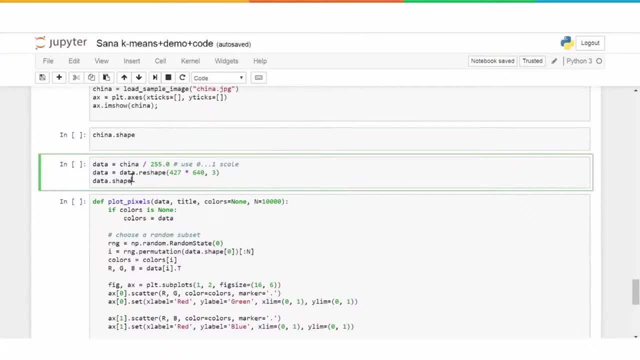 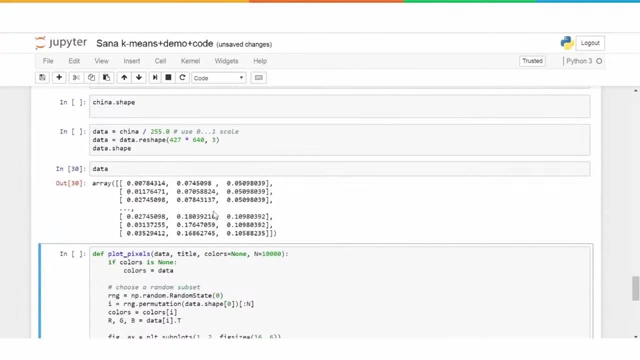 let me just insert, probably a cell here and take a look at how data is looking. alright, so this is how data is looking. and now you see, this is the values are between 0 and 1, right? so, if you earlier noticed, in case of china the values were large numbers. 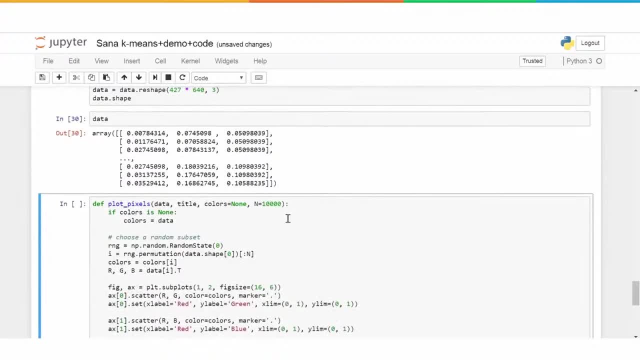 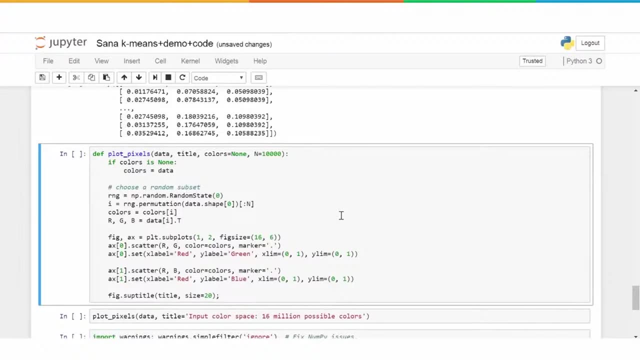 now everything is between 0 and 1. this is one of the things we need to do, alright, so after that, the next thing that we need to do is to visualize this, and we can take random set of maybe 10,000 points and plot it and check. 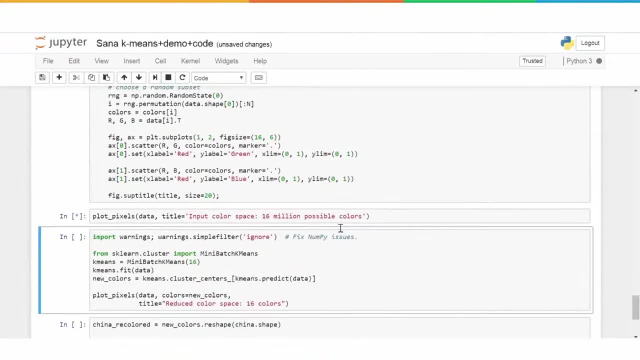 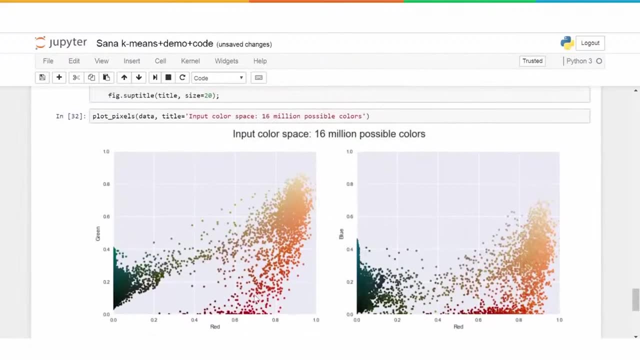 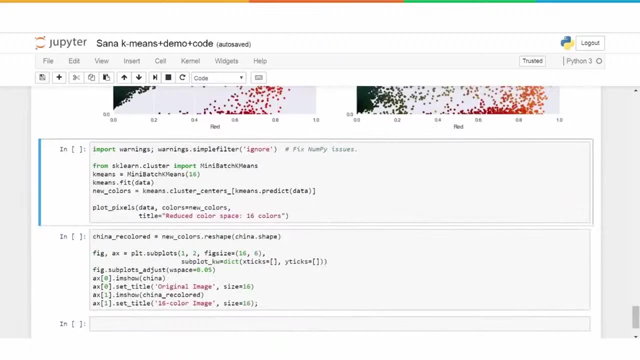 and see how this looks. let us just plot this. and so this is how the original, the color, the pixel distribution is. these are two plots: one is red against green and another is red against blue, and this is the original distribution of the color. so then, what we will do is we will. 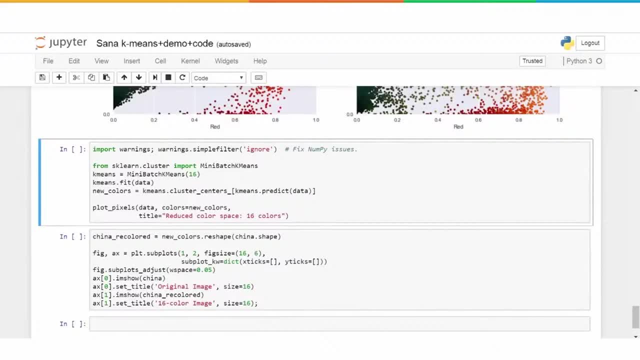 use k-means clustering to create just 16 clusters for the various colors and then apply that to the image. now what will happen is, since the data is large, because there are millions of colors, using regular k-means may be a little time consuming. so there is another. 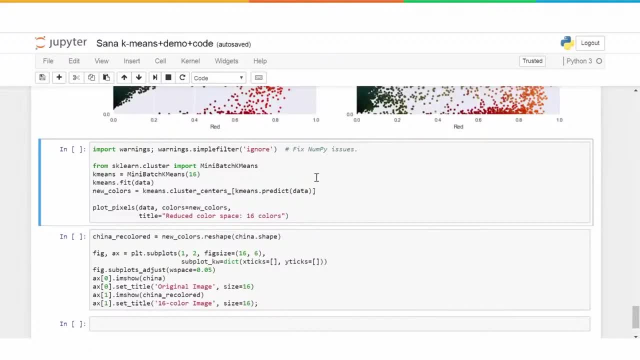 version of k-means which is called mini batch k-means. so we will use that which is, which processes in. the overall concept remains the same, but this basically processes it in smaller batches. that's the only thing. okay, so there is a little bit of a difference between. 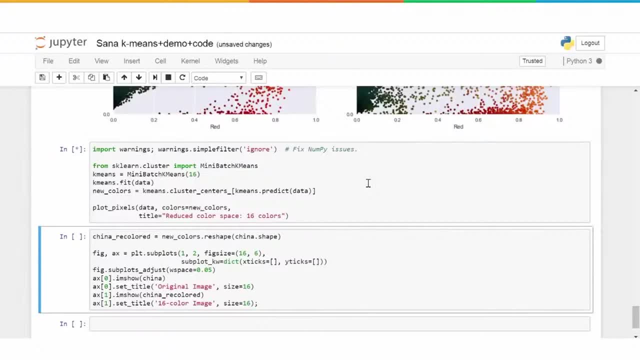 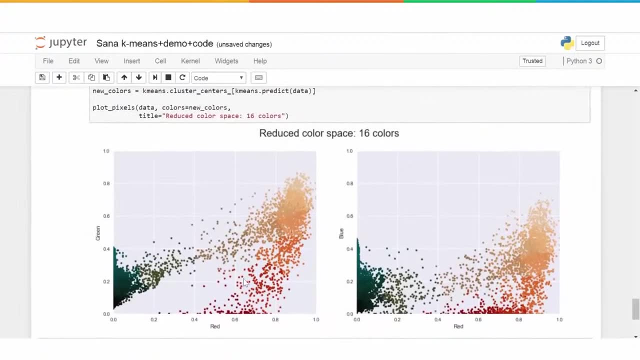 the original and the new, so the results will pretty much be the same. so let's go ahead and execute this piece of code and also visualize this so that we can see that there are these. this is how the 16 colors would look. so this is red against. 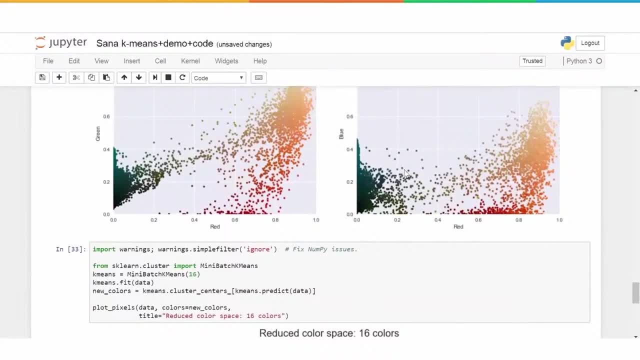 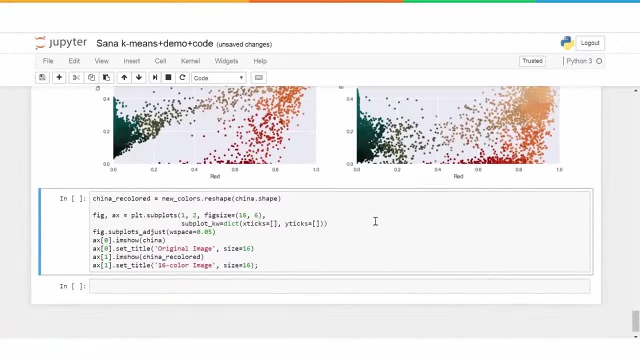 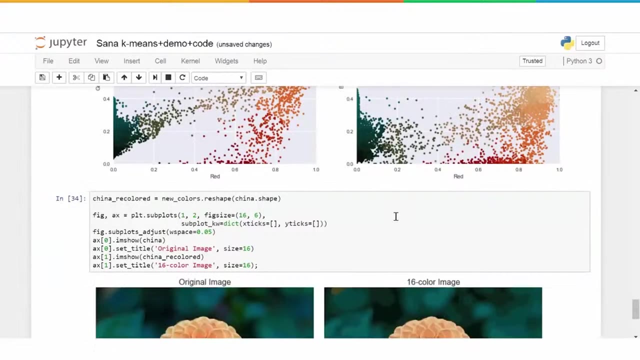 green, and this is red against blue. there is a quite a bit of similarity between this original color schema and the new one, right, so it doesn't look very, very completely different or anything like that. now we apply this, the newly created image, to the image and we can take a look how this is. 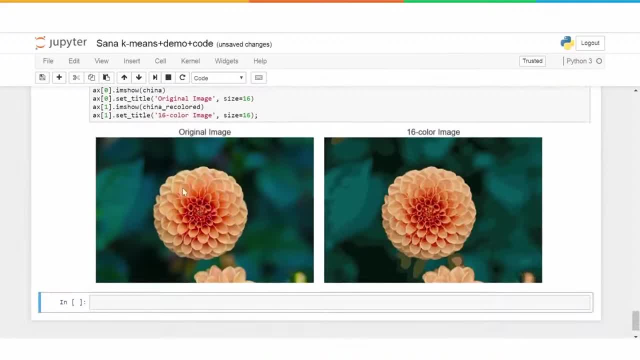 looking. now we can compare both the images. so this is our original image and this is our new image. so, as you can see, there is not a lot of information that has been lost. it pretty much looks like the original image. yes, we can see that. for example, here there is a little. 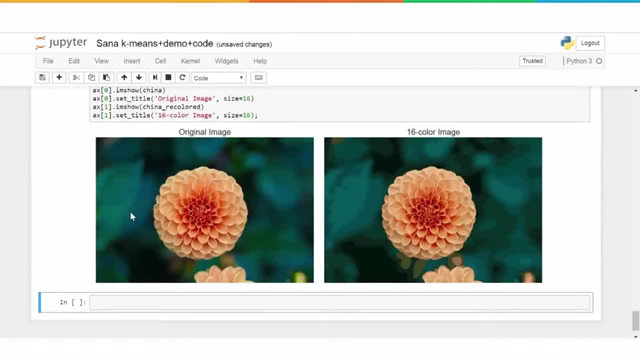 bit. it appears a little dullish compared to this one right, because we kind of took off some of the finer details of the color, but overall the high level information has been maintained. at the same time, the main advantage is that now this can be. this is an image. 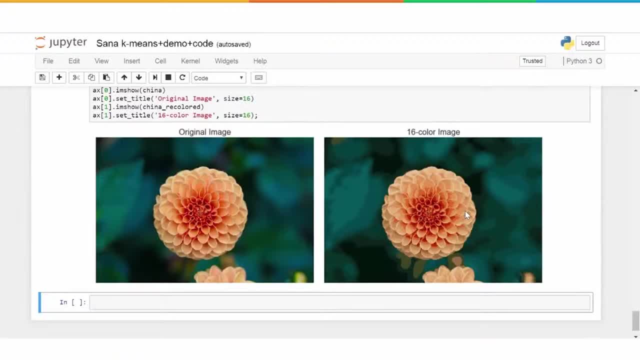 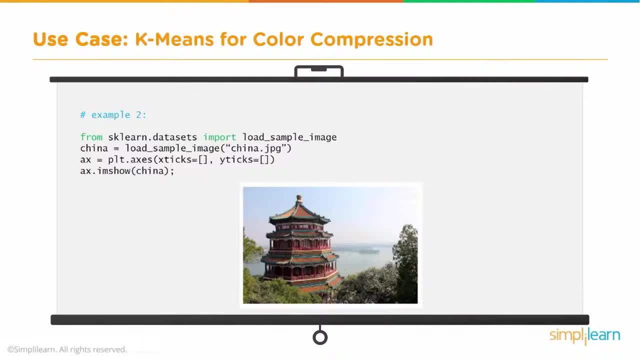 which can be rendered on a device which may not be that very sophisticated. now let's take one more example with a different image. in the second example we will take an image of the summer palace in china and we repeat the same process. this is a high definition. 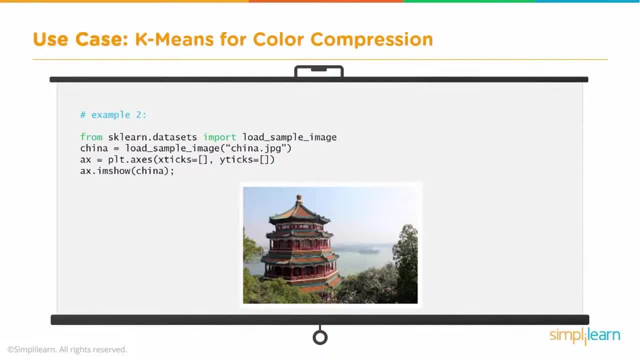 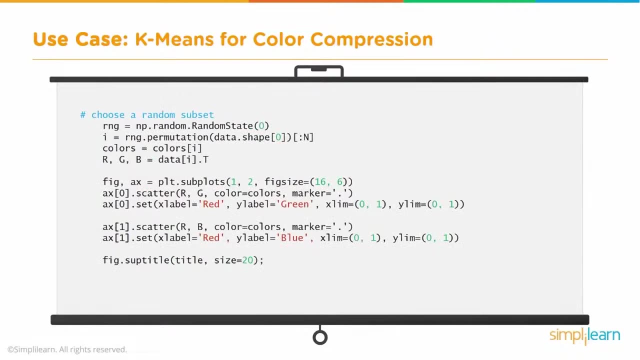 color image with millions of colors and also three-dimensional. now we will reduce that to 16 colors using k-means- clustering, and we do the same process like before. we reshape it and then we cluster the colors to 16 and then we render the image once again and we will see. 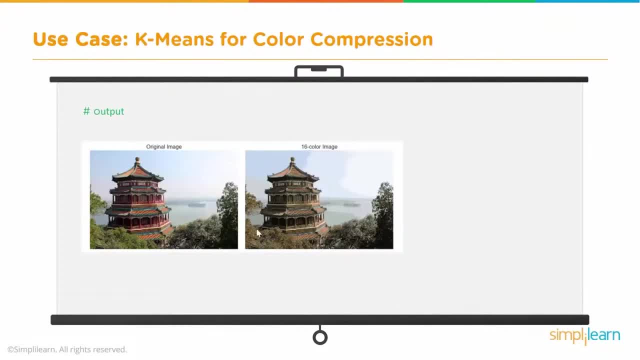 that the color, the quality of the image slightly deteriorates, as you can see here. this has much finer details in this which are probably missing here, but then that's the compromise, because there are some devices which may not be able to handle this kind of high density images. so 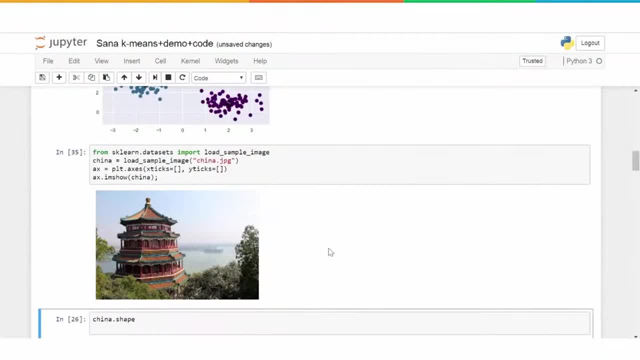 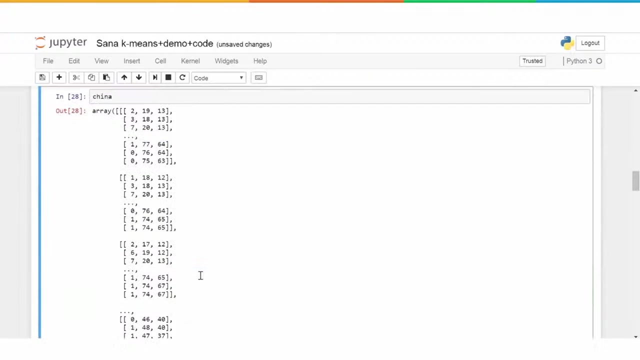 let's run this code in python notebook, all right. so let's apply the same technique for another picture which is even more intricate and has probably much complicated color schema. so this is the image. now, once again, we can take a look at the shape, which is 427 by 640 by. 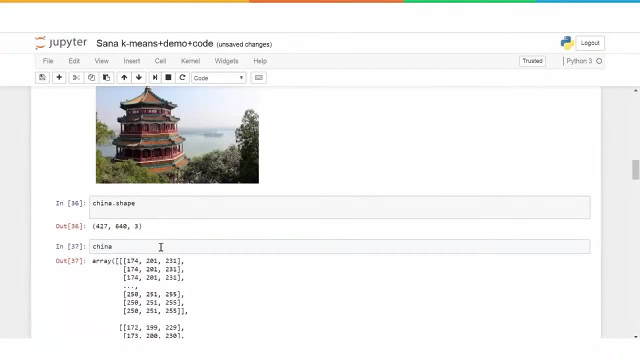 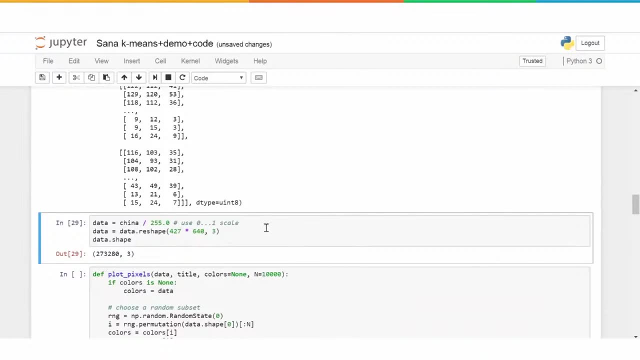 3, and this is the new data- would look somewhat like this compared to the flower image. so we have some new values here and we will also bring this. as you can see, the numbers are much big, so we will much bigger, so we will now have to. 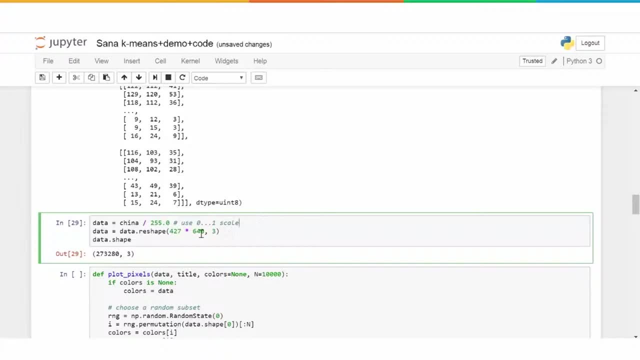 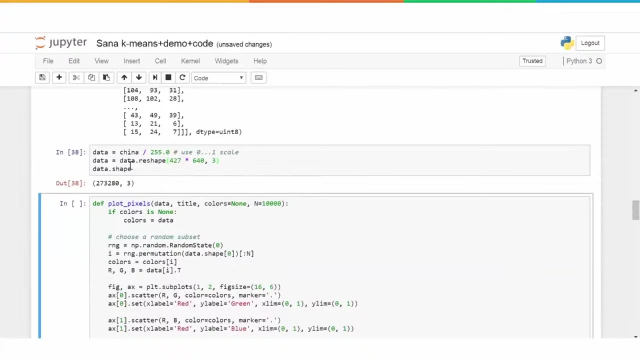 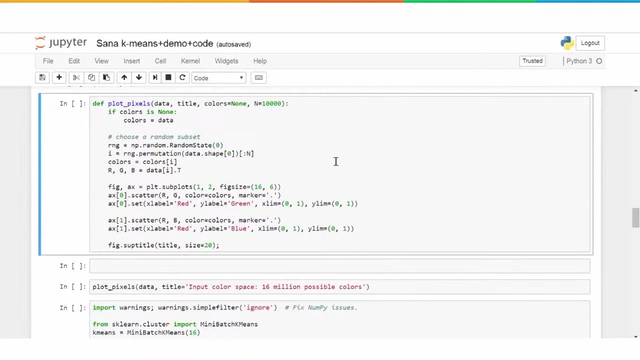 scale them down to values between 0 and 1, and that is done by dividing by 255. so let's go ahead and do that and reshape it. okay, so we get a two dimensional matrix and we will then, as a next step, we will go ahead and visualize this how it. 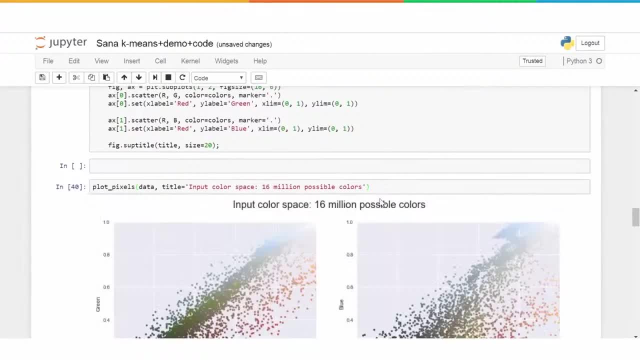 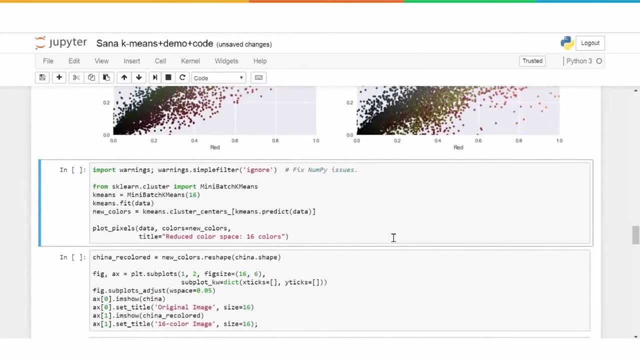 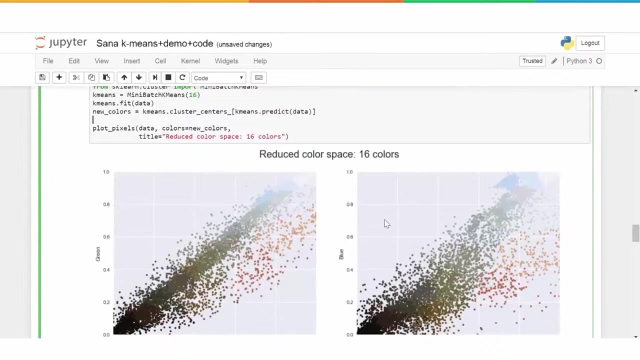 looks: the 16 colors and this is basically how it would look: 16 million colors. and now we can create the clusters out of this, the 16 k-means clusters we will create. so this is how the distribution of the pixels would look with 16 colors and 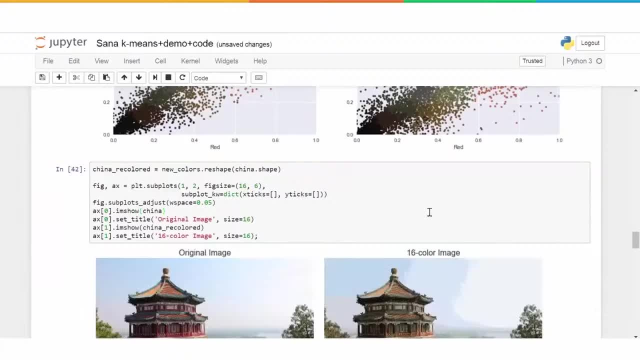 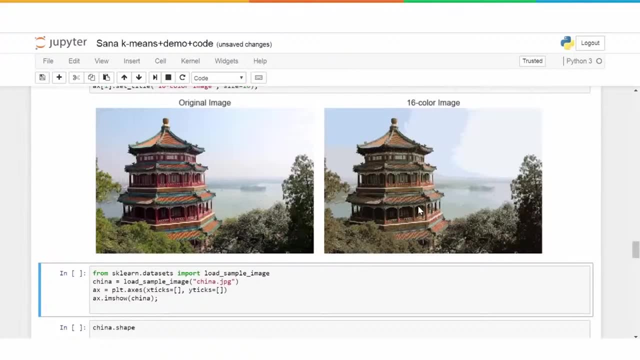 then we go ahead and apply this and visualize how it is looking for with the new, just the 16 colors. so, once again, as you can see, this looks much richer in color but at the same time- and this probably doesn't have, as we can see it- 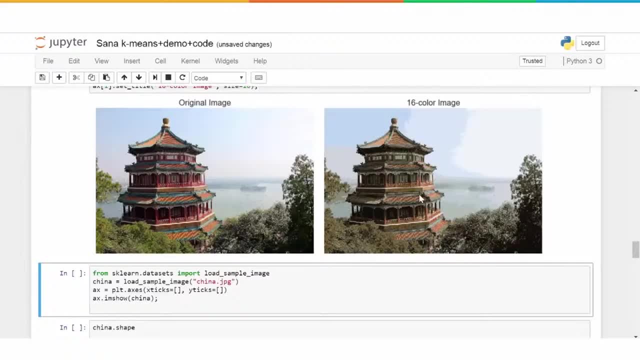 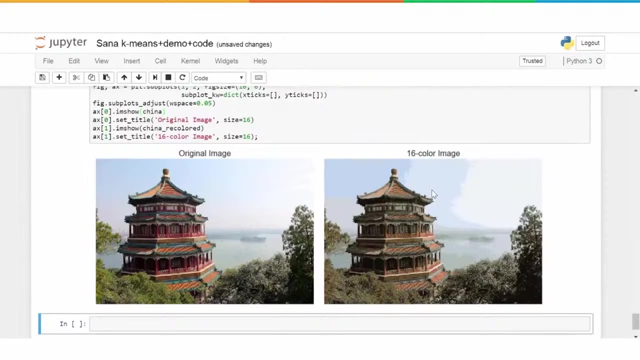 doesn't look as rich as this one, but nevertheless the information is not lost: the shape and all that stuff, and this can be also rendered on a slightly a device which is probably not that sophisticated. okay, so that's pretty much it. so we have seen two examples. 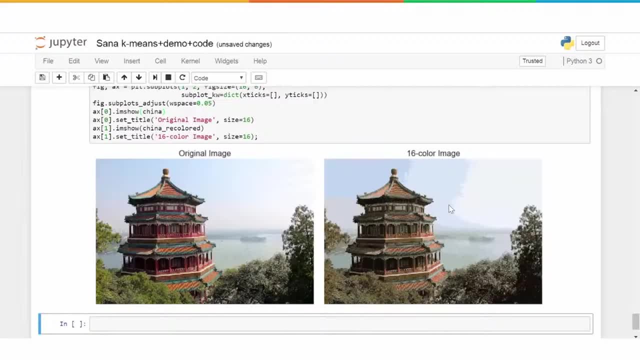 of how color compression can be done using k-means clustering and we have also seen in the previous examples of how to implement k-means the code to roughly how to implement k-means clustering, and we use some sample data using blog to just execute the k-means clustering. we talk. 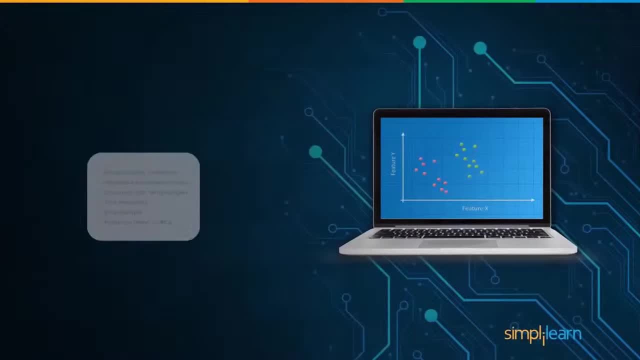 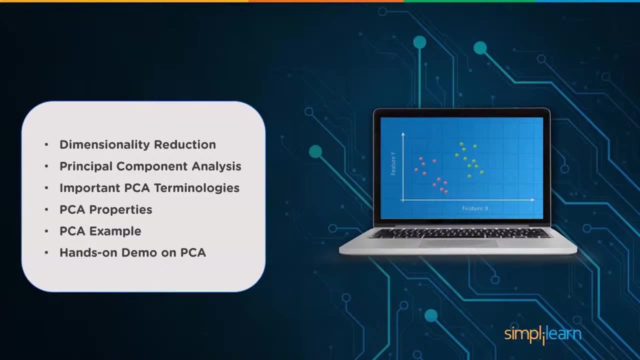 about the principal component analysis. we're going to cover dimensionality reduction. principal component analysis. what is it important? pca terminologies- and you'll see it abbreviated normally as pca- principal component analysis, pca properties, pca example, and then we'll pull up some python code in our jupyter notebook and have some hands. 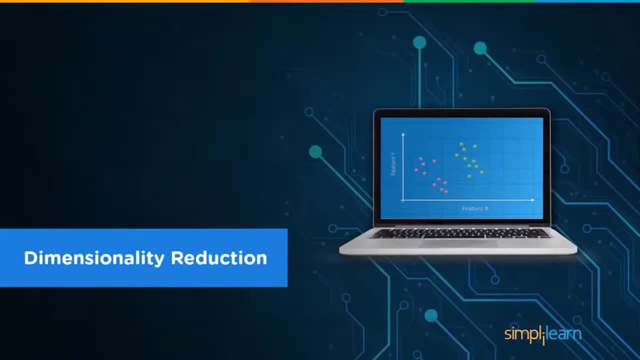 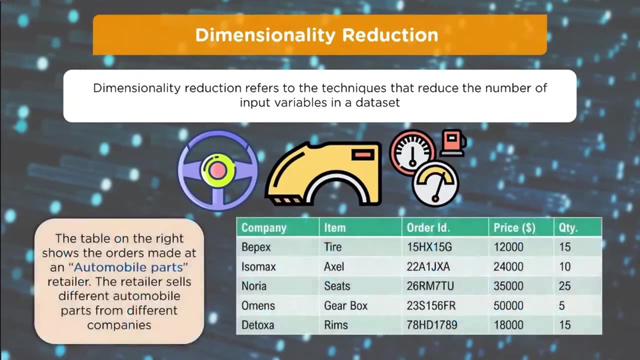 on demo on the pca and how it's used. dimensionality reduction: dimensionality reduction refers to the technique that reduces the number of input variables in a data set, and so you can see on the table on the right shows the orders made at an automobile parts retailer. 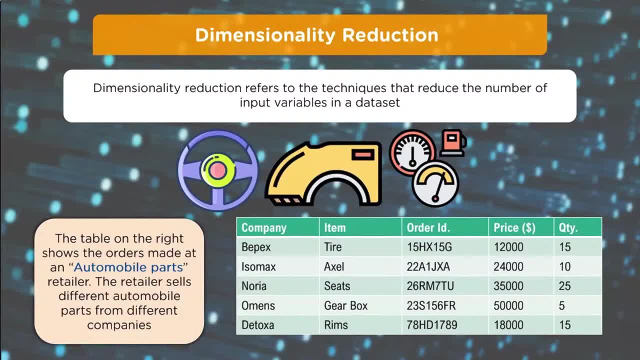 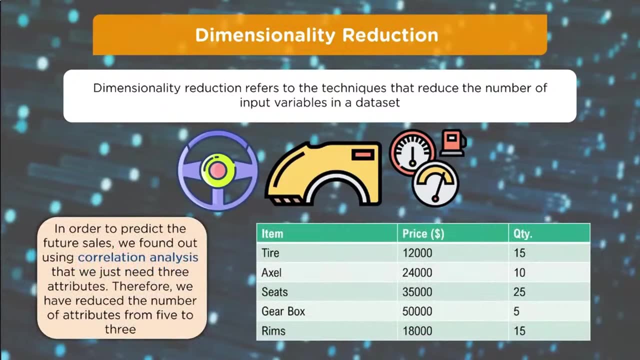 the retailer sells different automobile parts from different companies and you can see we have company bpacs, isomacs, and they have the item, the tire, the axle, an order id, a price number and a quantity in order to predict the future sales. we find out that using correlation analysis 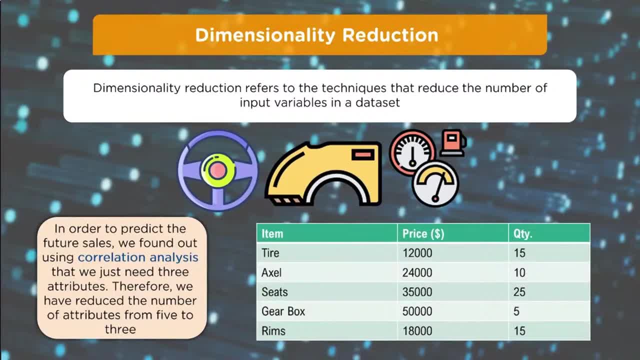 that we just need three attributes. therefore, we have reduced the number of attributes from five to three, and clearly we don't really care about the part number. i don't think the part number would have an effect on how many tires are bought, and even the store who's buying them probably does not. 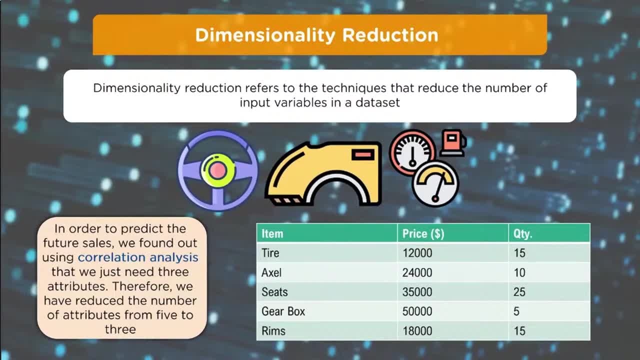 have an effect on that. in this case, that's what they've actually done is remove those, and we just have the item, the tire, the price and the quantity. one of the things you should be taking away from this is: in the scheme of things, we are in the 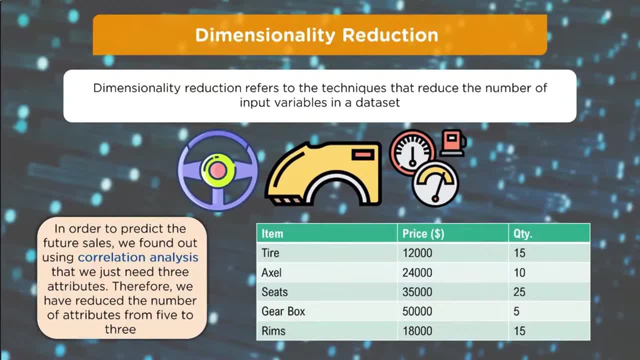 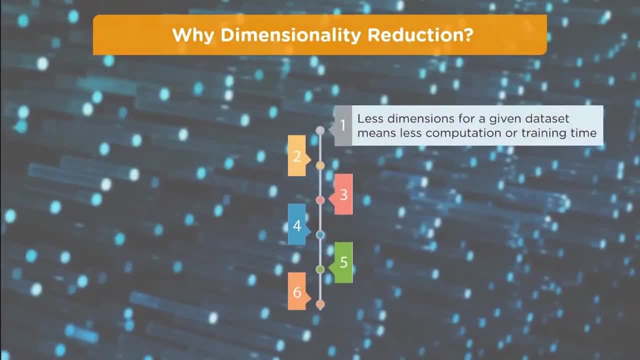 descriptive phase. we're describing the data and we're preprocessing the data. what can we do to clean it up? why dimensionality reduction? well, number one: less dimensions for a given data set means less computation or training time. that can be really important if you're trying a number of different models. 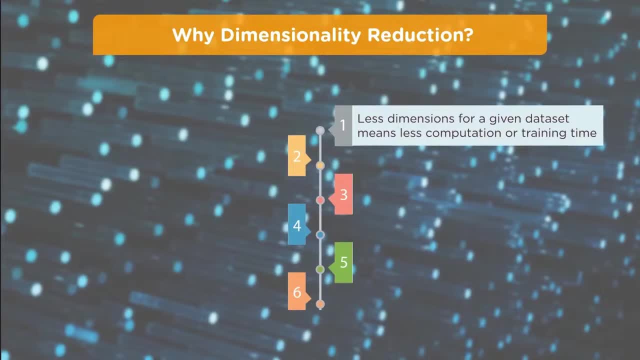 and you're rerunning them over and over again, and even if you have seven gigabytes of data, that can start taking days to go through all those different models. so this is huge. this is probably the hugest part as far as reducing our data set redundancy is removed. 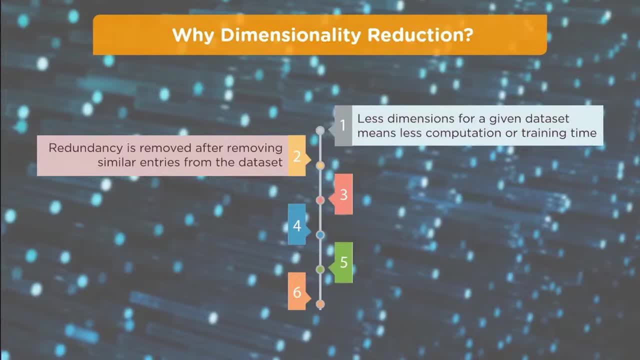 after removing similar entries from the data set, again preprocessing some of our models. like a neural network, if you put in two of the same data it might give them a higher weight than they would if it was just once. we want to get rid of that redundancy. it also increases the processing time. 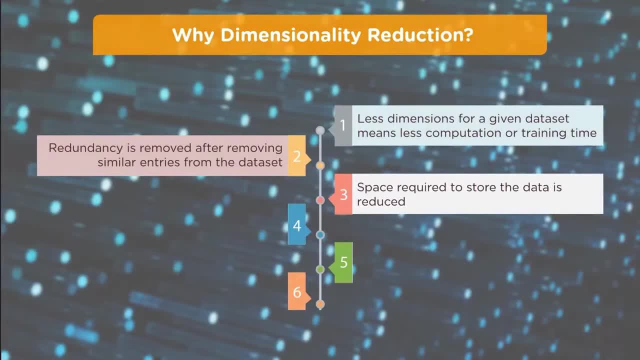 if you have multiple data coming in, space required to store the data is reduced. so if we're committing this into a big data pool, we might not send the company that bought it. why would we want to store two whole extra columns when we add it into that pool of data? 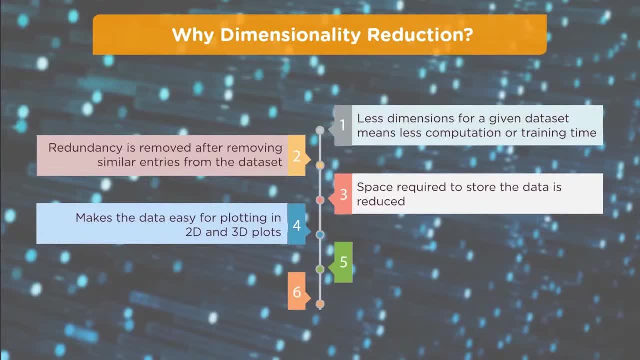 makes the data easy for plotting in 2D and 3D plots. this is my favorite part, very important. you're in your shareholder meeting. you want to be able to give them a really good, clear and simplified version. you want to reduce it down to something people can take in. 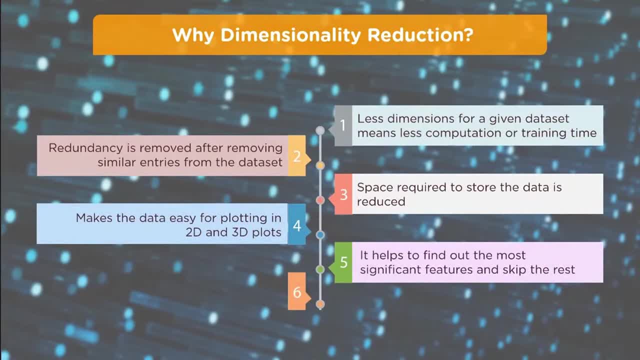 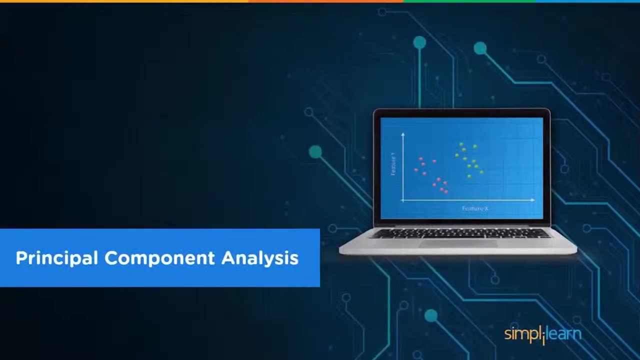 it helps to find out the most significant features and skip the rest, which also comes in in post scribing leads to better human interpretation. that kind of goes with number four. what makes data easy for plotting? you have a better interpretation when we're looking at it. principal component analysis. 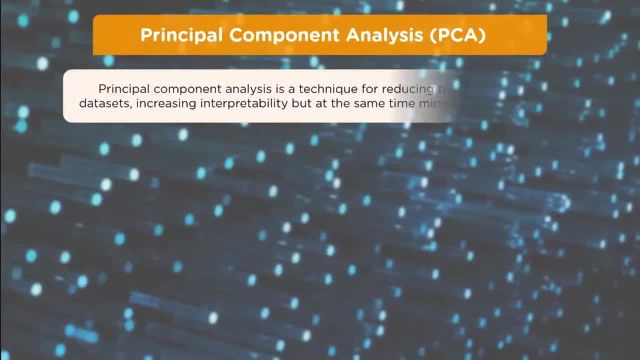 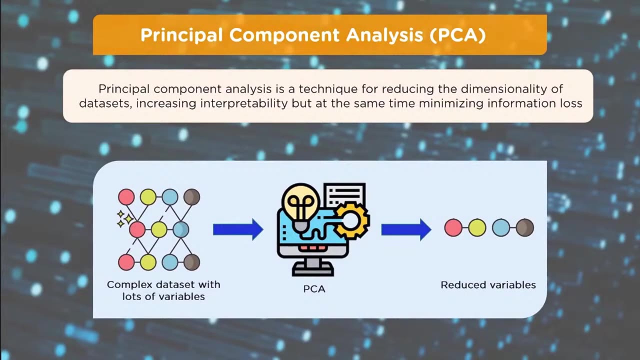 so what is it? principal component analysis is a technique for reducing the dimensionality of data sets, increasing credibility but at the same time minimizing information loss. so we take some very complex data set with lots of variables, we run it through the PCA, we reduce the variables, we end up with a reduced variable set up. 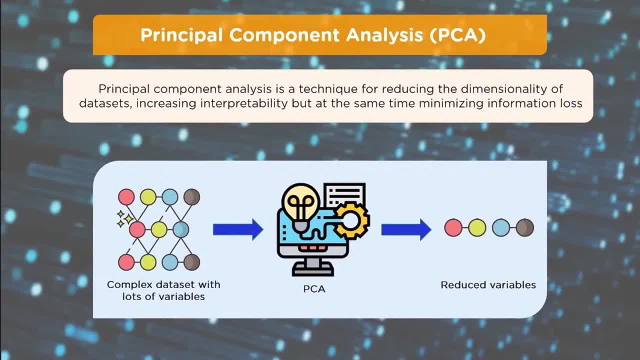 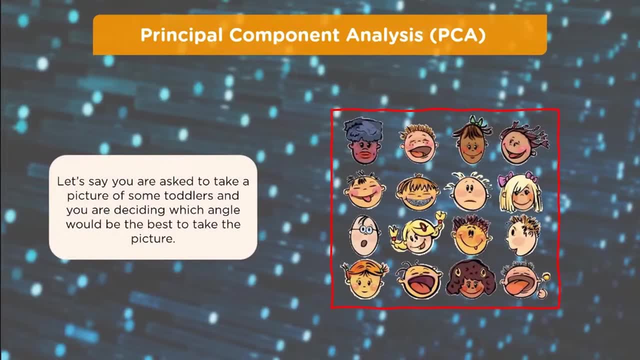 this is very confusing to look at because if you look at the end result, we have the different colors all lined up. so what we're going to take a look at is: let's say, we have a picture here. let's say, you are asked to take a picture. 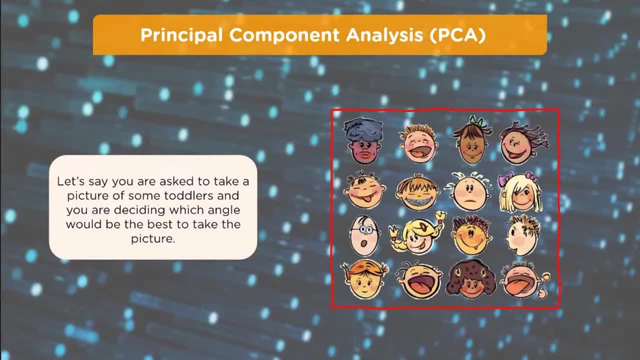 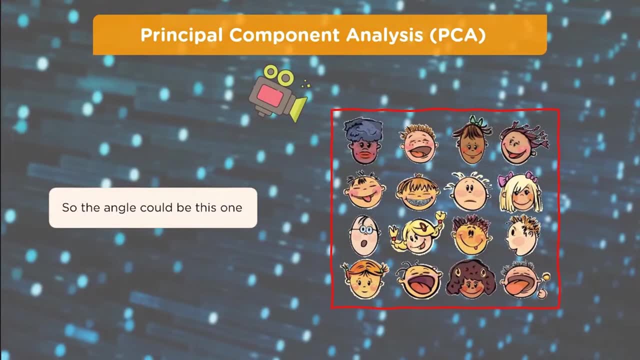 of some toddlers and you are deciding which angle would be the best to take the picture from. so if we come up here and we look at this, we say, okay, this is one angle, we get the back of a lot of heads, not many faces, so we'll do it from here. 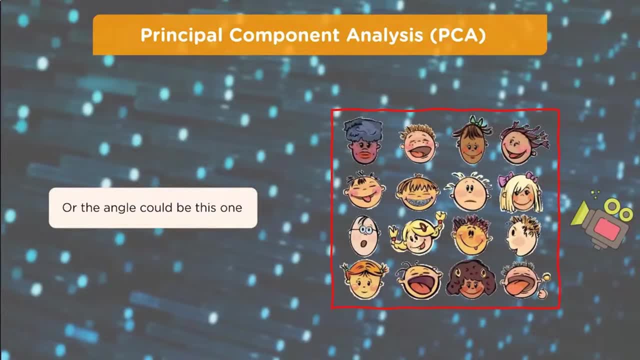 we might get the one person up front smiling. a lot of the people in the class are missing, so we have a huge amount off to the right of blank space, maybe from up. here again we have the back of someone's head and it turns out that the best angle 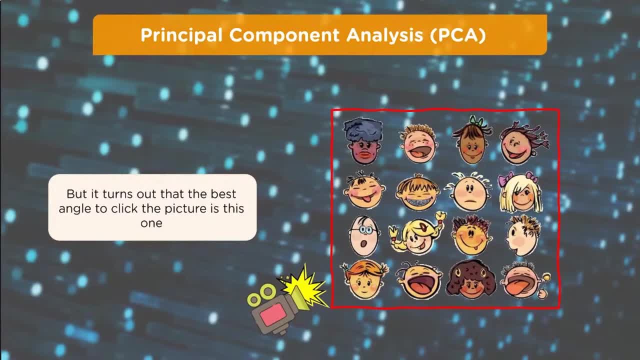 to click the picture from might be this bottom left angle. that makes sense. it's a good configuration of all the people in the picture. now, when we're talking about data, it's not. you really can't do it by what you think is going to be the best. 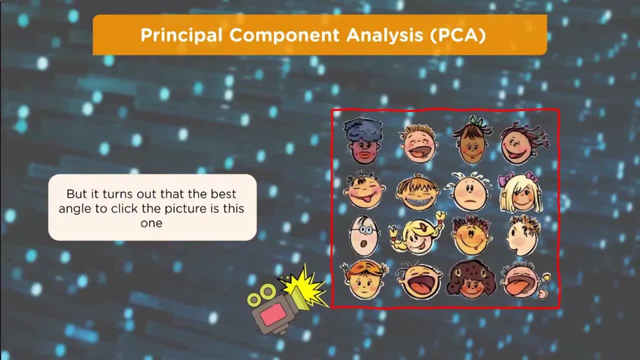 we need to have some kind of mathematical formula so it's consistent, so it makes sense. in the back end. one of the projects I worked on many years ago has something similar to the iris. if you've ever done the iris data set, it's probably one of the most common ones. 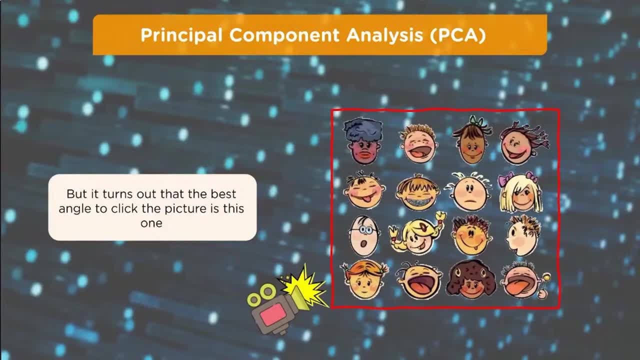 out there where they have the flower and they're measuring the stamen and the petals, and they have width and they have length of the petal. instead of putting through the width and the length of the petal, we could just as easily do the width to. 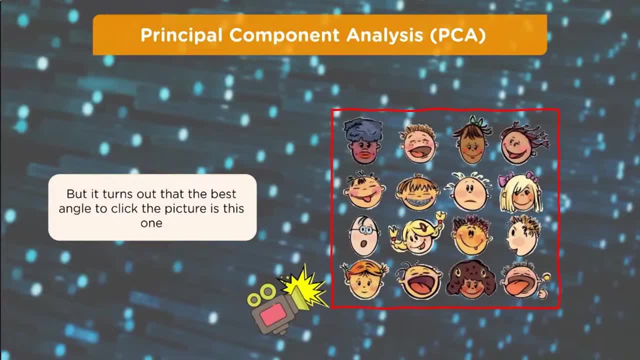 length ratio. we can divide the width by the length and you get a single number where you had two. that's the kind of idea that's going on into this in pre-processing and looking at what we can do to bring the data down. a very simplified example on my 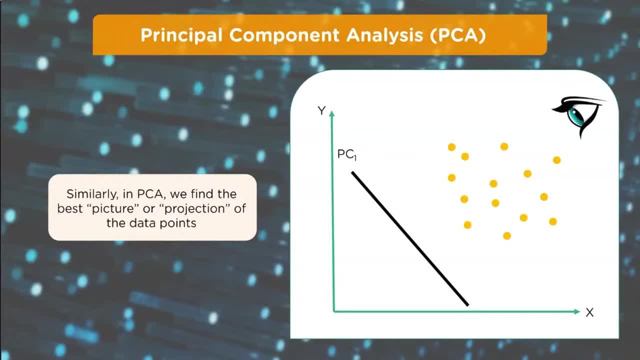 iris petal example. when we look at the similarity in PCA, we find the best picture or projection of the data points, and so we look down from one angle- we've drawn a line down there. we can see these data points based on- in this case, just two. 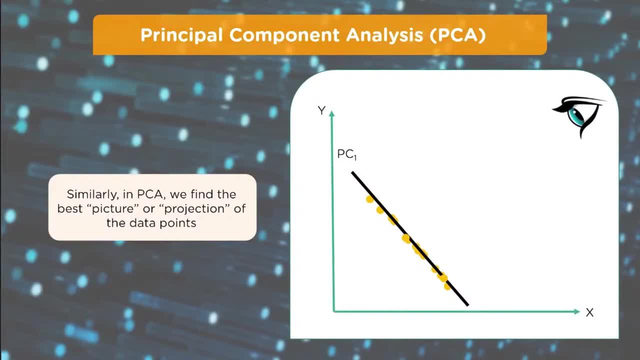 variables. now, keep in mind we're usually talking about 36- 40 variables. almost all of your business models usually have about 26 to 27 different variables. they're looking at same thing with, like, a bank loan model. we're talking 26 to 36 different. 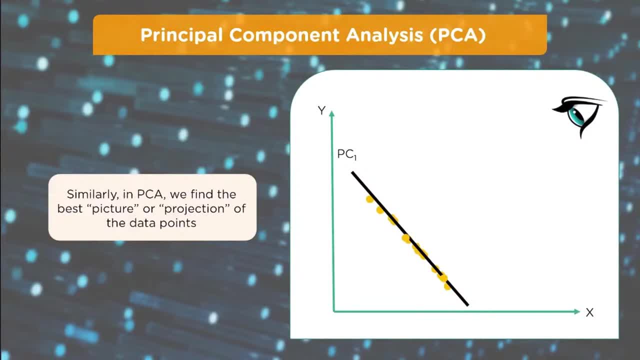 variables they're looking at that are going in. so what we want to do is we want to find the best view. in this case, we're just looking at the XY, we look down at it and we have our second idea, PC2, and again we're looking at 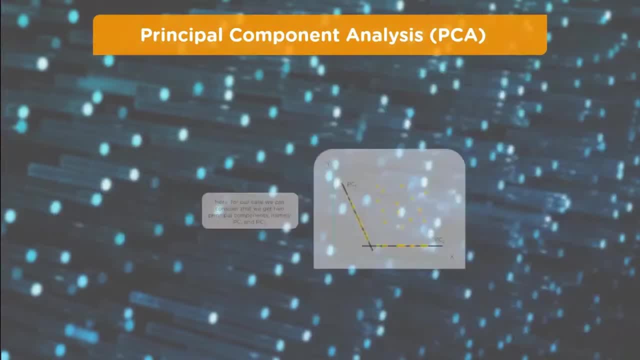 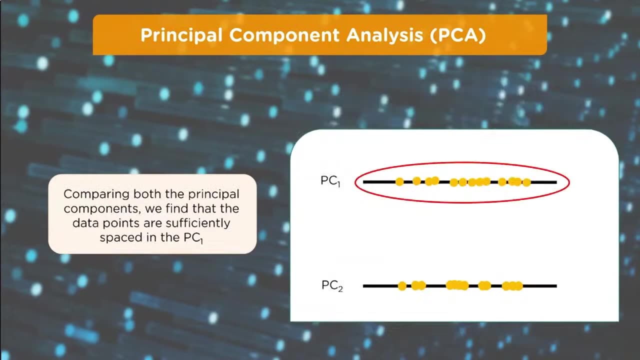 the XY, this time from a different direction. here for our E's, we can consider that we get two principal components, namely PC1 and PC2. comparing both the principal components, we find the data points are sufficiently spaced in PC1. so if you look at what we 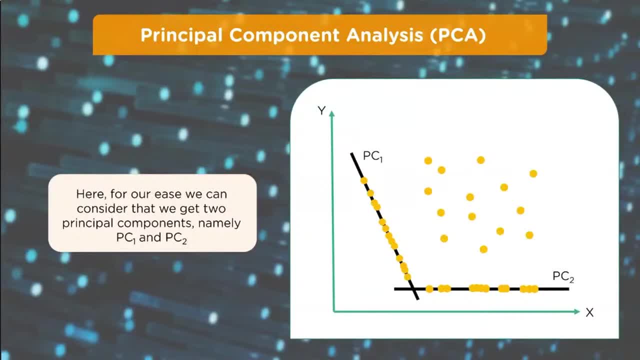 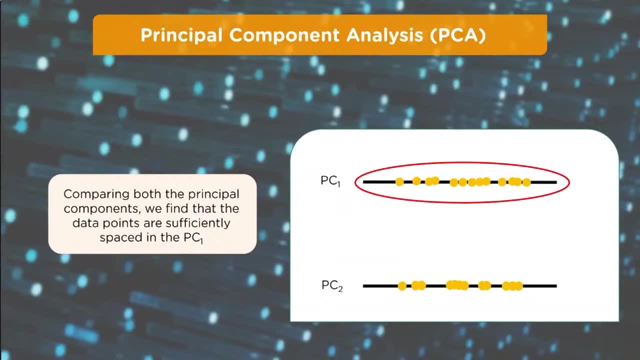 got here. we have PC1. you can see along the line how the data points are spaced versus the spacing in PC2 and that's what they're coming up with. what is going to give us the best look for these data points when we combine them and we're looking at them from just a single angle. 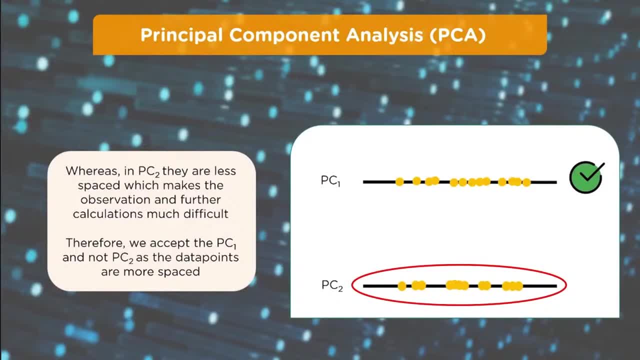 whereas in PC2 they are less spaced, which makes the observation and further calculations much more difficult. therefore we accept the PC1 and not the PC2, as the data points are more spaced now. obviously the back end calculations are a little bit more complicated when we get into the math of how they 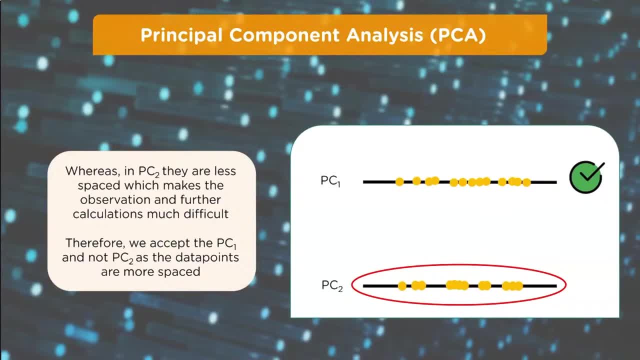 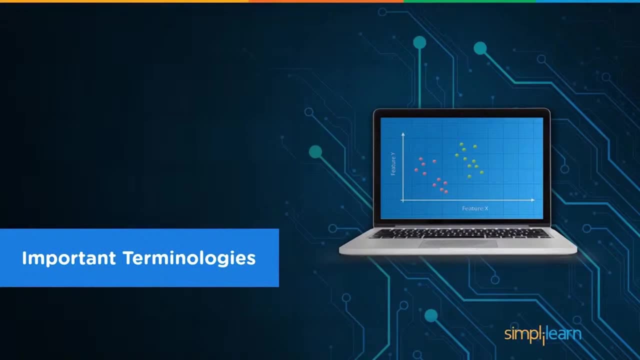 decide what is more valuable. this gives you an idea, though, that when we're talking about this, we're talking about the perspective, which would help in understanding how PCA analysis works. what we want to go ahead and do is dive into the important terminologies under PCA, and important terminologies are views. 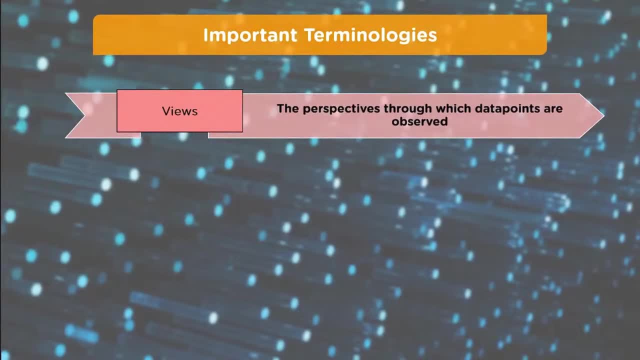 the perspective through which data points are observed, and so you'll hear that if someone's talking about a PCA presentation and they're not taking the time to reduce it to something that the average person shareholders can understand, you might hear them refer to it as the different views. what view are we taking? 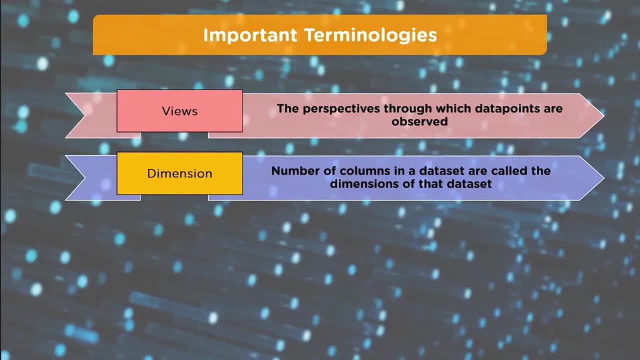 dimension, number of columns in a data set are called the dimensions of that data set we talked about. you'll hear features dimensions. I was talking about features. there's usually, when you're running a business, you're talking 25, 26, 27 different features, minimal- and then you have the principal component. 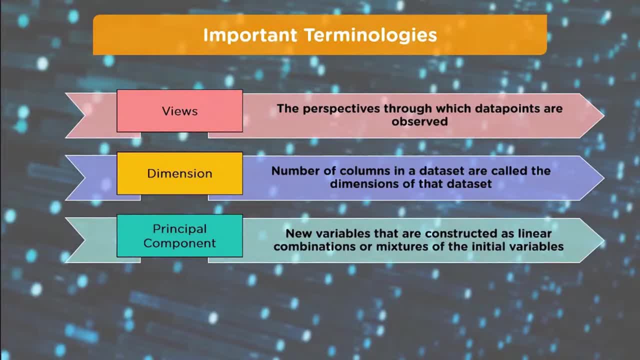 new variables that are constructed as linear combinations or mixtures of the initial variables. principal component is very important. it's a combination. if you remember my flower example, it would be the width over the length of the petal, as opposed to putting both width and length in. 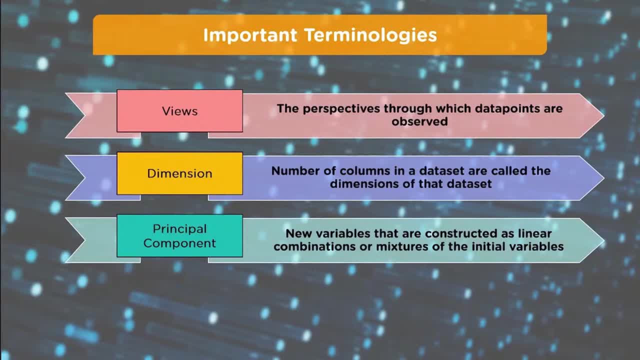 you just put in the ratio instead, which is a single number versus two separate numbers, projections, the perpendicular distance between the principal component and the data points and that goes to that line we had earlier. it's that right angle line of where all those points fall onto the line important properties. 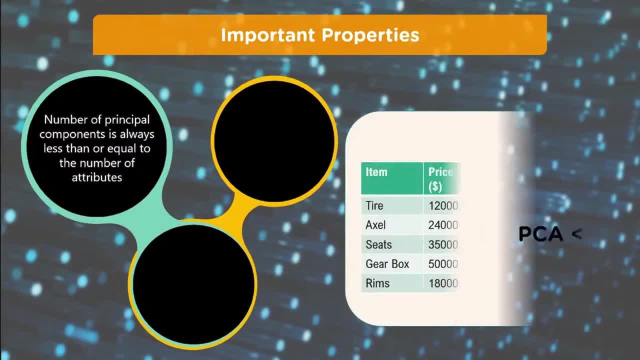 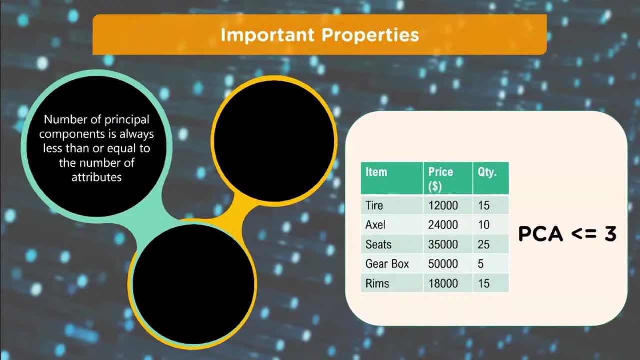 important properties. number of principal components is always less than or equal to the number of attributes. that just makes common sense. you're not going to do ten principal properties with only three features. you're trying to reduce them. so it's just kind of goofy, but it is. 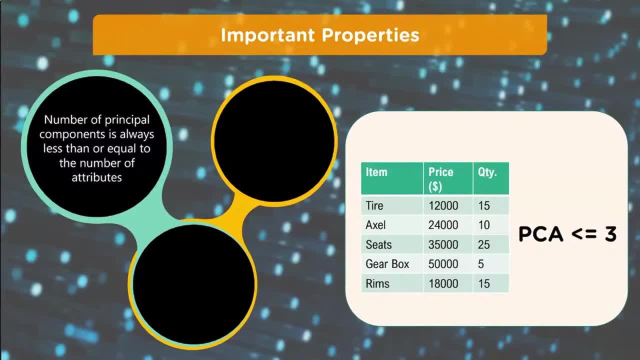 important to remember that people will throw weird code out there and just randomly do stuff instead of really thinking it through. principal components are orthogonal and this is what we're talking about- that right angle from the line. when we do PC1, we're looking at how those points fall onto. 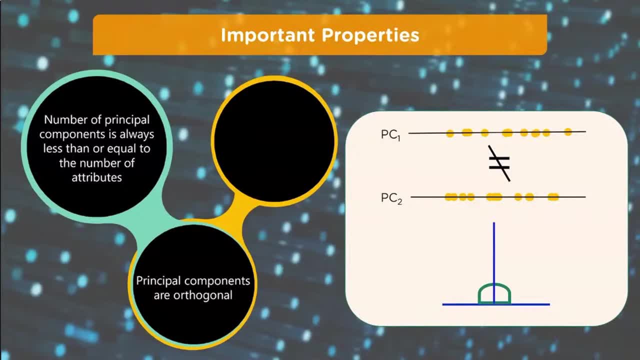 that line. same thing with PC2. we want to make sure that PC1 does not equal PC2. we don't want to have the two principal points. when we do two points, the priority of principal components decreases as their numbers increase. this is important to understand if you're going to create. 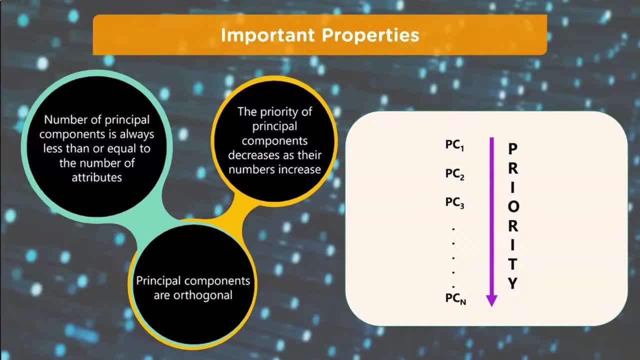 one principal component. everything is summarized into that one component. as we go to two components, the priority, how much it holds the value decreases as we go down. so if you have five different points, each one of those points is going to have less value than just the one point. 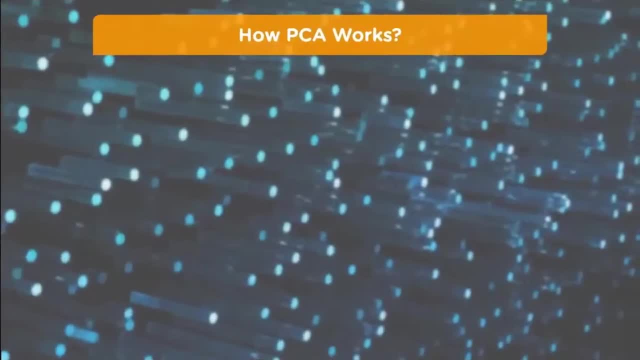 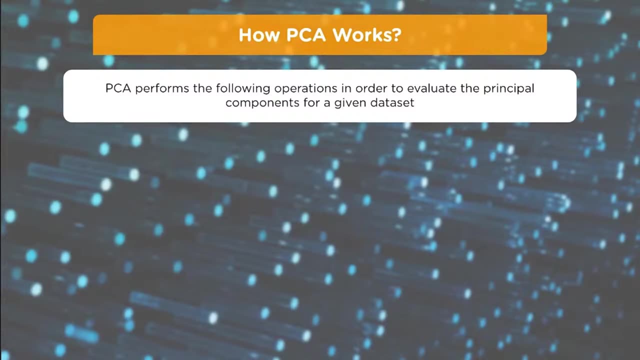 which has everything summarized in it: how PCA works. I said there was more in the back end. we talk about the math. this is what we're talking about is: how does it actually work? so now we have an understanding. you're looking at a perspective. now we want to see how that math side works. 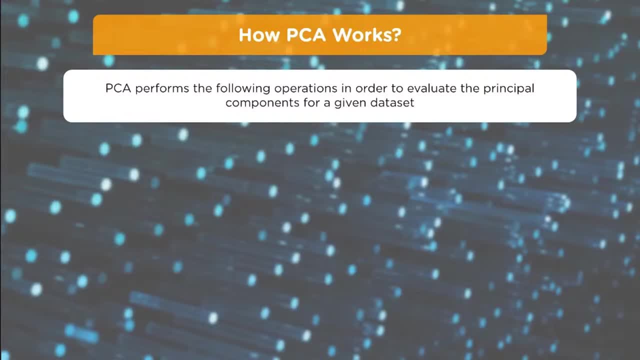 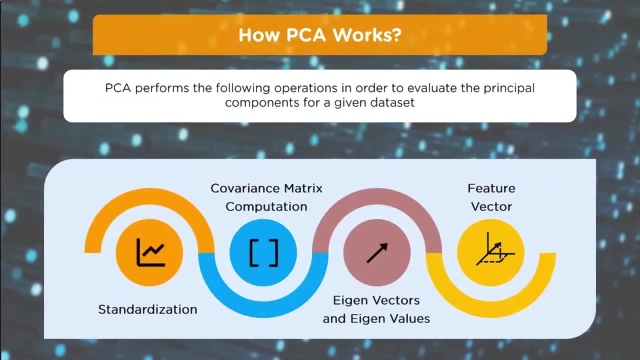 PCA performs the following operations in order to evaluate the principal components for a given data set. first we start with the standardization, then we have a covariance matrix computation and we use that to generate our eigenvectors and eigenvalues, which is the feature vector and, if you remember, the eigenvector. 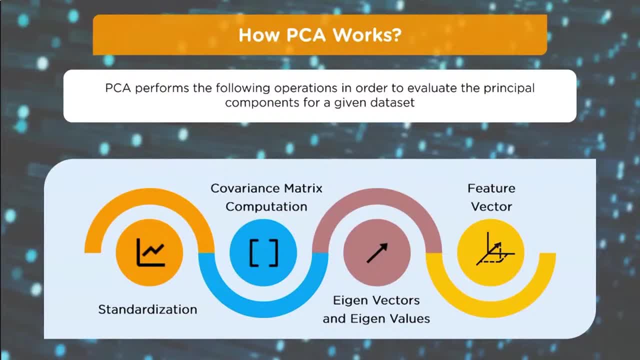 is like a translation. if we're moving the data from x equals one to x equals two or whatever, altering, it is the final value that we generate. when we talk about standardization, the main aim of this step is to standardize the range of the attributes. 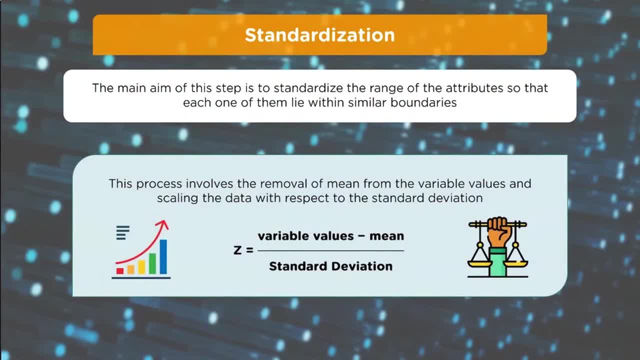 so that each one of them lie within similar boundaries. this process involves removal of the mean from the variable values and scaling the data with respect to the standard deviation, and you can see here we have: z equals the variable values minus the mean over the standard deviation. the covariance matrix. 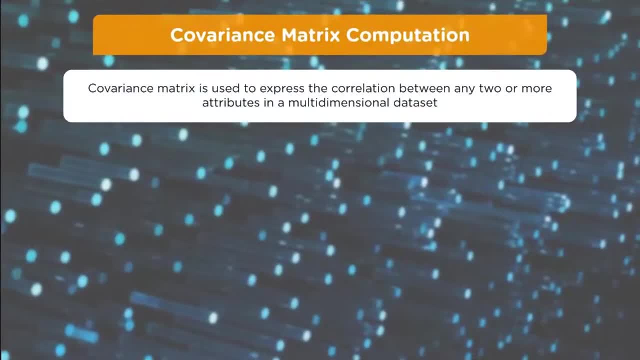 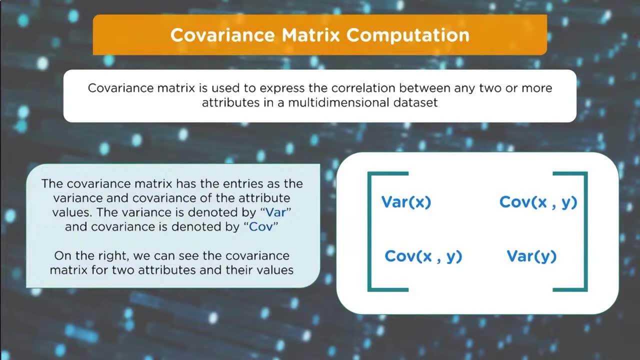 computation covariance matrix is used to express the correlation between any two or more attributes in multidimensional data set. the covariance matrix has the entries as the variance and the covariance of the attribute values. the variance is denoted by var and the covariance is denoted by co. 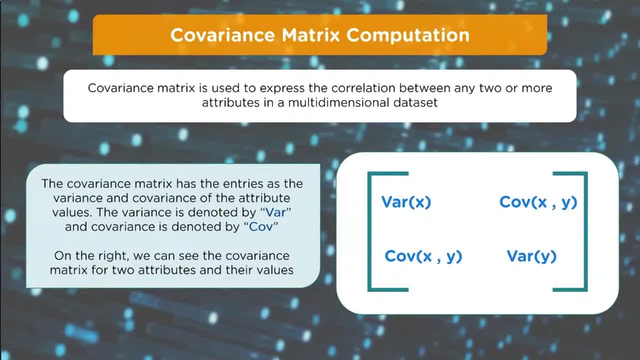 on the right we can see the covariance matrix for two attributes and their values. when we do a hands-on look at the code, we'll do a display of this so you can see what we're talking about and what that looks like. for now, you can just notice that this is a matrix. 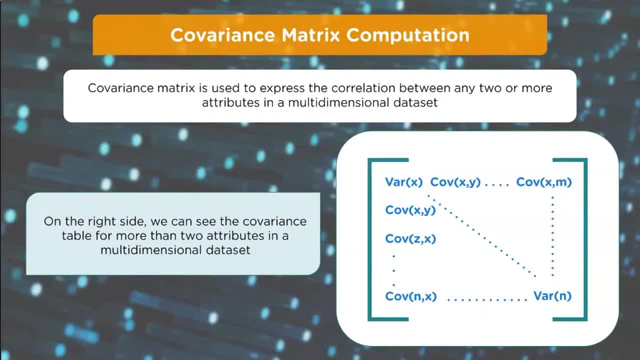 that we're generating with the variance and then the covariance of x to y. on the right side we can see the covariance table for more than two attributes in a multidimensional data set. this is what I was talking about. we usually are looking at not just one feature or two features. 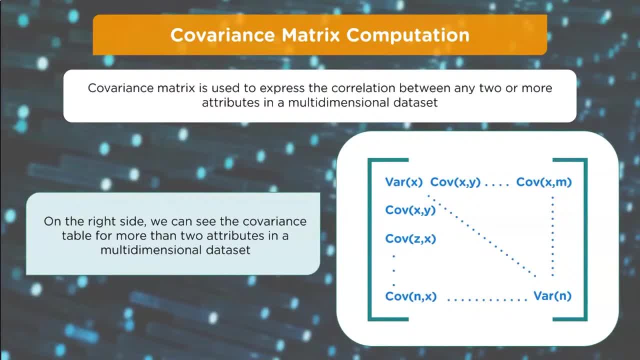 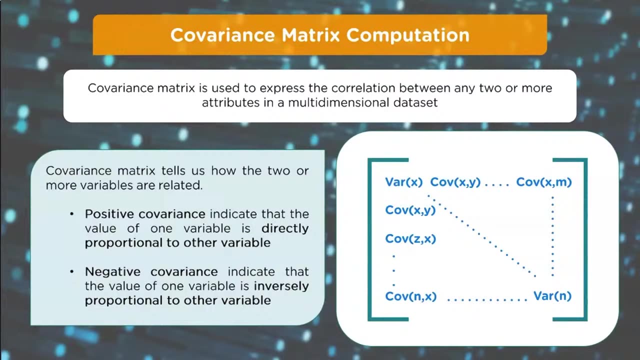 we're usually looking at 25, 30 features going on, and so if we do a setup like this, we should see all those different features as the different variables covariance matrix tells us how the two or more variables are related. positive covariance indicate that the value of one variable is directly. 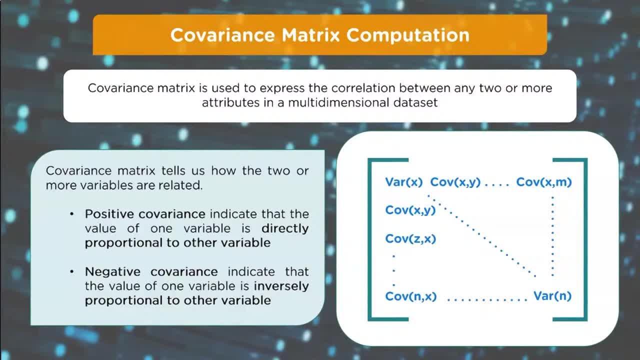 proportional to the other variable. negative covariance indicate that the value of one variable is inversely proportional to the other variable. that is always important to note whenever we're doing any of these matrices that we're going to be looking at that positive and negative, whether it's inverted or not. 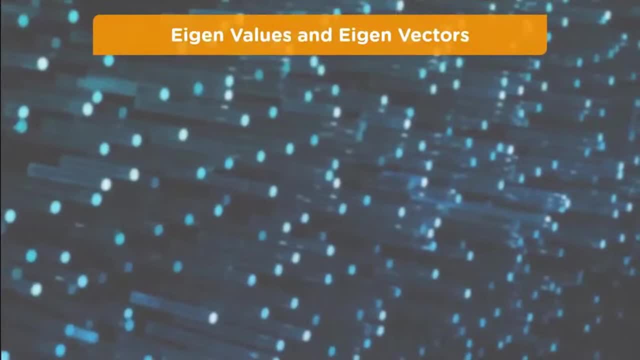 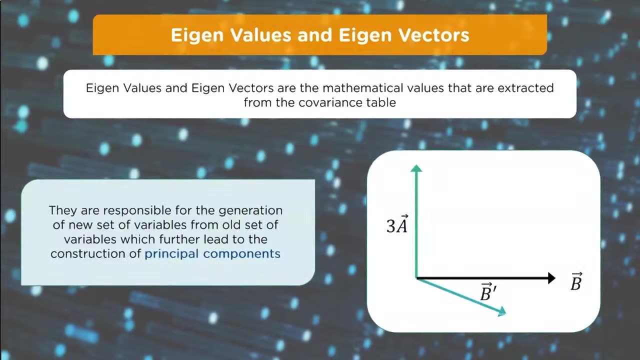 and then we have the eigenvalues and the eigenvectors. eigenvalues and eigenvectors are the mathematical value that are extracted from the covariance table. they are responsible for the generation of a new set of variables from the old set of variables, which further lead to the construction. 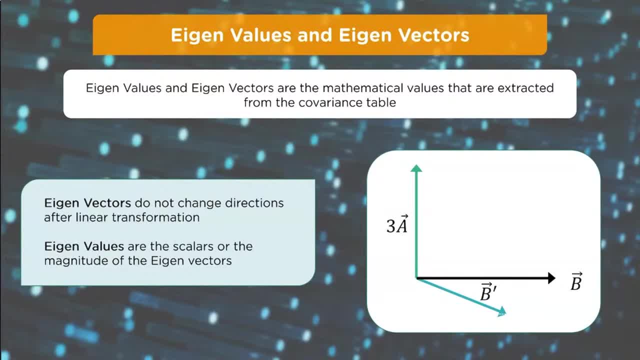 of the principal components. eigenvectors do not change directions after linear transformation. eigenvalues are the scalars or the magnitude of the eigenvectors, and again this is just transforming that data. so we're going to change the vector b to the b prime as denoted on the chart. 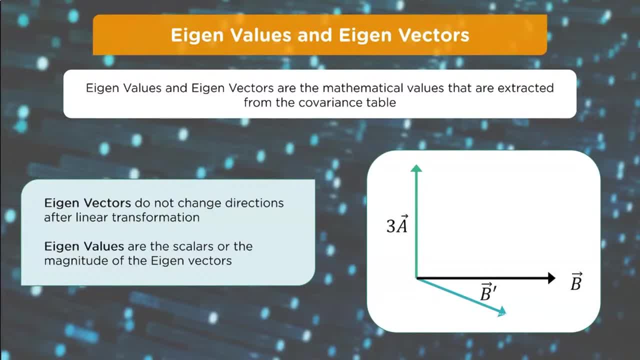 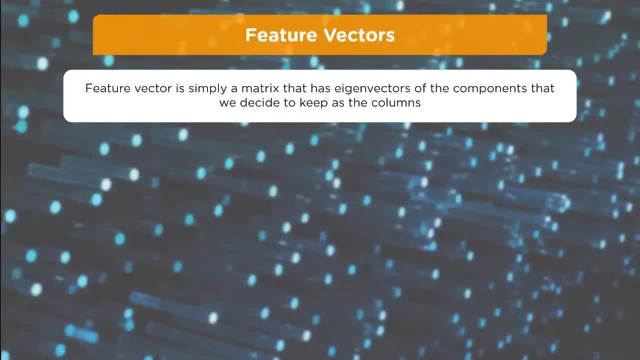 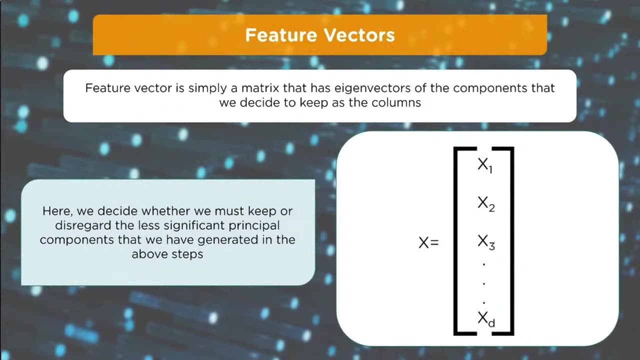 and so we have like multiple variables. how do we calculate that new variable? and then we have feature vectors. feature vectors is simply a matrix that has eigenvectors of the components that we decide to keep as the columns. here we decide whether we must keep or discard the less significant principal. 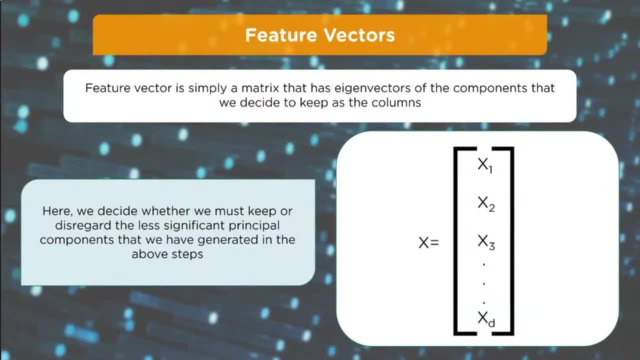 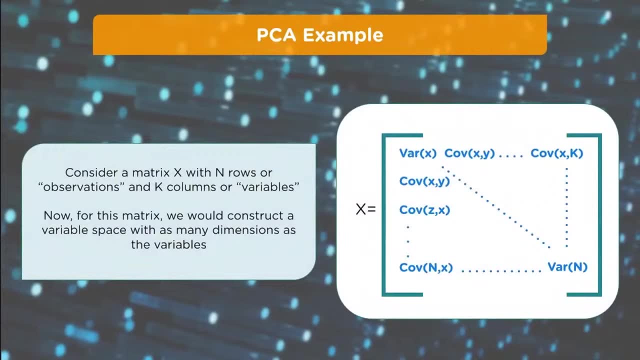 components that we have generated in the above steps. this becomes really important as we start looking at the back end of this, and we'll do this in the demo. but one of the more important steps to understand, and so we have the PCA example. consider matrix x with 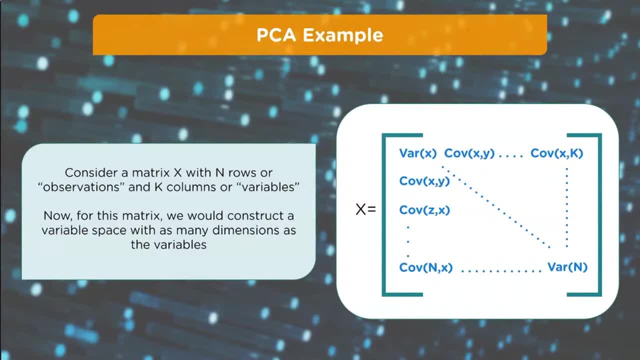 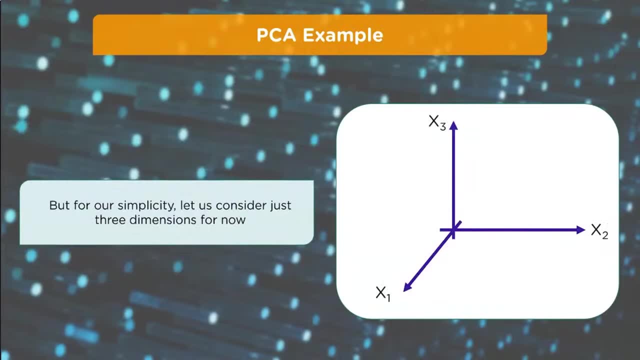 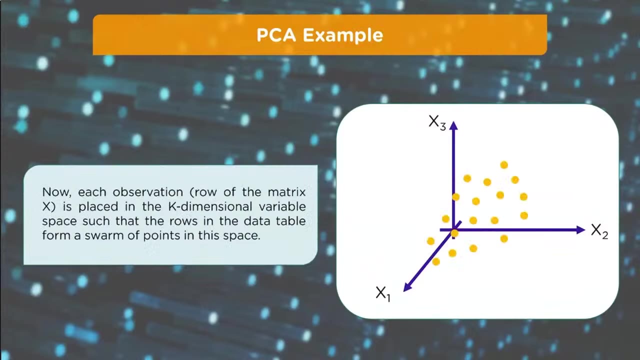 n rows or observations, and k columns or variables. now for this matrix. we would construct a variable space with as many dimensions as the variable, but for our simplicity let's consider this three dimensions for now. now, each observation row of the matrix x is placed in the k dimensional variable. 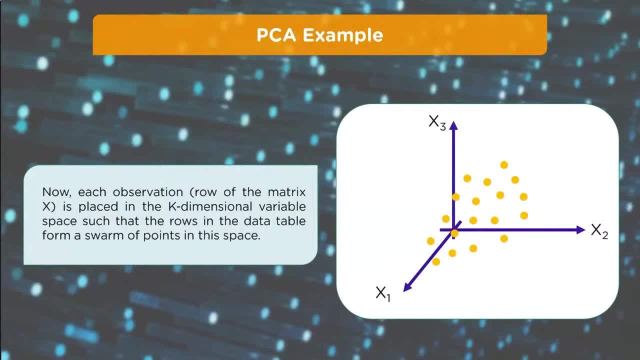 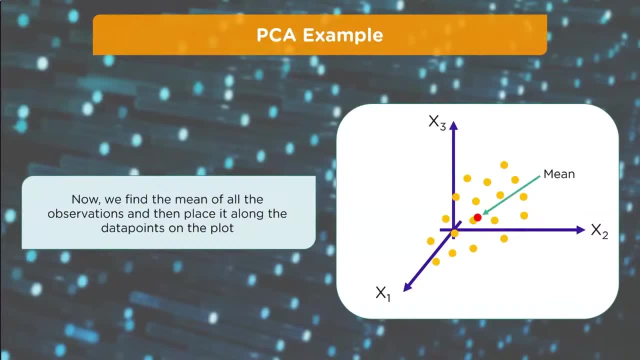 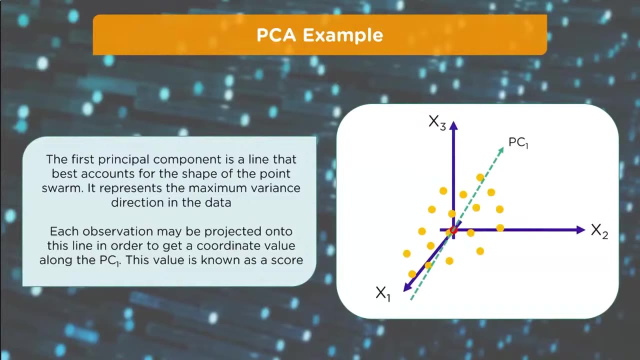 space such that the rows in the data table form a swarm of points in this space. now we find the mean of all the observations and then place it along the data points on the plot. the first principal component is a line that best accounts for the shape of the point swarm. 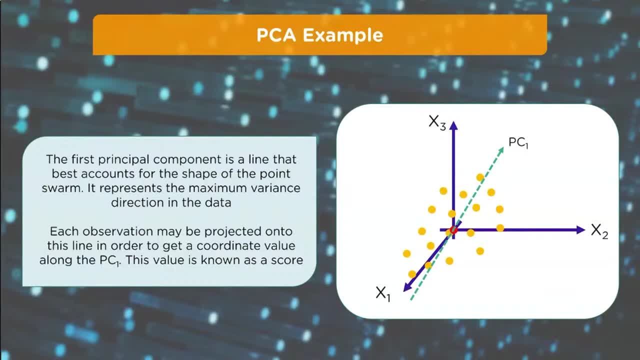 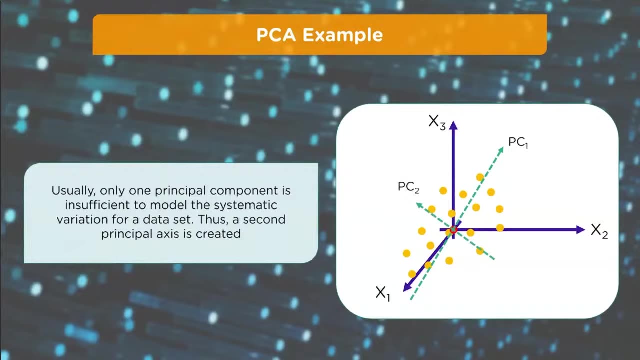 it represents the maximum variance direction in the data. each observation may be projected onto this line in order to get a coordinate value along the PC1. this value is known as a score. usually, only one principal component is insufficient to model the systematic variation for a data set. thus, 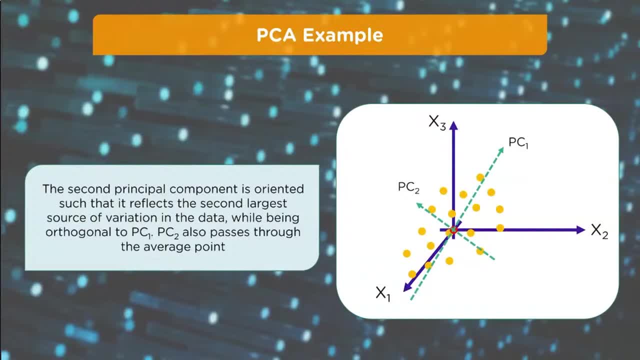 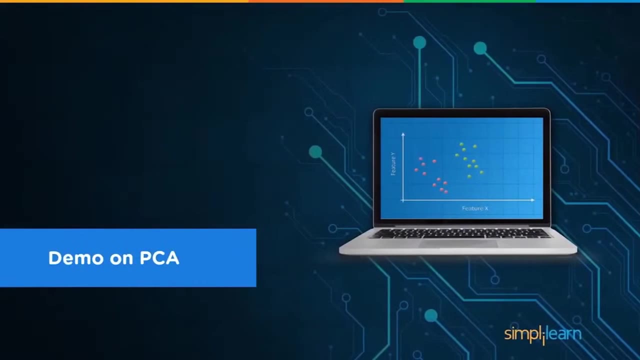 a second principal axis is created. the second principal component is oriented such that it reflects the second largest source of variation in the data, while being orthogonal to PC1. PC2 also passes through the average point. let's go ahead and pull this up and just see what that means. 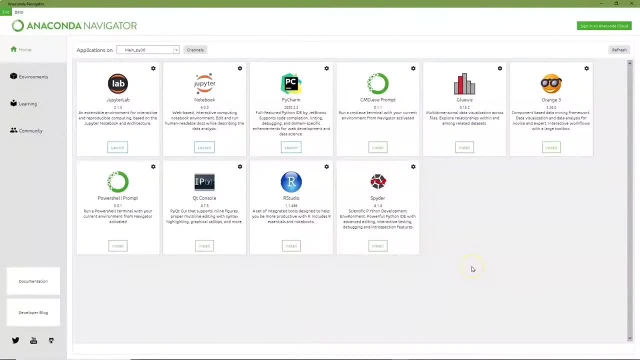 inside our python scripting. I'm going to use the anaconda navigator and I will be in python 3.6. for this example, I believe there is even like a 3.9 out. I tend to stay in 3.6 because a lot of the models I use. 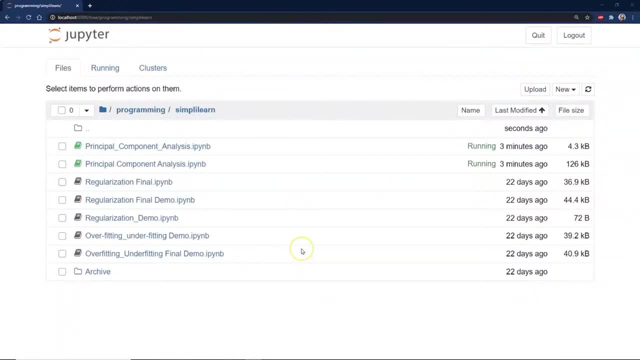 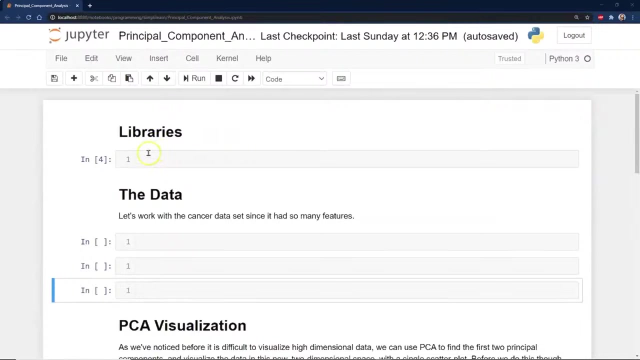 especially with the neural networks, are stable in 3.6. and then we open up our jupiter. I'm in chrome. go ahead and create a new python 3 and, for ease of use, our team in the back was nice enough to put this together for me and we'll go ahead. 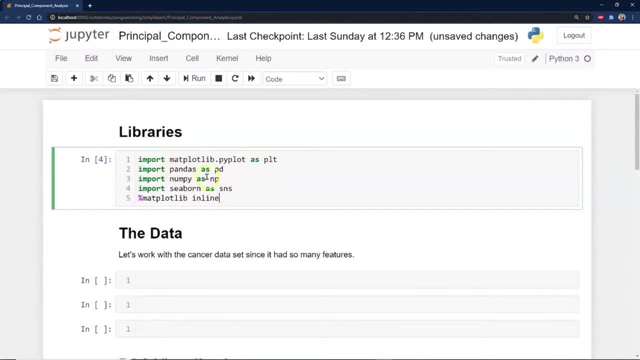 and start with the libraries, the first thing I like to do whenever I'm looking at any new setup. well, you know what? let's do the libraries first. we're going to do our basic libraries, which is matplotlib, the plt from the matplotlib pandas, our dataframe. pd numpy, our numbers array. 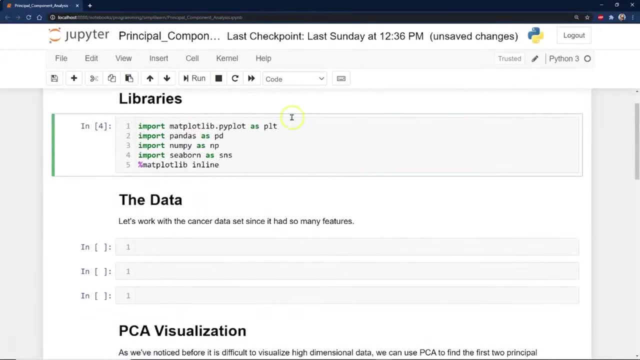 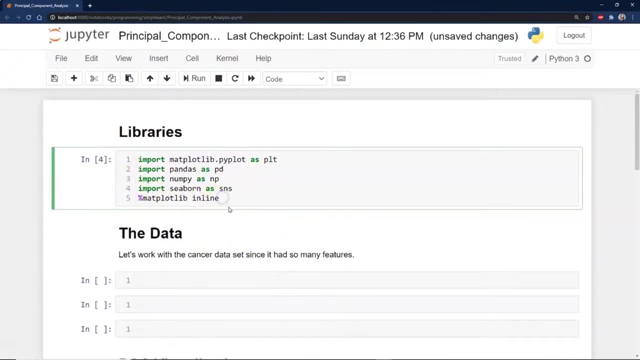 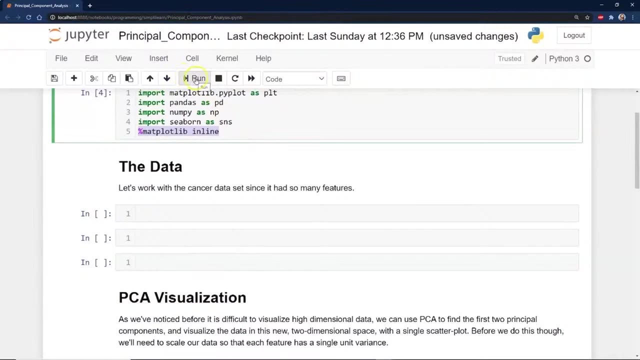 np seaborn for graphing sns. that goes with the plot that actually sits on matplotlib, so the seaborn sits on there and then we have our amber sign because we're in jupiter notebook matplotlib inline. the newer version actually doesn't require that, but I put it in there either. anyway. 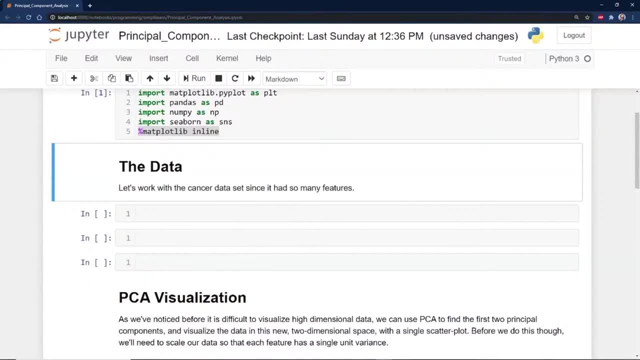 just because I'm so used to it, and then we want to go ahead and take a look at the data. in this case, we're going to pull in. certainly you can have lots of fun with different data, but we're going to use the cancer data set. 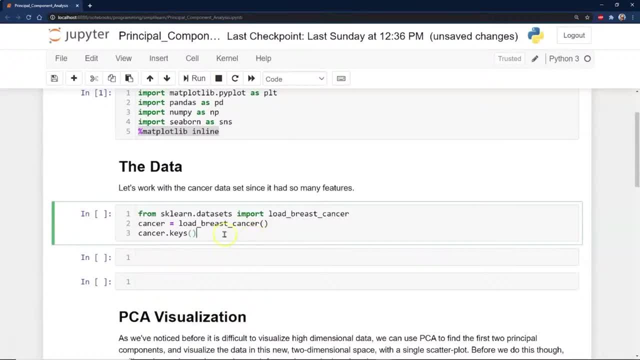 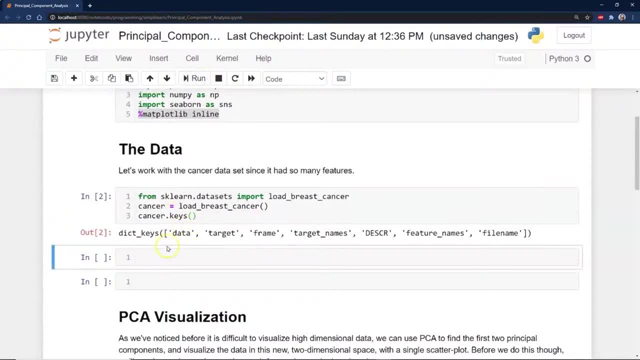 one of the reasons the cancer data set is it has like 36- 35 different features, so it's kind of fun to use that as our base for this. then we'll go ahead and run this and look at our keys and the first thing we notice in our 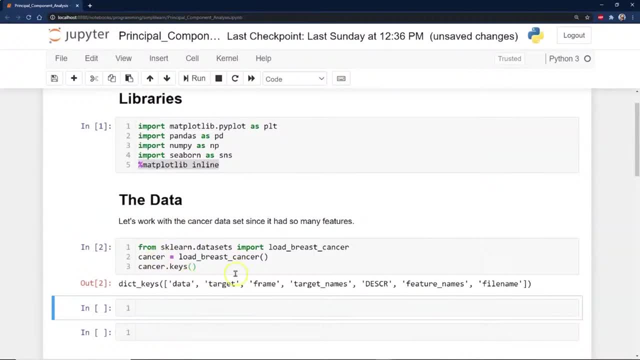 keys for the cancer data set is: we have our data, we have our target, our frame, target names, description, feature names and file name. so what we're looking for in all this is: well, let's take a look at the description. let's go in here and pull up the description. 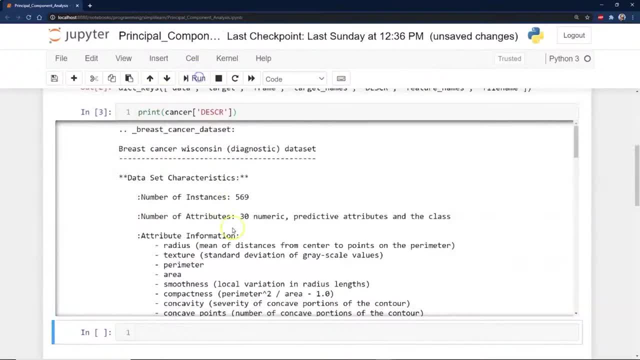 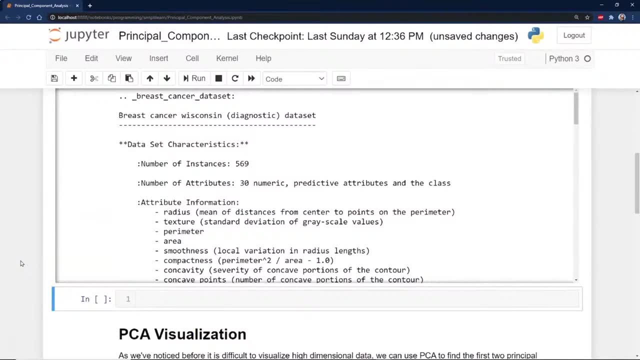 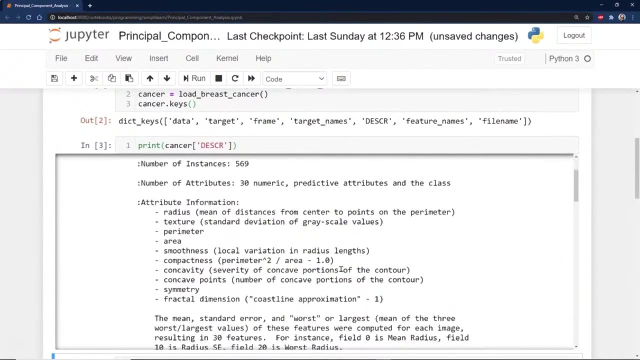 on here. I'm not going to spend a huge amount of time on the description, because this is. we don't want to get into a medical domain. we want to focus on our PCA setup. what's important is you start looking at what the different attributes are, what they mean. 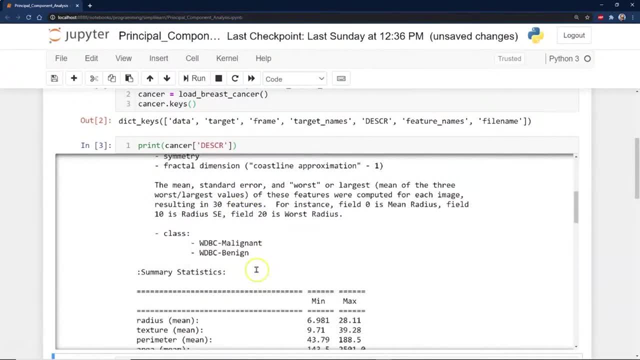 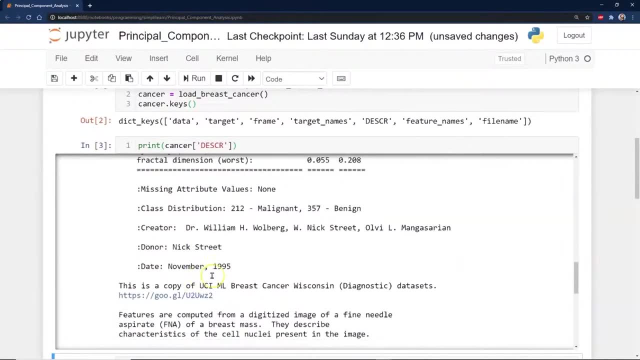 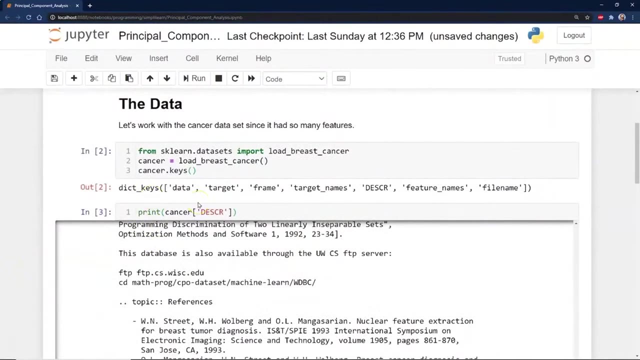 if you were in the medical field, you'd want to note all these different things, whether what they're measuring, where it's coming from, you can actually see the actual different measurements they're taking, no missing attributes. we page all the way to the bottom and you're going to have your data. in this case, 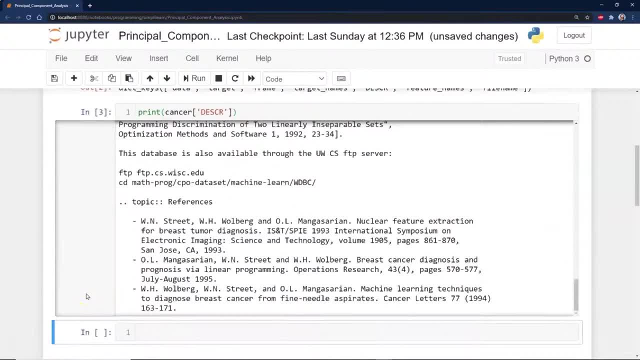 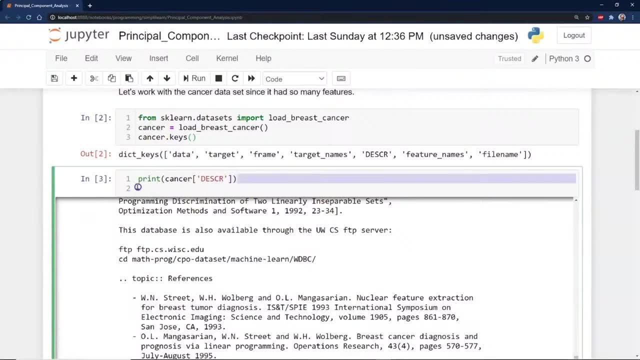 our target, and if you dig deep enough to the target, let's actually do this. let's go ahead and print names real quick here. I always like to just take a look and see what's on the other end of this. target names run that, so the target name is. 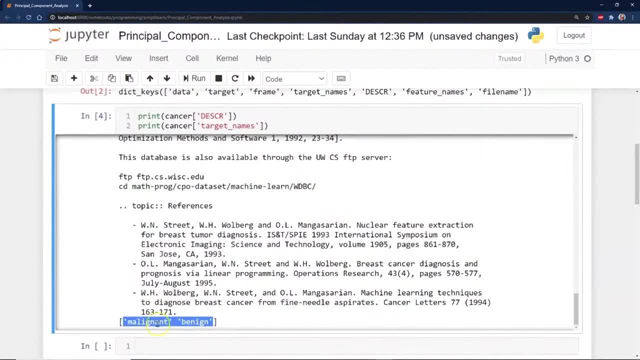 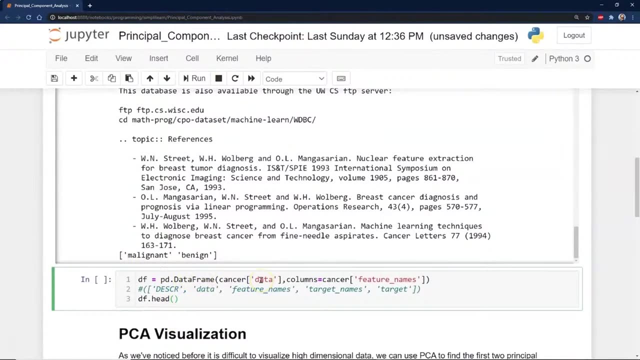 is it malignant or is it benign? so, in other words, is this dangerous growth or is it something we don't have to worry about? that's the bottom line with the cancer in this case, and then we can go ahead and load our data, and let me go up just a notch. 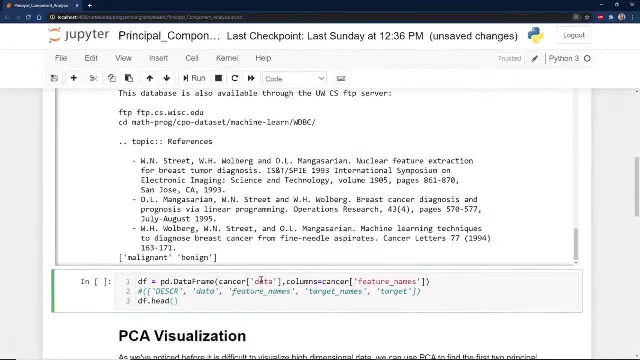 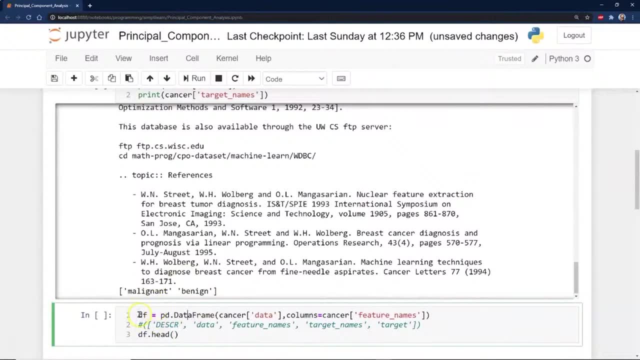 here for easy of reading. it's hard to get that just right. so let's go ahead and look at our data. we're going to use our pandas and we're going to go ahead and do our data frame. it's going to equal cancer data columns. equals cancer feature. equals feature names. 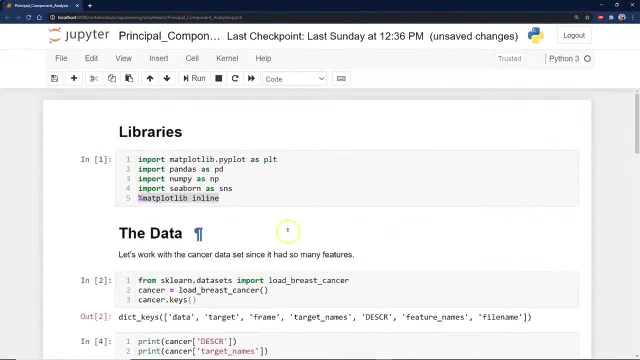 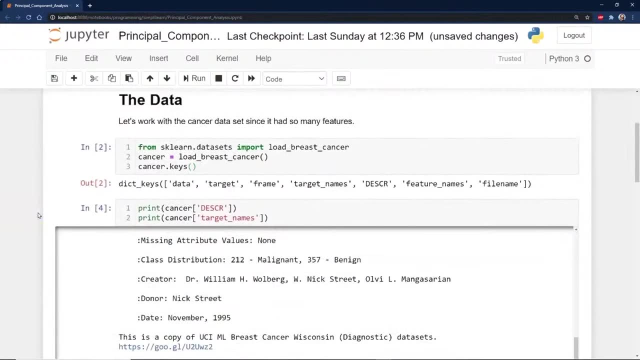 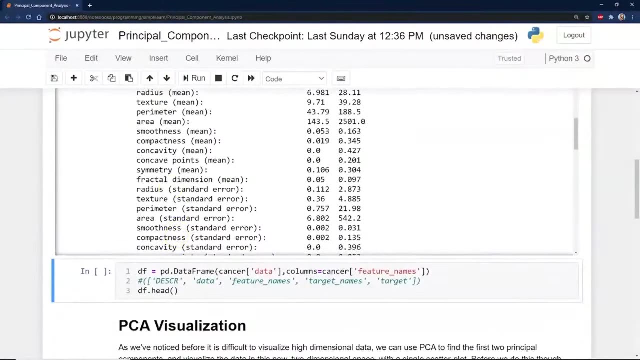 so remember up here we already loaded the names up of our of the features in there. what is going to come out of this? let me just see if I can get to that. it's at the top of target names. that's just this list of names here. 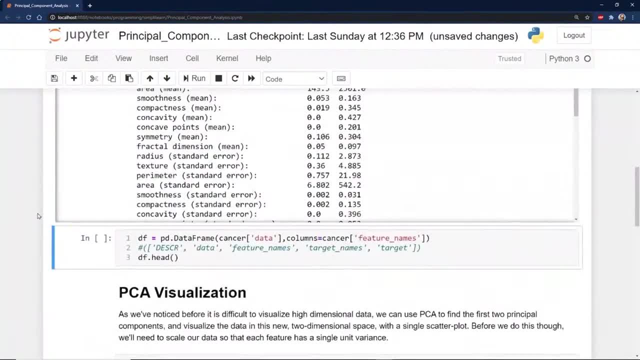 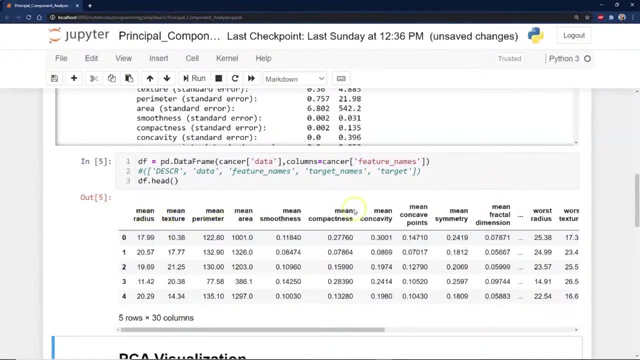 in the setup and we can go ahead and run this code and it'll print the head and you can see. here we have the mean radius, the mean texture, mean perimeter. how about you? this is a wonderful data set, if you're playing with it, because, like most of the data that comes in, 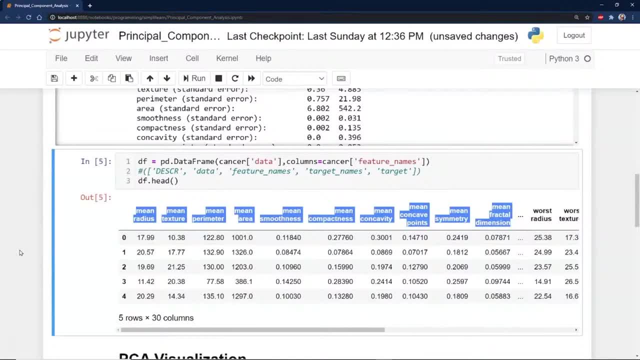 half the time, we don't even know what we're looking at. we're just handed a bunch of stuff as a data scientist going what the heck is this? and so this is a good place to start, because this has a number of different features in there and we have no idea what these feature means. 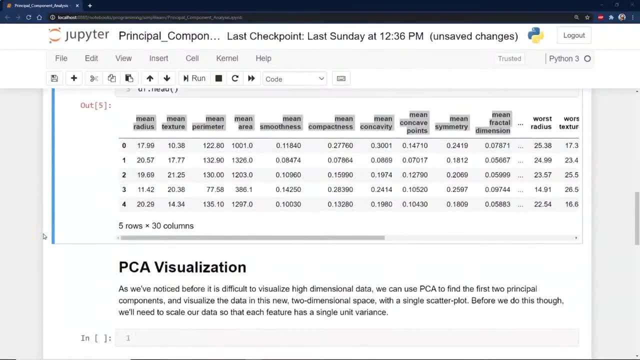 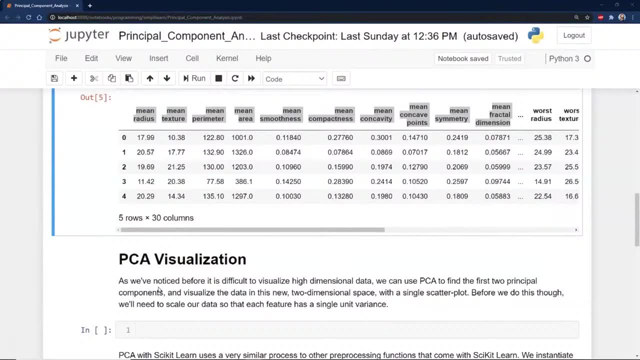 or where they come from. we want to just look at the data and figure that out. and now we actually are getting into the PCA side of it, because it's difficult to visualize high dimensional data. we can use PCA to find the first two principal components and visualize the data. 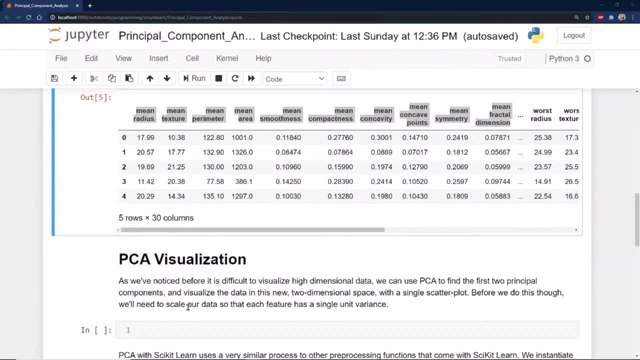 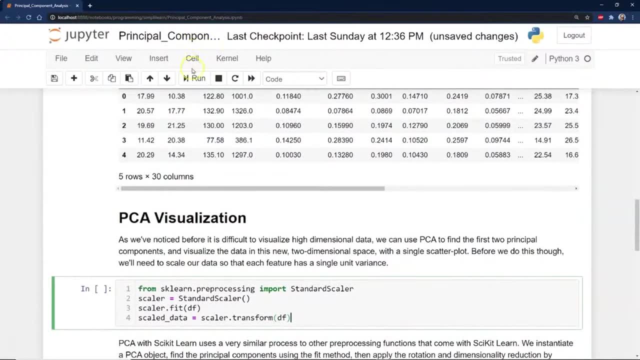 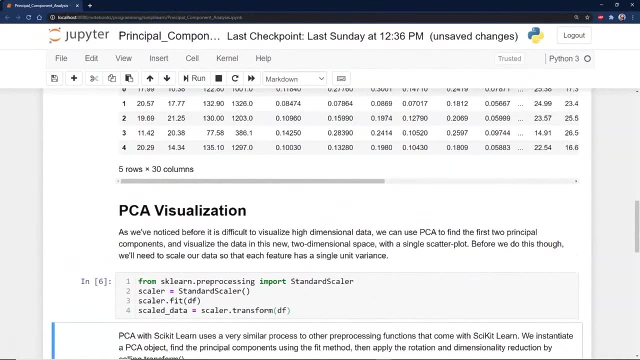 this new two dimensional space with a single scatter plot. before we do this, we need to go ahead and scale our data. now I haven't run this to see if you really have to scale the data on this, but as just a general run time, I almost do that. 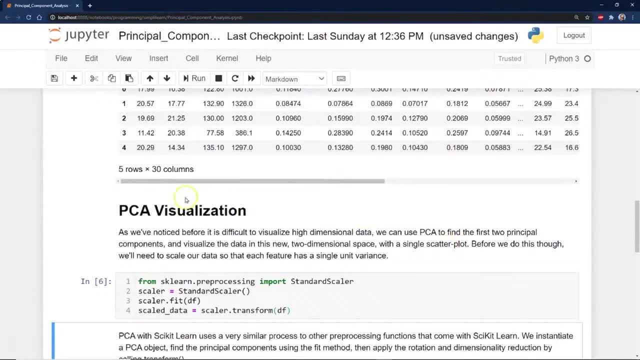 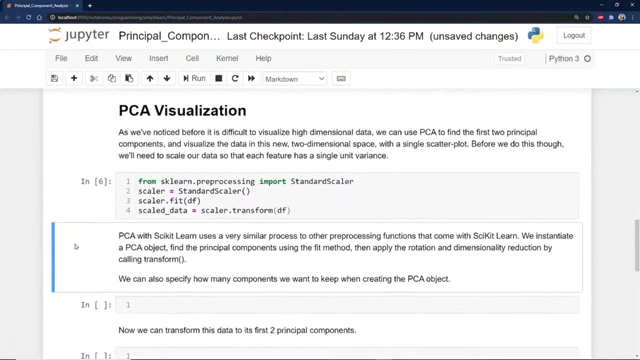 as the first step of any model, even if it's pre-modeling, as we're doing here in neural networks. that is so important with PCA visualization. it's already going to scale it when we do the means and deviation inside the PCA, but just in case, it's always good to scale it. 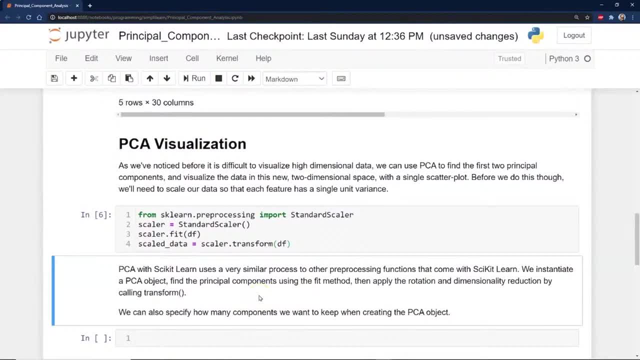 and then we're going to take our PCA with the scikit-learn uses. very similar process to other pre-processing functions that come with scikit-learn: we instantiate a PCA object, find the principal components, then apply the rotation and dimensionality reduction by calling transform. 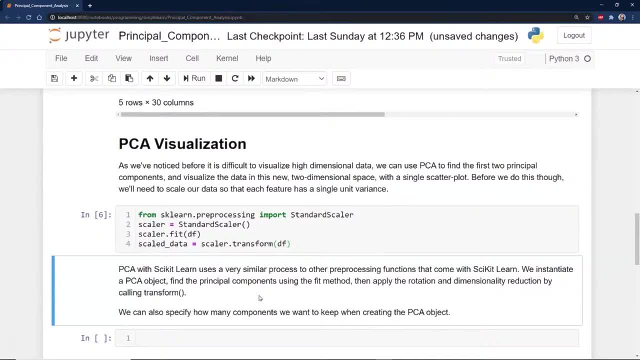 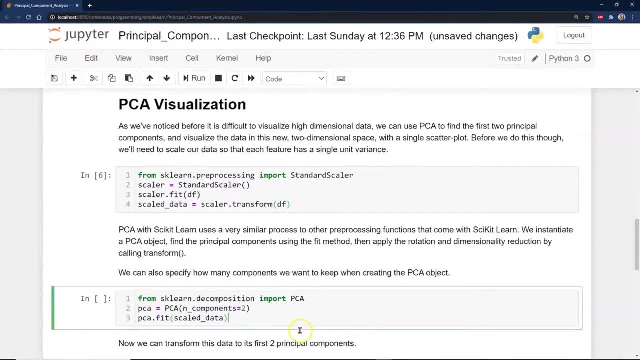 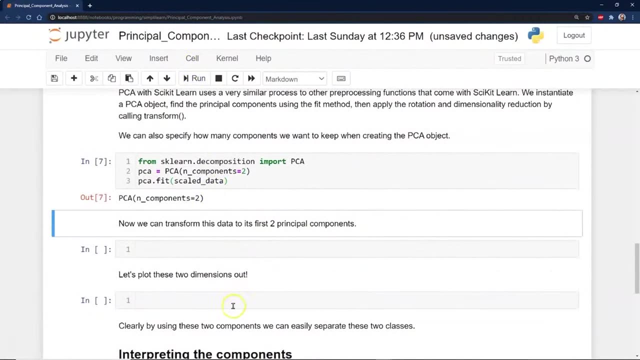 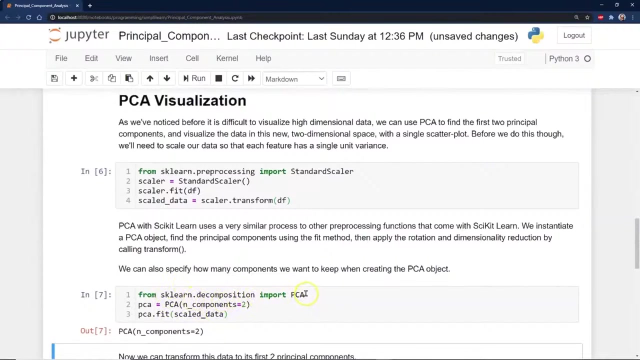 we can also specify how many components we want to keep when creating the PCA object, and so the code for this- oops, getting a little bit ahead, I'm going to run this code. so the code for this is from sklearn decomposition input: PCA. PCA equals PCA and components equals two. 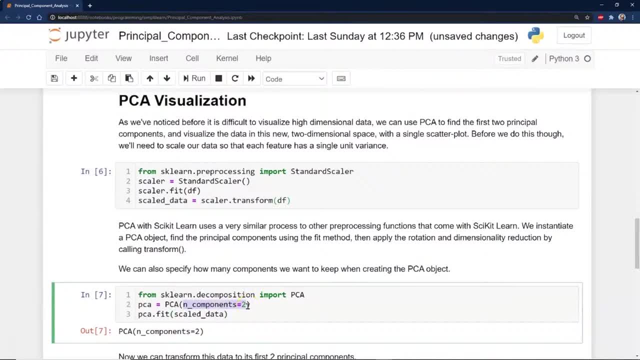 and that's really important to note that, because we're only going to want to look at two components. I would never go over four components, especially if you're going to demo this with somebody else. if you're showing this to the shareholders, the whole idea is to reduce it to something. 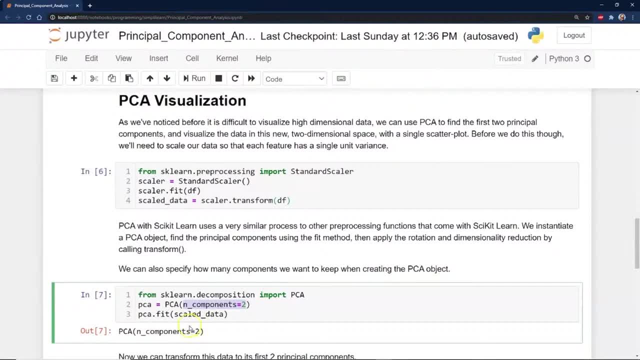 people can see, and then the PCA fit is going to take the scaled data that we generated up here and then you can see we've created our PCA model with: in components equals two. now, whenever I use a new tool, I like to go in there and actually 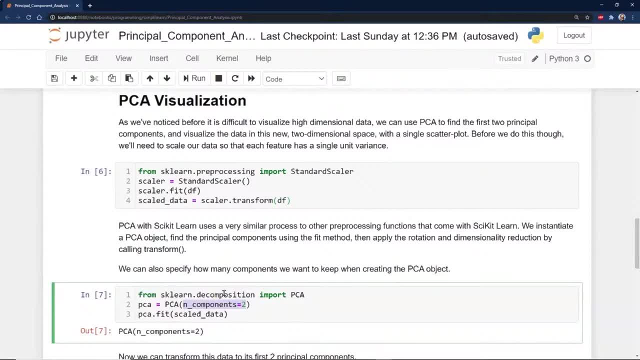 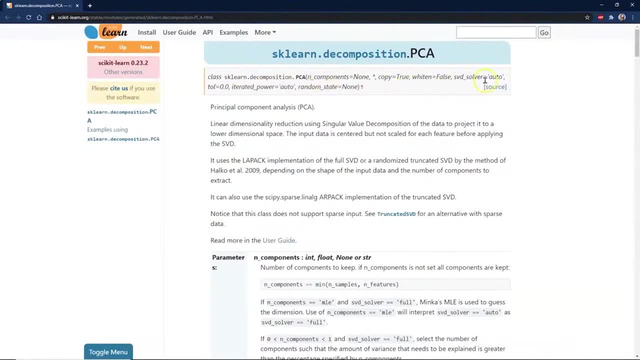 see what I'm using. so let's go to the scikit webpage for the PCA and you can see in here. here's our call statement. it describes what all the different setups you have on there- probably the biggest one to look at- would be. well, the biggest one is your components. 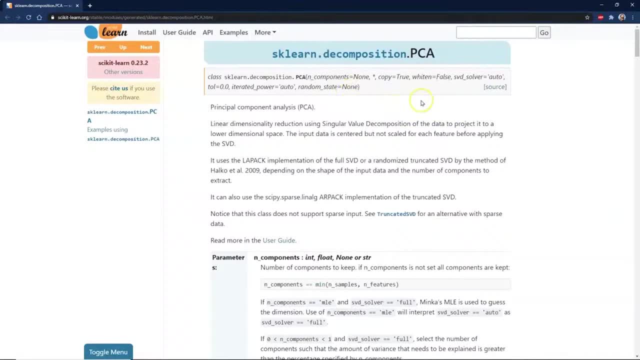 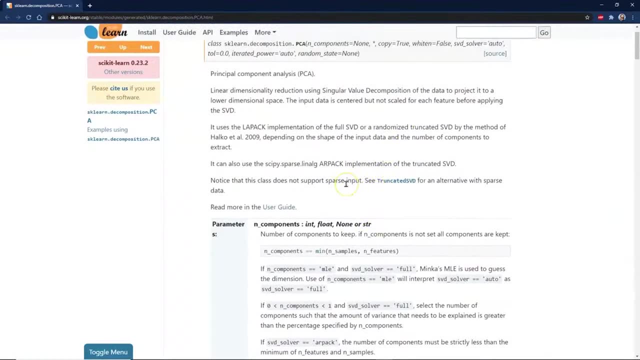 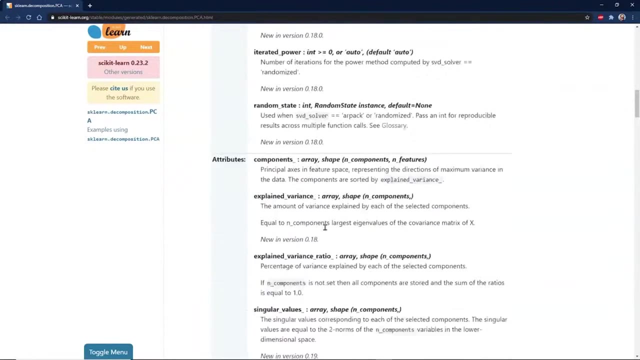 which you have to put in there pretty much, and then you also might look at the SVD solver. it's on auto right now, but you can override that and do different things with it. it does a pretty good job as it is, and if we go down. 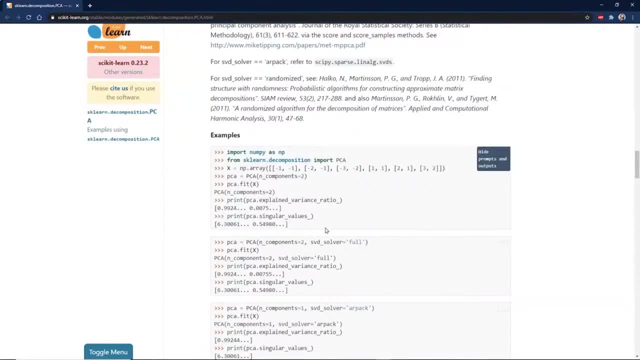 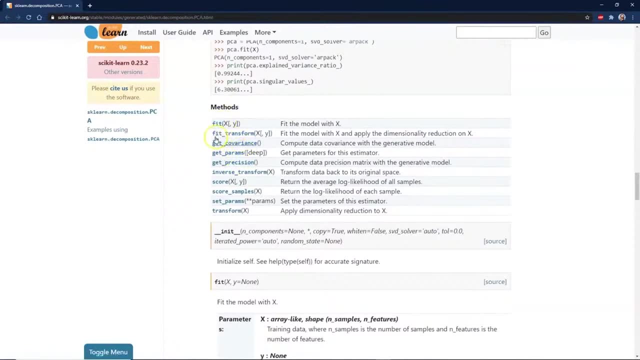 all the way down to there. we go to our methods. if you notice we have fit and transform. nowhere in here is predict, because this is not used for prediction. it's used to look at the data again. we're in the describe setup. we're fitting the data. 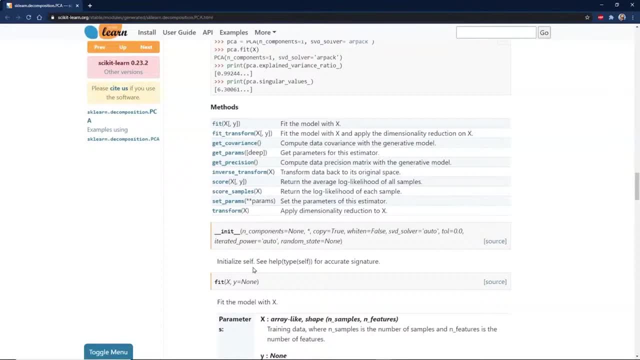 we're taking a look at it. we've already looked at our minimum maximum. we've already looked at what's in each quarter. we've done a full description of the data. this is part of describing the data. that's the biggest thing I take away when I come zooming in here. 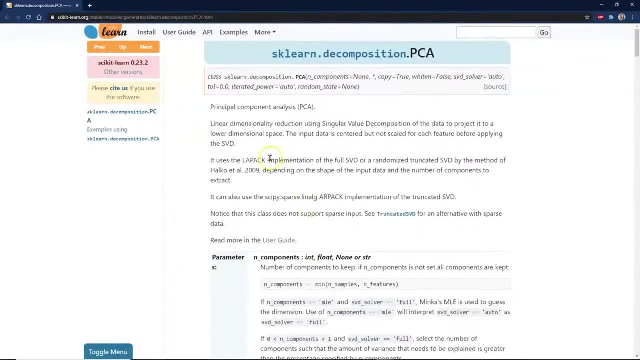 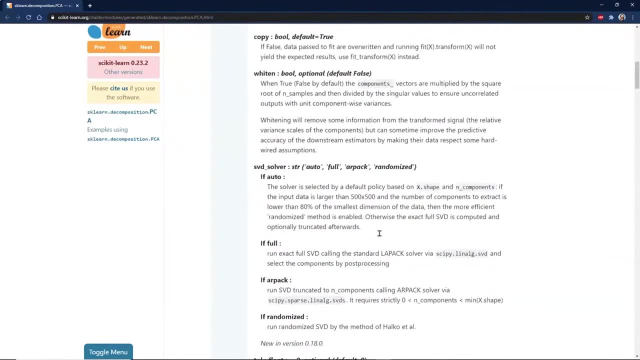 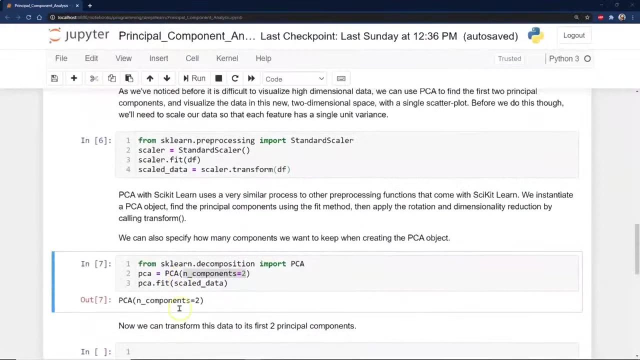 and of course they have examples of it down here, and the biggest one of course is the number of components and then the rest. you can play with the actual solver, whether you're doing a full or randomizer. it does pretty good on the auto and now we can transform. 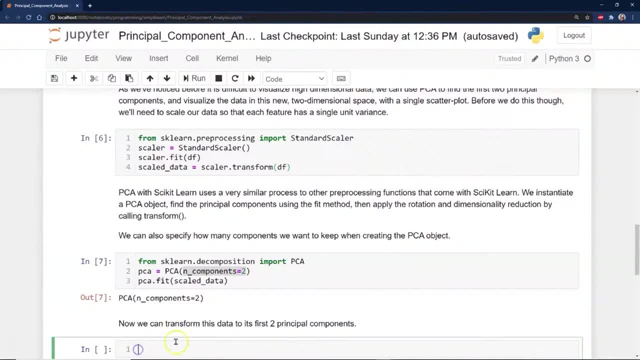 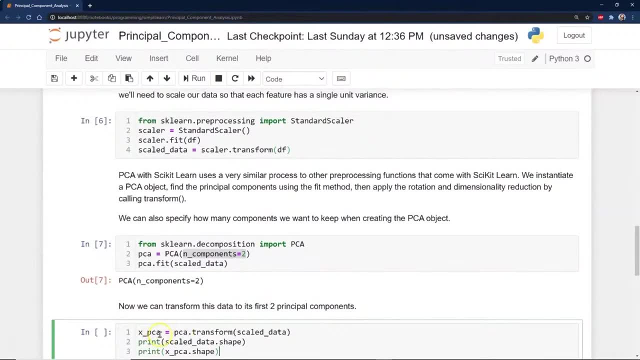 this data to its first two principal components, and so we have our XPCA. we're going to set that equal to the PCA transform scaled data. so there we go, there's our first transformation, and let's just go ahead and print the scaled data shape and the 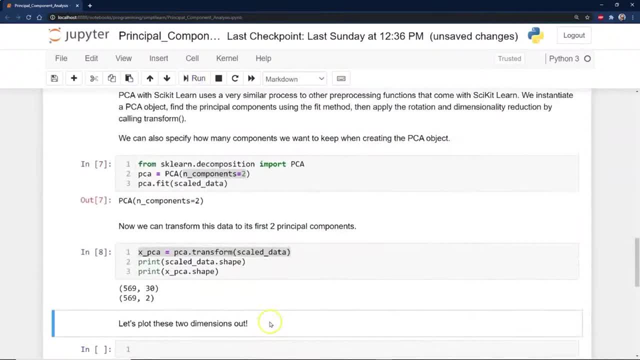 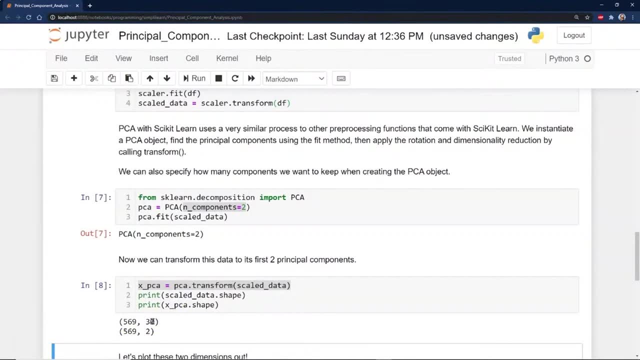 XPCA data shape, and the reason we want to do this is just to show us what's going on here. we've taken 30 features- I think I said 36 or something like that, but it's 30- and we've compressed it down to two features. 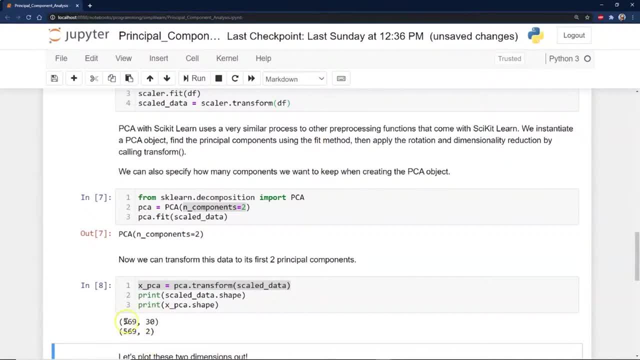 and we decided we wanted two features. and that's where this comes from. we still have 569 data sets. I mean data rows, not data sets. we still have 569 rows of data, but instead of computing 30 features, we're now only doing our model on two. 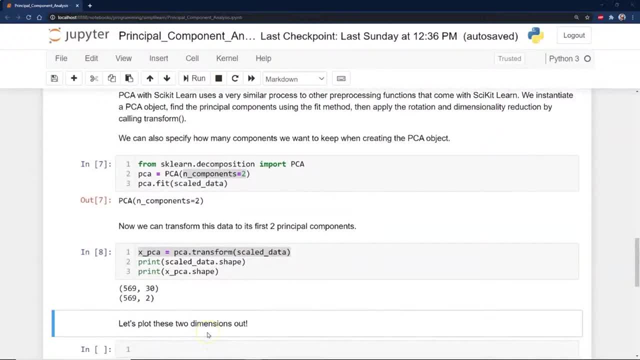 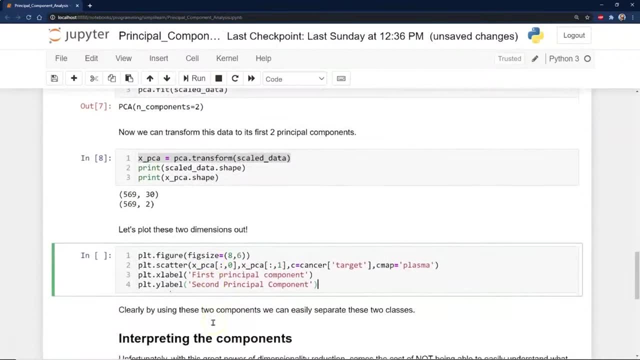 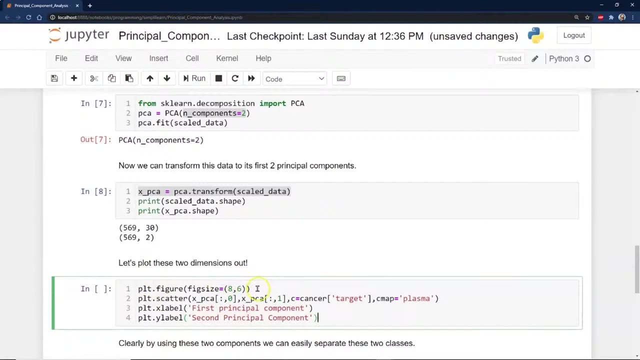 features. so let's go ahead and plot these and take a look and see what's going on, and we're just going to use our PLT figure. we're going to set the figure size on here. here's our scatter plot: XPCA X, underscore PCA of one. 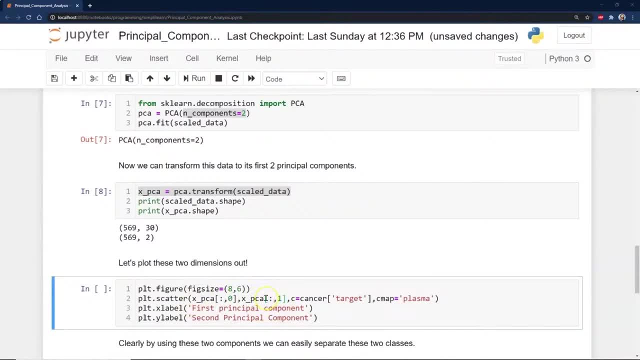 these are our two different perceptions we're using, and then you'll see right here: C for color cancer equals target, and so remember, we have zero, we have one, and, if I remember correctly, zero was malignant, one was benign. so everything in the zero column is going to be one color and the other color is: 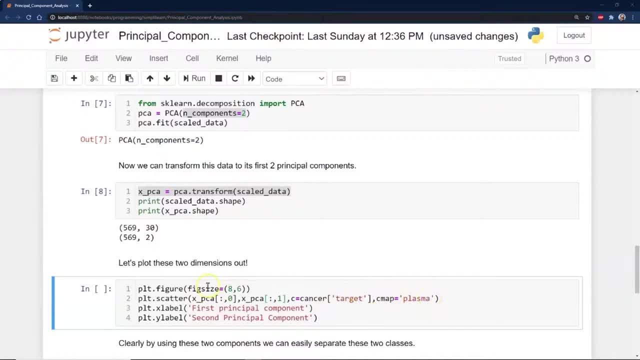 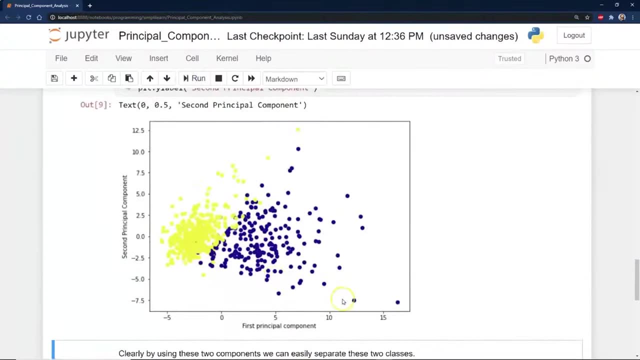 going to be one, and then we're going to use the plasma map just kind of telling you what color it is, add some labels- first principal component, second principal component- and we'll go ahead and run this and you can see here, instead of having a chart, one of those heat maps with 30. 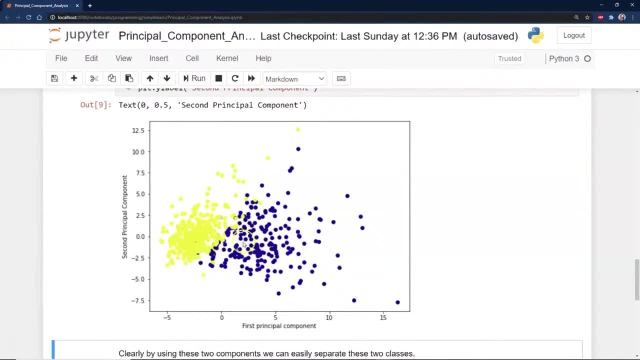 different columns in it. we can look at this and say, hey, this one actually did a pretty good job of separating the data and a couple things. when I'm looking at this that I notice is: first, we have a very clear area where it's clumped together. 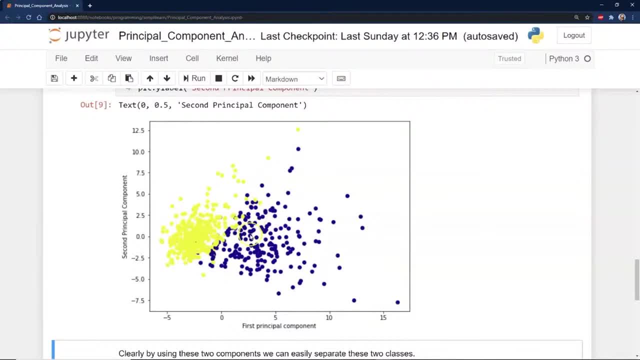 where it's going to be benign and we have a huge area, it's still clumped together, more spread out where it's going to be malignant, or I think I had that backwards and then in the middle because we're dealing with something, in this particular case, cancer. 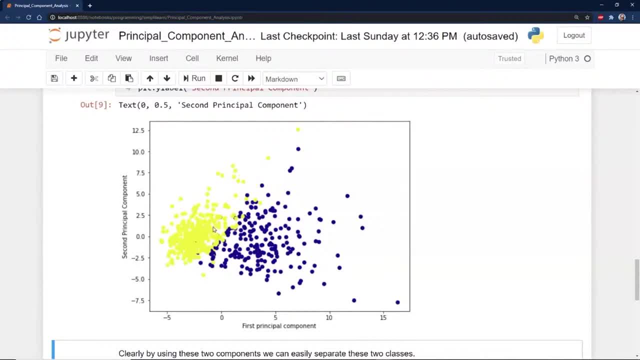 we would try to separate. I would be exploring how to separate this middle group out. in other words, there's an area where everything overlaps and we're not going to have a clear result on it just because those are the people. you want to go in there and have extra tests. or treat it differently, versus going in and saying just cutting into the cancer so the body absorbs it and it dissipates, versus actively going in there, removing it, testing it, going through chemo and all the different things. that's a big difference, you know, as far as what's going to happen. 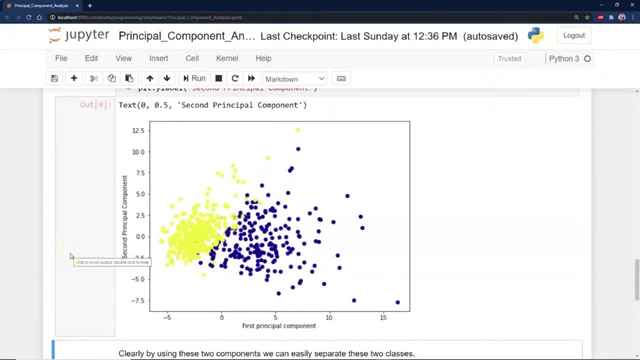 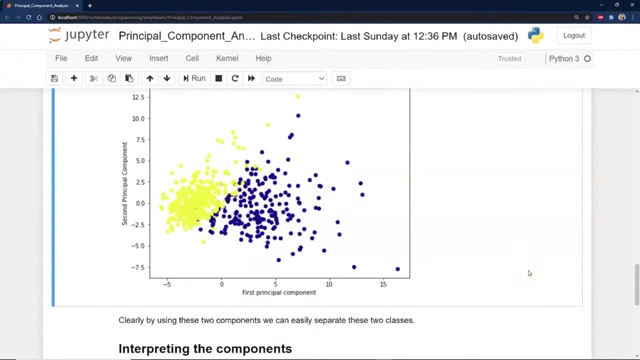 here in that middle line where they overlap, is going to be huge. that's domain specific. going back to the data, we can see here: clearly, by using these two components we can easily separate these two classes. so the next step is: what does that mean? interpreting the components? 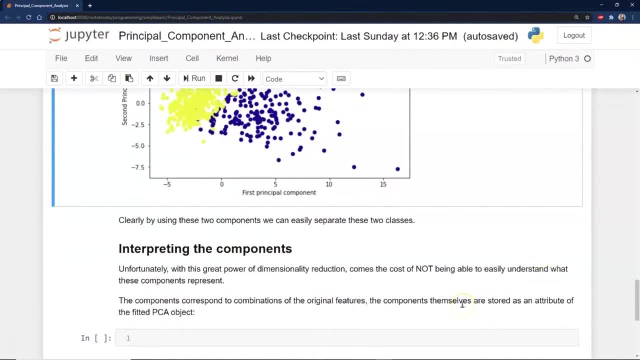 unfortunately, with this great power of dimensionality reduction comes the cost of not being able to easily understand what these components represent. I don't know what principle component one represents, or second principle. the components correspond to combinations of original features. the components themselves are stored as an attribute of the 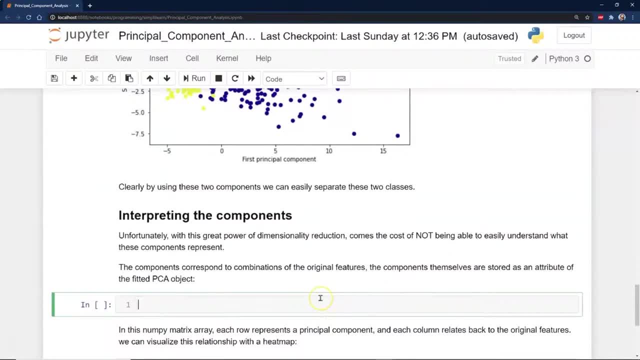 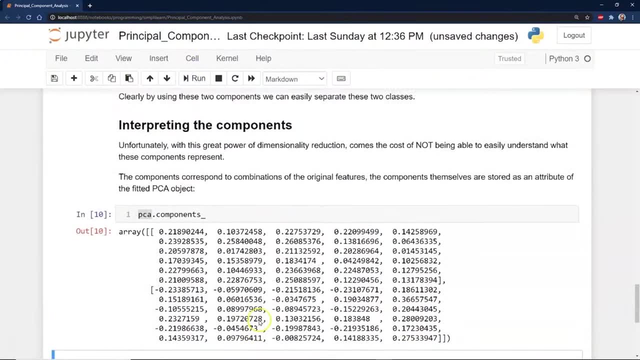 filtered PCA object and so when we look at that, we can go ahead and look at the PCA components. this is in our model we built, we've trained it. we can run that and you can see. here's the actual components. it's the two components each have their own array. 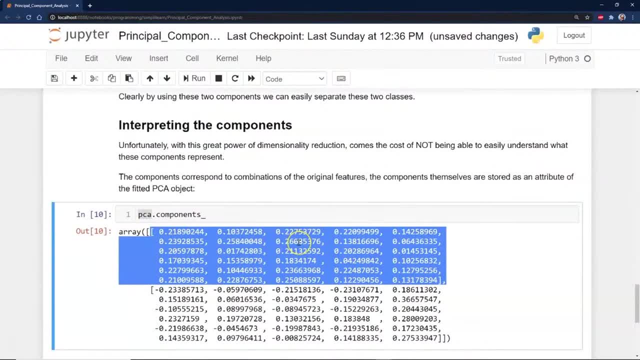 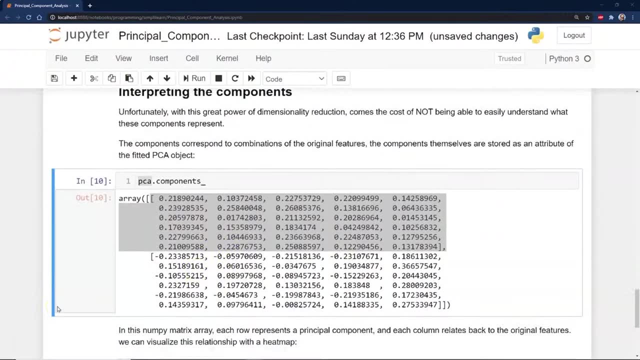 and within the array you can see the scores they're using, and these actually give weight to what features are doing what. so, in this numpy matrix array, each row represents a principle component and each column relates back to the original features. what's really neat about this is we can now 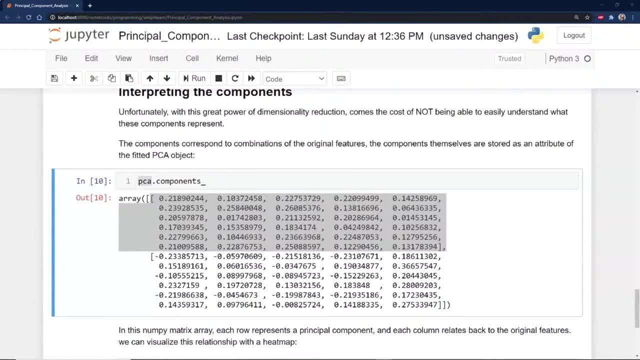 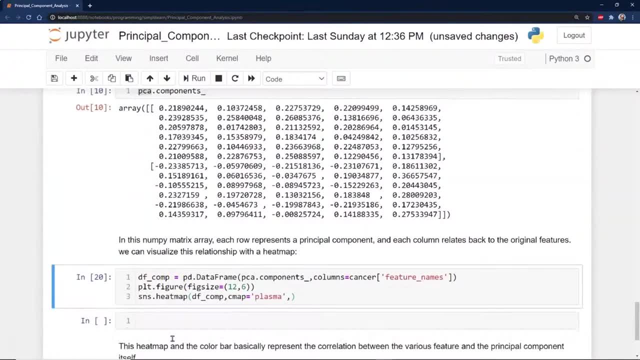 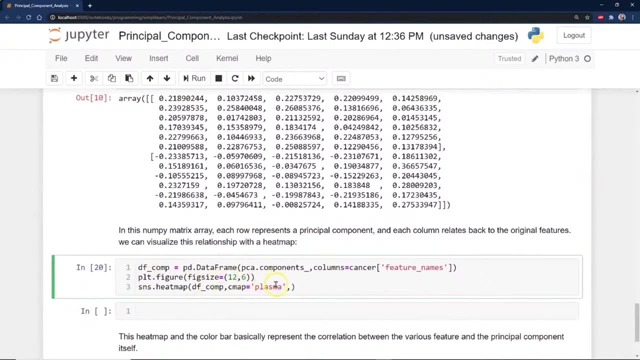 go in reverse and drop this onto a heat map and start seeing what this means. so let me go ahead and just put this down. we go ahead and put this in here. we're going to use our DF comp data frame and we do our PCA components, and I want you to notice how. 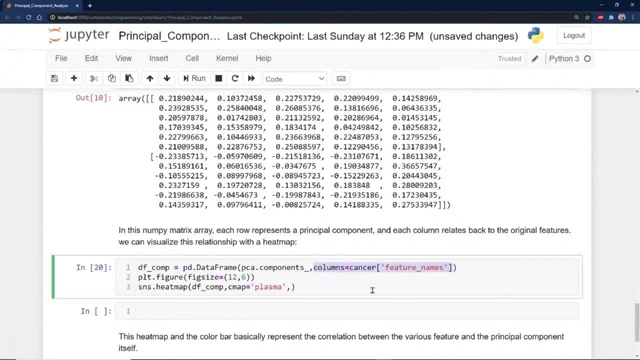 easy this is. we're going to set our columns equal to cancer feature names. that just makes it really easy, and we're dumping it into a data frame. what's neat about a data frame is when we get to seaborn, it will pull that data frame apart and set it up for us. 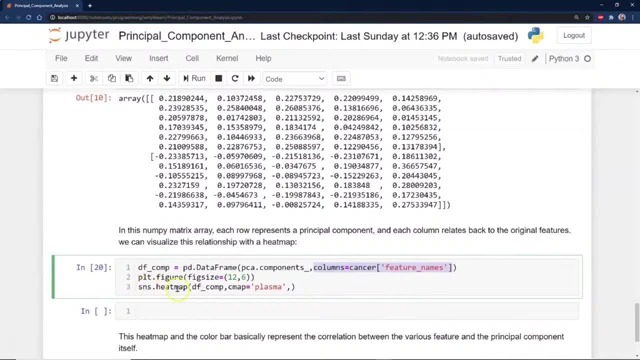 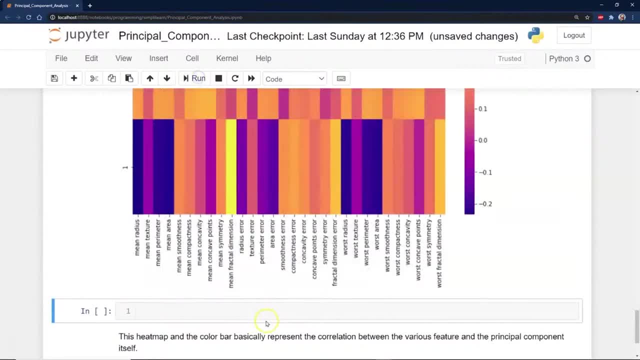 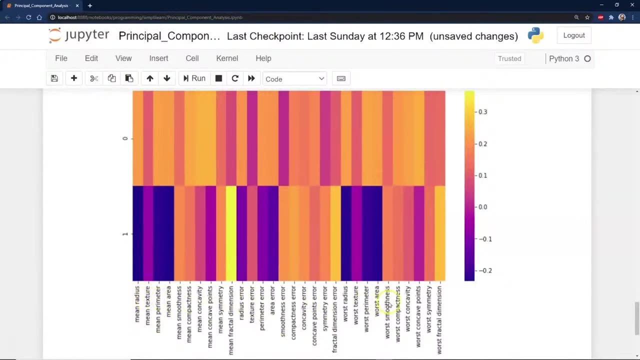 what we want, and so we're just going to do the seaborn heat map of our data frame composition and we'll use the plasma coloring and it creates a nice little color graph. here you can see we have the mean, radius and all the different features along the bottom on the right. 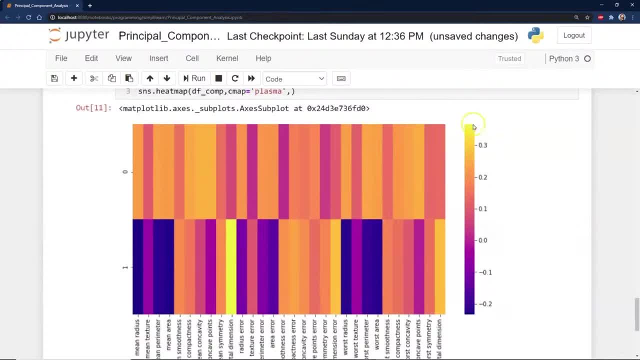 we have a scale so we can see. we have the dark colors all the way to the really light colors, which are what's really shining there. this is like the primary stuff we want to look at. so this heat map and the color bar basically represent the correlation. 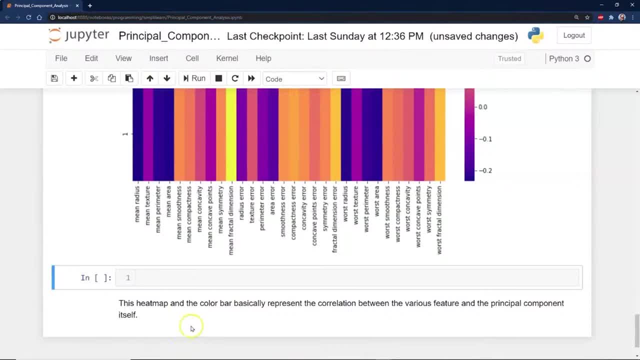 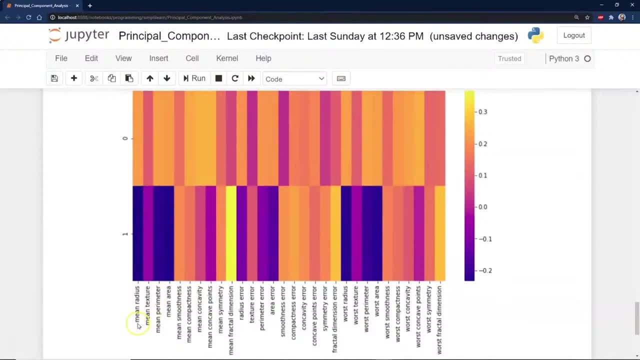 between the various features and the principal component itself. so you know very powerful map to look at and then you can go in here and we might notice that the mean radius. look how on the bottom of the map it is on some of this. so you have some interesting correlations. 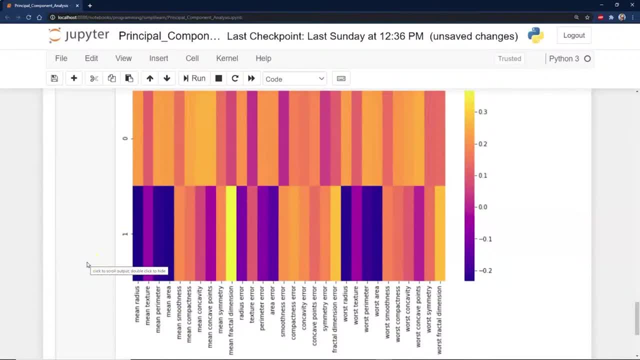 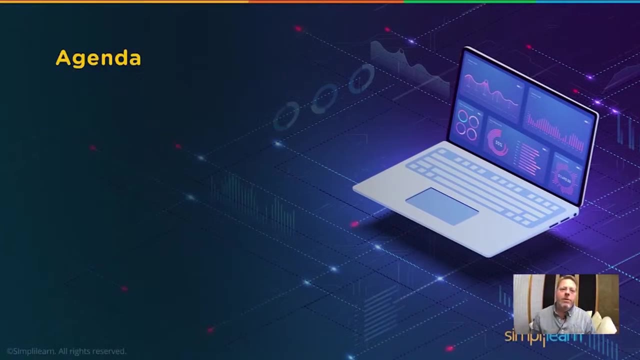 here that change the variations on that and what means what this is more, when you get to post scribe, you can also use this to try to guess, as what these things mean, what you want to change to get a better result: regularization in machine learning. so our agenda on this one is: 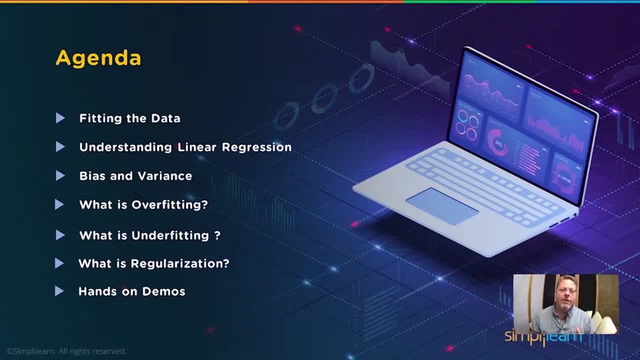 fitting the data, understanding linear regression, bias and variance. what is over fitting, what is under fitting- and those are like the biggest things right now in data science- is over fitting and under fitting. what does that mean? and what is regularization? and then we'll do a quick hands-on demo. 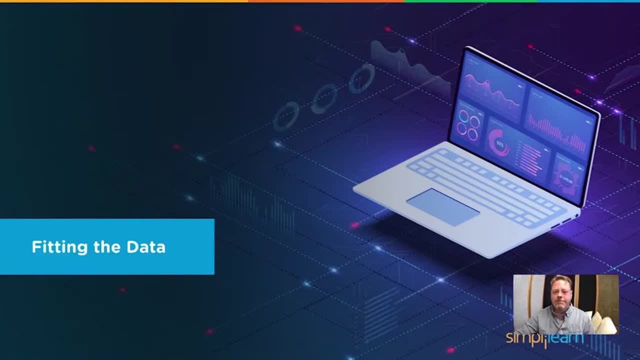 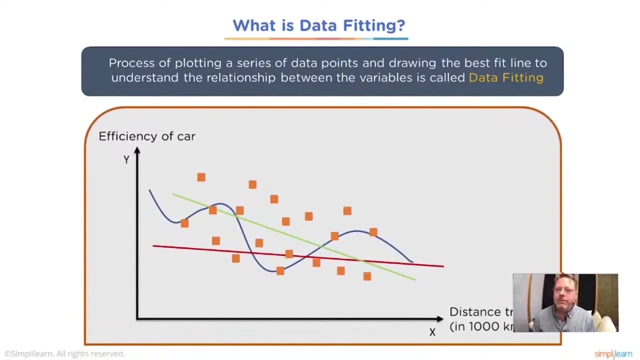 to take a look at this. so, fitting the data. let's start with fitting the data, and we talk about what is data fitting? it's a process of plotting a series of data points and drawing the best fit line to understand the relationship between the variables, and this is what we call data fitting. 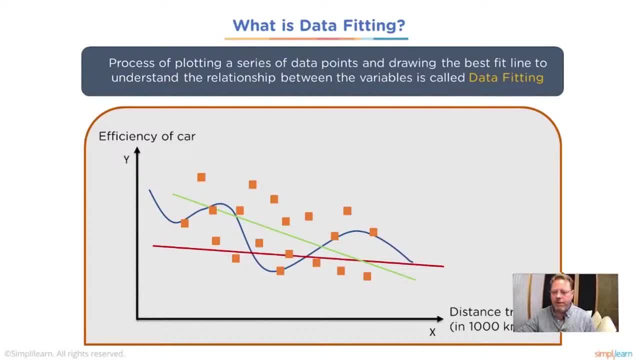 and you can see here we have a couple of lines we've drawn on this graph. we're going to go in a little deeper on there, so we might have, in this case, just two dimensions: we have an efficiency of the car and we have the distance traveled in. 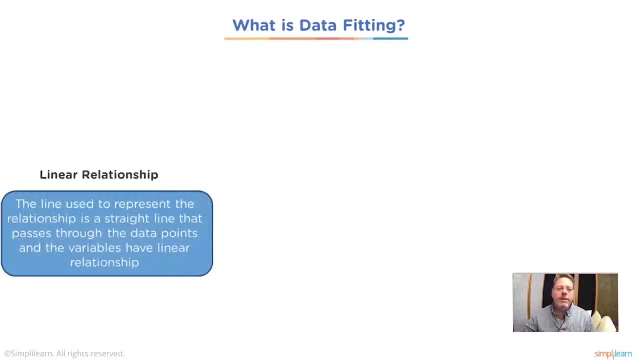 1000 kilometers. and so what is data fitting? well, it's a linear relationship and a linear relationship. very specifically, linear means line. the line used to represent the relationship is a straight line that passes through the data points and the variables have linear relationship, linear regression. so let's start with. 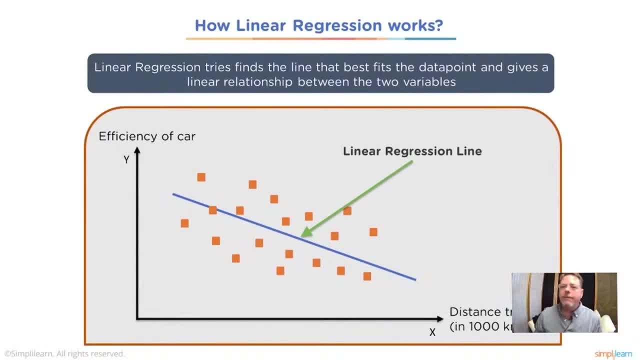 how linear regression works. linear regression is a line that best fits the data point and gives a relationship between the two variables, and so you can see here we have the efficiency of the car versus the distance traveled, and you can see this nice straight line drawn through there. 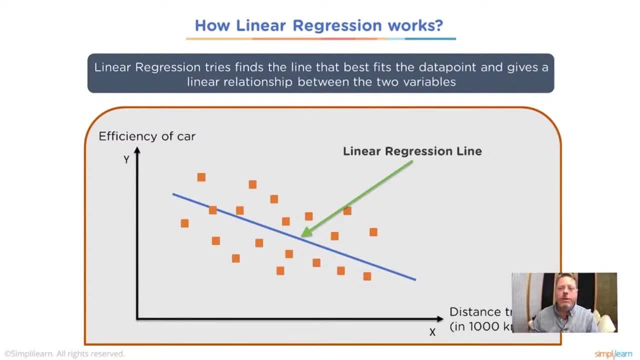 and when you talk about multiple variables, all you're doing is putting this: instead of a line, it now becomes a plane. it gets a little more complicated with multiple variables, but they all come down to this linear kind of drawing a line through your data and finding what fits the data. 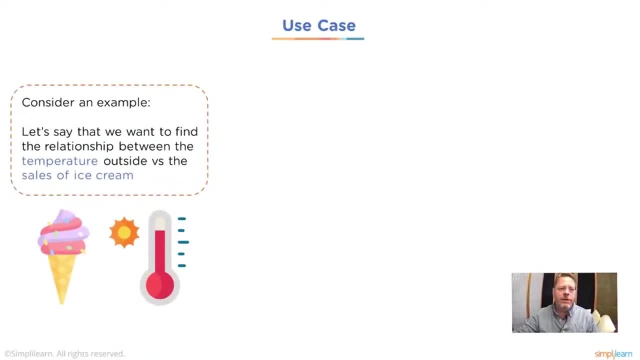 best. and so we can consider an example. let's say that we want to find the relationship between the temperature outside versus the sales of ice cream, and so we start looking at that. we're looking at how many ice cream cones we're selling or how much money we sold on ice cream. 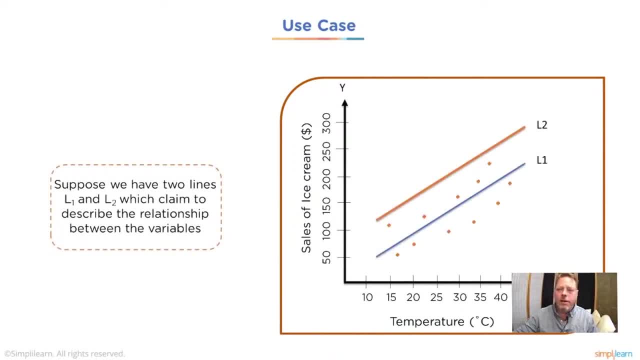 and we're looking at how warm it is outside, which would hopefully draw a lot of people into the ice cream store, and suppose we have two lines. we're going to draw L1 and L2 and we're going to kind of guess which one we think is the best fit. 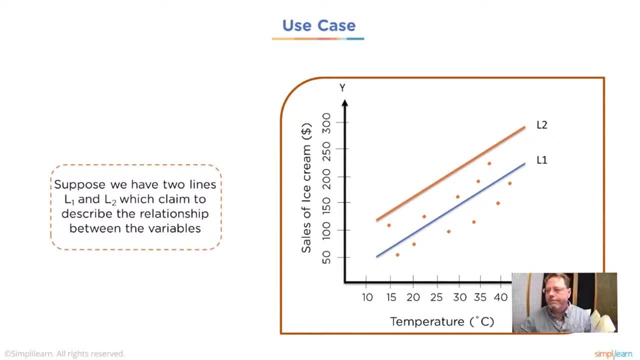 and which claim to describe the relationship between the variables. and so first we find the square of the distance between the line L1 and each data point and add them all and find the mean distance. and I want you to think about that: when we square something, if it's a negative or positive number, it no longer 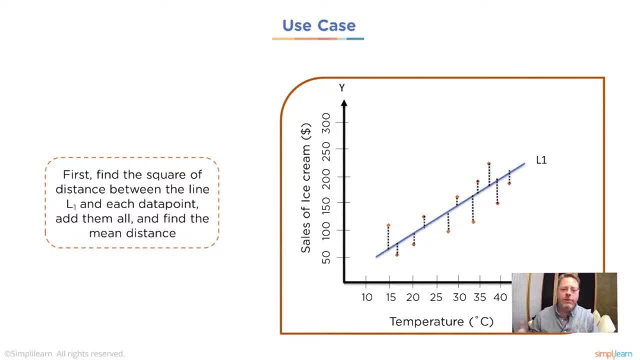 matters, because a minus 2 squared is 4, 2 squared is 4. so we're removing what side of the line it's on and we're just looking for the error, in this case the mean distance of each of the little dotted lines you see here. 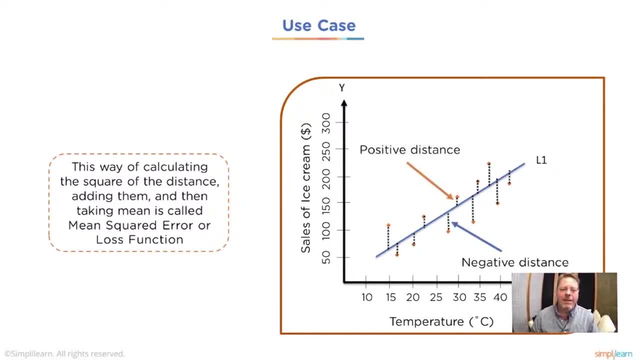 this way of calculating the square of the distance. adding them and then taking the mean is called mean square, error or loss function, and we talk about loss. how far off are we? that's what we're really talking about. what did we miss? and we have a positive distance. 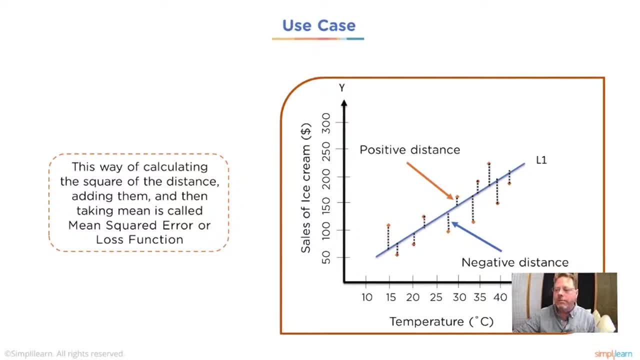 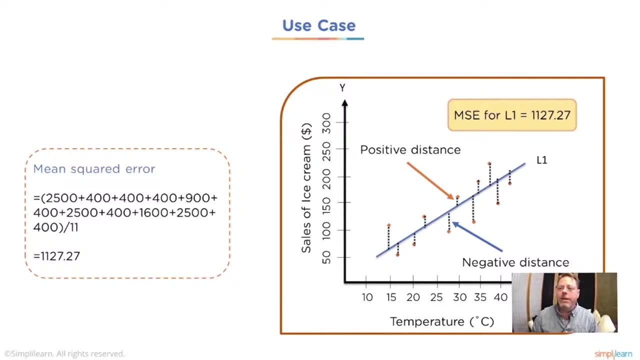 and a negative distance and of course, when we square it it is neither. it just becomes a positive error and so we take the mean square error and a lot of times you'll see it referred to as MSE. if I look in the code and I'm going through my python code, 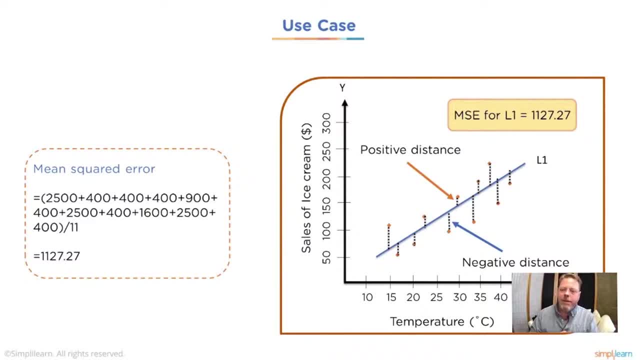 and I see MSE- I know that's the mean squared error- and we take all the dotted lines and we calculate this error and we add them all together and then we average it or find the means. and in this case they ran a demo on this and it was. 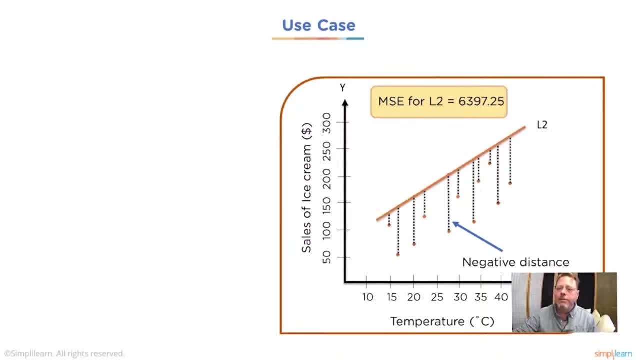 1127.27 for our L1 line. now we find the loss function for line L2 in a similar fashion and we get the mean square error to be 6397, and it's computed the same way. so maybe you put this line just way outside the. 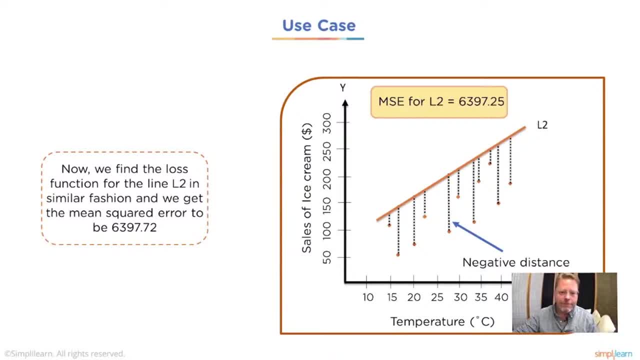 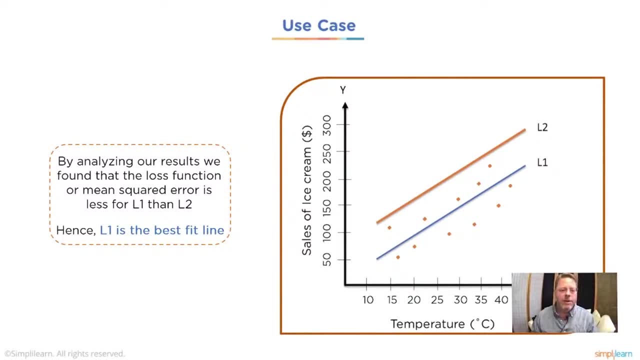 data range and this is the error you get. by analyzing our results, we find that the loss function, or the mean square error, is less for L1 than L2, hence L1 is the best fit line. this process describes a lot of machine learning processes. we're going to keep guessing and get as close as we can. 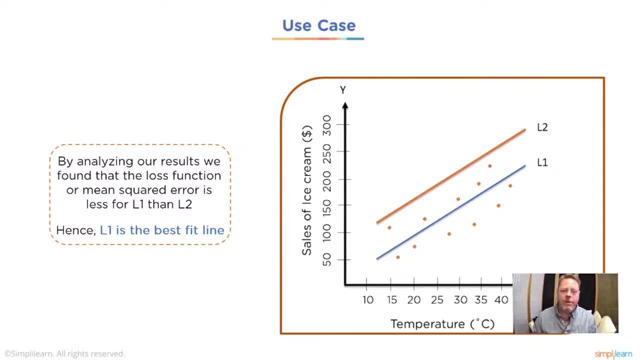 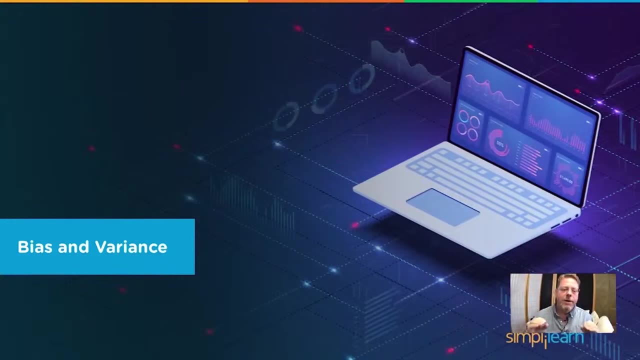 to find the right answer. we have to have some way to calculate this and figure out which one is the best, and the mean square error is one of the better fits for doing this and most commonly used. we really want to talk about bias and variance, very important terms to know in machine. 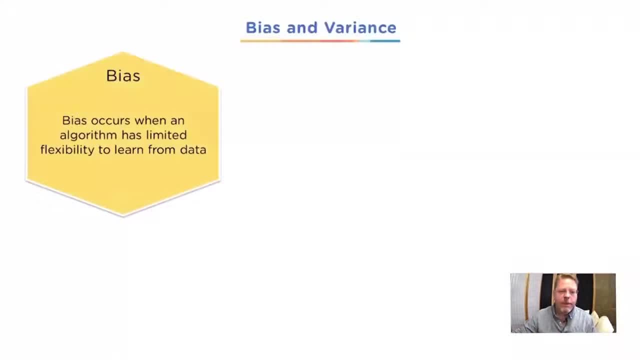 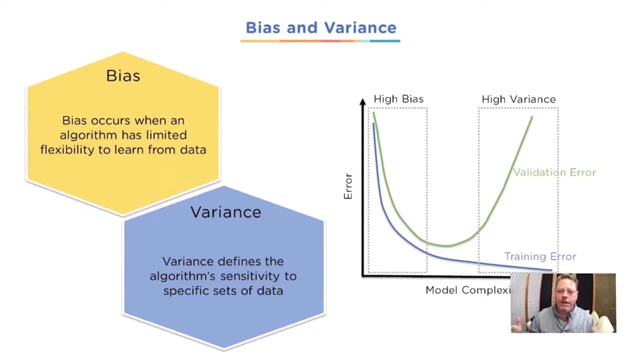 learning and with linear regression. so bias: bias occurs when an algorithm has limited flexibility to learn from data. variance defines the algorithm's sensitivity to specific sets of data. let's start with bias and variance. you can see here we have the two different setups. bias- you can think. 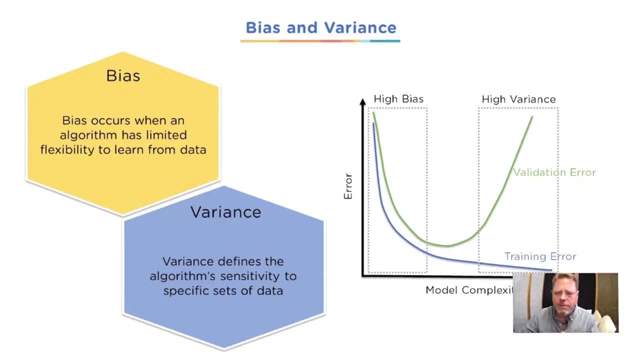 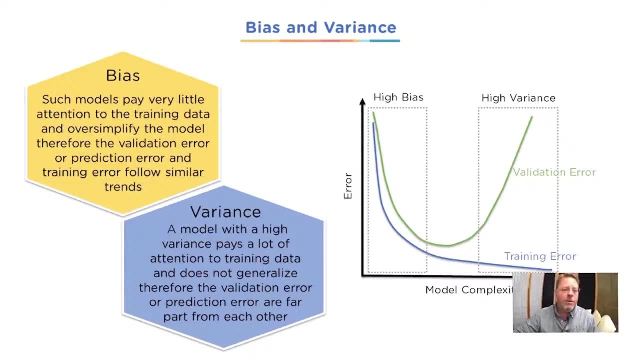 is very generalized, where variance is very specific, and so when we talk about bias, such models pay very little attention to the training data and oversimplify the model. therefore, the validation error, or prediction error, and training error follow similar trends and, with bias, if you oversimplify it so much, you're going to miss. 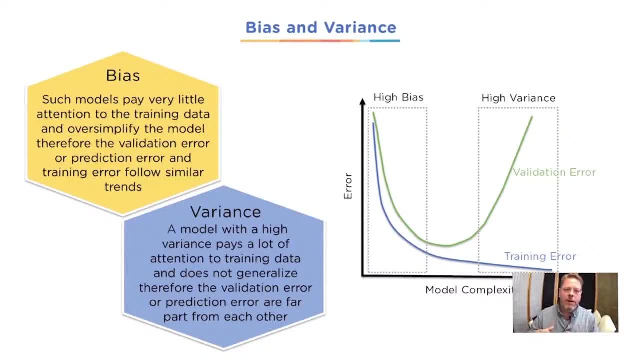 your local. if you have like a really good fit, you're going to miss it. you're going to just kind of guess what the average is and that's what your answer is going to be. with variance, a model with a high variance pays a lot of attention to. 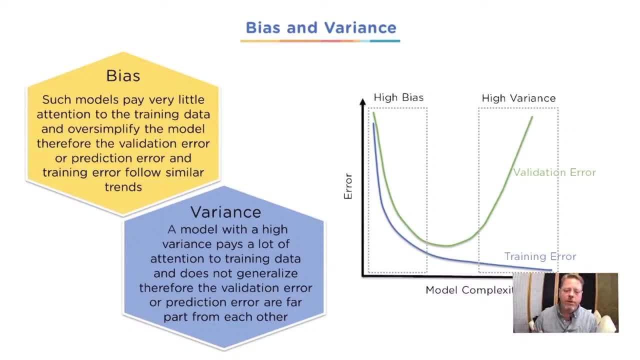 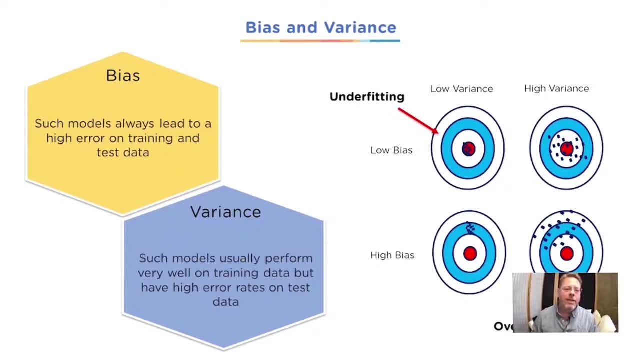 training data and does not generalize. therefore, the validation error or prediction error are far apart from each other. such models always lead to a high error on training and test data, as a bias does where variance. such models usually perform very well on training data but have high error rates on test data. 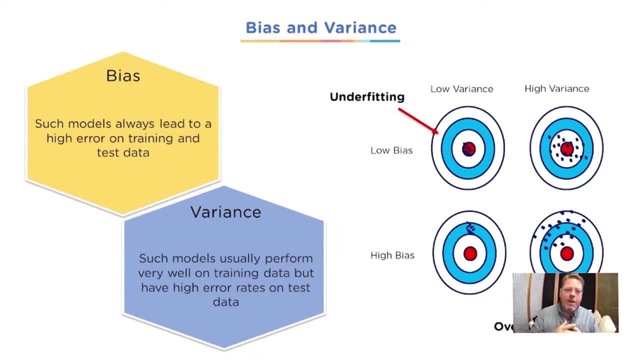 and I want you to think about this: when we're talking about a bias, the error is going to be high, both when you're training it and you're fitting it. why? because we're just kind of getting an average. we're not really fitting it close with variance. 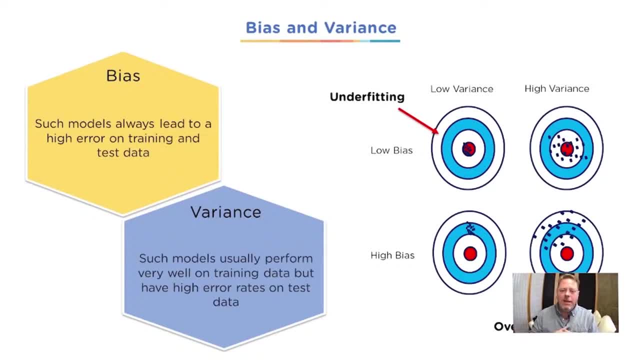 we're fitting it so close that the test data does really good. it's going to nail it every time. if you're doing categorical testing, that's a car, that's a truck, that's a bicycle, but with variance. suddenly a truck has to have certain features and it might have to. 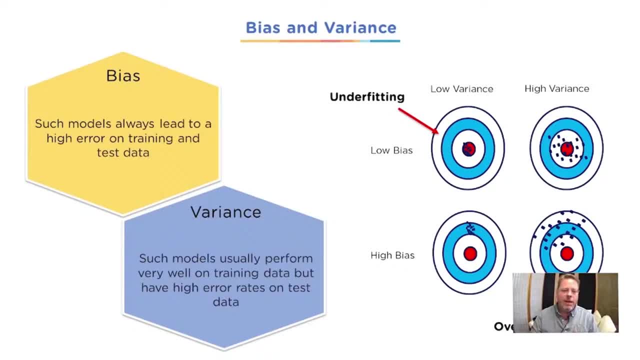 be red, because you had so many red pictures. so if it has, if it's an 18-wheeler, it has to be red. if it's blue, then it has to be a bicycle. that's the kind of variance we're talking about, where it picks up on something. 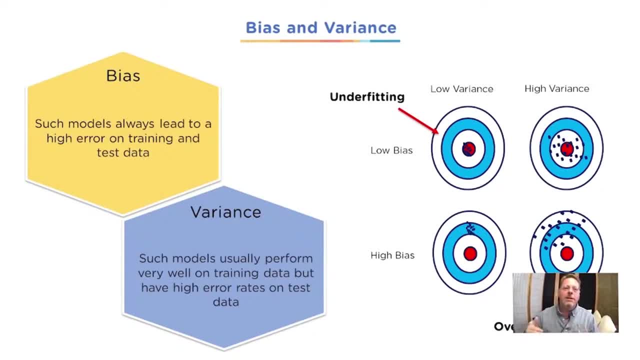 and it cannot get the right answer unless it gets a very specific data. and we see that so that as you're testing it, your models and you programmed it, you got to look for how I trained it, what is coming out and if it's not looking good on either. 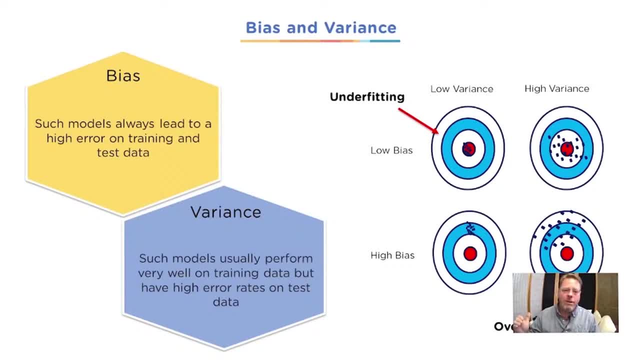 bias. or if it's not looking good on the training or on the test data, then you're biased in your data. if it really looks good on the training data, then that's going to be your variance. you've overfitted the data, and those are very important things to know. 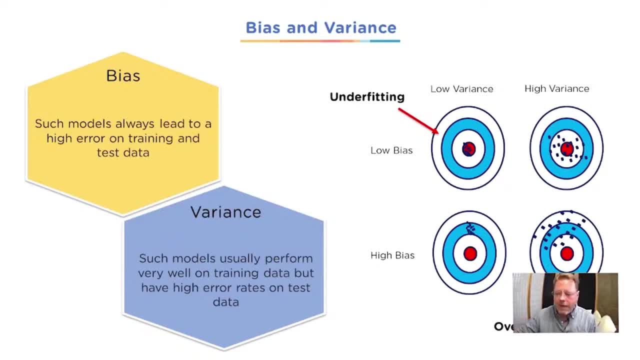 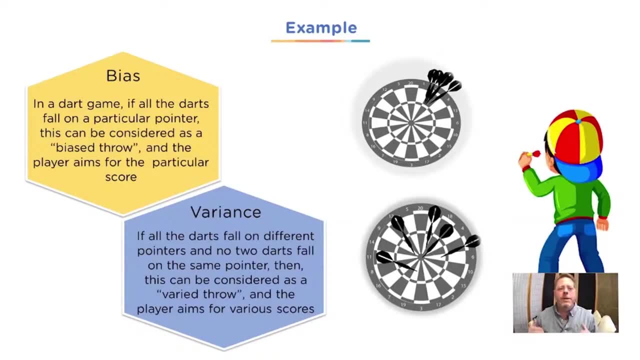 when you are building your models in regression of any kind or any kind of setup for predicting. so in dart games, if all the data fall on a particular pointer, this can be considered as a biased throw and the player aims for the particular score for variance, if all the 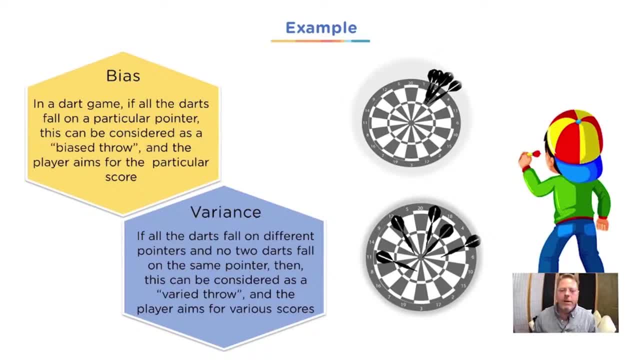 darts fall on different pointers and no two darts fall on the same pointer, then this can be considered as a varied throw and the player aims for various scores. again, the bias sums everything up in one point, kind of averages it together, where the variance really looks for the individual. 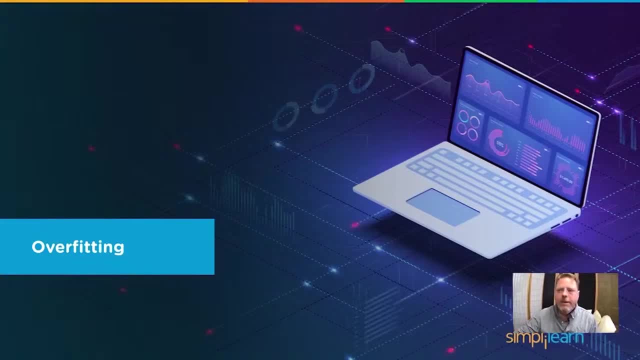 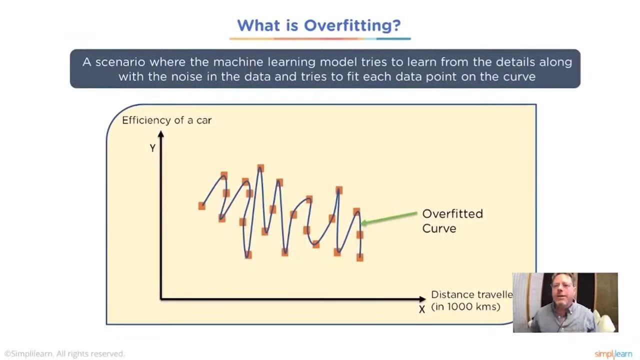 predictions coming out, so let's go ahead and talk about overfitting. when we talk about overfitting, it's a scenario where the machine learning model tries to learn from the details, along with the noise and the data, tries to fit each data point on the curve. you can see. 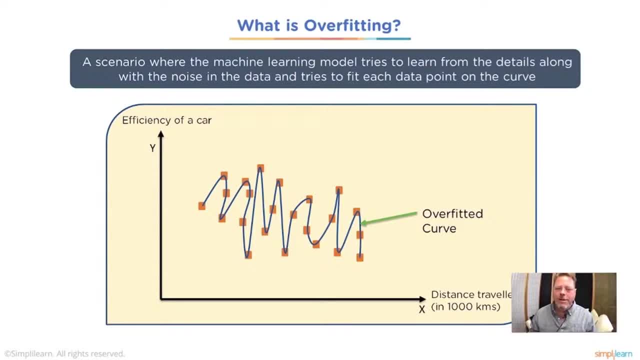 that if you plug in your coordinates you're just going to get the whatever is fitted, every point on the data stream. there's no average, there's no two points that might have why it might have two different answers. because if the wind blows a certain way and the efficiency 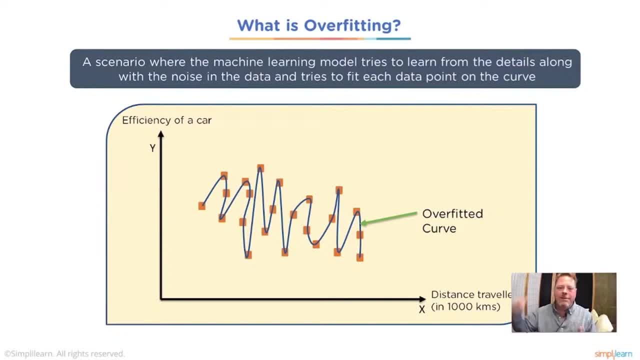 of your car. maybe you have a head wind, so your car might alter how efficient it is as it goes. so there's going to be this variance on here and this says no, you can't have any variance. it's going to be exactly this. you can't be. 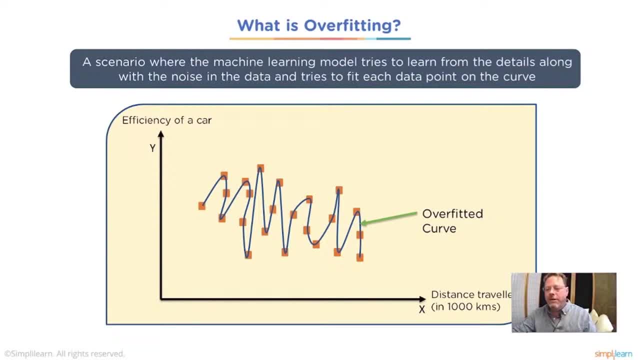 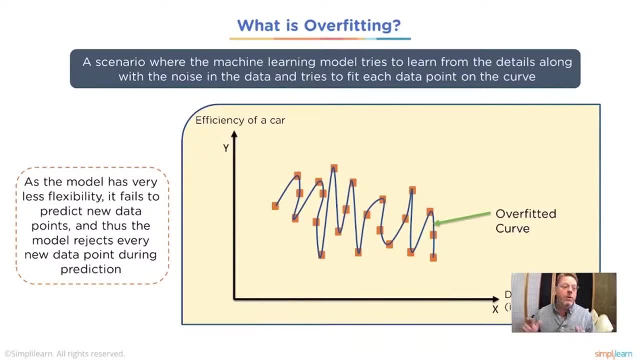 the same speed or the same car and have a slightly different efficiency. so as the model has very less flexibility, it fails to predict new data points and thus the model rejects every new data point during the prediction. so you'll get like a really high error on here. 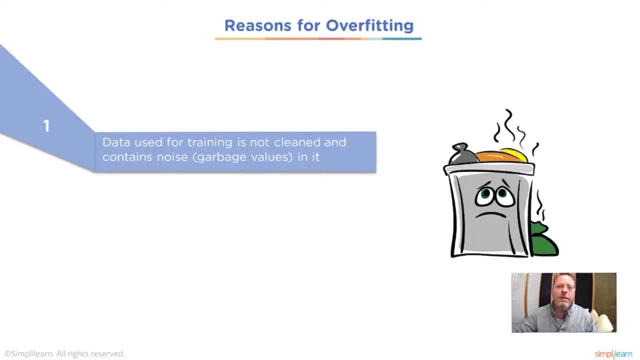 and so reasons for overfitting. data used for training is not cleaned and contains noise garbage values in it. you can spend so much time cleaning your data and it's so important. it's so important that if you have, if you have some kind of something wrong with the data coming in, 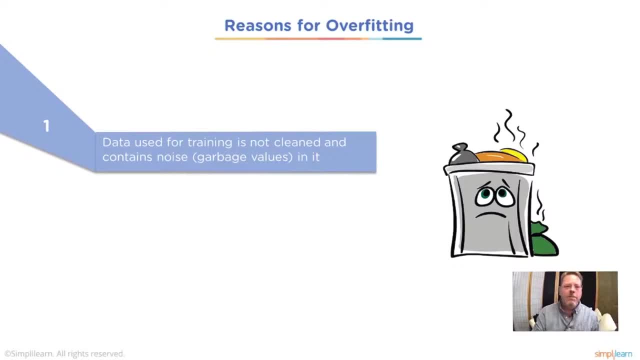 it needs to be addressed whether it's a source of the data. maybe they use in medical different measuring tools so you now have to adjust for data that came in from hospital A versus hospital B or even off of machine A and machine B. that's testing something and those numbers are coming. 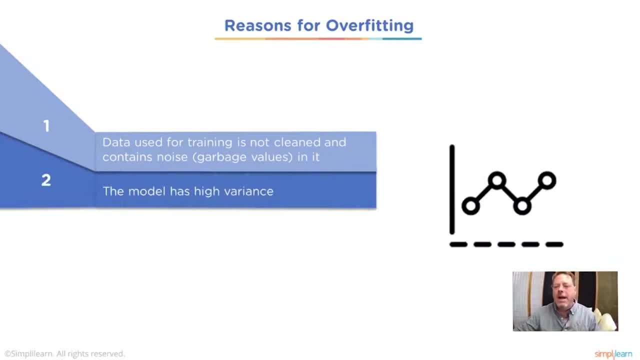 in wrong. the model has a high variance. again, wind is a good example. I was talking about that with the car. you may have a hundred tests, but because the wind's blowing, it's all over the place. size of training data used is not enough, so a small amount of data. 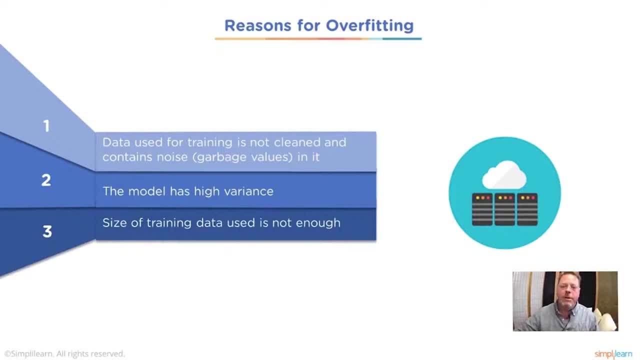 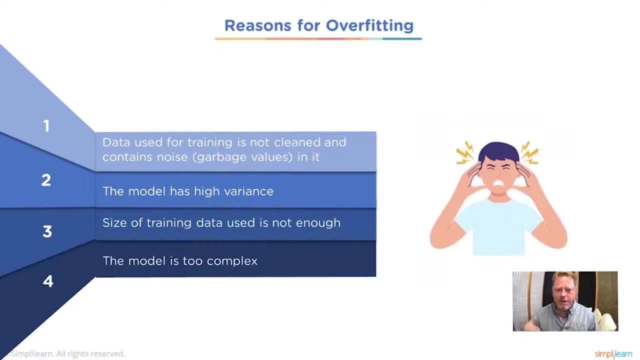 is going to also cause this problem. you only have a few points and you try to plot everything. the model is too complex. this comes up a lot. we put too many pieces together, and how they interact can't even be tracked, and so you have to go back, break it up. 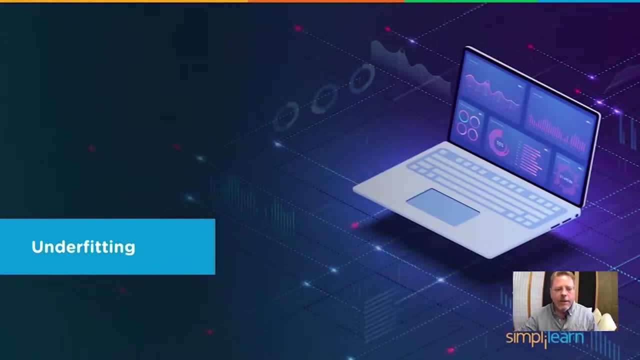 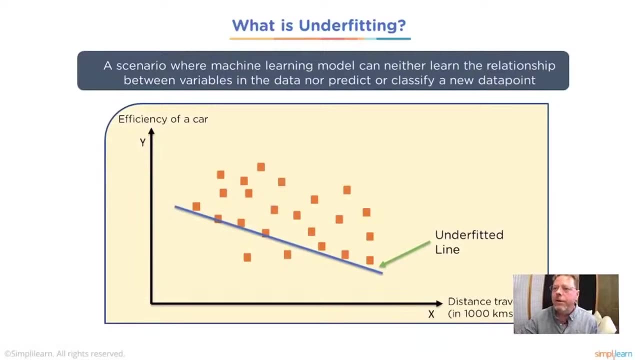 and find out actually what correlates and what doesn't. so what is underfitting a scenario where machine learning models can either learn the relationship between the data points, nor predict or classify a new data point? and you can see, here we have our efficiency of our car and our line drawn. 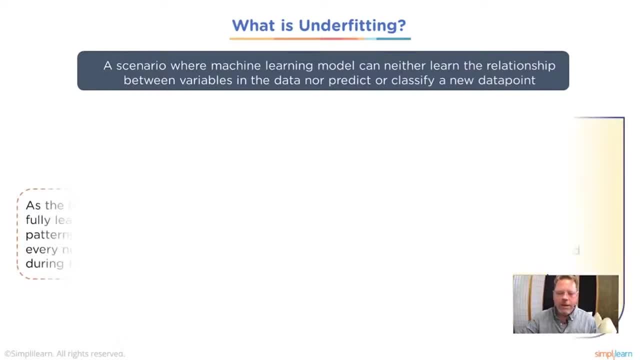 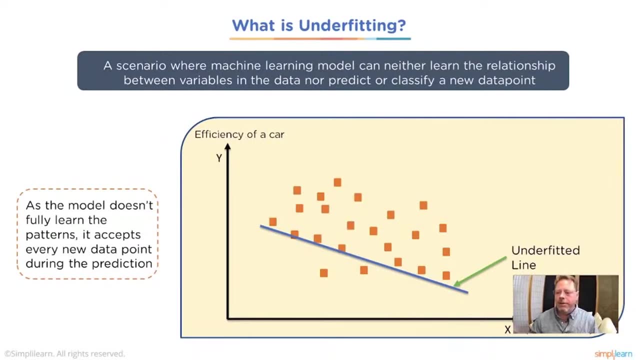 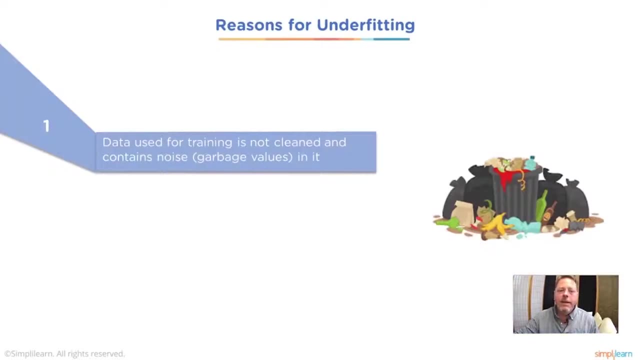 and it's just going to be way off for both the training and the predicting data, as the model doesn't fully learn the patterns. it accepts every new data point during the prediction. so instead of looking for a general pattern, we just kind of accept everything data used. 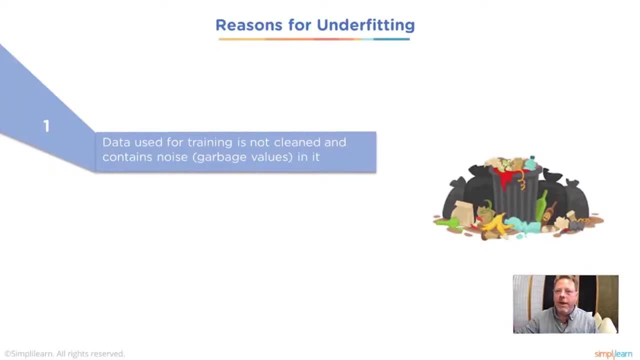 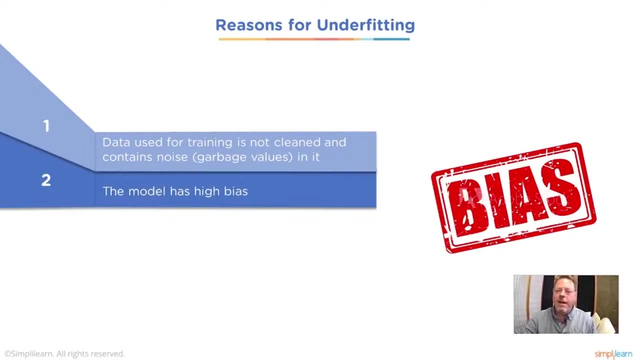 for training is not cleaned. it contains noise, garbage and values, again underfitting and overfitting. same issue. you've got to clean your data. the model has a high bias. we've seen this in all kinds of things from. the most common is the driving cars. 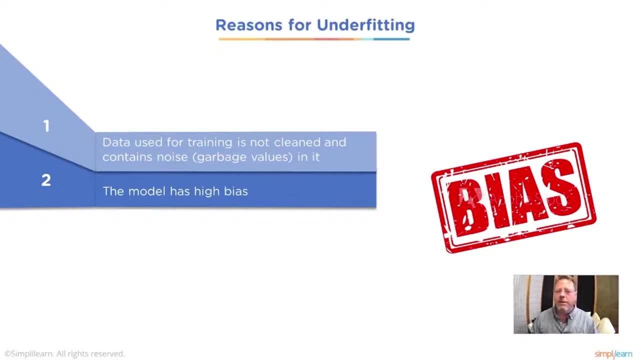 to facial identification or whatever. it is the model itself, when they build it might have a bias towards one thing, and this would be an underfitted model, would have that bias because it's averaged it out. so if you have five people from India and ten people from 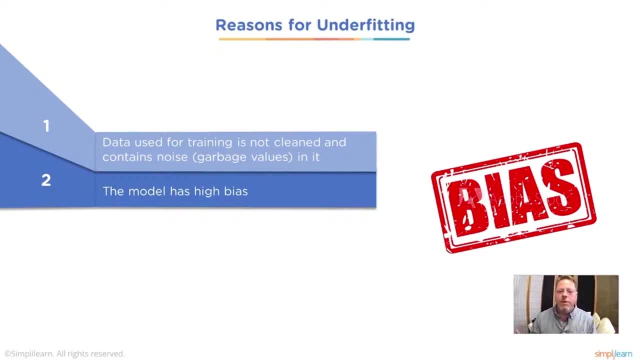 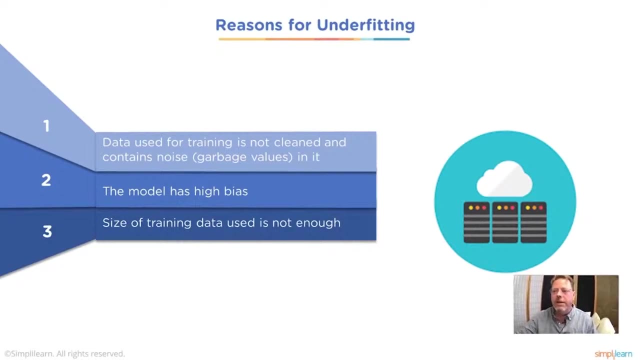 Africa and twenty people from the US. you've created a bias because it's looking at the twenty people and you only have a small amount of data to work with. size of training, data used is not enough. that goes with the size I was just talking about, so we have a model with a high bias. 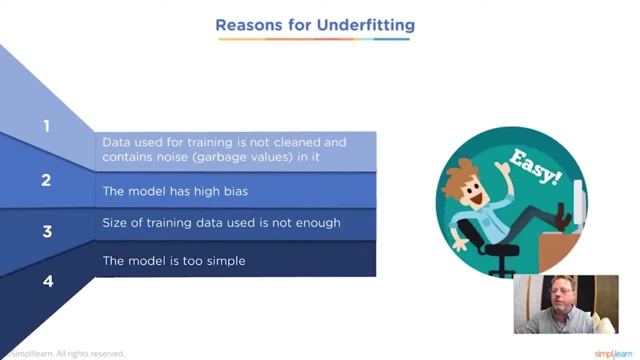 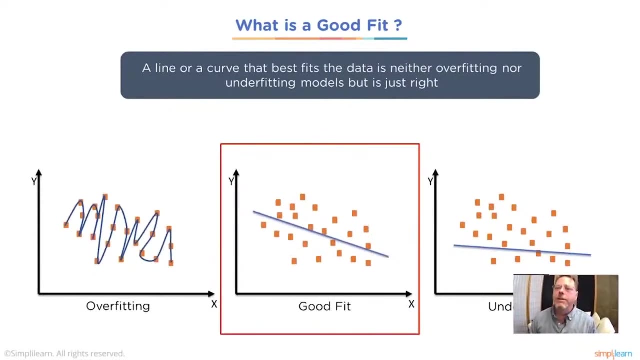 we have size of training. data used is not enough. the model is too simple. again, this is one straight line through all the data when it has a slight shift to it for other reasons. so what is a good fit? a linear curve that best fits the data is neither overfitting or underfitting. 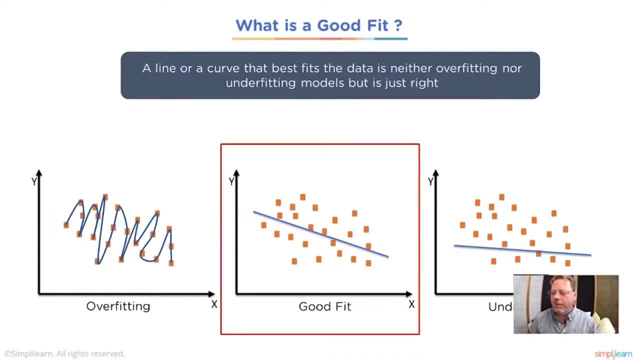 models. but is just right. and of course we have the nice examples here where we have overfitting lines going up and down. every point is trying to be included. underfitting the line really is off from where the data is and a good fit is minimize that. 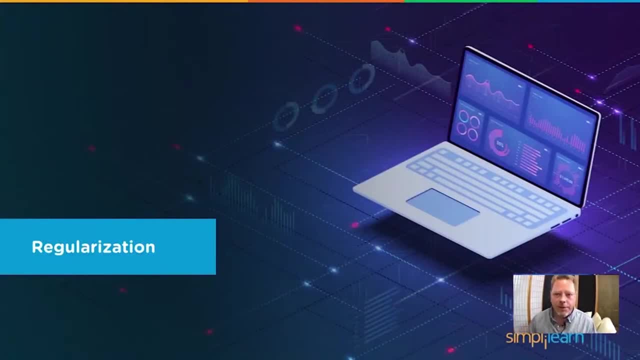 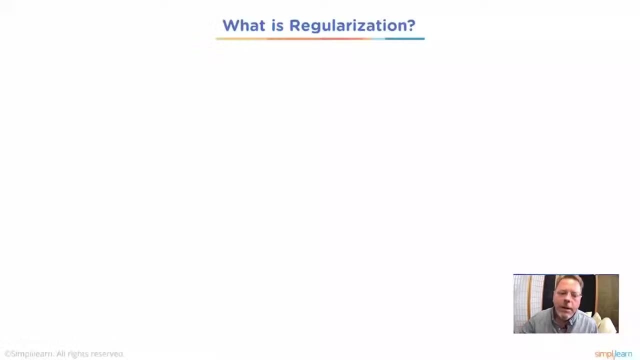 error coming through. regularization is taking the guesswork out. you're looking at this graph and you're going: oh, which one? is that really overfit or is that underfit? that's pretty hard to tell. so we talk about regularization. regularization techniques are used to calibrate. 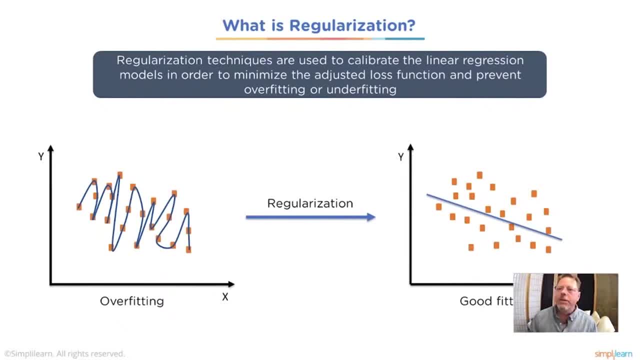 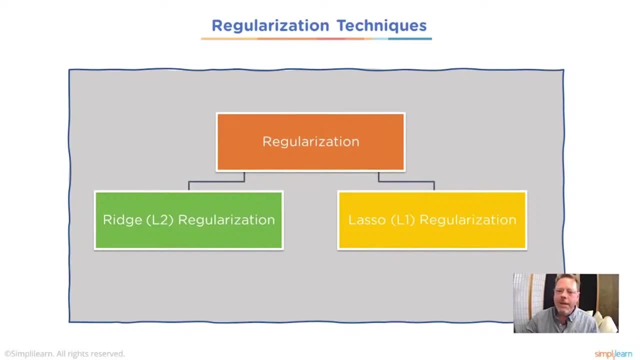 the linear regression models and to minimize the adjusted loss function and prevent overfitting or underfitting. so what that means in this case, we're going to go ahead and take a look at a couple different things. we're going to look at regularization, which we'll start with a linear model. 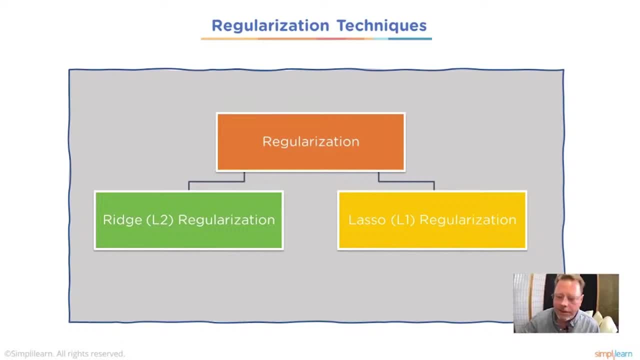 we'll look at the ridge regularization and the lasso regularization and these models are just like- just like we did the MLP, the multi-layered positron in the sklearn module. you could bring in the ridge module and you can bring in the lasso module. so 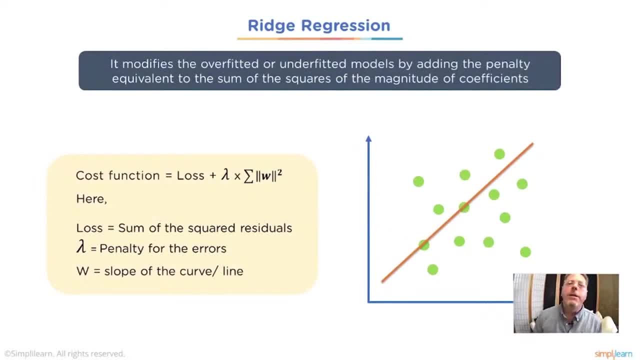 when we talk about ridge regression, it modifies the overfitted or underfitted model by adding the penalty equivalent to the sum of the squares or the magnitude of the coefficients, and so we have a cost function equals loss, equals lambda times the sum of w squared or the absolute value of w. 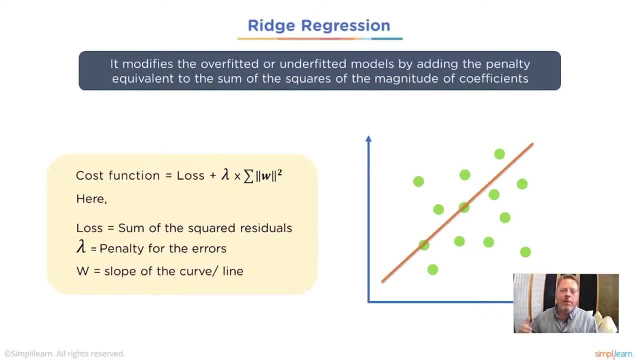 depending on how you're doing it. now, remember we talked about error, where we either square it or we absolute value it, because that removes the plus or minus sign on there and there's reasons to do it either way. but it is more common to square the value. 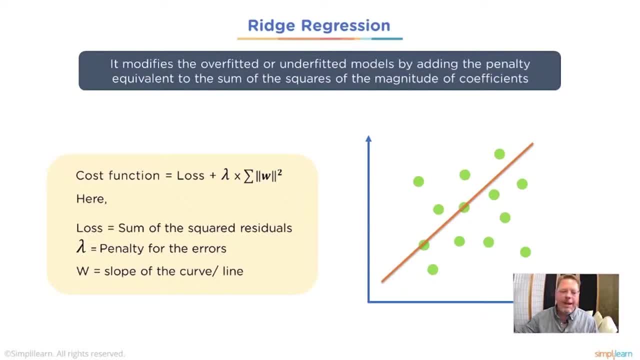 and then we have our. in this case, the lambda is going to be the penalty for the errors. we've thrown in a Greek character for you just to confuse everybody, and w is the slope of the curve of the line. so we're going to look at this and we're going to draw a line. 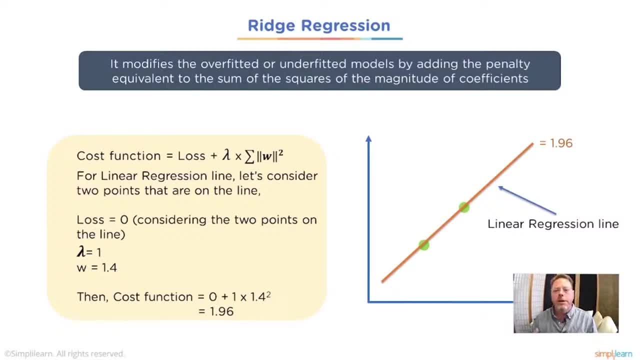 this is going to be like a linear regression model. so if you had in sklearn you could import just a standard linear regression model. it would plot this line across. whatever data we're working on and we look at this and of course we're just extrapolating this. I know they use some specific 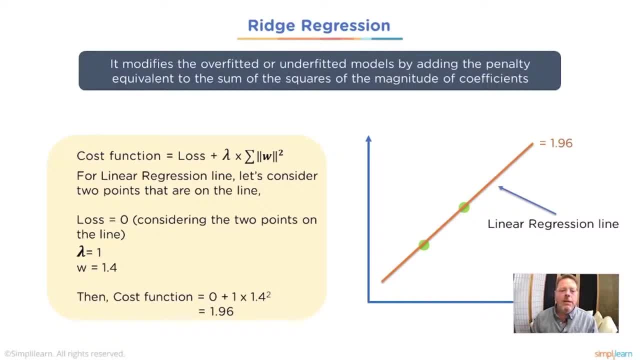 data but don't want to get into the actual domain, and so for a linear regression line. let's consider two points that are on the line, and we'll go ahead and have a loss equals zero. considering the two points on the line, we'll go ahead and do lambda equals. 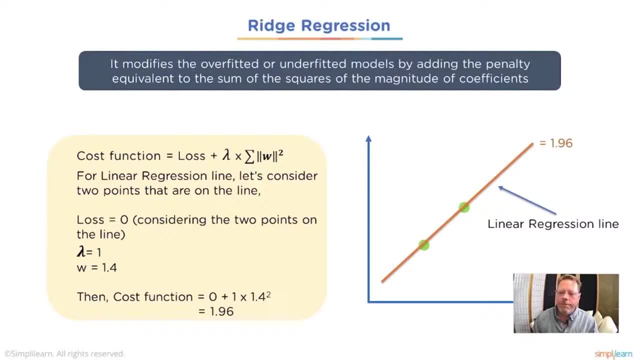 one. we'll set our w is going to be one point four, then the cost function equals zero plus one times one point four squared, which equals one point nine six. so really don't get caught up too much in the math on this, other than understanding that this is something that's. 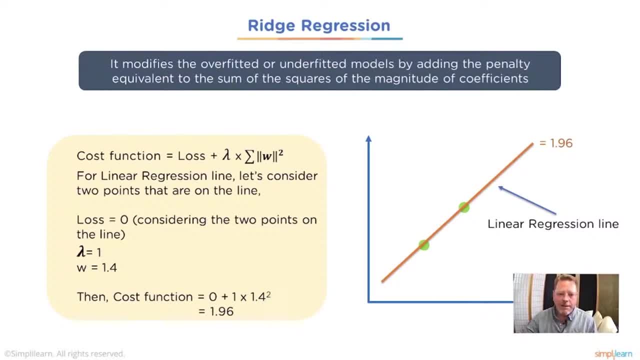 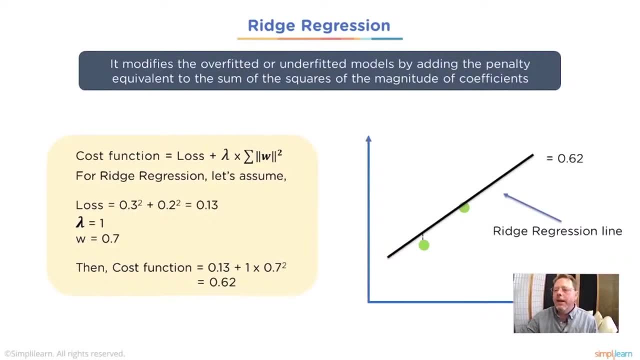 very easy for a computer to calculate and if you ever see the loss plus the lambda times the sum of w squared. and then let's say we have a ridge regression line and it does this, we go ahead and plot it and we do the calculations on the data. 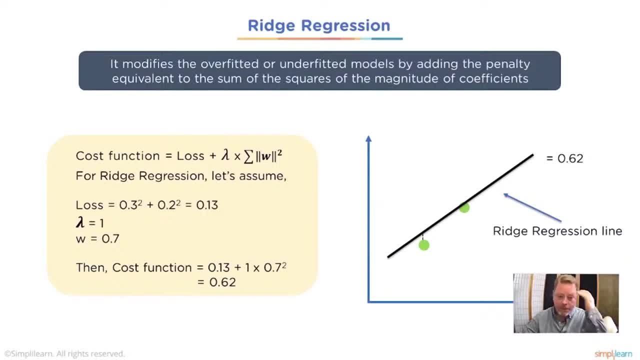 and for the ridge regression, let's assume a loss equals point three squared plus point two squared equals point one, three, and we put all the calculations through of the two points, we end up with point six, two. so we now had a linear regression model, we now had a ridge regression. 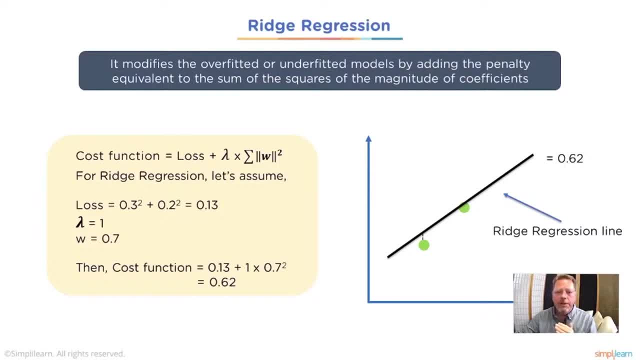 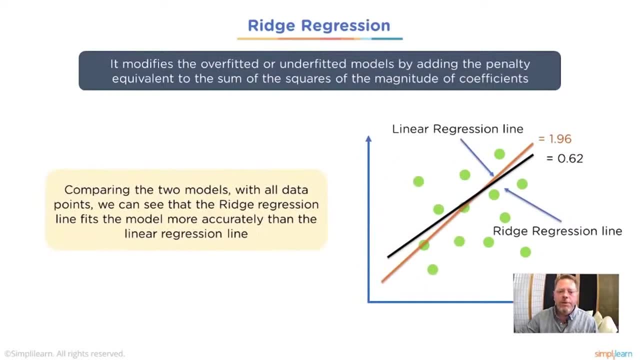 model and the ridge regression model plots a little differently than the standard linear regression model and comparing the two models with all the data points, we can see that the ridge regression line fits the model more accurately than the linear regression line, and I find this true on a lot. 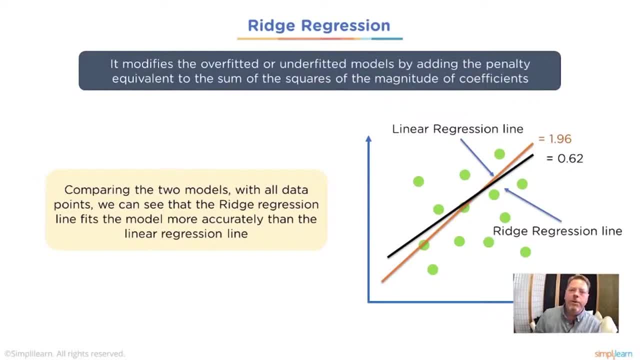 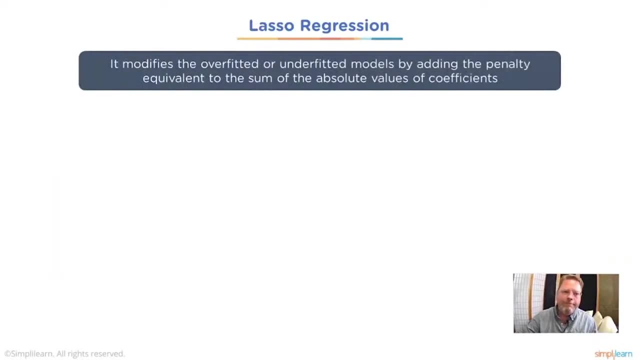 of data I work with, I'll end up using either the ridge regression model or the lasso mars regression model for fitting, especially dealing with a lot of like stock markets daily setup. they come out slightly better, you get a slightly better fit and so we have our lasso we just talked about. 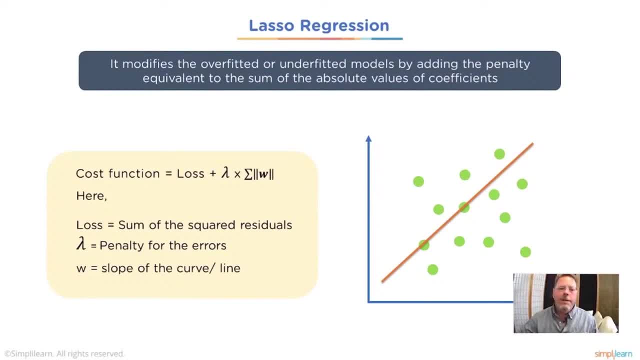 lasso coming in here and the cost function equals. instead of doing squared, we're just going to do the absolute value, and so, if you remember, this is where ridge regression changes. where's my ridge regression model? we're squaring the value here and if you look at this, we're not squaring. 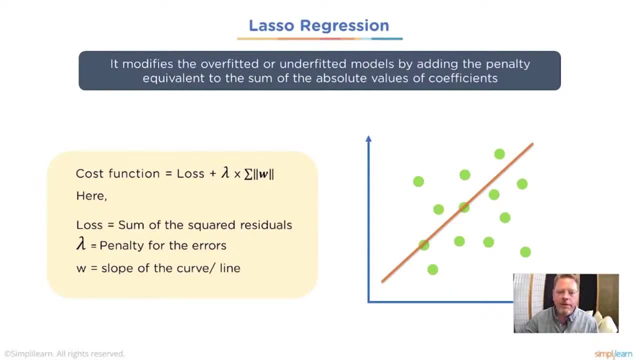 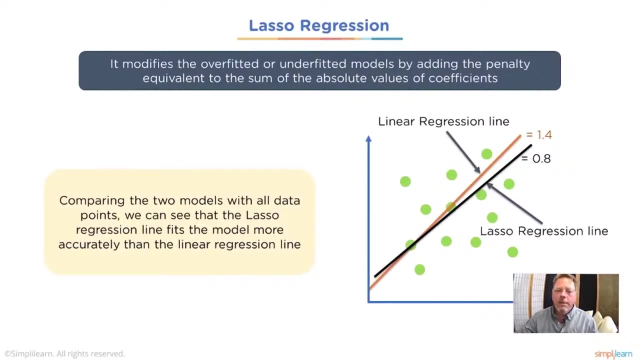 the value, we're just finding the absolute value on here, and so the lasso of the squared individuals- and here is our lambda symbol again: penalty for errors- and w equals the slope of the curve, and comparing the two models with all the data points, we can see that the lasso regression line fits the. 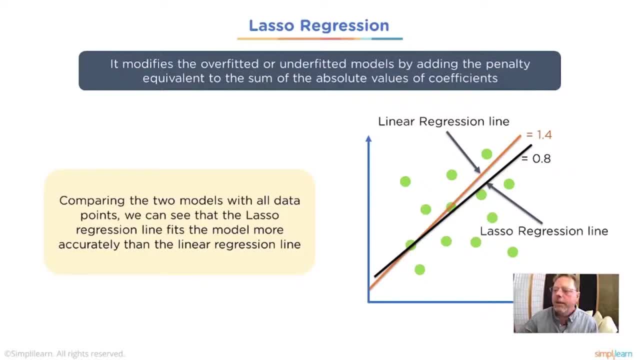 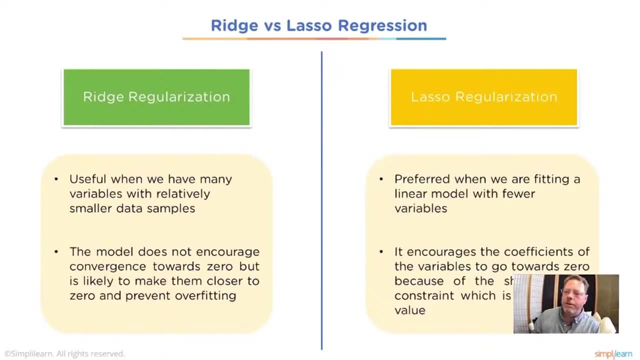 model more accurately than the linear regression line, and this is like I said. I use these two models a lot: the ridge, and this is important. this is kind of the meat of the matter. how do you know which one to use some of it is? you just do it a bunch of times and then you figure it out. 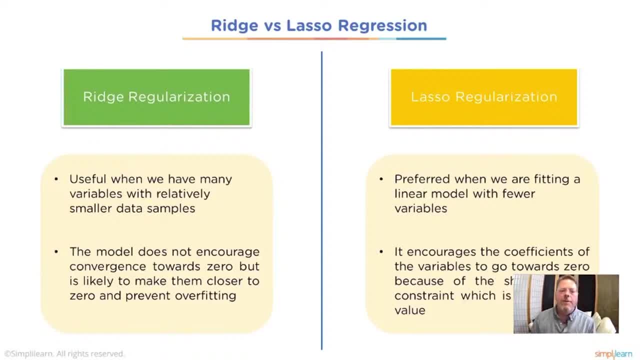 ridge is useful when we have many variables with relatively smaller data samples. the model does not encourage convergence towards zero, but is likely to make them closer to zero and prevent overfitting. the lasso regularization model is preferred when we are fitting a linear model with fewer variables. 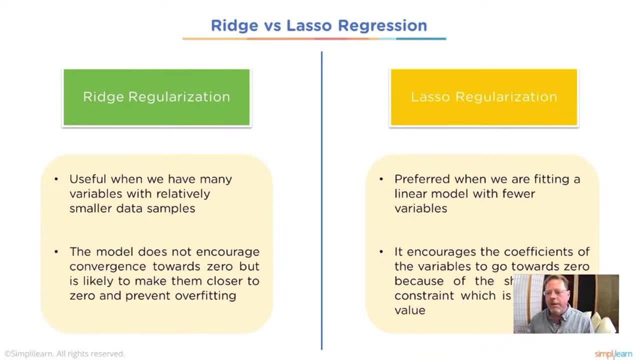 so in the iris thing we had four or five variables as we measured the different leaf pieces. you might be doing the measurements on the cancer project, which has thirty six different variables. so as we get down to the iris with four variables, lasso lar will probably work pretty good where you might use the ridge. 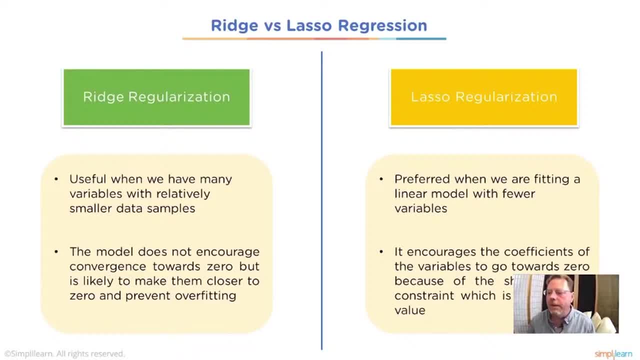 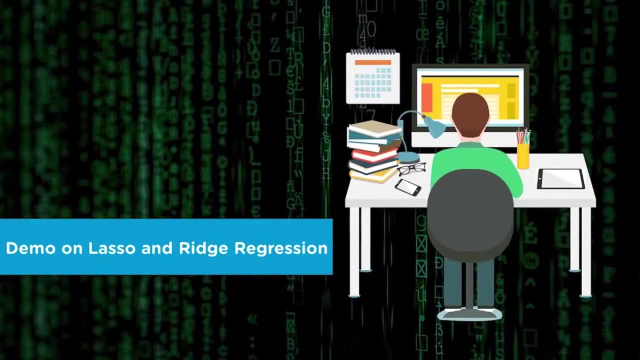 regularization, with more models, if you have something significantly larger, and it encourages the coefficients of the variables to go towards zero because of the shape of the constraint, which is an absolute value. and with any of this, we want to go ahead and do a demo in lasso. 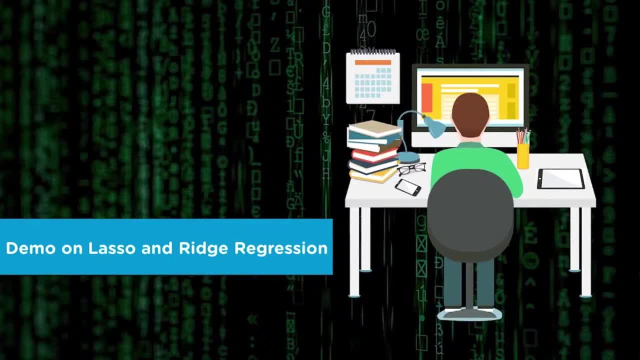 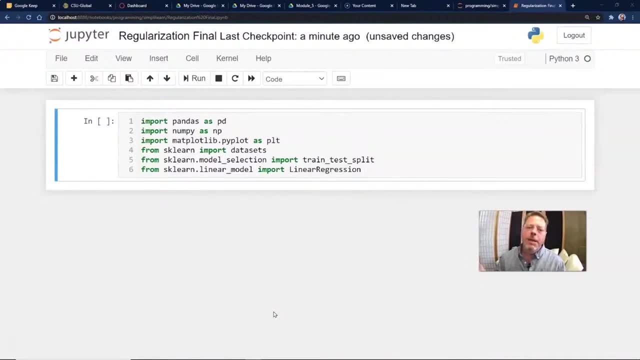 and ridge regression. so let's take a look and see what that looks like in our code and bring up our Jupyter notebook. we'll start with our imports: pandas as pd, import numpy as np. import matplotlib as plt. sklearn: we're going to import our data sets. 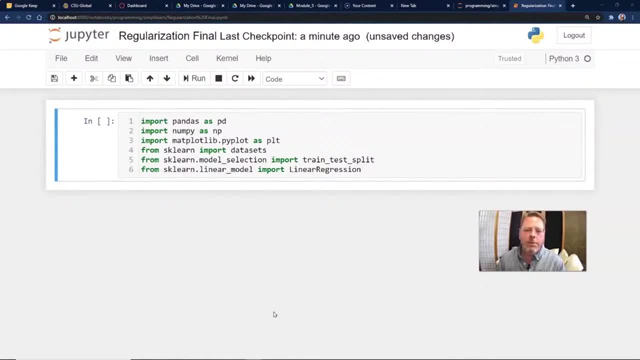 it's kind of more generic. we usually just import one data set instead of all of them. but you know quick and dirty when you're putting some of these together. we have our sklearn model selection. we're going to import our train test split for splitting our data up, and then we'll 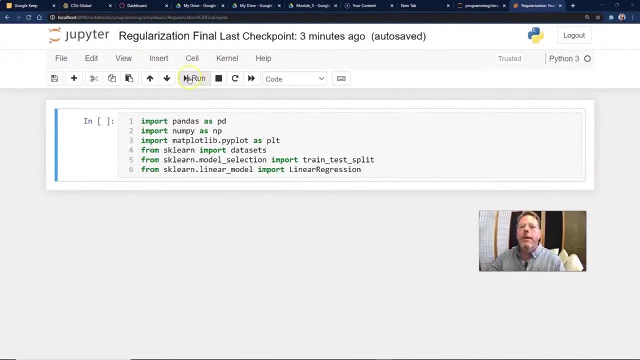 bring in our linear regression model and we'll go ahead and run these just to load them up and then load our data set. we were just talking about that. you could just have imported the load boston data set in there instead of loading all the data sets. 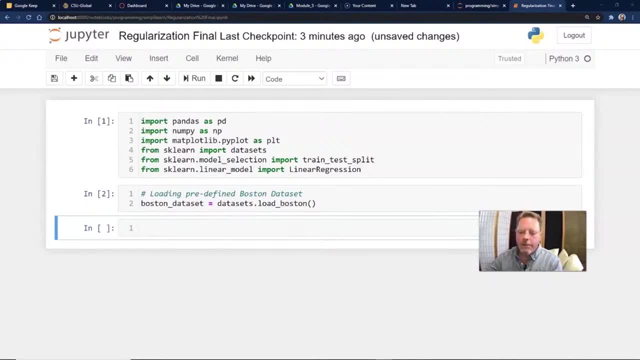 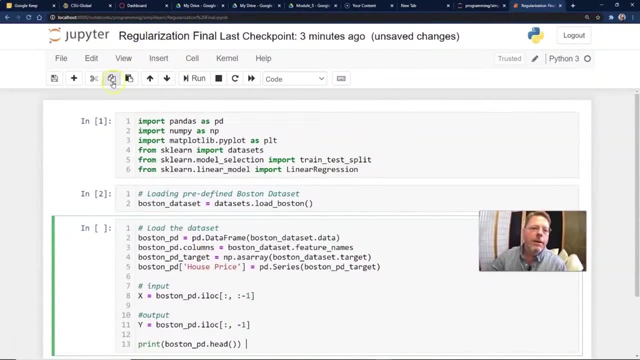 and then, once we've loaded our data set, we want to go ahead and take a look at that data and see what we've got here. let me just go ahead and pop that down there and go ahead and run it, and so we've gone ahead and taken our 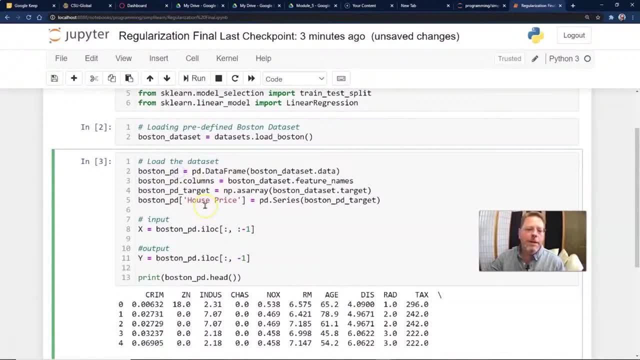 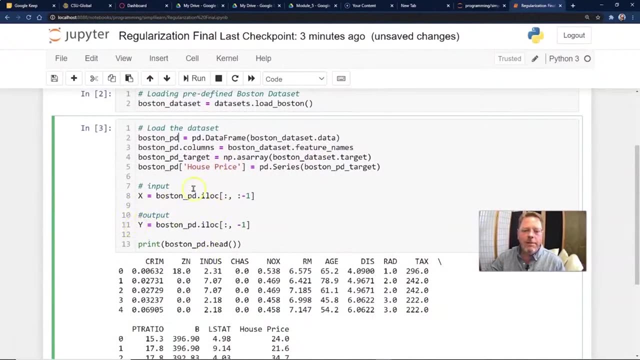 boston data we're going to. we've put it into our pandas data frame, the boston data set and then the boston columns, so we want to see what's going on with them. we have our target, we have the house price, etc. and so our x equals boston. 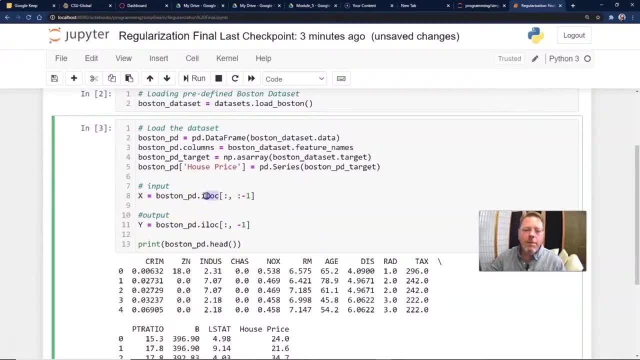 i location. now remember in pandas the new updates to pandas. they want i location if you're going to pull data. we used to be able to leave this off, but it does something different. it creates a slice versus a direct setup, so make sure you're using that i location. 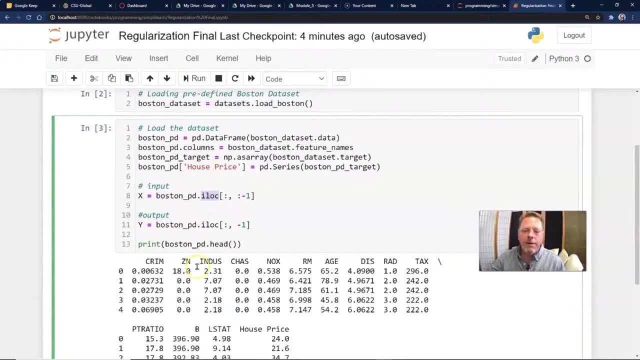 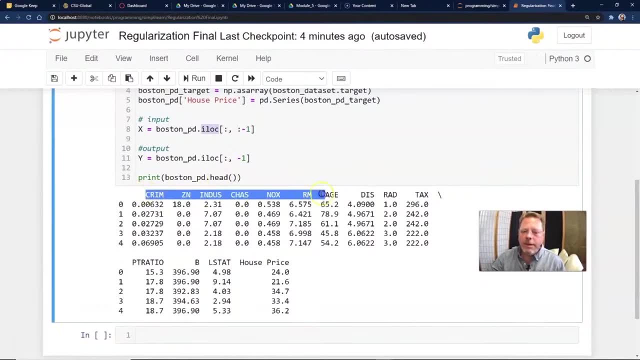 and the i the output. so this is all just bringing our data together and we can see here, if we do, we print the boston pandas head. we can see here all of our different aspects we're looking for and if you're following the x and the y, 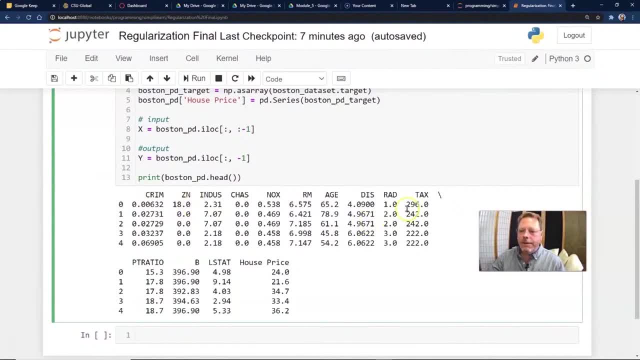 the x is everything except for the last column, where y is all the. that's what this means: all the rows except for the last column. and then y is all the rows but just the last column. so y is our house price and the x is the crim zn industry chas. 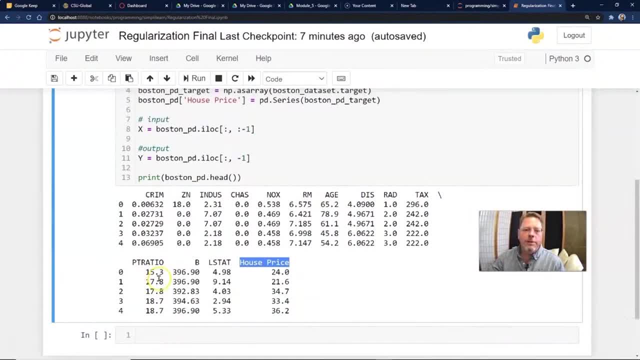 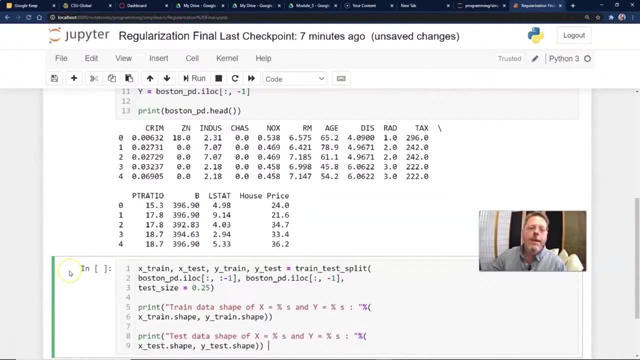 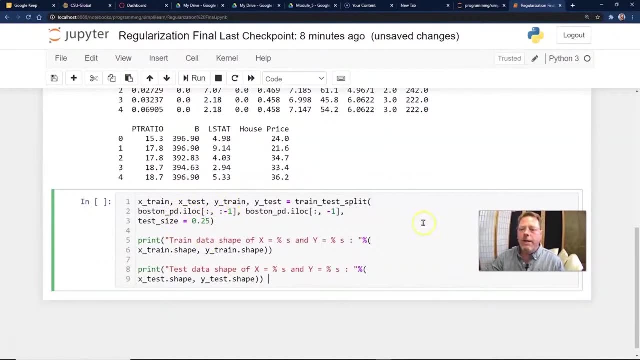 knox and all these other different statistics they've collected for house sales in boston. there we go. whoops, control, ah, so we'll go ahead and split our data- x train and our x test, y train. y test equals the train test split which we imported. 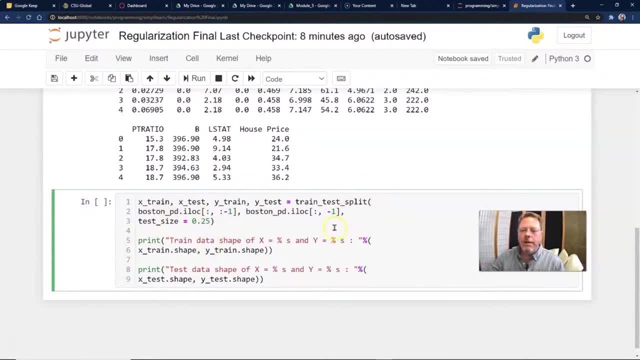 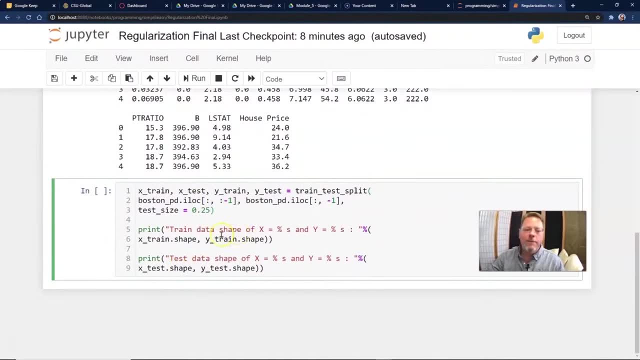 and we have our boston. you could have easily used the x and y on here as opposed to boston i location, and we'll create our test size. we're going to take 25% of the data and put it in as a test and then 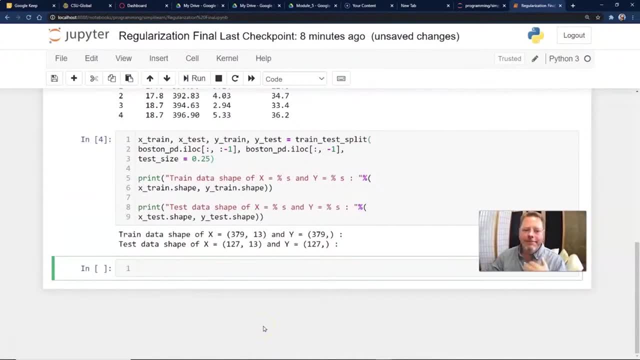 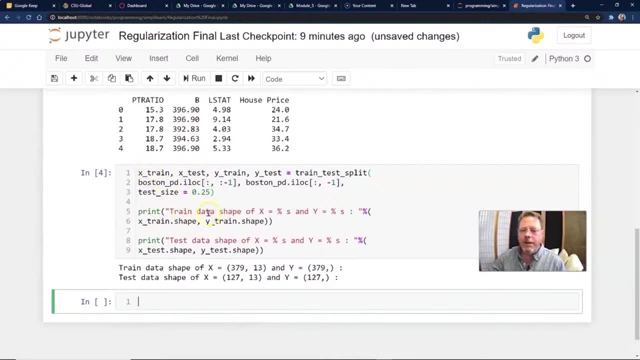 we'll go ahead and run this need an extra drink there. so we have our train and test. and then, of course, the print: the train data shape. i love doing this kind of thing whenever i'm working with this data: print out the shape, make sure everything looks correct. 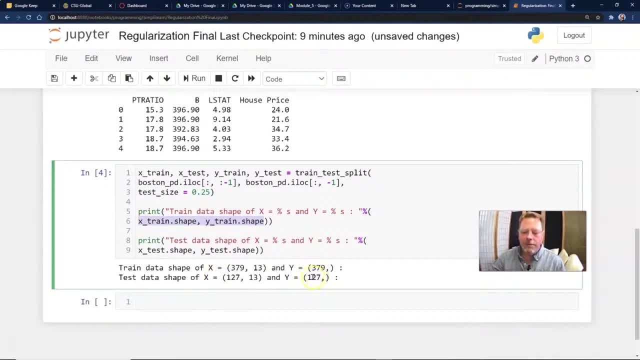 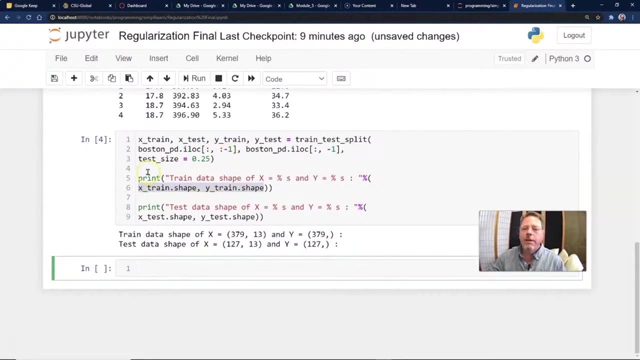 so that we have 127 by 13 and 127 by 1, 379 by 13. they should match and if the data sets are not quite matching, then you know something's wrong and you're going to get all those errors. i'm going to run through here. 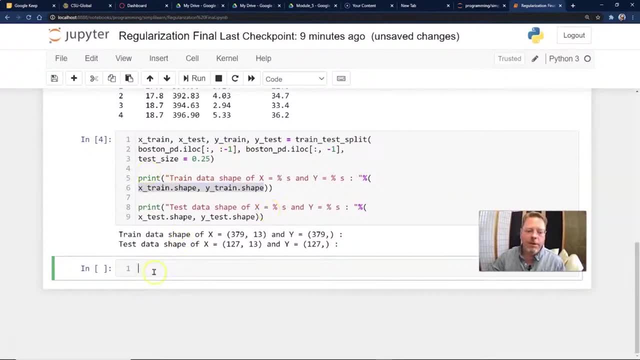 and it's dropped a row on one of them and not on the other, or something weird has happened when i'm cleaning the data. this is pretty straight forward and simple because the data comes in a nice prepacket and is all clean for you, so let's go ahead and apply. 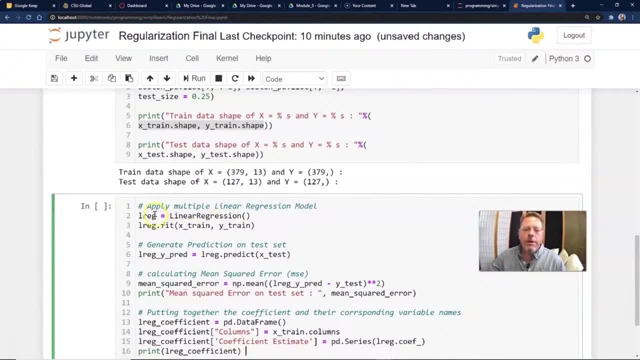 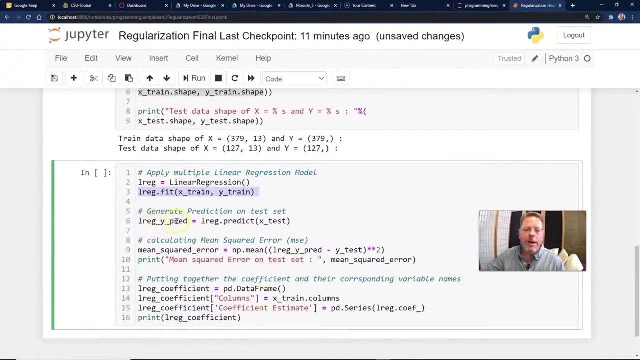 the multiple linear regression model and we'll call this lreg linear regression and we're going to go ahead and fit that linear regression model to the test set. then we'll generate the prediction on the test set. so here's our lreg predict with our xtest going into the prediction. 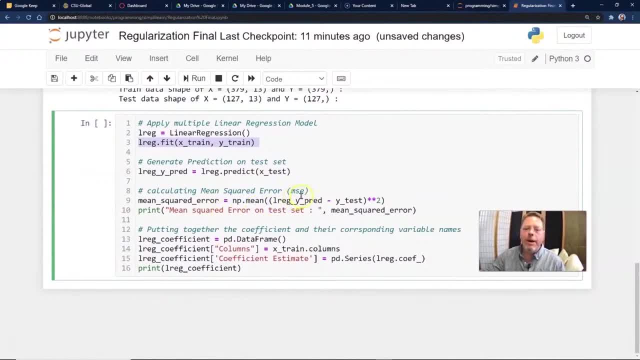 and let's calculate that mean square error, mse. i told you, you'll see, mse used a lot. people use it in variables and things like that. it's pretty common and we get our mean squared error equals. this is just the basic formula we've already been talking about. 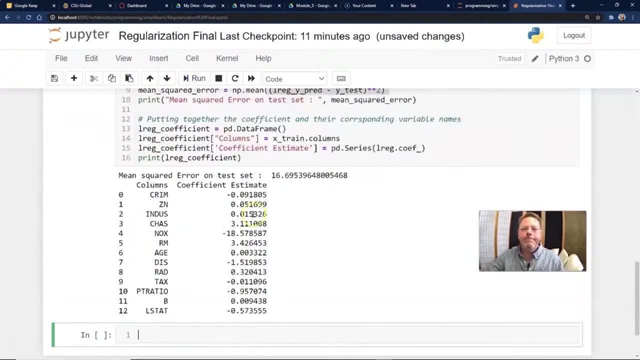 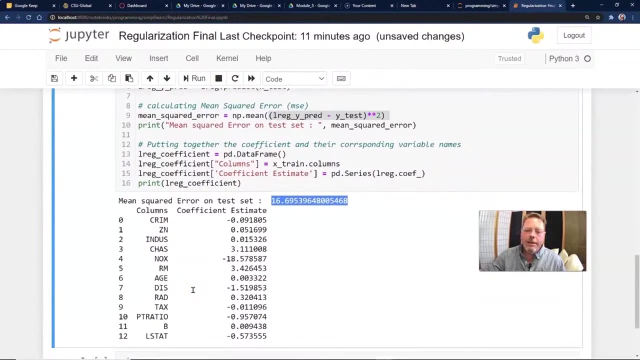 the average of that and we'll go ahead and just run this and you can see when we get through the end of this. we have our mean square error on test, we have our total and then we have each column coming down and at this point, unless you really know the data, 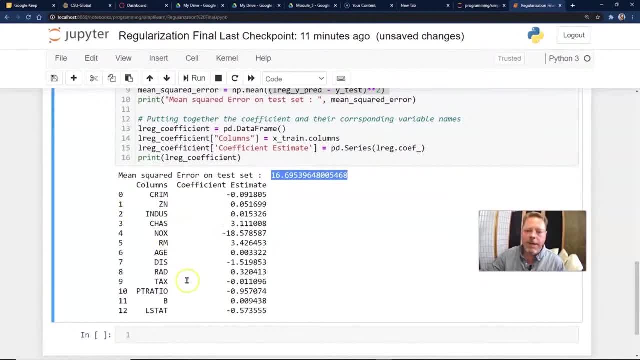 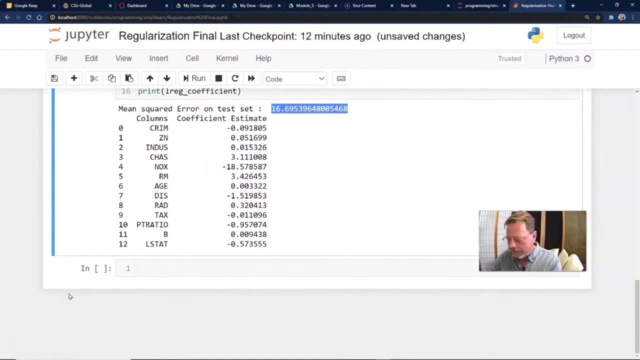 you're working with, it's not going to mean a whole lot. so if it's in your domain, you might know what you're looking at when you see these kinds of numbers coming up. and that's okay, at least that's okay for this demo. and then we're going to go ahead and plot these. 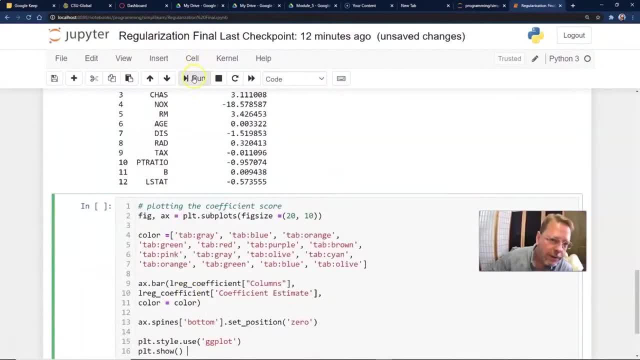 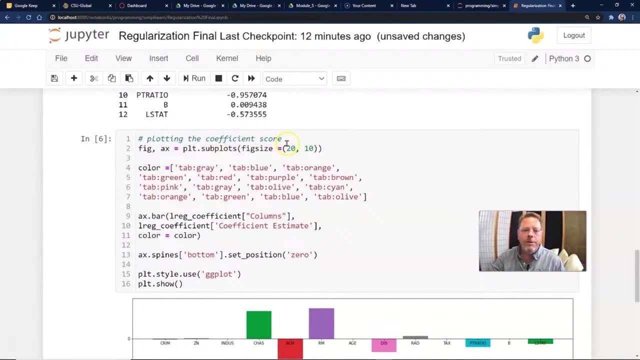 so we can see what's going on, and this is always kind of fun. it's always nice to have a nice visual of what you're looking at and you can see here when we plot the coefficient scores on here, and we, the guys in the back, did a great job. 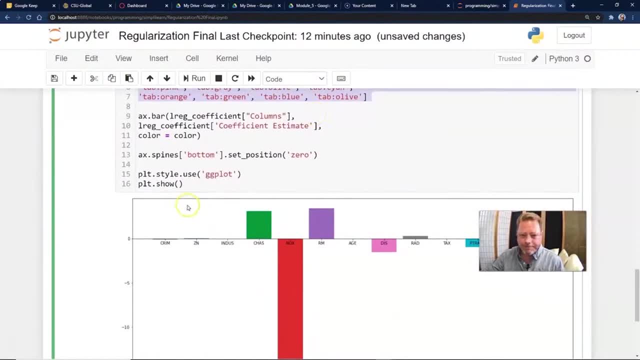 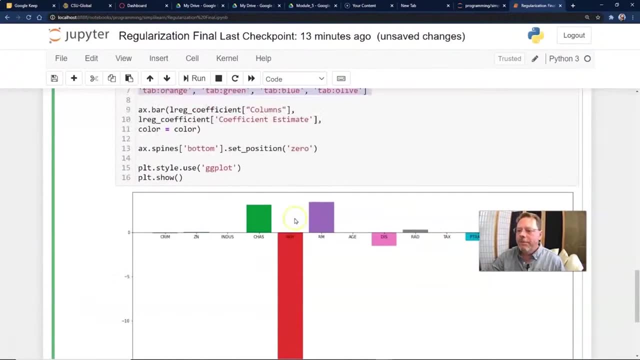 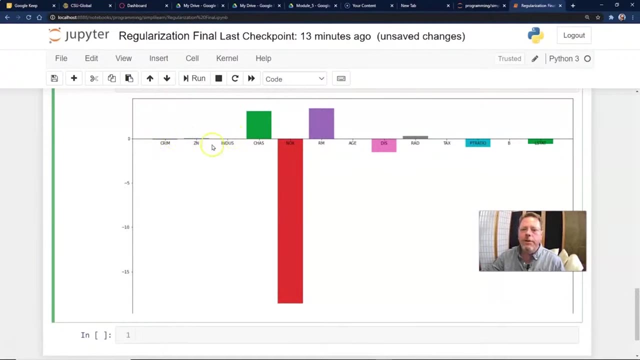 putting some pretty colors together, making it look nice and setting up the columns. you can see here this is a huge coefficient. when I look at a table like this, I look for what has very little different coefficients- they're not using a huge change- and what has huge changes. 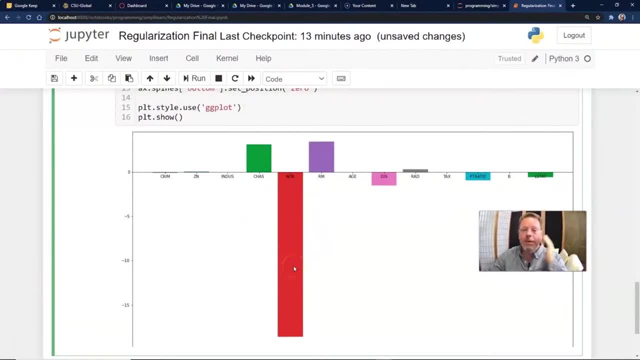 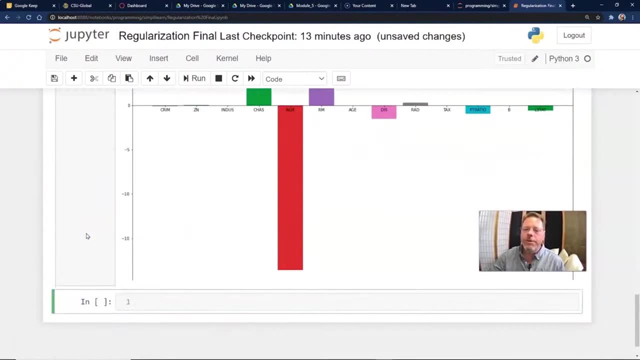 and that flags you for all kinds of things as you're working with the data, but it depends so much on the domain you're working with. these are great things, though, as just a quick look to see what's going on with your data and what you're looking for. 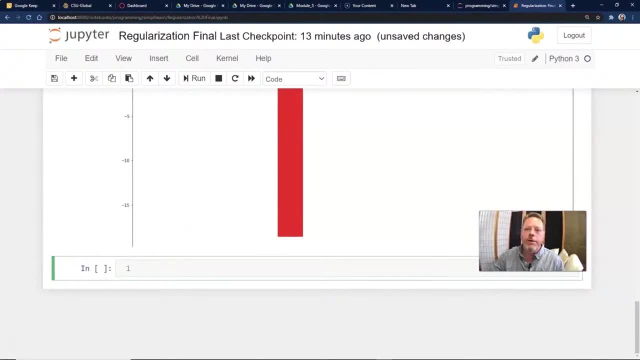 and, of course, once we look at this now, our motive is to reduce the regression score. so now we want to take these and bring them down as much as we can, and for that we're going to work with the ridge regression on here. so let's start by going. 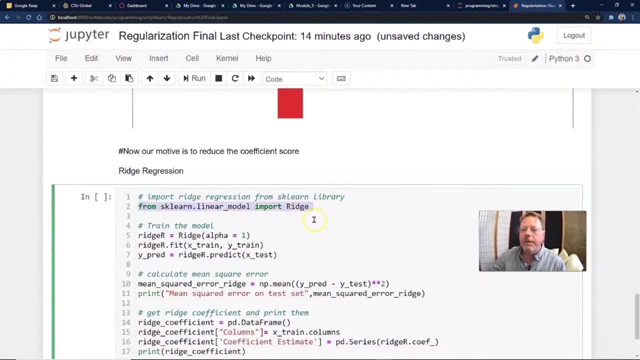 and we're going to import our ridge model, the ridge regression, from the sklearn library or the scikit and we're going to go ahead and train the model. so here's our ridge: r equals alpha equals one, and I mentioned that earlier when I work with the ridge model. 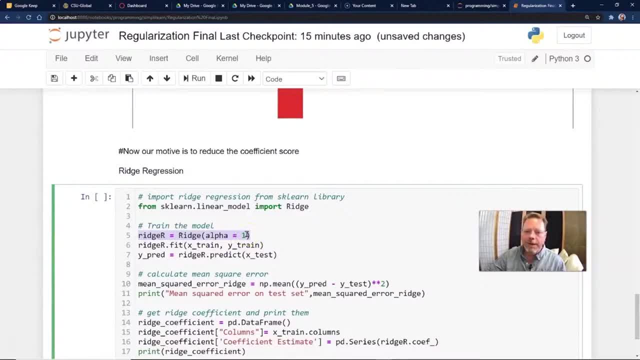 you'll see alpha equals one if you set alpha equal to zero. that's a standard linear regression model. so you have alpha equals one, two, three, four and you usually use one, two, three, four and a standard integer on there and we'll go ahead and fit the ridge model. 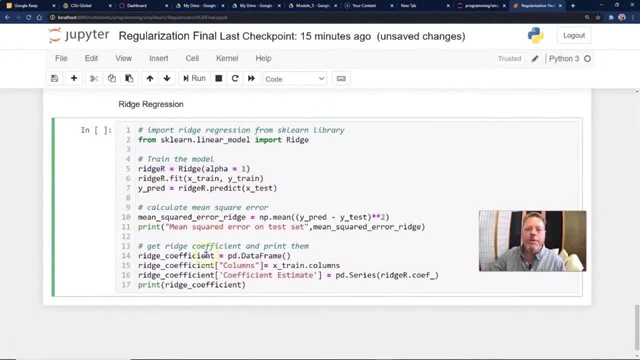 on there with our x train and our y train. data generate a prediction for that, for our x test, and we'll calculate the mean square error just like we did before. this should all look familiar and we'll go ahead and print that out and we'll look at the. 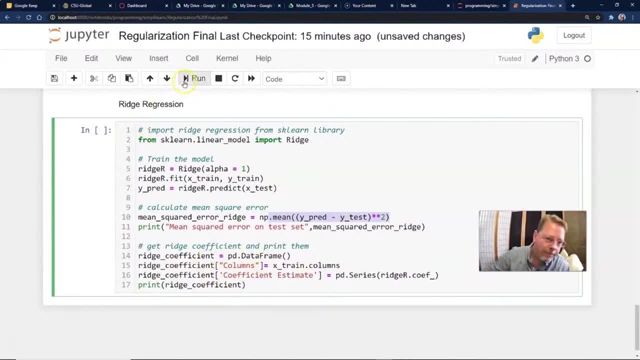 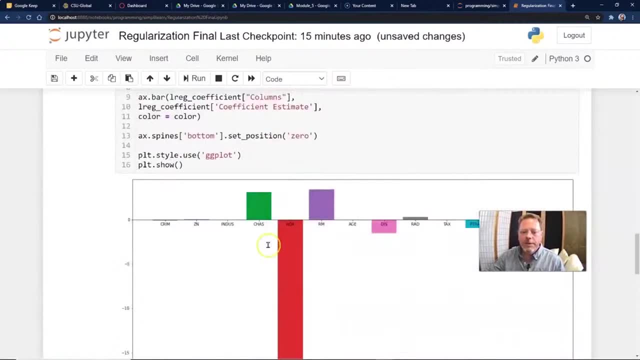 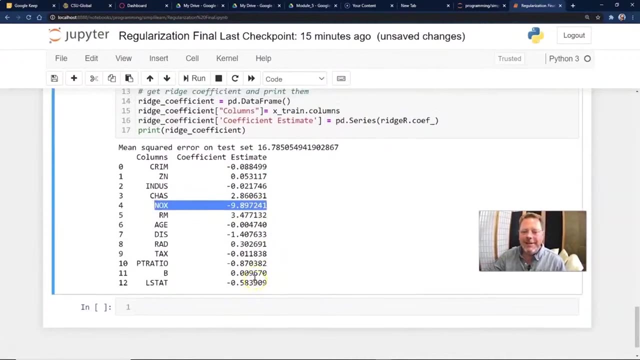 ridge coefficients for our data and see what that looks like now. if I jump up and down between these two, you'll get a headache. you'll still see the nox value. let's just look at the nox, because that was the biggest value. it's a minus nine here. 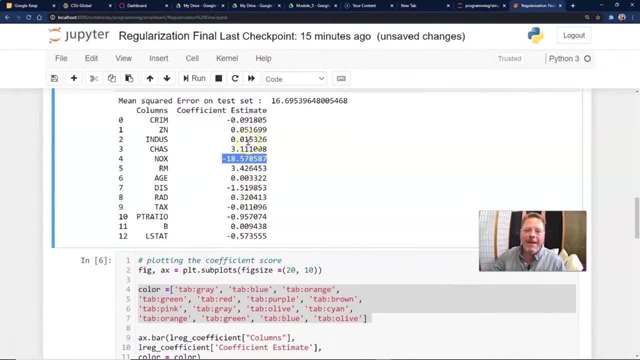 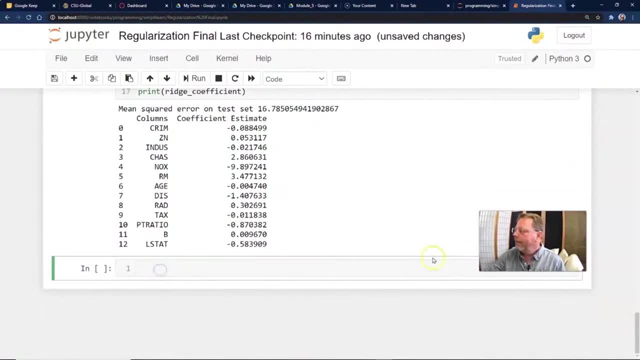 and if we go back up here, the nox value is a minus eighteen. so right off the bat I'm seeing a huge change in the coefficient there. so if we're going to do that nice set up, we want to go ahead and just print it and see what that looks like. 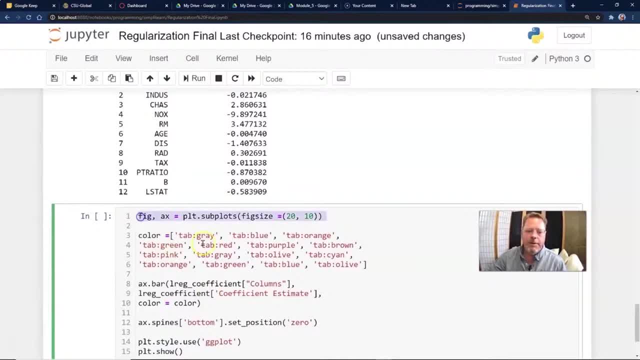 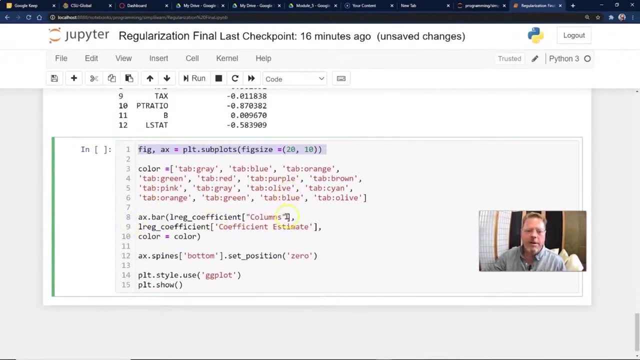 here we go and we've set up our plots, subplots, and again the team put together some nice colors so it makes it look good. and we're doing an x bar based on the columns and our l regress coefficients. color equals color x, spine bottom and so forth. 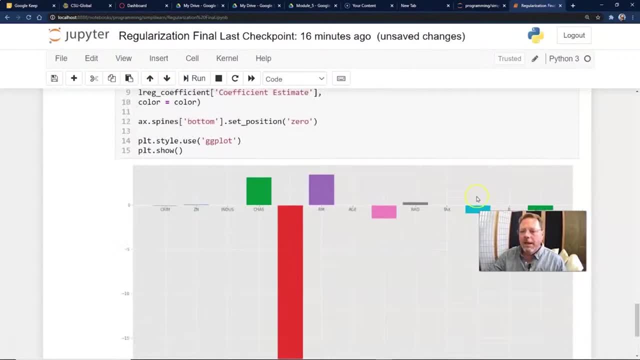 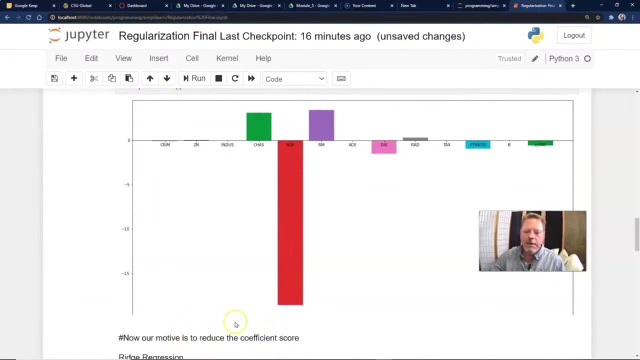 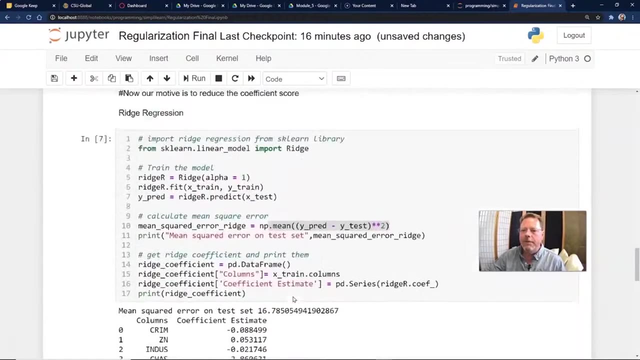 so it just puts together a nice little graph and you're starting to see, when you compare this, if you put it on the same graph as this one up here, this is up here at minus eighteen, this is at minus nine, and so this graph is half the size of the graph above. 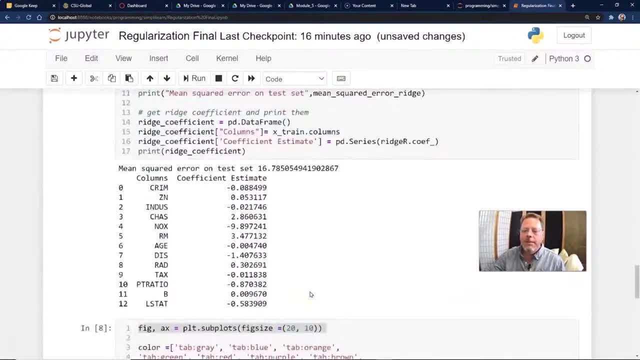 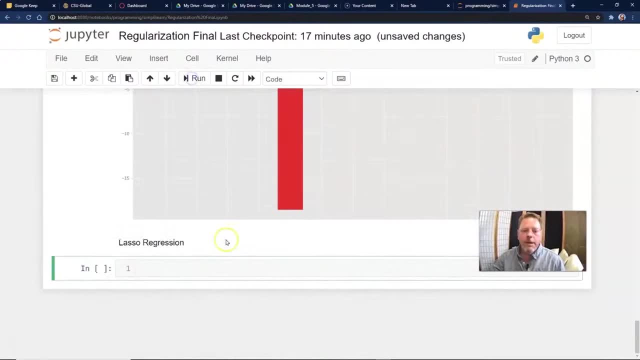 the same thing with these values here. they might look the same, but they're actually all almost half the value on here. and then, finally, you can do the same thing for the lasso regression. this will all look very similar as far as what we worked on before. 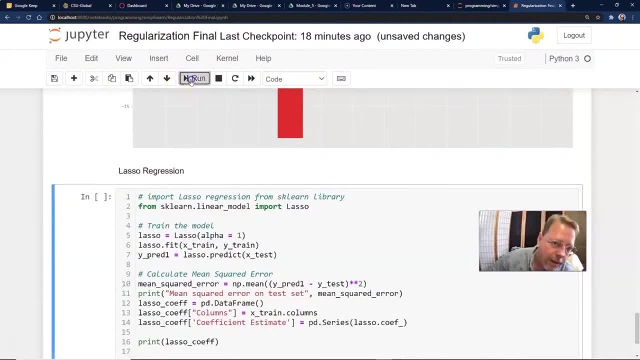 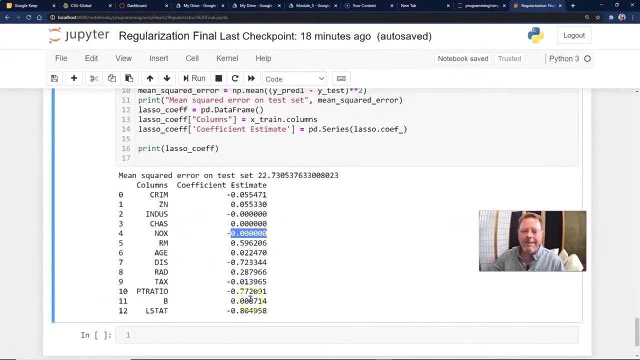 and I'm just going to go ahead and print that on here and run it. and again, let's go up to NOX. look where NOX is. it's all the way down to zero and if we look at our next biggest coefficient, it's minus .8. 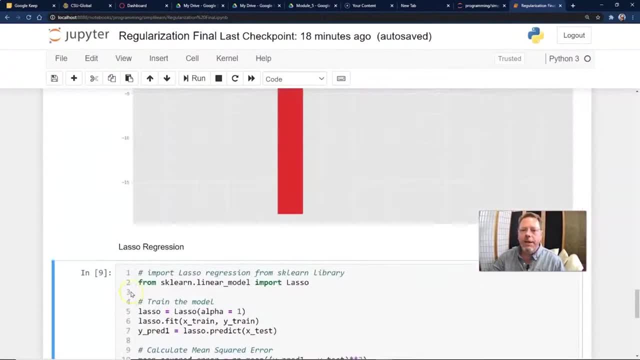 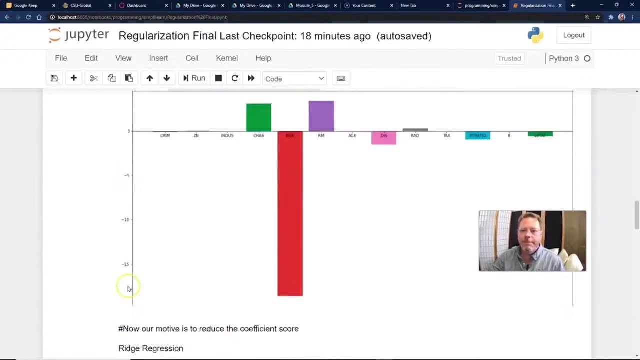 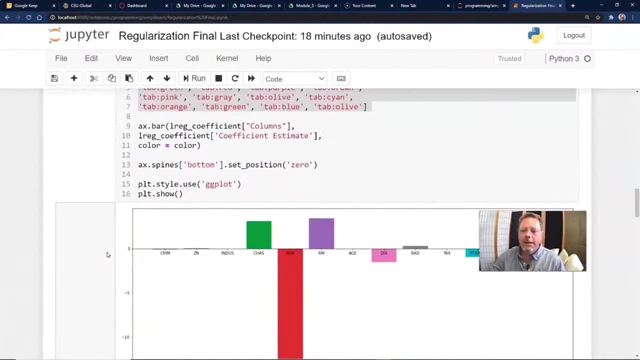 and really here's our 22.73. we go up here 16.7, and we go up here and we look at the same number, 16.69, and so we look at this. if I was running this and working on a project with this,